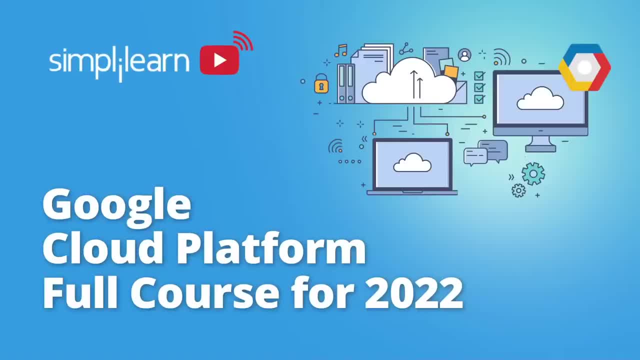 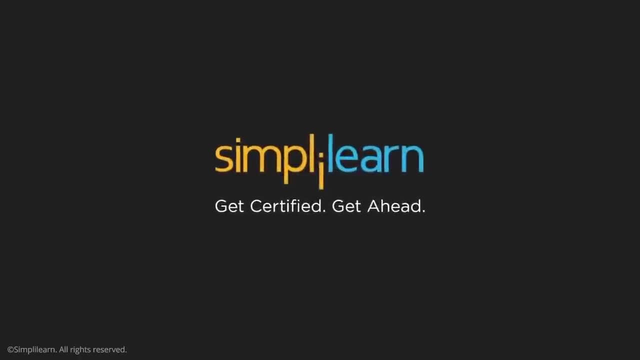 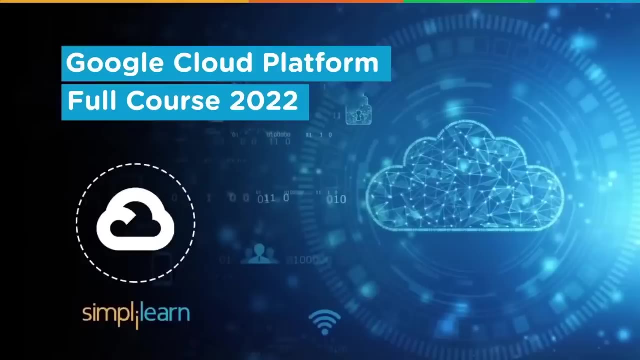 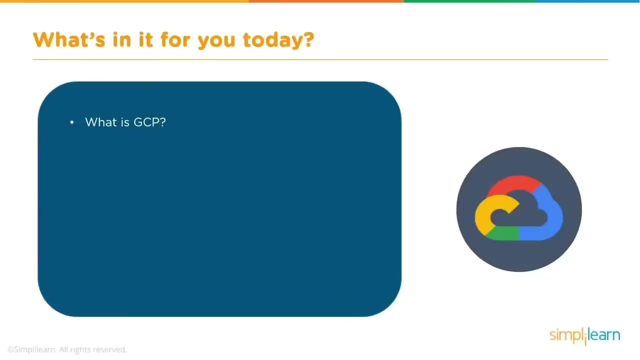 Hello everyone, welcome to this interesting video on Google Cloud Platform full course. In this video, we will explore and understand all the important concepts revolving around Google Cloud Platform, starting with the basics of what is GCP and its following concepts, like GCP domains comprising various services like compute, storage, networking, IoT, etc. 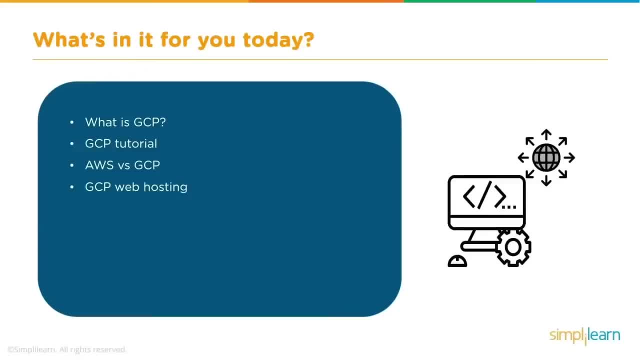 With a proper hands-on demonstration on these services. Following that, we will have a comparison between GCP, AWS and Azure and we'll see how they differ from each other and how they hold their individuality, And then, at the end, we will understand some of its depth. 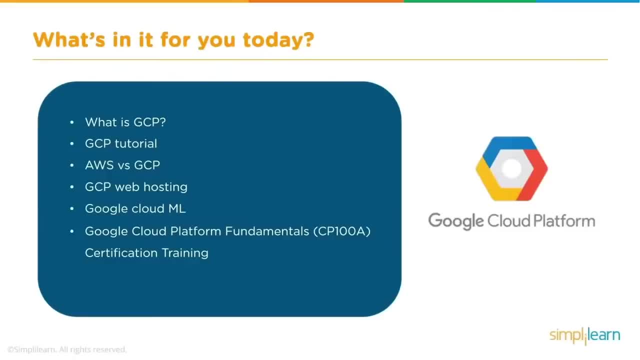 concepts like GCP web hosting and GCP Cloud ML, And towards the end, we will take you through GCP fundamentals and certification training that will help you gain this certification. So for this training, with me I have our experienced GCP specialist Together. we will take you. 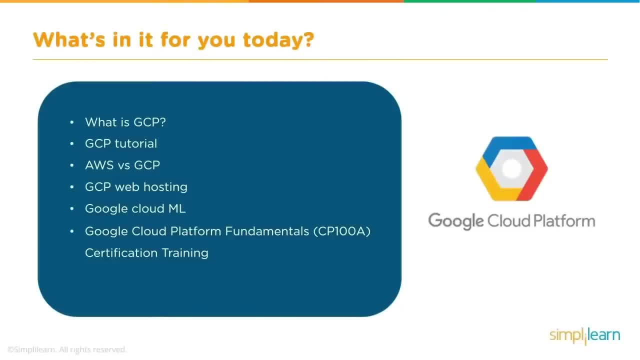 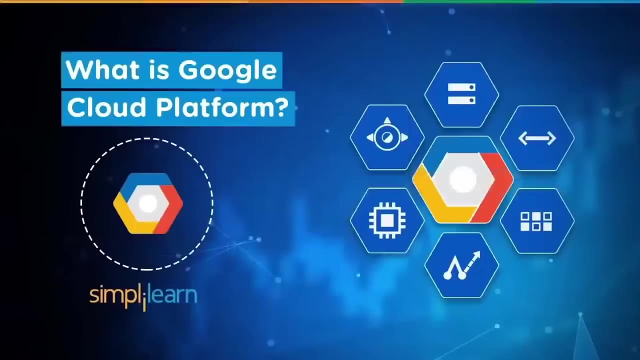 through the various important keynotes. So let's start with an exciting video on Google Cloud Platform full course. Before we begin, make sure to subscribe to our YouTube channel and hit the bell icon and never miss an update from SimplyLearn. Good morning and good evening everyone, So welcome to this session on Google Cloud Platform. 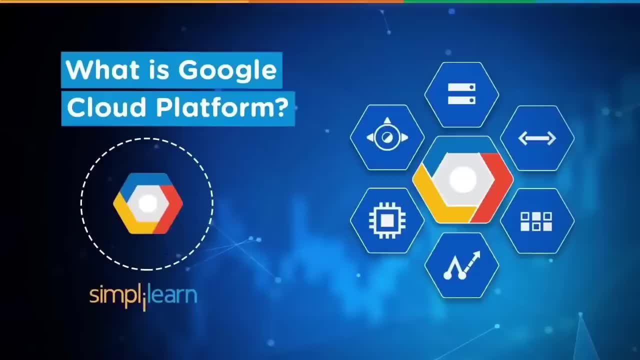 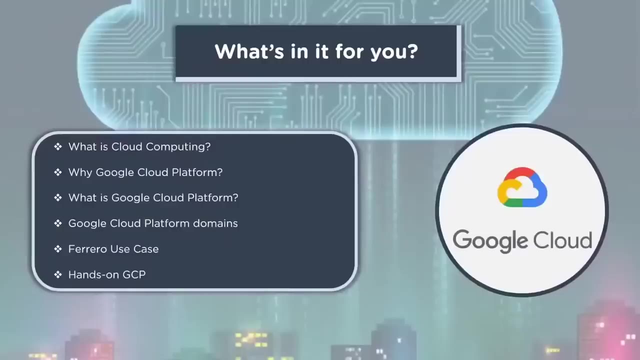 My name is AJ and I'm an instructor with SimplyLearn and also working as a big data and cloud architect for various clients across the globe. In this session, we learn about Google Cloud Platform, wherein we will learn about what is cloud computing, why Google Cloud Platform, what is GCP- that is Google Cloud Platform. 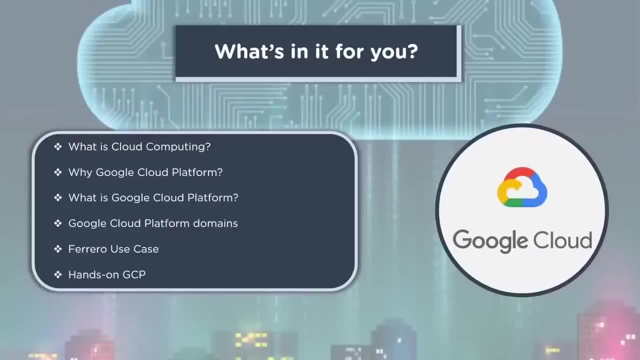 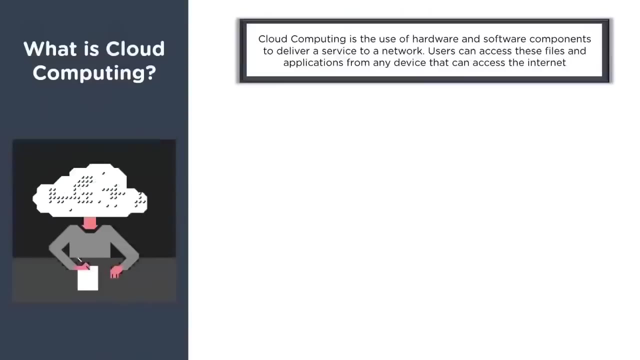 Google Cloud Platform domains about a use case- that is, Ferrero use case, and also a quick demo on using services from Google Cloud Platform. So when we talk about Google Cloud Platform, we know what is cloud computing. So cloud computing is the use of hardware and software. 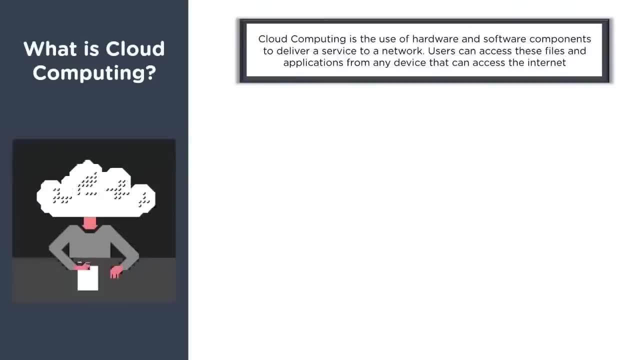 components to deliver a service to a network. Users can access these files and applications and services provided by a cloud provider from any device that has access to internet. In short, cloud computing is a way where cloud provider provides access to different services, such as resources. 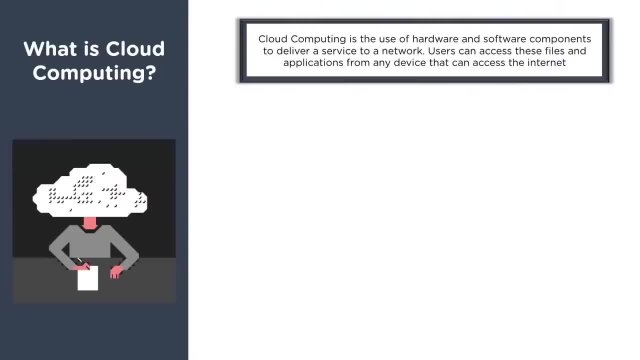 When we talk about resources here, we talk about computing, we talk about memory, we talk about processing power, we talk about storage and we also talk about different services which cloud providers make available for the users. Now that allows us for automatic. 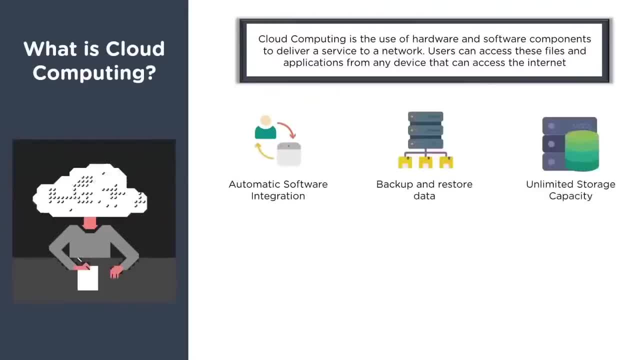 software integration, backup and restoring data, unlimited storage capacity, having a reliable use of different services And having a cost-efficient solution. Now we know that cloud computing's models. there are different service models. So you have platform as a service, you have infrastructure. 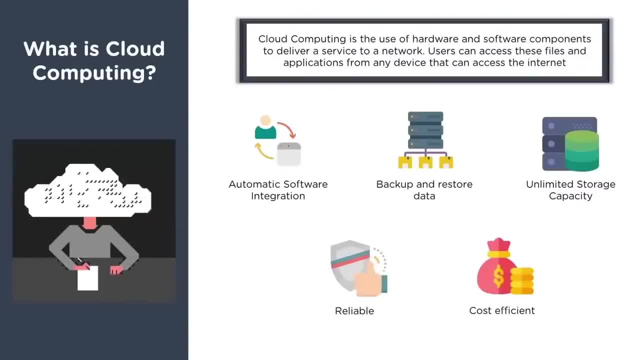 as a service and you have software as a service, And these are the prominent models which are offered by different cloud providers, such as Google Cloud, such as Google, you have Amazon, you have Azure and also some organizations such as Google Cloud Platform. So these are. 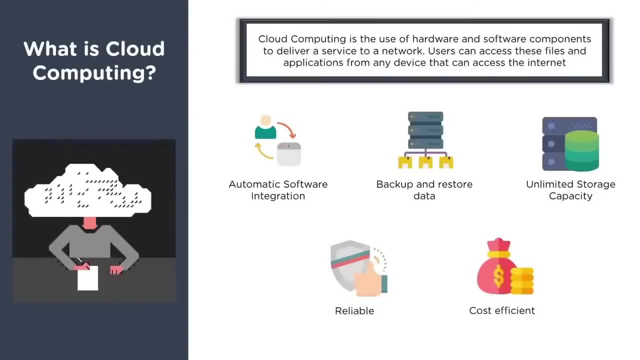 some of the things that cloud providers can do to help organizations build their own private clouds using open source, open stack. Let's focus more on Google Cloud Platform and what it has to offer and how it is gaining popularity in the market, with different organizations which would want to work on a cloud platform. 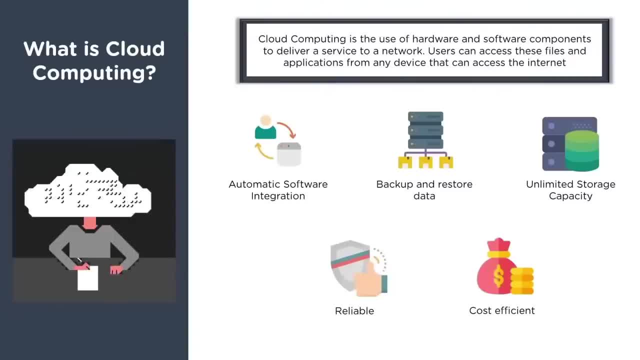 or which would want to work on an infrastructure which is modernized. So when we talk about cloud computing, So this is one of the approach which organizations can take to instantaneously benefit from modernization using different services, different platforms and also newer technologies for their various 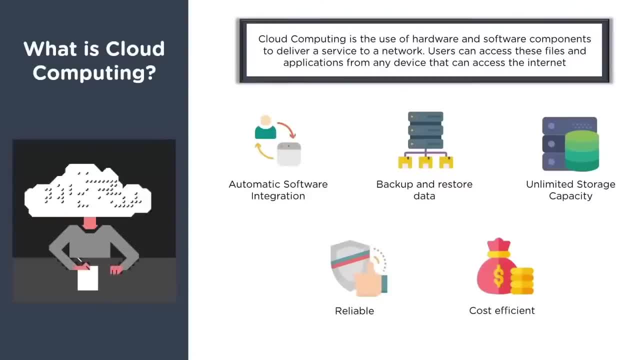 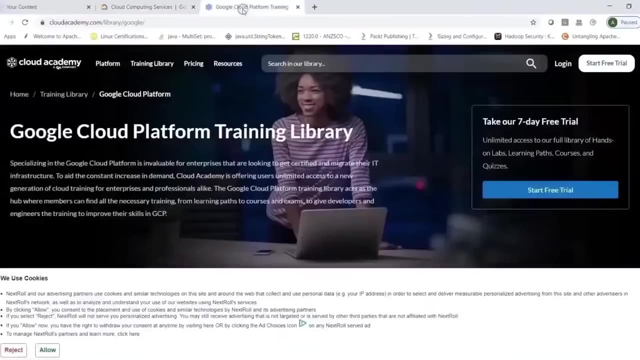 requirements such as scalability or dynamic businesses. Before we get into Google Cloud Platform, it is also good to understand where you can find some useful resources about Google Cloud Platform, And here you have a website which is from your Google Cloud, So this is cloudacademycom. 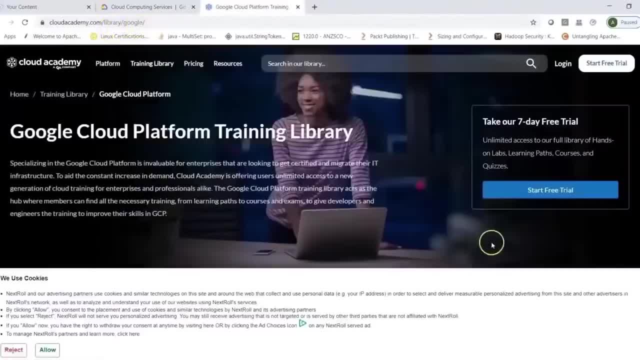 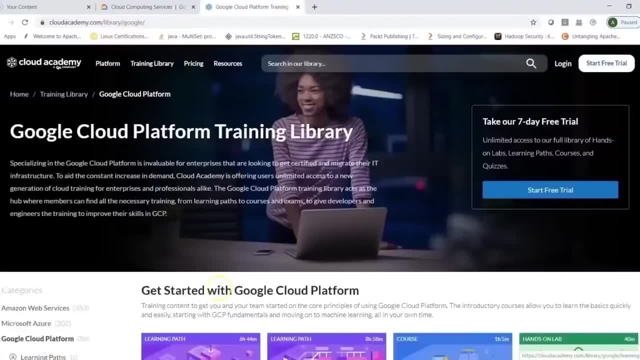 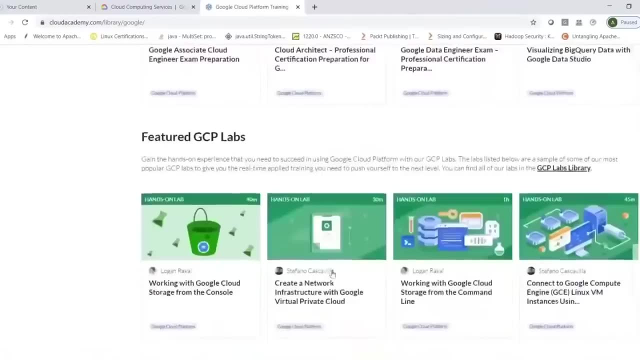 slash library, slash Google, And here you can create a free account Now. that would give you just seven days trial, but that has a lot of videos which talk about your Google Cloud Platform and essentials, and it has various certification related videos which you can access. 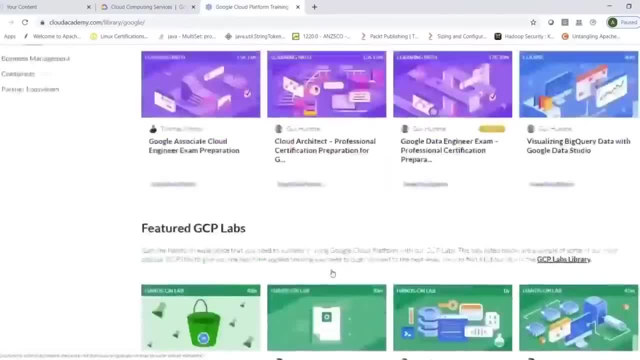 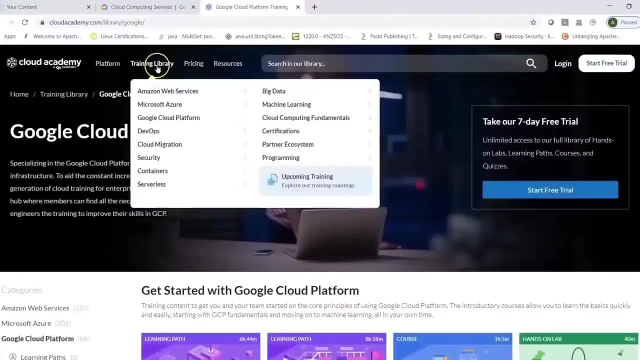 And then, after seven days, after you have tried, You can obviously go for a paid account where you can take detailed learning from here. Now this is your training library, which shows you a different cloud providers, such as Amazon, Microsoft Azure, GCP, and then you have various other topics which are specifics to organization. 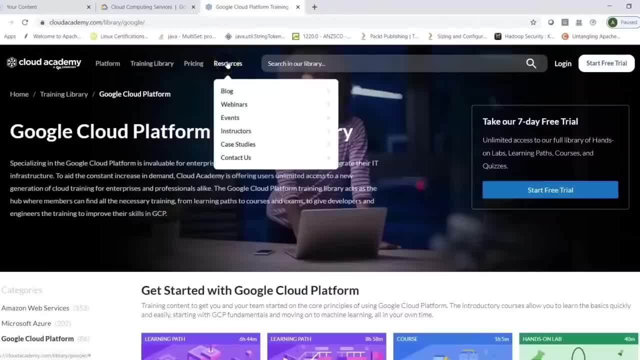 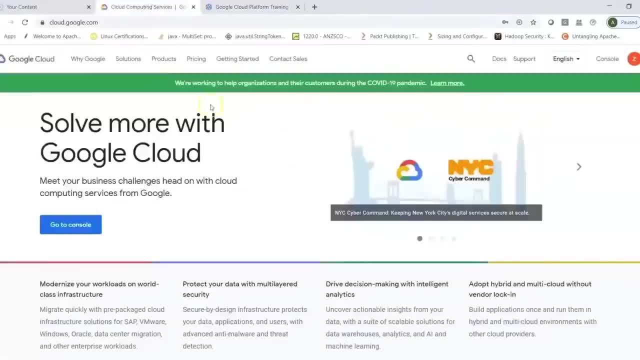 You can obviously look at the pricing and you can also look at resources, which will give you a good experience in learning from these videos. You can also create a free account, which I will walk you through later, So you can create a free account on cloudgooglecom. Now, when I say free account, that basically means it. 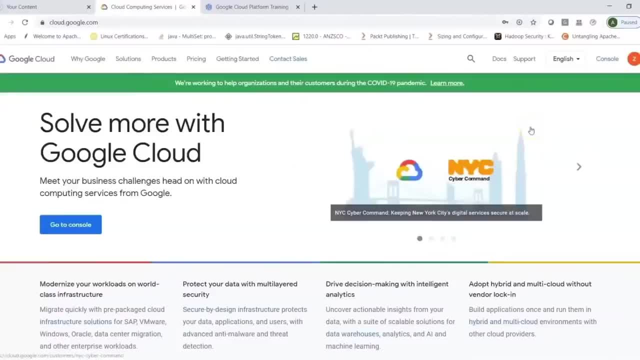 allows you to create an account, and every user who creates an account gets a $300 free credit which can be used to practice, brush up your skills and also explore and learn about different Google Cloud products, Which are free, Which are offered by Google. 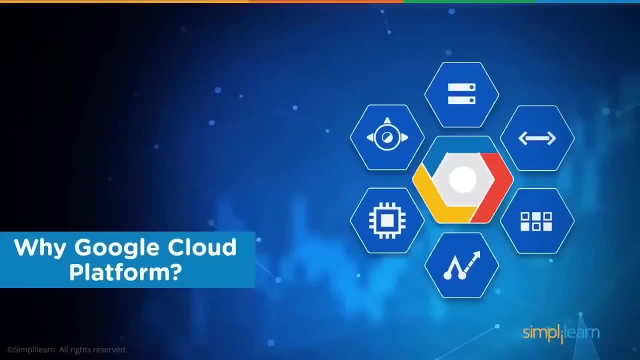 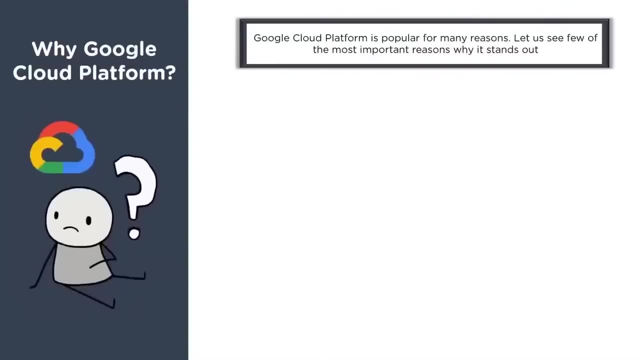 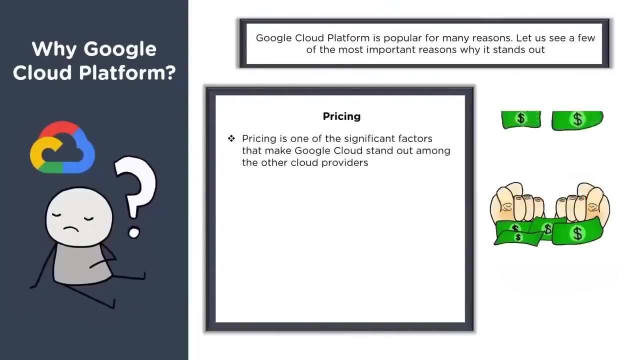 Now coming back to our Google Cloud Platform, let's understand why Google Cloud Platform, So Google Cloud Platform- is popular for many reasons. Now let us see few of most important reasons why it stands out. When you talk about pricing, pricing is one of the significant factors that make Google. 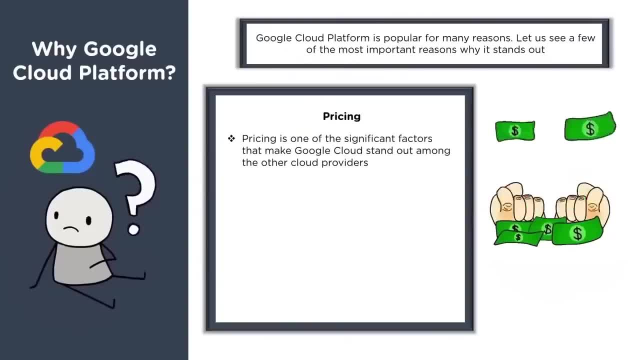 Cloud stand out among the other cloud providers. It offers a monthly pricing plan Which is billed according to monthly usage, And when we talk about billing here, the billing can be in hours, it can be in minutes and it can also be in seconds. 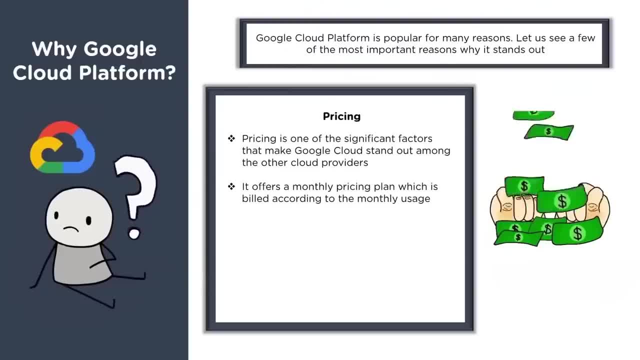 There are different options when you talk about your pricing, which can be found from your Google Cloud web page. Now, pricing could be based on preemptive machines. Pricing could be based on reserved instances or reserved resources. I'll show you the links. I'll show you the link where you can find more details on pricing- part of it. 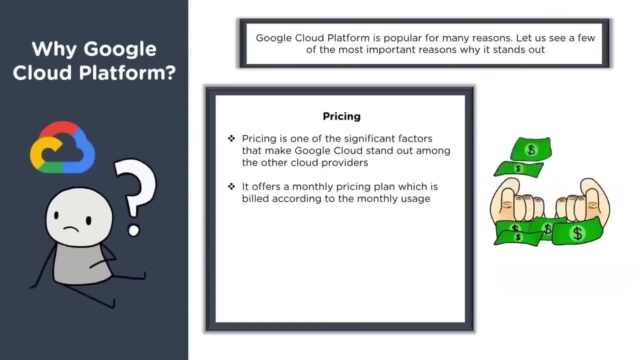 So Google Cloud really has various pricing options which help customers in their different requirements, whether they would go for any of the service models, such as infrastructure as a service, platform as a service or even software as a service. One more attractive thing about Google Cloud pricing is that it provides committed use. 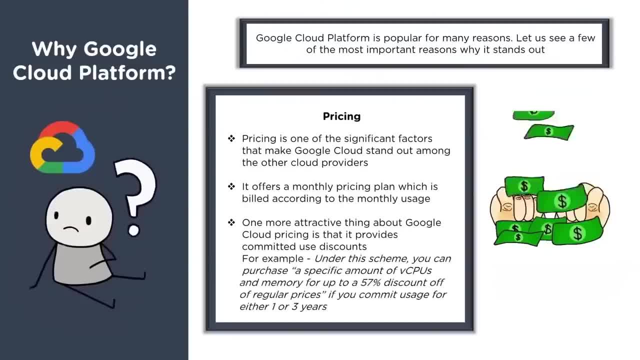 discounts. For example, Right Under this scheme you can purchase a specific amount of virtual CPU cores and memory for up to 57% discount off regular prices if you commit usage for either one or three years. Now, this is just one option. 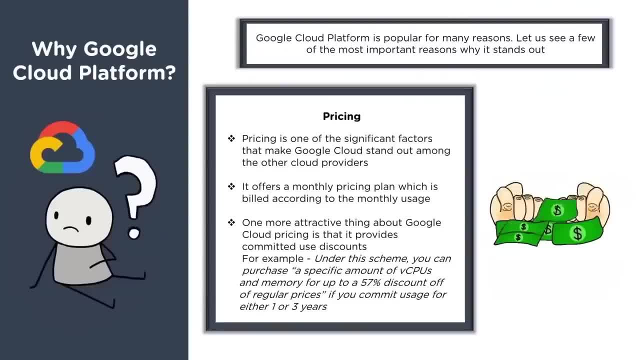 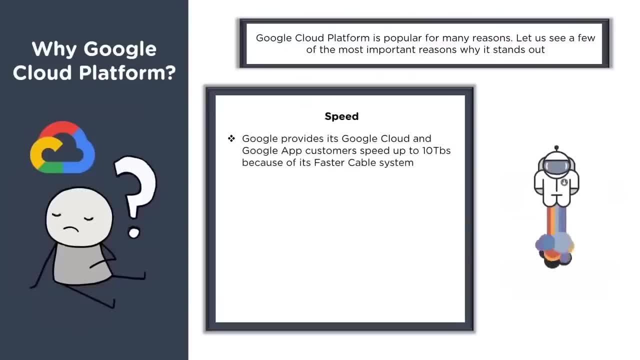 There are various such options, which you can learn about from the Google Cloud's page, And that really suits different customers for their different requirements. Now, when we talk about speed, we don't need to really challenge this Aspect when it comes to Google services. 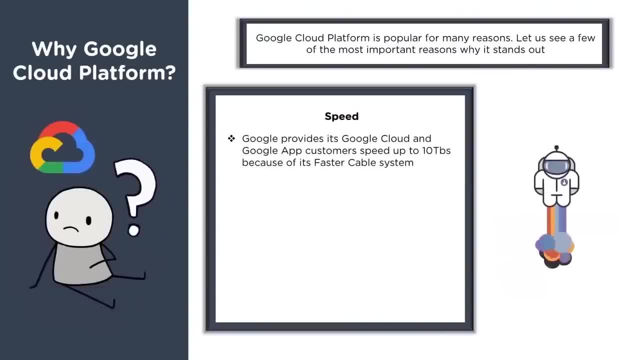 So Google provides its Google Cloud and Google App customer speed up to 10 terabytes because of its faster cable system. There are different kinds of machines which can be used: if you're talking about computation, if you're talking about memory hungry applications or even storage intensive workloads. 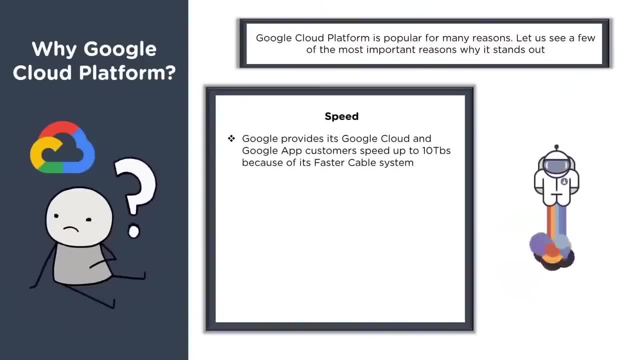 All in all, speed is one of the defining characteristics of Google Cloud, And that's what we're going to talk about today. Thank you, Cloud services. The cable has connections over US West Coast, Main cities in Japan and even major hubs in Asia. 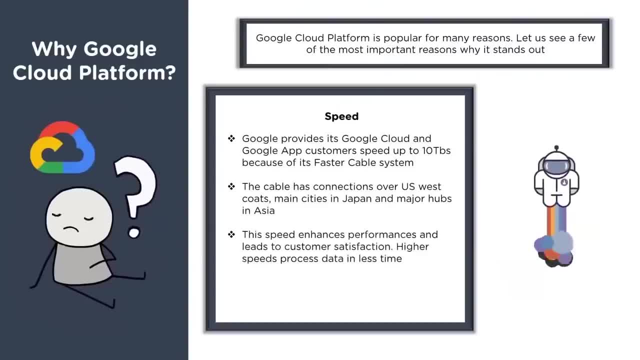 This speed enhances performances and leads to customer satisfaction. Now, when we talk about customers, any or every customer would prefer to have low latency, high throughput-based services. They would want to use higher speeds to process their data in as less time as possible. 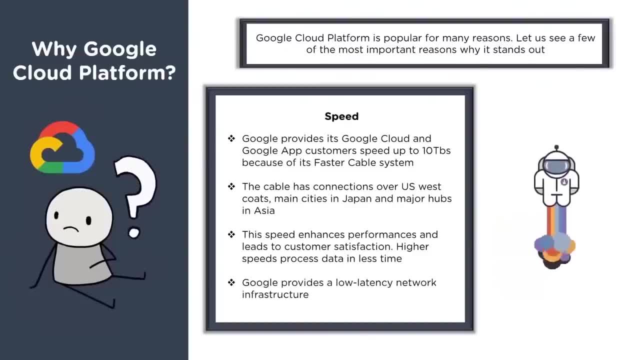 So, all in all, this means the vengeful Internet user is getting a bit of a challenge. I'm sure as possible, Google provides a low latency network infrastructure. In fact, you can say that when you are using Google Cloud services, you are using the services from the same infrastructure. 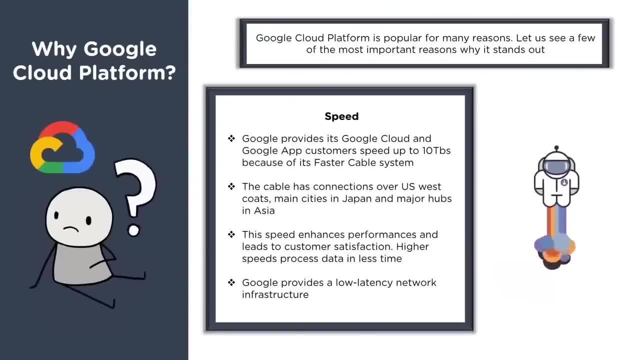 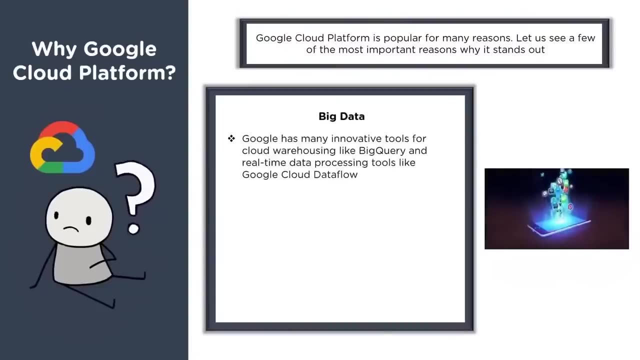 which Google uses for its popular services, such as Google search or even YouTube, which is one of the second largest repository which can be accessed for videos. Now, when we talk about big data, big data is data which is very complex, has a lot of other characteristics. 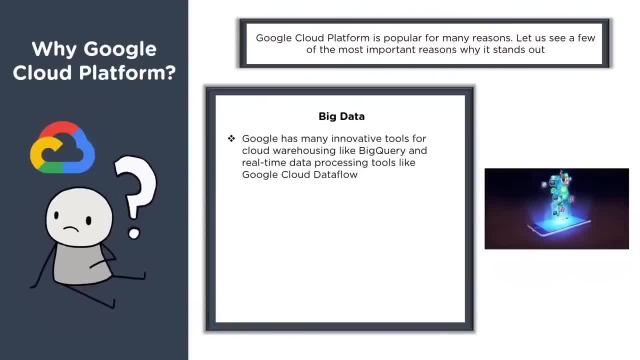 such as your volume, you have velocity, you have variety, you have veracity, validity, volatility, virality and so on. So if an organization is working on big data, Google Cloud can be a better choice, because Google has many innovative tools for cloud warehouse. 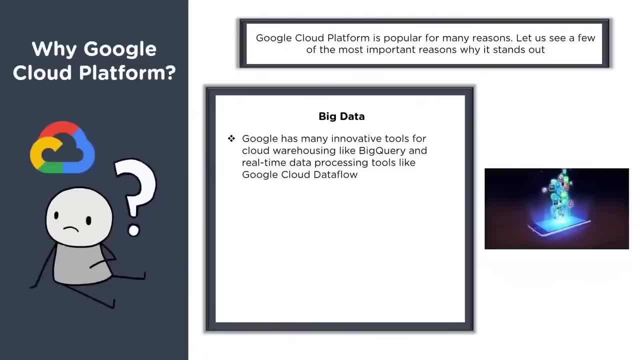 processing, for example, such as BigQuery, and even real-time data processing tools such as Dataflow. BigQuery is a data warehouse that allows massive processing of data at high speeds, basically working on your structured data. Google also has launched some new machine. 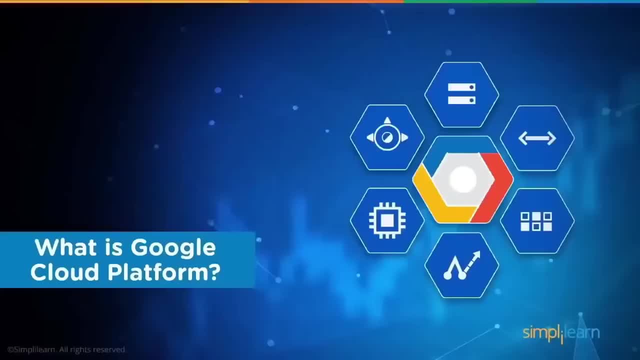 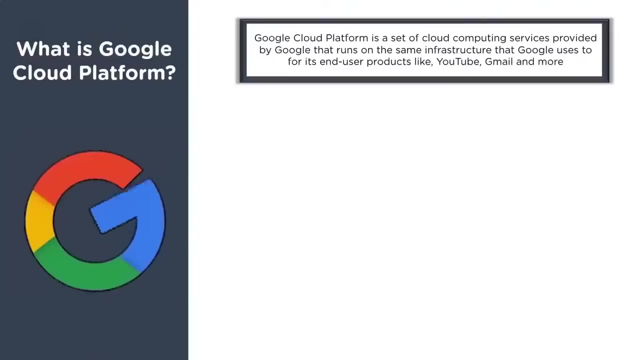 learning from artificial intelligence tools. Now there are various other services which we can use from Google Cloud platform, but let's understand what is Google Cloud platform and what are some of the services. Even the services which are not listed here can be found in your console from Google Cloud. So what is Google Cloud platform? GCP It is. 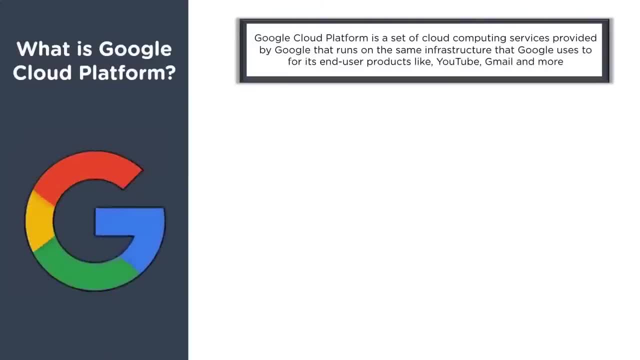 a set of cloud computing services provided by Google that runs on the same infrastructure, as I mentioned, that Google uses for its end user products like YouTube, Gmail and even Google search. The various set of services offered by Google Cloud platform are mentioned here, So you have services which are specific to computing requirements and 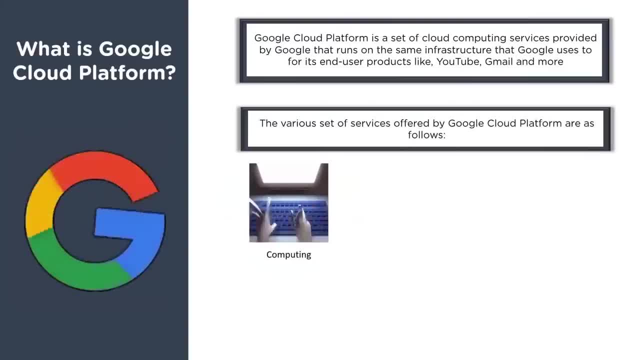 again, in computing you have various different options available. You have machines which are compute optimized, machines which are memory optimized, machines which are storage optimized, and also we have certain machines such as pre-emptive, which basically means that you could get a machine to work on at a far lesser price. 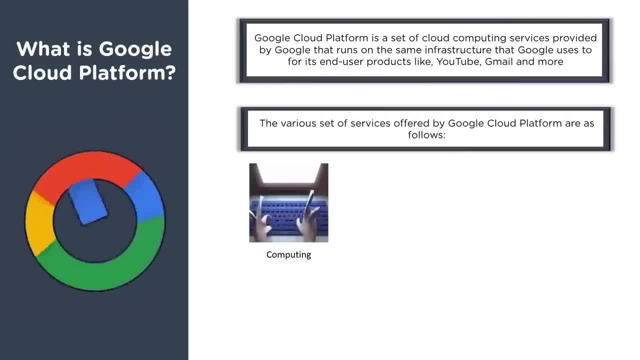 than any other machine. But when we talk about preemptive, these are the machines which can be requested on demand and they can be taken back by Google at any time. You have networking related services which can be very useful when you are setting up your applications or your services. 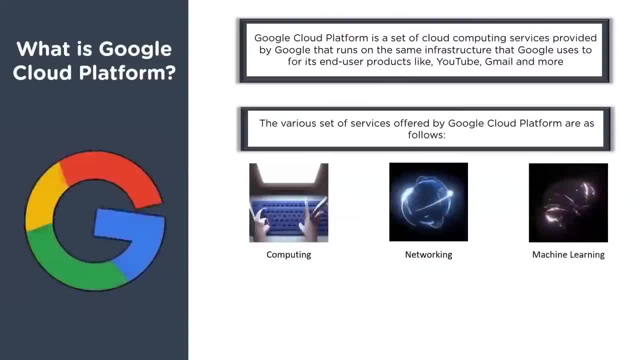 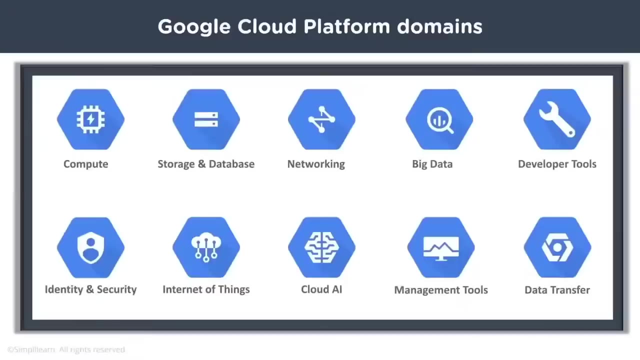 across globe. You also have different services which are specific to machine learning, and organizations which would be interested in working on machine learning or artificial intelligence would be really interested in using these services. There are also innovative solutions to work on big data and big data related technologies. Now, when we talk about Google Cloud Platform domains. 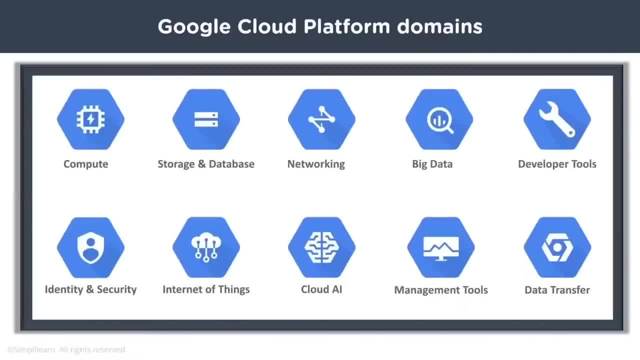 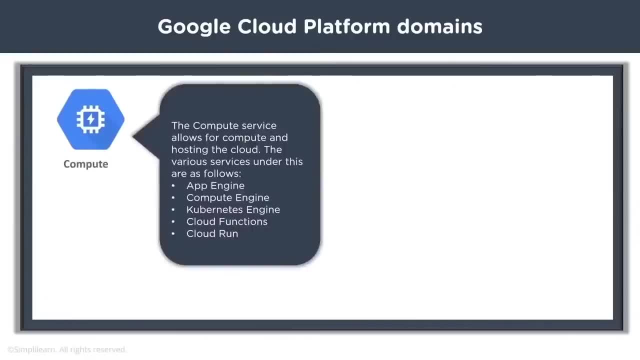 so we can break down these services into specifics, such as: you have compute, Now the compute service allows for computing and hosting The cloud. Now, when you talk about computing here, there are different services, such as app engine. You have compute engine. You have Kubernetes, You have cloud functions and cloud run. When you talk 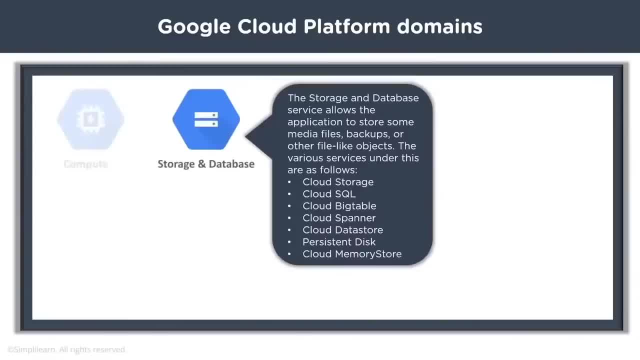 about storage and database. so the storage and database service allows application to store media files, backups or other file like objects. Now, various services under this are as follows: You have cloud storage, Cloud SQL cloud big table for unstructured data. you have cloud Spanner, cloud datastore, persistent. 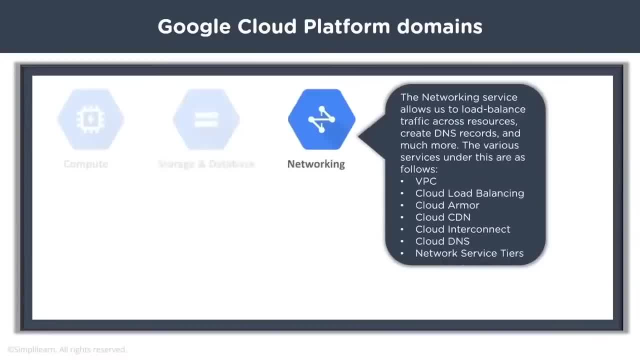 disks and cloud memory store. When we talk about networking, the networking service allows us to load balanced traffic across resources. Now, as I mentioned earlier, resources could be your different resources which you would be using from a cloud platform, such as your devices, your. 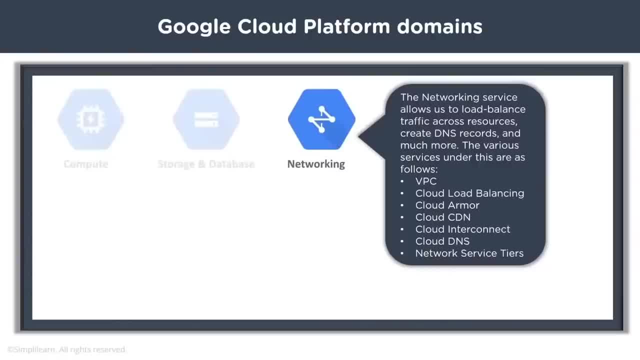 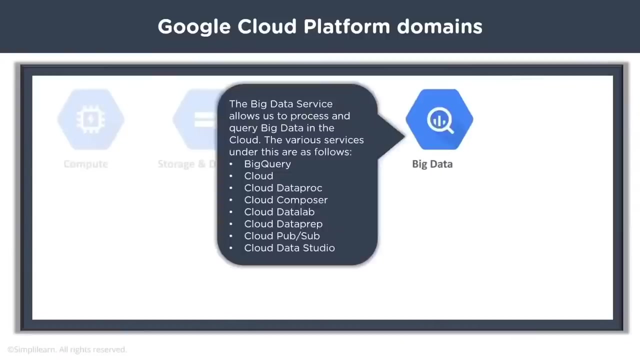 instances, memory or CPU, optimized instances or other resources- creating DNS records and much more so. various services under this are VPC, that stands for virtual private cloud. you have cloud load balancing, cloud armor, cloud, CDN. you have cloud interconnect, DNS and network service tiers. when we talk about the big data, 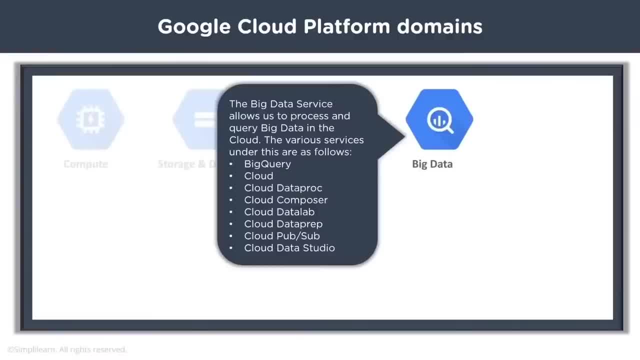 service. this allows us to process and query big data in cloud. now, various services under these are as follows: you have big query cloud cloud data proc, cloud, composer, cloud data lab, cloud data prep, cloud, pub, sub, which is publish and subscribing system. you have cloud data studio. now you also have the developer. 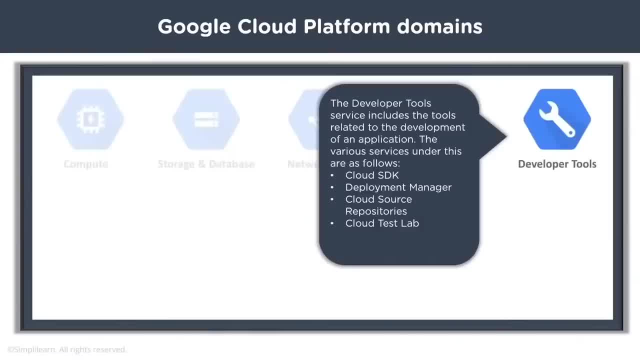 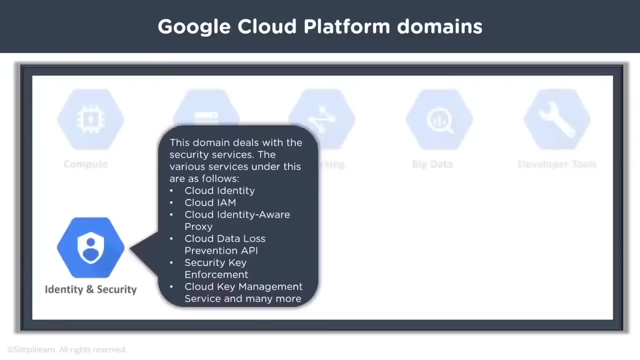 tools and developer tools. service includes tools related to development of an application. now, various services under these are as follows. that is, you have cloud SDK software development kit, you have deployment manager, cloud source repositories and cloud test lab. when we talk about identity and security, which is one of the primary concerns for any 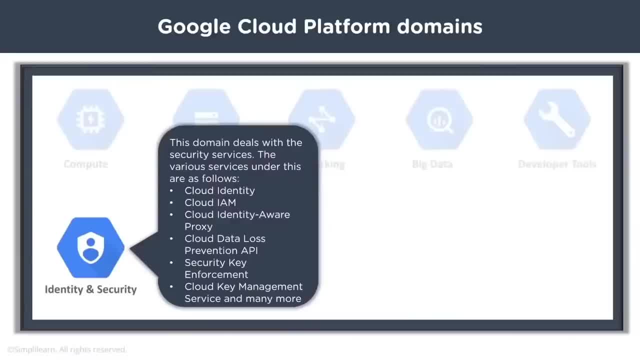 organization or any user who would be interested in using a cloud platform. Google Cloud really has taken care of this. so when you talk about identity and security domain, this deals with security services. now, various services here are cloud identity- you have identity- and access management- that is, cloud IAM- you have identity aware. 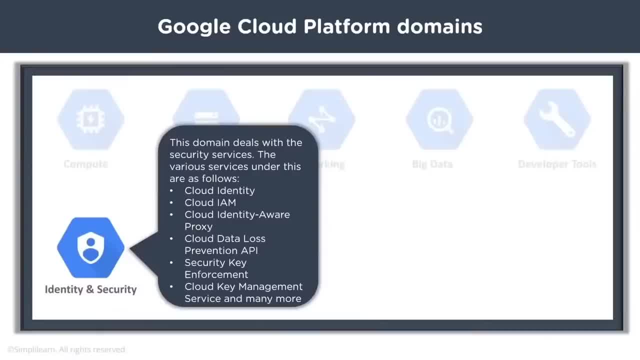 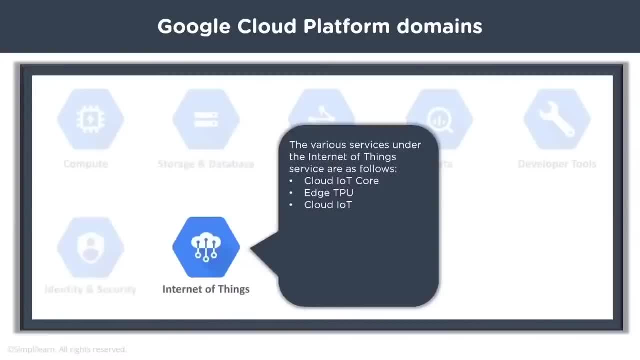 proxies. you have cloud data loss prevention, API, security, key enforcement, key management service and many more. you also have cloud services which are related to Internet of Things, so very much would be used by organizations who would be working on IOT devices or the data generated by these devices. 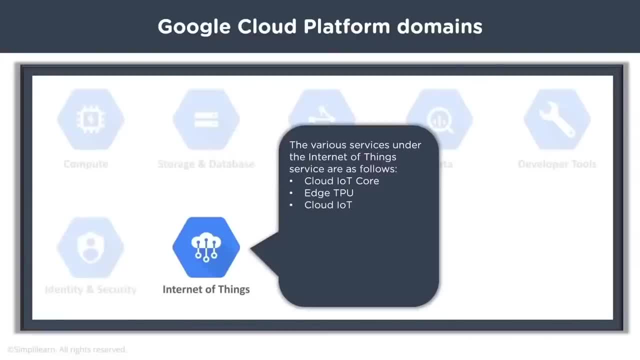 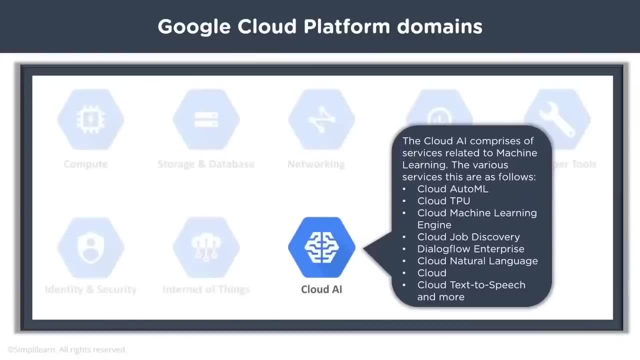 so these services here are cloud IOT core. you have edge TPU and cloud IOT also. when we talk about cloud AI, that is artificial intelligence. this comprises of services related to machine learning and much more. so you have cloud auto, ml, cloud TPU, cloud machine learning engine, job discovery, dialogue, flow, enterprise. 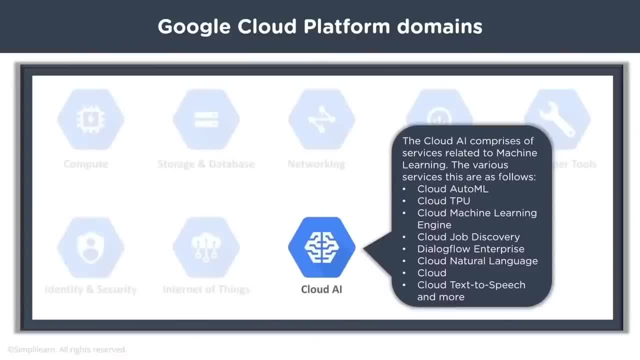 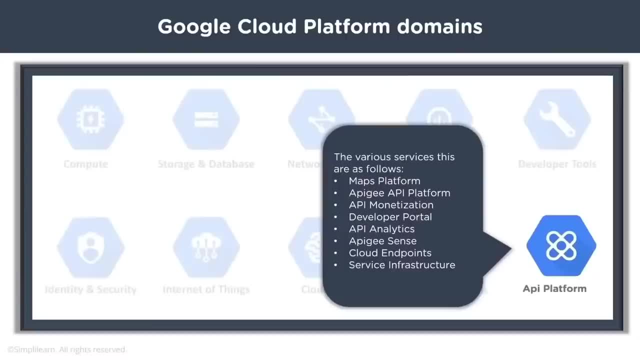 natural language, cloud, text-to-speech and much more. you would be interested in services related to API platform. then there are different services under this category or this domain. so you have maps platform, you have APG API platform, monetization, developer portal, analytics- that is, API analytics, APG sense, cloud endpoints and service infrastructure. so these are some. 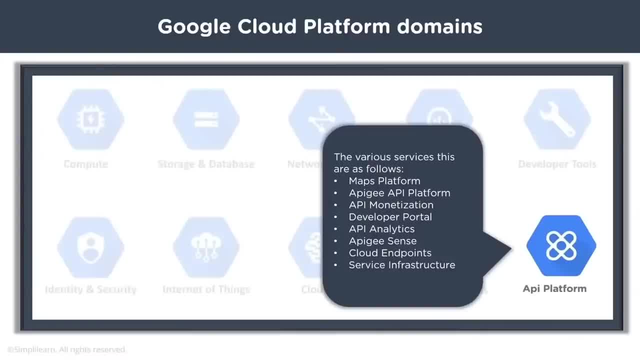 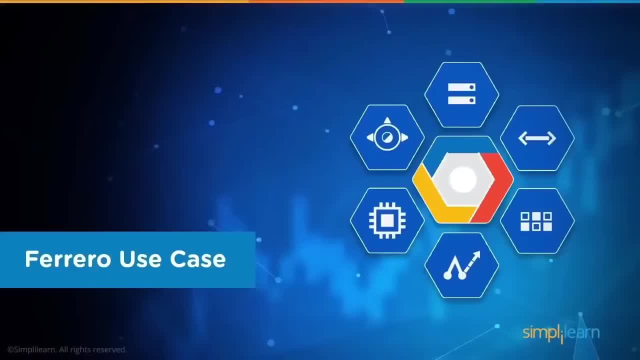 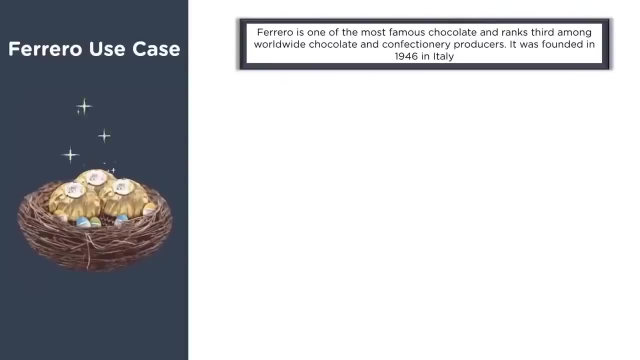 of the listing of services under each cloud platform domain. now let's look at further, oh use case, and let's also understand what was done here. so federal is one of the famous chocolate and ranks third among worldwide chocolate and confectionery producers. it was found in 1946 in Italy. I'm sure you 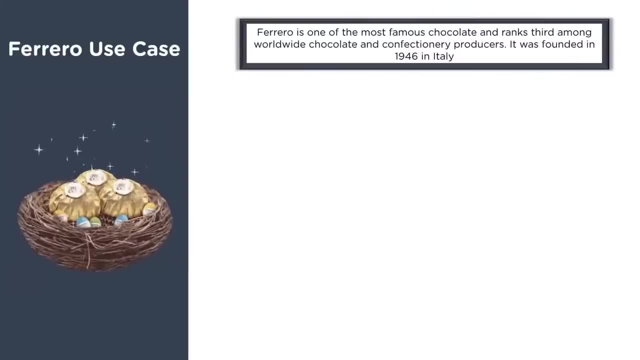 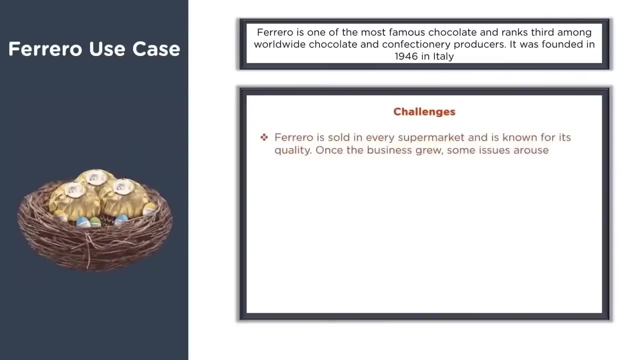 would have seen the federal chocolates, then you would have gone out to buy some chocolates. so the challenges here was that federal, as we know, is sold in every supermarket and is known for its quality. once the business grew, some issues arose. right, and that's what happens. when the business grows, you have issues popping up which could be related. 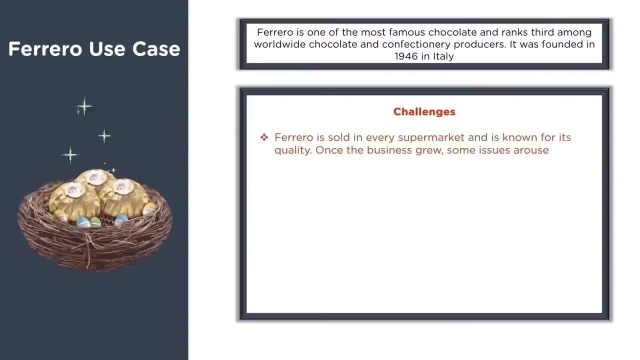 to the volume of data, the speed with which the data is getting generated, the variety of data and also looking at your platforms, which support different dynamic applications, or your scalability requirements, performance requirements and so on. so it needed data storage, processing and analysis system for a wide customer database. there was a huge gap between the company and the people who 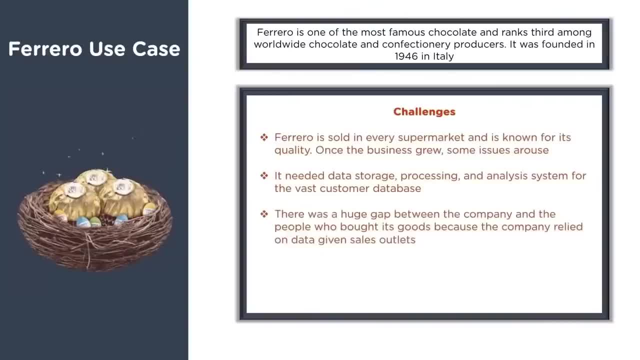 bought its goods because the company relied on data given sales outlets. now, that's one of the challenge ferrero wanted to create a digital ecosystem where there was a point of contact with its customers and also a foundation for an innovative data-driven marketing strategy. what was the solution here? so, one of the service. 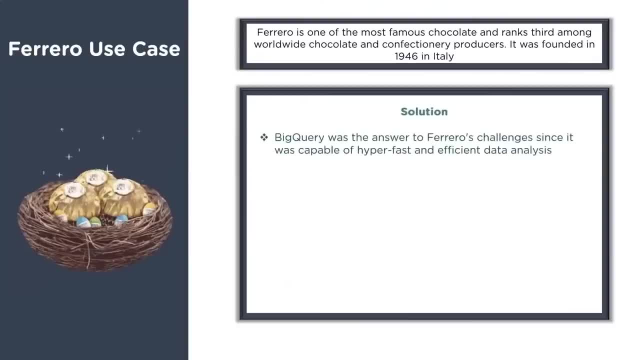 of cloud platforms, or google cloud platform, is bigquery, and this was an answer to ferrero's challenges, since it was capable of hyper fast and efficient data analysis as a solution. now, as i mentioned, bigquery is a data warehouse which allows you to store structured data. now this could 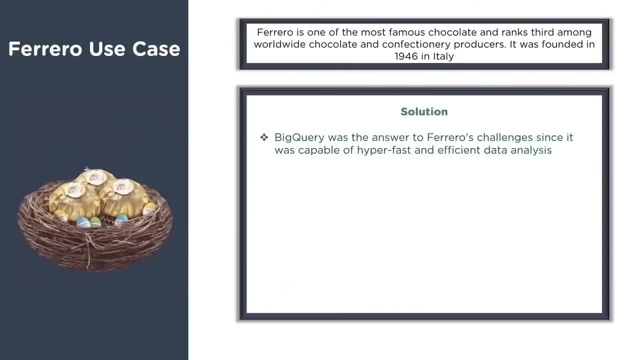 directly be used as a service to store structured data and also to store structured data where you could store in any amount of data and you would not be paying for storage. so there are different pricing models and for data up to one terabytes you would not be charged anything and 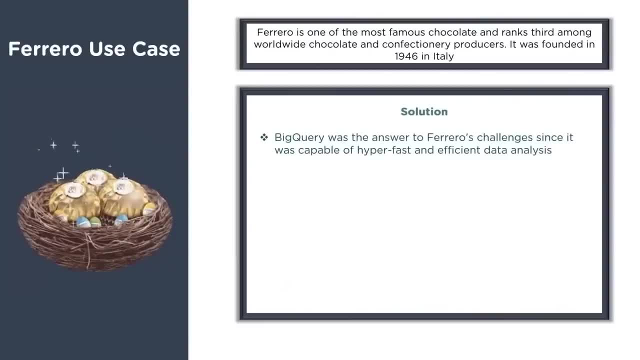 if you would be accessing the data, that is, reading the data or processing the data from bigquery. that's where the pricing model kicks in now, using google cloud's bigquery, business analysts of ferrero were able to store and analyze massive data sets in a very reliable 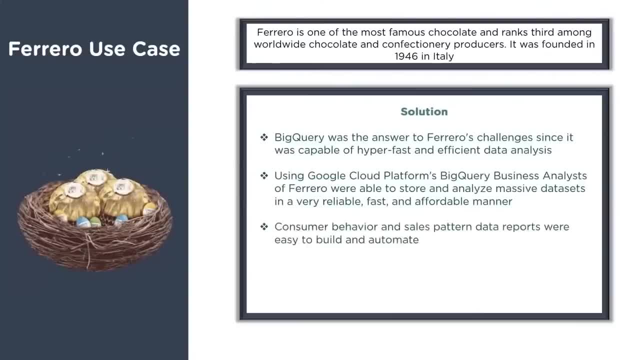 fast and affordable manner. consumer behavior and sales pattern data reports were easy to build and automate, and the analysis also followed ferrero to adopt advertising across various marketing channels to serve the customer needs in a better way. what was the result? they could divide their database into real-time actionable consumer clusters to generate more accurate user profiles. ferrero was 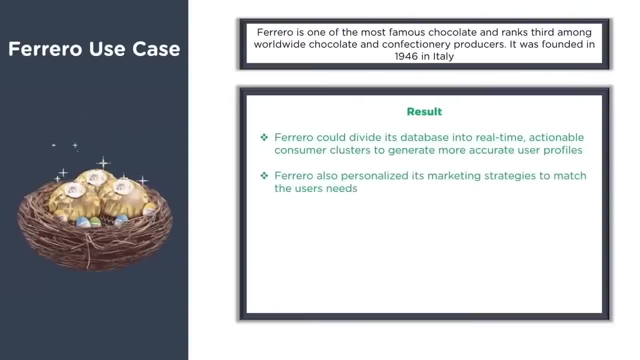 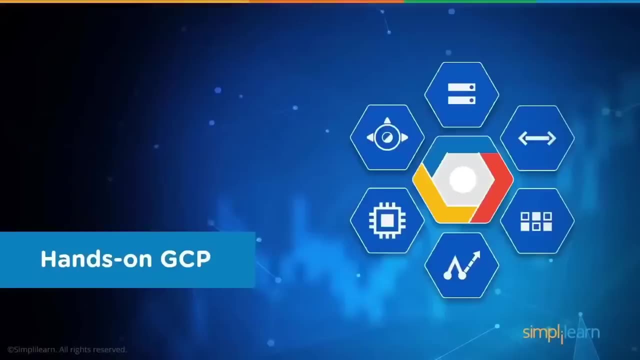 also able to personalize its marketing strategies to match the user needs. now, google cloud platform completely tailored the website, mobile content and advertising, and created a very cost-effective media buy strategy. now, these were some basics on google cloud. now, as i said, you can always find a lot of details about pricing, about services and also all the 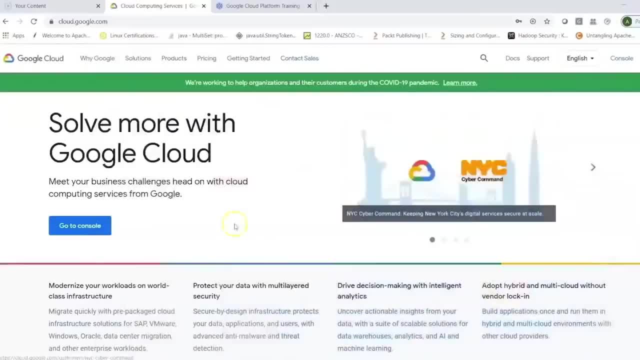 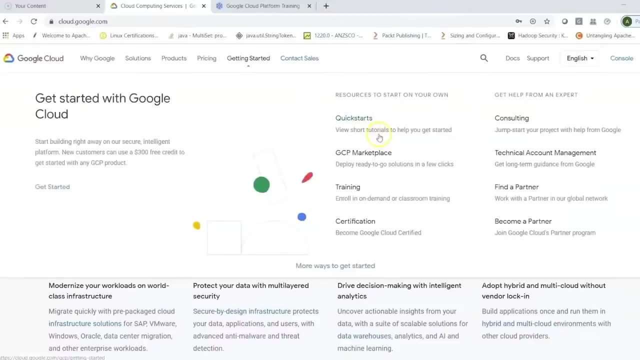 services are accessible in your free trial account. now let me just walk you through here. so one is: you could always find details on documentation on each of these services. so if i would click on getting started, you have quick start which basically shows you short tutorials. you have 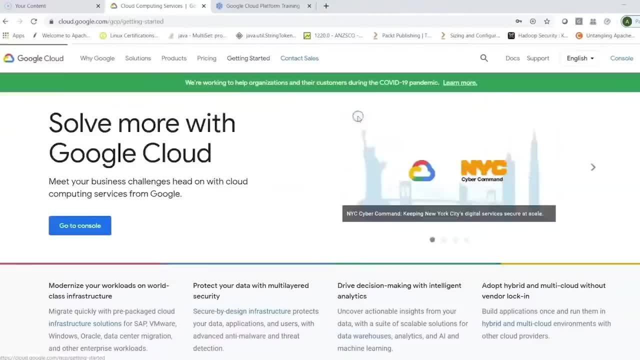 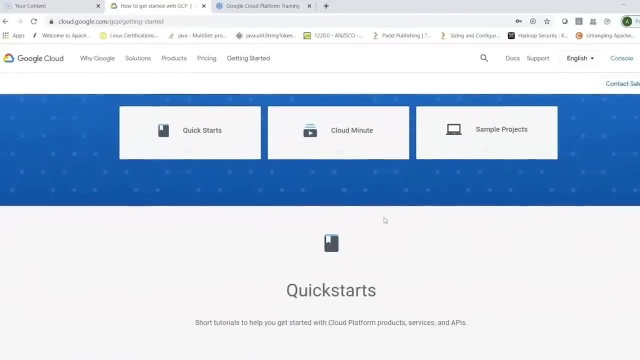 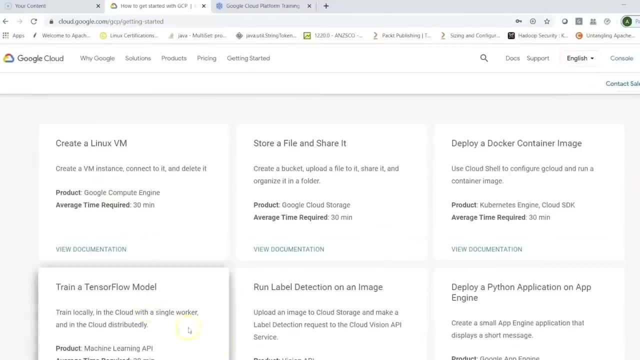 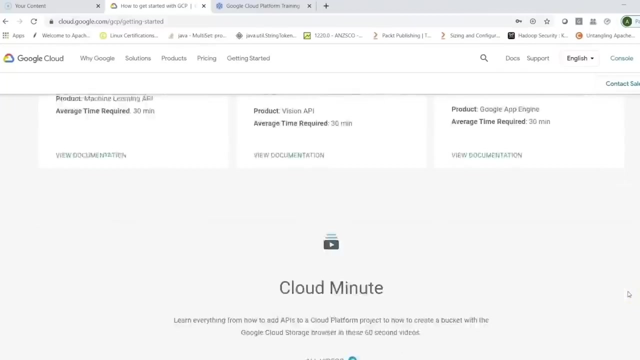 trainings and you have also certifications and you have a lot of details about pricing and services. Now, if we click on Quick Start- now that takes me to this page which shows me Quick Starts- or if you would want to understand about different projects, if you would want to look into the documentation of creating a Linux virtual machine or storing a file and sharing it, deploying a container, Docker container image, and so on, 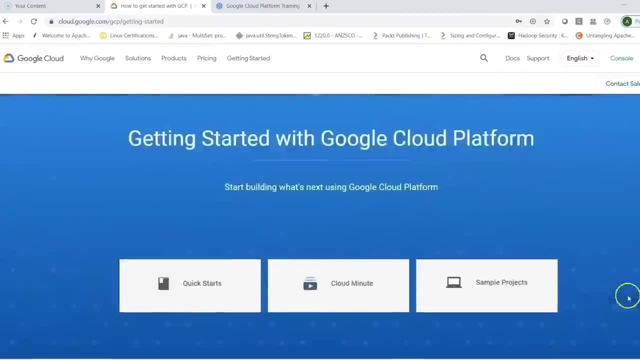 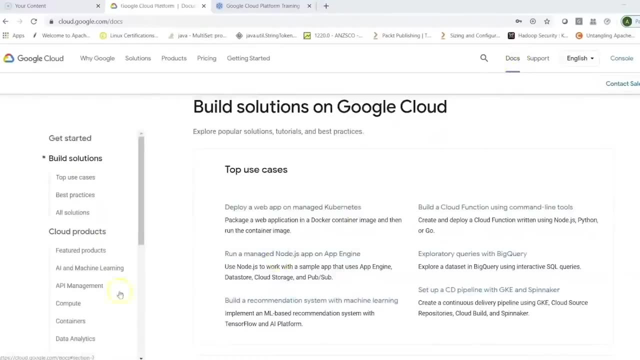 So you have a lot of Quick Starts here. You can also look at Cloud Minute. On the same page, on the right side, you have Docs and once you click on that it takes you to these links. Now this shows you Build Solutions, which shows you top use cases, best practices, all the solutions. It's always good to learn from these use cases which are available. 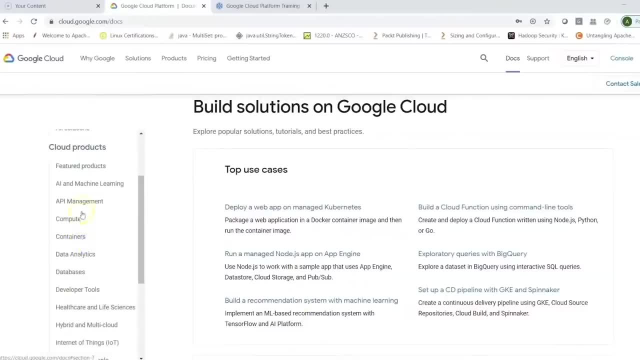 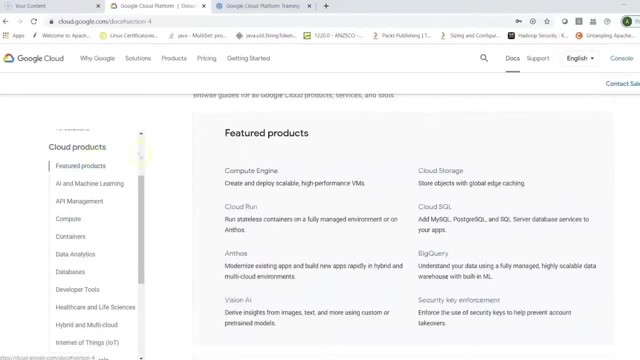 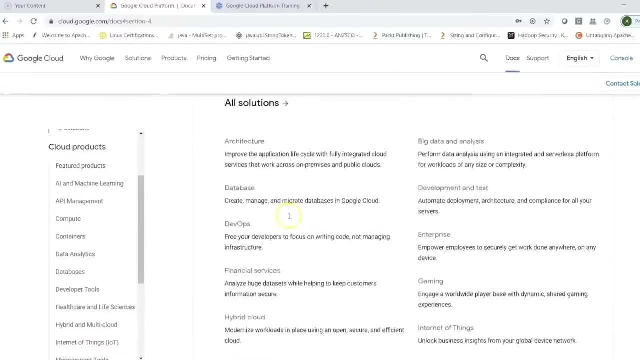 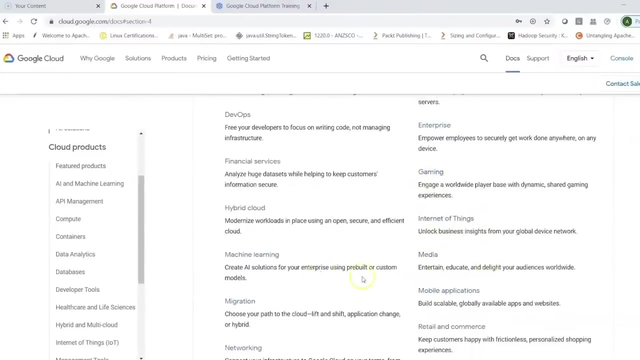 And here you have different feature products and all the different services which Google Cloud offers. Now you can click on Featured Products and that basically shows you a list of these products. Now here we have all the solutions which you can look at: Architecture, Database, Enterprise Level, Big Data and Analysis, Gaming Related, Internet of Things, and so on. 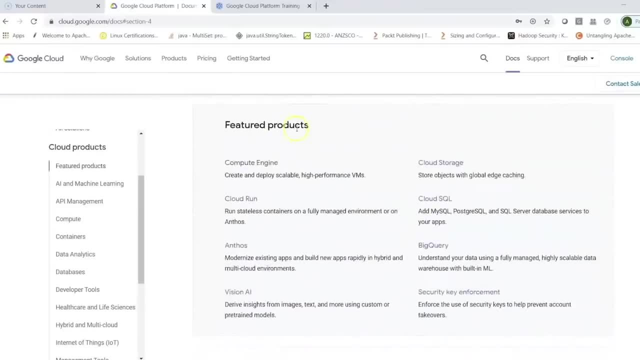 Now, if you go down here, it shows you Featured Products and that shows you some of the important products, such as Compute Engine, which is belonging to the compute domain. You have Cloud Run, You have Apps, You have Panthers, which is for migration, and basically cloud adoption, when organizations would want to move from on-premise to cloud-based solutions. 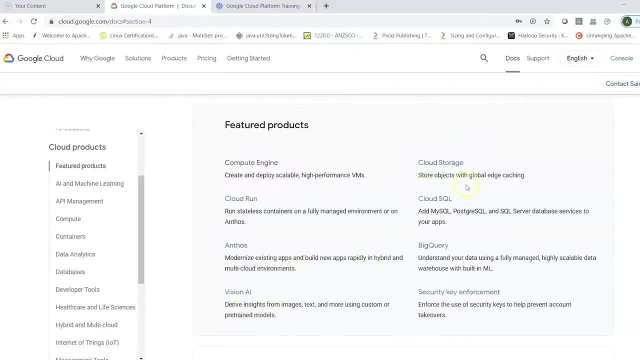 You have Vision AI. You have Cloud Storage. Now, that basically allows you to store any kind of data, whether that's an object. So this is acting as an object storage. You have Cloud SQL, which is basically a ready-to-use service where you would be using MySQL, Postgres or any other. 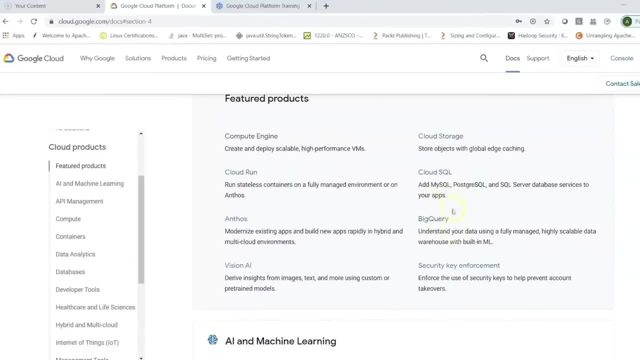 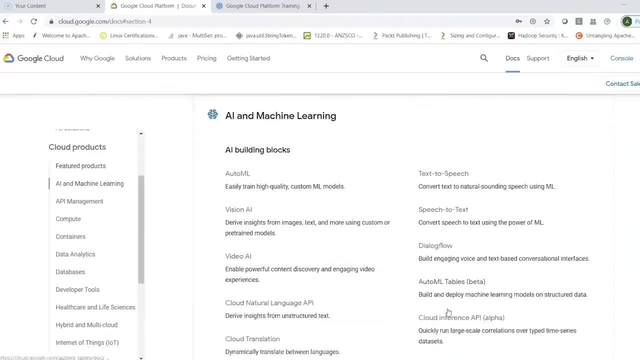 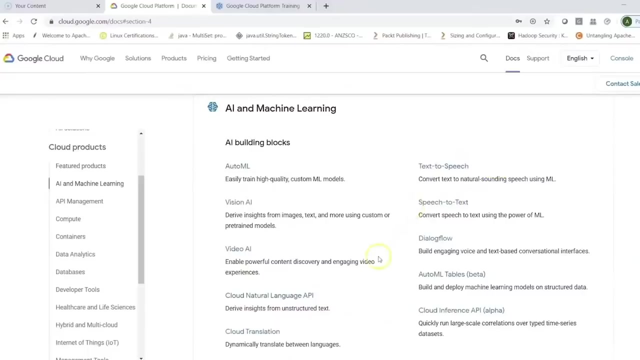 You have Cloud SQL Server Database services. You have BigQuery, which is a data warehouse which basically allows you to store your structured data, And then you have your AI and machine learning-related products. So you have AutoML, Vision, AI, Video, AI, Text-to-Speech, Speech-to-Text, and so on. 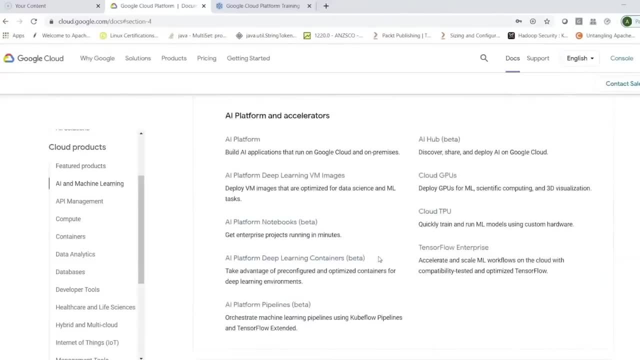 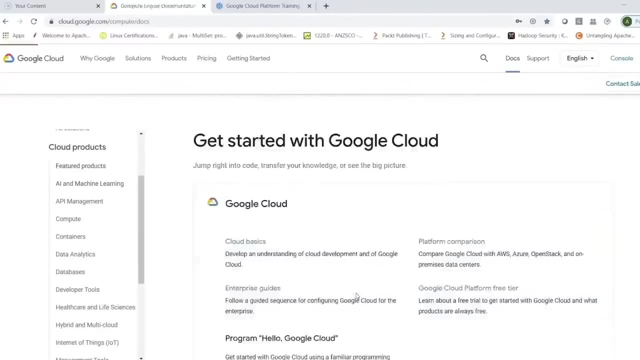 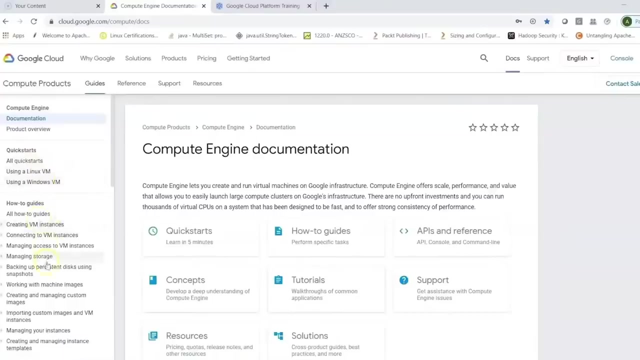 Now you also have different platform accelerators which can be used, And in any of these cases, for example, if I would click on Compute Engine, which is a featured product from Google Cloud, now that shows you basically your quick starts using your Linux machines. 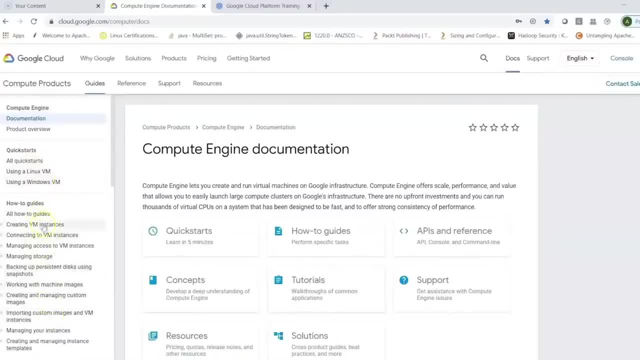 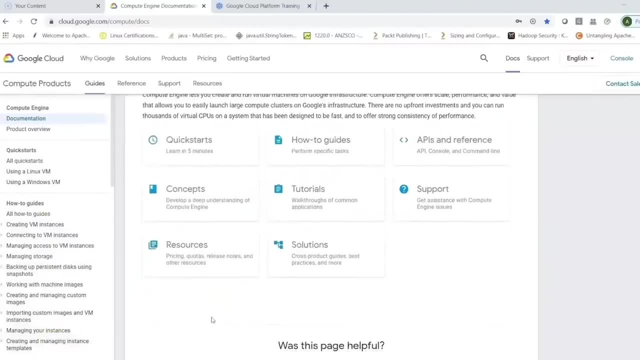 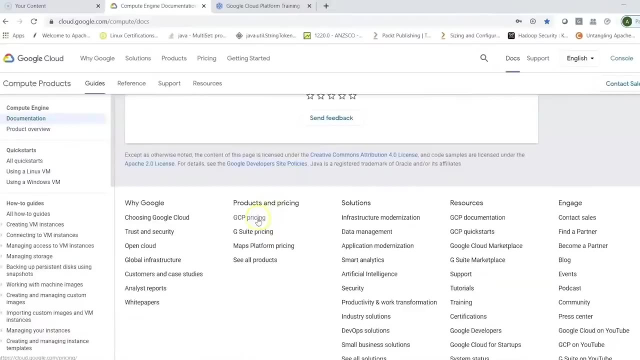 how-to guides which tells you completely working on a VM instance or working on storage, working on persistent disks and so on, and it shows you the documentation here. now you also have products and pricing option which you can see for GCB pricing and you could straight away go to the pricing you. 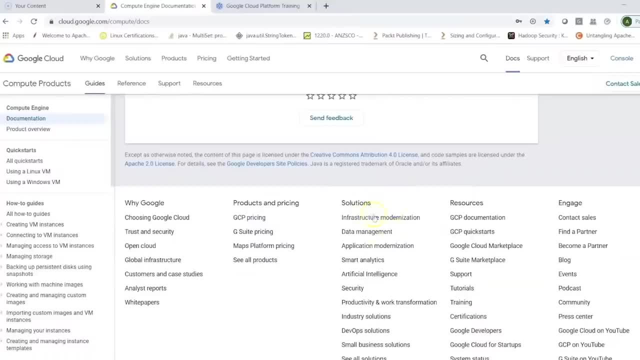 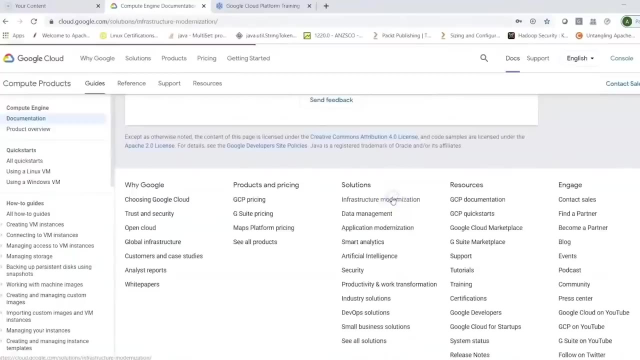 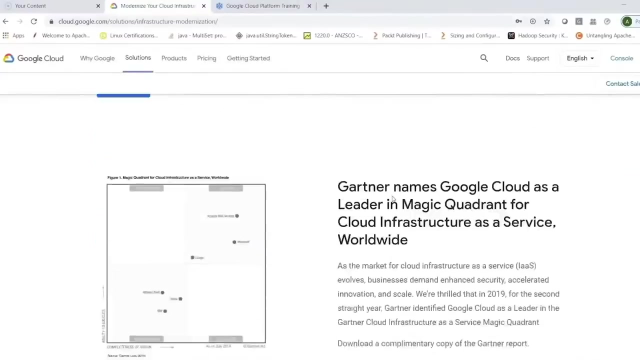 could be looking at solutions which talks about infrastructure modernization. now, this is something which organizations are interested in when they would want to move from their on-premise solution to your Google Cloud. now, here I can say, for example: I click on infrastructure modernization, you can always find some case studies. what are the different solutions you we have here? 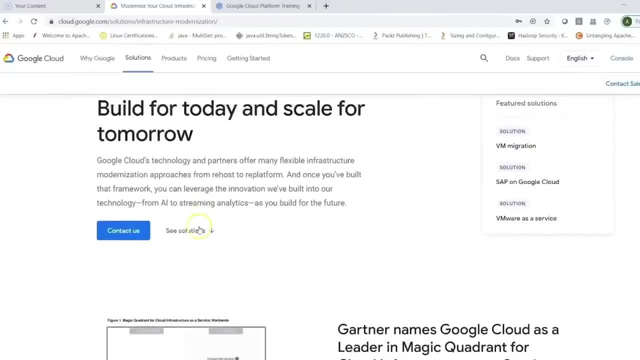 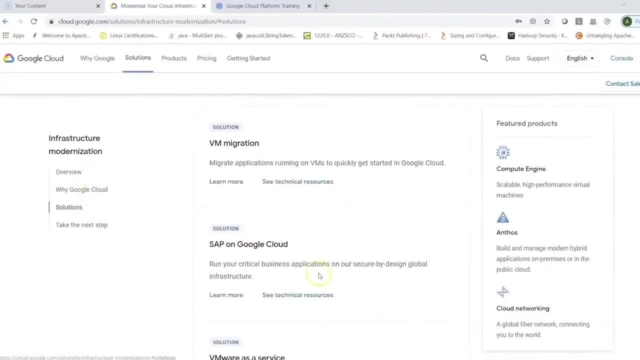 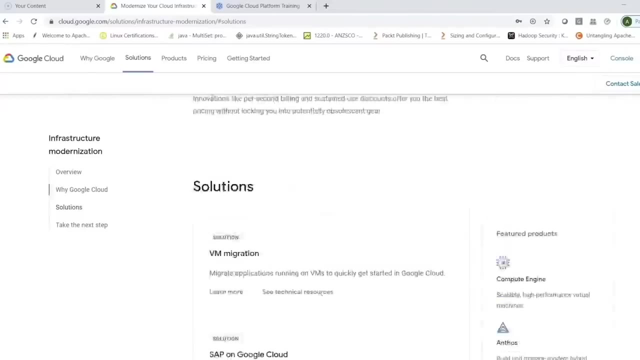 right when you talk about Google Cloud, so you can always click on see solutions and you can look at VM migration or SAP cloud right by Google Cloud, what it can be used for, VMware as a service or HPC- that is, high performance computing, and about these services we will learn. 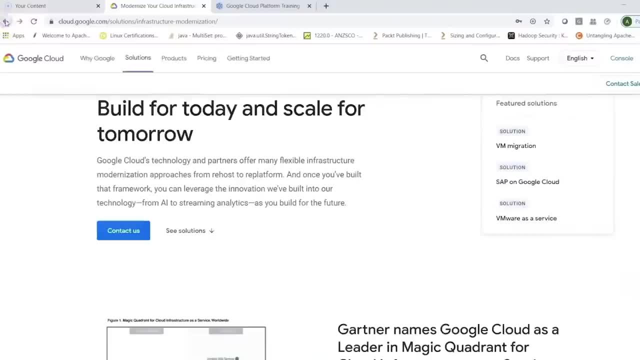 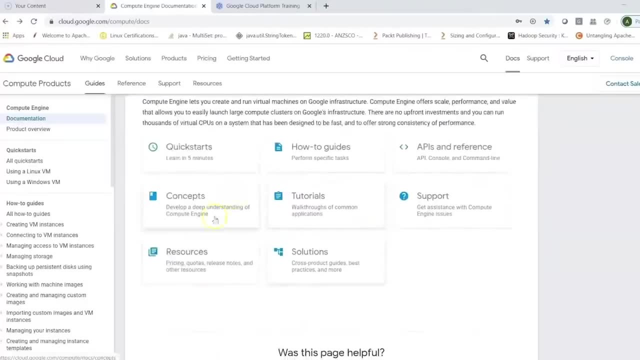 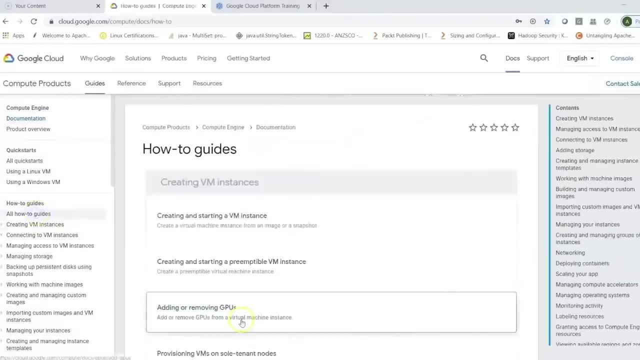 in detail later. now I can go back on the same page where I was clicking on the services. so you have quick starts, you have how-to guides, you have deep understanding of different concepts- right, and here I click on all how-to guides so that shows me what are the different ways in which you can work. 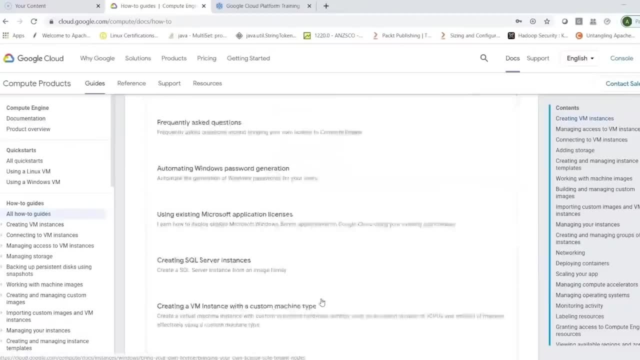 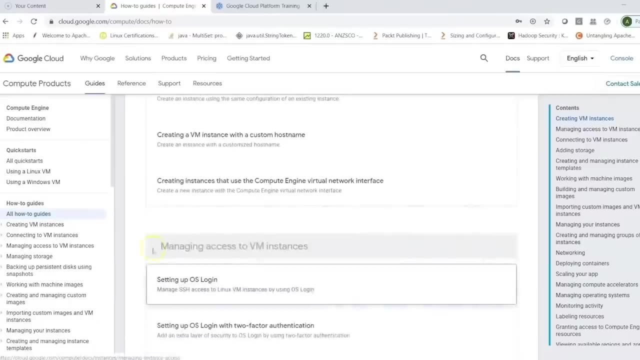 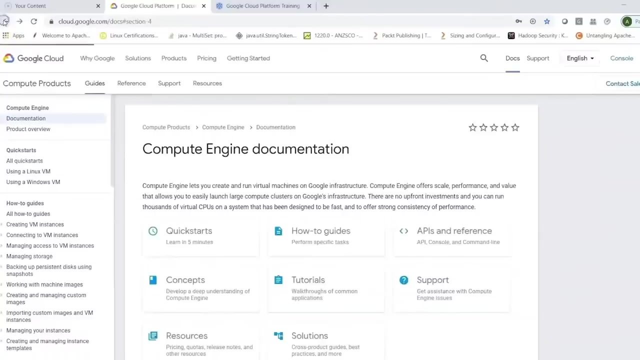 with compute engine and working with different instances, although it's quite exhaustive content, but then if you follow steadily, then you can learn a lot about Google Cloud. now here I can just go back, so this is just giving you some idea on the different products which are available from Google Cloud. looking into different sections, finding 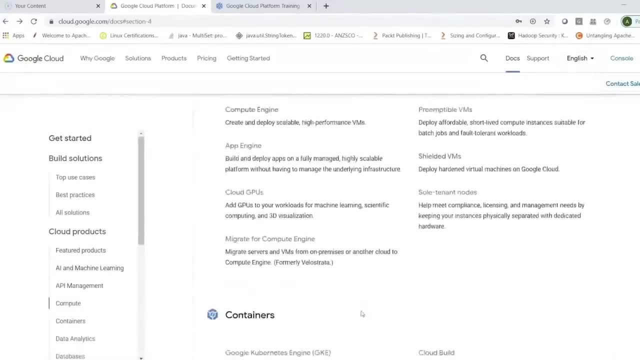 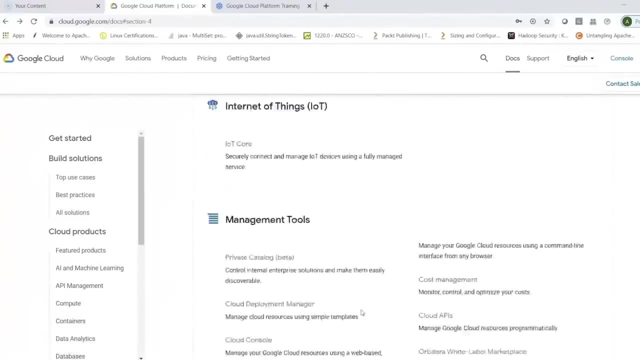 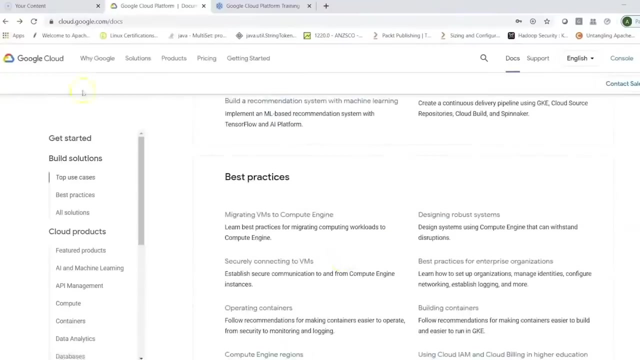 right documentation here. right, and you can always look into each one of these in detail for each product which Google Cloud offers. now, if we scroll down, we could see all the options or all the domains which we see here. right, let me just go back, because we got into 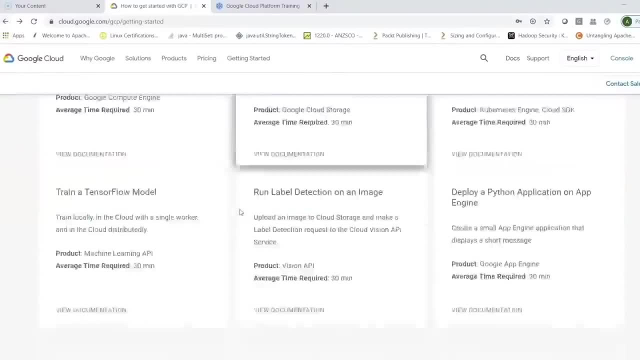 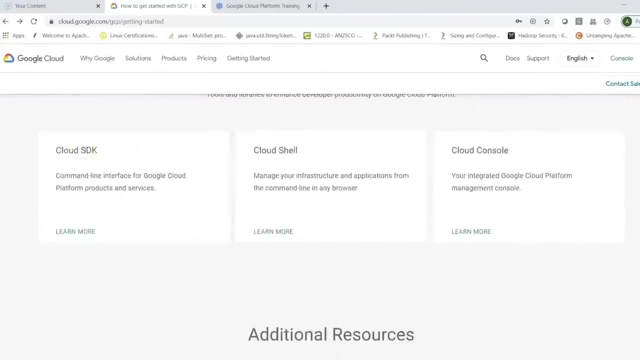 solutions. now we have quick starts right, and then you can basically scroll all the way down to look at all the different options. so, just like I said, we have quick starts right and then you can scroll down to a few of these options and then you can see the different options here. 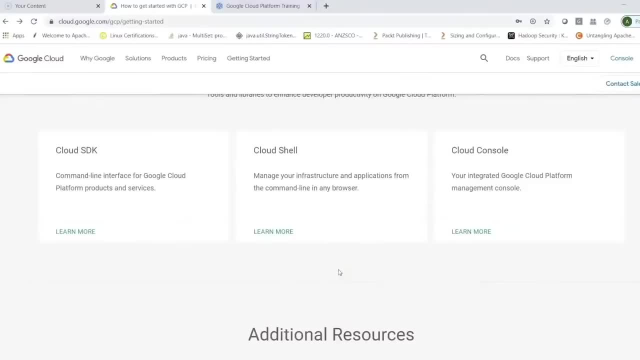 so you can choose the one you want to use. for example, you can choose your best option and then you can go back to your custom options, which can be set up on your Windows machine, like I have set it up on my Windows machine. plus, when you use Google console, you have a GUI which I'll show you in a couple of minutes and also a cloud shell where you can use your command line options to work with Google Cloud Platform. you have Cloud Console, which is nothing but your GUI, to access your resources. now you can also look at in-depth tutorials, pricing, and you have a website where you can look at your devices. you can also look at your products. you can also look at your products and you can also look at your sources. 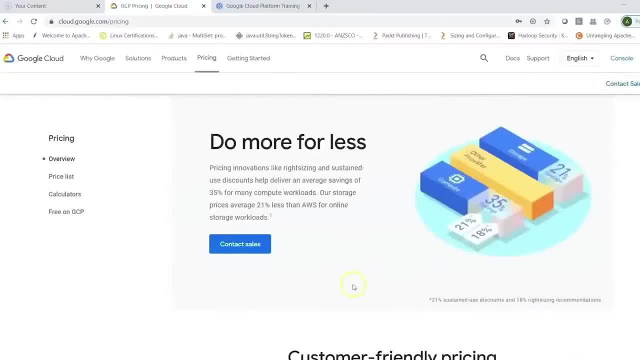 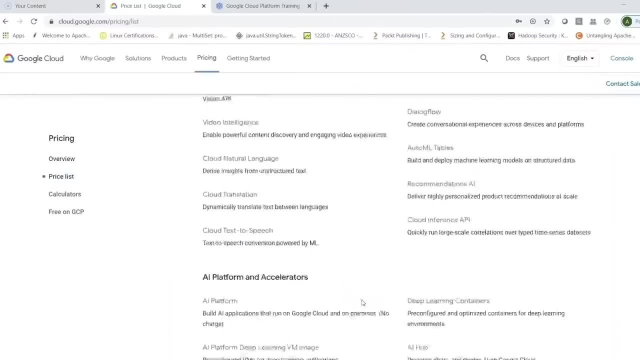 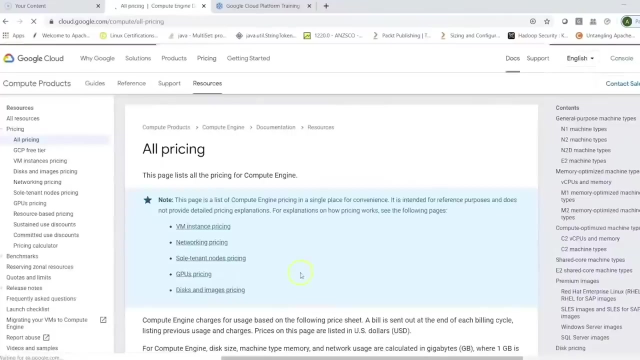 different other options. so let's just click on pricing here and then we have your price list which basically gives you details of different services: what are available and what are the services or what are the prices. so, for example, if I click on compute engine right and this shows me the pricing aspect of compute, 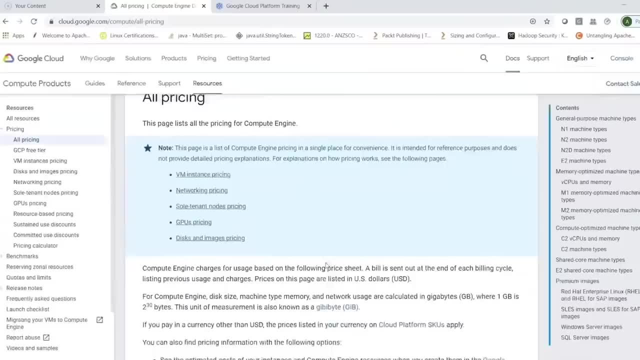 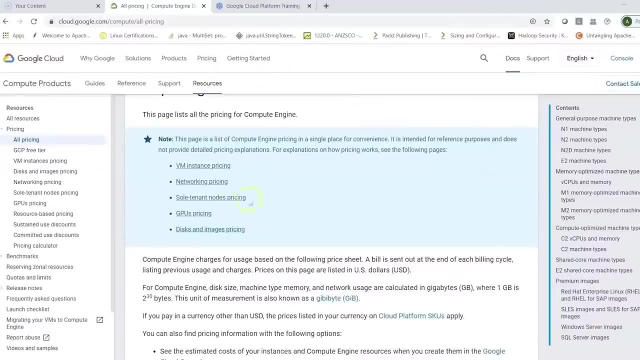 engine which belongs to compute domain, and here you can see, you have VM instance pricing. you have networking pricing, sole tenant nodes which are specific to particular organizations or if organizations would want to have dedicated nodes. you have GPU based pricing, right so general processing units. you have disk and image pricing and you can click on any of the links. 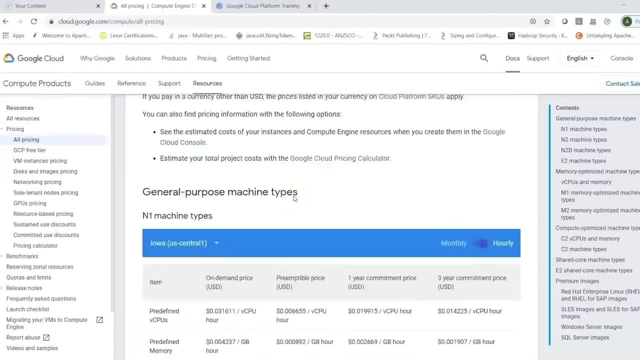 and you can see pricing which also shows you your different kind of machine types. so here you have different kind of machine types, which says n1, n2, n2d, e2. you have memory optimized machine types, you have compute optimized, you have premium images and you can basically look at all the categories. you can look at disk. 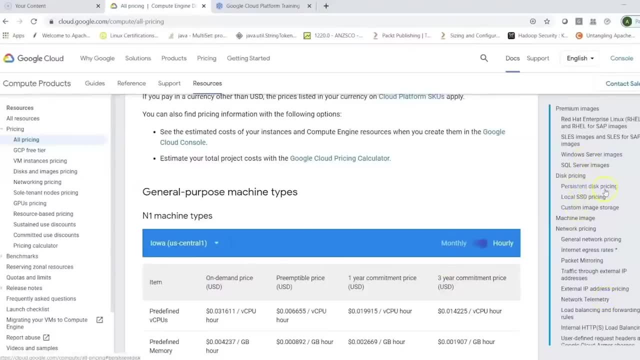 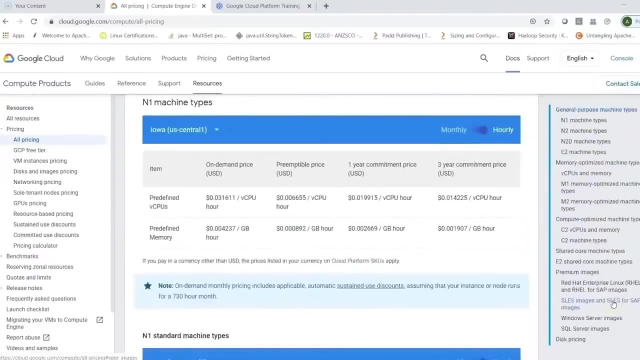 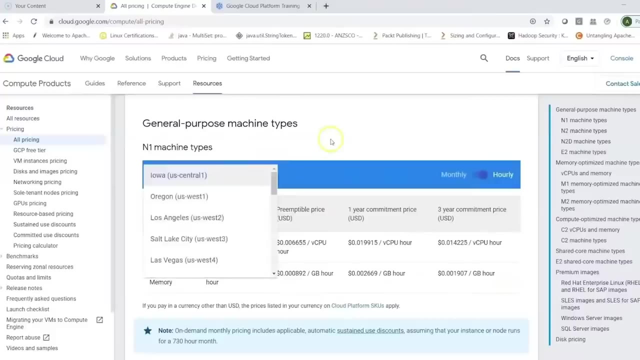 pricing, which involves your persistent disk pricing for SSDs or HDDs. what are the kind of images? what are the different network services? right, and you can always look at your machine types. you can choose a particular region. right. there is the concept of region and availability zones here, and I 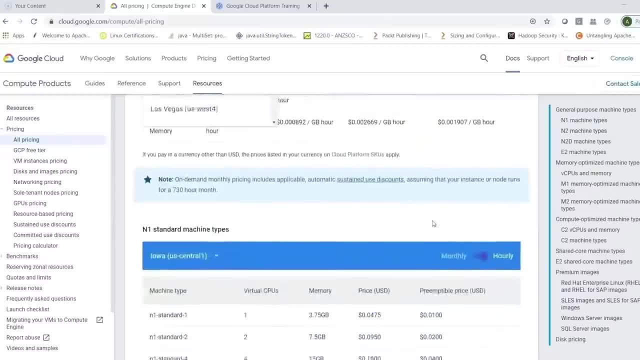 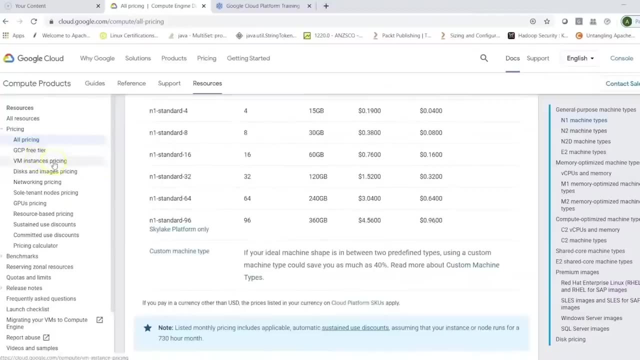 am going to show you how you can choose a particular region right, and you can also look at the prices. you can also look at standard prices. you could be looking for what are the free tier machines. if I am specifically looking for VM instance pricing, I can click on this one and that takes me to the VM. 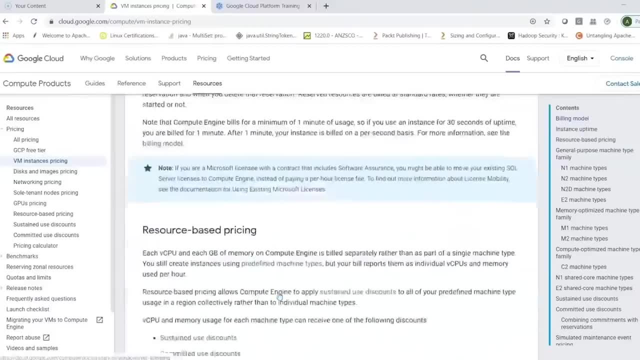 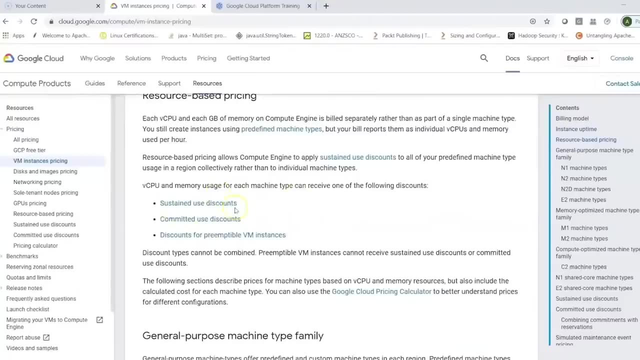 instance pricing. what is the billing module? what is the instance uptime, what is it? a source based pricing? and then you can also look at different kind of discounts, such as sustained use discounts, committed use discounts, discounts from preemptible VM instances and so on, and this is how you can be looking at pricing for all. 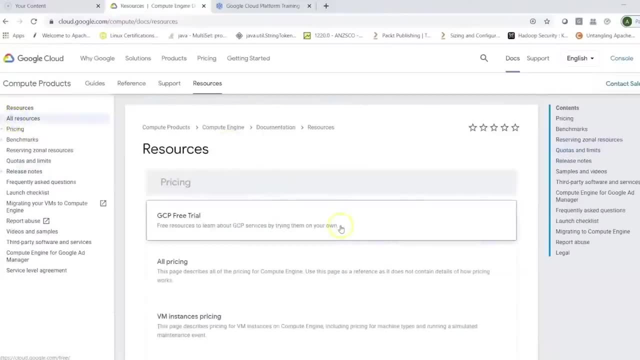 different resources and you can choose the resource which you are interested in and then look for the pricing, benchmarks, reservations, if you would want to use and you would want to benefit, if you would want to look at what are the quotas and limits, and so on. so please explore this link and you can. 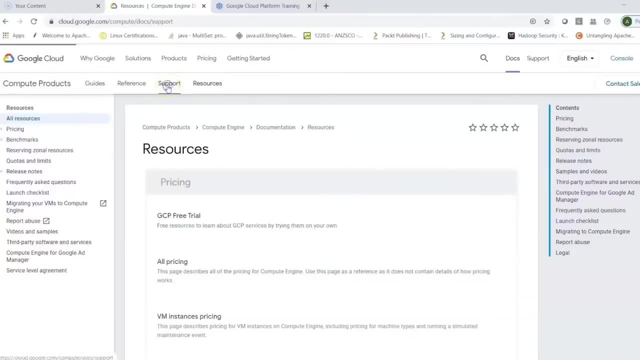 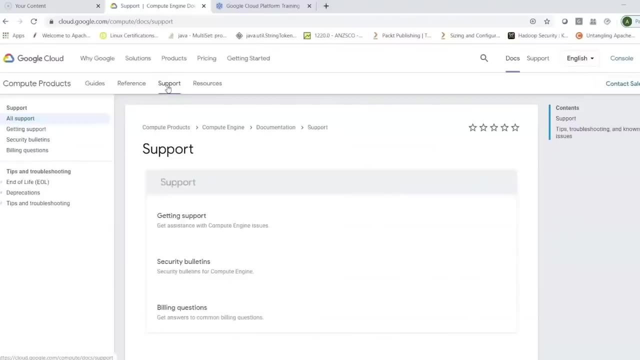 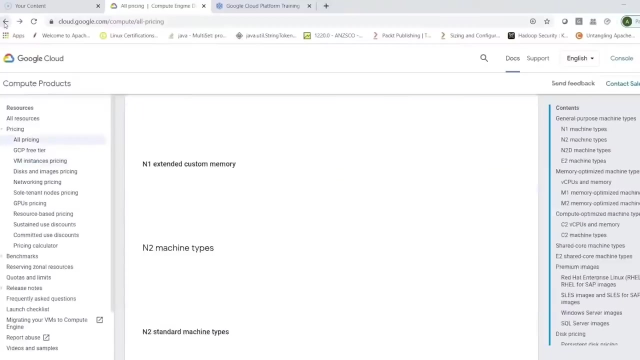 find a lot of information when it comes to technical options, looking at different Google Cloud products, which we briefly discussed, when it comes to domains and what each product can be used for. you can always come back to the main page where I was showing you different services. we went into pricing straight away. right now. you can always come back. 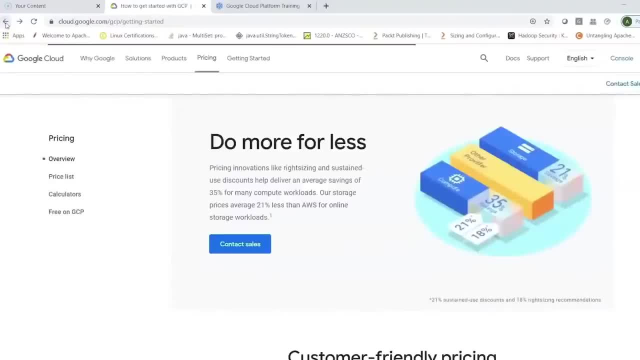 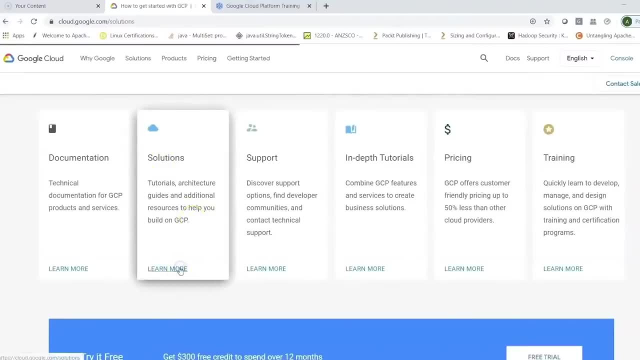 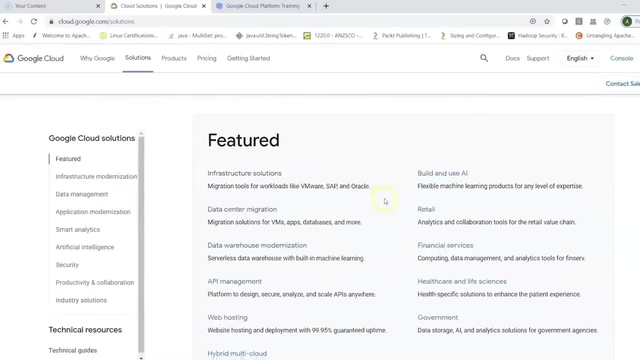 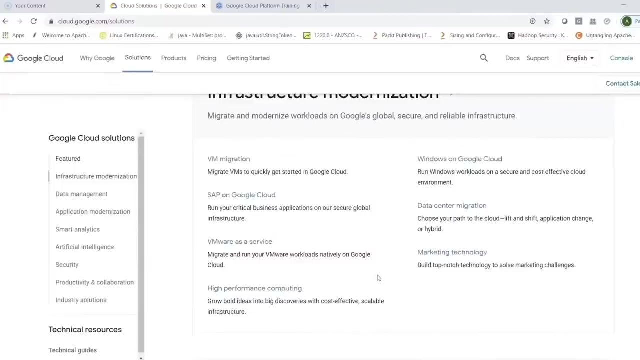 to this page on your cloudgooglecom and then you have your solutions, which talks about different products, right, and you can click on these or you can look into technical documentation. so this talks about your different features, solutions, infrastructure solutions. you have data center, migration related and so on. so I could be talking more and more about Google Cloud platform. it's a 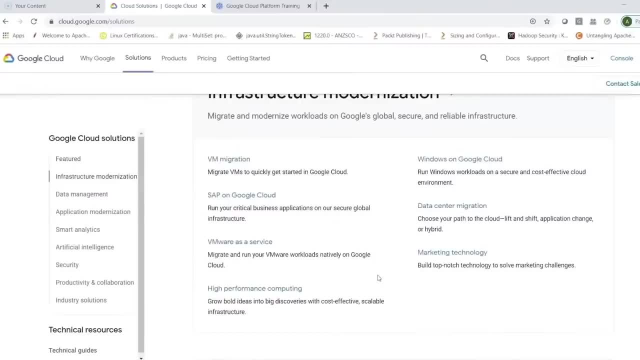 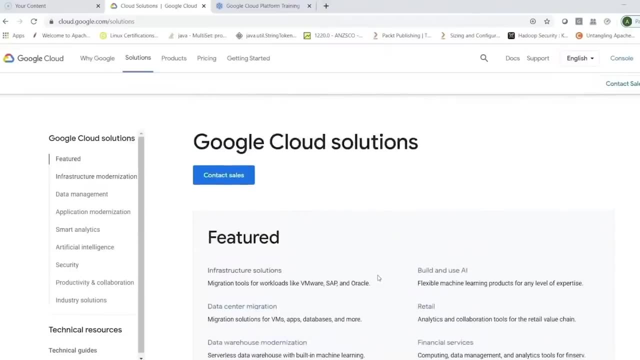 ocean. it's a huge chunk of different services for different organizational requirements. so look into this link and also, what you can do is create a account on Gmail. I mean you could create a free account, or you could go to cloudgooglecom and then you could create a free account like I have created here, and I can just 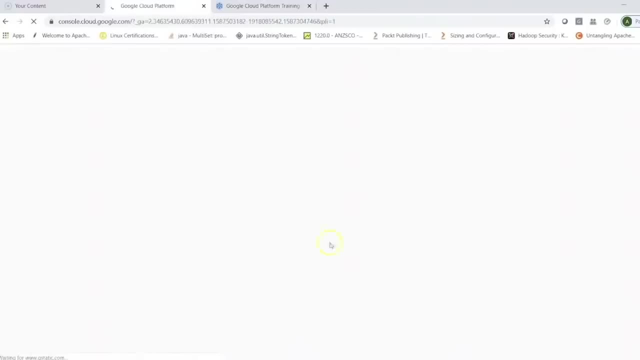 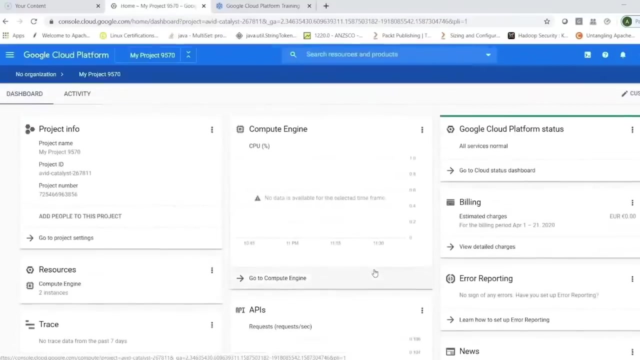 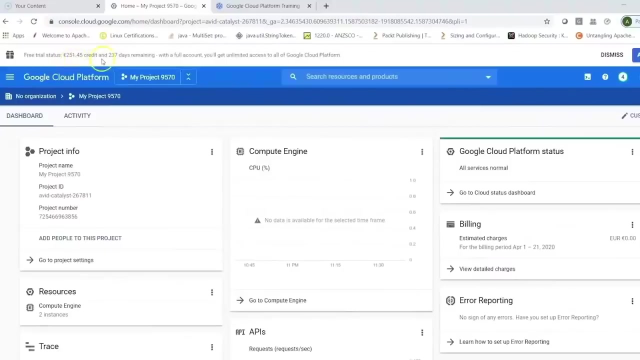 click on console- now that's my GUI, or Google Cloud console, which basically allows me to work with Google Cloud. now there are a lot of options here by default when you create an account. now, in my case, on the top it says it's a free trial account. I have three hundred dollars credit and out of that, two fifty. 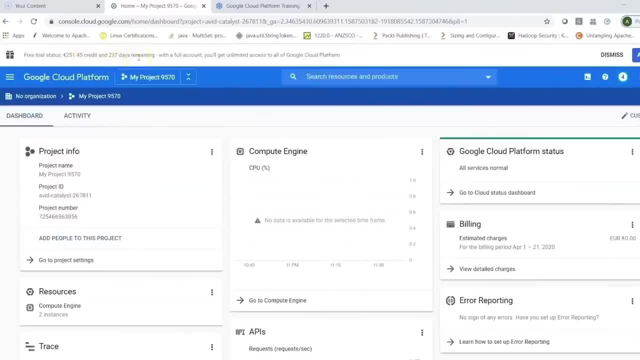 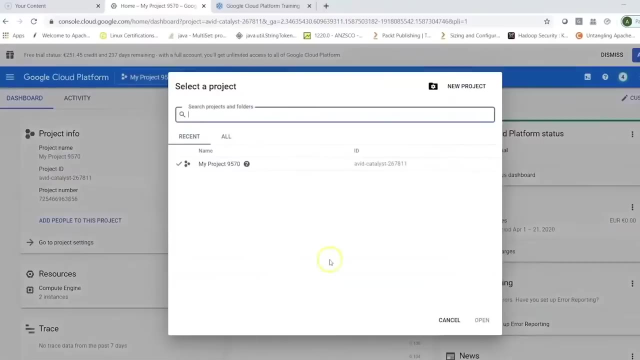 one dollars is left and two thirty seven days out of a year are left for my account. now here I can basically see the project right and by default we can create and project, or by default there is a project existing for any user, so when you log in, it creates a particular project and you could create a new. 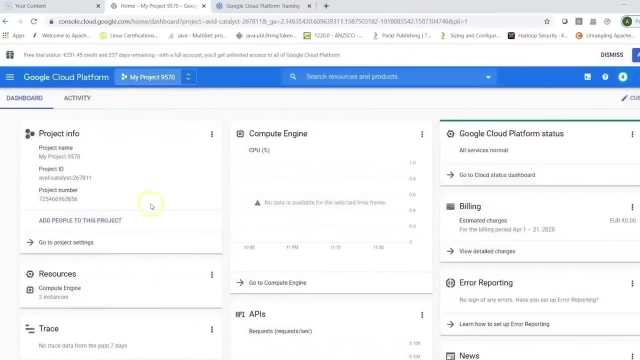 project, and project would be to dedicate your different services or different resources for different project. so this is your dashboard, which basically shows your project, which shows you a project number and a project ID which is always unique. now you can click on this and this. if you would want, you can hide this information. you can also look into the 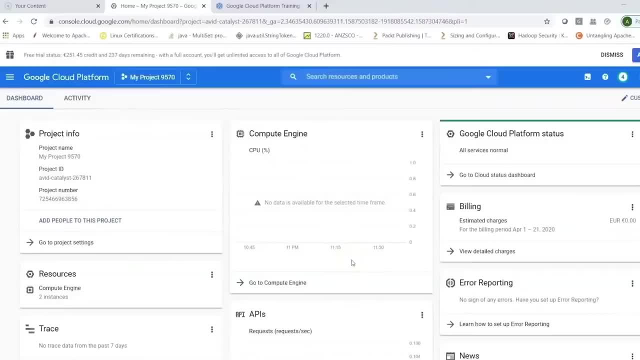 documentation part of it. then it shows you the different services or a graphical information of services which you might have used in past. so you have Compute Engine, which shows you how much percentage of CPU was used. you can always go to Compute Engine as a service. you can look at your Google Cloud. 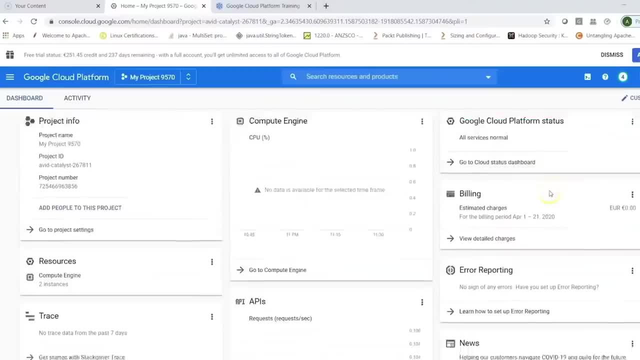 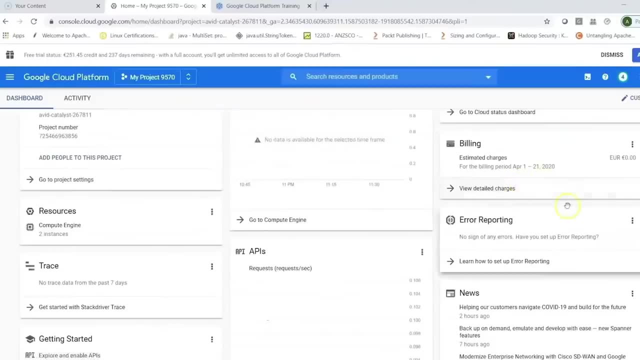 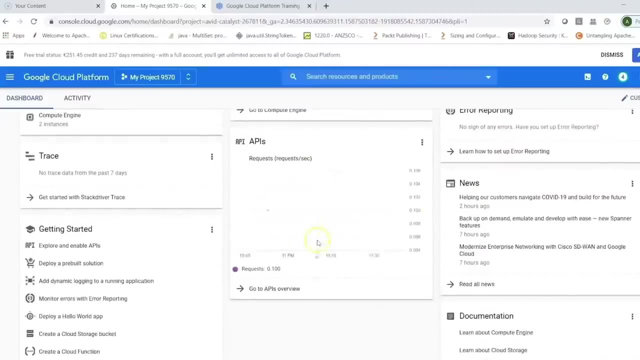 platform status and look at the Google Cloud status. now this is billing now, since this shows me the billing period for April month and I can always look at detailed charges. I can look at reporting. I can look at different API's which Google offers and for your different kind of work, you can always go to the API overview or the API. 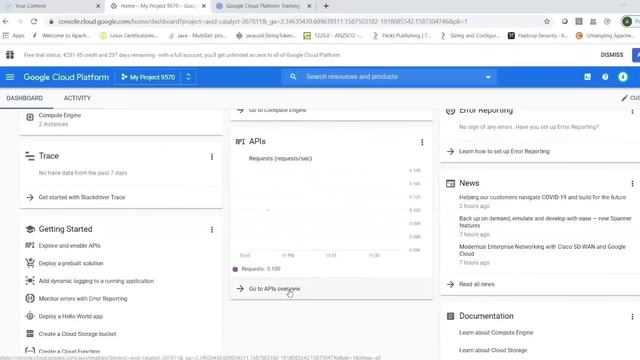 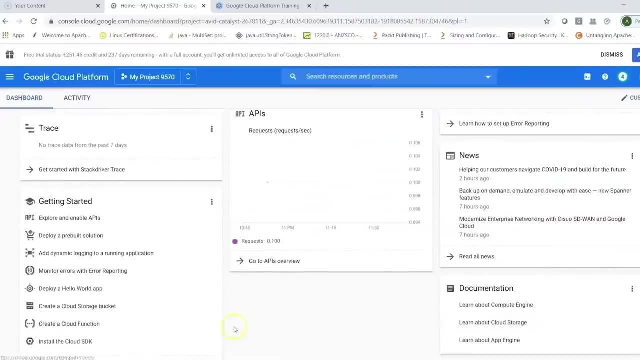 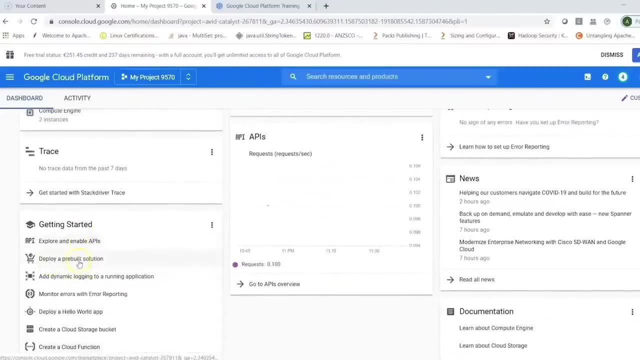 link and enable or disable any API. now, once you enable or disable any API, then you can use that. so you have new section, you have documentation and you have getting started guides which tells you how to work or enable different API's if you would want to deploy a pre-built solution at dynamic logging monitoring. 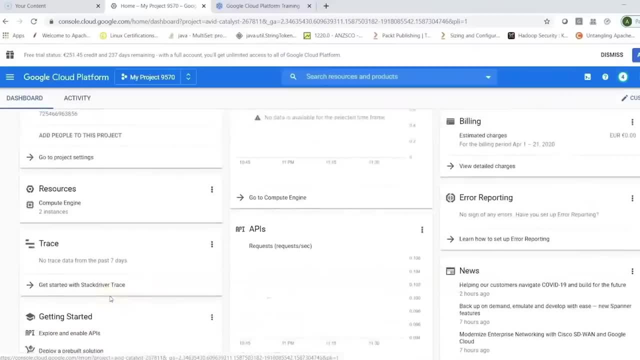 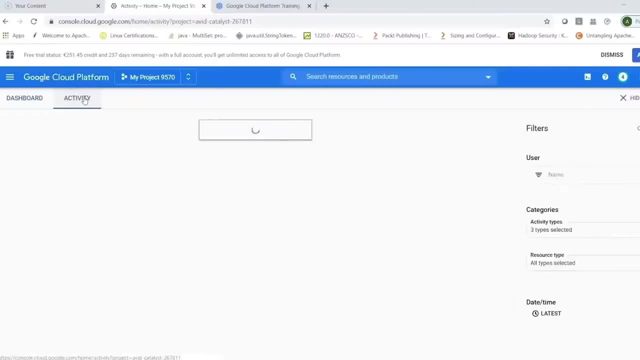 errors, deploying a hello world app, and so on. now this is your dashboard. I can click on activity and that would show me what kind of activity I would have done in my cloud platform. I can always choose the kind of activities by saying activity type. I can choose the resources. now it shows me that I 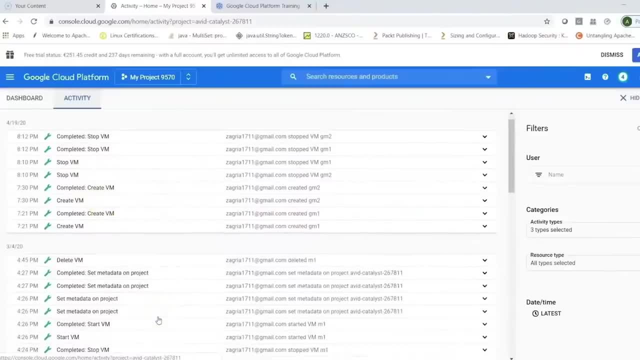 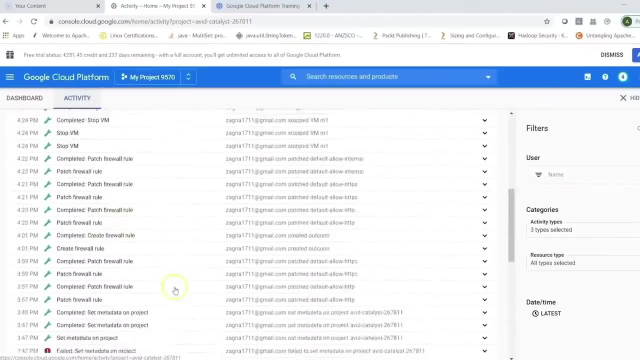 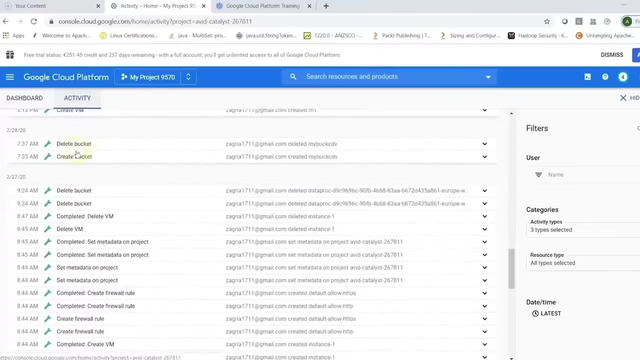 created some VM instances, I deleted them, I updated some meta data. I basically worked on instances. I change some firewall rules here. I have then also worked on some other services or API. so I created some buckets, which is for object storage, and again I have been working with some playing in instances. 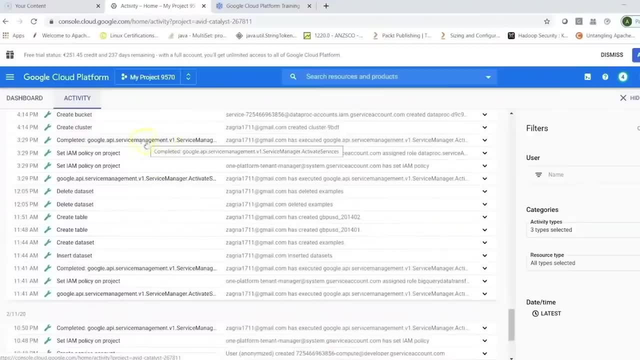 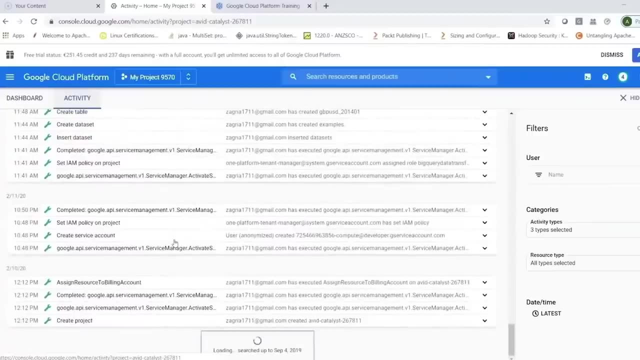 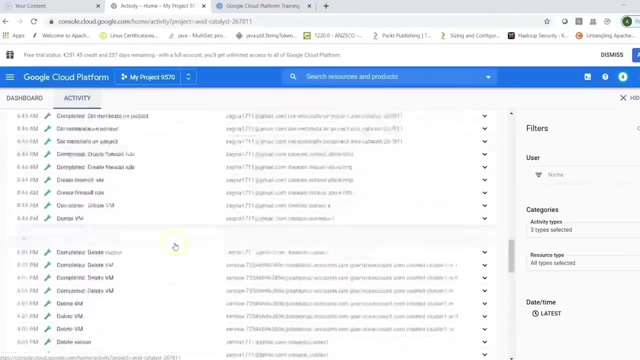 and creating some firewall rules. here I have granted some permissions. I am setting up a policy right, so this activity gives me a history of what things I have done over the past couple of months while working on Google Cloud Platform. Now on the top left corner, you have the hamburger menu, which you can click. 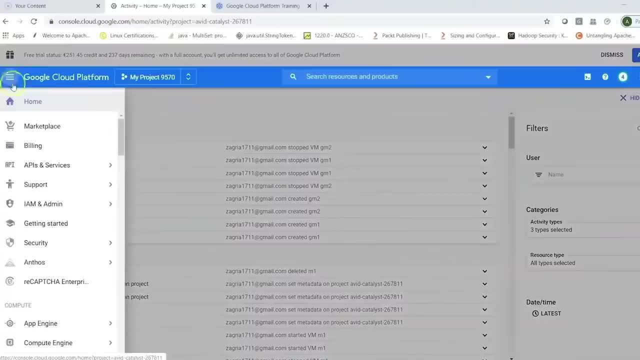 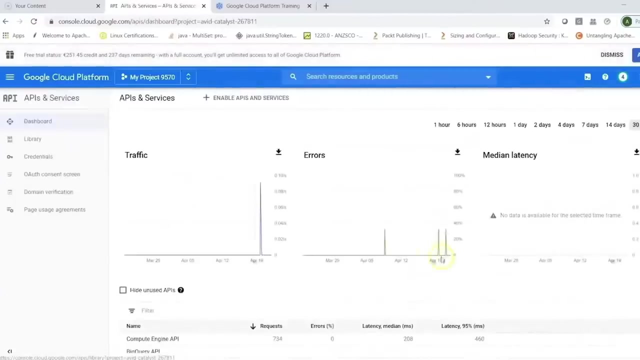 on this, so that's your navigation menu and when you click on this, this shows you home. it takes you to the marketplace. it specifically takes you to billing. you can always look at APIs and services. so here in API services, I can pretty much go to a dashboard and I can see a report. 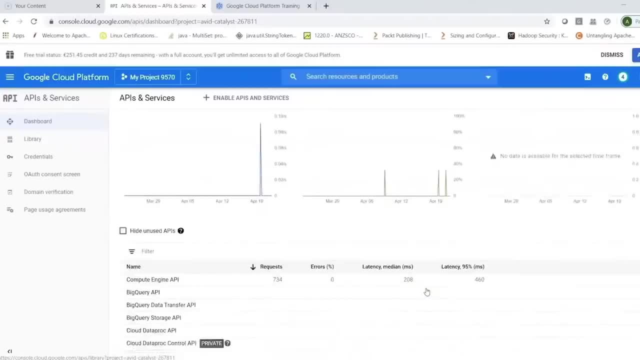 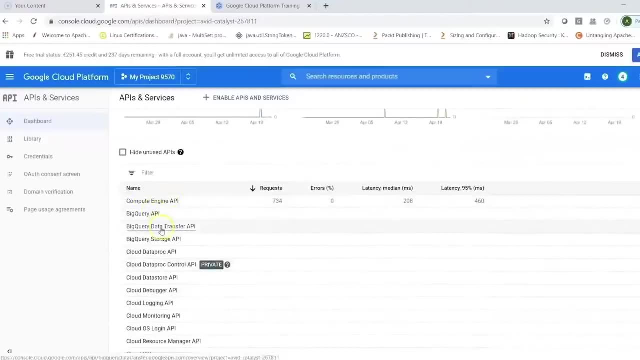 on the traffic or errors or latency and the kind of APIs which are available. so you have compute engine API, you have BigQuery API, BigQuery data transfer API, BigQuery storage, Cloud, Dataproc. so these are some of the APIs or services I've used in past. 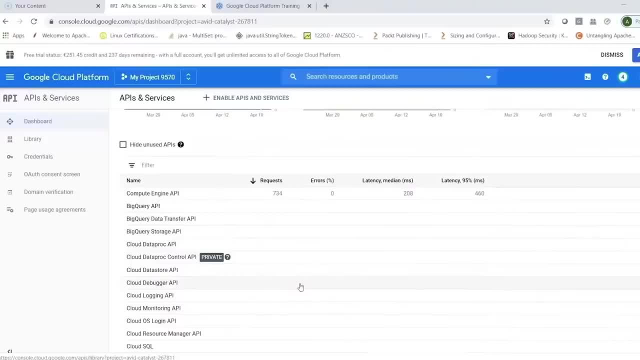 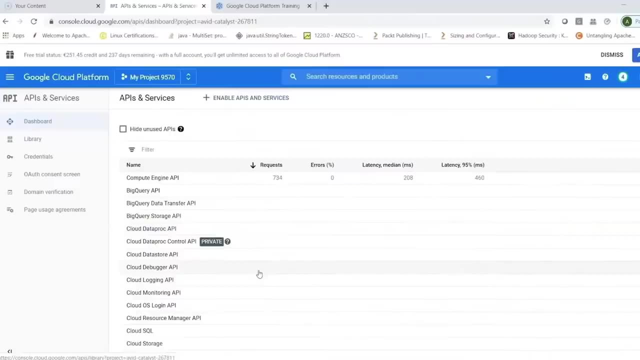 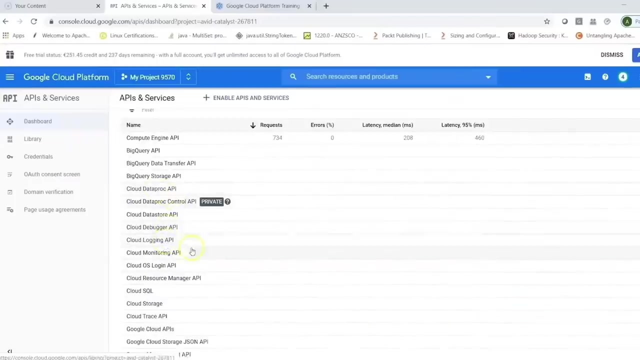 Might be I was evaluating a product. might be I was using a particular product. so you have. whenever you would want to use a particular service from Google Cloud Platform, you would be enabling these APIs. so here we see some APIs for Dataproc. you have logging, monitoring, you have resource manager. 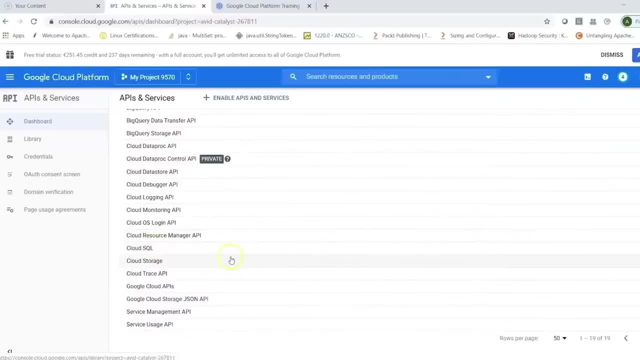 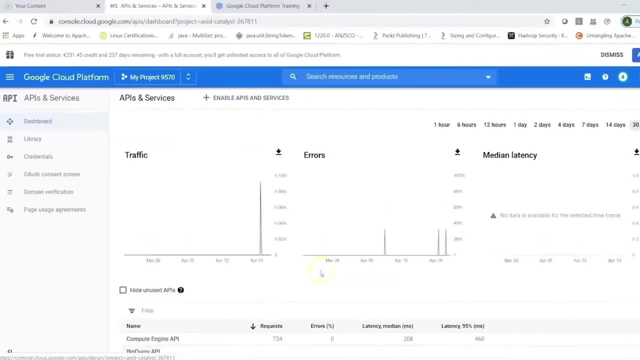 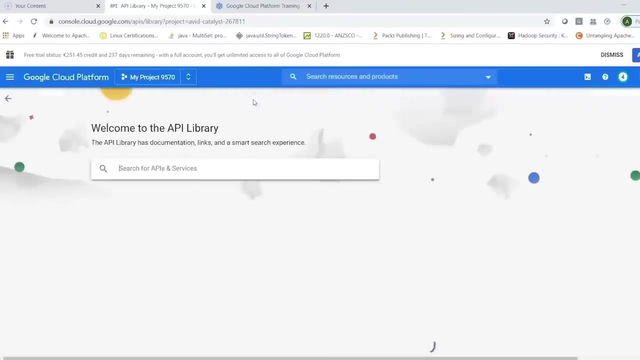 API. you have cloud SQL, which allows you to directly use MySQL or Postgres, you have cloud storage right and so many APIs. So if I would want to enable a particular API which is not right now required, but then it's good to know, you can always click on this one, you can search for an API. so, for example, if I would say: 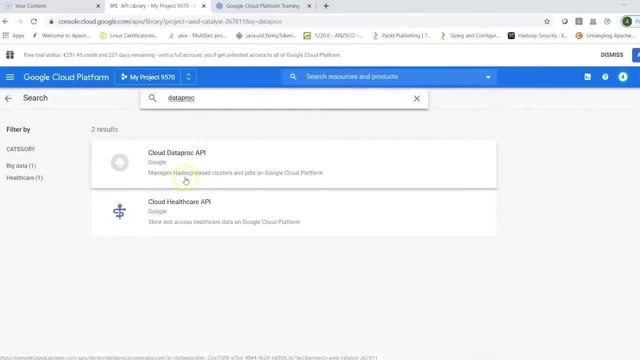 Dataproc right, and that shows me the cloud Dataproc API, which manages Hadoop based clusters and jobs on Google Cloud Platform. so I can spin up a Hadoop cluster and I can start running some jobs on a Hadoop cluster on demand and, as I'm done with it, I can just get rid of it. 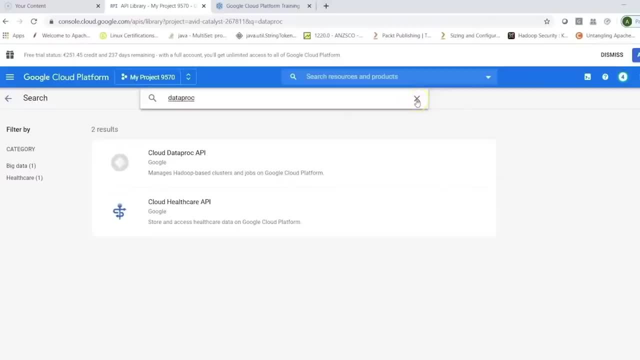 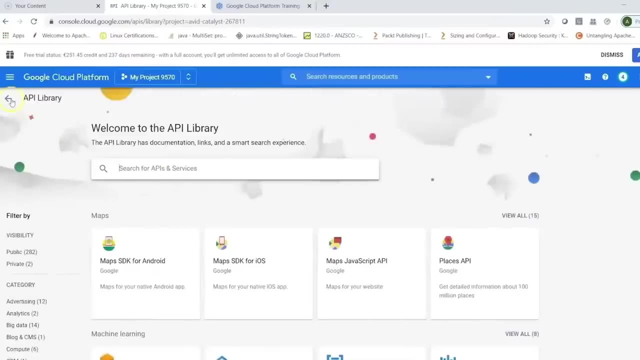 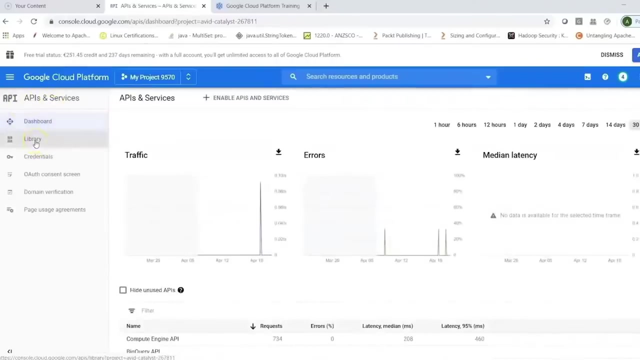 So this is an API which I would have to enable and then for every particular service, you also have an admin API which you would enable. Now, going back, so coming out from this API library, I got into API and services. Now there is, you can look into the library, you can look at credentials and you can also look at 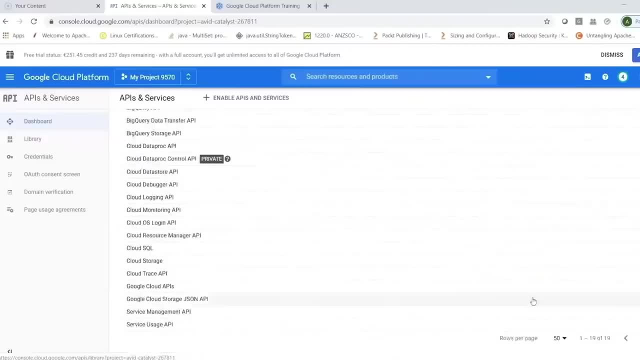 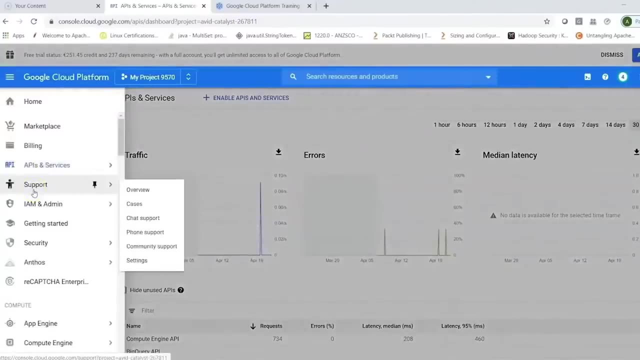 different time intervals for which you can see the usage of your different APIs. Now, going back to the menu, You have support, wherein you can always reach out to the Google support team. If you are using a paid version, even with free trial, you can try to reach out and you will find. 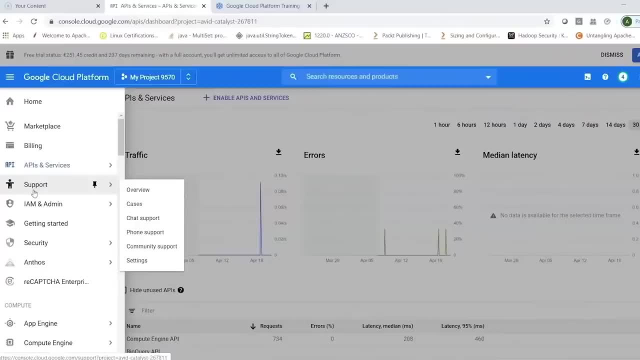 someone to help, but it is always good when you have a billing cycle reaching out the customer care. You have identity access, management and admin and this is required when you are working with different APIs or services when you would want to have relevant access. You have getting started. 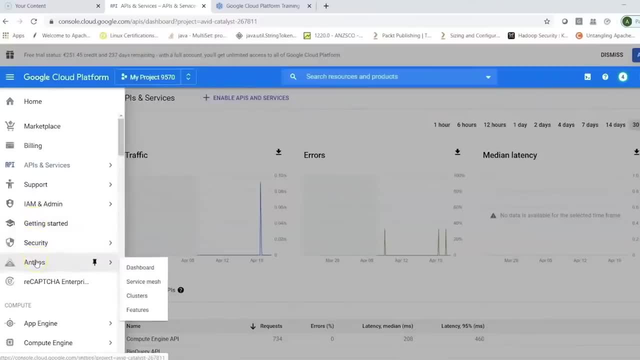 You have Security related options. you have Anthos, which is mainly for migration. Now, here you can look at your different domains, such as which we discussed. so you have compute and in compute, you have different services. so you have app engine, you have compute engine, Kubernetes, you have cloud functions and cloud run. you can look into the storage aspect, which 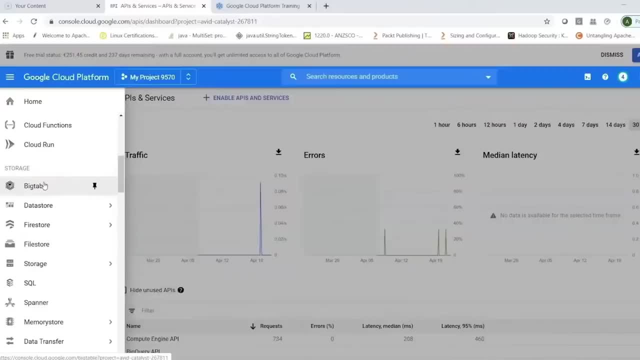 shows you big table, which is usually and mainly for your unstructured data, big table which is something which gave rise to Popular no SQL databases like HBase and Cassandra. you have data store which can be used. you have fire store, file store storage which can be used to put in data of any kinds you have. 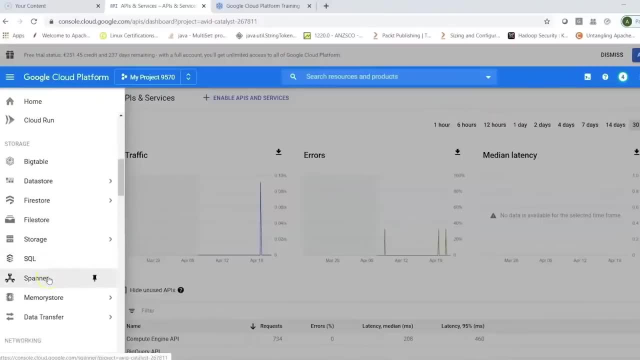 SQL for structured data. you have spanner as a service, you have memory store and you have data transfer. Now, when it comes to the networking domain, you have all these services, such as VPC, virtual private network, Network related Related services for your load balancing, for using a cloud based DNS or cloud defined network. 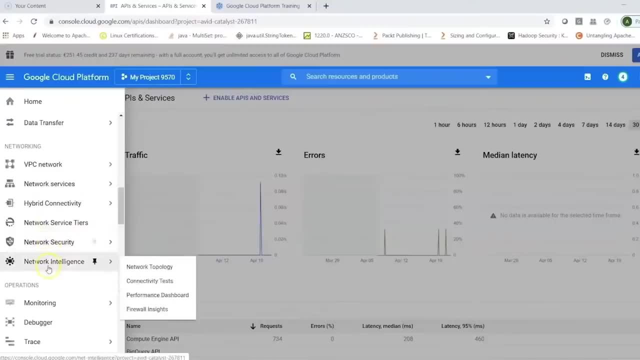 You have hybrid connectivity, network service, tiers, security and intelligence. Then you have other options for your operations which can be used, and here you have different other tools which can be used, such as cloud build. You have cloud tasks, containers, registry, deployment manager and many more big data specific. 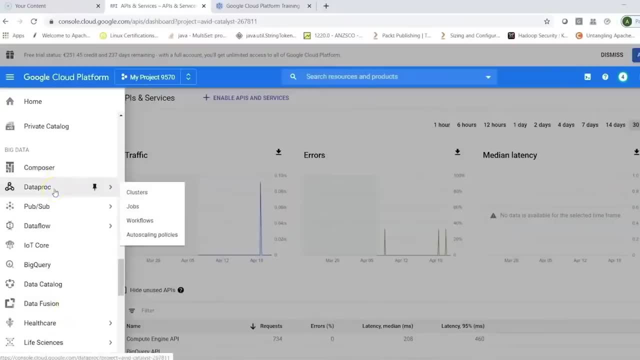 You have the services here, So you have data proc, which can be used to spin up your clusters. you have published subscribe messaging systems such as now Kafka, which you might have heard of, originates its idea from here, So pub sub. you have data flow. you have IOT core BigQuery, which is a data warehouse package. 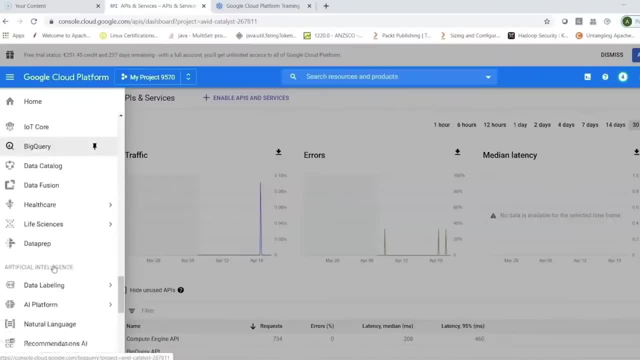 or data warehousing solution from Google Cloud. Now then you have your artificial intelligence related services and other Google solutions, So you can always find a huge list of services. So you can always find a huge list of services- Or you can say, at high level solutions offered by Google Cloud and we can use these to basically. 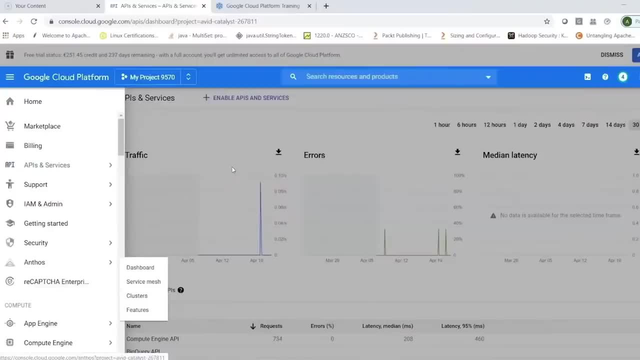 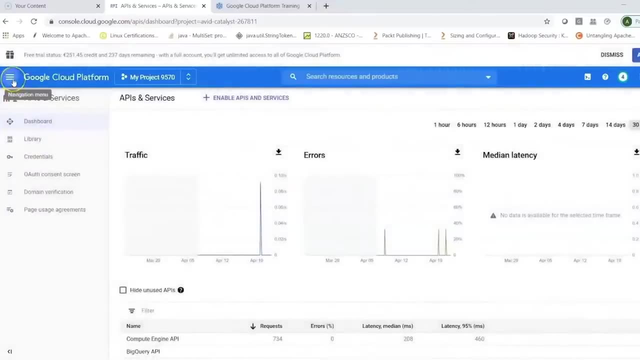 test some of the solutions, use them and work on them. So I'll give you a quick demo on different services which can be used here from your Google Cloud platform. Now, this is your Google Cloud platform and this is your console. Now, this also gives you a cloud shell which can be activated. 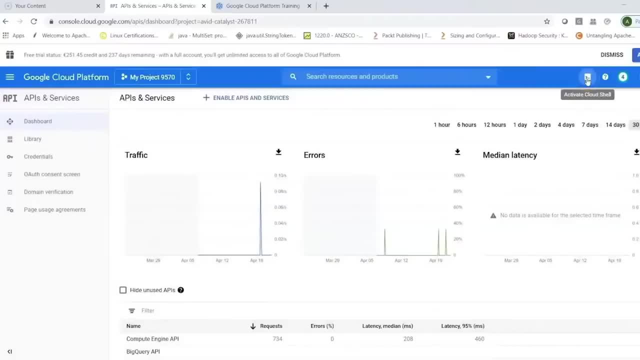 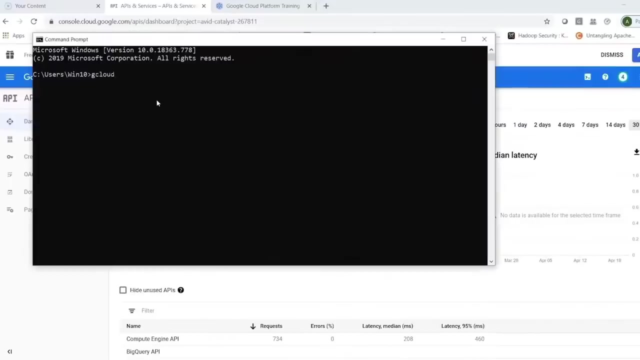 So that you can work from command line, and you can always find a lot of documentation on that. So you can also set up your cloud shell, that is, SDK, on your Windows machine And if you have set it up, then basically you could be doing something like G cloud, right. 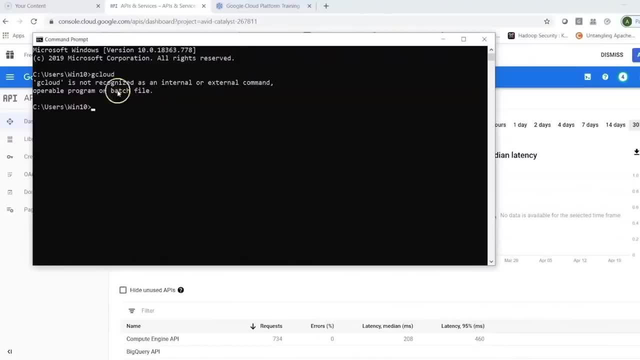 If the cloud has been set up. So in my case I had set up the cloud SDK and basically I can get into that by looking at what path. I have set up Cloud SDK and then I can be using it from my Windows machine as per my comfort. 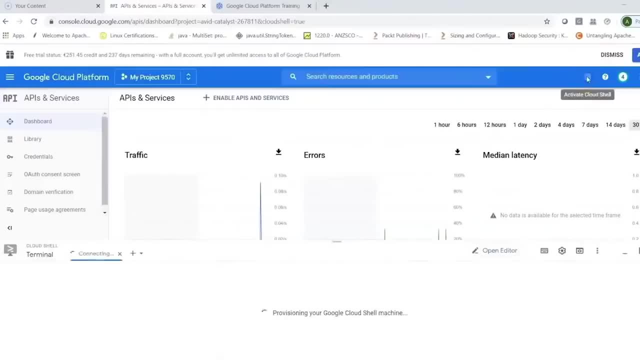 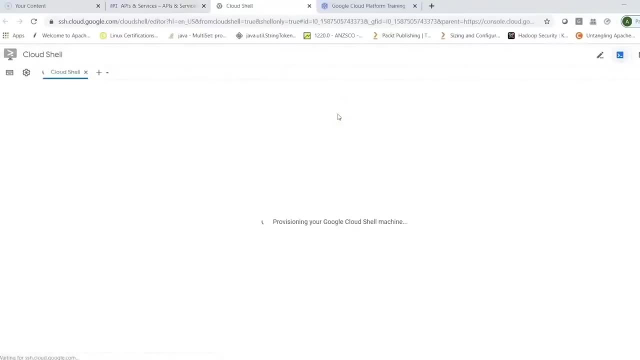 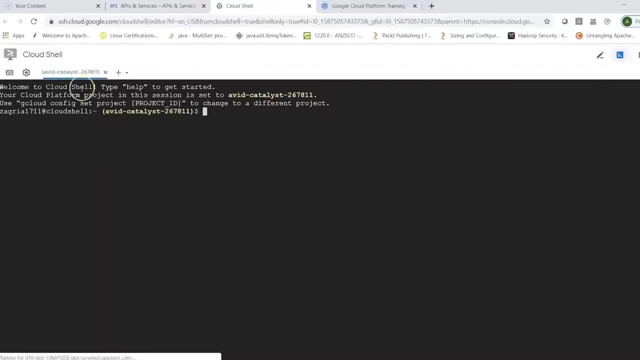 I can also activate the cloud shell here, which will basically open up a terminal and at any point of time you can open up this one cloud shell in a different window. It is preparing the cloud shell where it will, by default, set up your project. It will set up the metadata and now I am logged into my Google Cloud account from command. 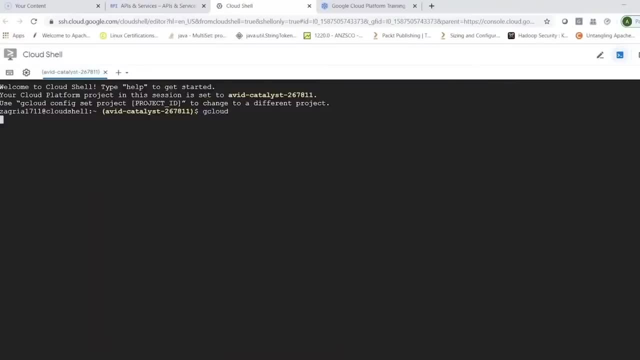 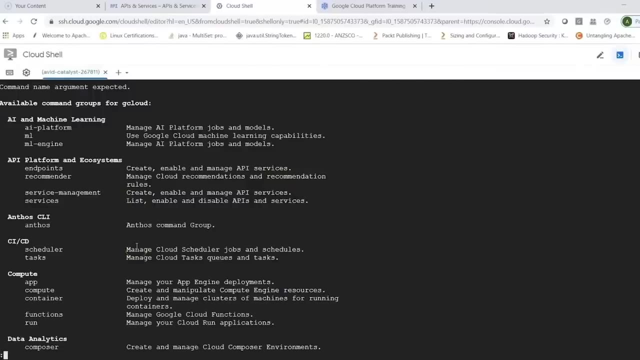 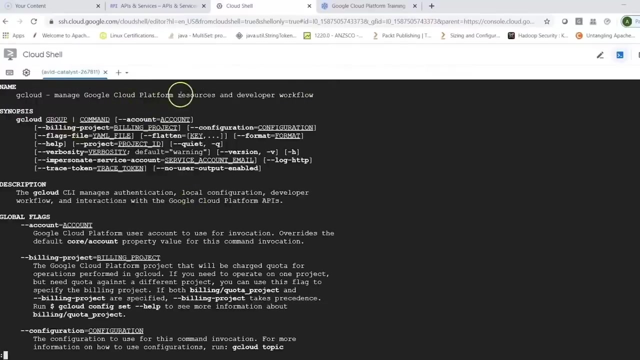 line, And here I can basically use G cloud Right and that basically shows you the different options which are available which you can be using. So if you would want to use a particular service, you can also try giving a help and that shows you how do you manage your Google Cloud platform right. 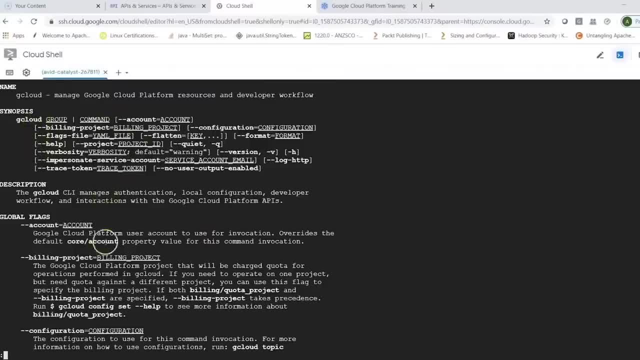 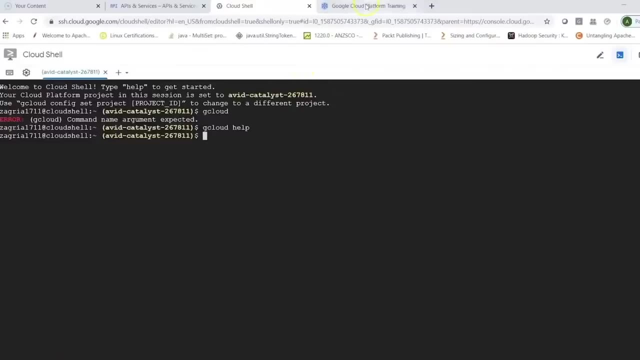 So you have different options for billing to work with your different services and basically you could be working on Google Cloud using this cloud shell from your command line. Usually, for people who are learning Google Cloud in the beginning, it is always good to go for console and use your different. 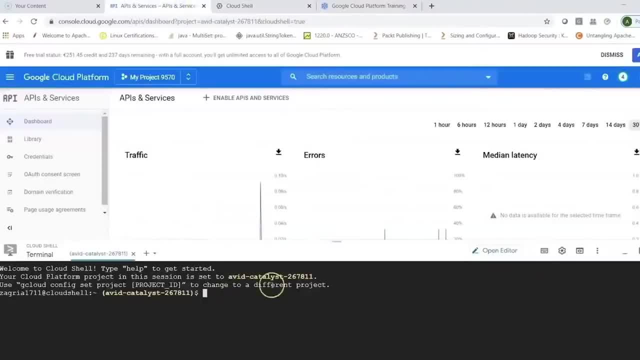 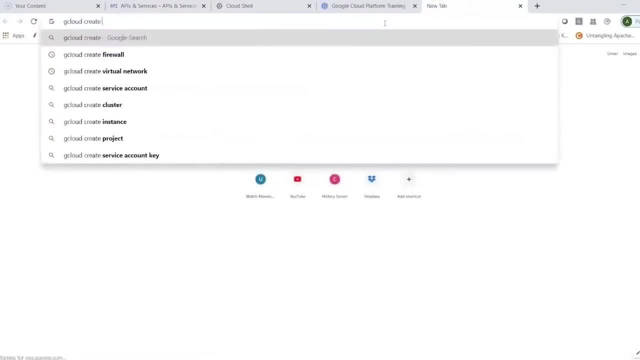 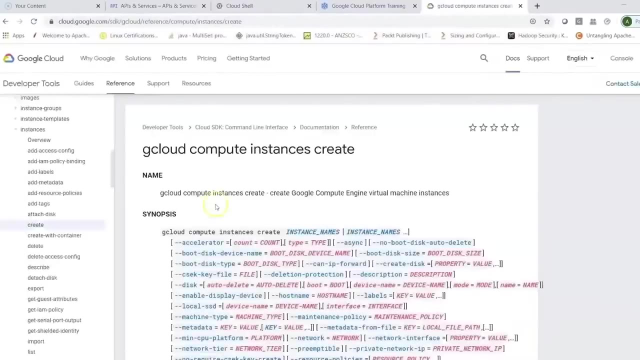 services from here in an easier way. But, as I said, you can always use the command line. For example, if I would just go ahead and type G- cloud, create instances, and that will directly take me to a cloud console documentation which shows you different options which you can. 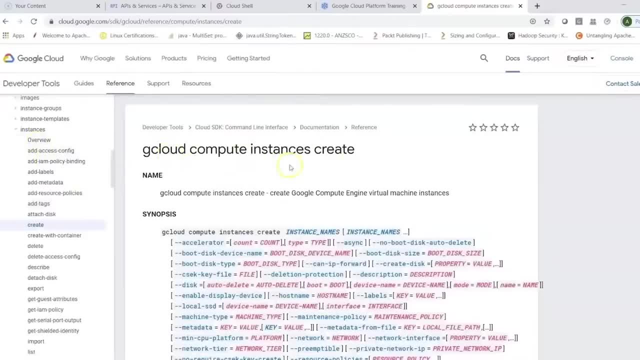 use to work with instances. So I could do a G cloud Mute, instances create and then I can give my instance name and so on, and I'll show you some examples on that. So you can be using your cloud console, right, that is your cloud shell and you can straight. 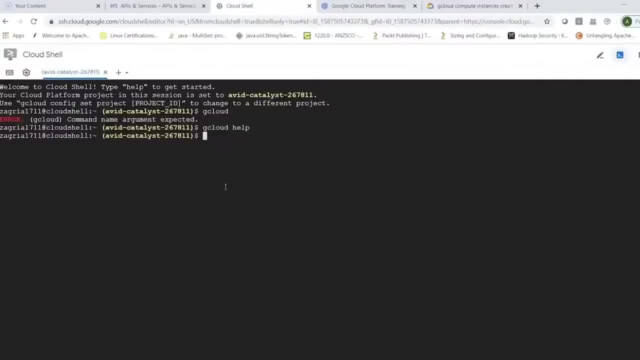 away start working from command line. However, I would suggest using console in the beginning, and when you are well experienced then you can start using cloud shell to do things from command line, and when you are fully experienced you can always switch and certain things are usually useful or easier. 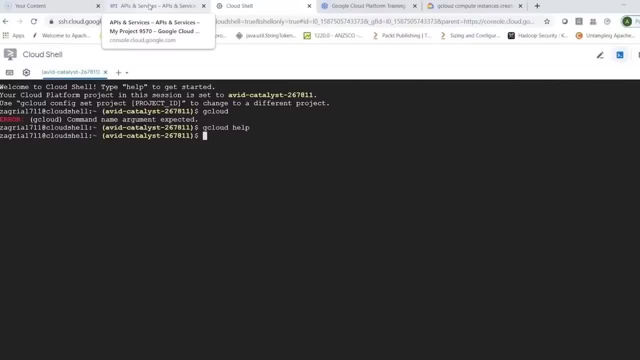 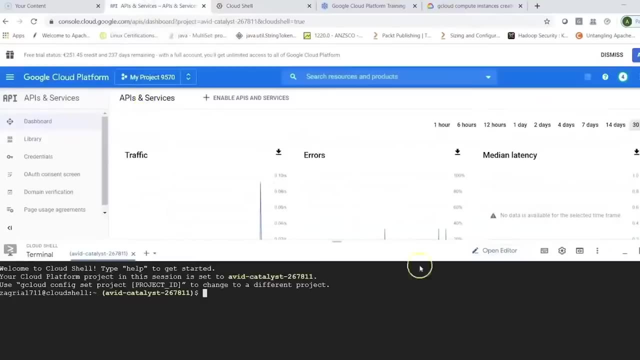 when done from command line, and some are easier when you do it from the console, and you can use any one of these options. Now we can go to Google Cloud console. now, as of now, I can close this one. I still have my cloud shell open, if I would want to look into it. 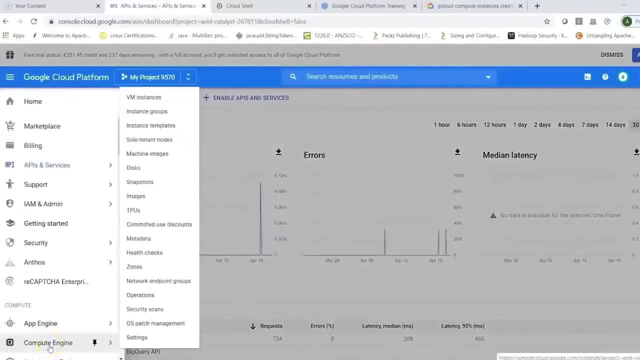 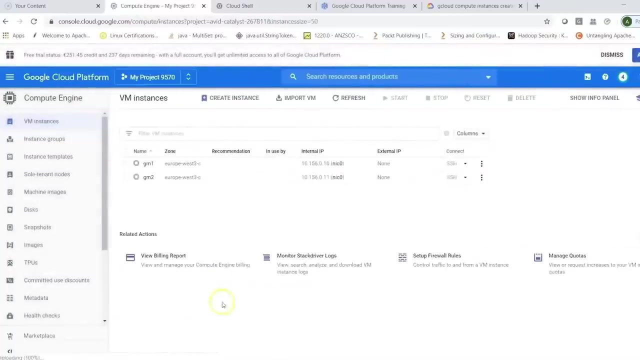 I can click on this one and I can straight away go to compute engine, where I would want to work on creating some instances on Google Cloud platform using the compute engine service and then basically connecting to those instances and basically trying out some basic things. So you can click on VM instances and then, once this comes up, I can always create some. 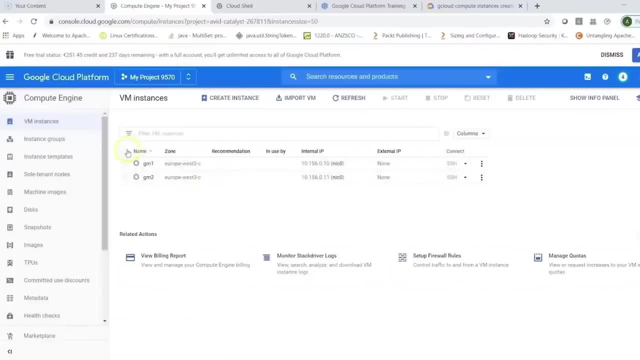 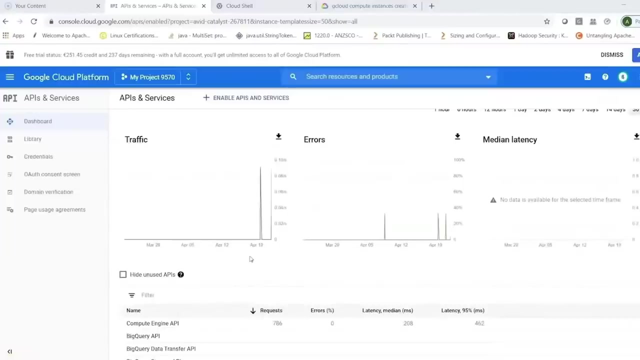 instances. Now, if you see here I have some instances already created, right, and I can continue working on those. I can create new instances. I can use different options while creating instances and I'll show you that in a demo in quick seconds. So let's have a quick demo. 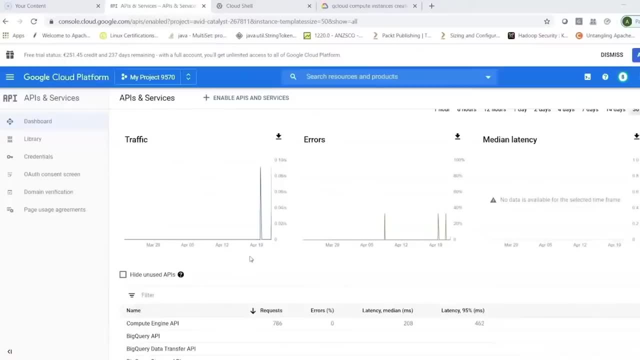 Let's have a quick demo on setting up GCP instances Now. before that, let's have a quick recap. So when you talk about instance or a virtual machine, it is hosted on Google's infrastructure, right, And you can create your Google Cloud instance using this Google Cloud console, that is, by. 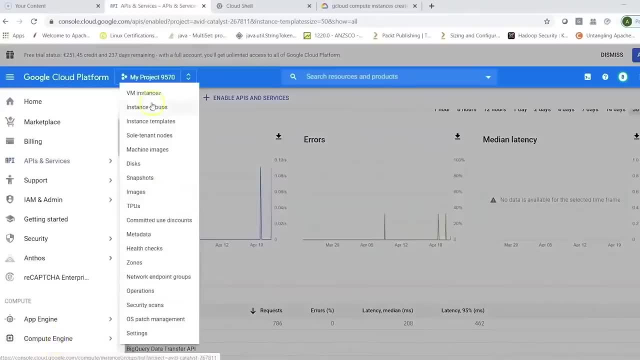 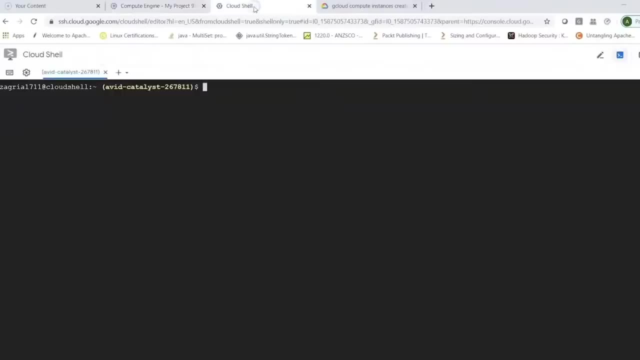 clicking on this and then going to compute engine and clicking on VM instances. Now you can also do that from Google Cloud command line. You can also do that from Google Cloud command line tool, that is Cloud Shell, and you can be doing that using compute engine API. 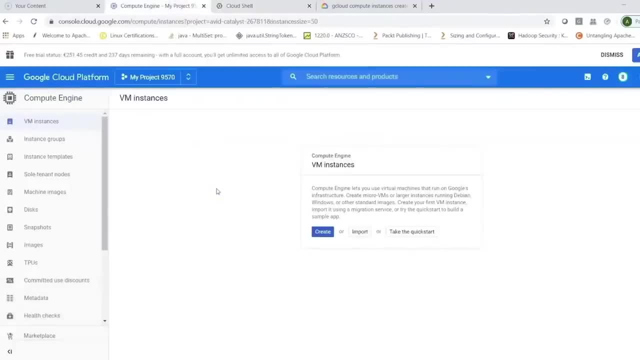 So compute engine instances can run the public images for Linux or Windows servers that Google provides. You also have option of creating or using custom images that you can create and import from your existing systems. You can deploy Docker containers which are automatically launched on instance running. 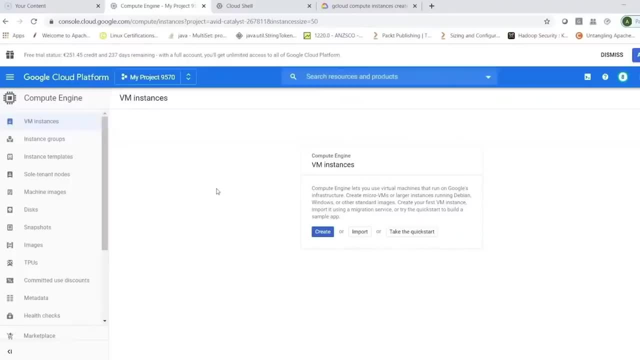 containers. Now, when you talk about instances and projects, always remember that in each instance belongs to a Google Cloud console project and a project can have one or more instances. When you talk about instances and storage options, each instance has a small boot persistent disk, which I will show you in further screens, that contains the OS. 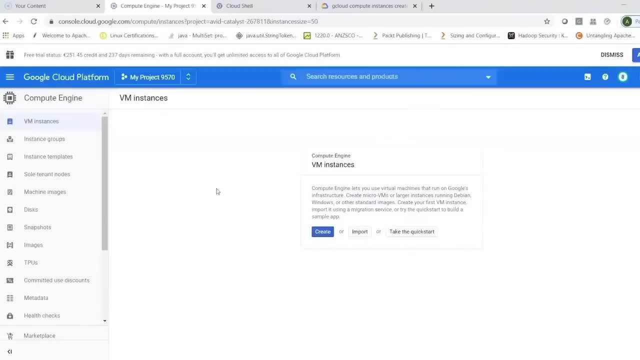 You can add more storage space if needed. And when you talk about instances and network, a project can have up to five VPC networks. So VPC network is virtual private networks wherein you can. virtual private cloud networks, where you can have your resources within your own subnet and each instance belongs. 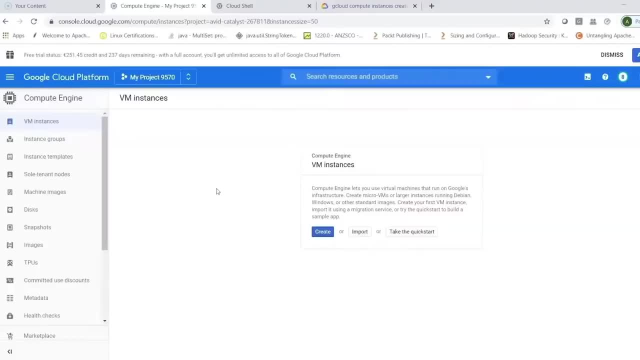 to one VPC network. Now instances in same network can communicate with each other through local area network protocol. An instance uses internet to communicate within any machine, So that could be virtual, physical or outside its own network. When you talk about instances and containers, you should remember that compute engine instances 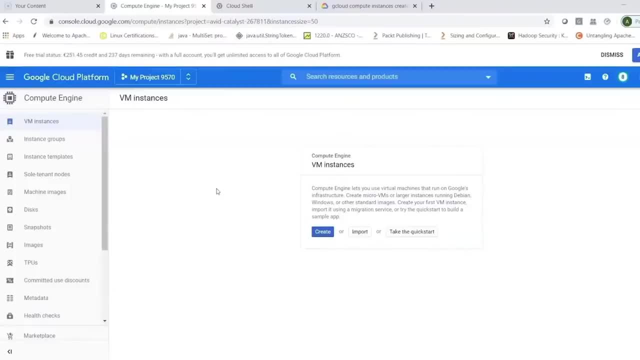 support a declarative method for launching your application using containers. Now you can create a VM instance or a VM instance template. You can provide a Docker image and launch the configuration. There are different ways in which you can create these instances, And once you create these instances, you can say, for example, you are creating a Linux instance. 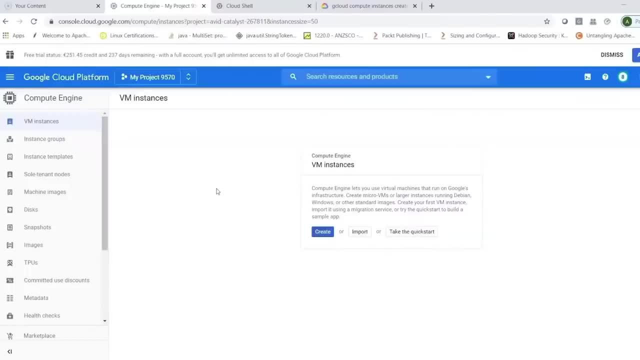 You can associate SSH keys with your Google account or your G Suite account and then manage your admin- non admin access to the instance using IAM roles. If you connect to your instance using G cloud or SSH from console, which we will see later, compute engine can generate SSH keys for you. 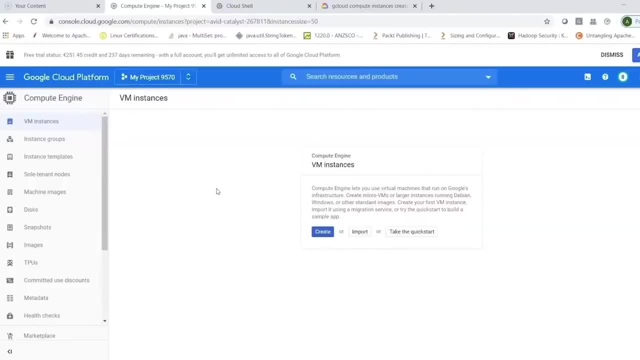 So you can create a VM instance. If you connect to your instance using G cloud or SSH. from console, which we will see later, compute engine can generate SSH keys for you And apply that to your Google cloud or G suite account. Now what we can do is we can see how we can create your Google cloud instances from your 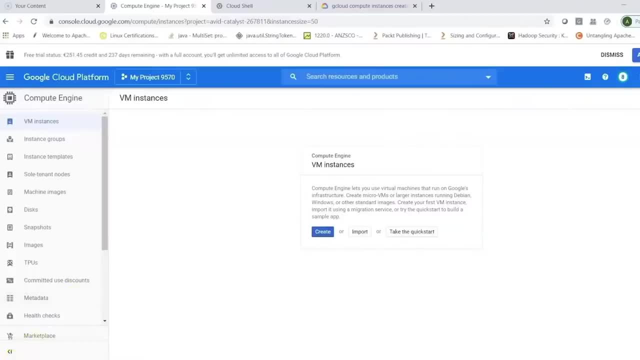 console or from the command line. Let's have a look in creating instances using GCP console, Now that we have learned on some basics of Google cloud platform. What are the different services? What are different domains? Basically looking at your Google cloud console or even cloud shell, 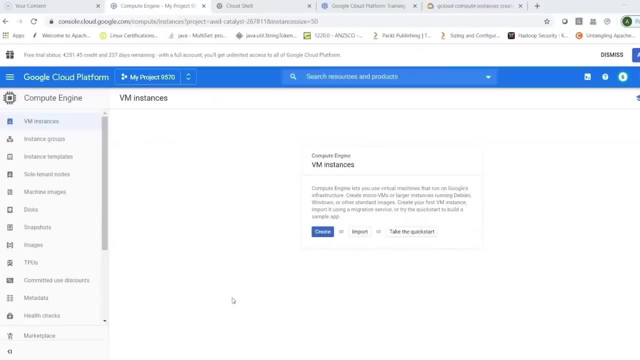 Let's go ahead and create some VM instances Now, that's from your compute engine service, and let's try connecting to these instances and see how this works. Let's also see what are the different options which are available when you would want to create the virtual machine instances here. 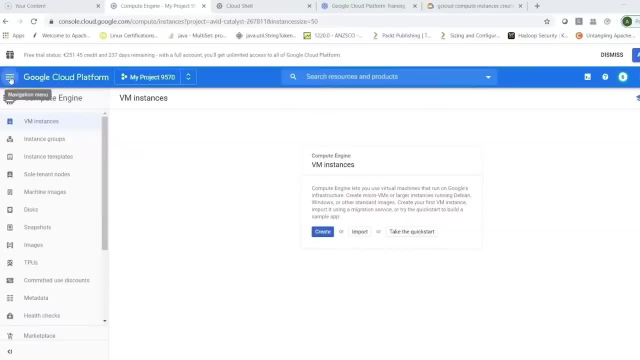 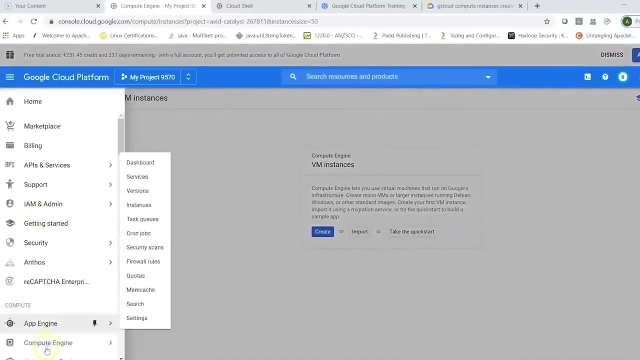 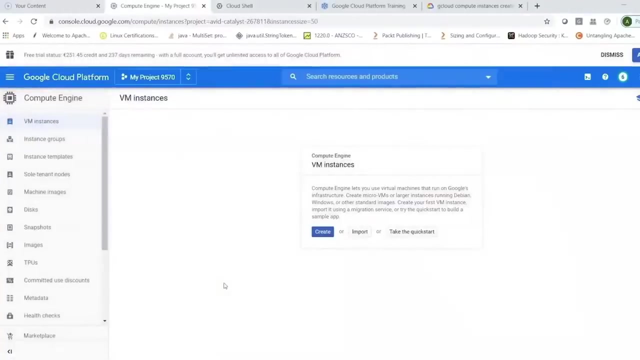 So when you click on your drop down from the top left and choose compute engine, so it brings you to this page. So I can show that again. so you can click on compute engine, click on VM instances, and that basically brings you to this page. Now, here it tells you: compute engine lets you use virtual machines that run on Google's. 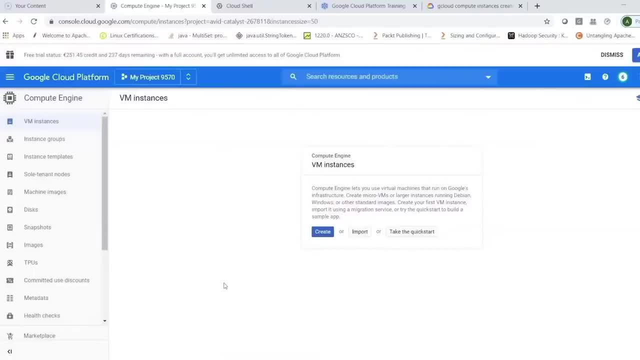 infrastructure so we can create micro VMs or large instances running different distributions of Linux or Windows using standard images, that is, public images, and you can also have your own image. So let's create a VM instance By clicking on create Now. that's basically helping me to create an instance here. 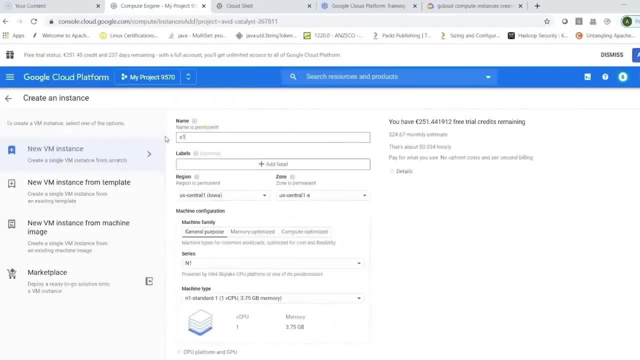 So it shows me the instance name. I can give it something, so let me say C1.. Now I can add labels. So what is label? It basically allows you to organize your project at arbitrary labels as key value pairs to your resources. So this is basically categorizing your labels and projects if you have multiple projects. 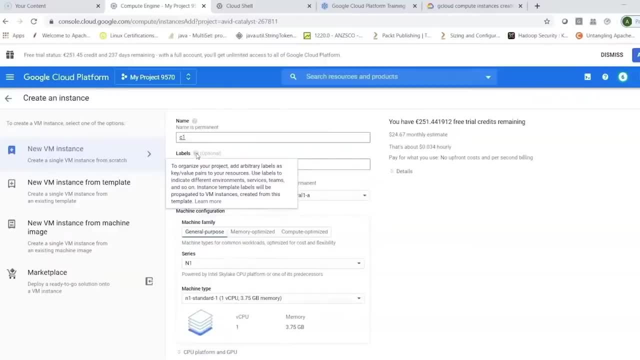 Now remember: If you have your cloud console And if you have created your free trial account, It will allow you to do these things. If not, you may have to go back to the billing section and see if the billing is enabled, Which also means that when you are creating your Google Cloud account, it will ask you. 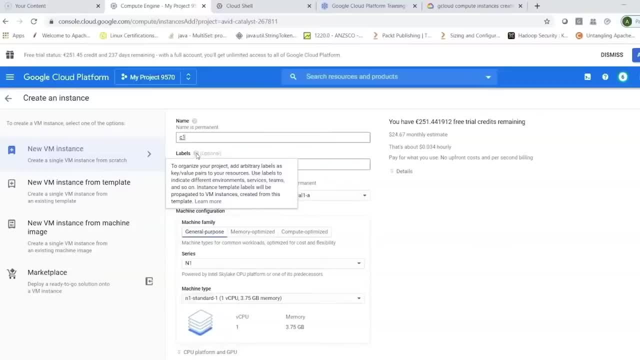 to key in your credit card details, but they do not charge anything, or they might charge. might be one dollar or one rupee, depending on your location, and that's also refunded. but that's just to verify your card Now, Once I've given the name. 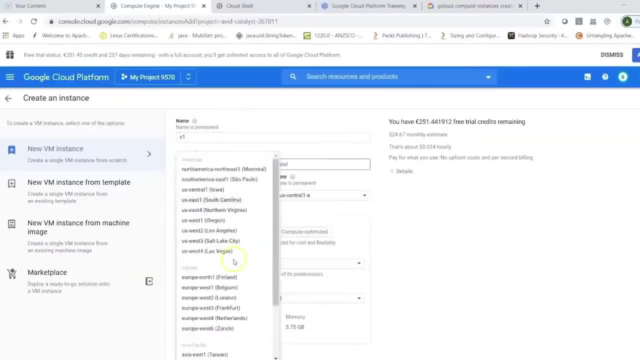 I can choose a region, So I would basically choose Europe. since I'm in Europe, I would be clicking on Europe West 3 and here I can choose an availability zone. availability zone is basically to make your services or instances or any other resources highly available. 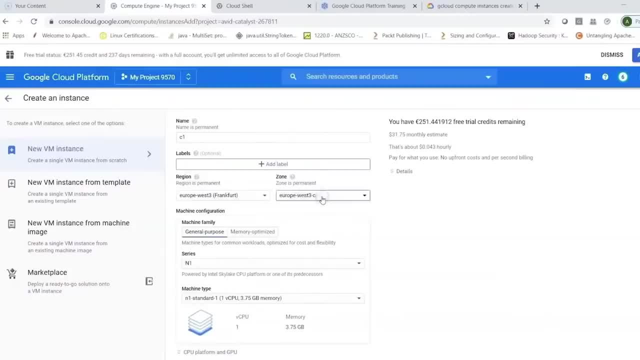 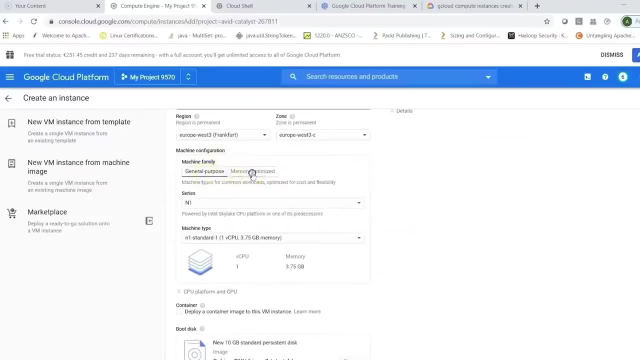 So you can choose one of the availability zones. Now I would choose, say, West 3.. Now this one, we can scroll down and here it says machine configurations. you have general-purpose machines, you have memory optimized machines, which is M1 series, and you can always go. 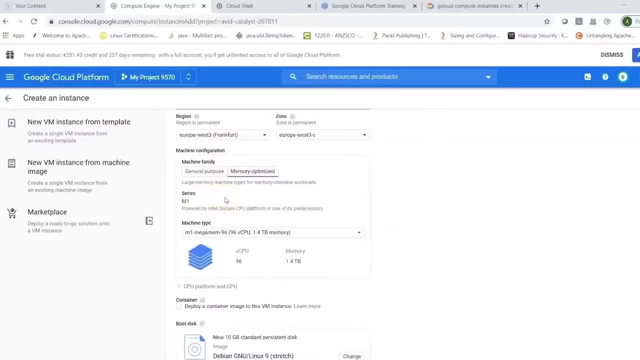 back to the Google Cloud page and see what a particular kind of machine specializes in. So I would click on general purpose. and in general purpose you have different categories. so you have N1, which is powered by Intel Skylake CPU platform, or you have E2, which is CPU platform. 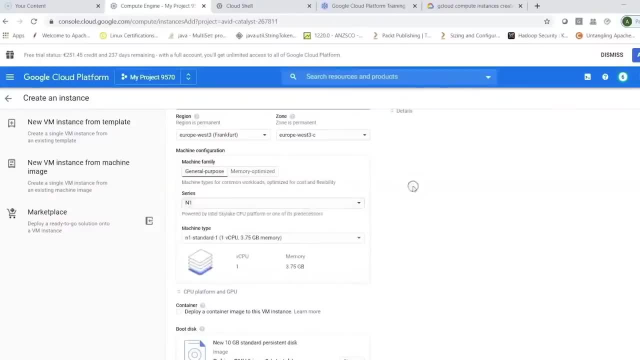 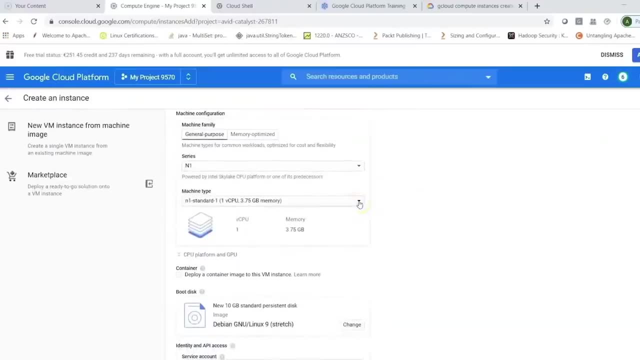 selected selection based on availability. So let's have N1 selected. Now. this one shows me the machine type And if you are using your free tier account, then you can start with correcting a micro machine, which is one virtual CPU core. You can go for a G1 small, which is one virtual CPU core and 1.7 GB RAM. 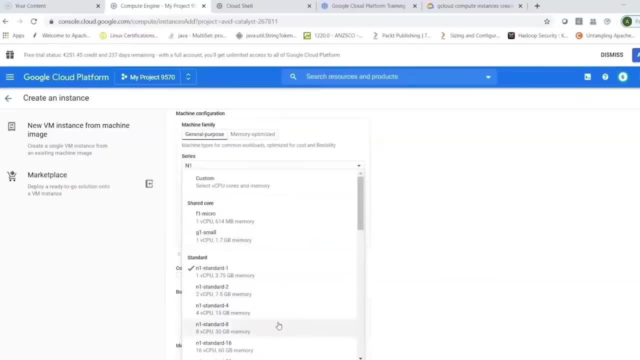 You can even go up to a high end machine, and then you can basically see if you are using a free account, how many of these machines you can use. If I would be selecting 8 virtual CPU cores and 32 GB of memory, Then it would allow me to create at least two instances by this configuration. 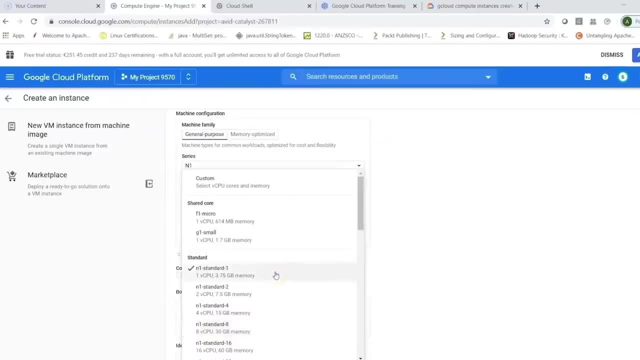 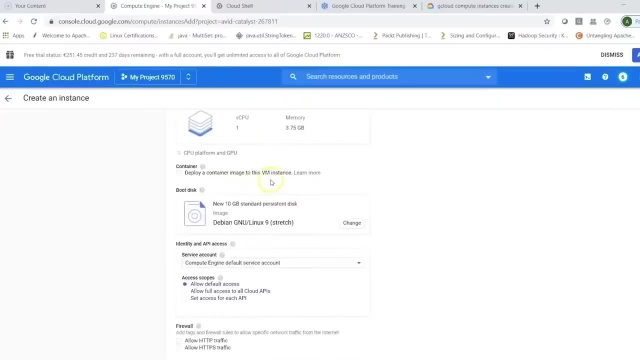 We will use N1 standard, which is one virtual CPU core, 3.75 GB memory. Now then, we can also deploy a container image to this VM instance, If you would be interested in deploying a container image. let's not get into that right now. 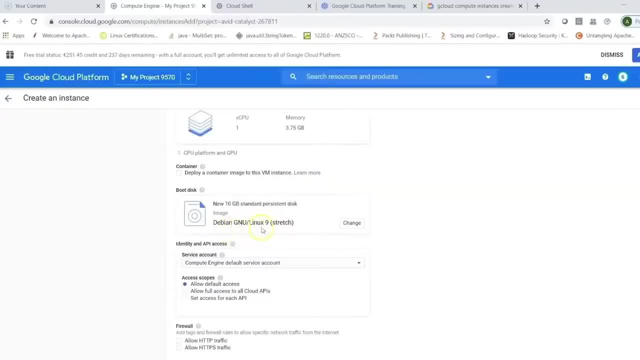 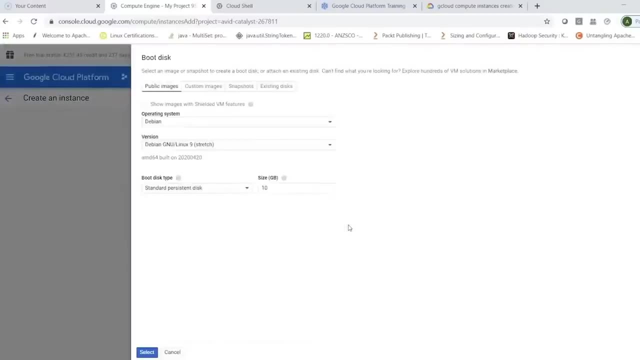 Here: it shows you the boot disk and it shows you DBN, GNU, 9, Linux, 9.. What I would do is I can go for this distribution Or I can choose a Linux distribution of my choice. So here you have public images, you have custom images. you also have snapshots, if you have. 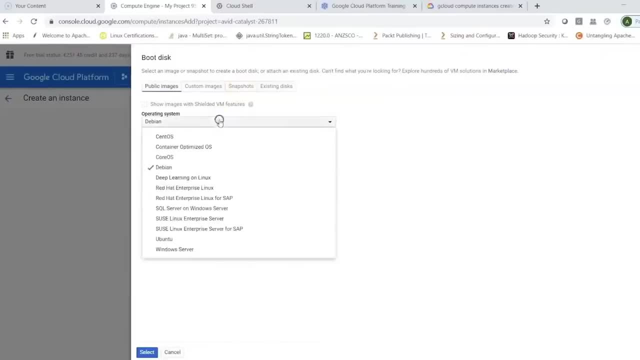 created backup of your previous images. Here I can choose, for example, Ubuntu, and then I can choose a particular version. So let's go for Ubuntu 18.04. you can go for the latest one also. 18.04 would be good enough. And here it tells me what is a boot disk. 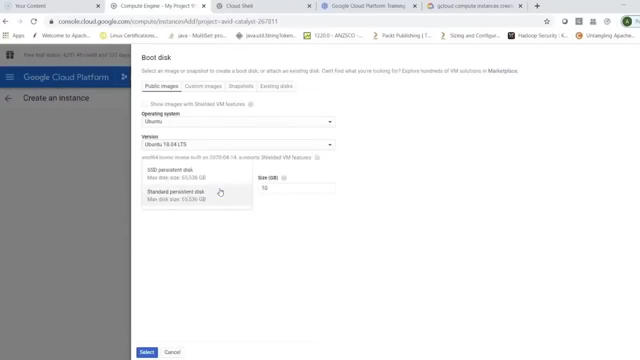 So you have SSDs or you have standard persistent disk. Now SSDs are little expensive in comparison to your standard persistent disk or your SDDs, But then SSDs are faster. So as of now we can choose standard persistent disk as it is and we can let the GB be 10.. 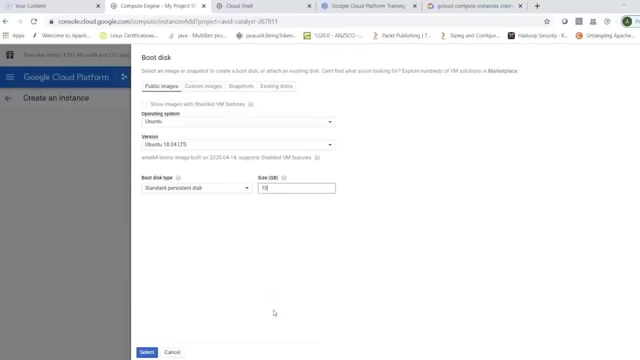 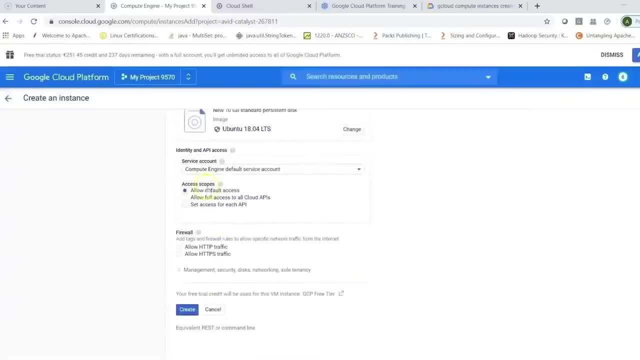 Now, depending on your requirement, you can increase this. You can even add disks later, that's not a problem. Click on select. Now here I have access Scopes. So here I will say: allow default access. You can also set access for each API, or you can give full access to all cloud APIs. 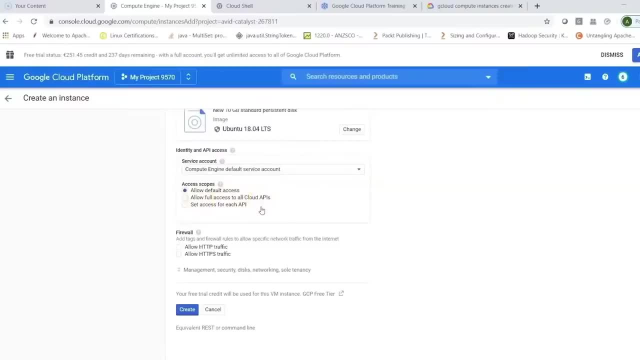 So that, based on your requirement, you can any time change later. also, We will also say allow HTTP traffic and we can also choose: allow HTTPS traffic. that basically allows me to access this machine or services which are HTTP based accessible from this machine. Now We can do that in different ways. 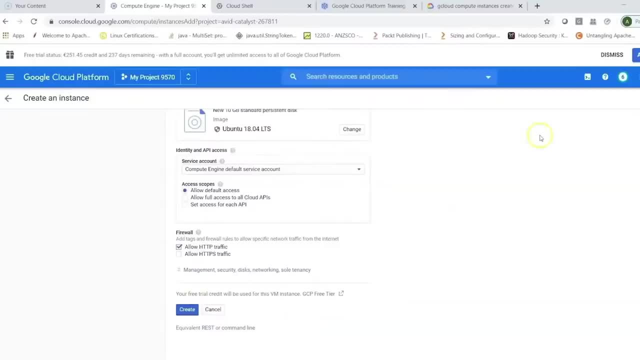 One is: when you bring up your machine, it will have an SSH access which you can log in from the cloud platform here itself. or what you can do is you can create a private and a public key using some softwares like Putty or Putty Gen. 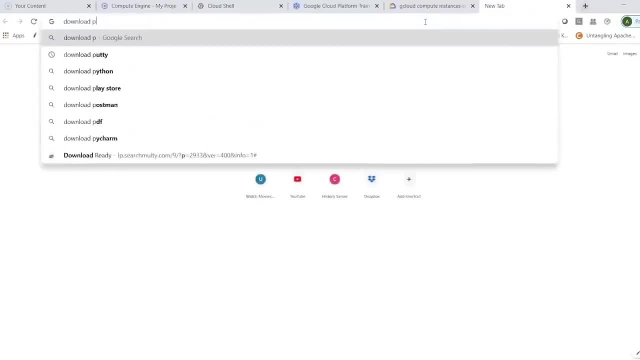 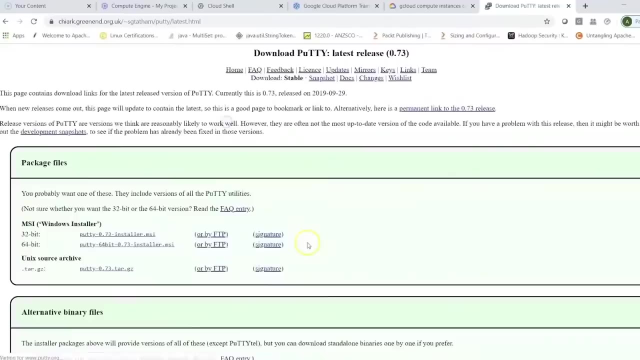 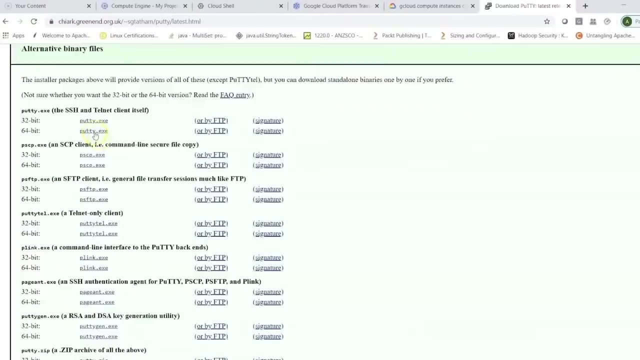 So, for example, if you do not have that on your machine, you can download. you can just type in download Putty. That takes you to the Puttyorg page and here you can click on download Putty and scroll down which shows you for your 64 bit machine, which I have in my case, you can download Puttyexe. 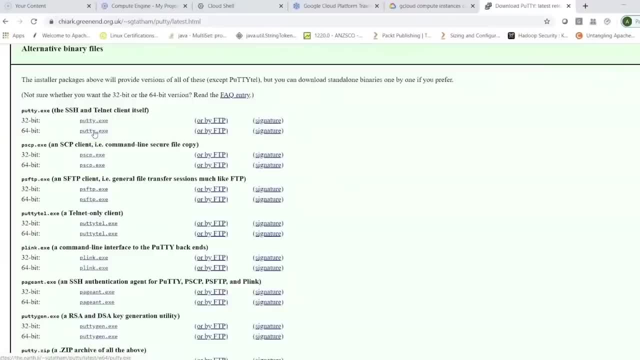 which is basically your SSH and Telnet client to connect to your machines. You can also use Putty Gen, which will be allowing you to create a private and a public key, which I have done in my case. Let me show you how. So what you can do is 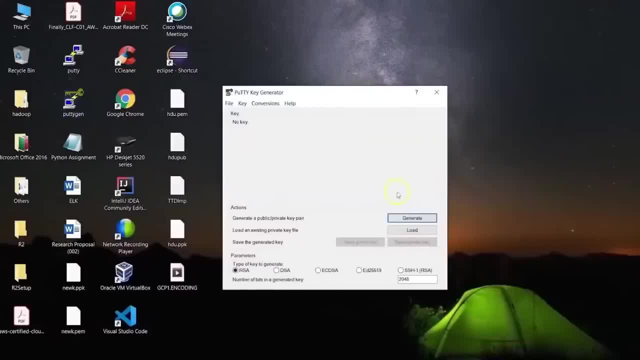 You can Go to Putty Gen to begin with, and here you can click on generate Now. then, to have this key generated, just move your cursor on the top here in the empty space and that creates your key. You can give it a name. 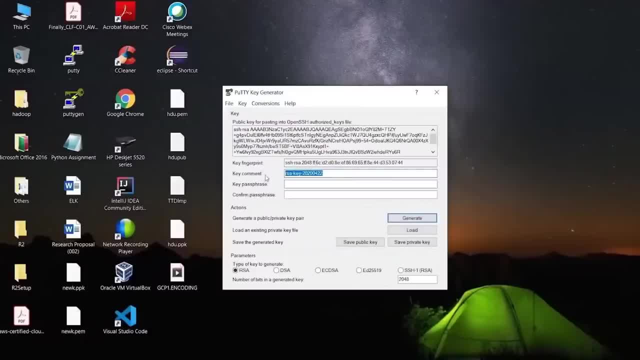 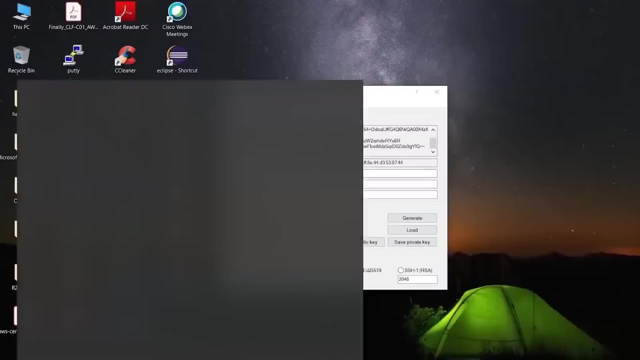 So, for example, let's give a user name- I would give HDEU. Now I can give a password for this one. So let me give a simple password, and what I can also do is I can copy this public key from here And, for my later usage, I can just keep it in my notepad file, which I can use later, and 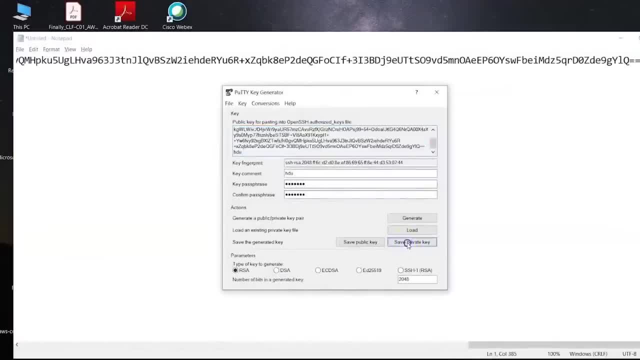 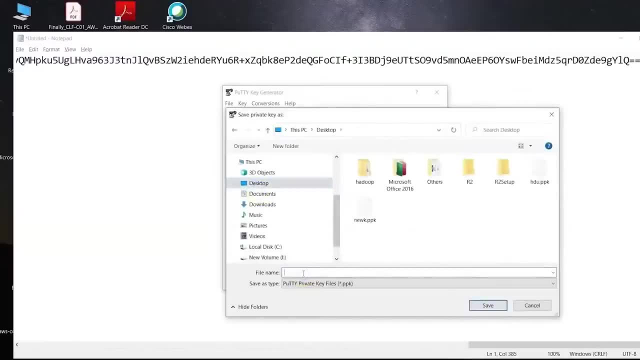 I'll show you when. So now we can save this private key and this will basically allow me to save my private key. I can choose desktop and I can give it a name. So let's say new key, new key, and that will be getting saved in a dot PPK file. 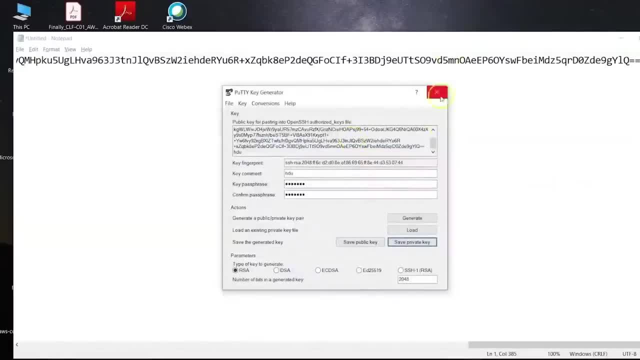 So let's save it and that's done. So we also have our public key And we have saved our private key. Now we know that when you would want to connect using SSH, you need your private keys to the client, and public key also has to be existing. 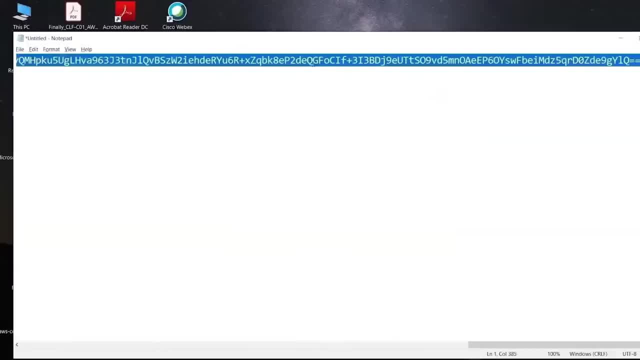 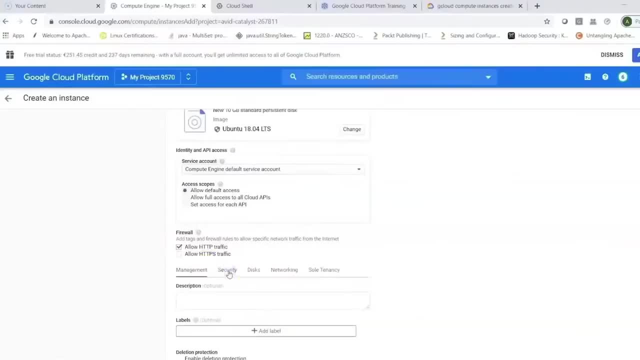 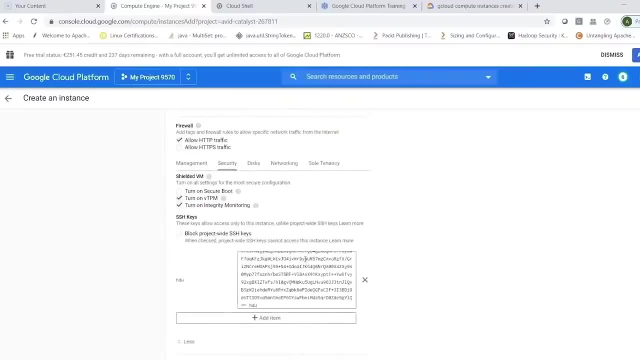 So let's take this public key, So let's do a control A. I'm going to copy this and I'm going to come back to my Google Cloud console and here you can click on security. So you can click on the security tab here, scroll down and just give you a public key. 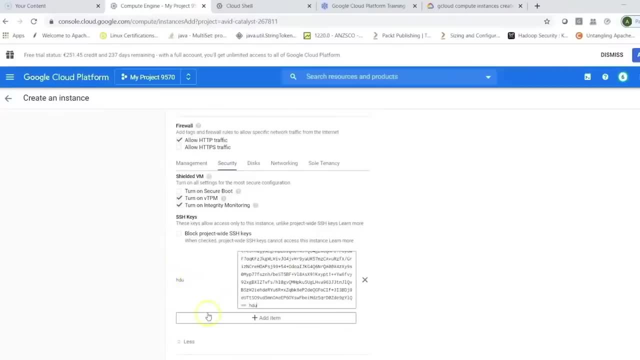 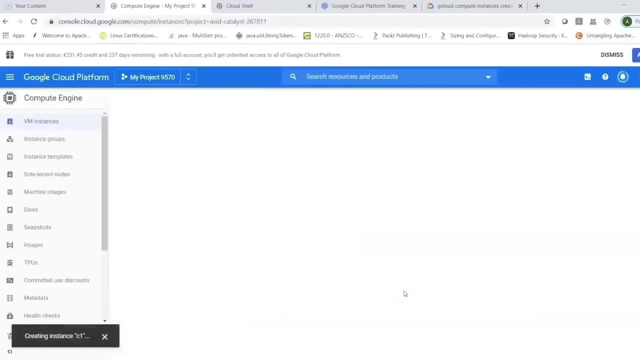 Once you give that, it resolves And shows you the name and this is good enough so that I can use my SSH client to connect to this machine. I can click on create and this will basically create my VM instance. It will take some time and then your instance will have an internal IP which will show up. 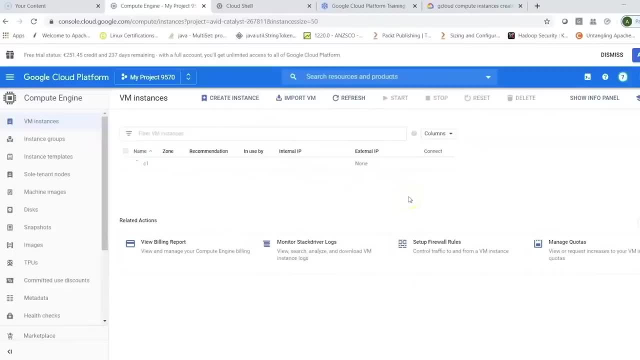 here external IP and it will also show you options to connect to these machines. So this is my internal IP. This is my external IP which I can use to connect from a client. I can easily connect from the option here which says SSH and I can say open in a browser. 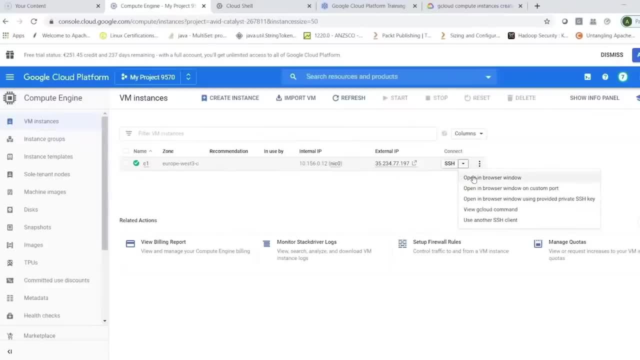 window. I can even open this in a custom port. I can look at the gcloud command which you can give from cloud shell, or you can use another SSH. So let's first do a open in browser window and let's see if this connects. 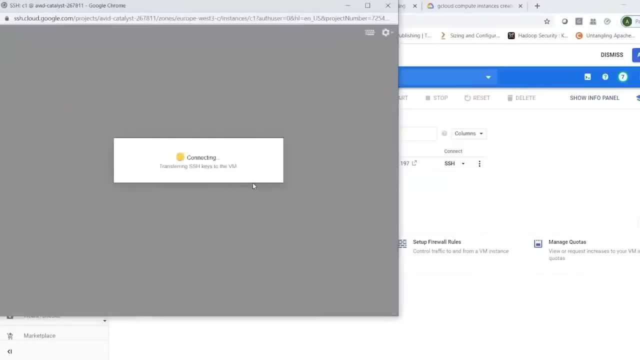 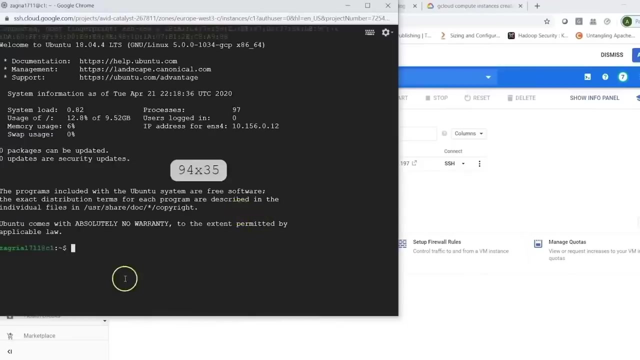 So we can easily connect to our instance in the Ubuntu 18 instance, which I just set up here easily in a couple of seconds. This is trying to establish a connection using your SSH keys, and when you do that, it also basically brings up this web browser. 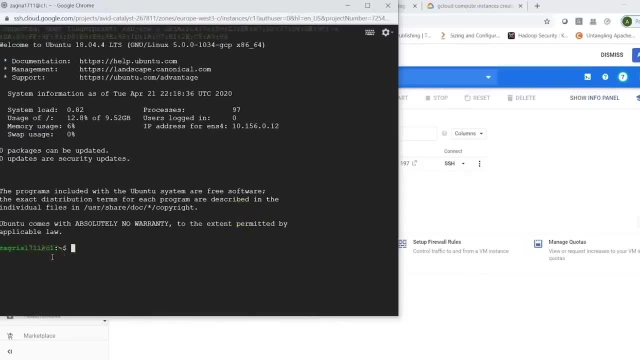 So I'm already connected. It shows my user name, which is my cloud account user name, and I have been connected to this machine here using SSH. It did not ask me for any password and basically now I can just check what do I have in my 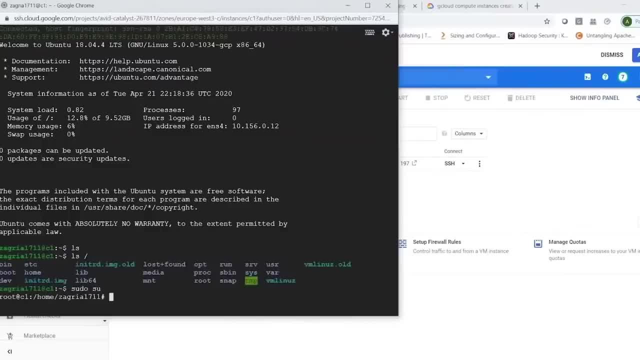 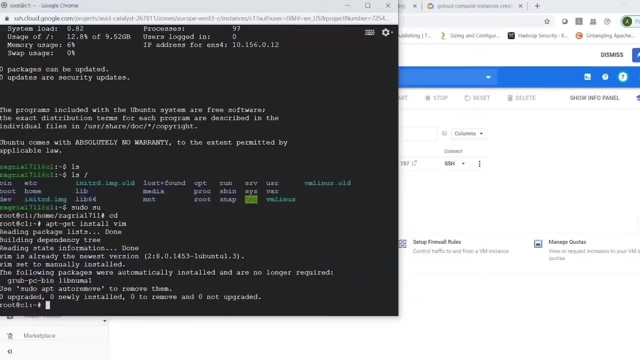 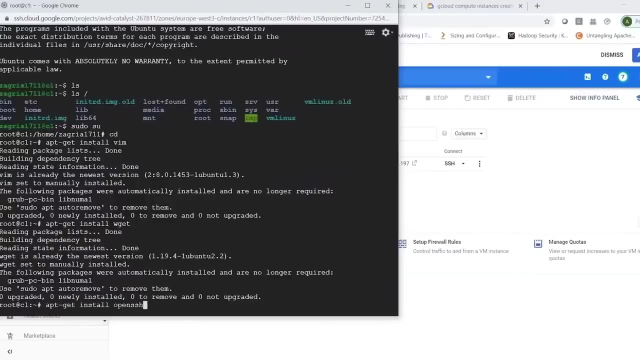 Linux file system And I can any time login as root By doing a script. So it is doing a script, sudo su. for example, let's try installing a package and i can say: apt-get install vim or apt-get install wget or apt-get install open ssh, and all these packages are already existing, so not an 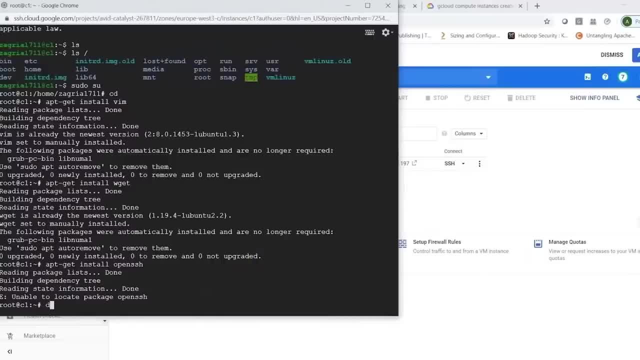 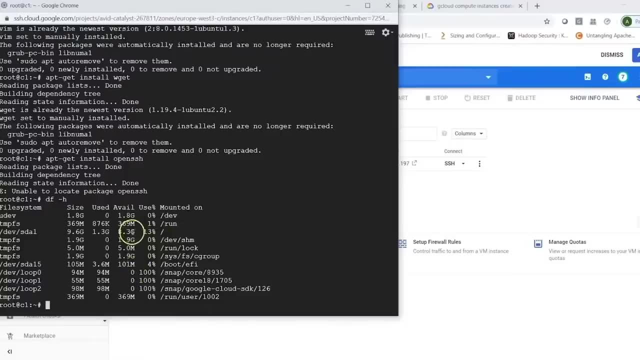 issue. now i can start using this instance. i can just look at the disk. what is available? okay now. we gave around 10 gigabyte, out of which we see 8.3 gigabyte here for the dev sda1 and then 1.8. 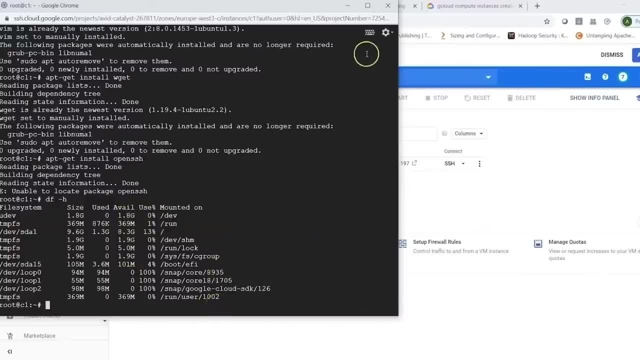 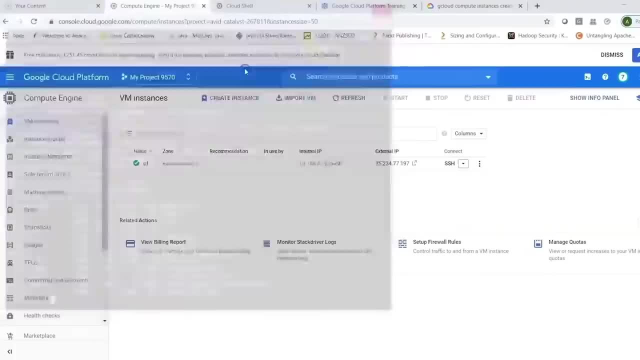 gigabyte available and you can continue using this machine. this was the easiest way of connecting to a vm instance using ssh. now, what we can also do is i can just leave this and i will now try to connect using an external ssh client. right and here you can copy the public ip, so when you want, 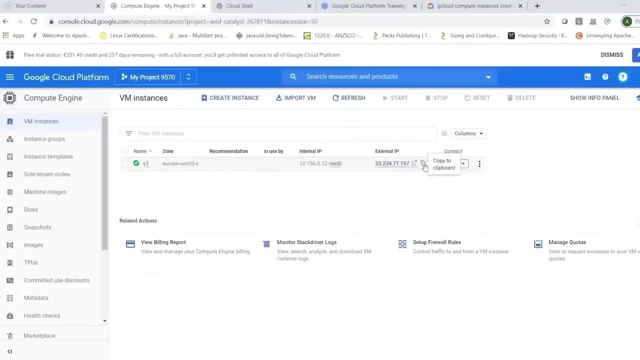 to connect to an instance, you will have to get the public ip. also, remember that if you select and stop this machine, which will stop your billing counter, and if you start it again, the internal ip will remain same, but the external ip is the one which will change. i can obviously select this machine anytime and i can. 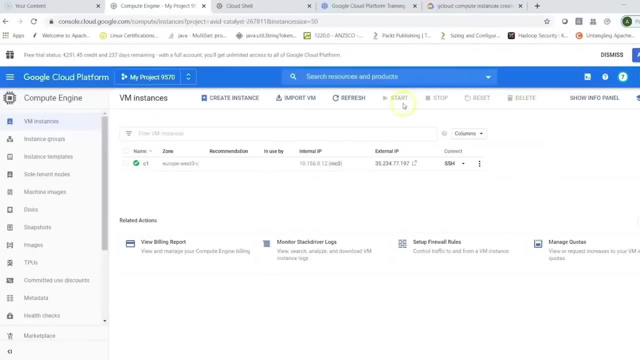 do a cleanup and i can delete it. i can do a start of the machine if it is stopped, and i can even import the virtual machine to be used later. so there are different options which you can always use. so this is my instance and if you would, 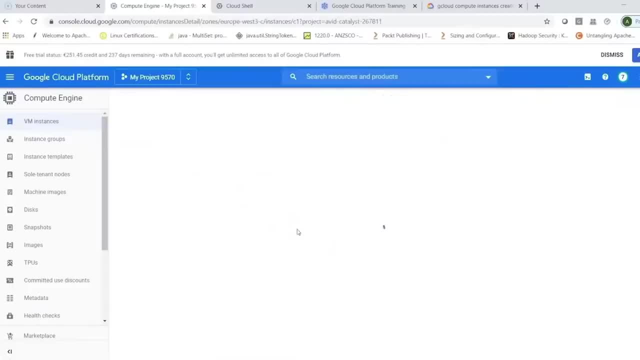 want to look at the details, click on this one, c1, and that should basically allow you to look at the details. so it shows you what is the instance id, what is the machine type, is it reservation specific? what is the cpu platform, what's the zone and all the other details at any point of time. if 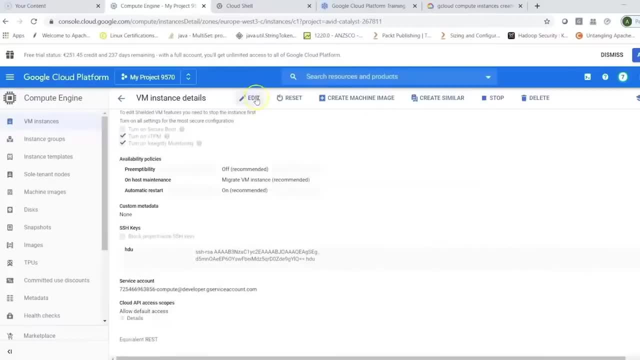 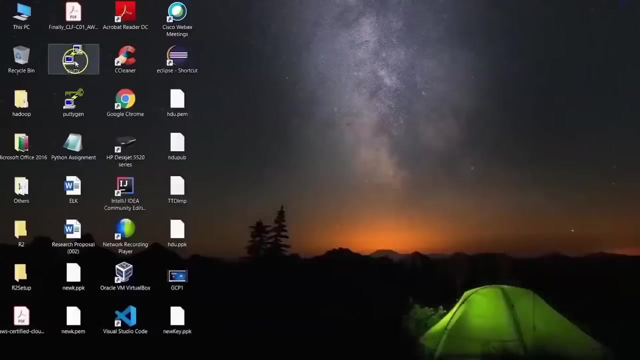 you would want to edit. you can always click on edit the details as you need. now you can also look at the equivalent rest command to basically use the rest api to connect to this instance. for now i have copied the public ip and i would want to connect it using putty, so let's go in here and let's give it the host name so i can give ubuntu. 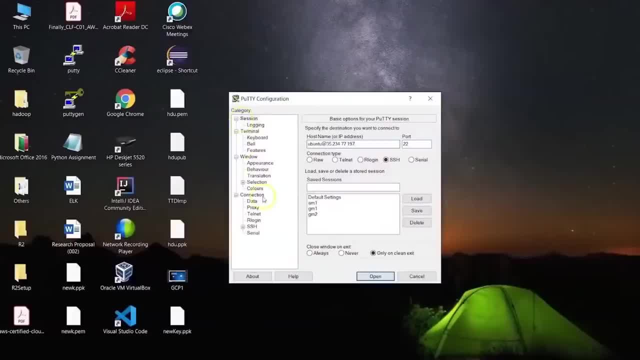 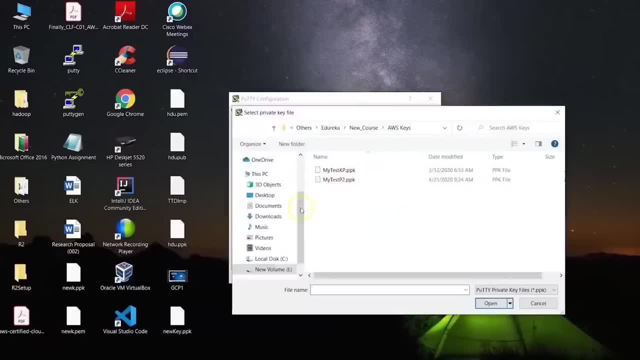 i can give my ip address, so that's in my session. now i will click on ssh, i would go into authentication, i'll click on browse and this is where i need to choose the ppk file. so this is the one which we created: new key. let's select this. 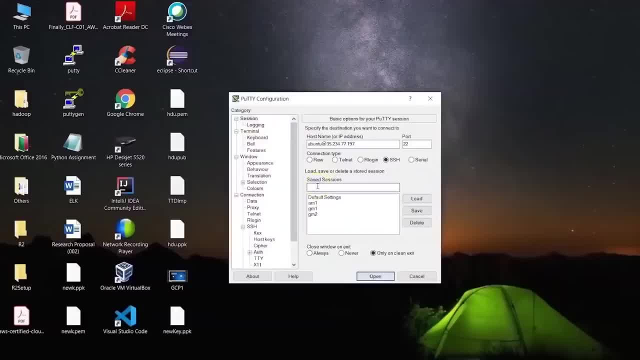 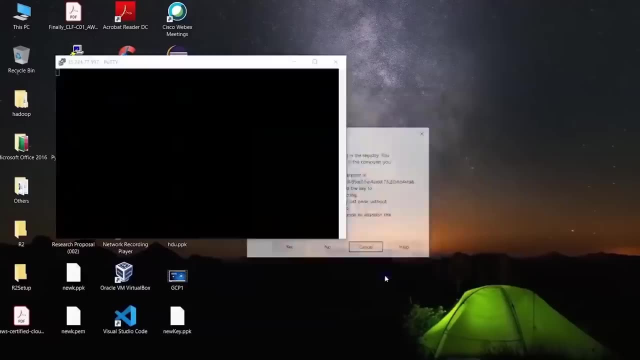 and then i can come back to session. i can even save this and i can call it as my instance one. let's save it- and you can create any number of instances. so you see, i have created different instances here for my google cloud or amazon related instances, and i can click on open. it says: 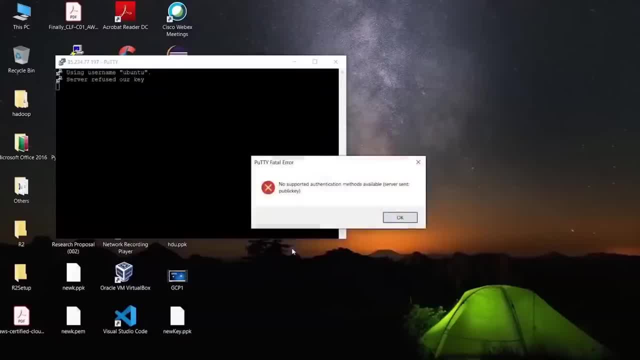 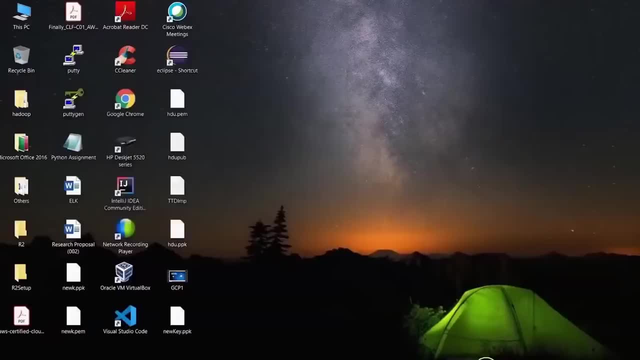 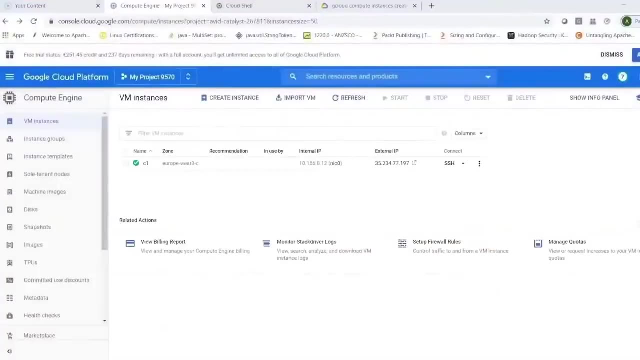 the server's host key is not cached in the registry. that's fine. just click on yes and basically it says no authentication method supported. now this could be because we have not enabled your ssh access, so let's look at that. so now let's see if we were trying. 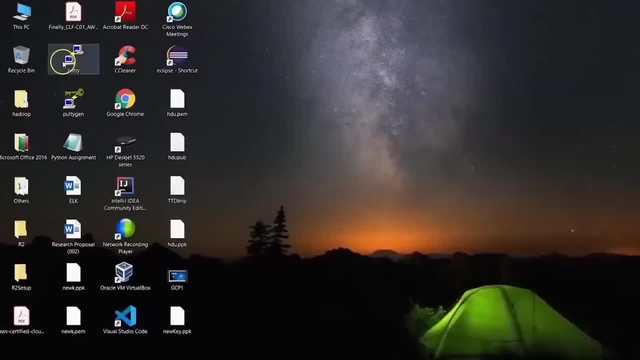 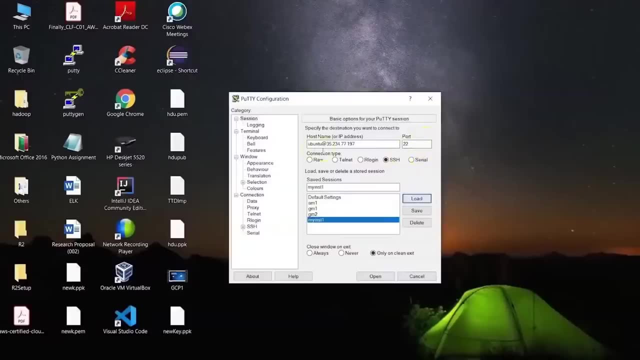 to connect using putty. what was the issue here? so if i go back to my putty, select my instance, load it. it says port 22. i am giving the username, which is ubuntu or. sorry, that's the wrong user name we gave and that might be the reason we had set up the user as. 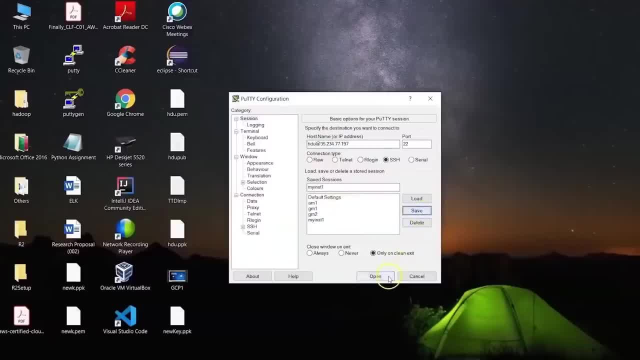 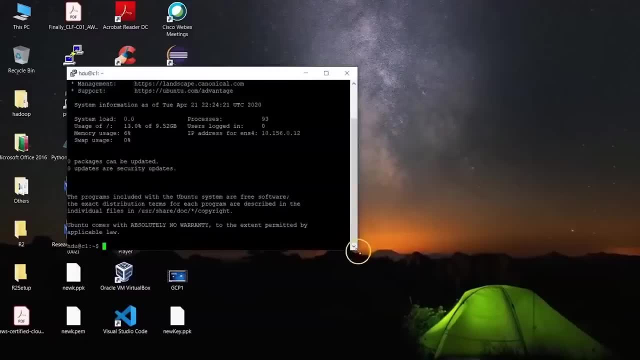 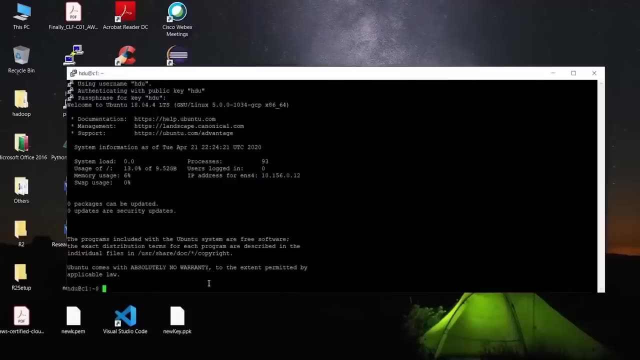 sdu. so let's save this again and now let's try connecting to this one, and it asks for my password and you are able to connect this right now. if there was any other issue related to network connectivity, then we could look at the rules- the inbound and outbound rules- which allow us to 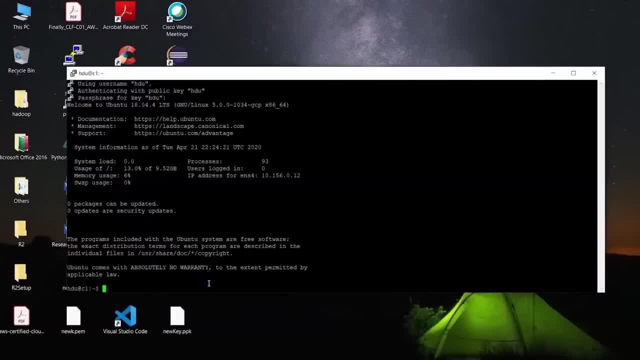 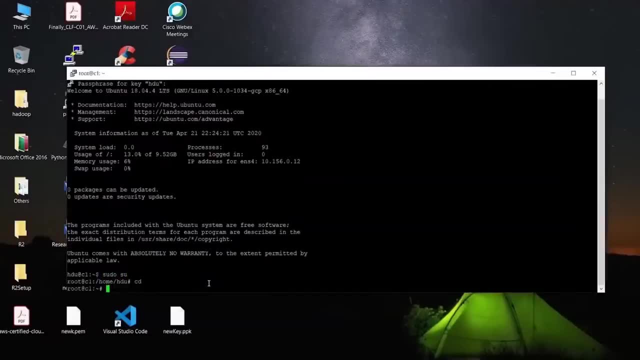 look into the machine now. we are connected to our machine here using hd you user, i can log in as root and i can continue working. so not only from the ssh within the cloud console, but you can use an external ssh client and connect to your machine. so this is your ubuntu machine and we can basically look at the space and that basically. 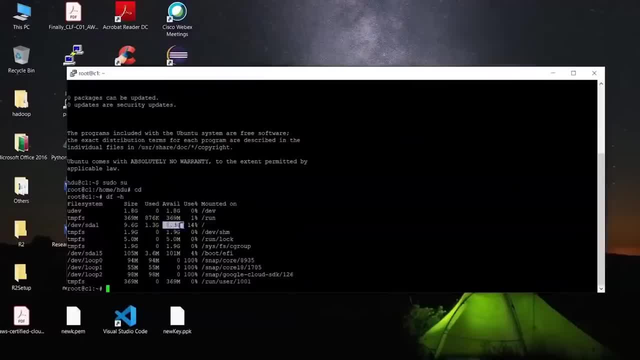 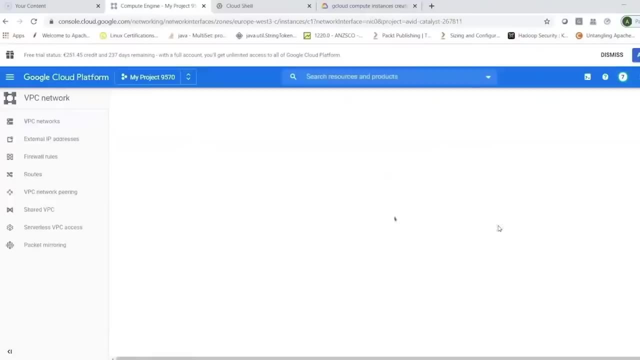 confirms we are connecting to the same machine, which shows 8.3 gigabytes here and 1.8 gigabytes here, which we were seeing from the ssh in the browser. now let's close this and let's go back to our instance page. now, here you can always look at the network details and this will show you. 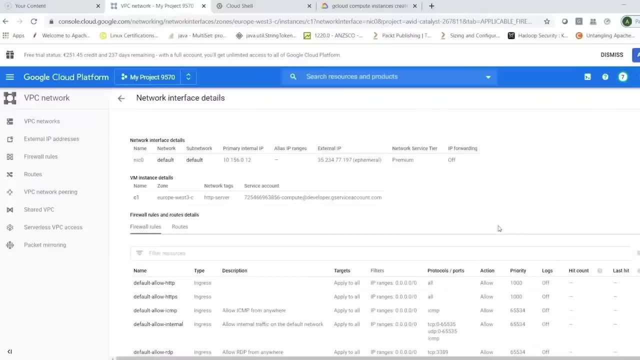 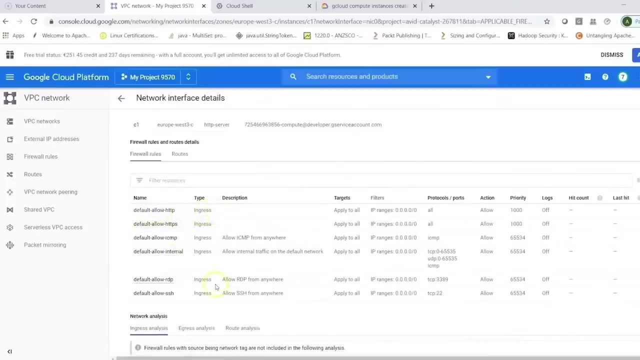 your different kind of rules, that is, ingress or egress rules, which basically allows to connect to this machine from an external network or for this machine to connect to an external network. so here we have different firewall rules. which shows default allow http. that's your ingress rule. 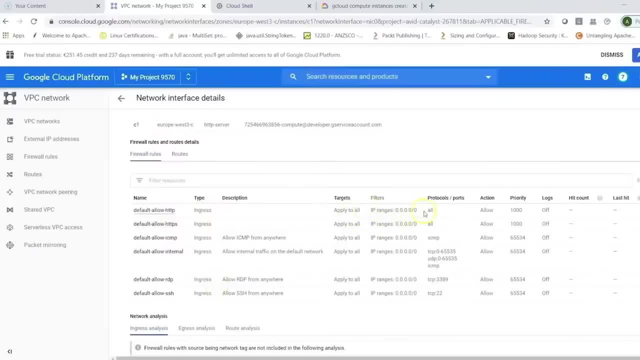 and it tells you: apply to all. it shows me what are the ip ranges where i can specifically give the ip of my machine. it shows the protocols. it shows what are the different ports which you have used for these services, for example rdp or ssh, which shows 22. you have icmp. 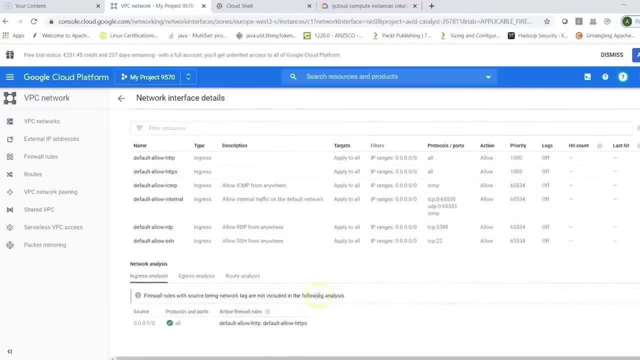 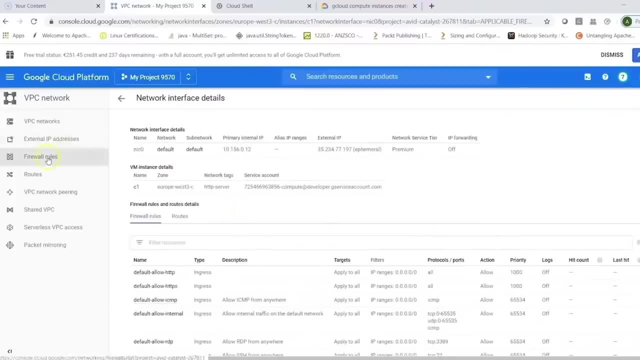 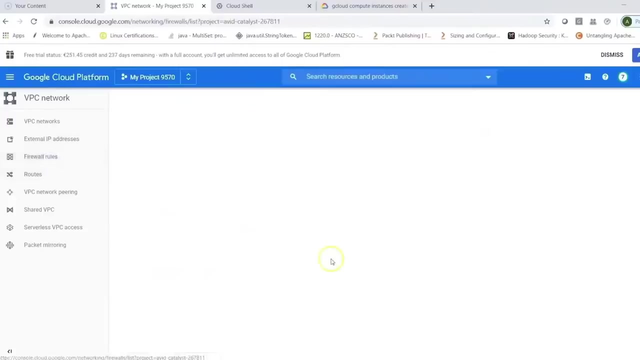 http and https now. anytime, if you would want to make a change to these rules, that can be done by going into your network details and say, for example, you would want to work on firewall rules. so we have these firewall rules here, you can click on this one. so right now we are looking into the network. 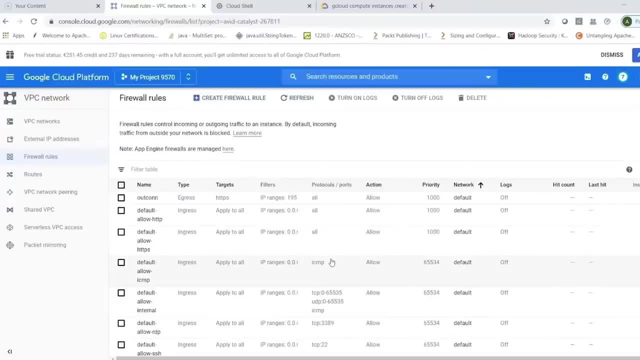 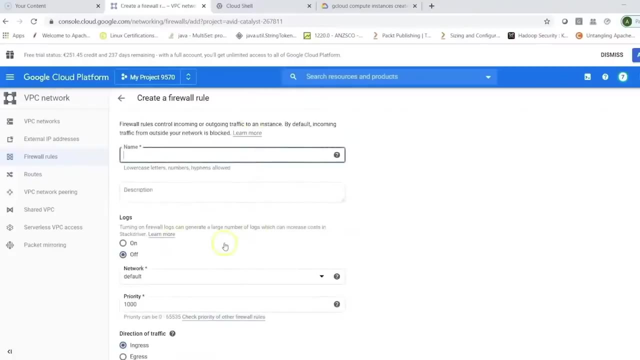 domain and we are looking into vpc network right, and this shows me what are the different rules we have. now, if i would want to create a different firewall rule for a different protocol, i can always click on create firewall rule. i can give it a name. okay, i can say what if you would want. 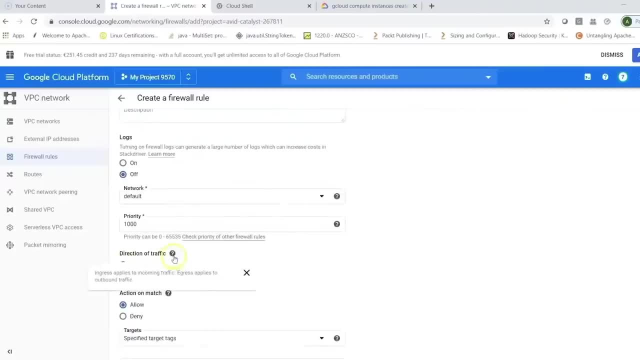 to turn all the firewall logs. you can basically say what is the kind of traffic- so ingress applies to incoming traffic and egress applies to outgoing traffic- and you can then basically choose what are the ip ranges from where you want that connection to be coming in or to going out. you can choose a particular protocol. you can give a protocol here with. 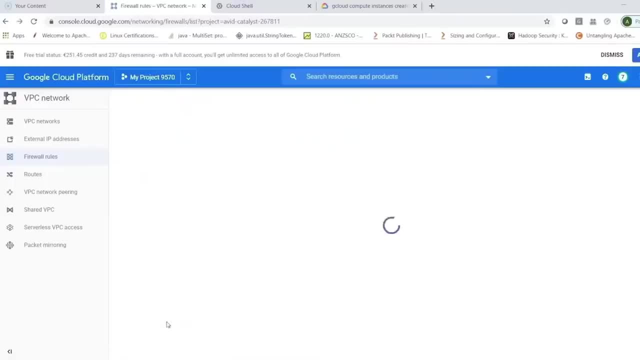 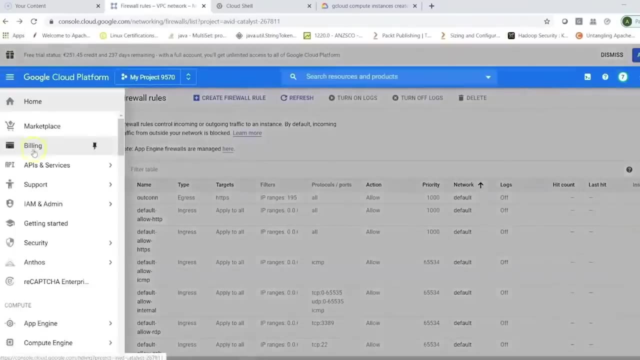 comma separated values and you can create a firewall rule. so this might be required depending on the services which you are running, wherein you might want to enable or disable a particular protocol. you might want to enable your access to your machine from an external service or to an external. 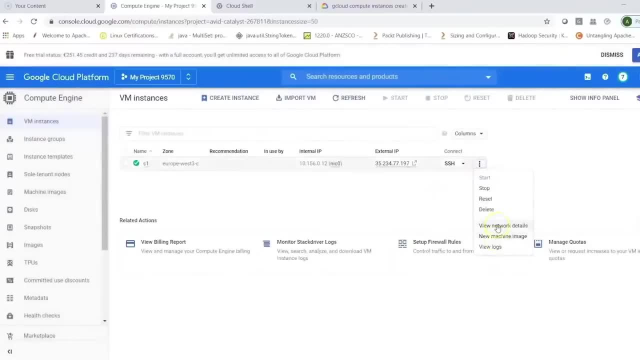 service so you can always go to network details from here. you can then go into firewall rules, create a firewall rule, apply that to your instance and restart your instance. so as of now we don't need to create any network details here, because my ingress or egress rules are already available. 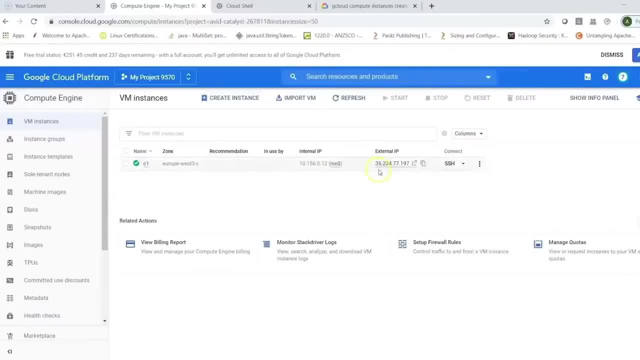 right now. i can basically then have my instance stopped and removed, so i can just do a stop, or, since this is running, the ideal way would be to do a stop- i could also do a reset. now, what does reset do? reset does not basically delete the machine. what it does is it does a cleanup of the machine and it brings it to the initial state. 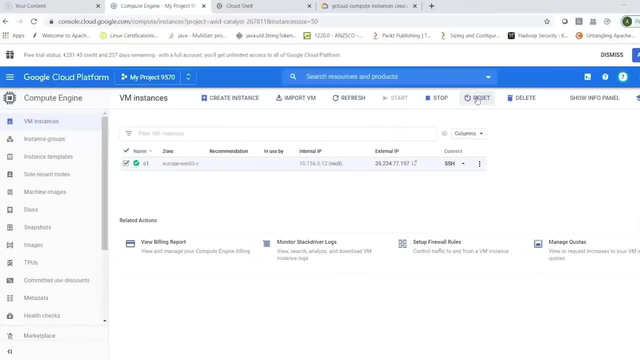 so sometimes we might have installed certain things on our machine. we would want to clean them up and at that time reset can be useful. i can basically click on delete right and i can select this and i can do a cleanup. and this is good, always when you are using a free trial account. 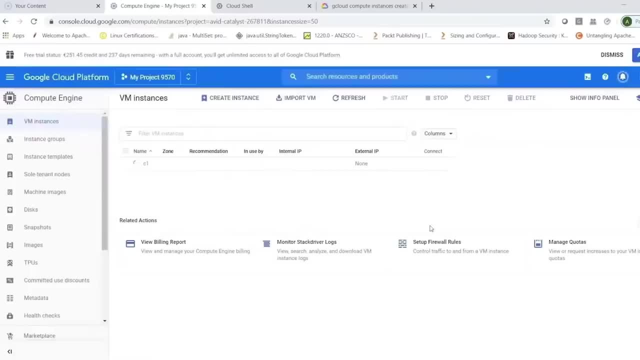 try to use different services, play around with them, and then you can clean up so that you do not waste your free billing credit right and you can use it for meaningful stuff. now i have clicked on delete and within few seconds, my instance, which i had created, will be. 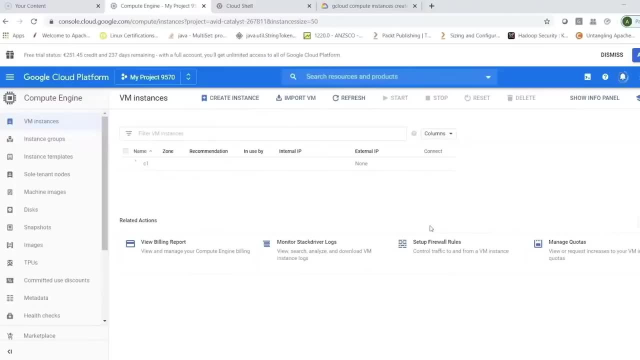 deleted. also to remember is if you are creating multiple instances, then you can connect from one machine to other machine using SSH, by using the private file. so for that we can learn in detail later. so this is just a simple example of using your compute engine, creating your instances, connecting to it from an 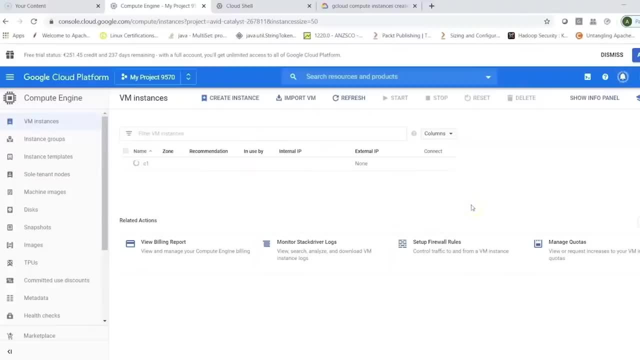 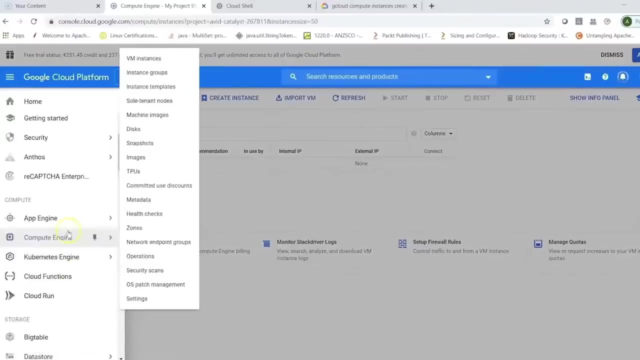 internal SSH or from an external SSH client, such as putty, where you have already created your private and public keys. now I can click on the browser here and then I can basically come out and I can basically be looking into any particular service. so we just looked into compute engine. right, you have? 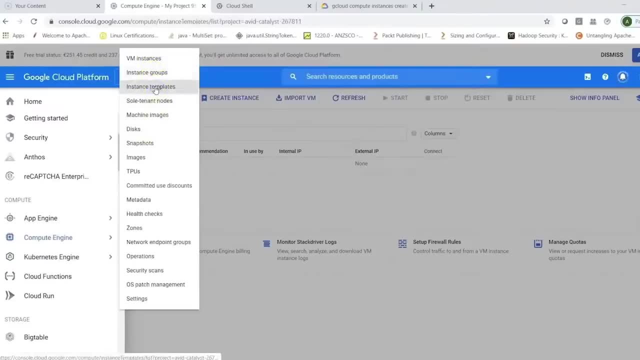 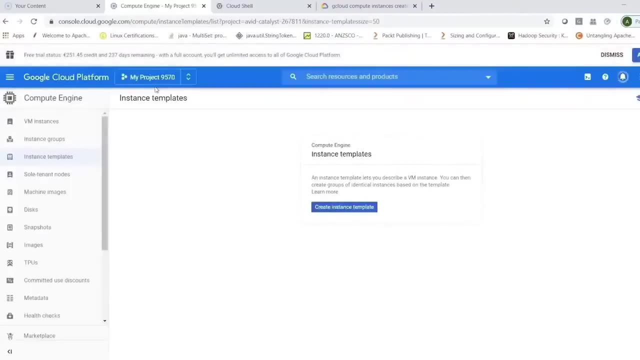 different other options. you have instance groups, you have instance templates. for example, let's click on instance templates here and that basically shows you that you don't have any instance template and this basically facilitates. say, for example, you are working as a admin and you would want to. 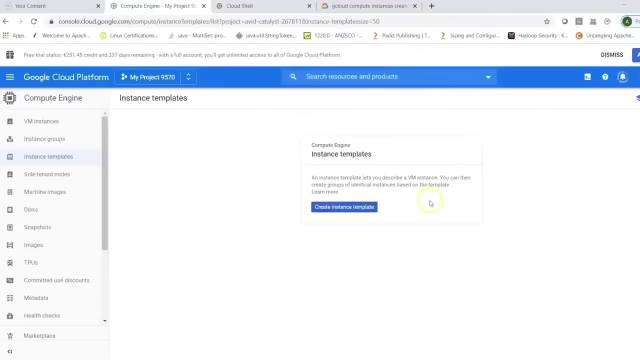 create an instance template so that, using that, you can, you can create an instance template so that, using that, you can describe a VM instance, and then you can basically use this template to create different instances. you can go for sole tenant nodes, you can look for machine images, you can also look at your tests, you can create a snapshots and you can. 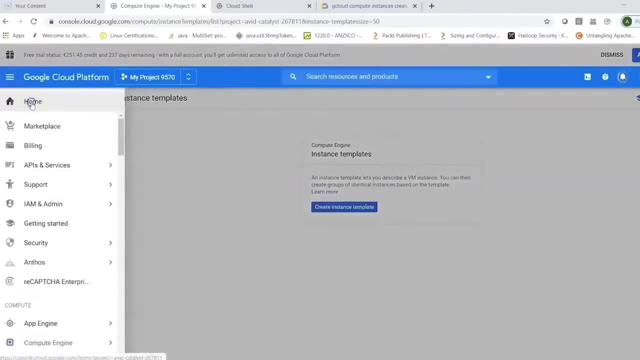 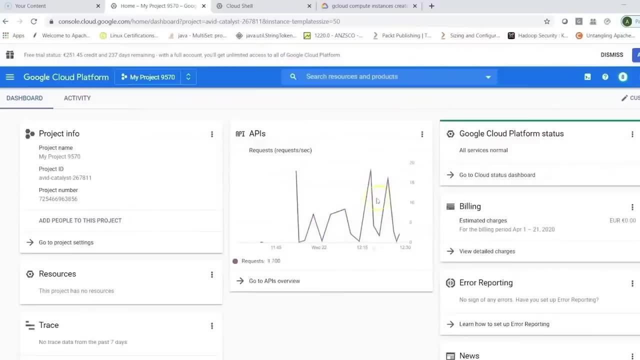 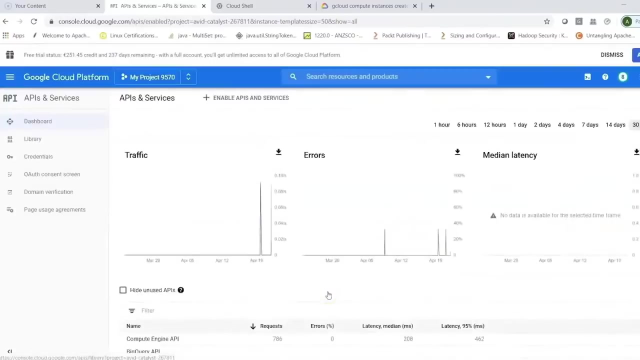 look at different options here. now let's come back here and let's click on home, and that should take you back to your home page, which basically shows you if a particular API which you have used recently, which shows me in the graph here so I can go to the API's overview- right, and that basically shows me if there. 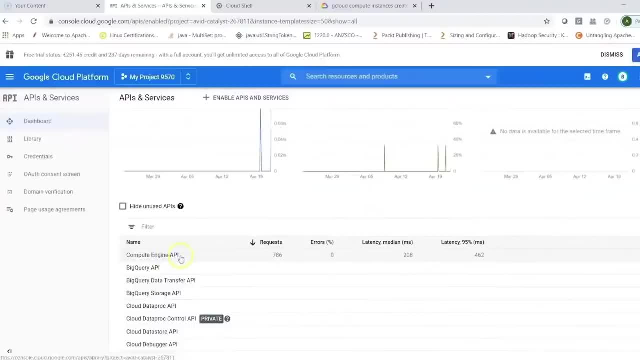 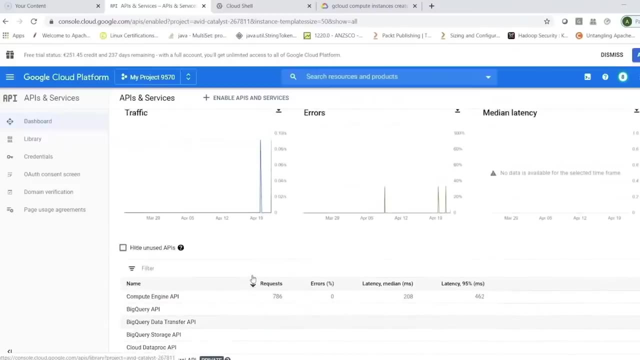 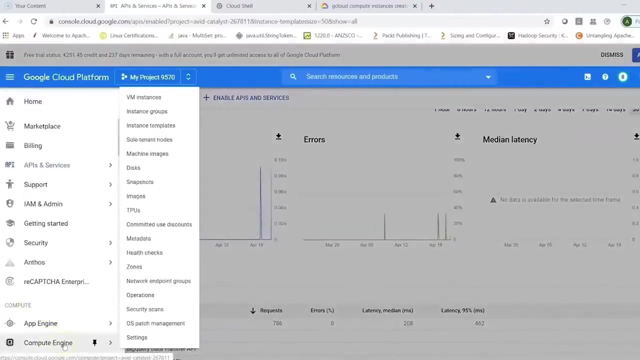 were any errors if I was using the Compute Engine API to basically create a VM instance, and that's why we were seeing some spike in the graph. so this is a quick demo of using your Compute Engine service, provided by Google Cloud, wherein you can create VM instances and use those VM instances for your 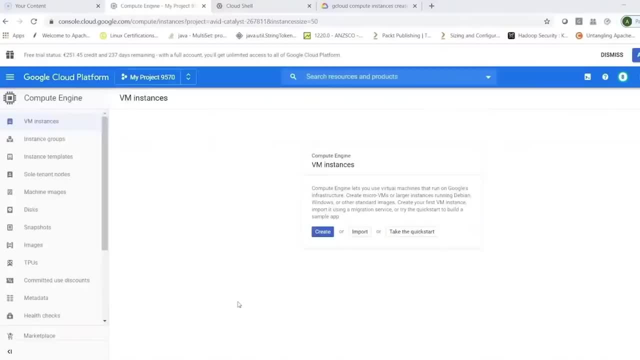 application installation for any other applications, other purpose. now that we have seen how you use your cloud console to create an instance and also clean it up, let's also understand how you can do using your command line options and let's see what it takes or what are the different. 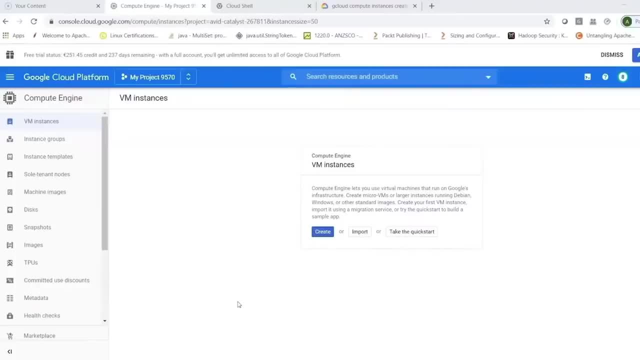 commands which you can use to create your instances. now you can always when, when you are creating an instance, you can use Compute Engine, which provisions resources, and you can also use the command line to create a VM instance, to start the instance. so instance basically has different states which we 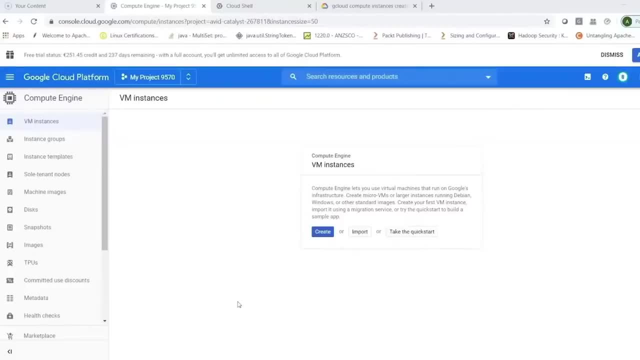 can see when we are creating the instance. so you basically start the instance, instance moves into staging that is prepared for your first boot. finally it boots up and then it moves into running. so when you look at instance states which we will create instance and see it will basically have. 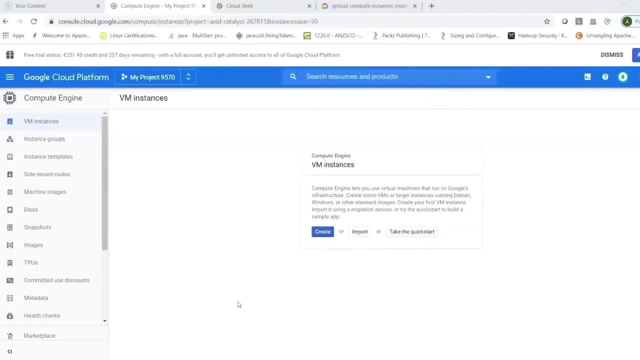 different states, such as provisioning where resources are being allowed to be allocated, for instance, but instance is not yet running. then it goes into staging, where resources have been acquired and instance is being prepared for your first boot. then instance is booting up and running and if you are, 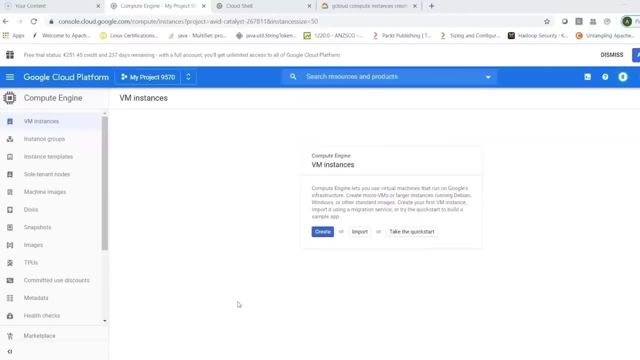 stopping an instance, it goes into being stopped status and it would be moved to the terminated option. you can also do a repairing of instance and finally, you can terminate your instance or clean it up by stopping and then deleting it. Now, when you say stopping and resetting an instance, 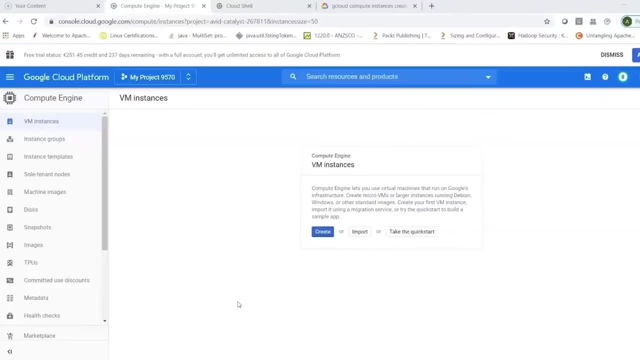 you can stop the instance, as I showed earlier, if you no longer need it. but if you need for future use, you can just use the reset option, which will basically wipe the contents of instance or any application state, and then, finally, you can stop it and have it terminated. 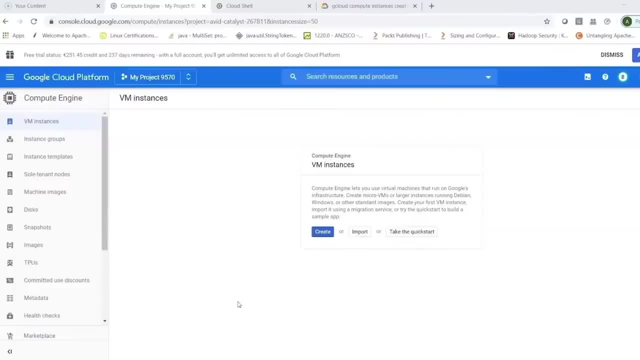 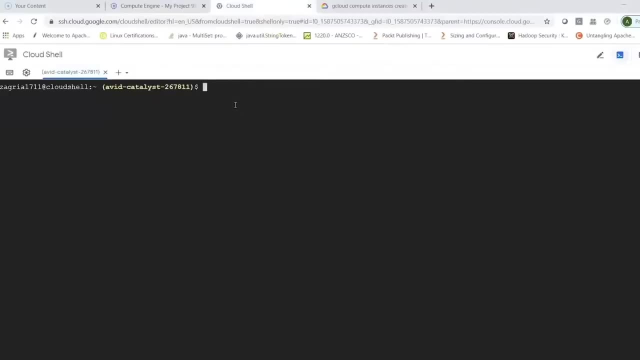 Now, when you would want to do that using your cloud console, we have seen the options. Now let's also see from the command line tool how you can do it. So here I have the cloud shell, which I brought up from here, and I basically opened it in a new window. 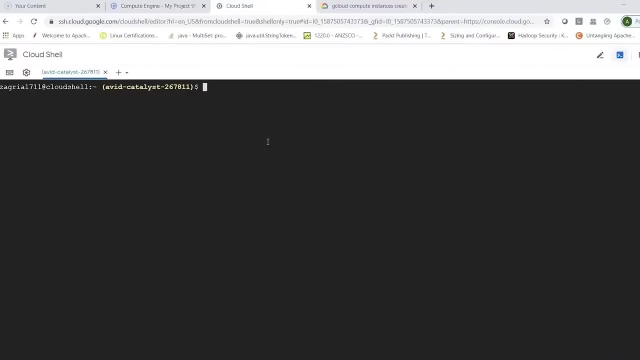 So command line tool enables you to easily manage your Compute Engine resources in a friendlier format than using your Compute Engine API. Now gcloud, which is part of cloud SDK, is the main command here and then you can always autocomplete the different options here. So when you would want to create or work on gcloud, 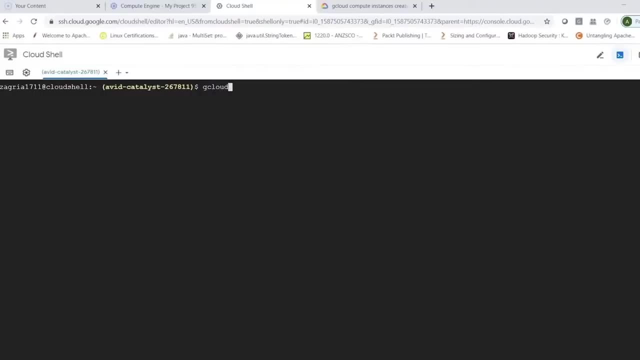 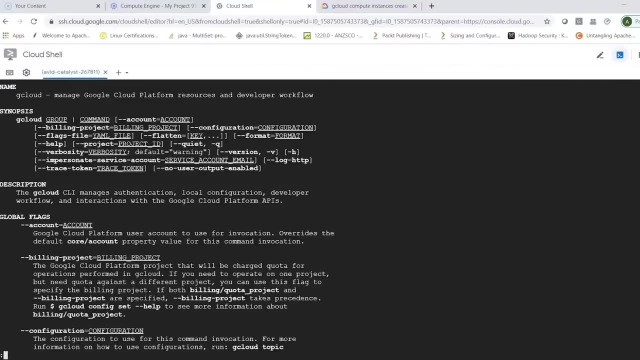 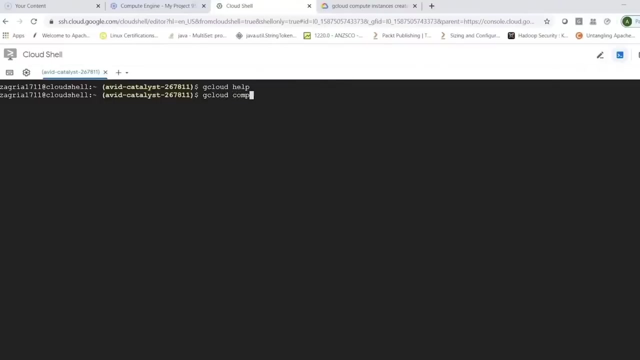 you can just type in gcloud here and then, for example, I could just say: help to see different options of gcloud, which will show me different options which you can use here. Now we would be interested in compute instances, so I could also do a gcloud compute. 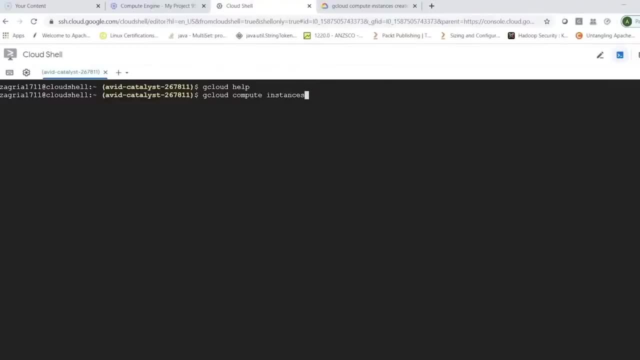 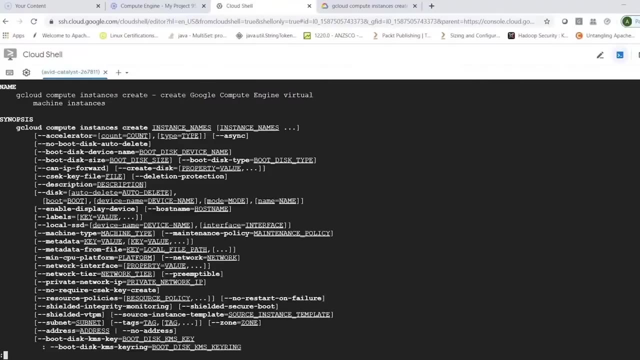 compute instances and then I can basically say create, and then I can do a help. Now that should show me different options which work with gcloud compute instances, create command, which is expecting an instance name. So your Google Cloud SDK which we can set up on our Windows machine. 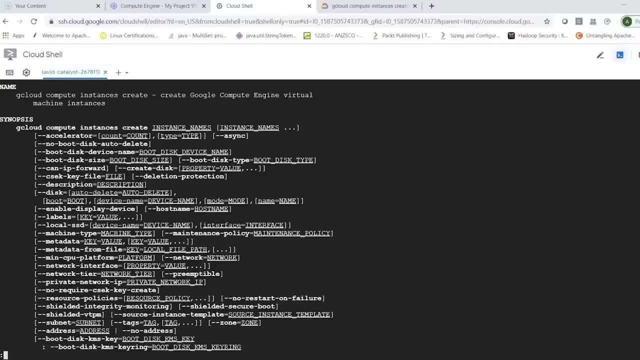 or even on your Linux machine, is set of tools that helps you to manage resources and applications hosted on your GCP. that is, your Google Cloud. Now, here you have options such as gcloud, which I'm showing you right now. you have gsutil and then you have bq. 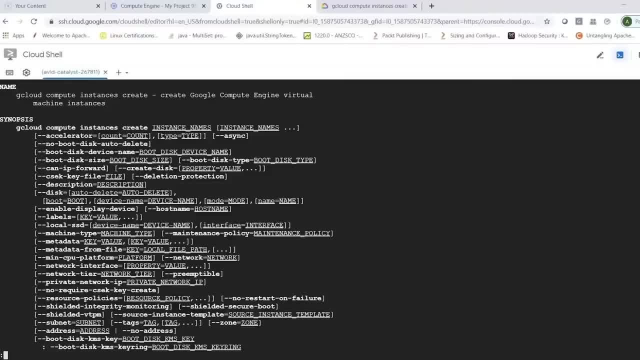 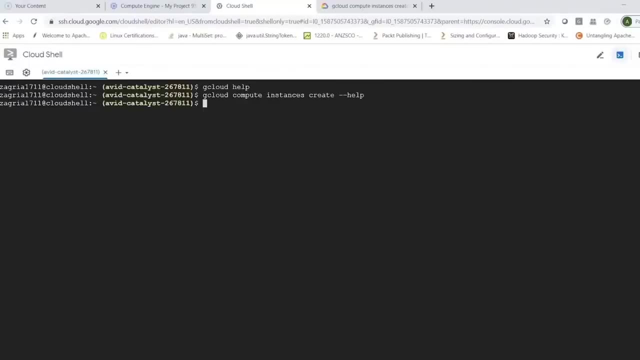 So that also can be used, So you can set up a Google Cloud compute if using gcloud. Now what we can do is, if we are setting up our SDK on our Windows machine, then we would have to do a gcloud init which basically initializes your configurations for gcloud. 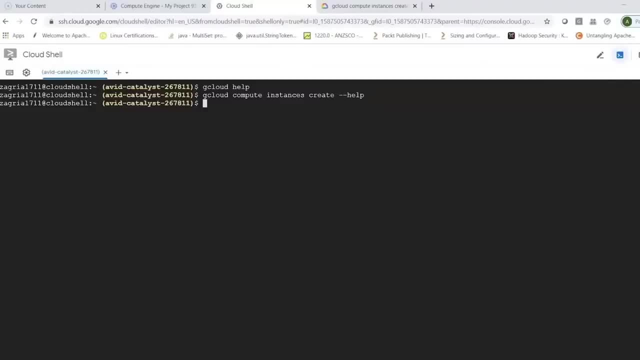 Now, here we are using a cloud shell which was started from the console and we don't have to basically give your gcloud init command because it's already initialized. Now you can always look at your default zone, you can look at your region. 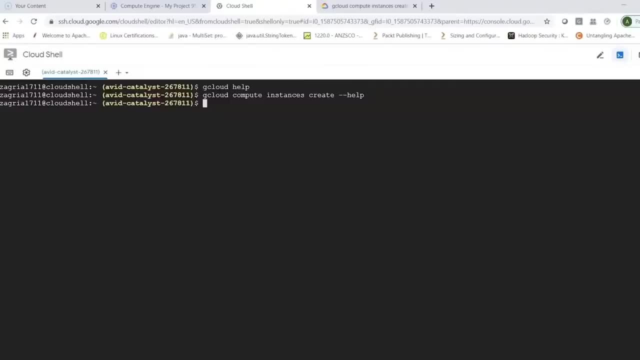 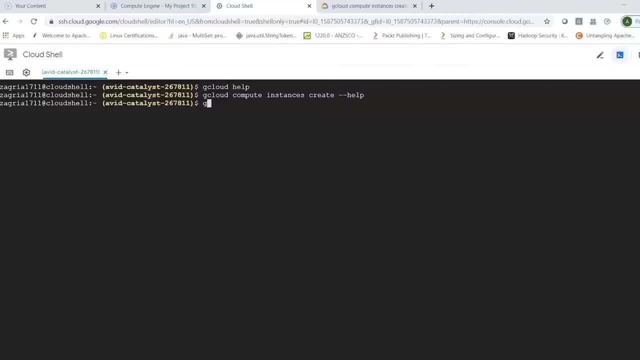 which is being used. So, for example, I could be looking at the metadata for my particular project by just doing a gcloud and then I can say compute and I would be interested in project info. So I can just do a project minus info. 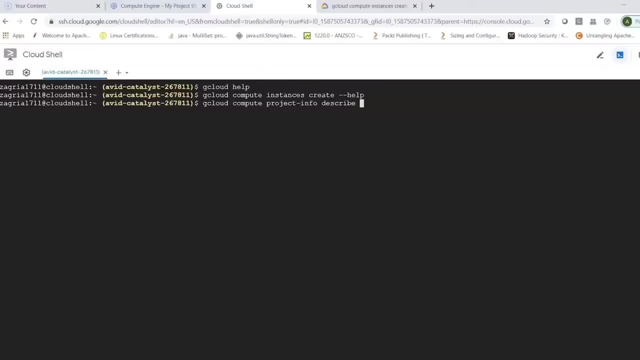 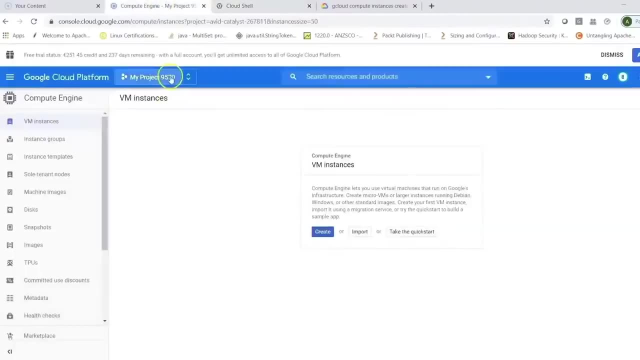 and then I can do a describe and then I need my project ID So I can say minus, minus, project. and I can get my project ID from here, So you can click on this one and that's my project ID, So I can click on this one. 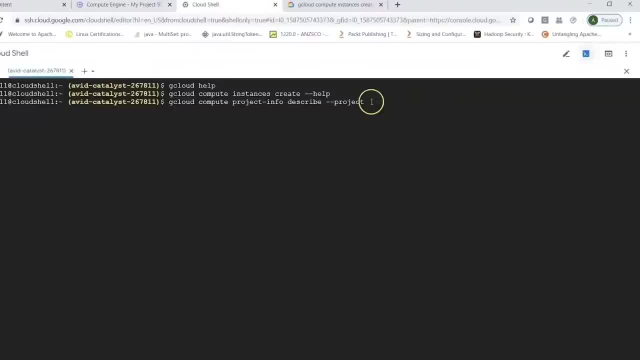 and here I can just do a right click, and if it does not paste, then you can do a control V and then I can try to look at my project info. So this basically will give me the metadata which is by default set. 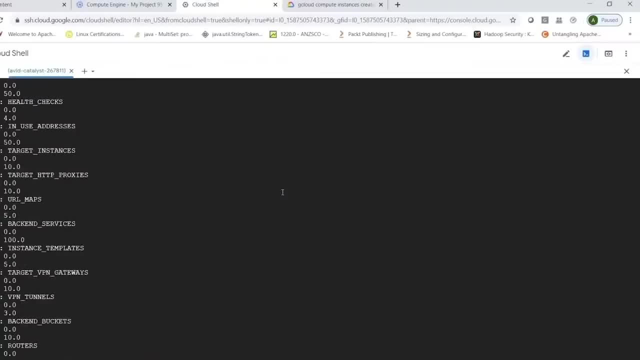 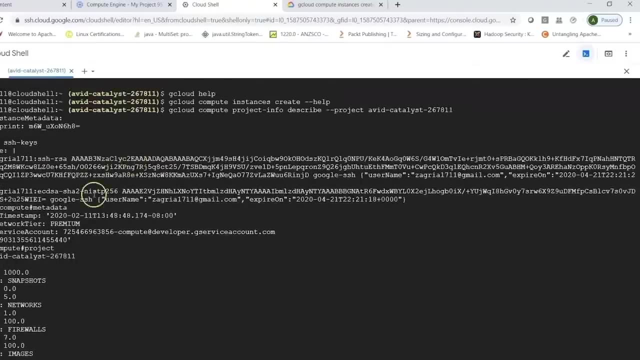 and we can always look at what are the regions or what is the zone which has been set. So if it has been set, so I'm looking at my details, it is showing me my SSH key and then it can be using your default region. 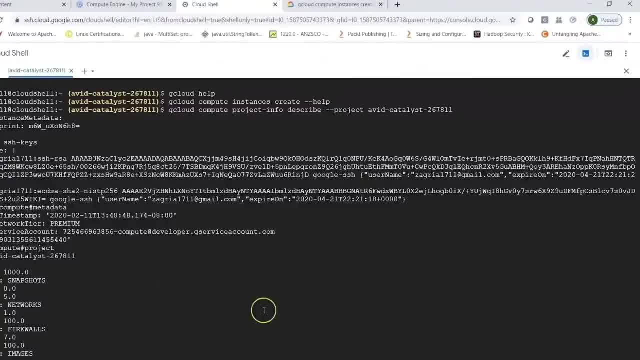 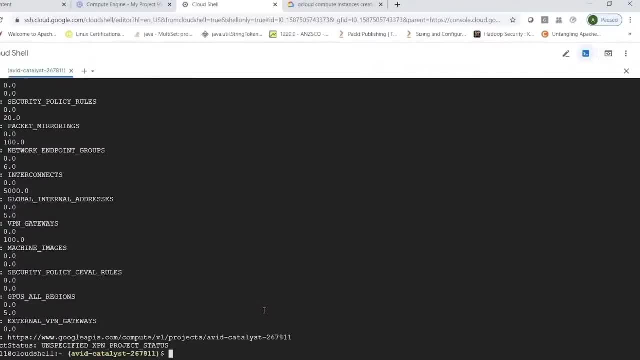 and your default available zones. It also shows my username and other details. So this is basically to look at the metadata which is available Now. at any point of time, I can basically say add metadata, I can basically choose metadata option and I can say my default region should be Europe. 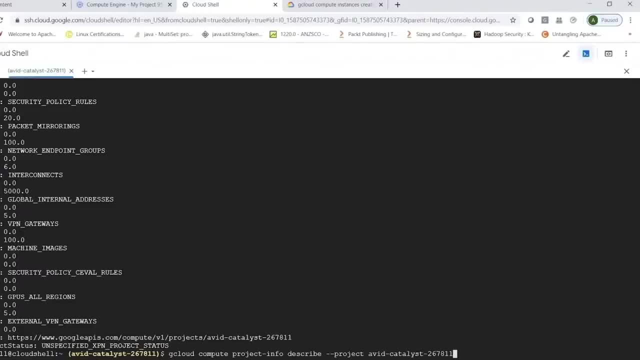 which I was choosing earlier, So I can just bring up this command again. and what I can do is I can say here, where I have gcloud compute project info, where I did a describe earlier. Now what I can also do is I can just say: add metadata. 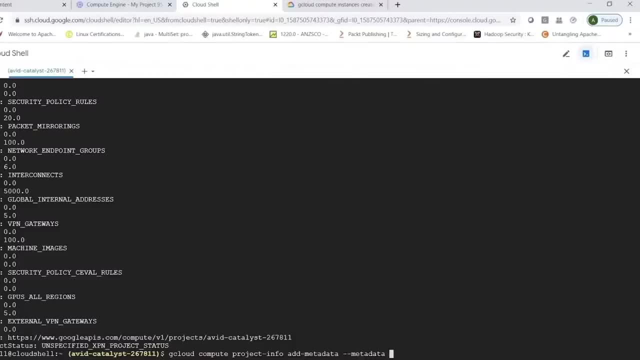 and then I can specify what is the metadata I would be interested in adding. I can then say Google compute default region and then I can basically give a region, for example Europe, and then I can say west three. And if you are not well experienced, 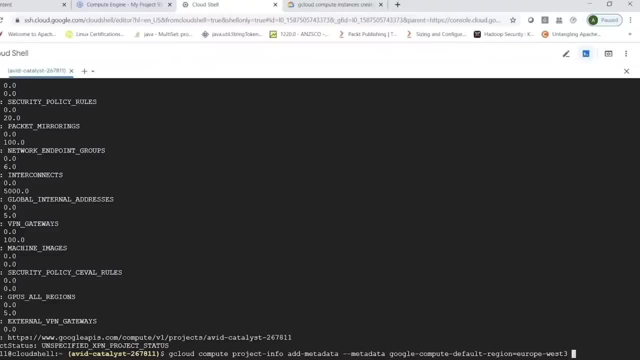 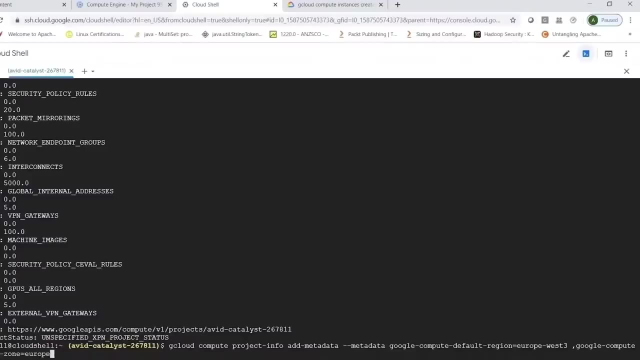 you can always do it from console or you can be doing it from here. So I'm giving Google compute default region, Then I can also give a Google compute default zone and then I can pass in a value for default zone. So I can say: Europe west three. 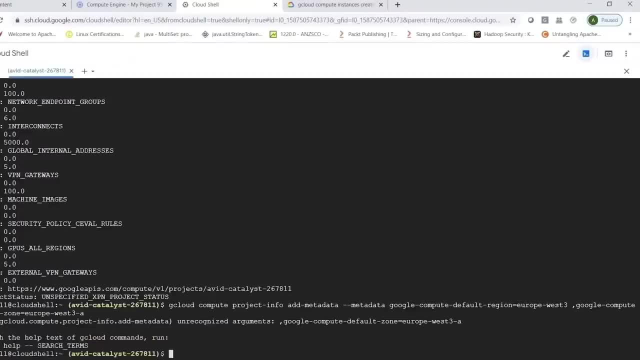 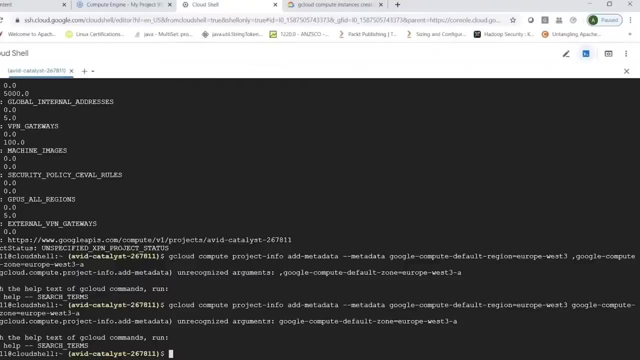 and then basically I can give an availability zone. So if it is basically giving me some error where I'm trying to pass in these values, so I can just give it this way. and then it basically says that if you can look into particular help to see what is the command. 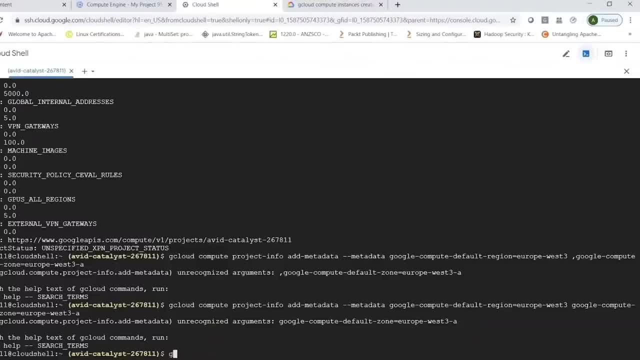 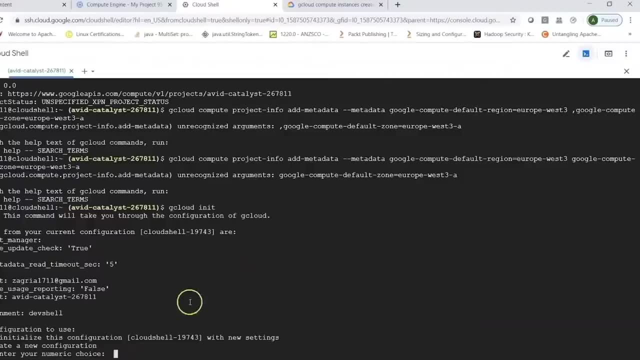 which you would have to do. Now. I can basically do a gcloud init here, initial configuration, and this basically says that it is initializing my default default configuration. It says: reinitialize this configuration from cloud shell. You want to create a new configuration? So if I had updated my metadata, then basically I could just do a gcloud init and I could be reinitializing my default configuration or properties which I have passed in. So as of now, I will not activate or change the default region. 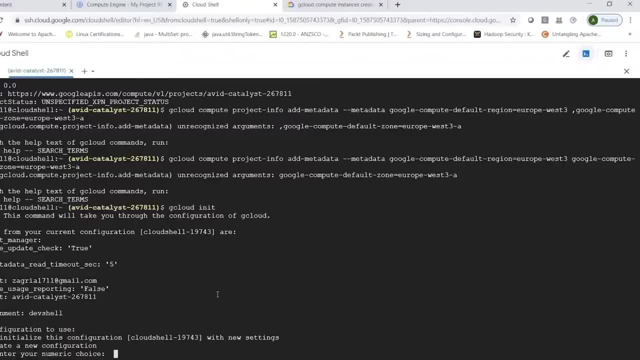 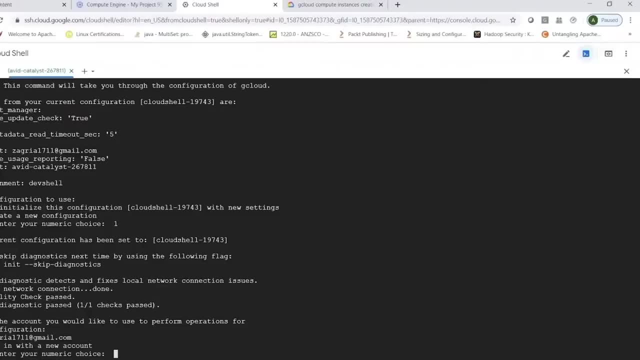 Let's go for a simple way in which you can create your compute engine. So, for example, I'll just say one, and it is reinitializing. It asks me what is the user name and let's select that. It says what is the project. 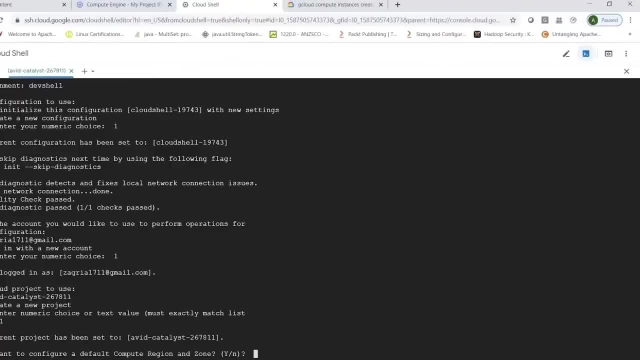 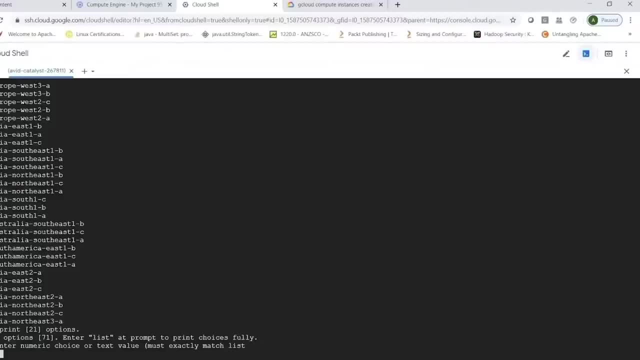 and let's select that. and do you want to configure a default compute, region and zone right? And I will just say yes, and basically then it shows me different options which we have here. So there are too many options here and then here: 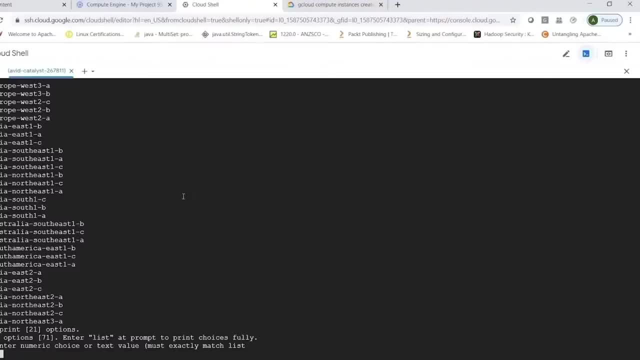 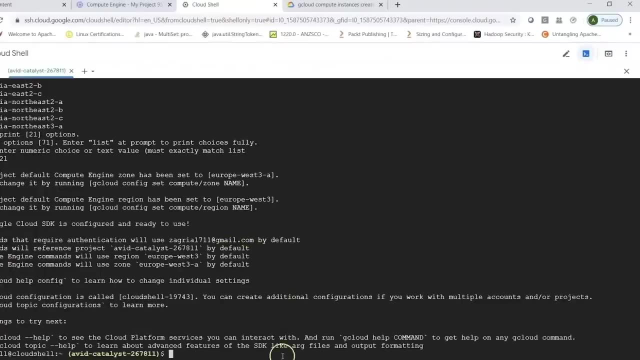 we were interested in Europe West 3, so let's choose 21,, right? And then that basically allows me to choose my region and my zone. So it also gives you some specifications. So it says your project default compute zone has been set to Europe West 3A. 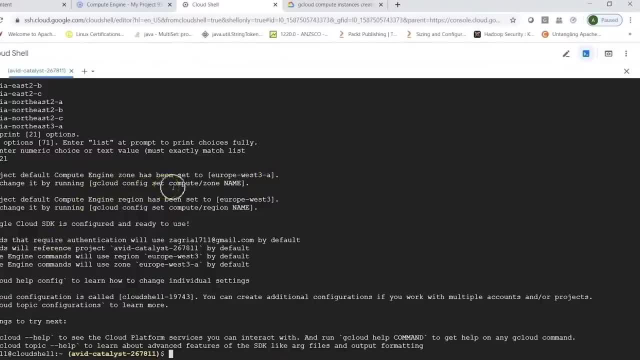 You can change it by running gcloud config set and you can give a compute zone right, So I can always give these commands. I can get help information here, So I can just say gcloud config set and I can be specifying the compute zone. 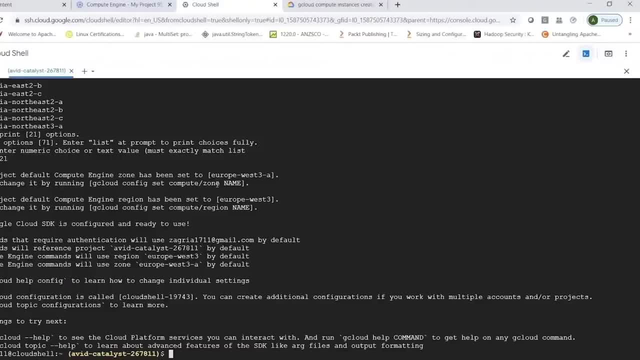 So I can say compute slash zone and I can give a zone. I can say compute slash region and I can give a region name if I would want to do it. or the easier way is like what I did right now. So you can basically do a command: gcloud init. 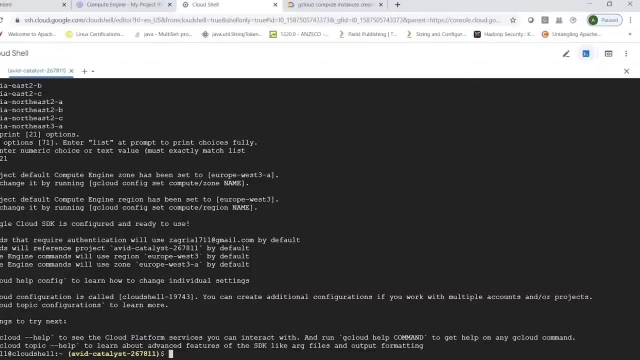 and then basically it allows you to change your configuration or set default things here All the times you can say gcloud config unset to basically remove a compute zone or a compute region. Now there are different ways. So if you were working on a Linux machine, 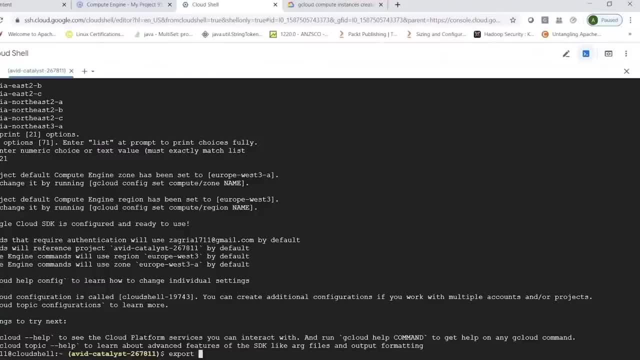 you could always use an export command, something like this, So you could do export compute- sorry, cloud SDK. and then you can say compute underscore zone and then give your zone Name or compute underscore region and give your region. or you could add it in your bash RC file, right? 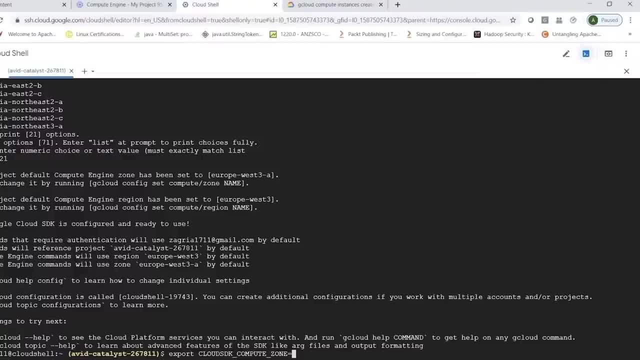 Now that is when you have your cloud SDK set up on your Linux machine or on Windows machine and you would want to specifically set a zone and a region for all your compute related resources. So we don't need to do that. The default settings are already given here, right? 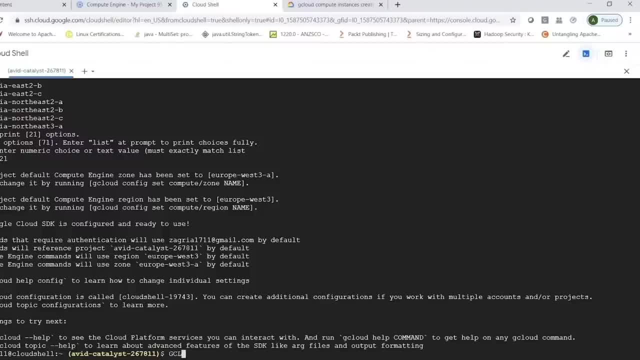 And what we can do is we can start by quickly looking into gcloud compute instances options. So I can say gcloud compute instances and then I can just do a list At any point of time. if you would need help, you can just do a gcloud compute and then say minus, minus, help. 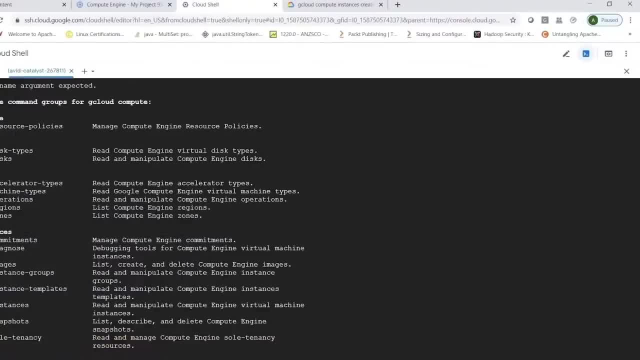 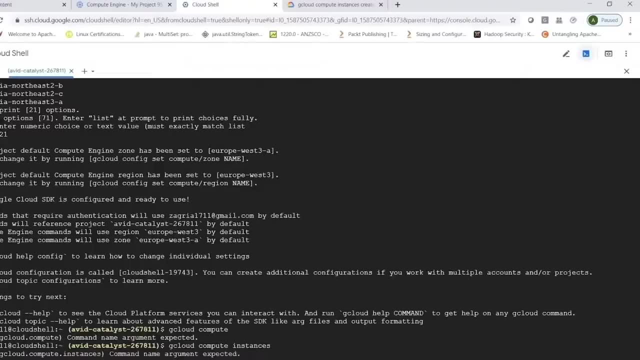 or I could just do a gcloud compute And that shows me different options which I have here, from which I use instances. I can always type instances and again hit enter and it shows me different options. What you would want to do. 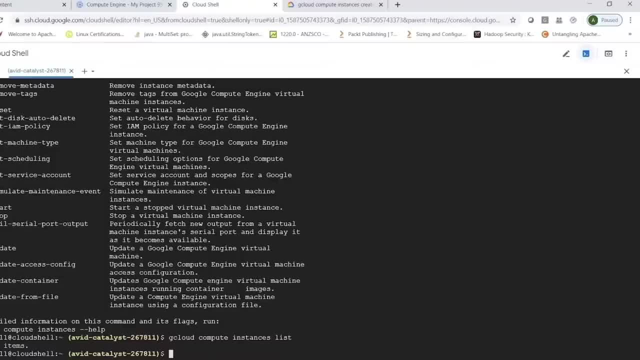 So I can initially just type list, which should show me what are the lists or what are the instances available, And as of now we don't have any instances. I can always do a list and then I can specify minus- minus format and then try to get the information in a JSON format. 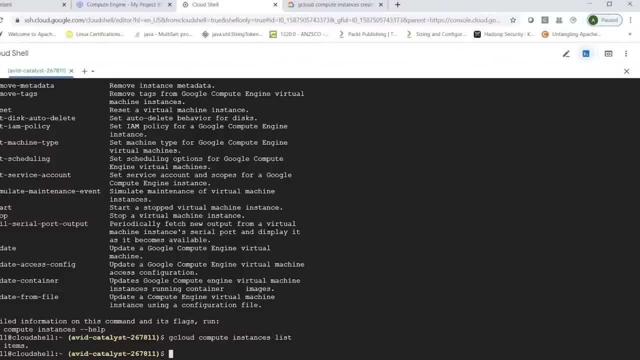 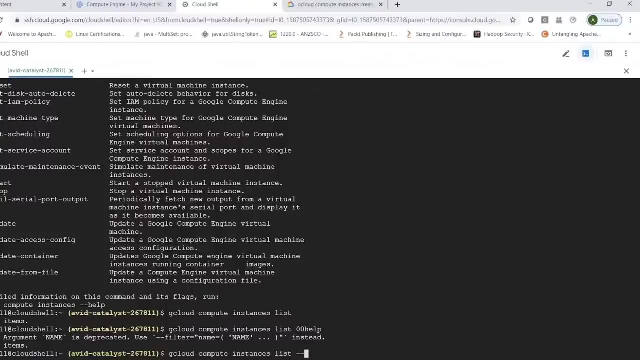 or YML or minus, minus format text, So you can always do a list, You can do a filter. So there are different options with your list and you can, you can try doing a help here And that basically shows you what are the options. 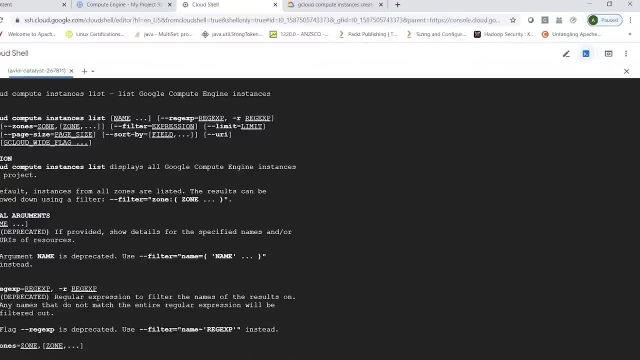 So, for example, if I do a help and it shows me with list, what are the things you can do So you can give a name, you can give a regular expression, you can say: in particular zone, you can use a minus filter. 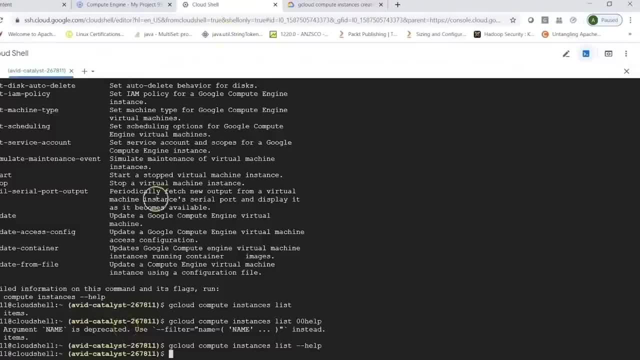 So there are different commands which are available, and you can always find all those options here, As I showed you earlier. so now what we would be interested in is basically going for your compute instances. I can always do a SSH and I can create an instance. 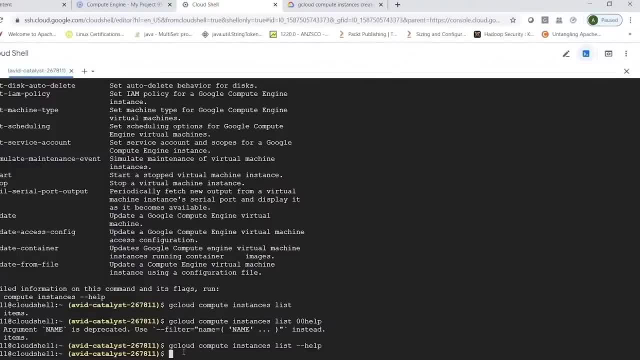 I can add and remove metadata right For my instances by giving a particular zone, by giving a particular region, And if you would want to do that Now here, what we can do is we can basically create an instance By just giving a name to that particular instance. 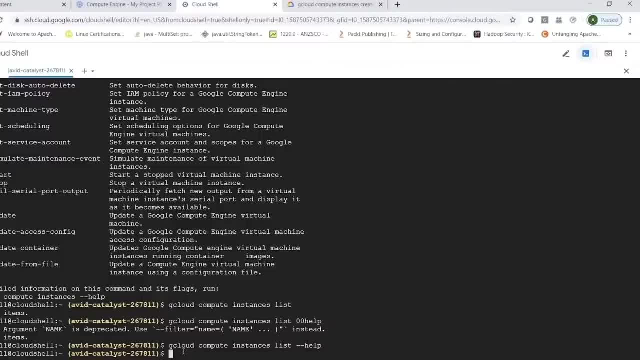 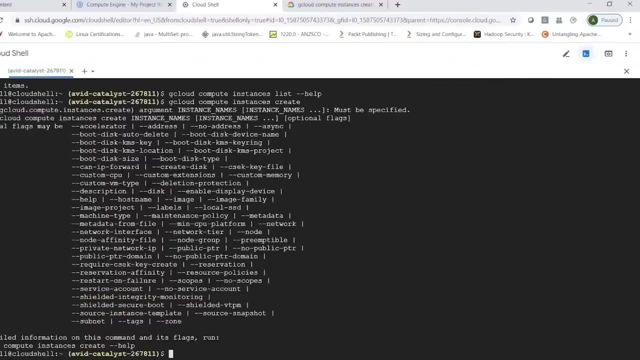 And we can then go back to our console and see what has it done. So I can say here: create, So that's an option, Let's see what does the create do. So it says, okay, you are giving a create option. 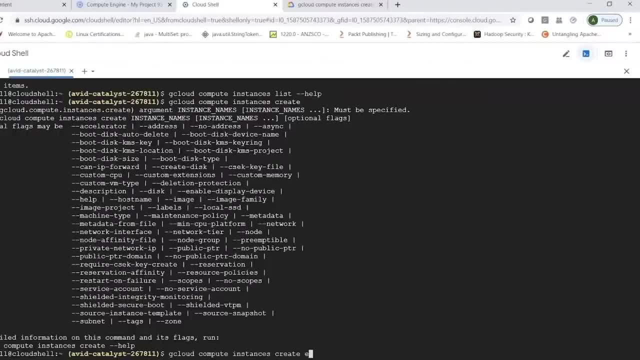 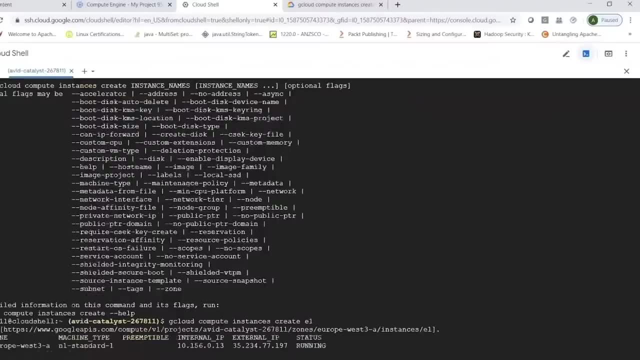 but you would have to give a name. So let's say let's call it E1 and that will be the name of my instance. And this one is an easy command from your Cloud Shell which basically creates an instance. you see the zone which has been set. it is the standard machine type. 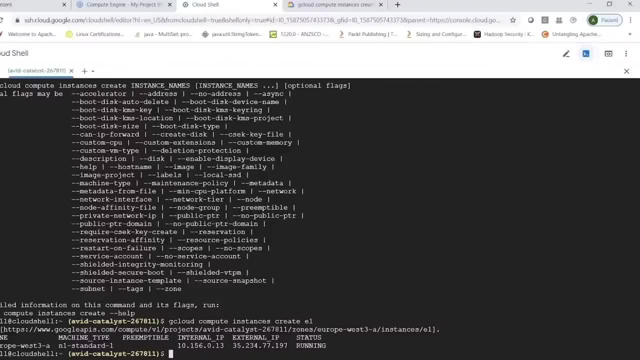 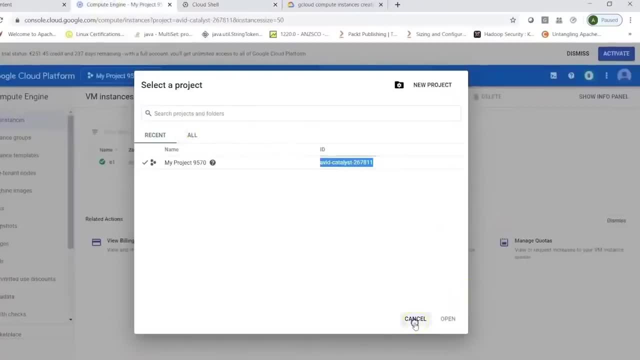 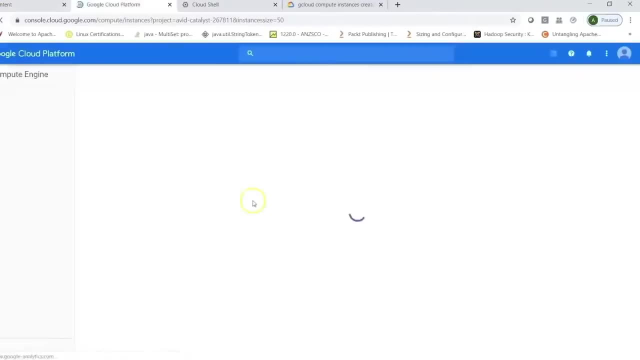 it is not pre-emptible. it has an internal IP and it has an external IP. now I have created an instance and here I can just go back, and then I can just do a refresh on this page and that already shows me the instance which I 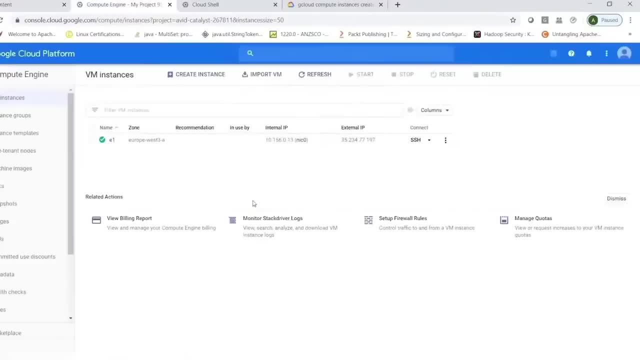 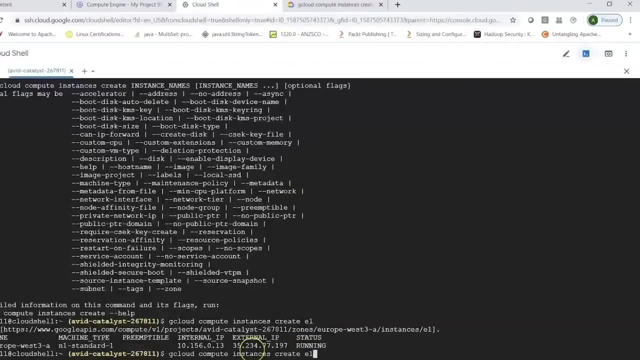 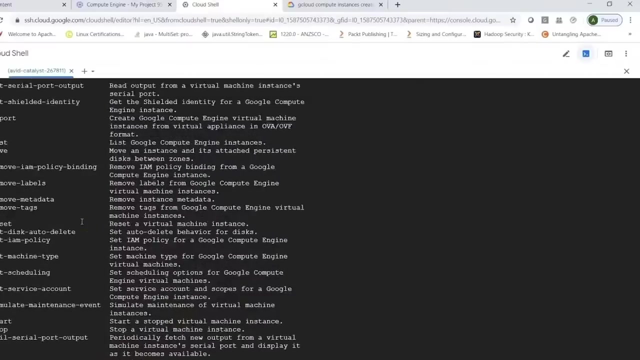 have created and then you can use the same method to connect to it using an SSH. so I have an instance created from my cloud shell and what I can do is I can basically look into instances and see what are the different options with instance. so if we did a create, right, you have an option delete. we did a create. 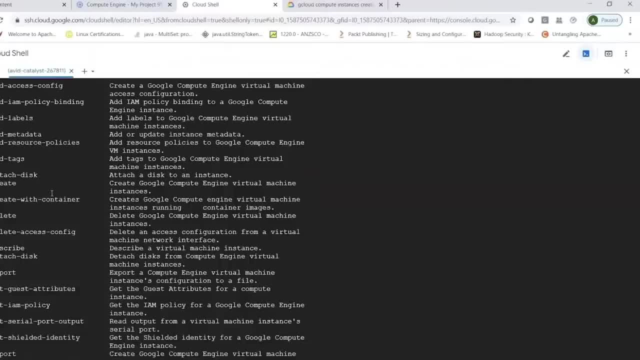 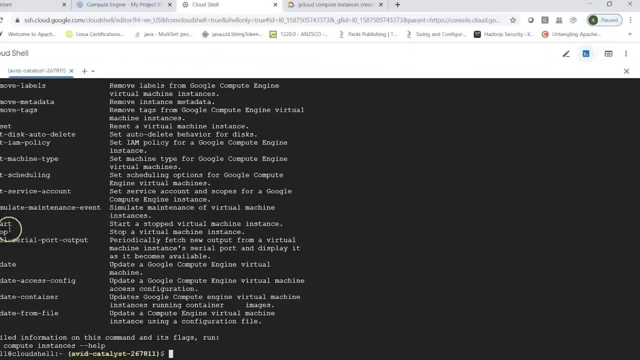 you have an option, delete, you can be in deleting the instance from the command line, or you can use other options so you can do a list, you can do a stop, you can start. so I can basically do is stop and let's say even, let's go ahead and do it stop. 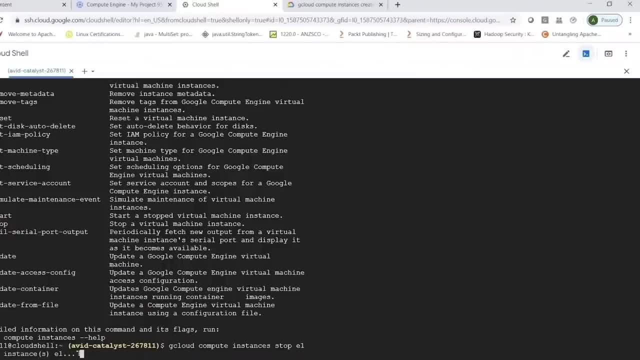 commands are pretty easy here to remember- or you can always use the help option- and now I'm trying to stop the instance and then basically I can go ahead and delete it. so this is a simple way where I created a instance from the command line or from the console which I showed earlier, and similarly you can be. 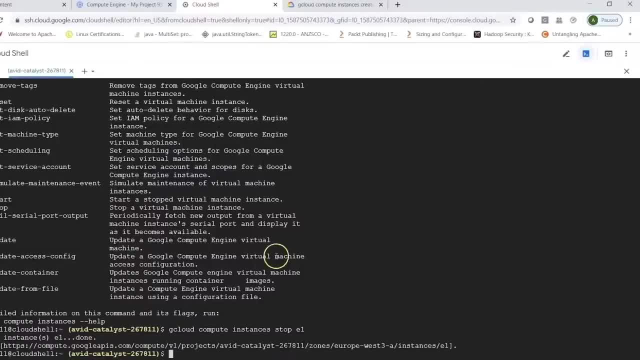 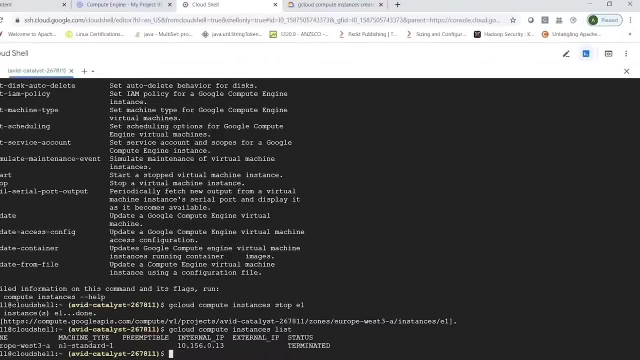 working with other options. So now I've created stop the instance, Let's do a listing to see if my instance shows up. It shows up right And it says the status is terminated. So you have stopped it. It's in the terminated status. 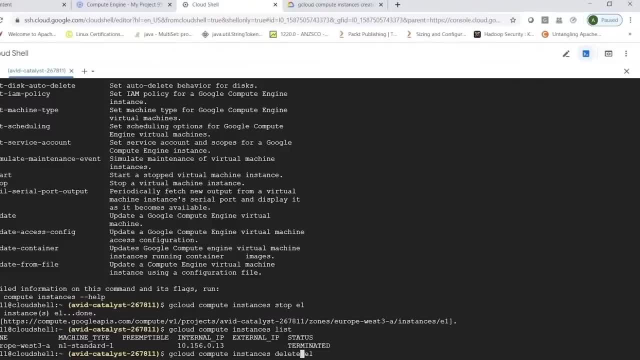 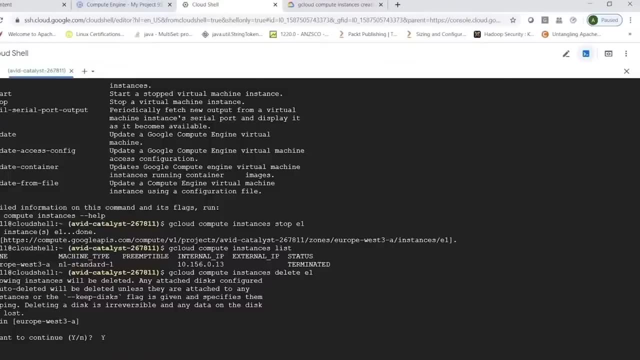 And now what I can do is I can go ahead and delete it. So it says this will be lost. Are you sure you would want to continue? Just say yes, And that should take care of deleting your instance. So this is a quick demo on creating your instance. 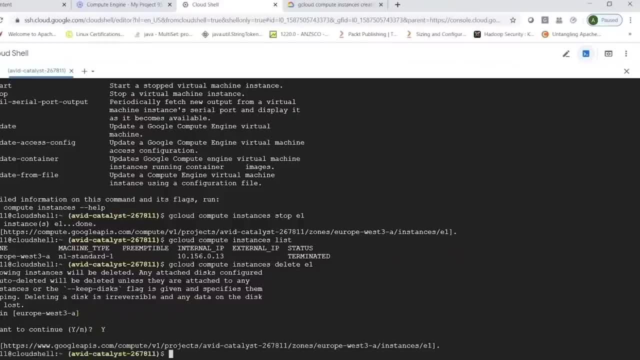 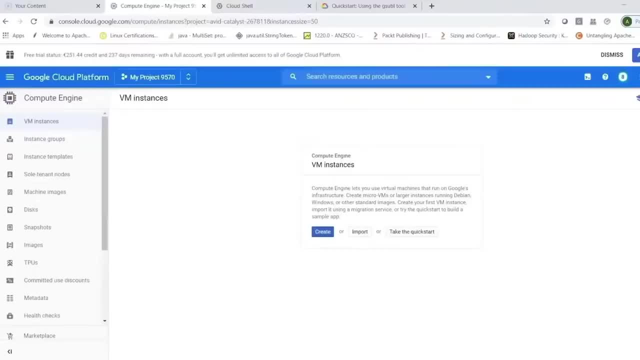 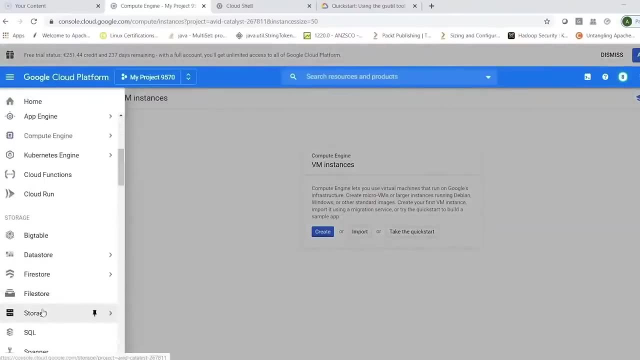 We have already seen how you can connect to these instances using SSH. Now that we have created instances, let's also see how to use Google Cloud's storage service, which can be used to load data or upload data. So for this, we will have to look into your Google Cloud storage options. 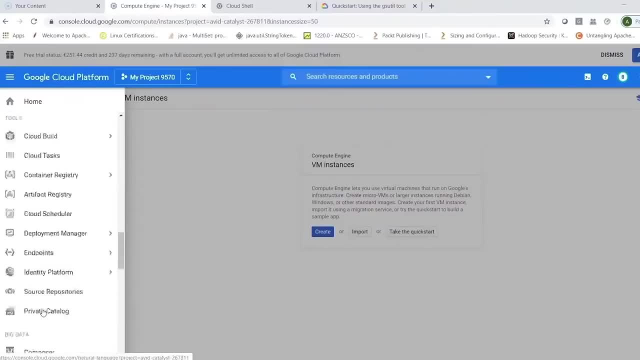 And here you can look in cloud storage. So let's go back here on the top, which shows me different services which we have here, And let's look into storage. So this one shows me your storage option. Now you can click on browser. 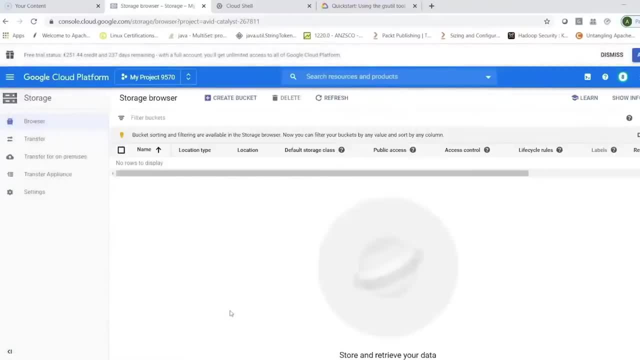 And that basically shows me your storage browser, which shows me on the top, you have options for creating a bucket. Now Google Cloud storage allows you to store any kind of data here. The easiest and the simplest, the easiest way would be by using cloud console. 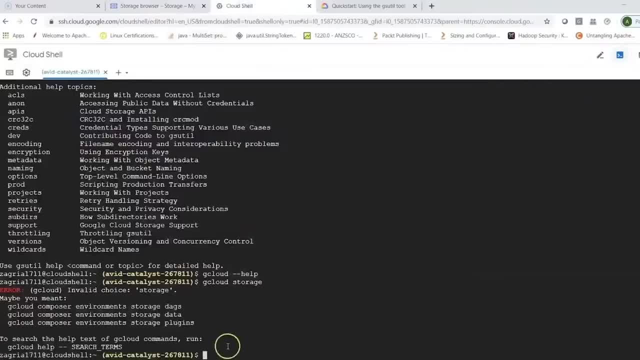 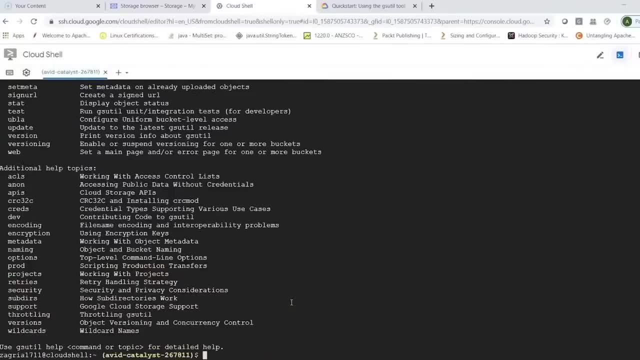 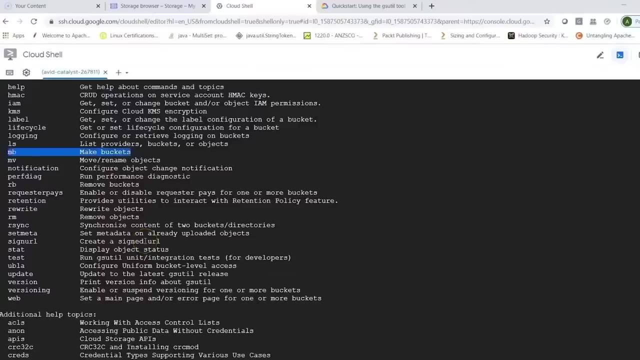 Although you can again use cloud shell And in that you can use your gsutil command, And gsutil basically has different options where you can be using. say, for example, I would want to work on buckets, So I can be using MB and then I can use my command line option to create buckets. 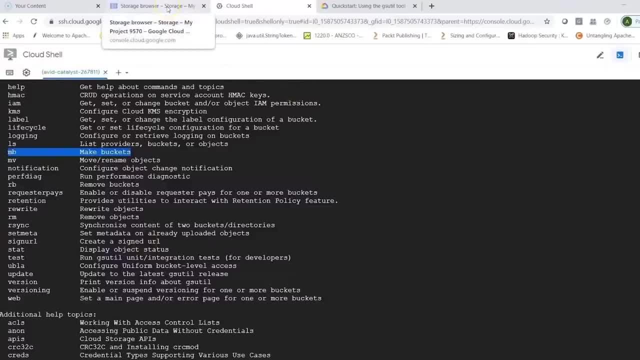 I can put in data there, I can browse it and I can access the data from command line. So I can put in data there, I can browse it and I can access the data from command line. So I can put in data there, I can browse it and I can access the data from command line. 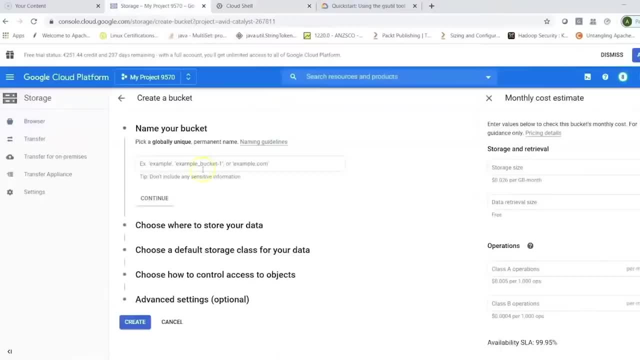 So let's create a bucket here, Let's click on this, Let's give it a name. So let's say my data important. That's the name. Now I can click on continue straight away. I can look into all of these options if I'm interested in. 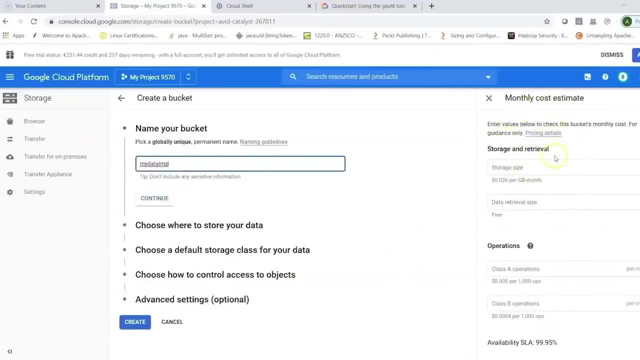 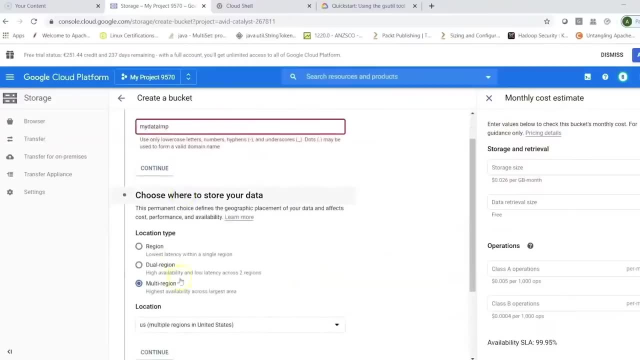 So you can basically be looking at your monthly cost estimate in the beginning. Now I can click on continue or you can say choose where to store your data, And this one shows you different options. So you have region specific. So let's also give the bucket name with all lower case. 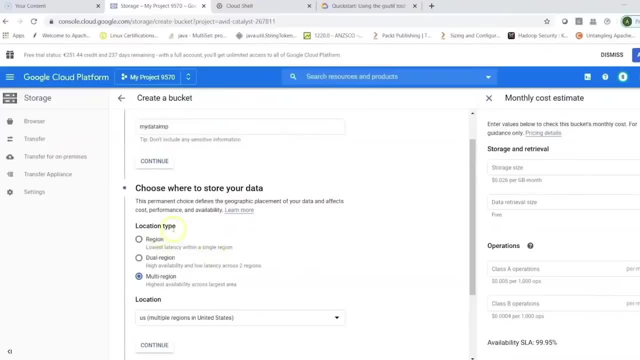 That's what is required. Yeah, So, coming back to the location type, you can choose multi region, which basically allows high availability, So your bucket or your storage option will be accessible across regions. You can also give dual region and high availability and low latency across two regions. 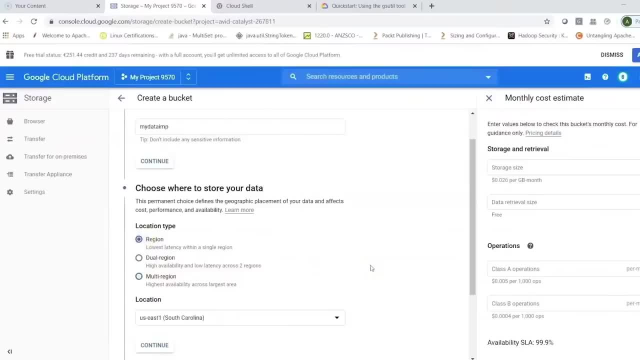 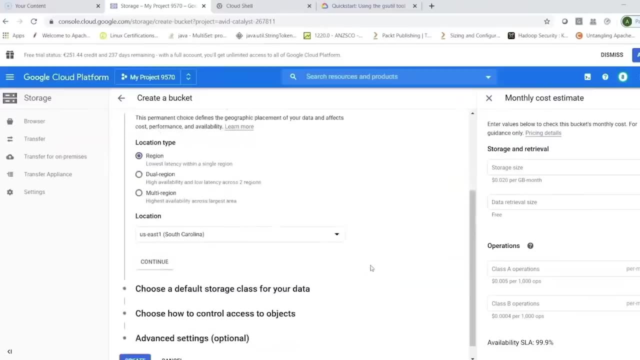 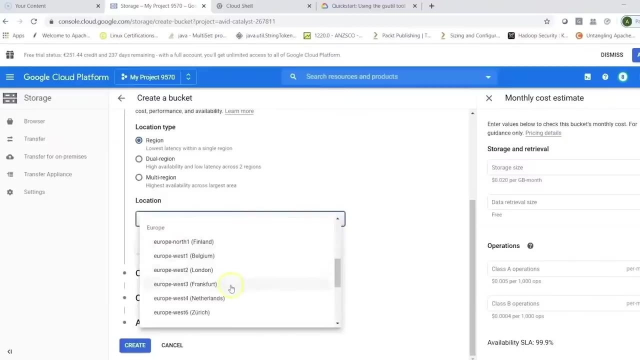 I can also say region specific. so for our use case We can just give region specific which can keep our costs low. But in business use cases you would be going for multi region. Now, here you have location and I would again go for say Europe, and let's choose Europe West 3, Frankfurt. 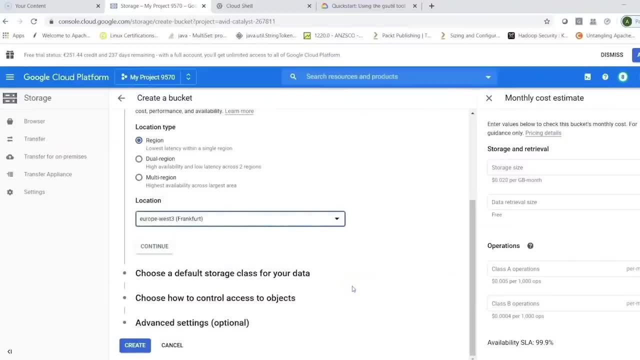 It is always a good practice that when you create your instances, when you create your storage or you use different services, try to have a geographical region chosen and then you would try to put Things or your services within the particular region, within a particular zone, unless you would want to make it accessible and available across regions. 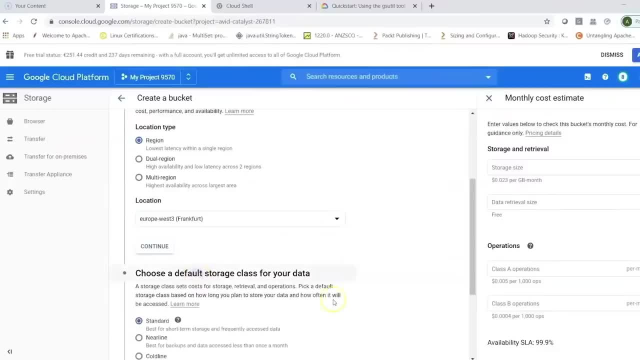 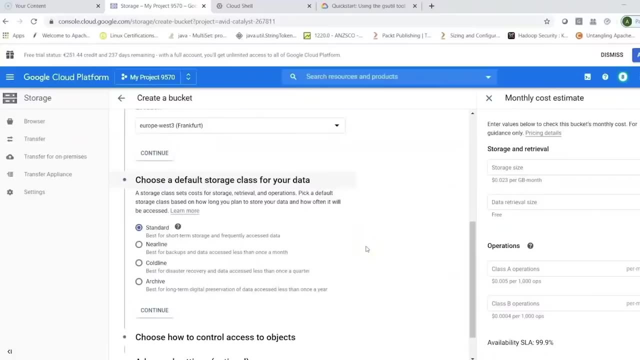 Now I can then choose a default storage class. So when you say default storage class, there are different storage class and each one is for a different use case. So you have standard which is best for short term storage and frequently access data you have near line. 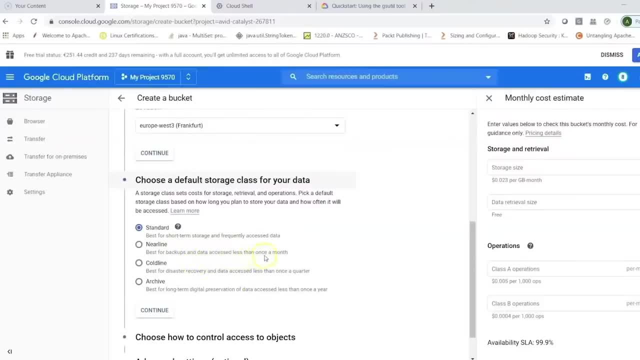 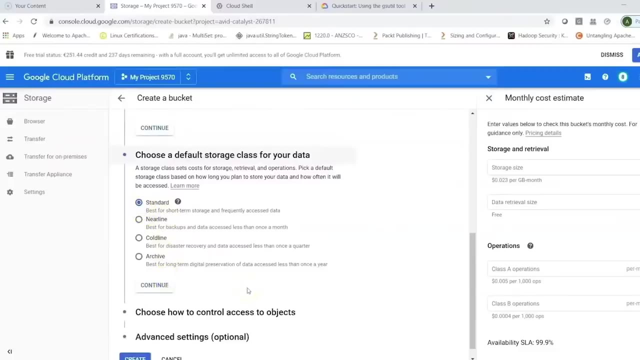 So this is basically best for backups and data access. less than one second. So you can also have cold line. So these are basically like your cold storage or freezing storage, which you might have heard generally as terms. So you can choose one of these storage classes depending on what will be the use case for this particular storage bucket. 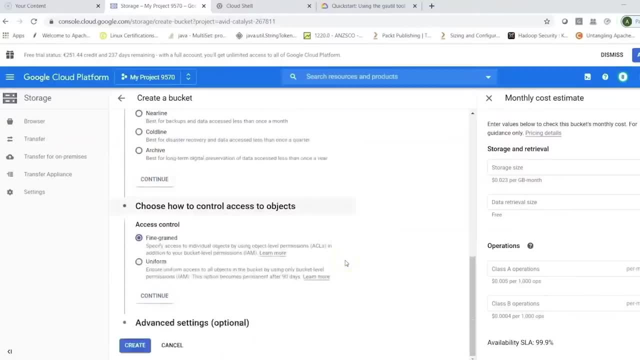 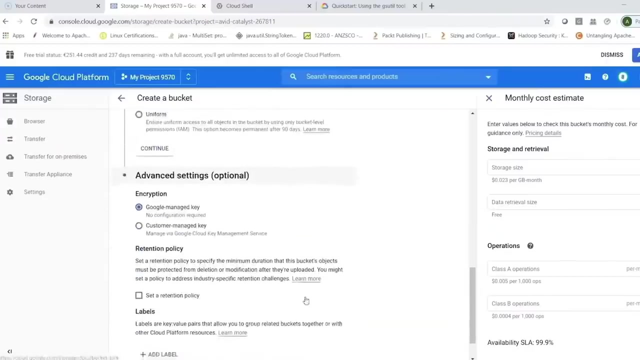 So let it be standard Now how to control access to objects. So you can basically say: specify access to individual objects by using object level permissions. Now you can give permissions to The bucket. you can just say uniform access to all objects in the bucket by using only bucket level permissions. so you can choose that. you can also go into advanced settings and here you can see different ways in which you can have configuration set up. 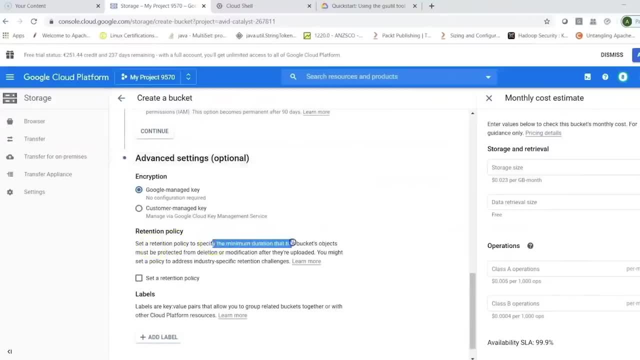 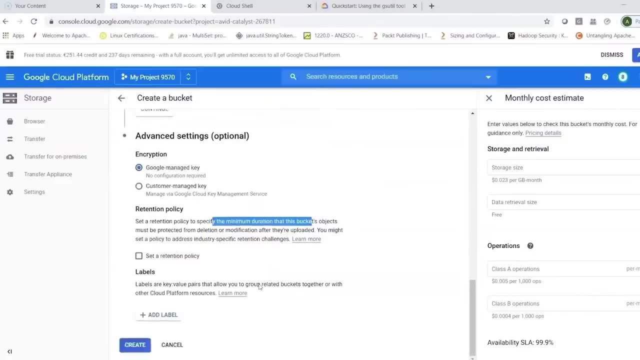 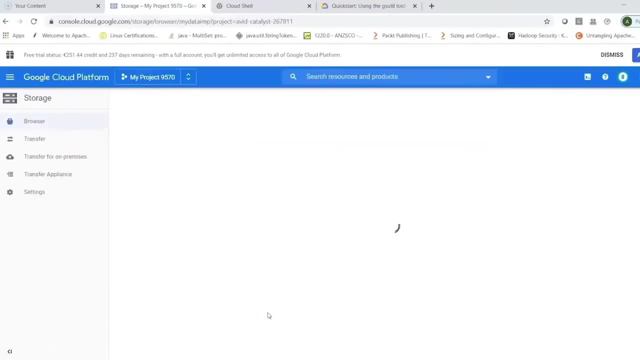 Now you can also have a retention policy to specify the minimum duration where that this buckets object must be protected from deletion and you can set a retention policy. will not get into all that, we will just first Just try creating a bucket. So just click on create and that should create your bucket. 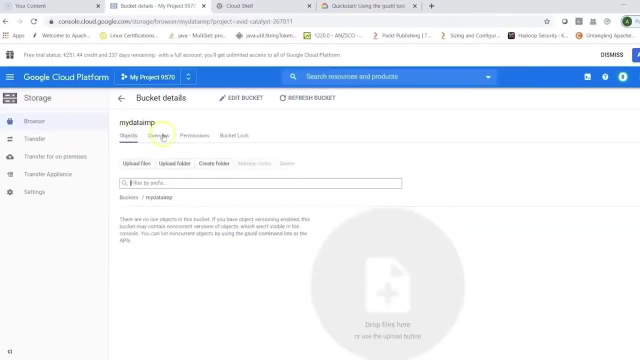 Where in I have my bucket. Now I can click on overview to see the details. What is the region, which region it belongs, What is the storage class? Any time you can always click on edit bucket and make some changes. here You can look at the permissions. so bucket uses fine grand access allowing you to specify access to individual objects. 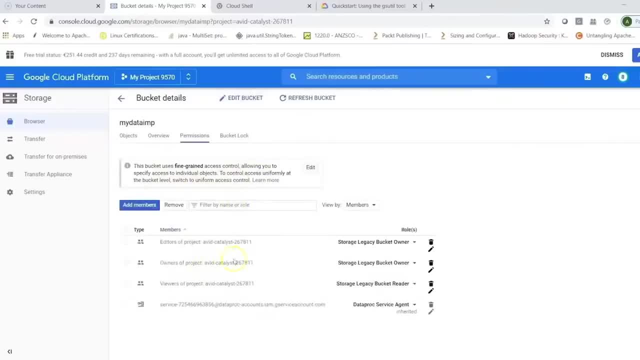 And then you can Basically look at who has access to this. so in my case, editors of the project- they basically are the bucket owners, owners of project, viewers of the project, right, and you can basically choose what kind of access you need. So for this you can always go into cloud storage and then you can decide what kind of access you would want to give: whether that's a storage admin, it's an object admin, object creator, object viewer and so on. 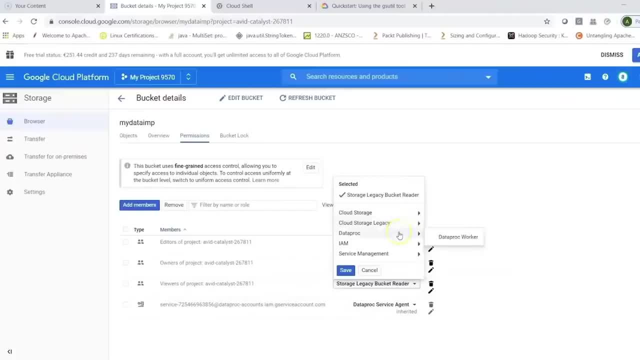 You can always look at storage legacy And for any other services, depending on what API is you have enabled right, you can always control your permissions. so right now it is storage legacy bucket reader, and that's fine, and this one is bucket owner, and then might be. I was using some other services, like data proc, which uses cloud storage, and that's why I've given data proc service agent also. so these are some of the members you can remove. 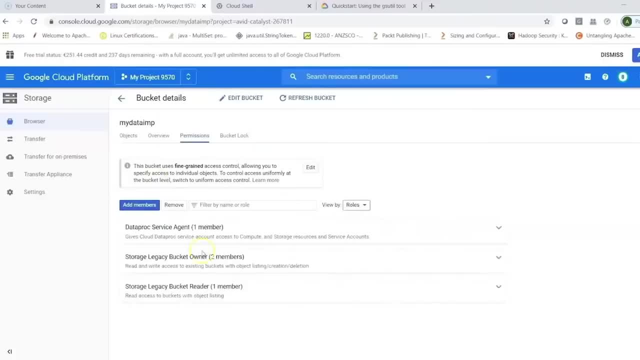 You can view by specific members. you can view by roles. so what are the different roles which have access to this? so it says storage legacy bucket owner. There are two owners based on this particular project, so these are auto controlled. but then you can add or remove machines. you can save storage cost by adding a lifecycle rule to delete objects after the duration of current retention. 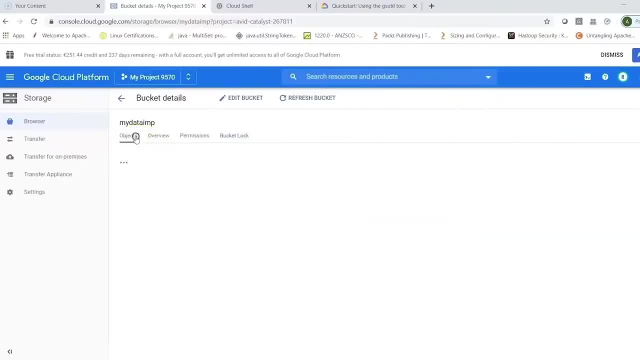 Policy, so you can add different policies And you can basically Control your bucket. now my bucket is already created, right, so i can go back, and then i see my bucket is already here. i can click on this option and you can anytime edit the bucket permissions you. 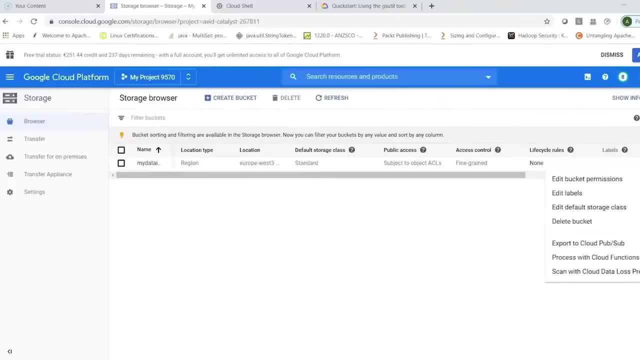 can edit the labels, the default storage class. you can just go ahead and delete the bucket. you can export it to cloud pub sub. so basically, if you would want to have the content from this bucket being accessible in a message queuing system, you can go for pub sub. you can process with cloud. 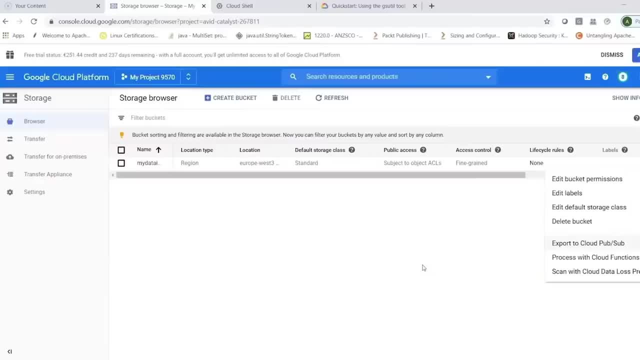 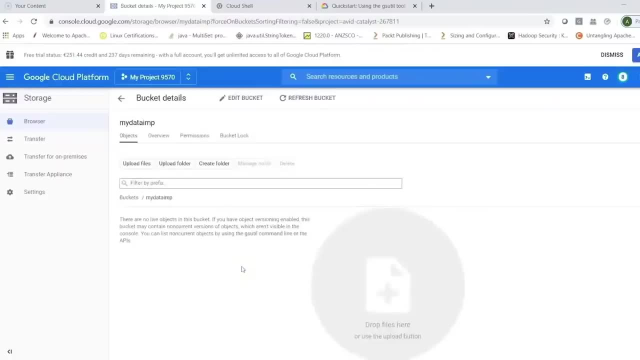 functions and you can scan with cloud data loss prevention. so there are different options which are available. we can always select this bucket and delete it. now i can click on the bucket and that basically shows me different ways in which i can upload some data here, so i can just 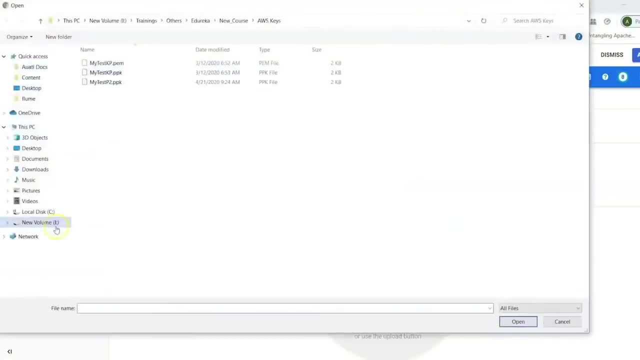 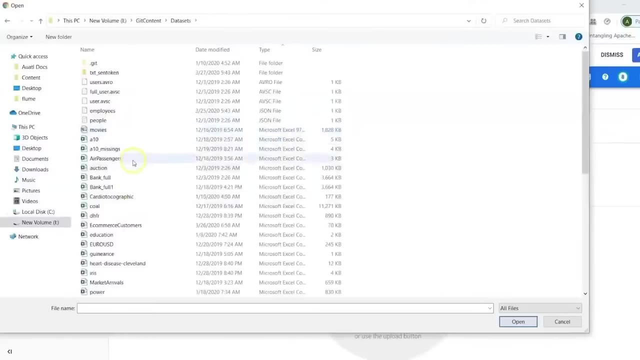 click on upload files and here then i can choose some files. so, for example, i'll go in here, i'll go into my bucket and i'll go to my bucket and i'll go to my bucket and i'll go to my bucket and i'll data sets and i have different data sets. so, for example, let's choose this one which is a csv file. 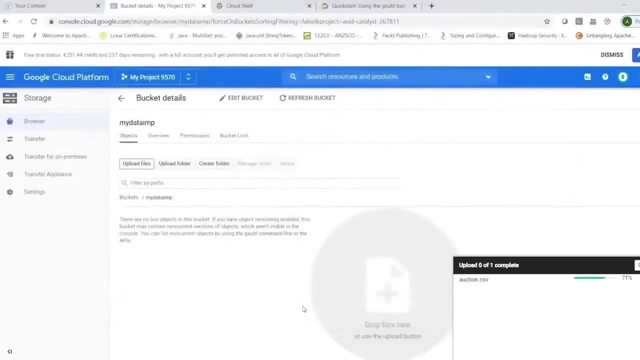 and then i'm just uploading this to my cloud storage. right, it's as simple as this. so you can drag and drop your files, or you can just upload your files and my file is uploaded here. now i can basically edit permissions for this one right. so this is in the bucket. so anyone who has 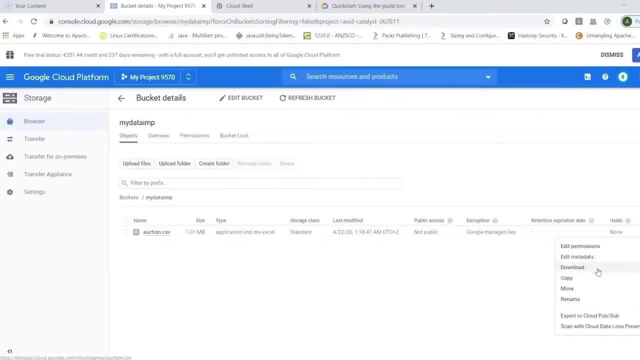 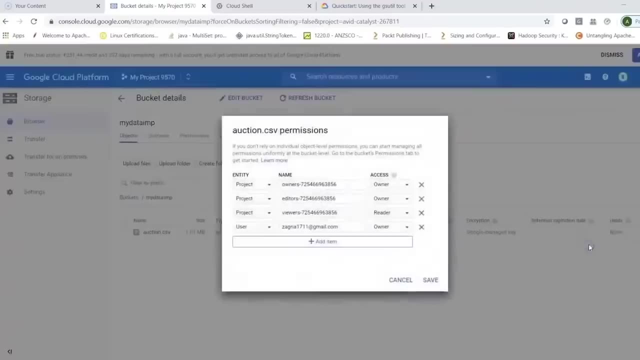 access to this bucket can basically download this file. it can. they can copy, move or rename this. you can export it and you can look at the permissions of this file. so let's look at edit permissions and it says for this project: whoever is the owner, it has access. i've also given a 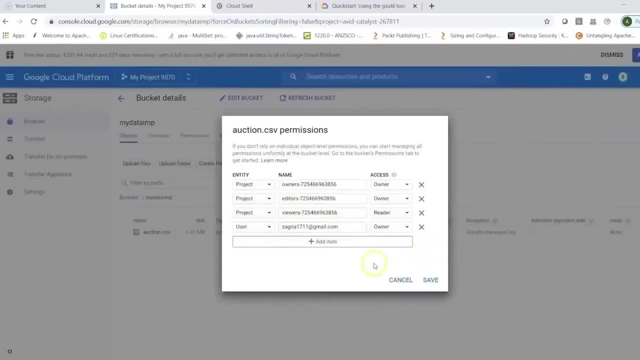 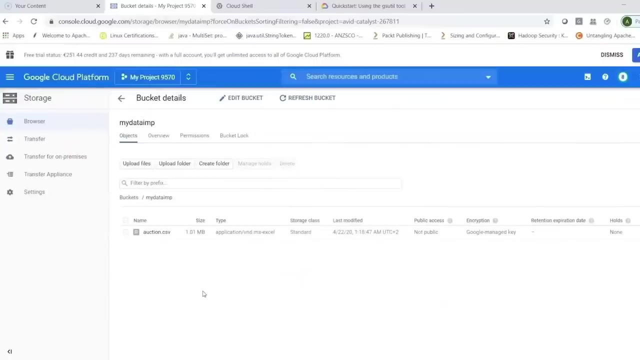 specific user, my gmail id and i've given access. so at any point of time you can just say add item and then you can start giving different kind of accesses. so let's click on cancel here. now my data is already uploaded into this particular bucket and that's a simple usage. 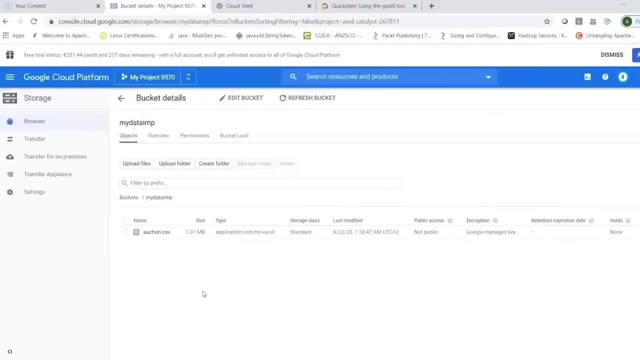 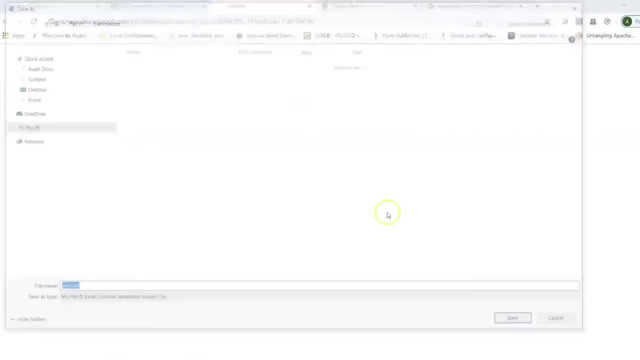 of your cloud storage. now what we can also do is i can basically select this and i can delete it. i can also create specific folders and then basically load data into it. i can click on this one, i can just do a download, and then i can download it anywhere on my machine. so 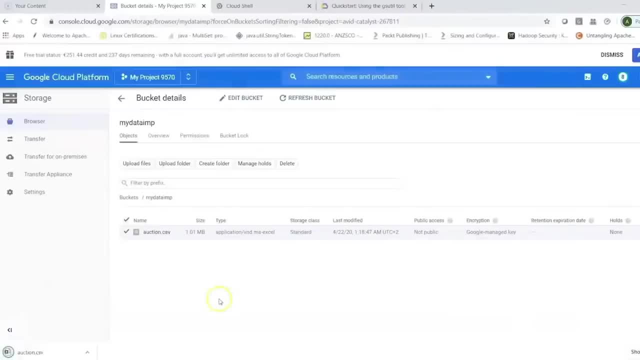 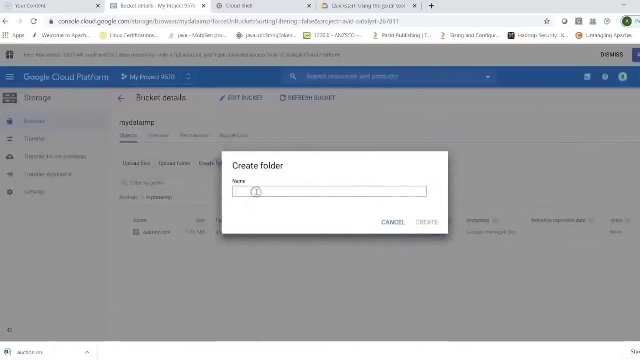 let's go to desktop and let's download this file. so we not only uploaded some content in the bucket, but we also downloaded that in a different location, which will be accessible now. what i could have also done is i could have created a folder here and i could have specified, say for: 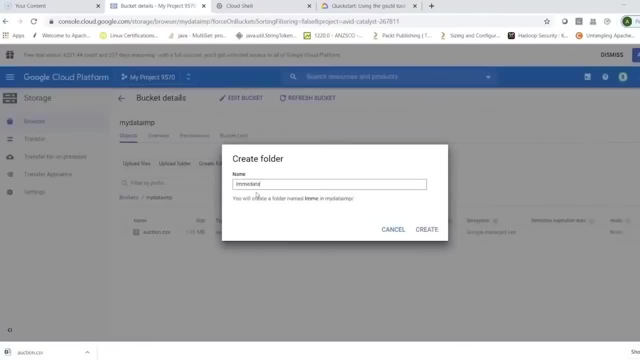 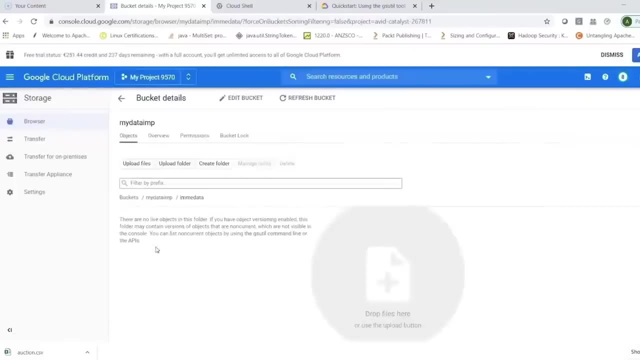 example, immediate, immediate data. okay, and i'm clicking on this one, so that's my immediate data. i can click on this one and now i can upload my data specifically to this particular folder by using the same mechanism. you can just do upload file. let's choose air passengers. 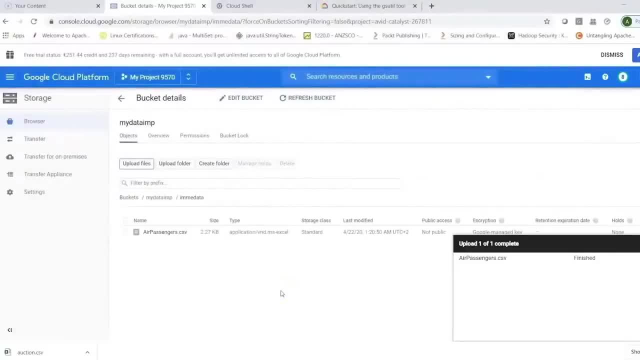 let's do a open and my file will be uploaded so you can always choose what is the retention expiry date for this one. so as of now, there is nothing right, but you can be deleted. objects can be deleted or modified until they reach their minimum duration. you can. 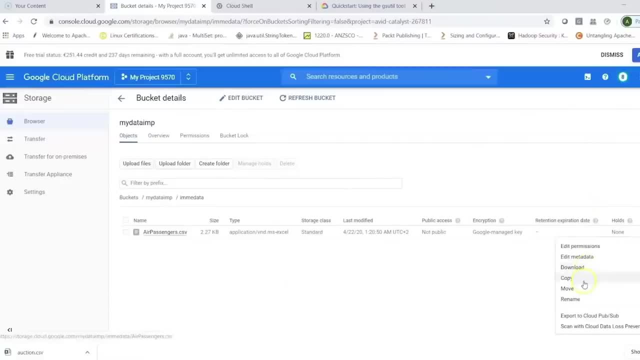 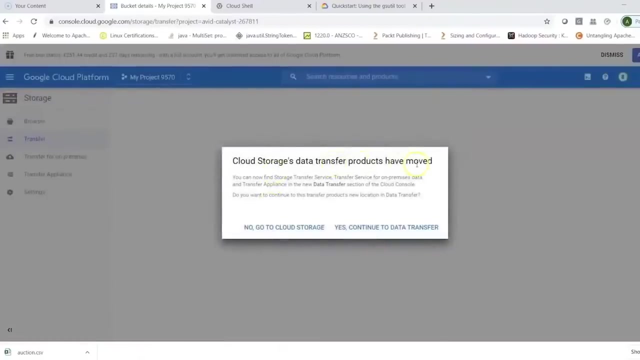 control all of that. you can basically download it right, you can copy it and you can move it and rename it. so this is a simple example where i created a particular bucket. right now if, for example, you click on this transfer so it says cloud storage data transfer products have moved. 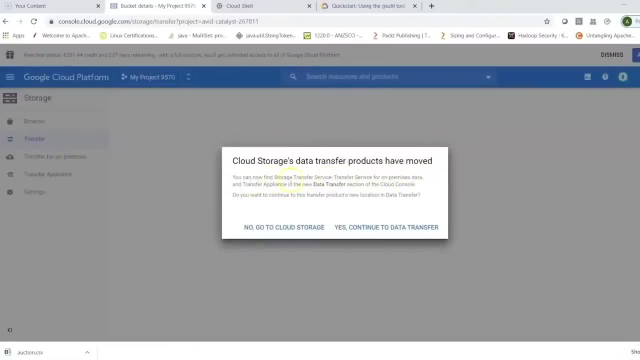 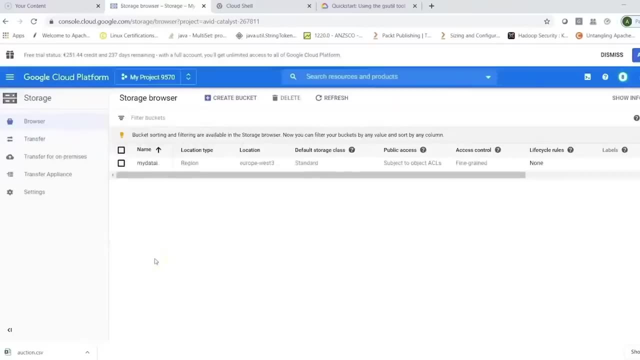 you can now find storage transfer service on premise data and transfer appliance in new data transfer section. right, so you can always go back to cloud storage. you can also look at transfer options, which are mainly when you are using a on-premise service and you would want to. 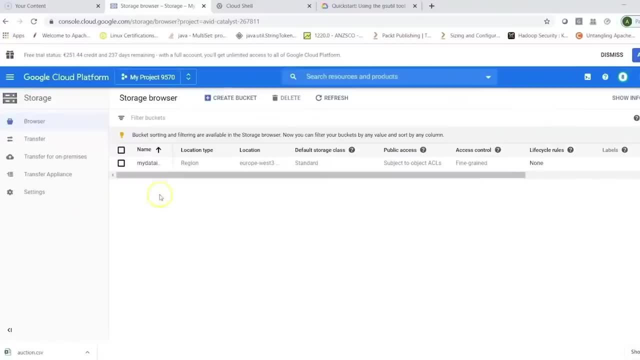 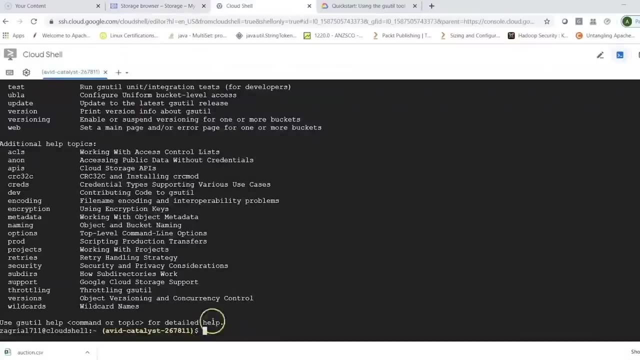 upload data in a google cloud right. so this is my bucket here. now i can go to cloud console and here what i can do is if i would be interested in working, so i can just say gsutil, right, and then we have, for example, let's try a help, okay, and that basically shows me my gsutil. 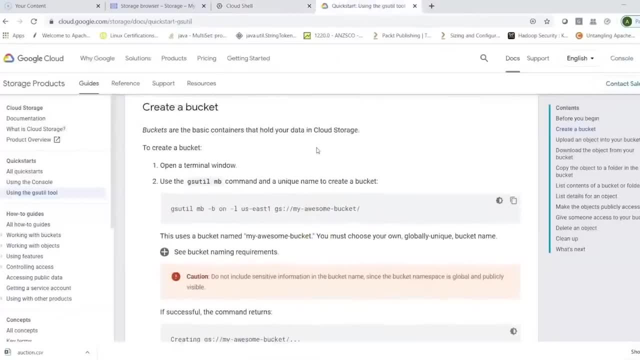 you can always go to quick start gsutil tool, and this is one more way wherein basically you can do it from the command line, so working with buckets. so you can do a gsutil mb minus b and then on a particular zone if you would be interested in, and then you can say gs colon and 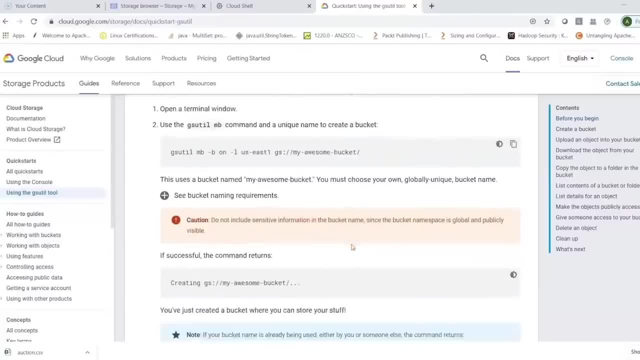 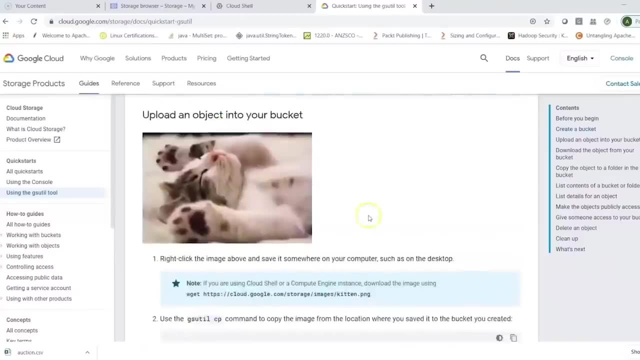 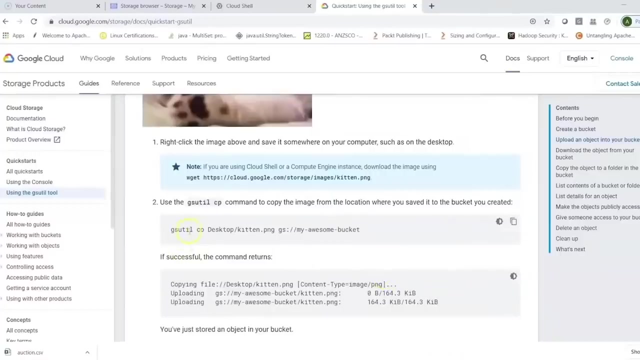 give a name. so my awesome bucket. this is how you will create a bucket which will show you it is creating a bucket and then, basically, you can upload an image or some data from internet. you can just do a wget, download the file and then you can just do a gsutil copy. 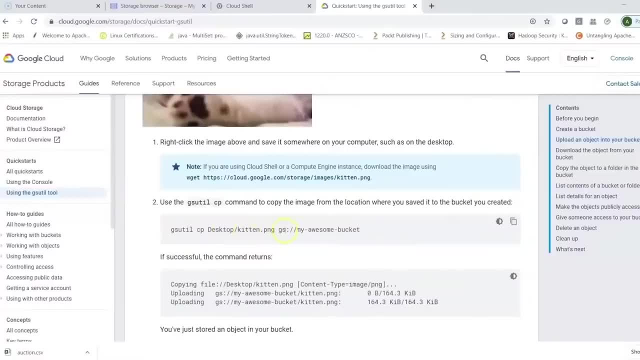 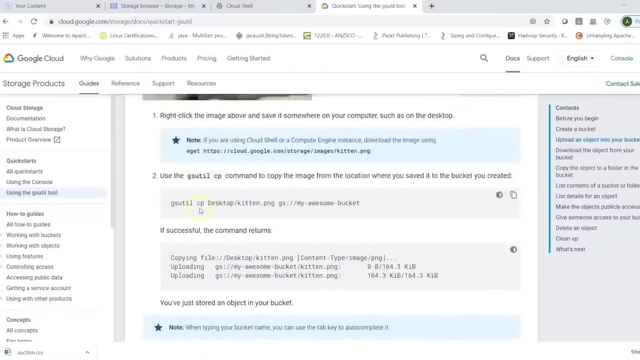 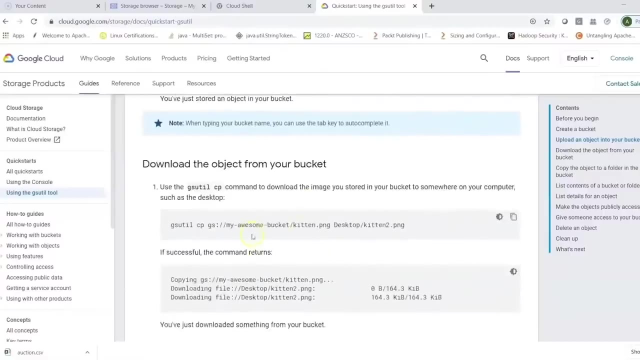 command and that, basically, will pick up the file from your cloud shell location, put it in your bucket. once you have done that, you can always do a copy right? so here you are doing a copy from your local machine, that is, your cloud shell machine, to your bucket, and you can do. 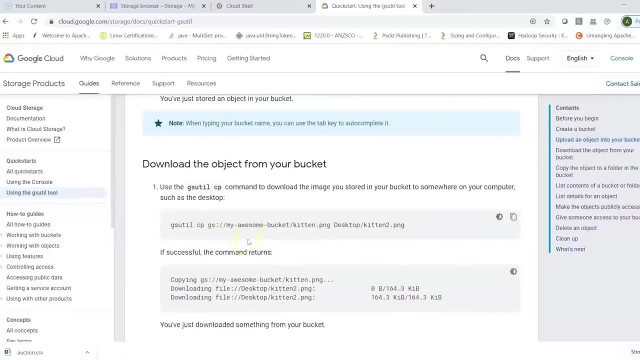 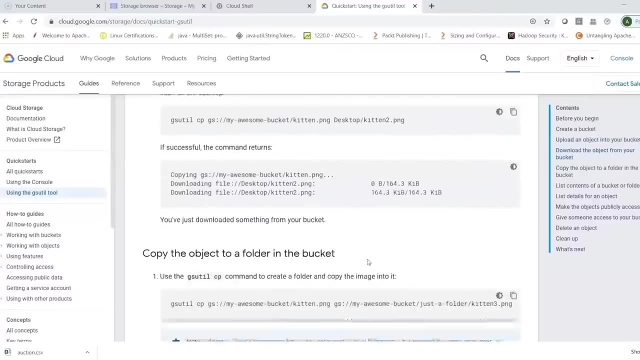 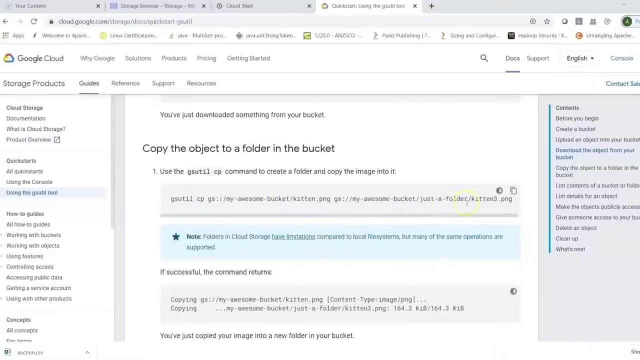 the reverse of that, that is, you can do a copy and you can point your bucket and the file and download it to your desktops. so you can just download that using the command line and you can copy the object to a folder in the bucket. so that is, by creating a particular folder. 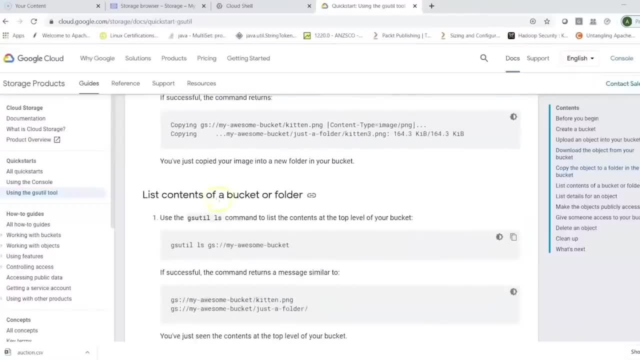 and you are pushing the file into a particular bucket. you can list the contents of a bucket using ls and then give your bucket name. so gs colon. so we can just try this one to be simple and rest. you guys can try. so here you can just do a gsul. 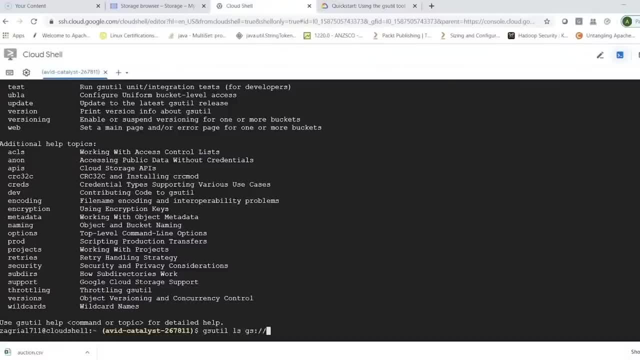 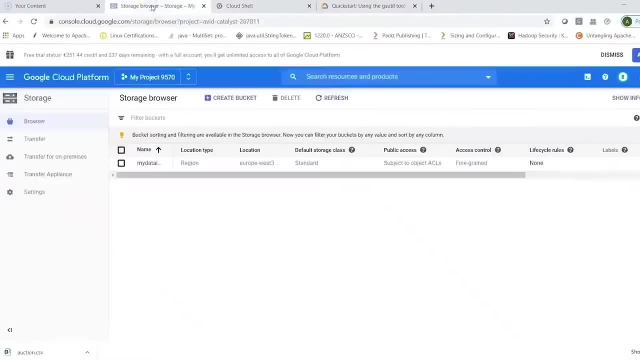 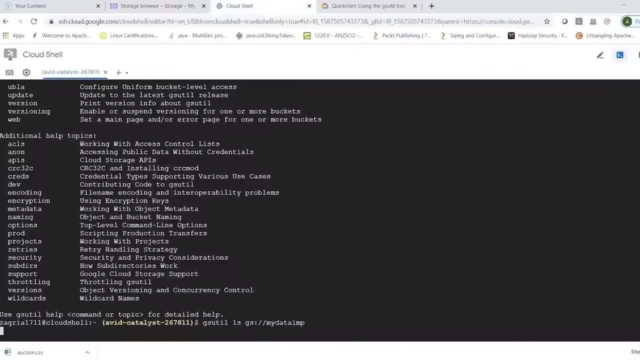 you can do a ls, gs, colon, slash, slash, and then i need to give my bucket name. so in my case the bucket name was my data important. so let's try that. so let's say my data important and i'm trying to list the bucket and the content it has right? and then 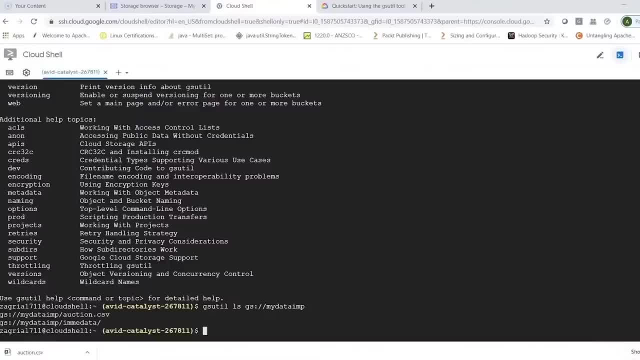 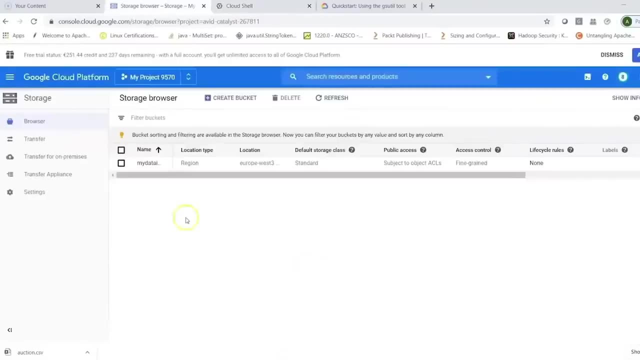 you have a folder and then you can look into the folder and look into the files. so this is a simple option wherein you can use your cloud shell. you could be using your google cloud sdk from your local machine, or you can be using cloud console to create a bucket. upload some data. 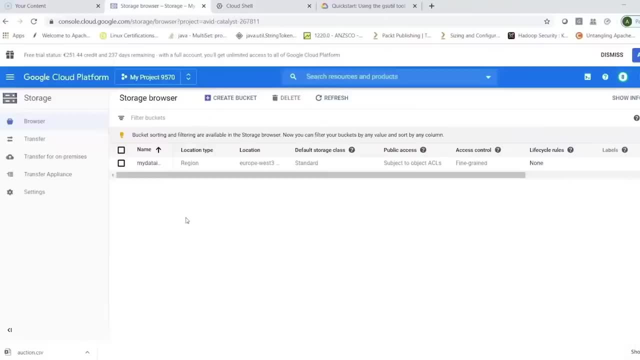 on it, download the data, see if the data is accessible, and that basically shows you the power of cloud storage, where you can easily upload any kind of data. now, what we can also do is, as you are using, a free account, or even a paid account, unless and until you would want to keep. 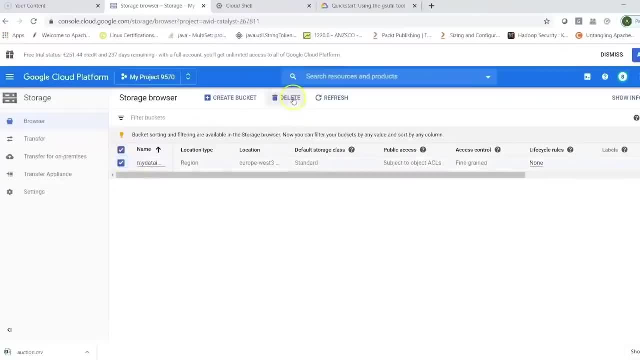 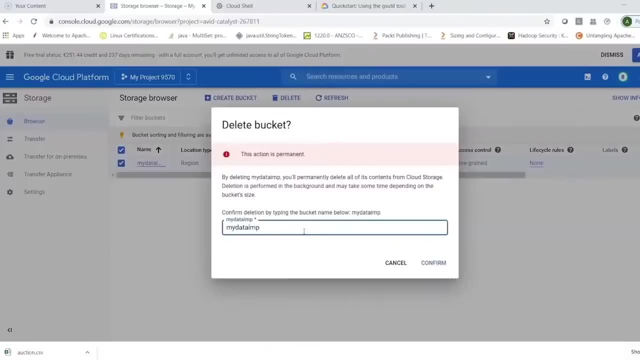 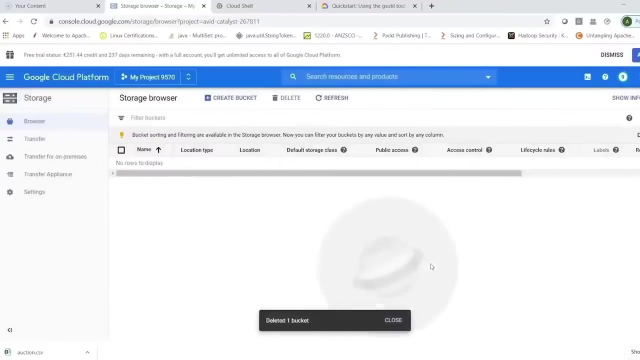 keep the bucket, you can select it and you can just go ahead and delete it. so this will basically ask you to key in the bucket name and, let's say, my data- important. you need to confirm your bucket name. click on confirm and you could have done that using gsutil and a delete command from the 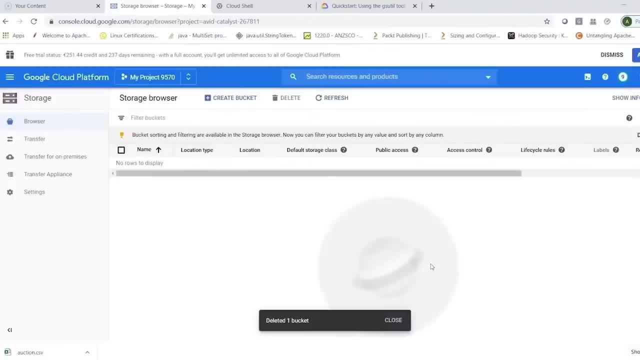 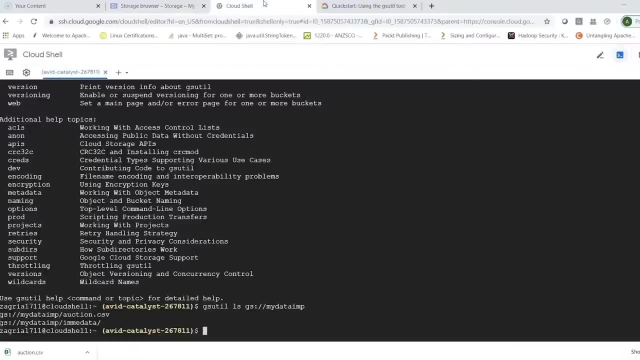 command line that is from cloud shell. so we have now created a bucket. we have uploaded some data into it. we saw how you can download it or create a folder and upload some specific data into it, and also you can do the same thing using gsutil tools, wherein you can list your bucket create. 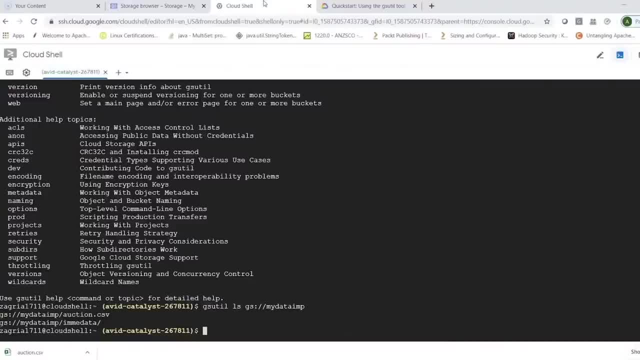 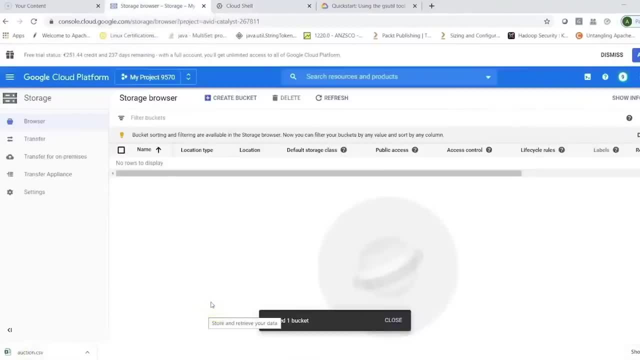 your buckets, delete it, create some folders into it and do everything from the command line. so this is in simple way. you can use your gcp, where either you can spin up your machines or you can use cloud storage to basically use a storage, storage storage or a easy to use instance on Google Cloud Platform. Welcome to this tutorial. 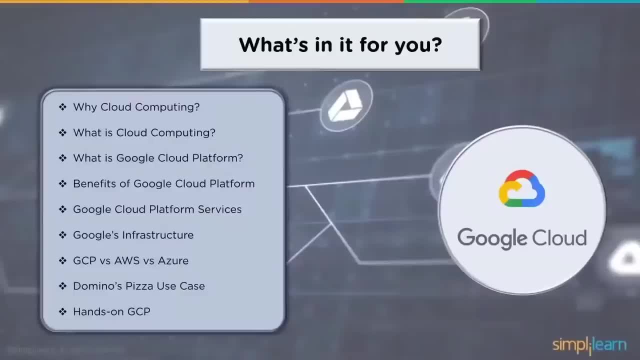 about Google Cloud Platform, and here we will learn about cloud computing. what is cloud computing? what is GCP? that is, your Google Cloud Platform. what are the benefits of Google Cloud Platform and what are its different services. a little bit about Google's infrastructure. a comparison of different cloud providers. 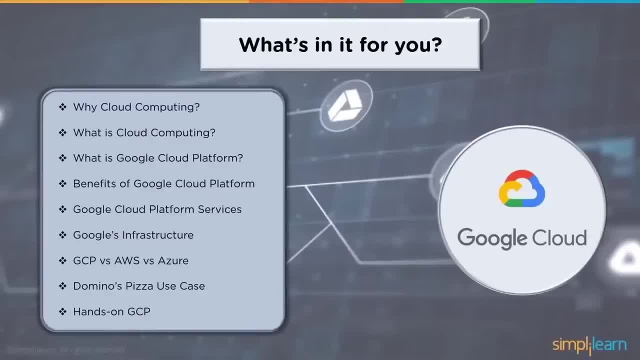 such as Google, offering GCP, that is, Google's Cloud Platform, Amazon offering Amazon Web Services, and Microsoft, which offers Azure. We will also learn about Domino's PISA use case and then have a quick demo on using some of the services on GCP. Before we begin, let's understand why. 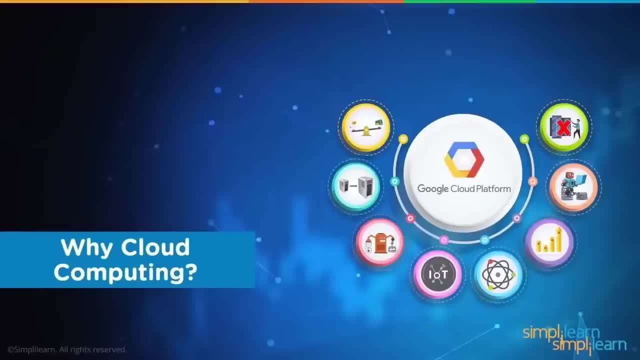 cloud computing is important And it would be always good to learn about cloud computing based on a use case. There are varied use cases where organizations are adopting or moving their solutions or their infrastructure into cloud, or I can simply say, integrating with cloud. Now here is one use case. Nina started a company that 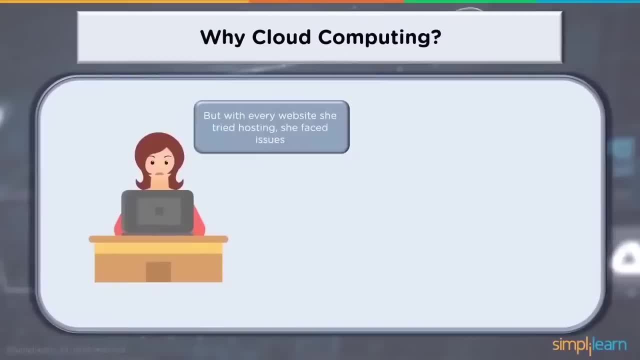 relates to website development. The challenges which Nina was facing were low memory space whenever required for processing or for any other kind of application related work, high traffic to website that crashed it, and also less number of servers. Now, with these challenges, she was then referred to concept of cloud computing and how that could benefit and help her. 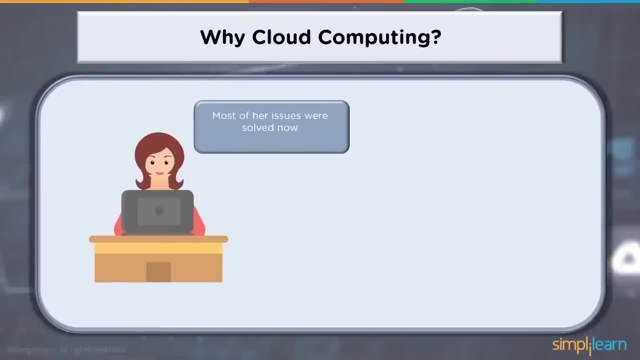 in solving her issues. Most of her issues were solved by cloud computing When she started using cloud computing, and with cloud computing she could increase her memory space as required. that is on demand. control the load to the website. that is basically load balancing and handling more requests on the website or requests per. 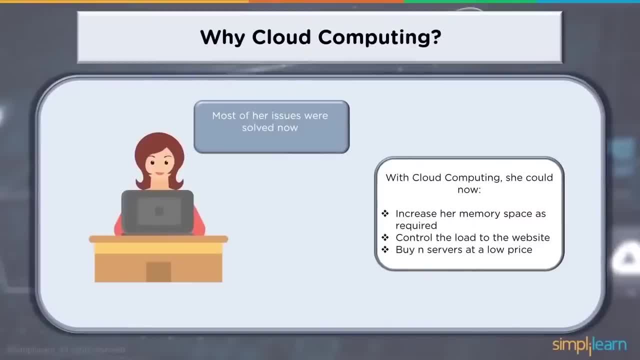 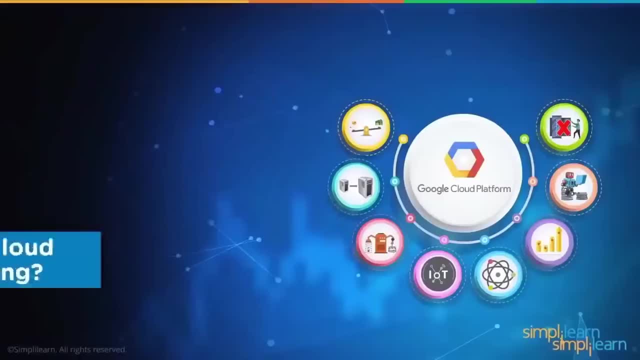 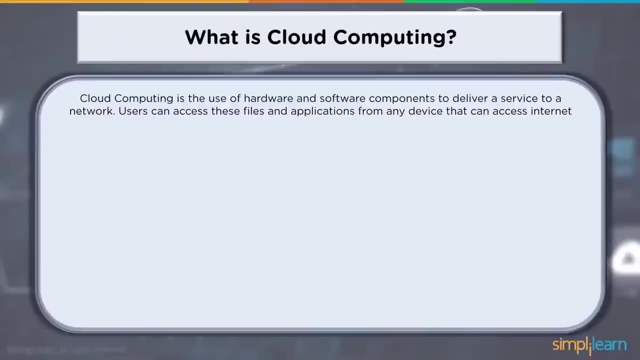 minute, buying servers at a lower price. that is, scaling up or down based on the requirement. When we talk about cloud computing, Cloud computing is use of hardware and software components which a cloud provider offers as a service which can be accessed over network. Cloud computing is use of these resources, which could be either dedicated resources or coming from a pool of resources which cloud provider offers to deliver a service to clients. 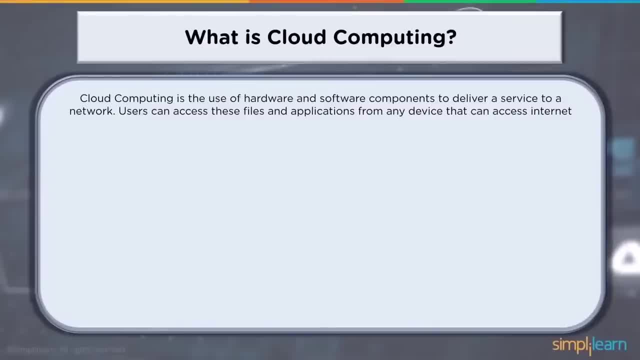 Users can access these different services, applications, files from any device which can basically access internet. Cloud computing allows automatic software integration. It allows backing up and restoring of data. It basically offers unlimited storage memory or computation capacity. It gives access to reliable sources which 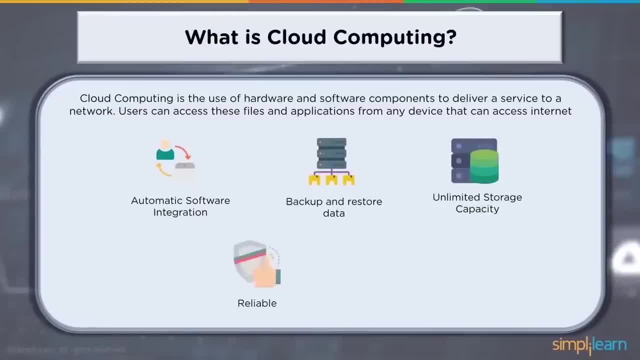 usually the cloud provider themselves are using for their use case, And it is a cost efficient model which helps organizations to quickly integrate or basically modernize their infrastructure. Cloud computing is usually used with IT or within IT space, wherein there are five traits: If there is a requirement of resources as the business dynamically changes or grows. 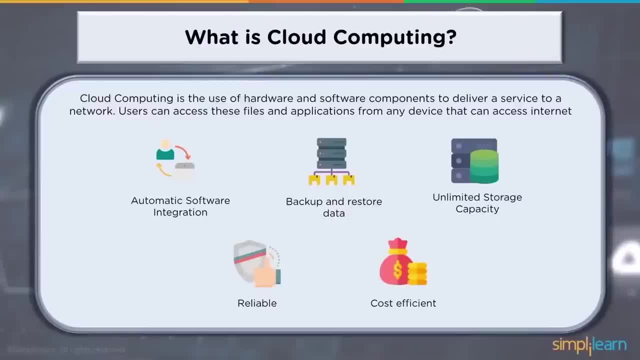 So for this, cloud computing offers on demand self service, So users could be using on demand computing resources or memory resources, storage network and so on provided by cloud provider and also do a self service. All this is possible using a simple interface And users can be using processing power storage network as they need and pay as they go. 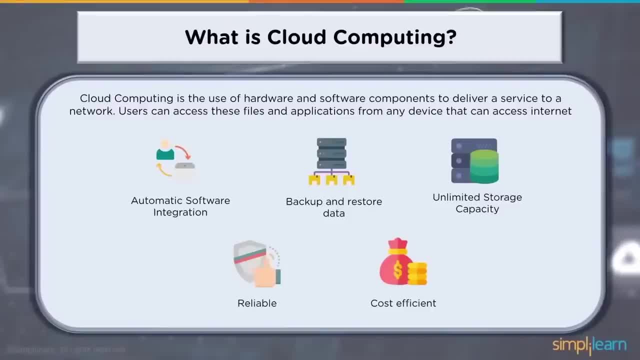 So there is least or no human intervention required When it comes to projects which might need scalable network access. cloud computing offers broad network access, that is, accessing resources over network across geographical regions, or what we call as availability zones, which might be multiple sites within a particular geographical region. 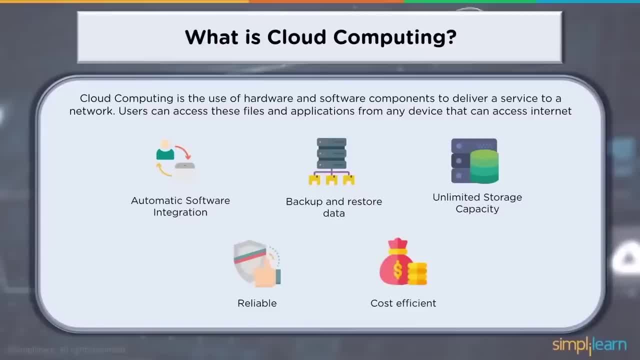 Cloud providers also have what we call as resource pooling, So this basically provides a huge pool of resources which are shared and can be accessed by customers at a lower cost. Now there might be customers which are interested in not sharing the resources and would be interested in dedicated resources. 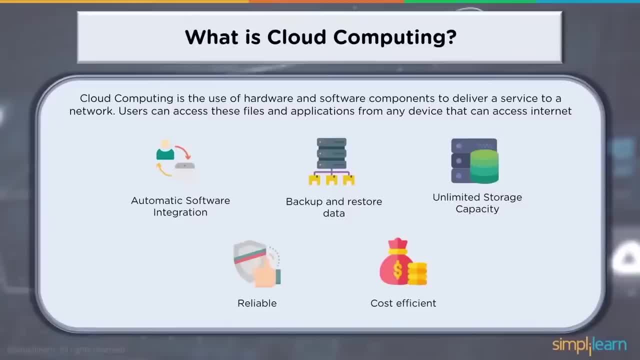 And in this case, cloud provider also have sole tenants And they would have to implement offerings which help such customers. If an IT business, or any other business, needs rapid elasticity, then cloud providers also have resources which are offered which are elastic. You can get more resources rapidly, as needed, and thus you can scale up and down. 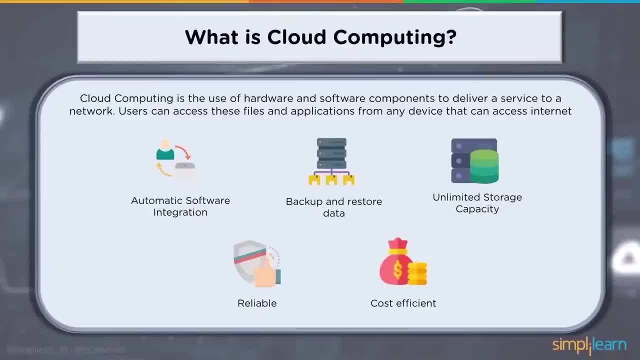 Think of a gaming company which would be interested in launching a new game and they would have predicted a certain number of users Which would get on to the portal playing the game. And what happens if the request per minute or if the number of users who are joining in might increase. 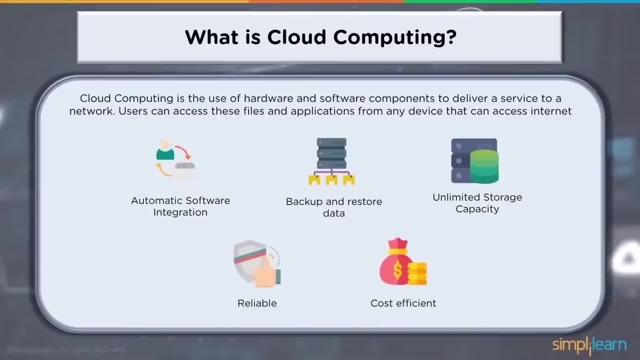 Now, in this case, organization would want an underlying solution which handles this dynamism, scales as needed on demand and, once the demand is done, scales down. This is possible using a cloud computing solution. Cloud computing solutions also include cloud computing solutions. 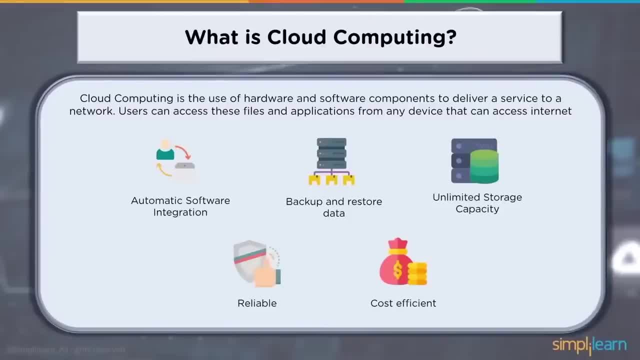 They include measured services, that is, pay-as-you-go model, for the usage or for the reservations which a user or organization would have made for resources offered by cloud computing. So when we talk about cloud computing, one of the questions which always arises is: why is this model so compelling? 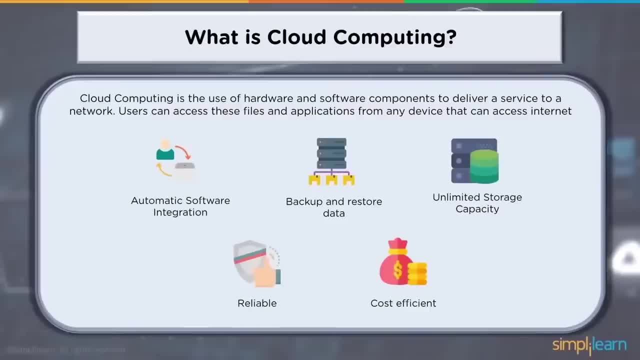 Why is this so interesting? for organizations or users who would want to use one or many services from cloud computing. So first wave of trend, which is cloud computing, is cloud computing. So first wave of trend, which is cloud computing, Which brought storage, cloud computing was what we call as colo, that is, co-location. 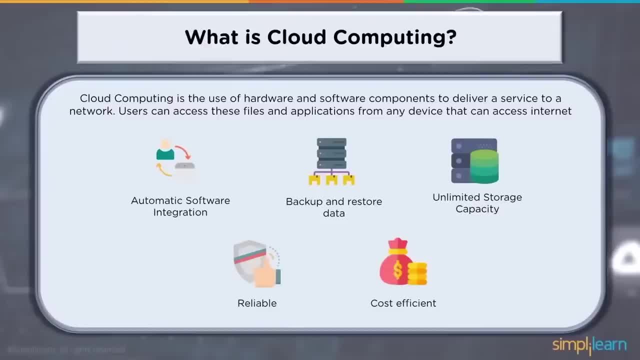 IT shops that have been using or managing huge amount of data from decades basically wanted to build their infrastructures to handle their business needs. Now, instead of building costlier data centers, they would rent space or share facilities, And this was being done by organizations. 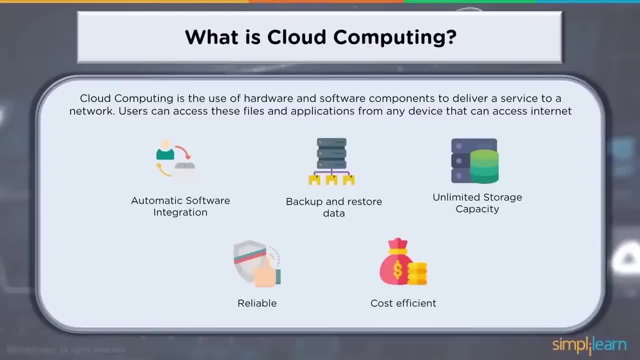 Even in past. Thus they would free up the capital for other use cases. Now this was more of user configured, managed and maintained by them. Later organizations started thinking of virtualization, So that was again user configured, but provider managed and maintained. 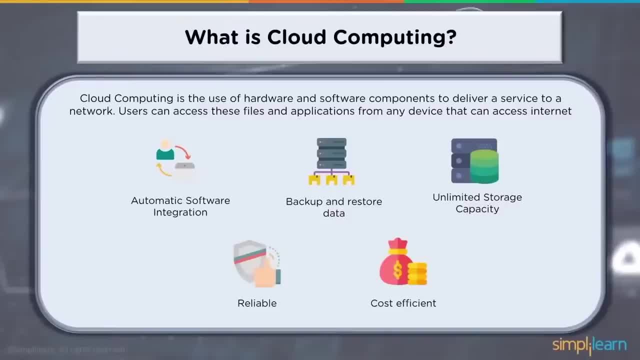 So components of a virtualized data center matched that of a physical data center, And Organizations would have virtual devices separately managed from underlying devices. Then later came container based architectures, or basically automated services. So within Google, services are automatically provisioned and configured, letting your infrastructure scale on demand. 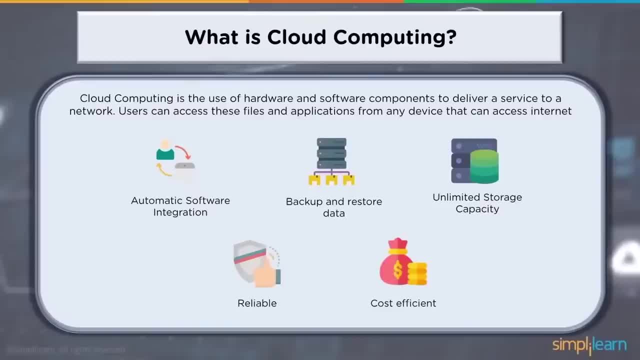 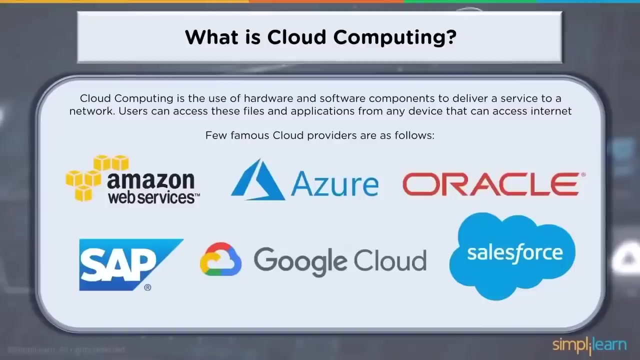 There are various reasons why an organization would think of integrating with cloud or Benefiting by using cloud and thus instantaneously reaping the benefits of modernizing their infrastructure. Now, few famous cloud providers are here, So you have Amazon, which offers Amazon Web Services, and a huge list of services which come in with this. 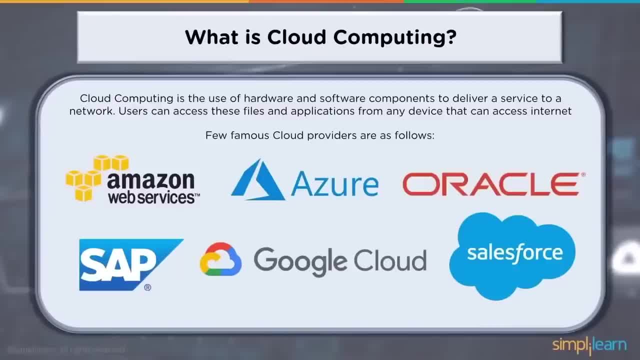 You have Microsoft Azure, You have Oracle's cloud, You have SAP's cloud solutions, GCP, Which is offered by Google, Salesforce, and so on. There are many other small players which are also providing different services which are cloud based, or organizations which are partnering with these main cloud providers, thus offering cloud services to their customers. 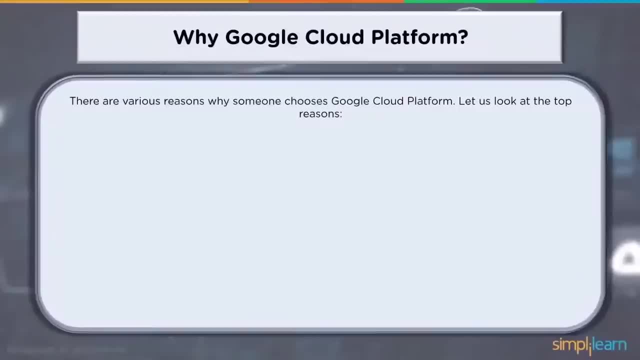 When we talk about why Google Cloud Platform, there are various reasons why someone would choose Google Cloud Platform. GCP has better pricing compared to To its competitors When it comes to speed and performance. it is very fast and increases the performance of the project. 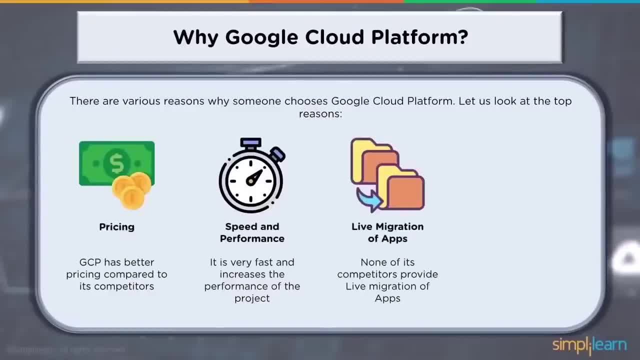 Live migration of apps, and there are huge number of solutions, which I will show you further in further screens, which help an organization to adapt to a cloud platform and integrate with cloud platform or even completely migrate into a cloud platform. None of Google's competitors provide. 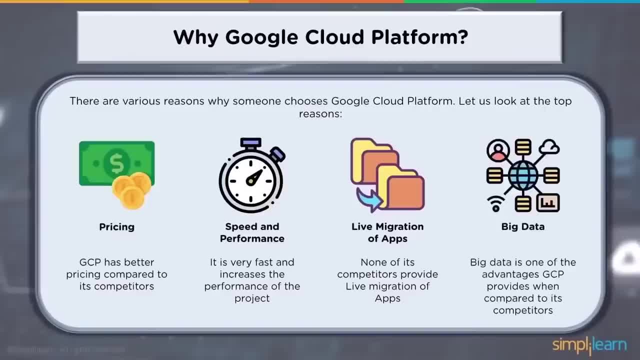 None of Google's competitors provide Live migration of apps. When we talk about big data, AI, machine learning kind of solutions, GCP provides a lot of innovative solutions in comparison to other cloud providers such as AWS, Azure and so on. So what is Google Cloud Platform? 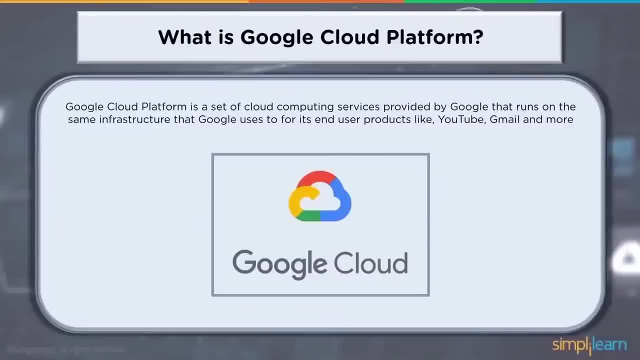 It is a set of cloud computing services provided by Google that runs on the same infrastructure that Google uses. It is a set of cloud computing services provided by Google that runs on the same infrastructure that Google uses To and for its end user products like YouTube, Gmail and so on. 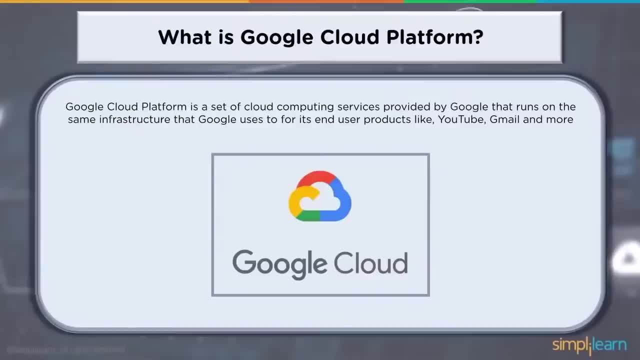 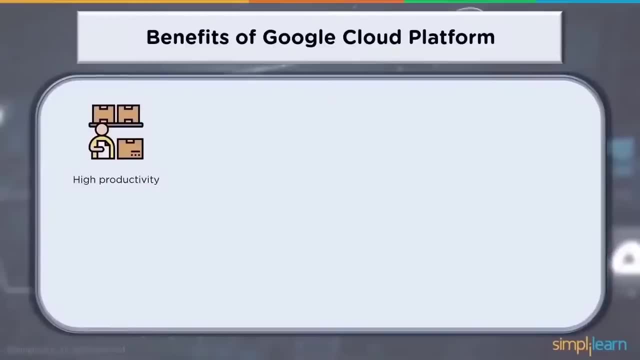 To and for its end user products like YouTube, Gmail and so on. Let's learn about benefits of Google Cloud Platform, such as high productivity, Working from anywhere. Working from anywhere, Quick collaboration, high security, fewer data stored on vulnerable devices. reliable resources which can be used across organization, across geographical regions, across countries. Quick collaboration, high security, fewer data stored on vulnerable devices, reliable sources which can be used across organization, across geographical regions, across countries. chama, we watch a lot of possible solutions. bey원� Mommy, I love my machine right. 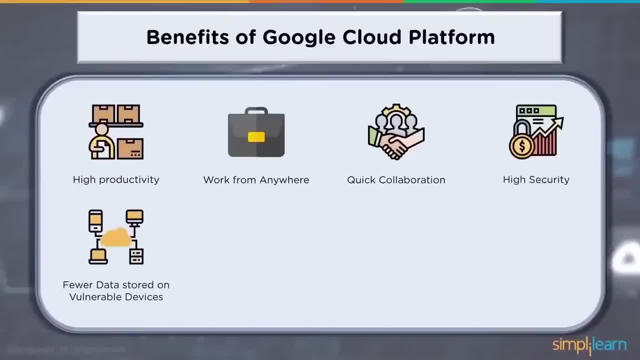 me. I do not know where I am, Creely Le sponsoring a business to develop these treasures. Today I am here with a Macbook Mini gün disaster on vulnerable devices, reliable resources which can be used across organization, across geographical regions, across countries. 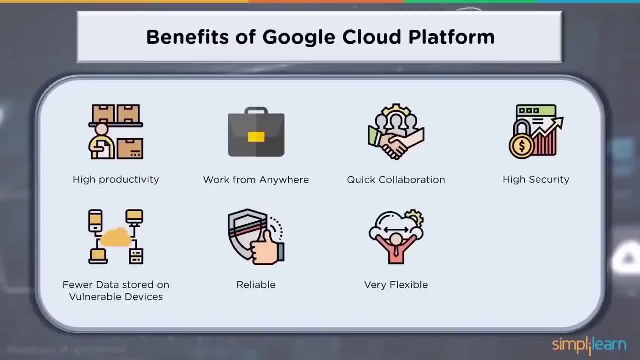 very flexible, which allows organizations to scale up and down as the demand rises or as the demand declines, and cost-effective solutions for various use cases. These are some of the benefits And if we look into different services which Google Cloud Platform offers, we could look into detailed benefits. 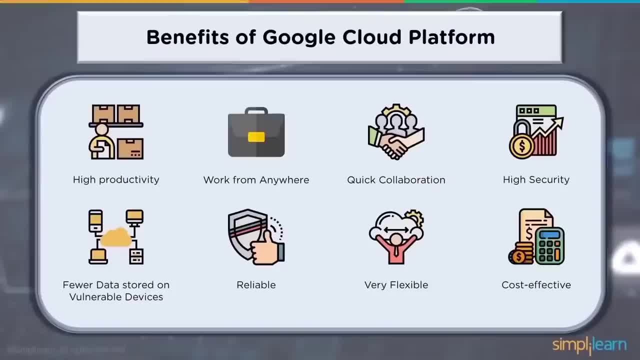 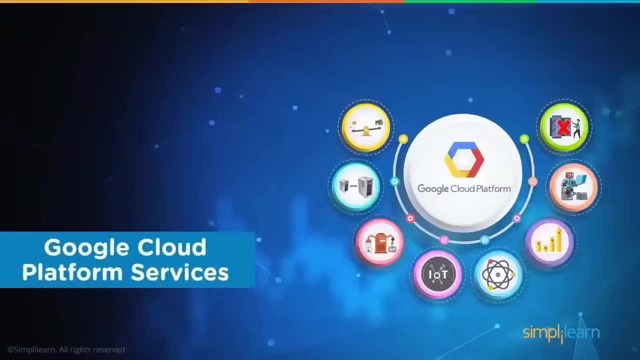 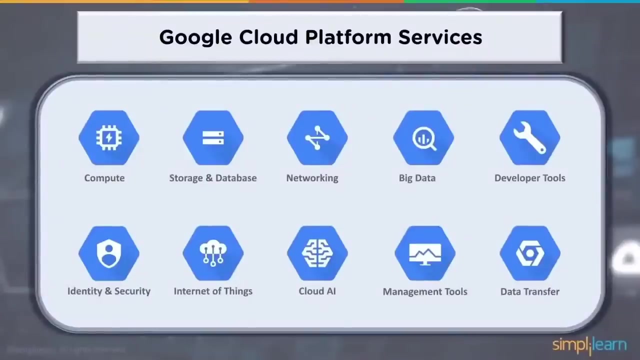 which each service offers in a different use case, which basically helps organizations working in different domains, handling different kinds of small, mid or larger businesses and with different business goals. When we talk about Google Cloud Platform services, here is a list of services or I could. 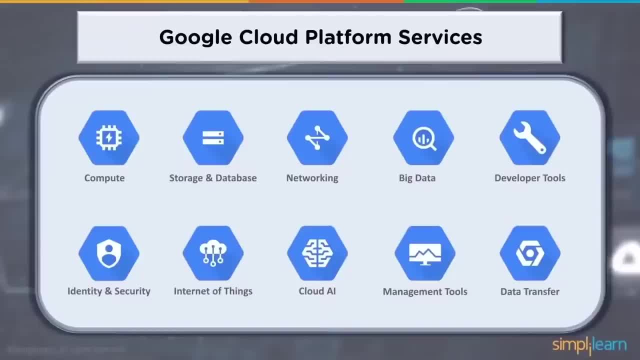 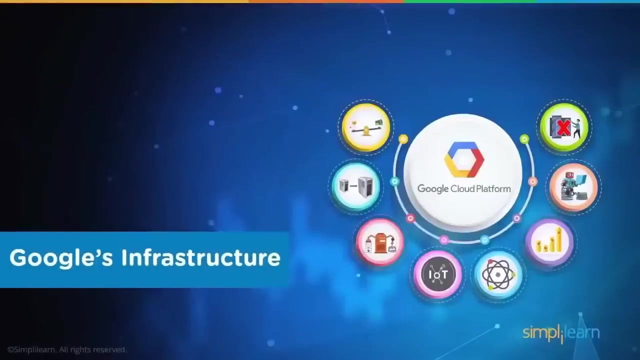 say, highlights. You have high-level domains or categories of services, So you have compute-related services, You have storage and database, You have networking, big data, developer tools, identity and security management, internet of things, cloud, AI management tools and also data transfer solutions. 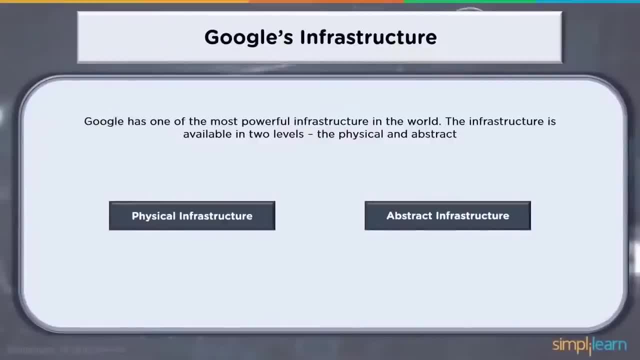 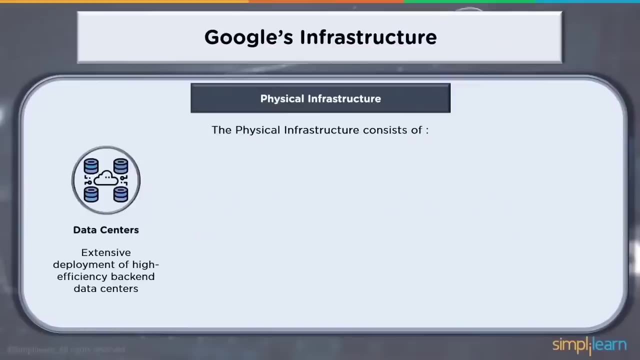 When we talk about Google's infrastructure. Google has one of the most powerful infrastructure in the world and that is the infrastructure that is available in two levels: the physical and the abstract layers. You have physical infrastructure and then you have the abstract infrastructure. 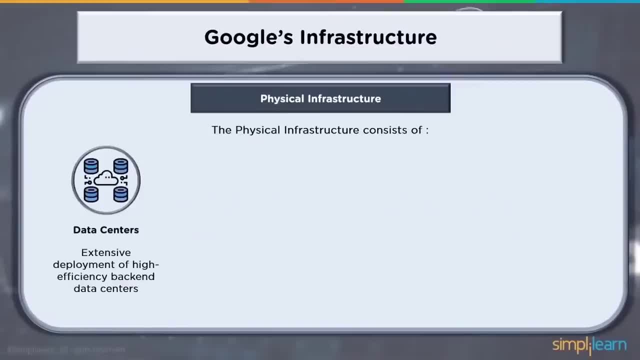 Physical infrastructure consists of data centers, extensive development of high-efficiency backend data centers. You have a very strong backbone network which is used by Google itself and also offered as services to customers. So you have a global, meshed, redundant backbone network. 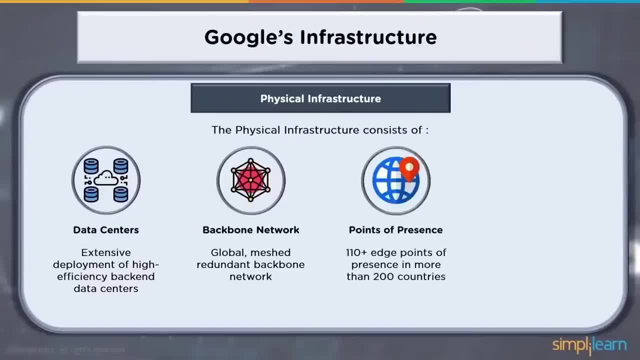 Points of presence. when we talk about Google, it has 110 plus edge points of presence in more than 200 countries. And when we talk about edge caching, edge caching platform at periphery of their network. So this is what defines the physical infrastructure. 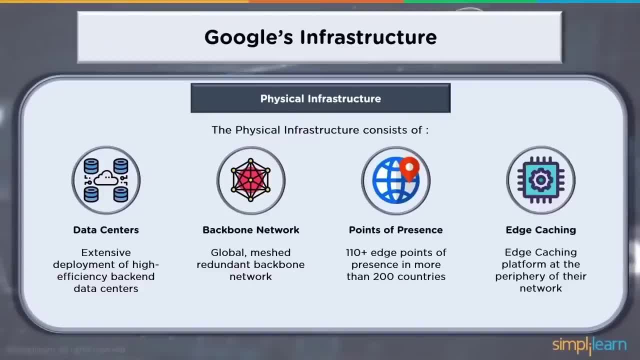 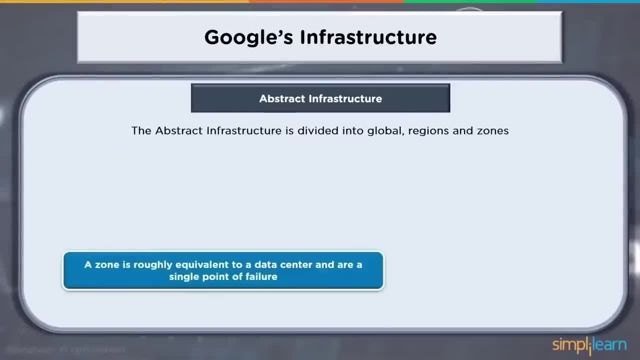 of Google. Now, there is much more to it, rather than just the physical infrastructure of Google. So this is what defines Google, Rather than just these four points. When we talk about abstract infrastructure, that is divided in global regions and zones. 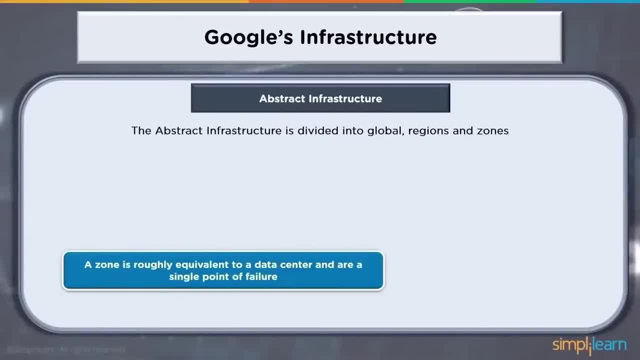 When we talk about zone. a zone is roughly equivalent to a data center and a single point of failure. So you could have your compute engine which is within a zone, Or you could say compute engine is a zonal resource. You have regions, which are geographical areas, which 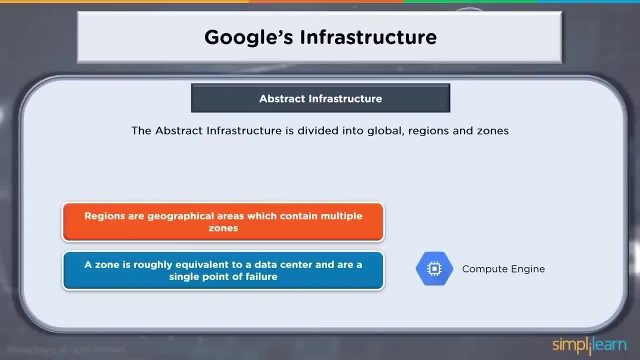 contain multiple zones. So you could have multiple zones. So you could have multiple zones. So you could have multiple zones. You could have a region for US Central or Europe Central, Europe West and so on, And within a region you would have one or multiple zones. 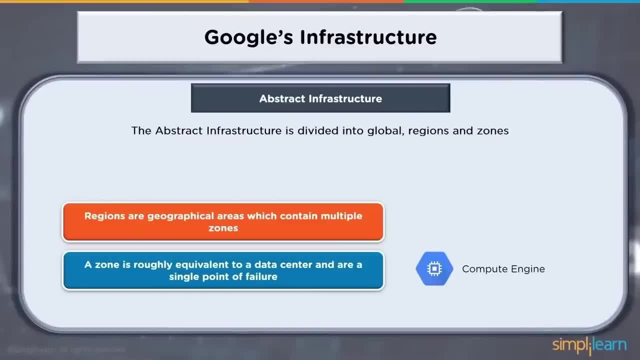 And zones, basically, would allow high availability of resources. So you have cloud Load balancer is an example which is regional resource. Then you have global resources and they are available and shared across the planet. So you have various global resources. So you have global resources. 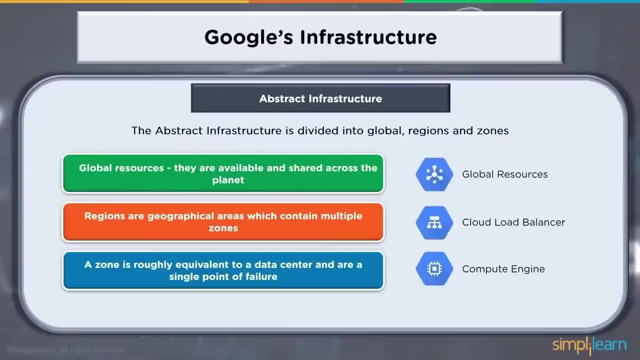 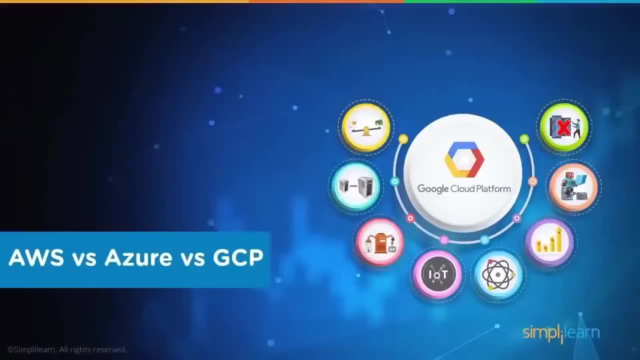 Such as network, which could be even your IP addresses, and so on. Now let's do a quick comparison of AWS with Azure, with GCP, And let's look at what each cloud provider offers. Later we will also look into different services in detail. 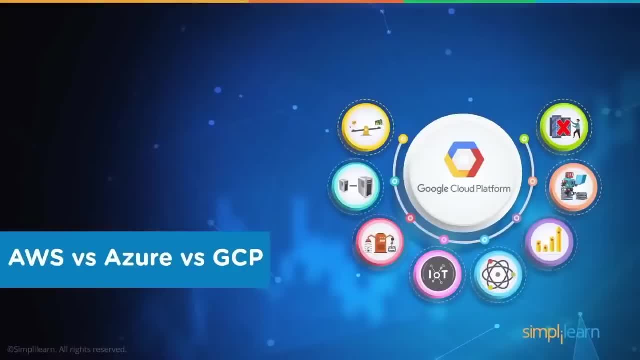 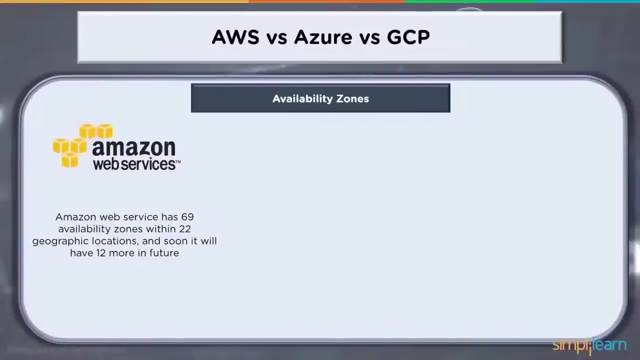 when it comes to Google Cloud Platform, What each service does, what you can benefit from. which service should you use in what case? We will learn about those in later slides If I compare your different cloud providers. when we talk about Amazon and its cloud offerings, 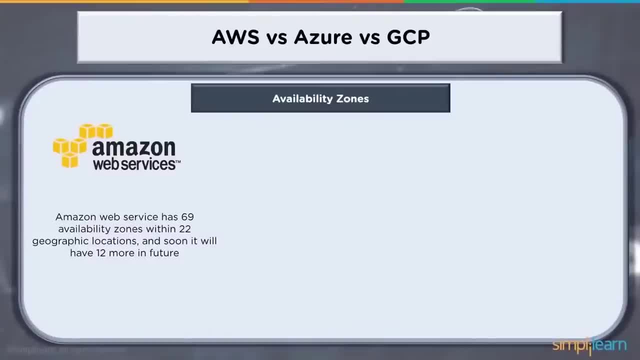 that is, Amazon Web Services, or AWS as we well know it. Amazon Web Services has 69 availability zones within 22 geographical locations, And soon it will have 12 more in future. So this number keeps growing, Based on the spread of the services. 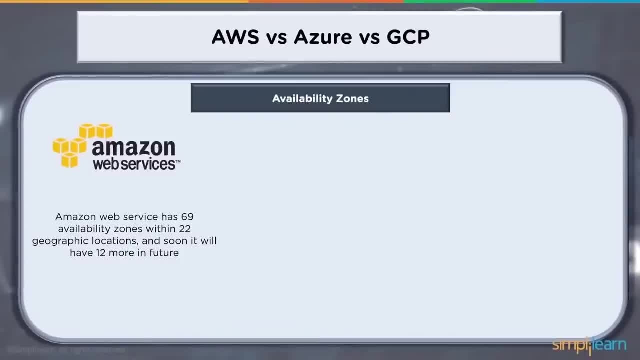 which a particular cloud provider offers. Here we are talking about availability zone specific information. When we talk about Microsoft's Azure, it has 54 regions worldwide and is available in 140 countries across the globe. When we talk about Google Cloud, Google Cloud Platform. 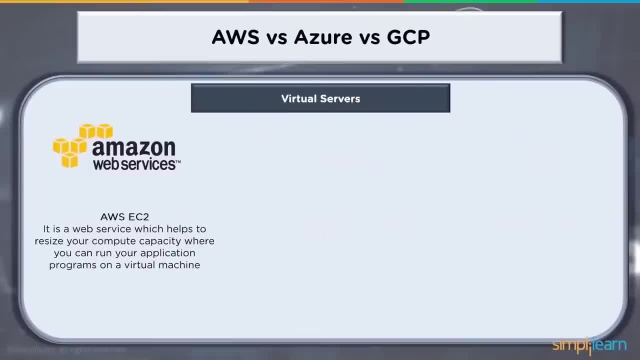 is available in 200 plus countries across the globe. When we talk about virtual servers, Amazon's EC2,, that is, Elastic Compute Cloud. It is a web service which basically helps to resize your compute capacity where you can run your application programs. 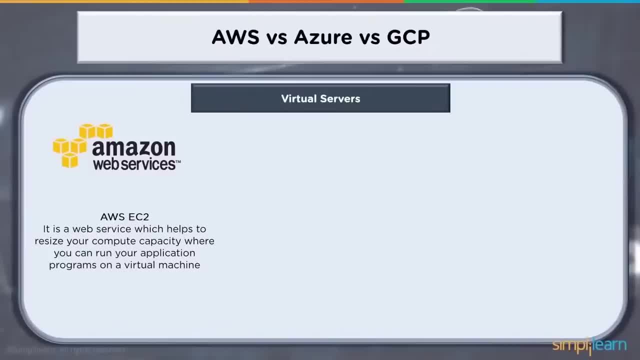 on a virtual machine. So, using EC2 service, you could launch virtual instances that could have any distribution of Linux, Windows. You could have different specifications when it comes to RAM or CPU cores or disk. You could also decide on what kind of storage a particular instance should use. 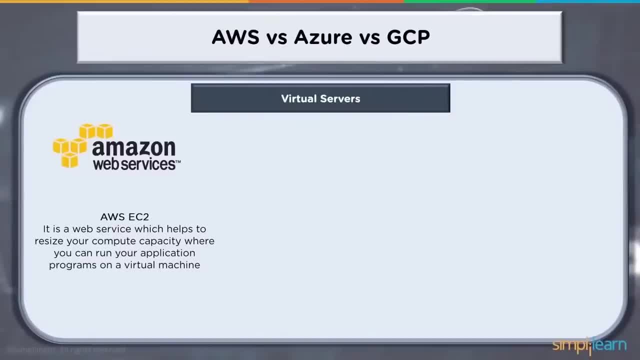 whether the storage should be local to the instance or whether that should be elastic file system or even an object storage. When it comes to Azure or Microsoft's offering, Azure Virtual Machine, that is, infrastructure as a service- gives a user the ability to deploy and manage. 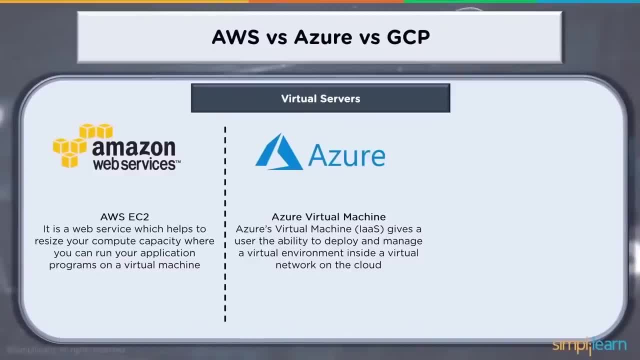 a virtual environment inside a virtual network on the cloud, And this virtual network on the cloud would be managed by cloud provider Google Cloud or the offerings from Google Cloud Platform, that is, GCP- VM instances- enables users to build, deploy and manage virtual machines in order to run. 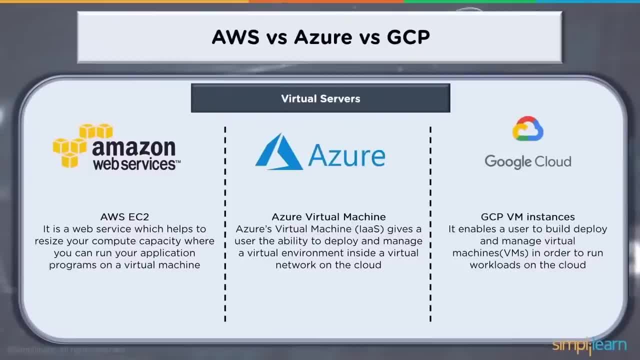 different kind of workloads on the cloud. Now, when we talk about Compute Engine here, it would be good to discuss a little bit more about Compute Engine and what are the different options which Google Cloud offers. So when you talk about your Compute Engine, 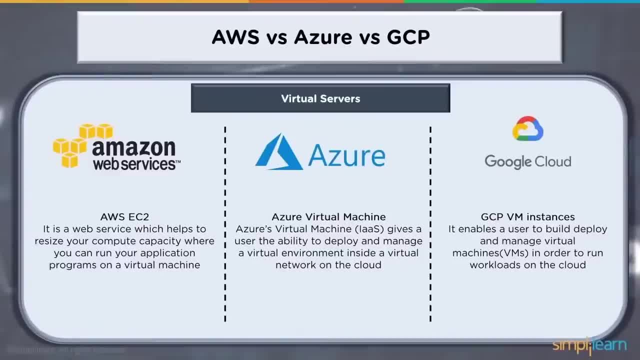 you have scalable, high performance virtual machines. Compute Engine delivers configurable virtual machines which run in Google's data center with access to high performance networking infrastructure and block storage, And you could select VMs for your needs. That could be general purpose or workload optimized. 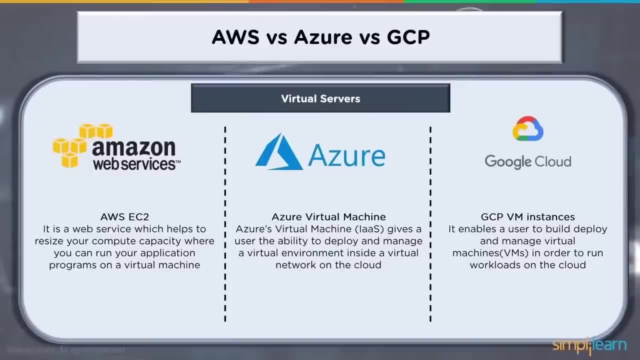 And when we talk about workload optimized, you have predefined machines or you have custom machine sizes. You can integrate, compute with other Google Cloud services, such as AI or ML, and go for your data analytics You have. when we talk about your GCP VM instances, 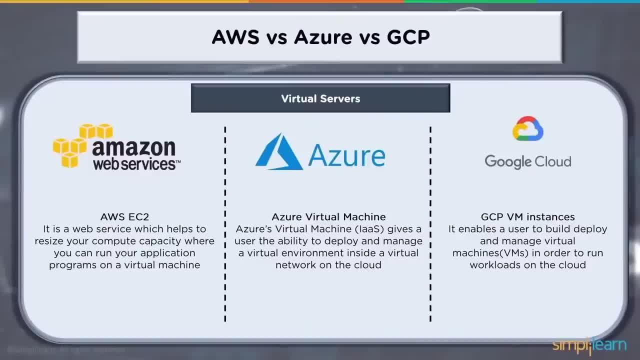 just to expand on that, you have general purpose instances, which we call as N2, which provide a balance between price and performance, And they are well suited for most workloads, including line of business applications, web servers and databases. Google Cloud also offers compute optimized instances. 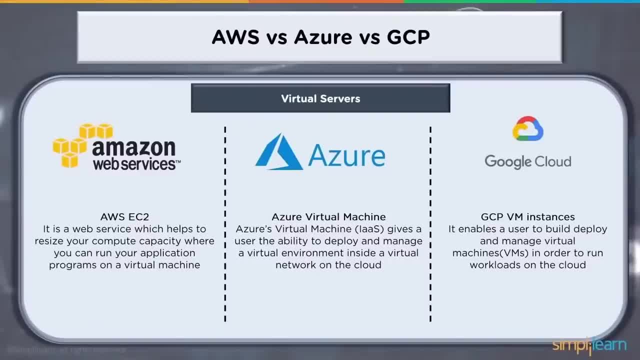 which we call as C2 instances, which offer consistent, high end virtual CPU performance, which are good for AAA, gaming, EDA, HPC and other applications. Now, when we talk about compute optimized- your general purpose- how would we leave memory? 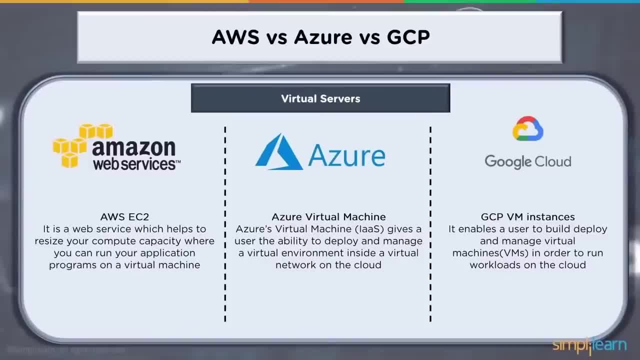 optimized instances. Those are M2 machines which Google offers, So these offer highest amount of memory. These VMs are well suited for in-memory databases such as SAP HANA, real time analytics and in-memory caches. So if I would summarize this: when 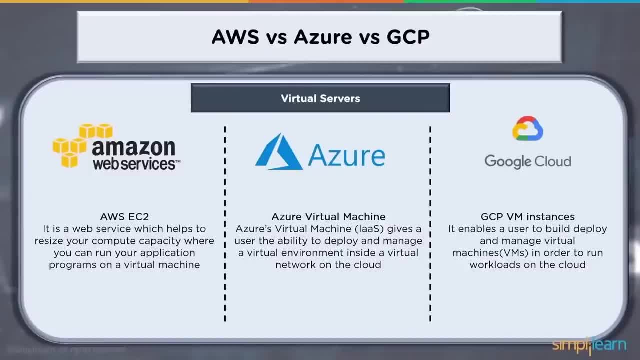 we talk about different instances. AWS also offers different kind of instances, which are memory or compute or disk optimized. You have general purpose and each category of machines has a different pricing model. You can always go to an AWS website, look for the pricing models and that. 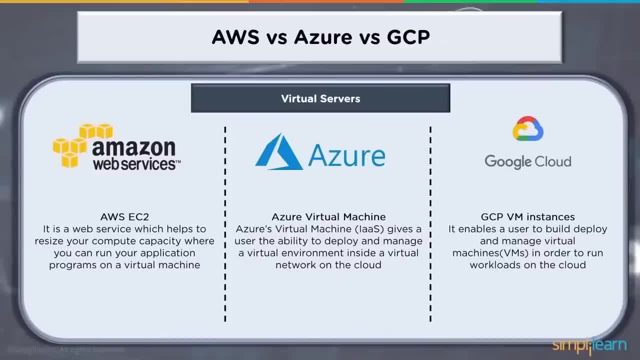 will give you an idea of on-demand instances or dedicated instances, reserved instances and so on. Similarly, if you talk about Google Cloud, Google Cloud also has instances with various options, which become the key features of why customers would choose Google Cloud. 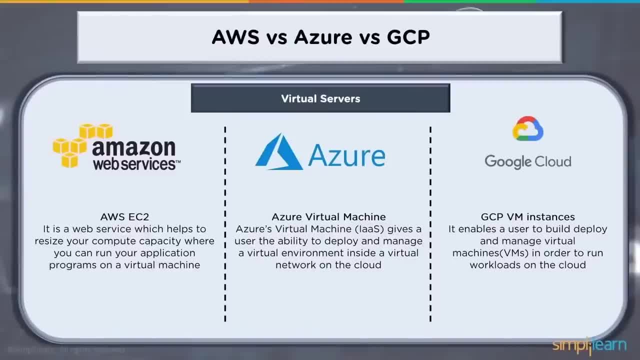 This is because there are various options in the platform, such as live migration for VMs, So Compute Engine within your GCP can live migrate between host systems. And when I say live migrate, it basically means without rebooting, which keeps your application running. 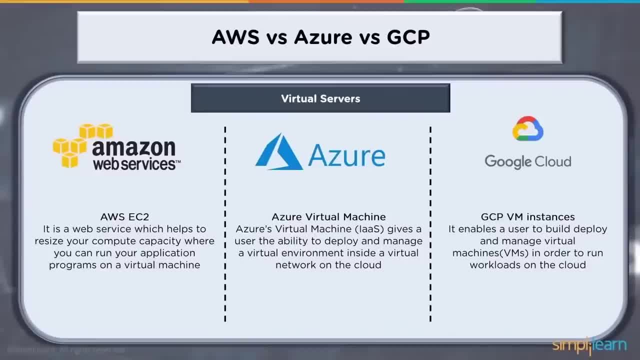 even when the underlying host systems require maintenance. You also have preemptable virtual machines wherein you can run bad jobs and fault tolerant workloads to reduce your virtual CPU and memory cost by up to 80% while getting the same performance. so these are your preemptive or preemptible virtual machines. the 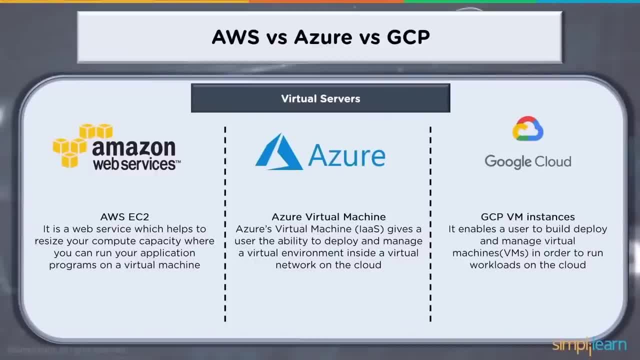 only demonet is. these can give you a really cost-efficient resource usage. however, can be taken off the shelf anytime and that's why we call them preemptible virtual machines. you also have sole tenant nodes, which are physical compute engine servers dedicated explicitly or exclusively for users use case, and when we talk about sole tenant nodes, these are usually good. 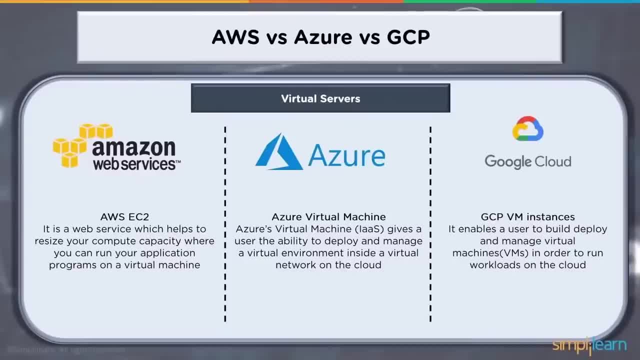 when you are dealing with or when you are working with your applications, which we call as bring your own license applications. so sole tenant nodes give you access to same machine types and virtual machine config options as regular compute instances. so there are different options which Google Cloud offers when it comes to. 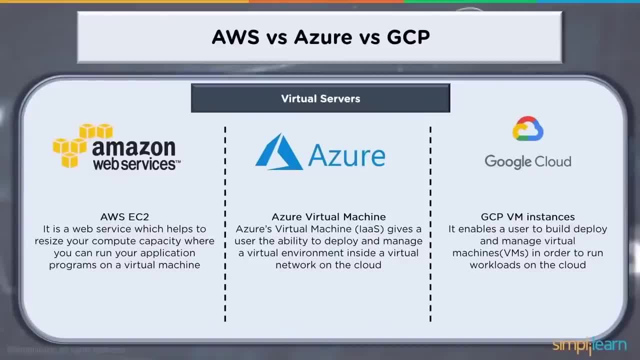 these instances which we are talking about and it takes care of different use cases in comparison to other cloud providers which are also offering these services, such as: you can have predefined machine types. you can have custom machine types, preemptible VMs, as I said, live migration of VMs you can use. 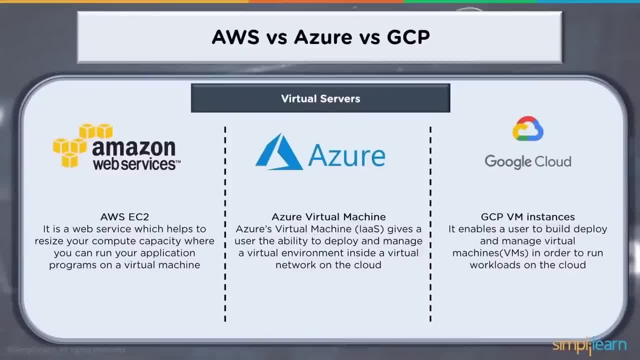 persistent disks which could give you durable, high-performance block storage. you have local SSDs. you also have GPU accelerators, which can be added to accelerate computational intensive workloads such as machine learning, simulation, medical analysis and so on, and you have features such as global load balancing, which makes Google 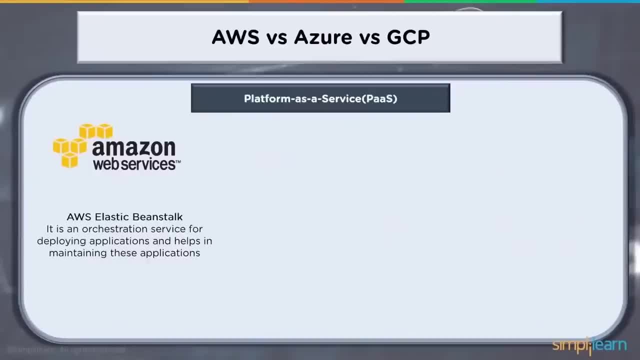 Cloud a unique choice when we talk about platform as a service. Amazon has platform as a service offering which we call as elastic beanstalk among one of its services. it's an orchestration service for deploying applications and helping in maintaining these applications, as your cloud service provides a platform to write the. 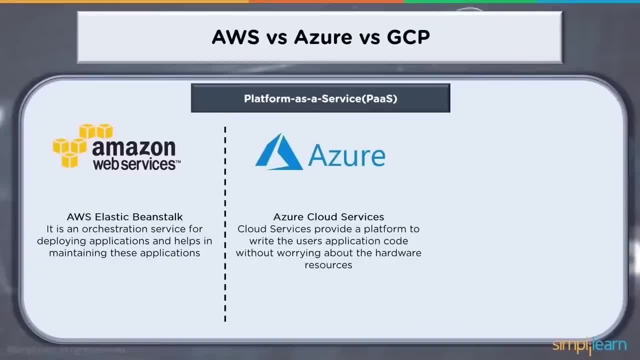 user application code without worrying about the hardware resources. Google App Engine is a service used by developers for building and hosting applications on Google's data centers. when we talk about server less computing, so Amazon's AWS lambda is a server less compute service. it is used to execute back-end code and scales automatically when required. when we talk 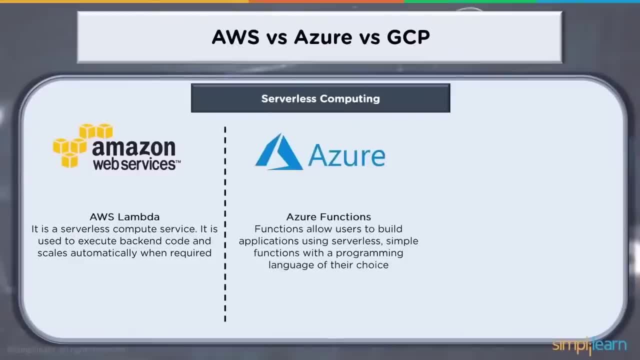 about is your. you have something called as functions, which allow users to build applications using server, less simple functions with a programming language of their choice. when we talk about Google Cloud, GCP has cloud functions, which is a very easy way to run your code in the cloud and it is highly available and fault. 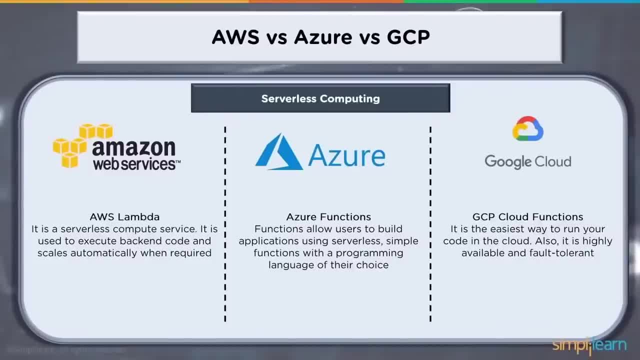 tolerant. so in these days, when we are talking about micro services architecture, which organizations are preferring, when we are talking about organizations which can scale, which can dynamically change their underlying architecture, organizations would be interested in server less computing, where they do not have to have a infrastructure, set up a plan in advance. 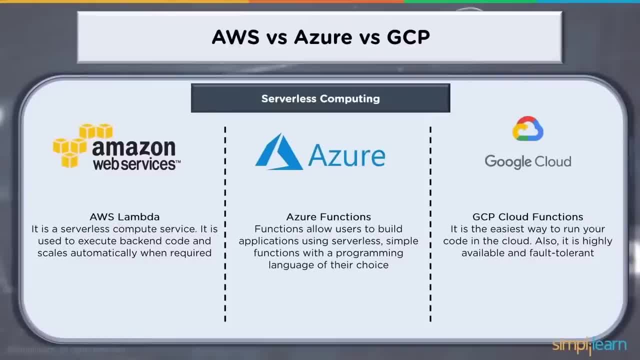 Once before going for their use case, and this is where monolithic applications are really not a preferred choice. lot of organizations are decomposing their applications into micro services based on business capability or decomposing based on subdomains. we can learn about micro services architecture later, but just to know that, server less computing, which basically 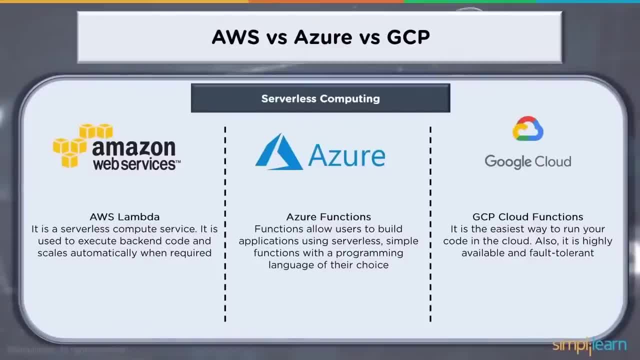 helps any organization. if, for example, if you have a web application that receives non-linear traffic and you cannot keep an eye on your server always, it would be good to have someone to auto scale your application server. less is basically a computing model where cloud service provider is responsible for managing the piece of code without the developer having 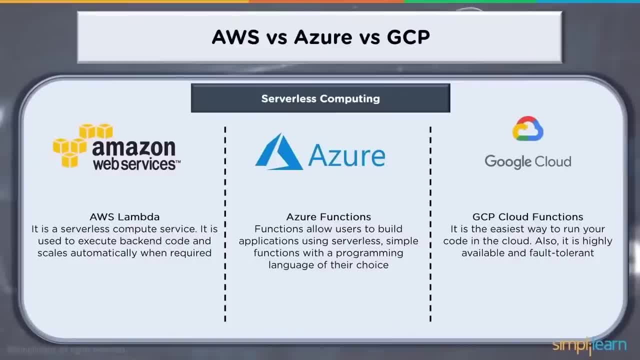 to bother about infrastructure, set up, management, maintenance and so on. Now, when we talk about applications being serverless or benefiting from serverless computing, one of the key things would be zero administration, so deploying application without any provisioning and management Auto-scaling capability, that is, let the service. 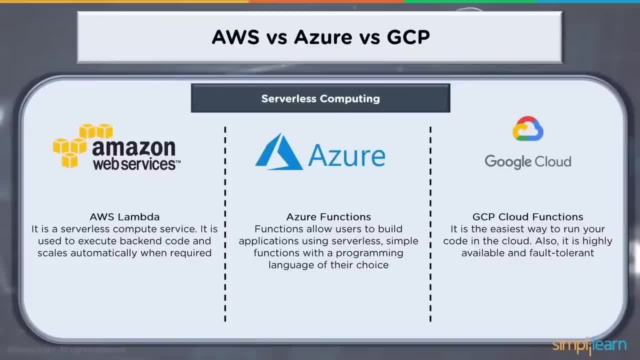 provider. worry about scaling the application up and down. You have pay-per-use model, which any customer would want to benefit from. that is, pay only for the resources that you have used or that you are continuing to use. right, Shorten the time between idea implementation and. 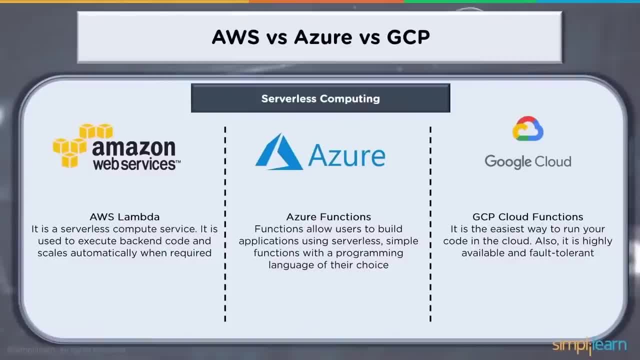 deployment- and this is something which any organization would want- that you would want a faster bring-to-the-market solution timeline in comparison to getting entangled with deployment, management and maintenance of your underlying infrastructure When your applications are facing a high demand. So when we talk about serverless, 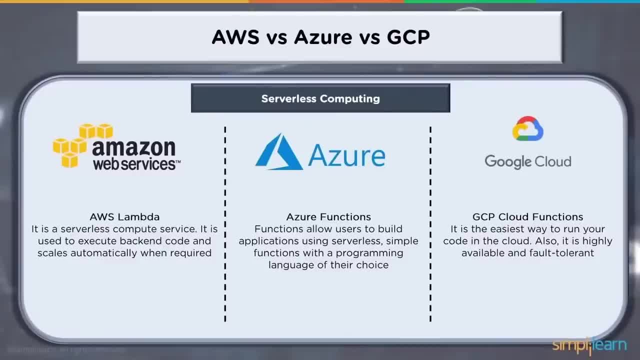 it is a function as a service, because each part of your application is divided as functions and can be hosted over multiple service providers. You have serverless apps, which are usually divided as separate units or functions based on functionalities or domains, and so on. 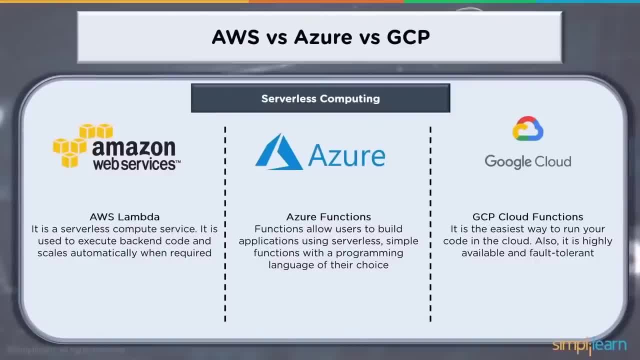 So serverless computing is gaining quite popularity. It is for a reason: because it is trying to utilize the existing infrastructure more effectively in comparison to the traditional 3-tier architecture where you had a presentation layer, you had an application layer, you have a database layer. Now that kind of infrastructure is not. 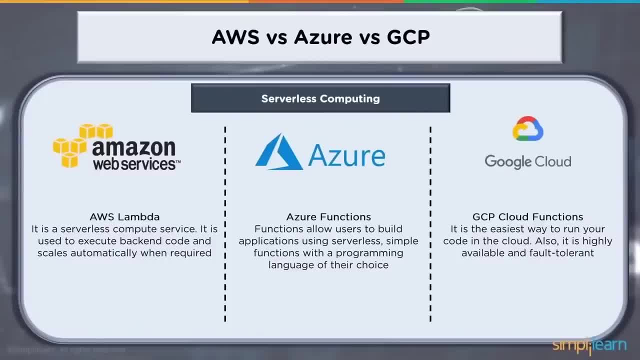 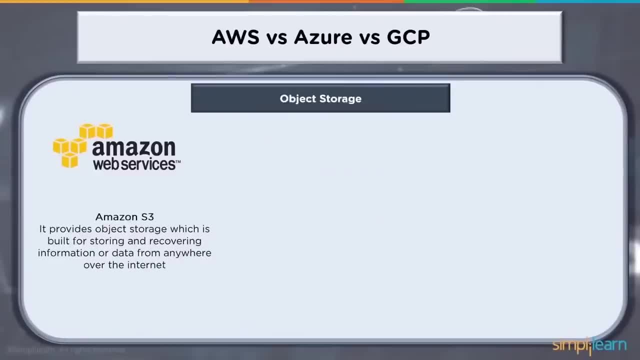 really preferred in today's modern times when organizations are working on different kind of newer applications. When we talk about object storage, Amazon has Simple Storage Service that is S3.. service that is S3: it provides object storage which is built for storing and recovering. 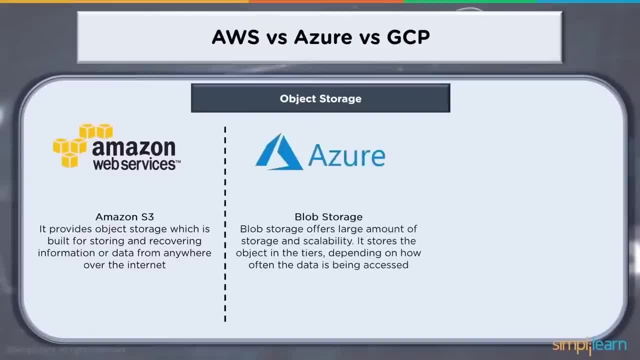 information or data from anywhere over the internet. Azure comes up with blob storage, that is, binary large objects storage offers large amount of storage and scalability. it stores the object in the tiers and depending on how often the data is being accessed. now same thing applies to even S3, which is from Amazon. so S3 also has different kind of storage. 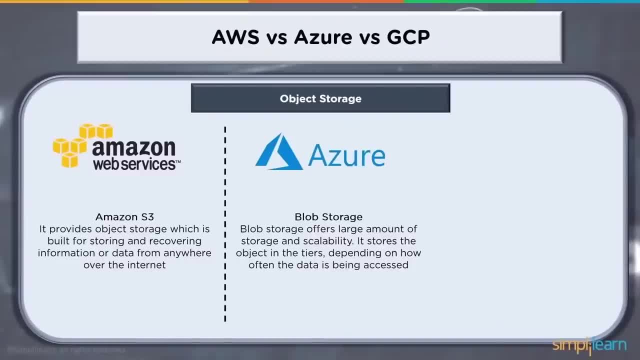 classes which can be selected when a user or an organization intends to use a storage service, and when I speak about storage classes, it basically means having a frequent access storage or a infrequent access storage, or what we call as just an archival solution. Google Cloud has cloud storage and it provides unified object storage for live or archive. 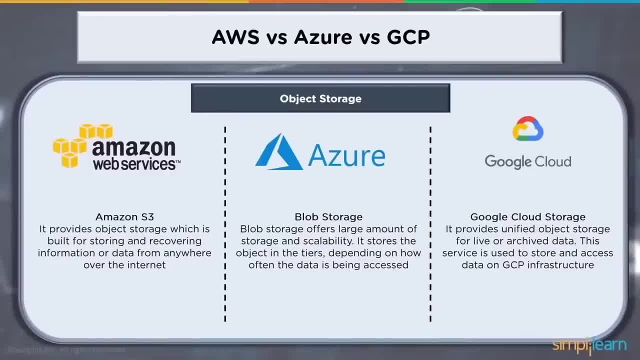 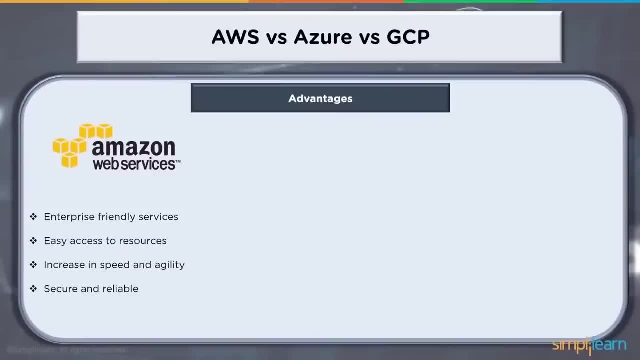 data. This service is used to store and access data on GCP infrastructure. when it comes to advantages, Amazon Web Services has enterprise-friendly services, easy access to resources, increase in speed and agility- and that, too, on demand- and takes care of your security and reliability of resources which are offered. when it comes to Azure, it has better development operations. 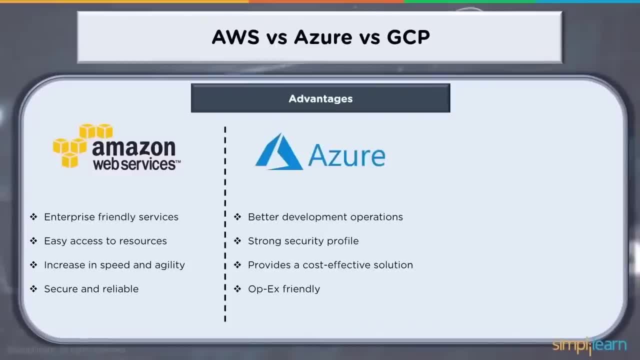 strong security profile. It provides a lot of cost-effective solutions and operation execution friendly. when we talk about Google Cloud, one of the key features here is better pricing than competitors. live migration of virtual machines, which really interests a lot of organizations would want to modernize their infrastructure without having any kind of disruption in their existing. 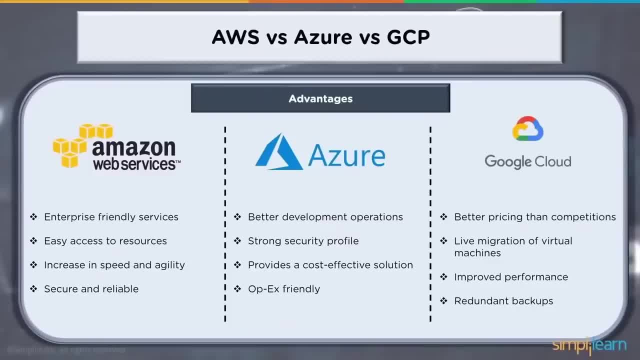 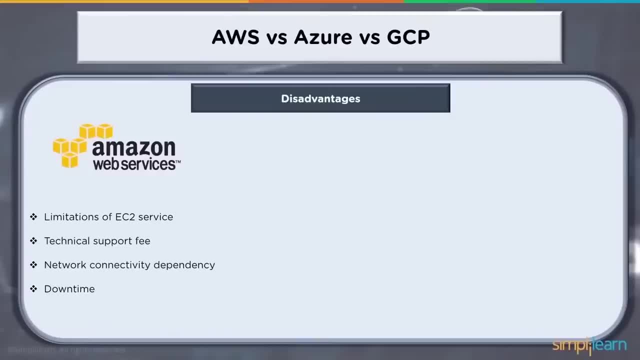 services, improved performance, redundant backups and so on. When it comes to cloud services, It comes to disadvantages. in AWS, you have limitations when it comes to easy to service. well, there are different options in the kind of machines which you can choose, which you can work on. you have a technical support fee which is incurred, network connectivity and 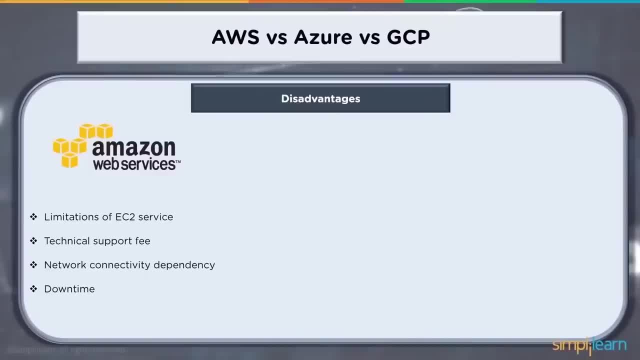 then also downtime, which might be in case when you're migrating as your. it has different code base for cloud and premise Platform as a service. The cloud system is not really as efficient as infrastructure as a service. poor management of GUI and tools. integrated backup- when we talk about Google Cloud support fee is quite 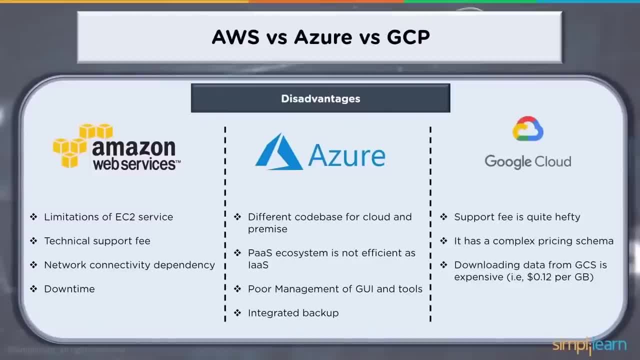 hefty. it depends on what kind of solution or support you would or organization would be interested in. it has a complex pricing schema, although it has different use cases for which any user or any organization can benefit from. Downloading data from Google Cloud services is an expensive option. 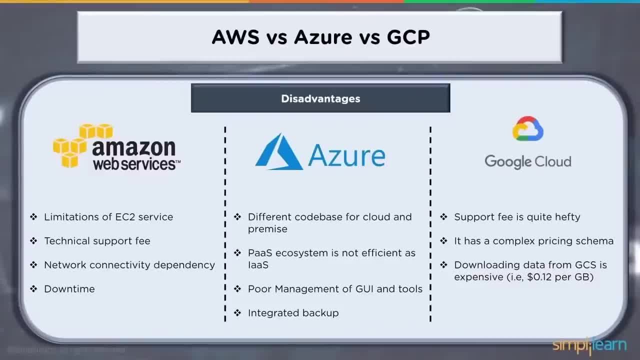 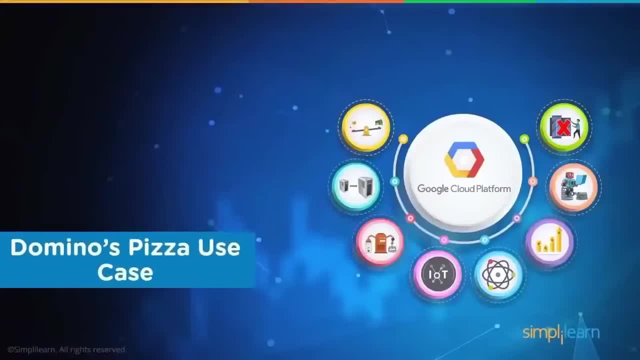 Storage might not be. however, uploading data or downloading data would be an expensive option when we talk about Domino's Pizza use case. now, while we were discussing over these features, I would really want to spend more time in discussing each of these features or services in detail. 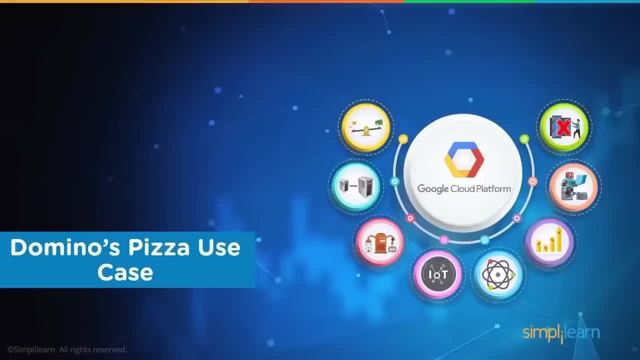 Such as you have Computers, You have Engine, You have Storage, You have Big table, You have Data proc, And so on. So there are huge list of services. now, before we get into your Domino's Pizza use case, let 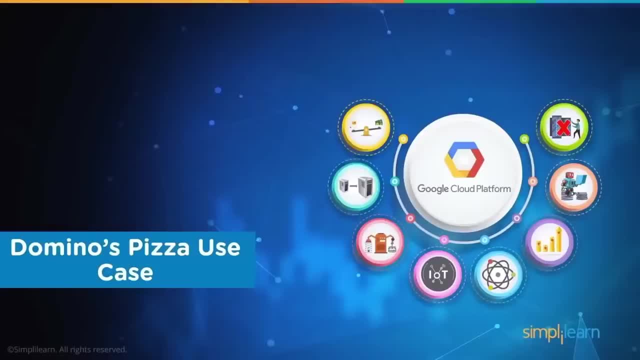 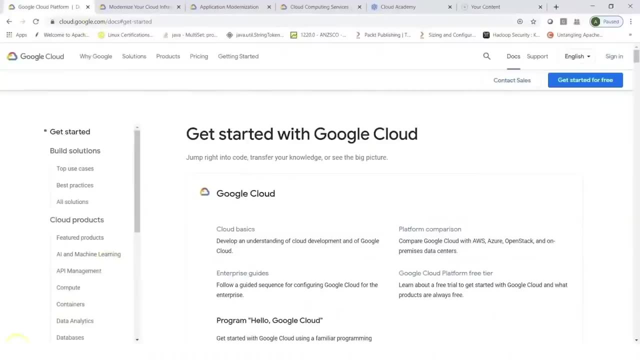 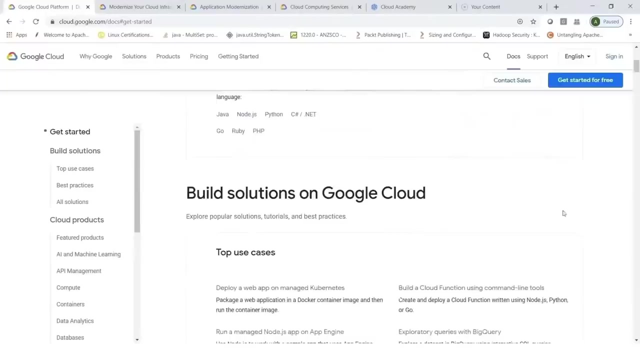 me show you this page on Google Cloud where you can look at different services. so if you go to cloudgooglecom and if you look at get started option under docs, so here you can find build solutions. Look at different use cases. Learn from basics of what is your Google Cloud. what are cloud basics, then you can look at. 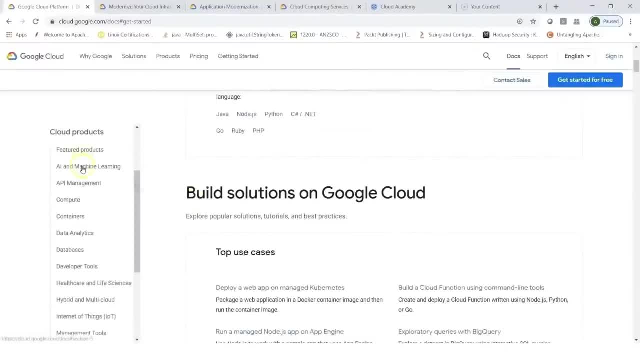 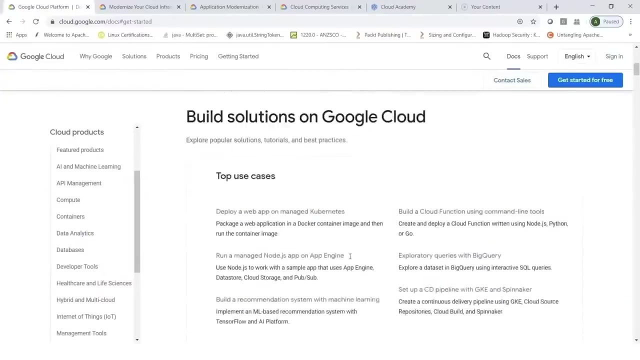 different cloud products. So here you have products in different categories, such as AI and machine learning, API, management, compute containers, data analytics, databases, developer tools and so on, and you can always click on any one of these to look into different solutions which are being offered. what are? 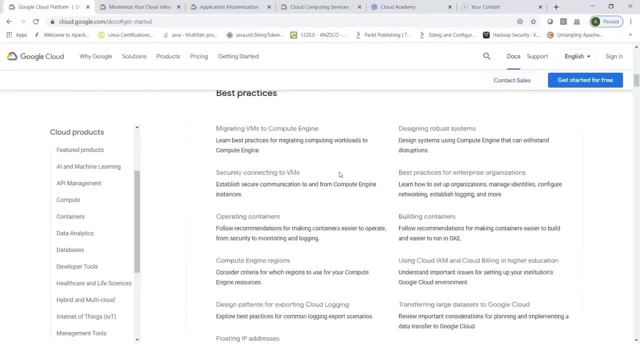 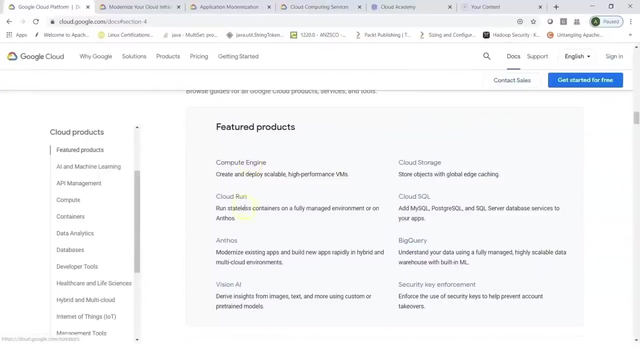 the different use cases? What are the best practices when it comes to migrating VMs to compute engine or operating containers or building containers and so on? You can always look at featured products and that gives you a quick snapshot of what are the different products, such as: you have compute engine, you have cloud run big query which? 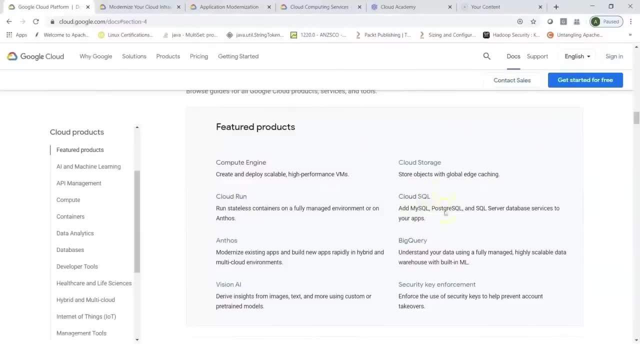 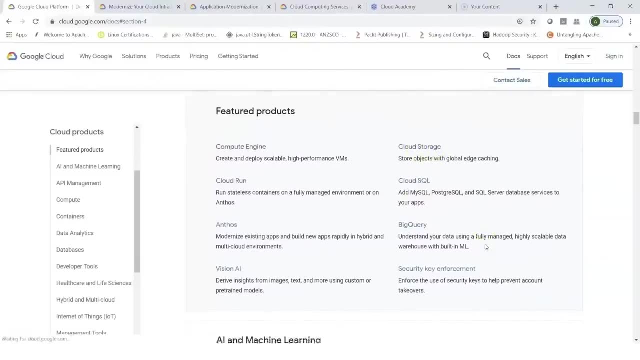 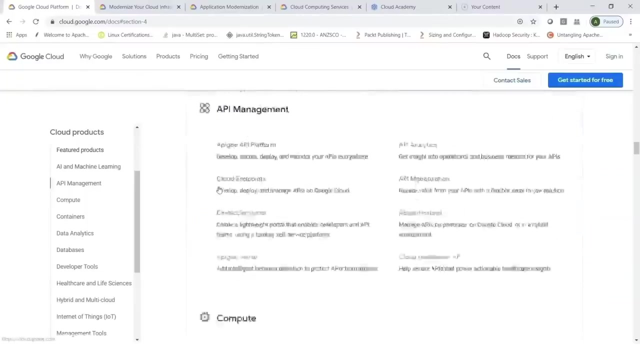 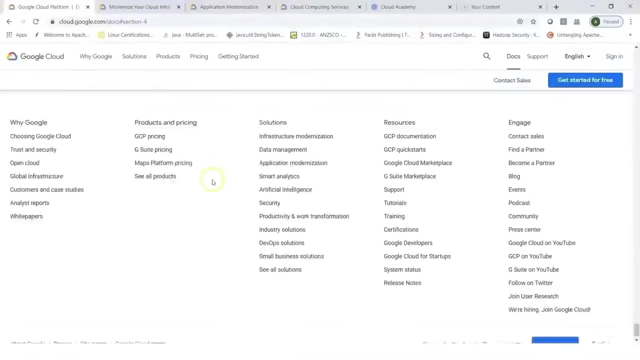 is a data warehouse. you have cloud SQL, which is a managed MySQL or Postgres. you have cloud storage to basically push in any kind of data there. You Key enforcement, AI and machine learning and so on. So you have different feature products. Now, if you scroll down to the lower end of this page, you can again look at different 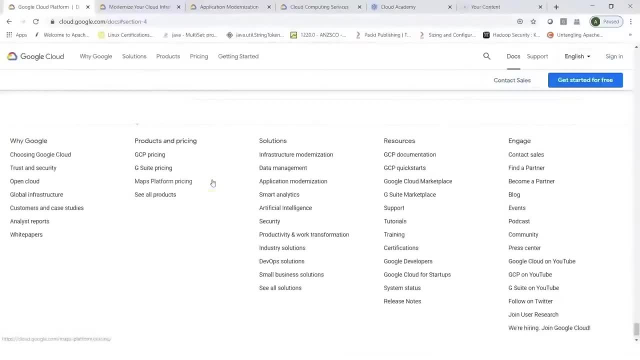 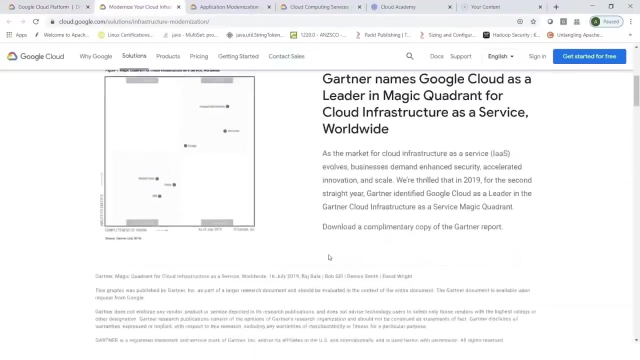 solutions and that would be really interesting to read and learn from. So you have infrastructure modernization, you have application modernization, you have data management and so on. So if I look at infrastructure modernization, You could- You could look at the solutions which Google Cloud offers and what it does when it comes. 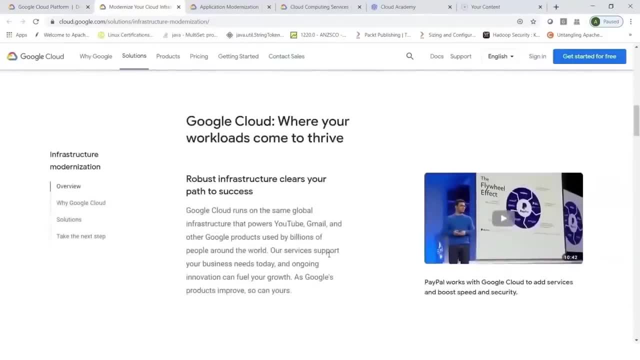 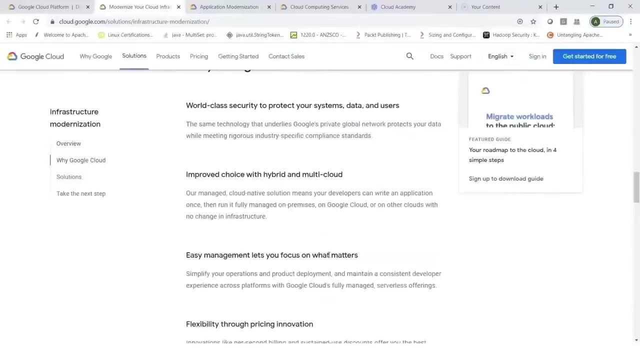 to having your infrastructure modernized or benefiting by integrating with cloud and having immediate benefits of infrastructure modernization. You can look at different use cases, what they are doing, how Google Cloud really helps when it comes to migrating the workloads to a cloud And 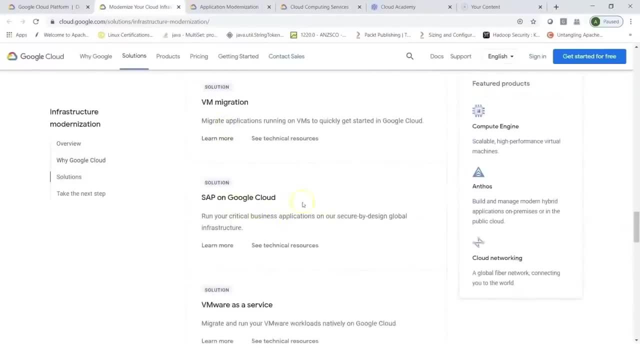 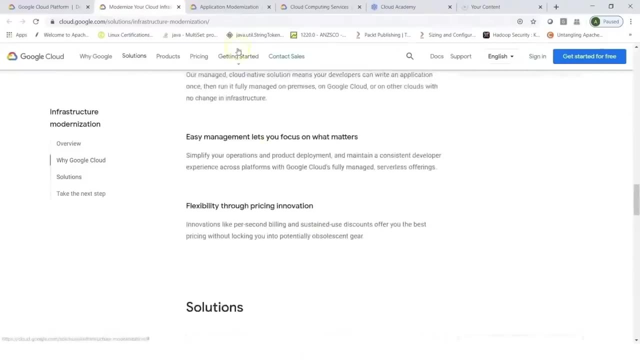 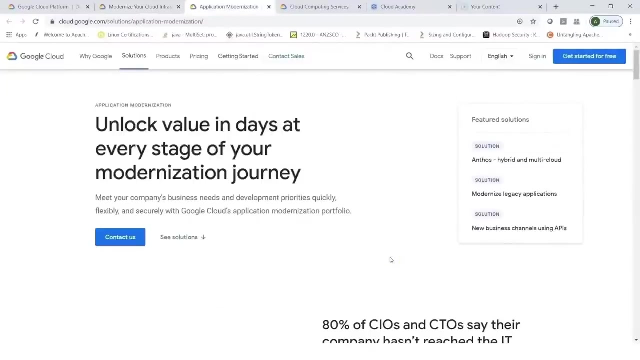 You have different cloud solutions, such as via migration, you have SAP on Google Cloud, VMware as a service and so on, And you could learn from these different solutions which are offered. You can also look at application modernization. so not only infrastructure modernization, but organizations would also be interested in relooking at their applications, relooking 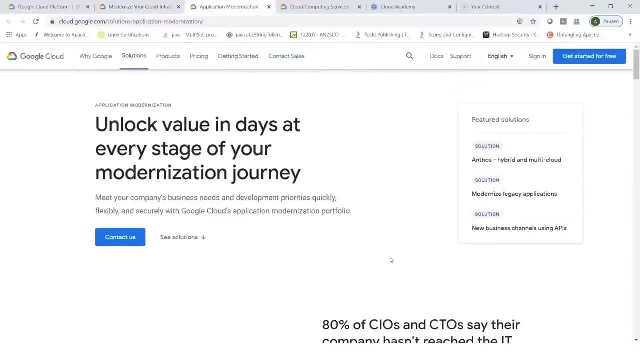 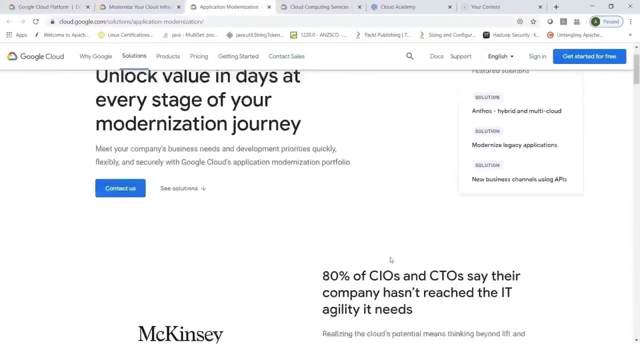 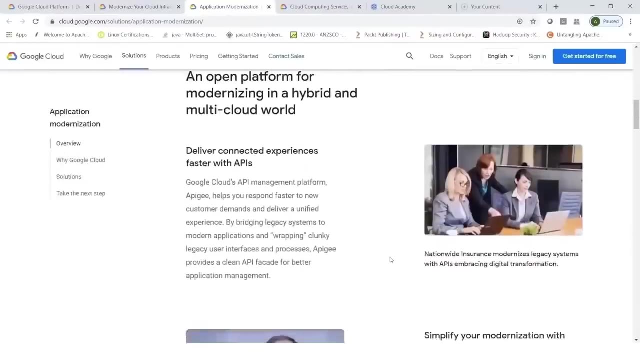 at how these applications could be moved from monolithic to microservices architecture or how Applications Could be adapted from modernization and cloud computing offerings. So you have again different use cases here and which talks about different ways in which Google Cloud can help, how you can modernize your applications, how you can use different 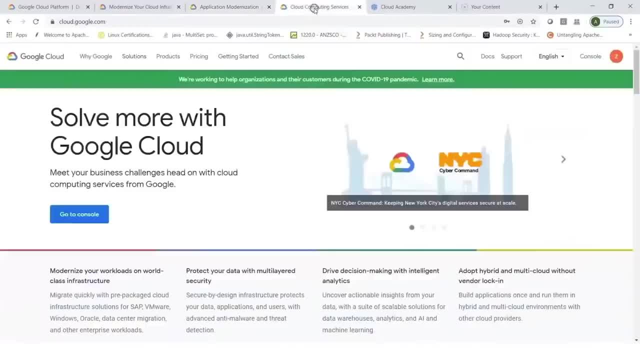 solutions which Google Cloud is offering. Now, when you talk about cloud computing services, you can always go into cloudgooglecom. if you have created a free account, Then you can just log in And every user by default gets a three hundred dollars free credit. 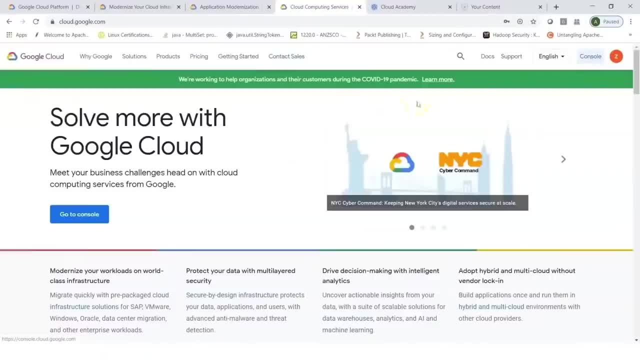 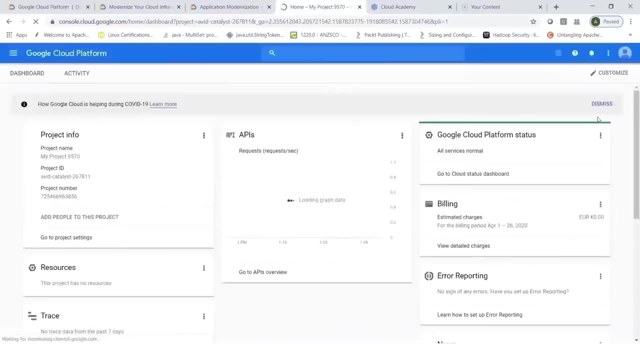 So when they can try out different products, where they can use different services. So here, if I click on console where I'm already logged in with my Gmail account or my Google Cloud account, where I have three hundred dollars free credit, out of which some is being used, 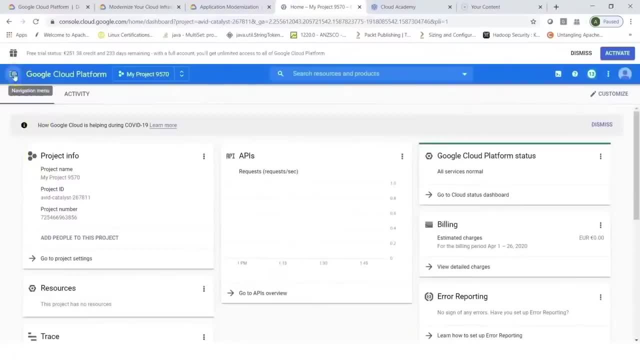 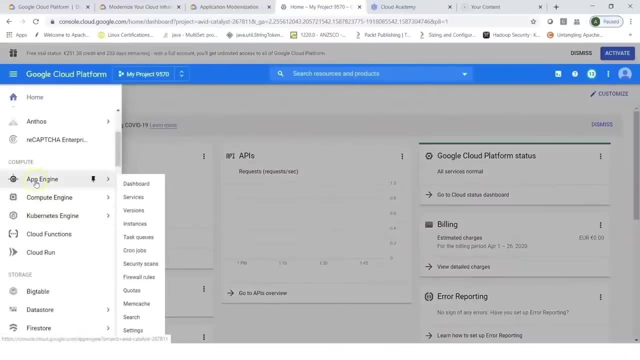 You have a Google Cloud console And here, from the hamburger menu, You can click and you can look at different services within different domains. so you have compute domain, which has different services, such as app. you have compute engine and that basically allows you to use your VM instances, which we were talking about previous slides. 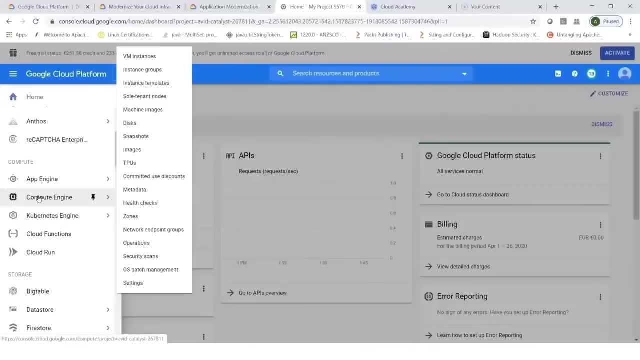 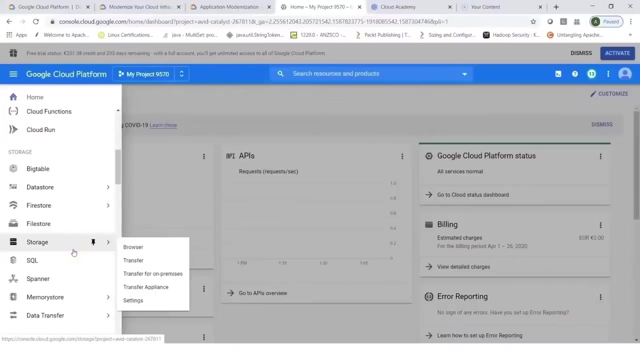 different instance groups. create your templates, use sole tenant nodes, create snapshots or backup of your data, use different zones. you can go for Kubernetes, which is containerized based engine. You have cloud functions, you have cloud run and then you have storage related different options, such as big table. you have data store, fire store, file store storage and so on. 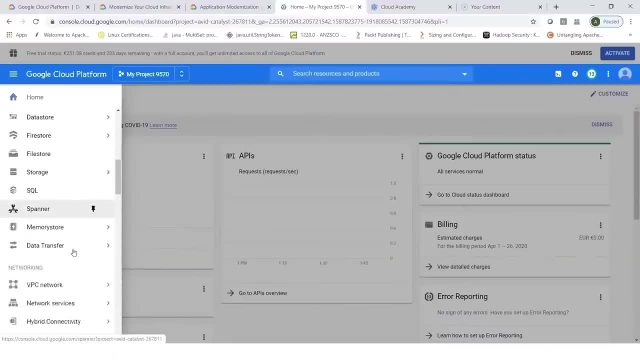 And for each of these services you can read about from the Google's documentation, or anyways, I will be explaining that later. You can also look at networking related, operation related and other tools which are offered by Google Cloud. So these are huge list of services. 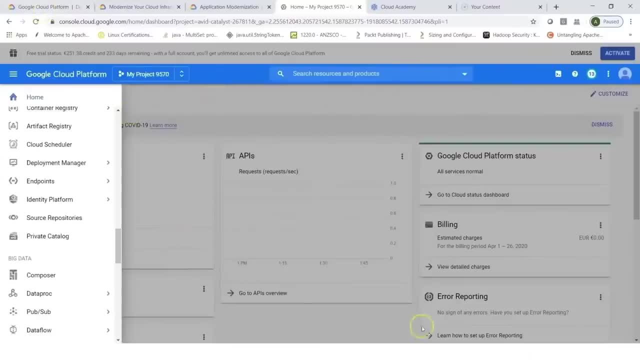 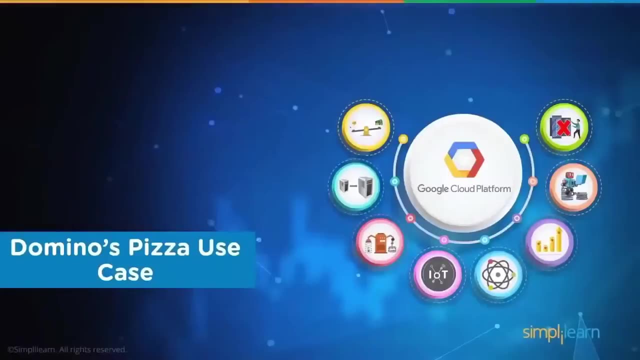 So these are huge list of services Which Google Cloud platform offers in different ways for different use cases. Now let's look at this Domino's Pisa use case and see what it helps us learn about. So you can always access this page by going to this link, which talks about customers and 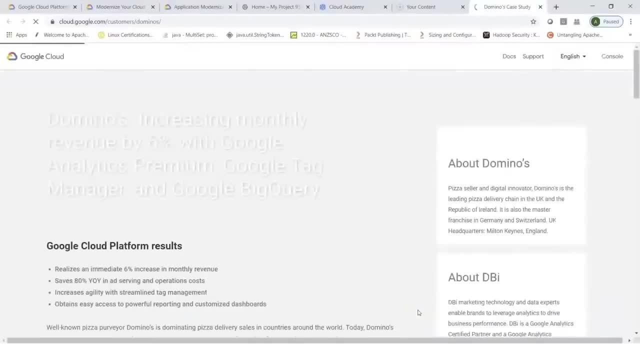 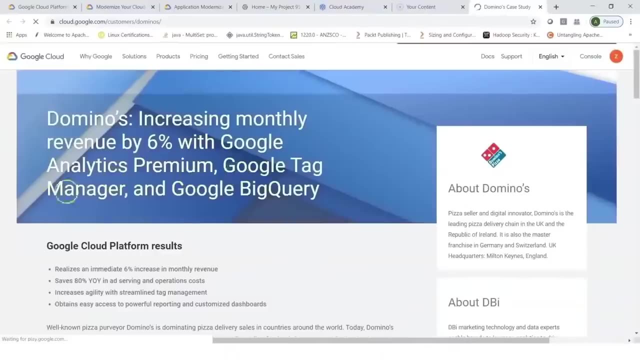 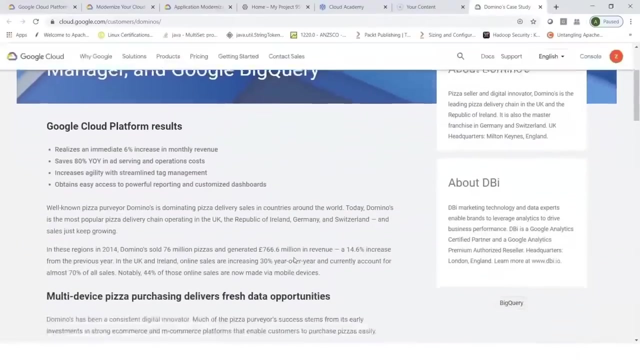 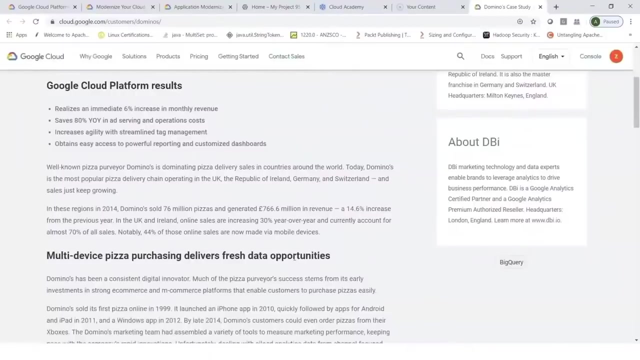 then, which shows you different use cases. So Domino's increasing monthly revenue by six percent with Google Analytics premium, Google Tag Manager and Google BigQuery. So this is basically when Domino's started using GCP, and what was the result of that? Now let's look further into this. 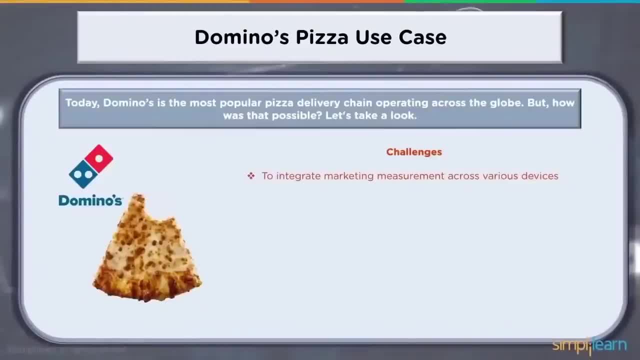 So we all know that Domino is most popular Pisa delivery chain operating across the globe. But how was that possible? Let's take a look. So the challenges were: they wanted to integrate marketing Measurement across various devices, connecting CRM and digital data to create a clear view. 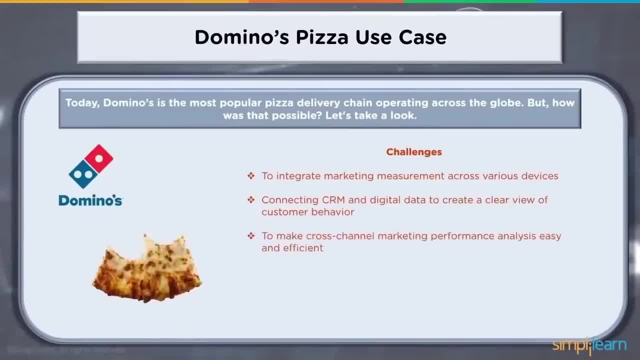 of customer behavior to make cross channel marketing performance analysis easy and efficient. Now, for these challenges which Domino's was facing, the solution was using Google Analytics premium, Google Tag Manager and BigQuery, which were used to integrate digital data sources and CRM data. Reporting was made easier and more efficient by implementing Google Analytics premium because 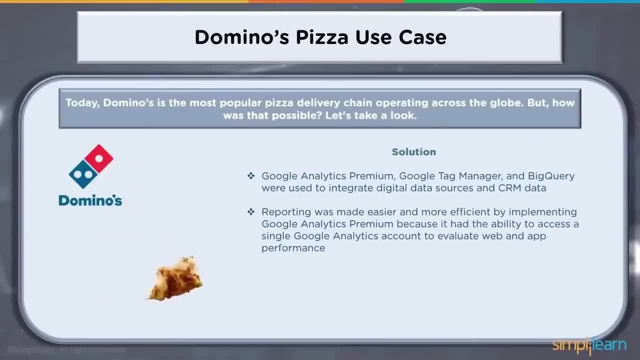 it had the ability to access a single Google Analytics account to evaluate web and app performance. By using the new Google Tag Manager implementation, Domino's were able to act fast. they were able to connect CRM data with digital analytics, which basically provided Domino with greater visibility on customer behavior. 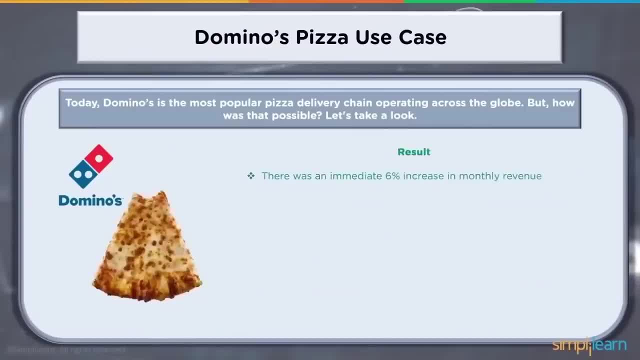 What was the result? There was an immediate six percent increase in monthly revenue. 80 percent of costs and ad serving and operations were saved. increases agility with streamlined tag management. They obtained easy access to powerful reporting and customized dashboards. Now, that was just one simple use case. before we go on to hands on. we can also talk a little. 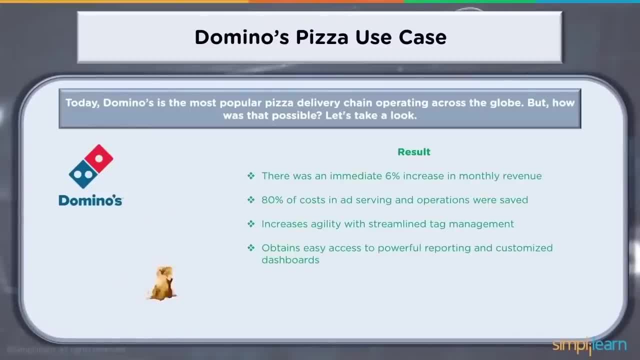 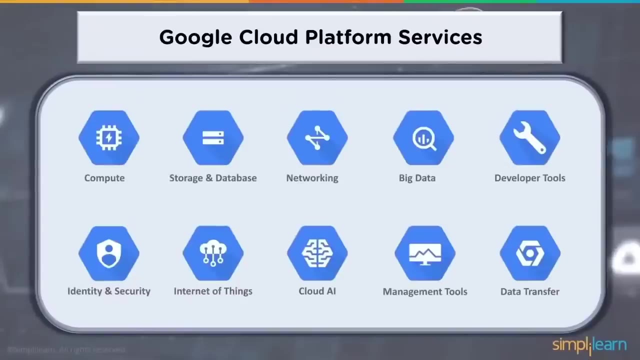 bit back about The services which Google Cloud offers, as we discussed, and some of these services which can really make you think: why not Google Cloud platform? So when we talk about your different cloud platform services, let's learn about some of these services in brief, in what each service is, what it does and how it can help us in. 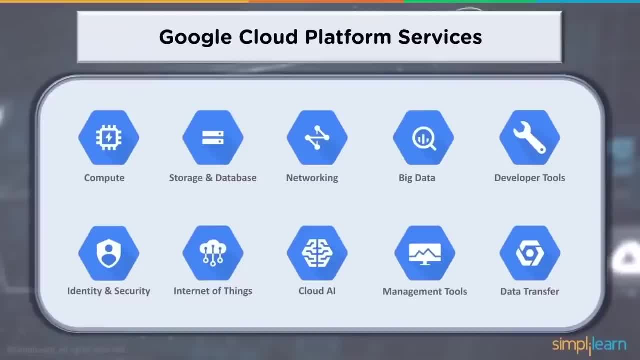 handling our use cases or working with Different Products. So let's learn briefly about different services which Google Cloud platform offers. Now, one of the domains is compute, and then let's look at the compute services which GCP offers. Now, here I can log into the console and this hamburger menu on the top left corner I can. 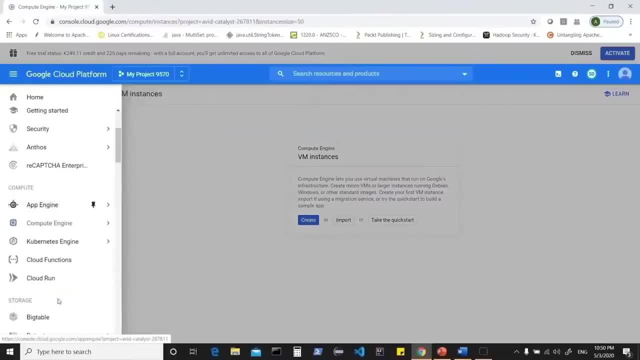 click on this one and go into the compute engine section. So this is the compute domain which has app engine, Kubernetes, engine, Cloud fact functions and cloud run. So these are your different services which are offered within the compute domain and here we can get into compute engine by clicking on this one and then basically going to VM. 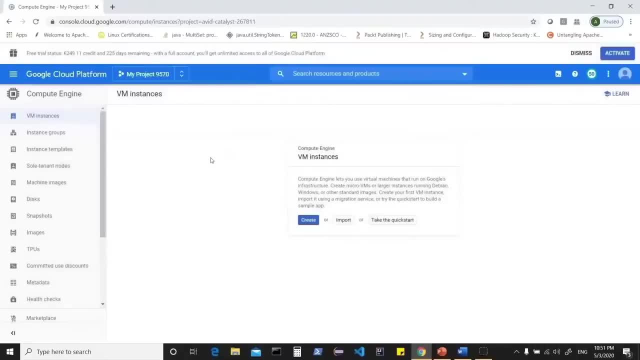 instances. So before we see how we can use this compute engine, let's understand about some of the features of compute engine, which basically offers scalable, high performance virtual machines which are configurable and which runs in Google's data center. So from here you can select VM for your needs, for your general purpose or workload optimized. 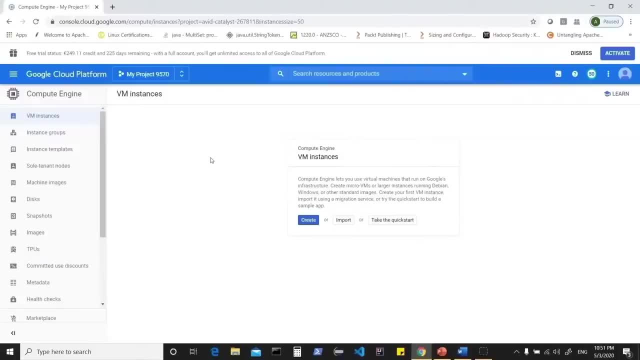 predefined or custom machines. Now, here you can integrate compute with other Google Cloud services, such as AI, ML and other data analytics services. You have different machines which are offered here, such as general purpose, which provide a balance In price and performance, which are well suited for most workloads, including line of business. 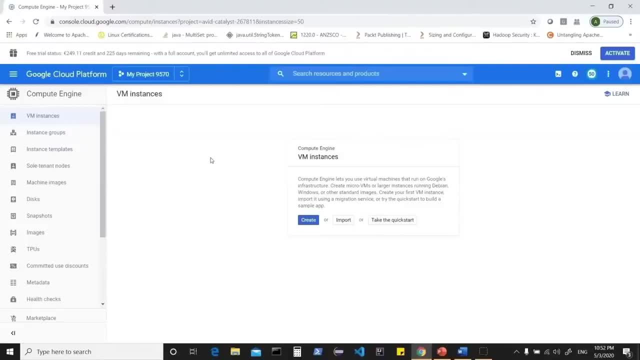 applications, web services and databases. You also have compute optimized machines which offer consistent high end virtual CPU core performance and which are mainly good for gaming, EDA, high process computing and other such applications. Apart from general purpose compute optimized, You also have memory optimized machines. 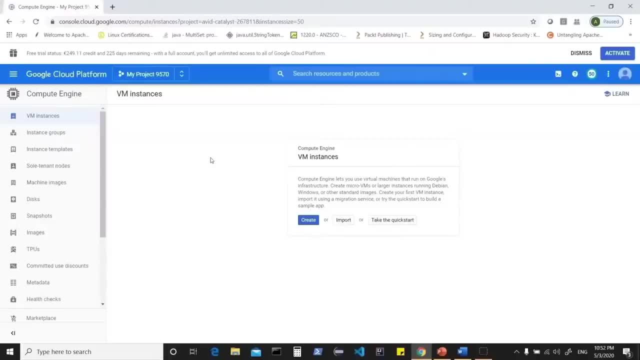 You also have memory optimized machines, Which offer highest amount of memory, and these VMs are basically well suited for in memory databases such as SAP HANA, real time analytics and in memory cache. Now we can see these options here. You can click on VM instances while you're logged in into your Google Cloud console. 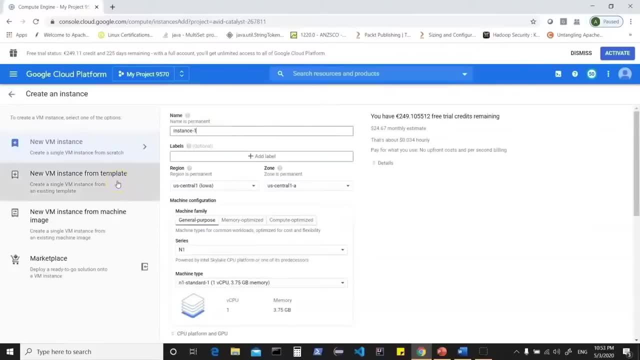 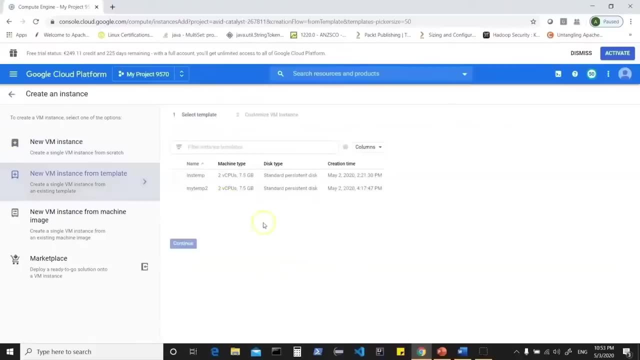 Here you can even create an instance template which can be used to spin up instances, For example, if I click on new VM instance from a template. There are some templates which I have already created for my usage. Now here I can basically use one of these templates, or what I can do is I can go back. 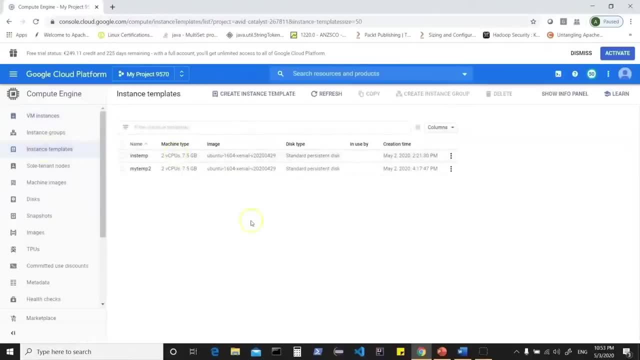 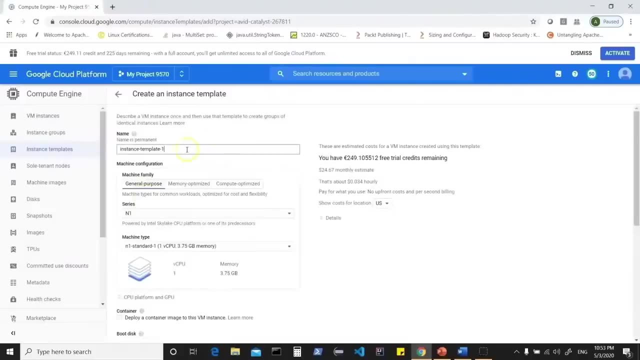 I can go into instance templates and this basically allows me to create a template. So you can click on create instance template, which basically allows you to create templates which can be used to spin up different instances. We can give a name to the template. For example, we can say template instance. 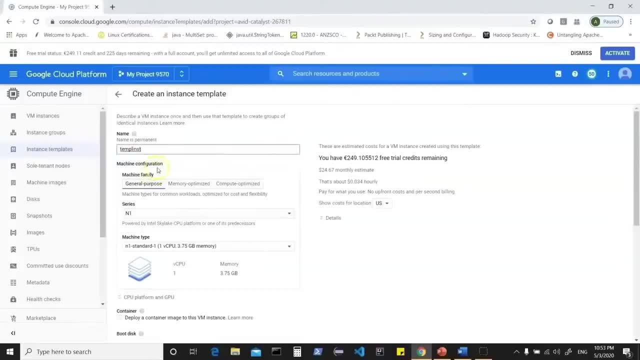 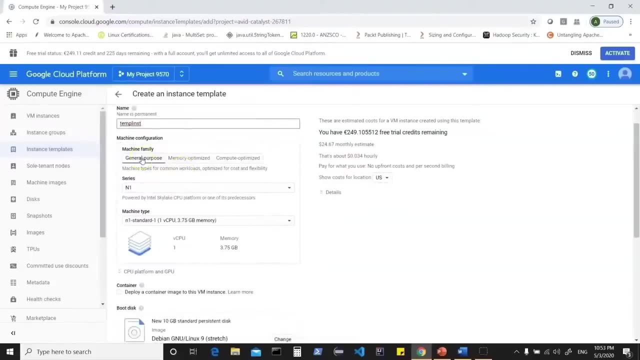 For instance, now here I can choose machine configurations and this is where you have different options, So you have general purpose, as I mentioned, which provide a balance between price and performance. You have memory optimized, which are large memory machine types for memory intensive workloads. 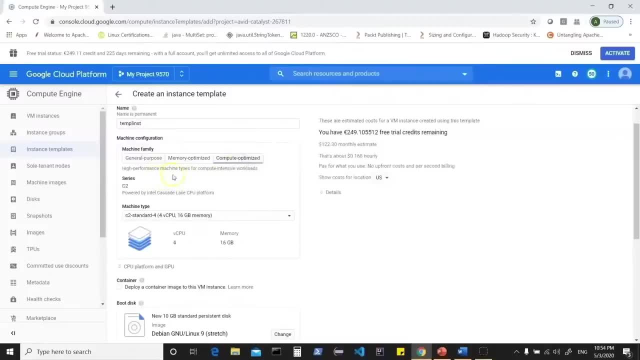 You also have compute optimized, which basically give you high performance machine types for compute intensive workloads. So you can choose any machine configuration which is available here Based on your requirements. Now, if you click on general purpose, that has different options here. So you look into the series where you have N1 series. 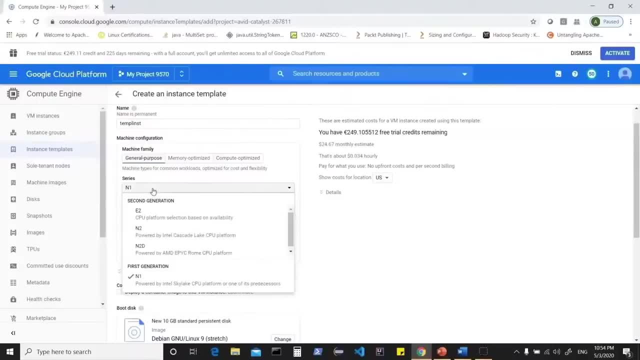 You have E2, which are CPU platform selection based on availability. You have N2 and N2D, So let's just have N1 selected. Now you also have here which talks about machine types, and here we can choose the configuration which we are interested in. 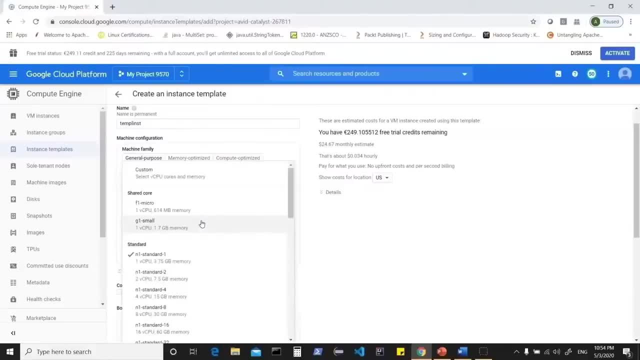 Depending on the application. So we can choose a machine. so by default it shows one virtual CPU core and 3.5 gigabyte of memory or RAM. You could choose a higher end machine. so as of now I'll just say N1 standard. 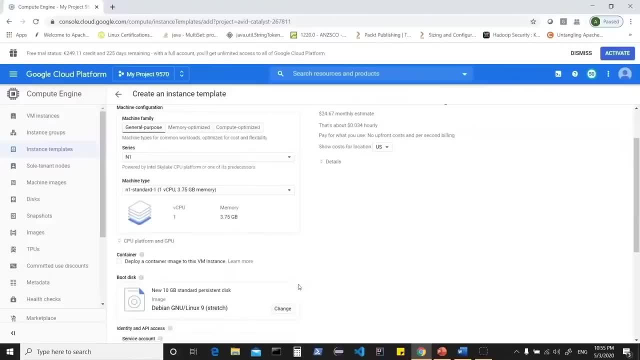 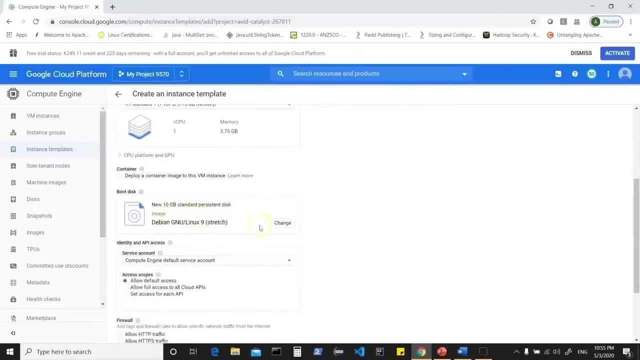 Now that basically allows me to choose these machines. So there are different features which your compute offers, such as you have live migration for VMs, You have preemptible virtual machines, You have sole tenant nodes, and all those options can be seen here. Now, in this machine, for my boot disk, I can select a distribution which I would be interested. 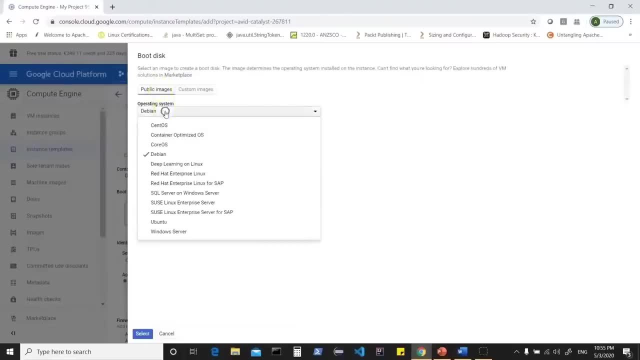 in, For example, I could be going for public images and I can choose, for example, Ubuntu, and then I can choose a version, So it shows me 16.04 and you also have latest versions, such as Ubuntu 20. You can choose one of these and here it asks you to choose the boot disk type. so that could. 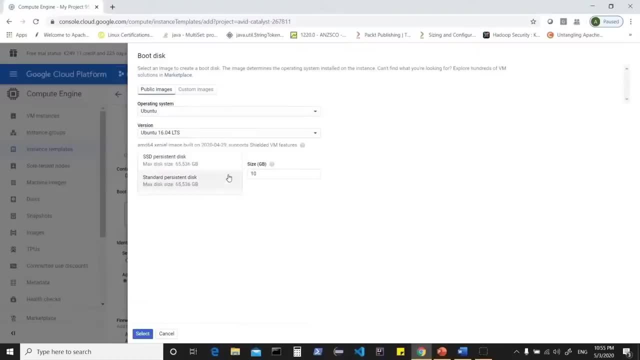 be standard persistent disk, which is HDD. So that's it. Now let's talk about SSDs which are low in performance and you can say low in cost in comparison to SSDs. So SSDs give you better performance, but then they are little expensive than using standard. 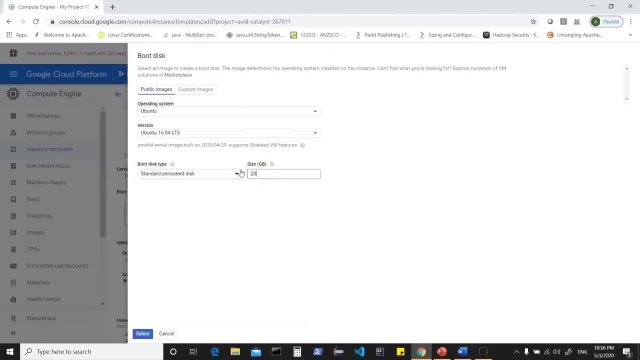 persistent disk. We can choose this and we can give a disk size, for example, 20 gigabyte, and I can click on select. Before clicking on select, I can click on custom images and that shows me. if you have any other images created in your project, you could use those. 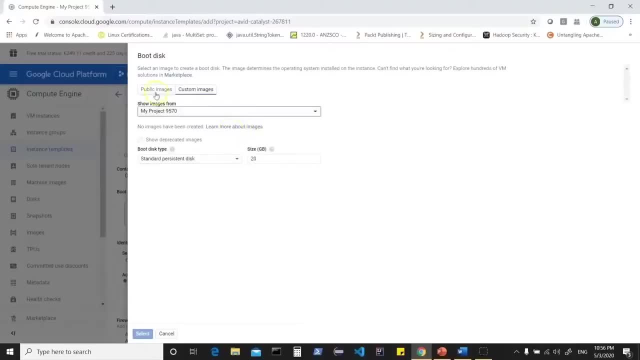 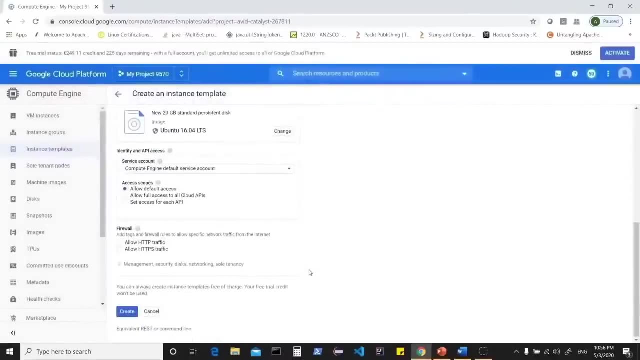 You could also learn how to use custom images. You can also learn about images by clicking on this link, So we'll click on public images. We have chosen this distribution. Let's do a select, and now, here you have identity and API access management. 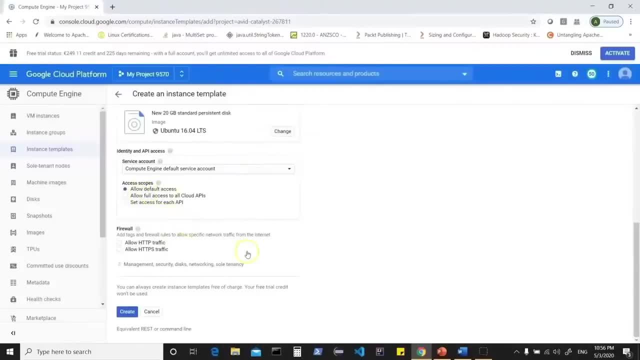 So let this be default. You can say: allow default access and what you need is, depending on the services we can choose. it allows HTTP and HTTPS traffic. Now we would also need some way to connect to these machines. So when you set up an instance, 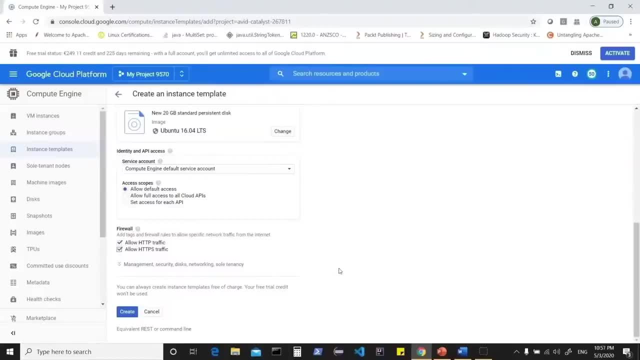 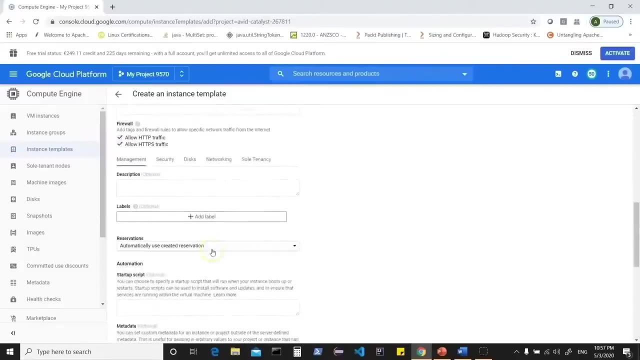 By default, you can do SSH into it using the Google Cloud console or from Cloud Shell. You can also give a private and a public key. So here you have the option where you can give all these details. So when it comes to management, it tells you: would you want to go for reservations and? 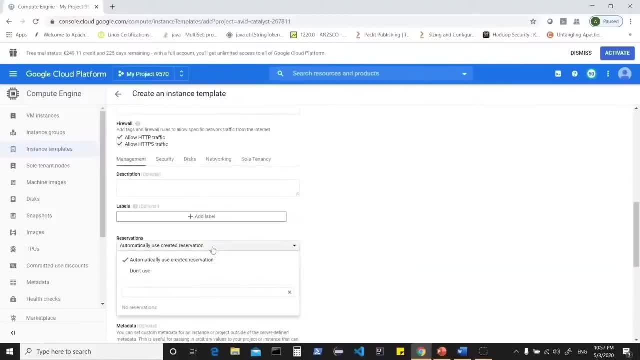 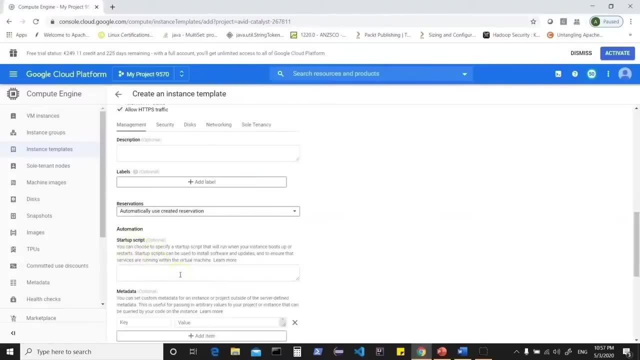 you can say: automatically use created reservation. You could also say no, you would not want to use a reservation. You can also set up or provide a startup script which you would want to give Whenever your machines come up. and here you have the options of preemptibility. 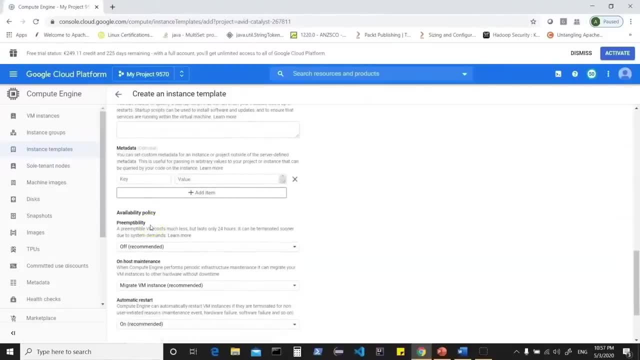 So compute offers preemptible virtual machines. so that is mainly when you would want to run bad jobs and fault tolerant workloads on these machines, and you can benefit with a reduced cost for your virtual CPU and memory by 80 percent. So these are virtual machines which would be lasting less than 24 hours. 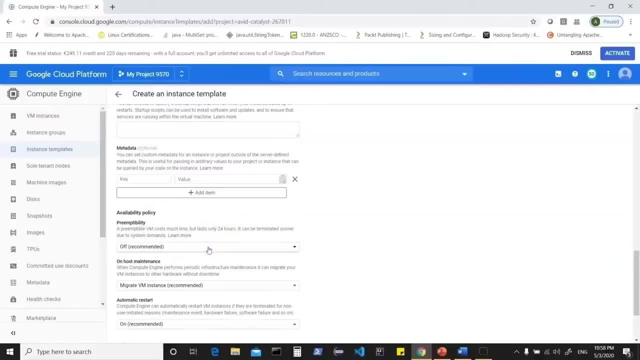 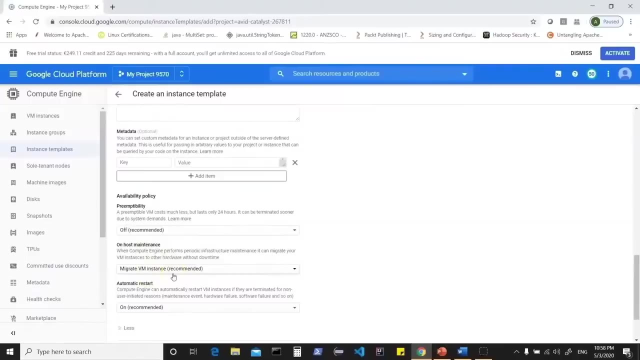 Now, by default, this is off. It purely depends on your workload, what you would want to run on these instances. I could just go ahead and select preemptible. being on that and use this feature of compute. You also have on host maintenance, which talks about what would be happening with this compute. 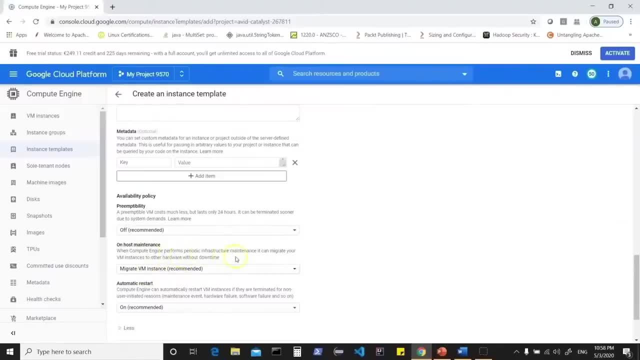 engine instance. So when compute engine performs periodic infrastructure maintenance it can migrate your VM instances to other hardware. and this is one of the features which compute engine offers, which we call as live migration for VMs. Here your compute engine can live migrate between host systems. that is the underlying. 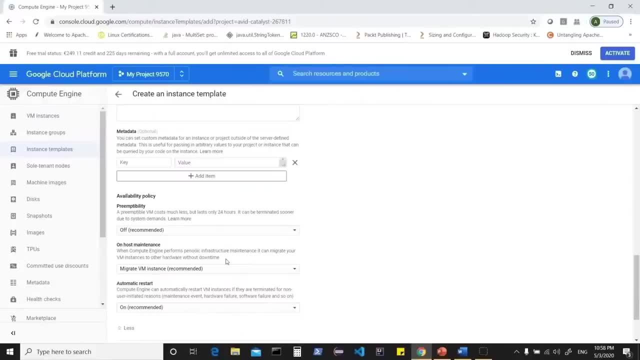 systems on which these VM instances are based on without rebooting, which will keep your application running even when host system require maintenance. And here it says migrate VM instance recommended and let that be as it is. You can also say that if there is a maintenance happening, you can terminate the VM instance. 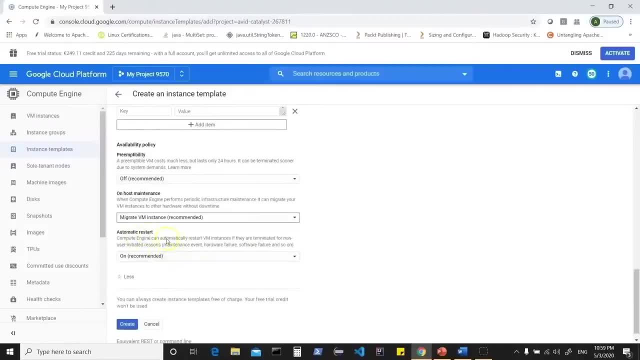 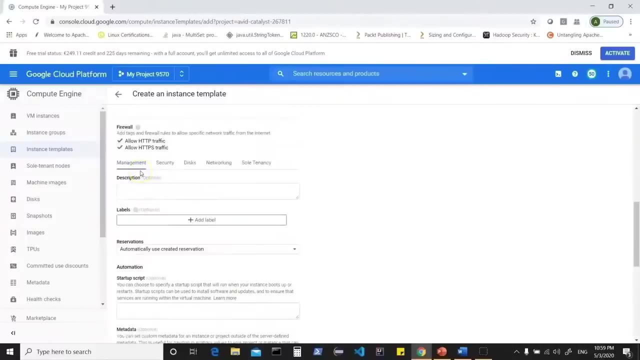 Now it also talks about automatic restart, which is on, Which basically means compute engine can automatically restart VM instances if they are terminated from non user initiated reasons. So these are all the settings which are available in management and it also tells us the different features which we have. 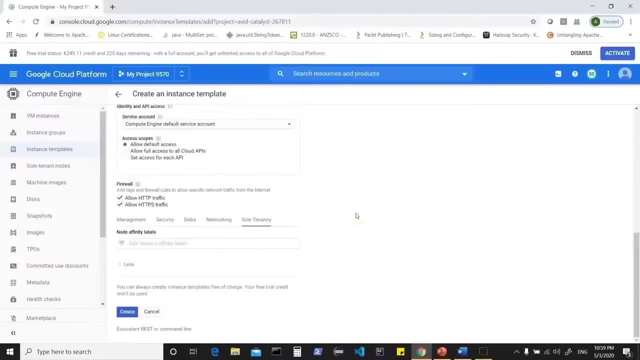 There is also a feature called sole tenancy, which basically means sold tenant nodes which can be chosen So you can have physical compute engine servers dedicated exclusively for your use- and this is usually good When you are talking about bring your own license applications. So sole tenant nodes give you access to same machine types and VM configuration options. 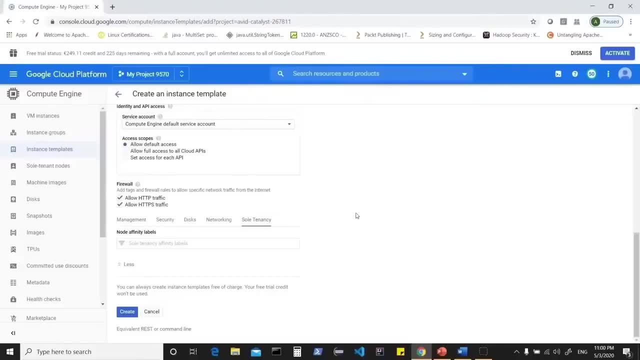 as a regular compute instances. However, these might be a little expensive. We can choose this one. We can also look into networking, which basically shows the default setup which goes for auto subnet. You can also choose a particular IP if that is required, but that would cost more. 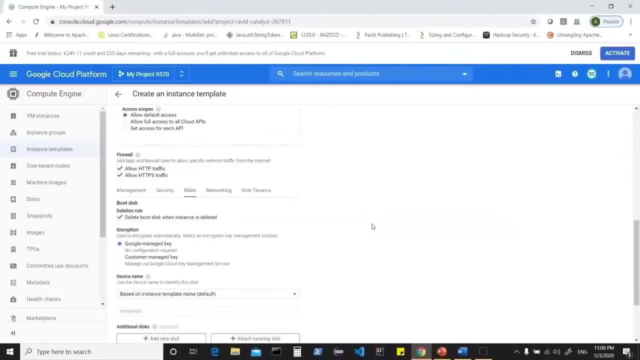 You can click on disks Which talk about: what do you want to do with the boot disk when the instance is deleted? What is the encryption mechanism you would want to use? and here, finally, you have security. So, basically, as I said, you can SSH into instance using the cloud console option and you can 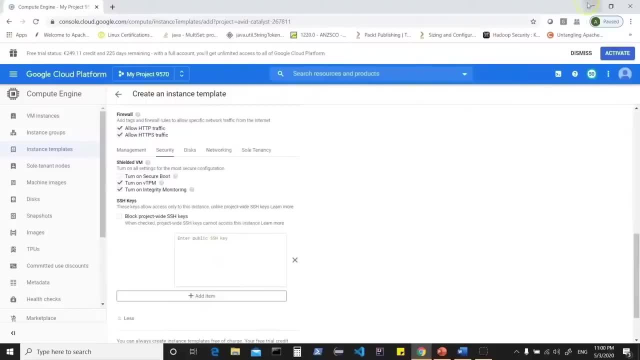 also provide a public SSH key. So one way of doing that: if you intend to use an external SSH client such as putty to connect, you can create a key. So, for example, I can go into putty gen and here I can say generate. 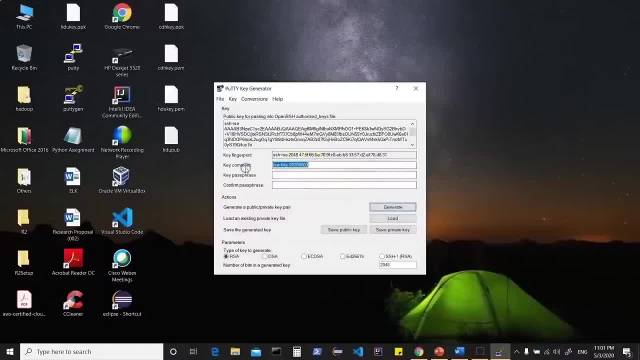 Just move my cursor over here and that will create a key. I can give a name to this one, So I'll say SDU will be user name. I'll give a simple password which I will use to log in to this machine, and then I can save. 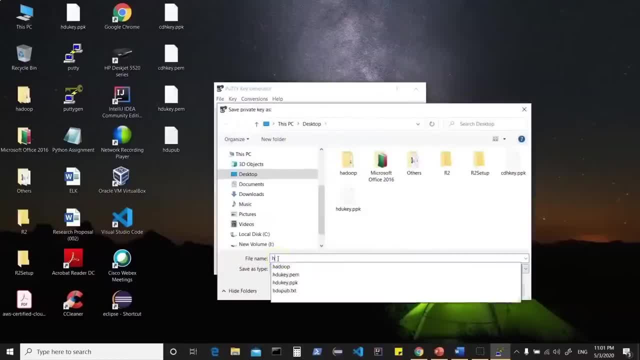 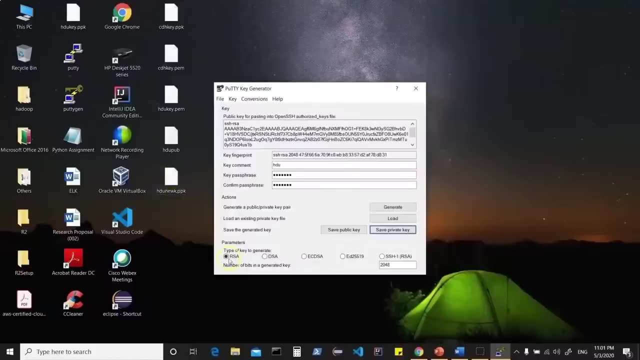 this private key which will get saved. So let's say it's SDU new key and this gets saved in a dot PPK file which is usually used when you use An external SSH client to connect. So save this one and that saves a PPK file on your desktop. 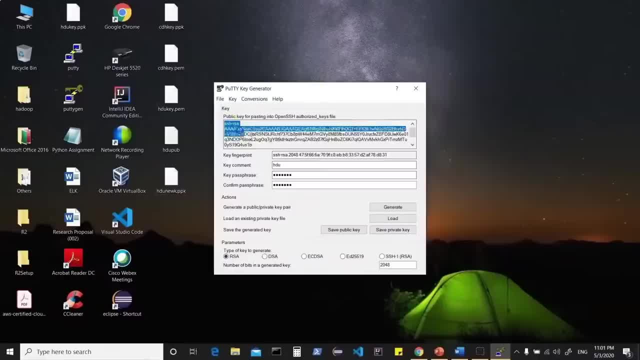 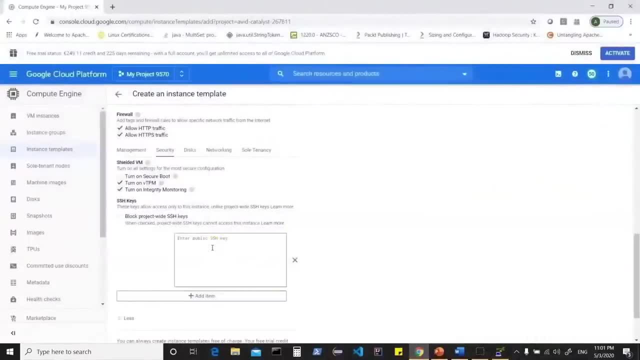 What you can also do is you can copy this public key content from here- and this is what we would want to give in our instance here- So so that the public key gets stored on the instance and private key is what we will use to connect. 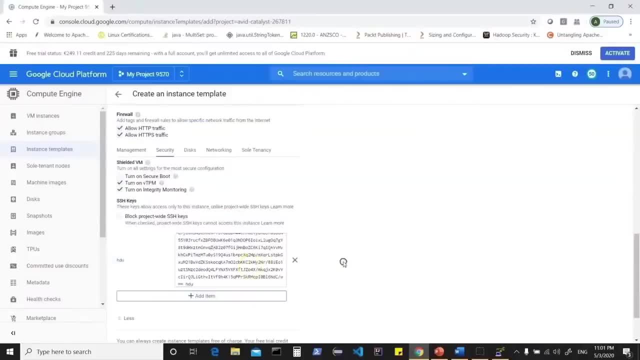 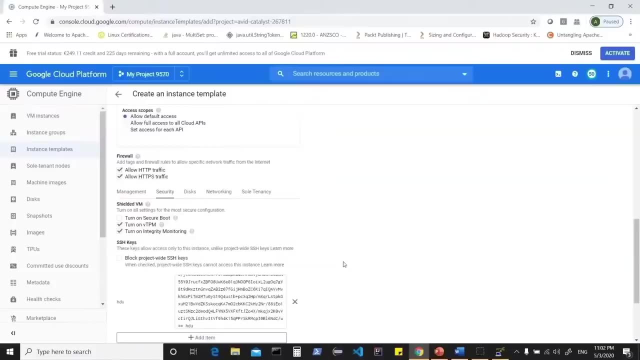 So once I paste it here, it resolves the name to SDU and we have given the public key. Now, in certain cases, you may want to use a software which uses SSH to connect to the machine, and that software might not be such as your putty. 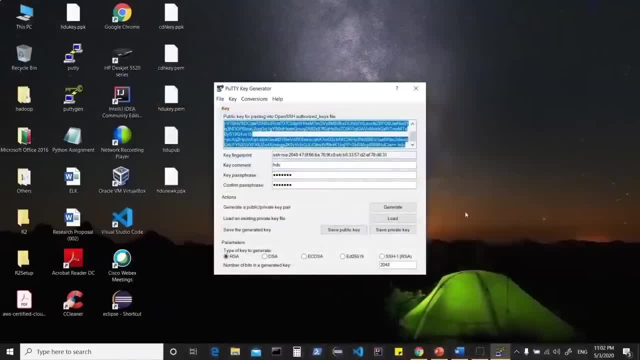 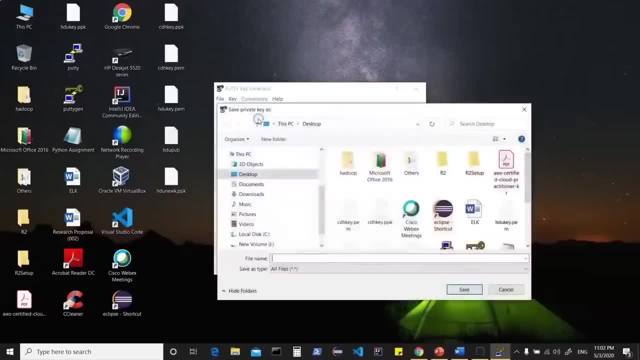 So in that case you may want a PEM file or a private key which is saved as a dot PEM file. So you can also do that by going to conversions and do export, open SSH key and then save it. So I'll say: SDU, new key. 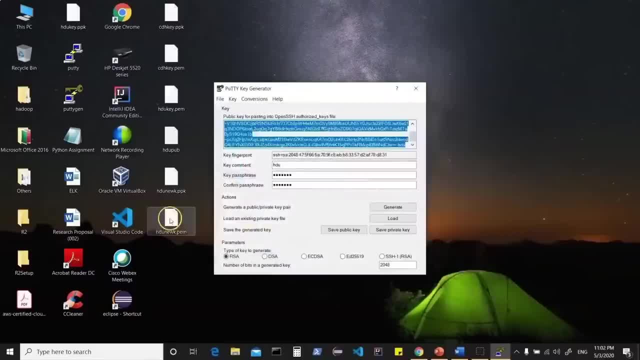 But then this one will be saved as a PEM file on my machine. So that's it. So you have PPK file which allows you to use putty to connect to the instance You have a PEM, in case a software needs directly SSH to these machines. 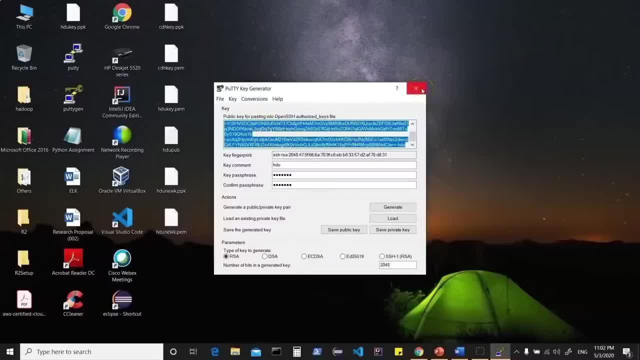 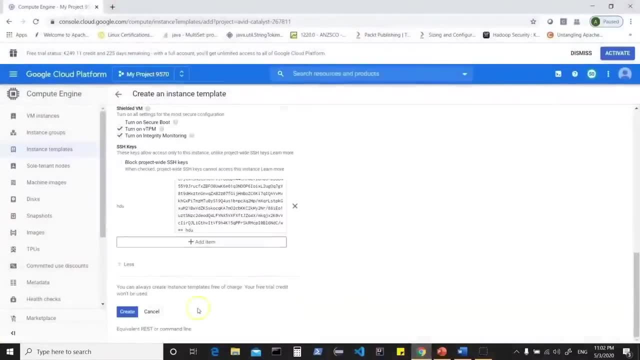 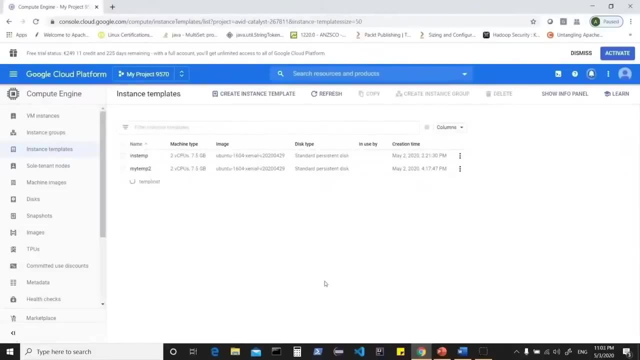 You also have the public key, which we have already provided in the machine. Now, once this is done, I can close PuttyGen. I can go back to this page where I'm creating an instance template, and then I can just click on create. So this has created an instance template which I can use to spin up my instances any number. 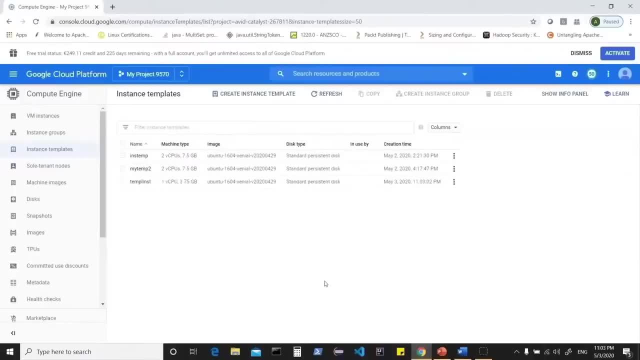 of instances using the same template. Only thing which I would have to do is change the region where I would want the instance to run. So now that we have created instance- and that's my this one- the third option- I can go back to VM instances. 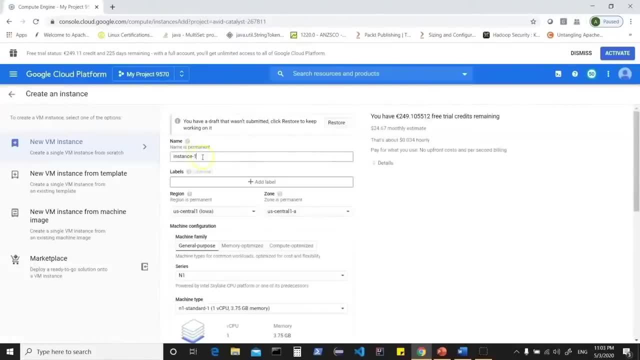 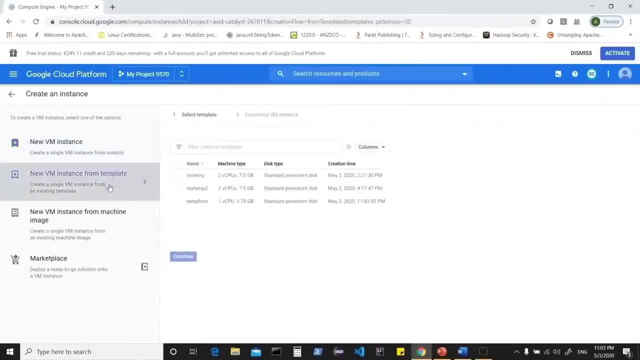 Now I can click on create, and here I can either create an instance from scratch by giving all the details again, or I can just use my template so I can click on new VM instance from a template. Choose my template, Click on Continue and once this is done, I can give my instance name. 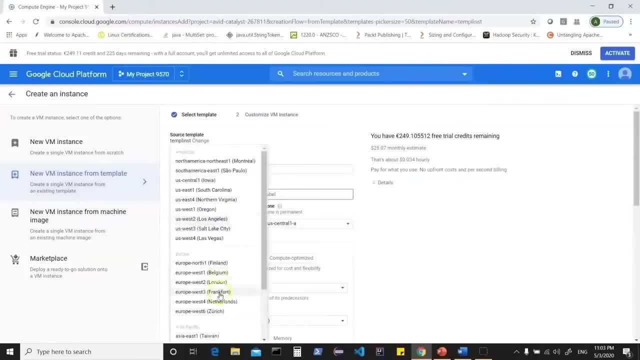 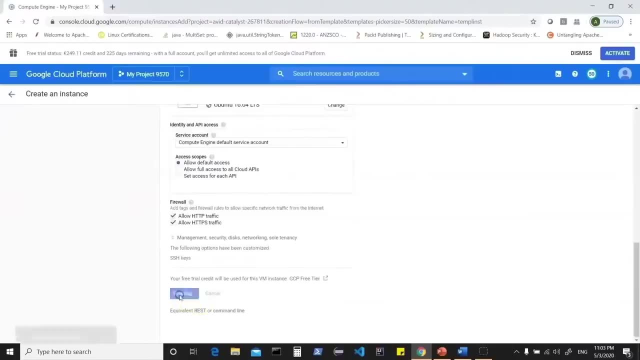 So let's say, see one, I can choose the region, so I will choose Frankfurt and then rest. everything is auto populated based on the template, what you have given and you click on create Now. this basically allows you to spin up an instance and you can create any number of 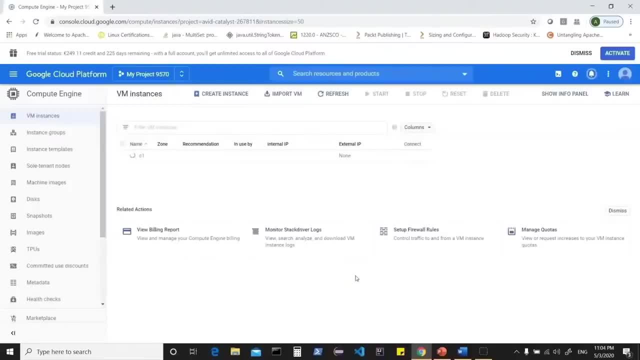 instances. using your template, You could have already created a new instance right from scratch. Now, once the instance is created, this has a public IP And a private IP. private IP will not change unless you would want to set up a new machine, but public IP will change every time you stop and start the machine. 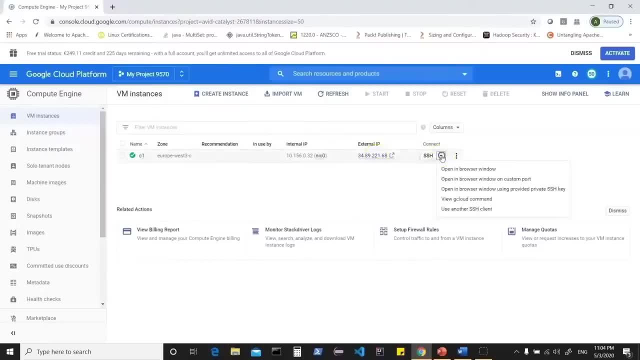 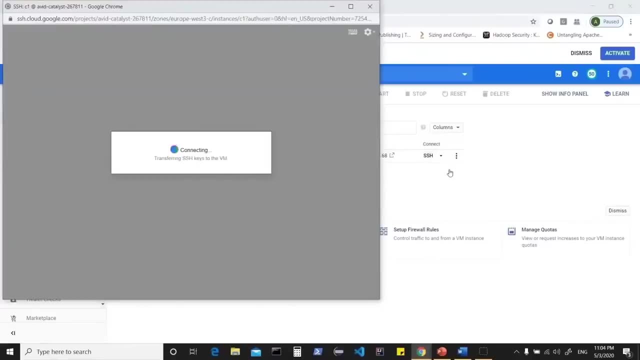 Now this is what we need to connect to this machine. I can also do a SSH from here by doing this and open in a browser window. Let's click on this. So this is an internal way of connecting to your instance using SSH. Let's wait, because it would be transferring the SSH keys to the VM. 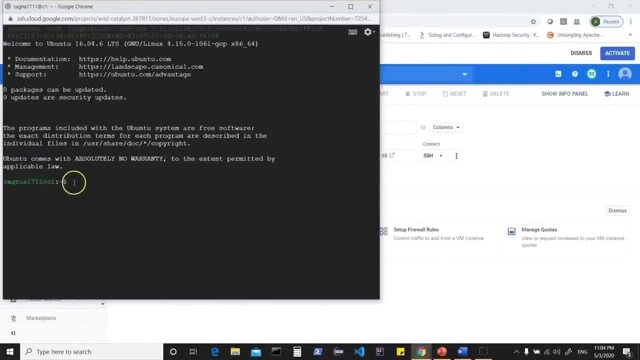 It establishes a connection and I am connected to my machine. What we can easily do is to confirm if we are in the right machine. We can just do a LS to look at the file system. What we can also do is we can basically log in as root by doing a sudo su, and that allows. 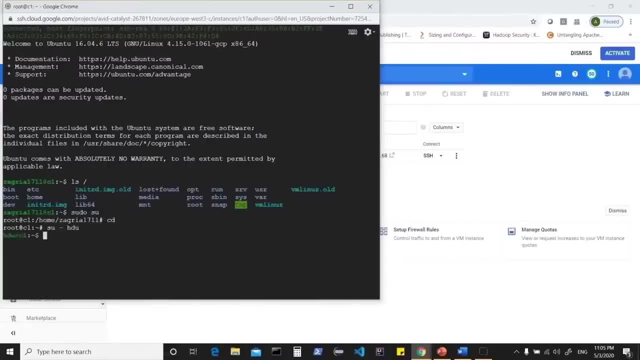 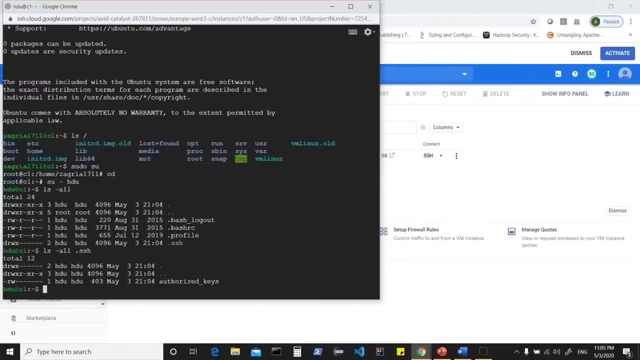 you to get into the machine as root And from here I can switch to HDU user, which will have a ssh directory in home and that basically has authorized keys, And if we would want to see if this one contains my public key, I can just do a catssh and 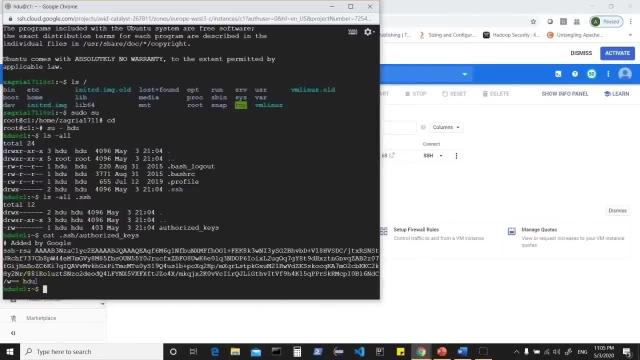 then look into authorized keys and this shows me the public key which we had initially added to our instance. So this confirms that we are logged into the machine which we created. Now I can close this and what I can also do is I can copy this public IP. 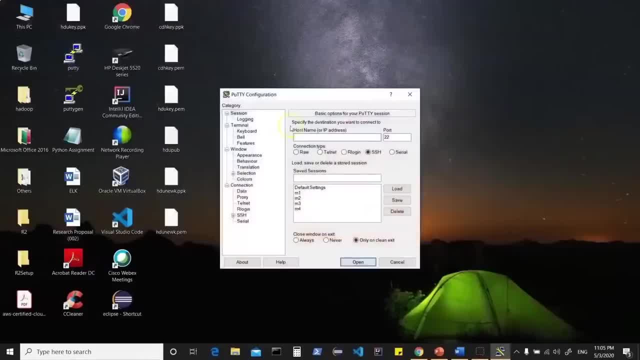 So let's do a copy to click board. Now go to putty And here I'll say host name, where I'll say HDU, Give my public key. I'll click on SSH and in SSH I'll go to authentication. Now here we need to give our PPK file. 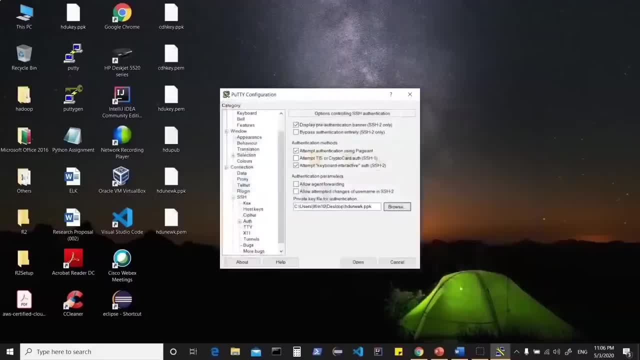 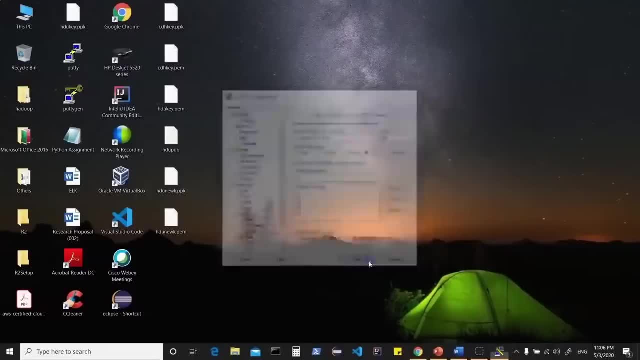 So the PPK file was HDU. new key. Select this one. Come back here, Come to the session, Give it a name, For example C1.. Save it And then you can just say open and say yes and you are logged in to your machine. 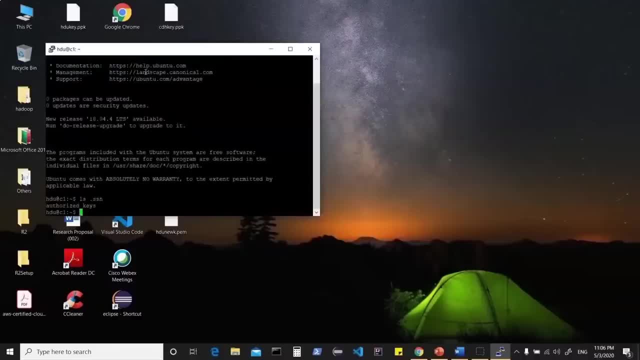 Now, once you're logged in, You can always do it Minus SSH, and that shows you the file. So this is how you have just used the Compute Engine to spin up an instance, But we used a template which basically allowed me to create this instance and then I can. 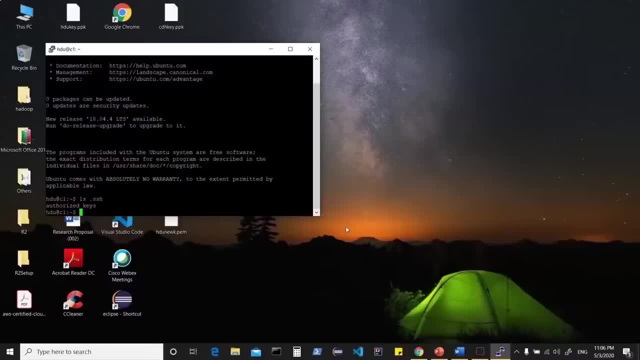 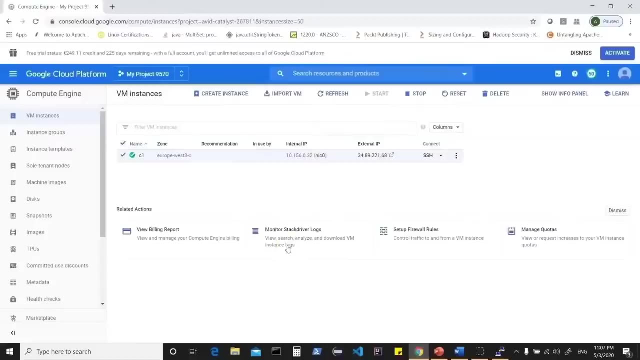 connect to this instance and then I can start working on this. So when we talk about features of Compute Engine, it has predefined machine types, as we saw. So Compute Engine offers different predefined virtual machines And this they have configurations for every need from small general purpose instances. 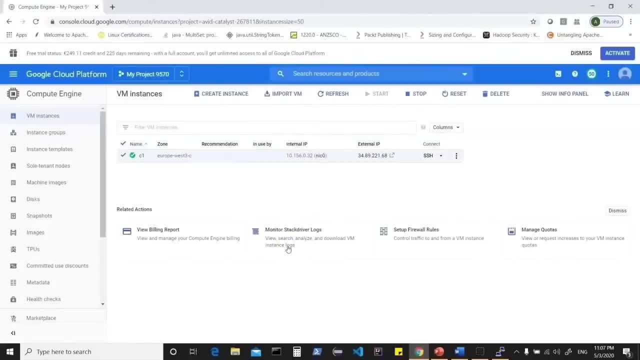 to large memory optimized instances with up to 11.5 terabytes of RAM. You can have fast compute instances, optimized up to 60 virtual CPU cores. You also have custom machine types so you can create a VM that best fits your workload, And by tailoring a custom machine type to your specific need, you can realize significant 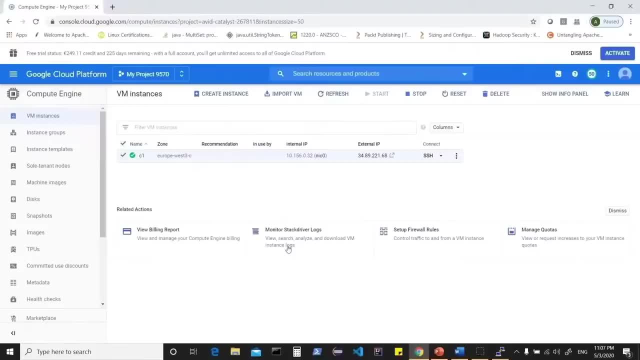 savings. There are preemptible VMs, Which we saw. there is also a facility which allows you to take the benefit of live migration For VMs. you have durable, high performance block storage for virtual machine instances in the form of persistent disks where data is stored redundantly for integrity, flexibility. 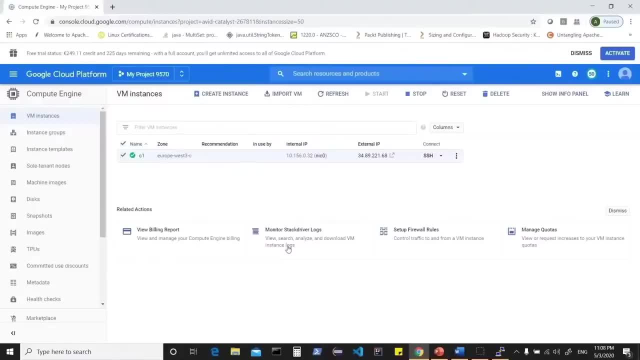 and to resize storage without interruption, And you could be choosing HDDs or SDDs for your instances. Now you also have options such as GPU. Exactly, You can also add GPUs. So, for example, if I just click on create instance and I can look into that. 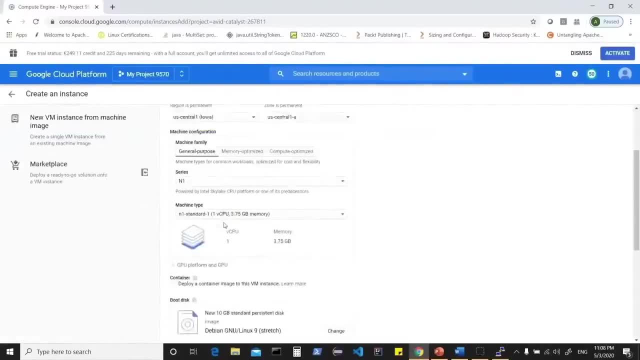 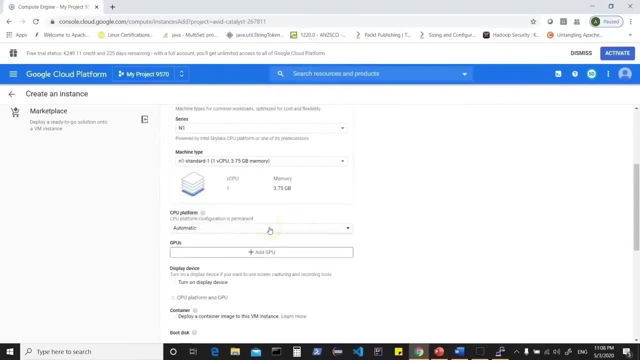 So here, let the instance name be instance one. And what I would be interested in looking at, this one which says CPU platform and GPU, So CPU platform configuration is permanent. You can also do add GPU, So GPUs can be added to accelerate computationally intensive workloads like machine learning. 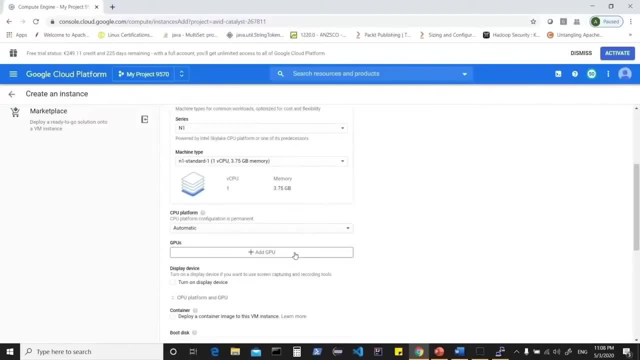 simulation, medical analysis and virtual workstation applications. So you can add and remove GPUs to a VM when your workload changes and pay for GPU only while using. So these are some of the features which basically Compute Engine offers, And we already know that Google builds in second level increments. 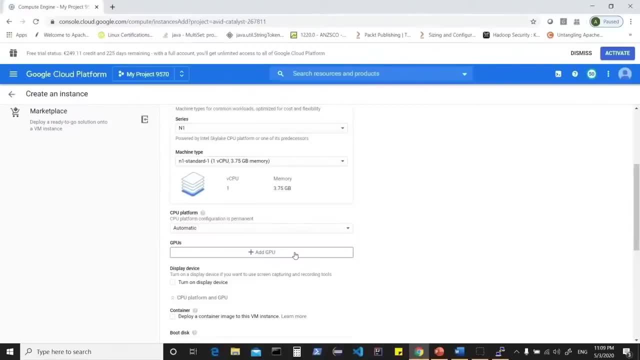 So we only pay for the compute time. Now there are different savings which are possible. So you have commitment savings, which basically means you can save up to fifty seven percent. with up Different cost, per instance type lock in, You have container support. 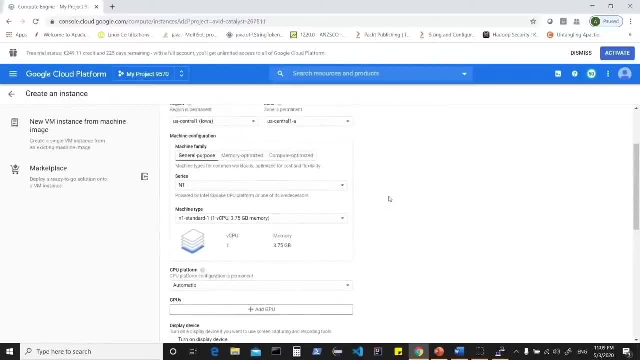 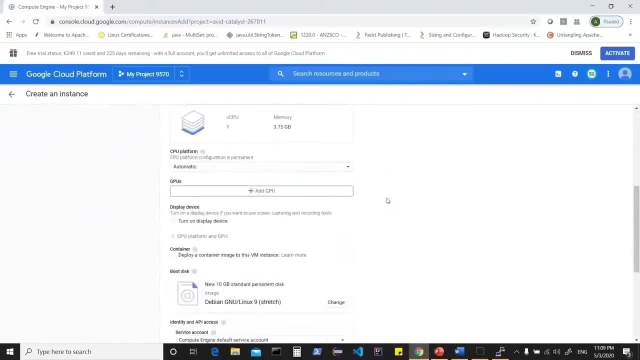 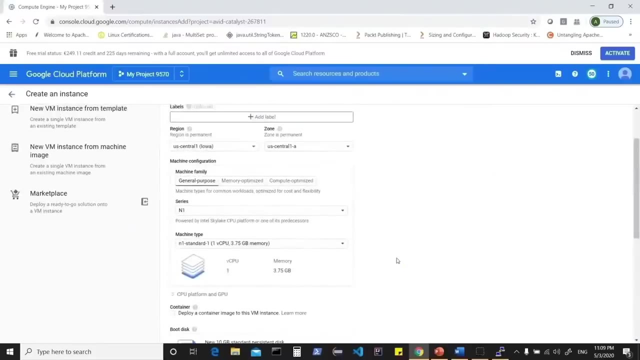 So you can basically run, manage and orchestrate Docker containers or Compute Engine instances. So here, when we are setting up our instances, there is an option which basically allows you to use or deploy Docker images. Now that can be done, You can also benefit from sustained use savings. 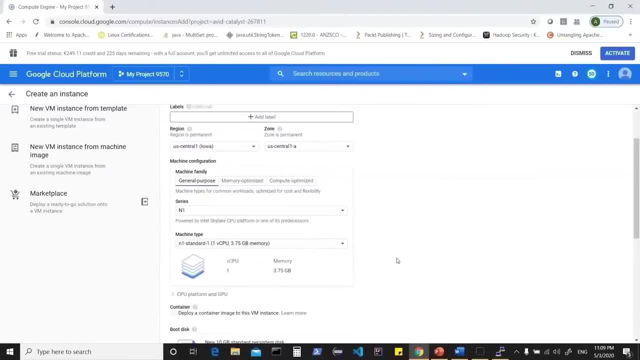 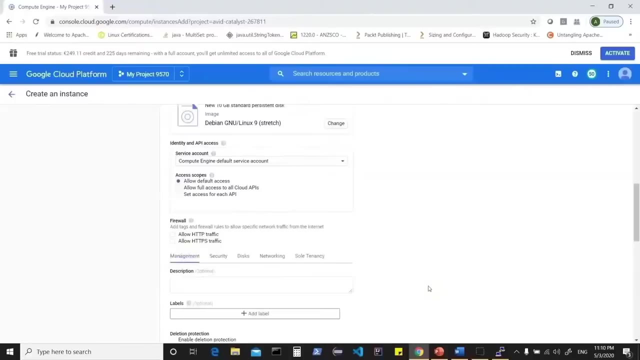 That is, sustained use discounts, which are automatic discounts for running Compute Engine resources for significant portion of the billing month. You can create a reservation for VM instance in a specific zone, which is basically seen under your management section here, And you can ensure your project has resources for future increases in demand. 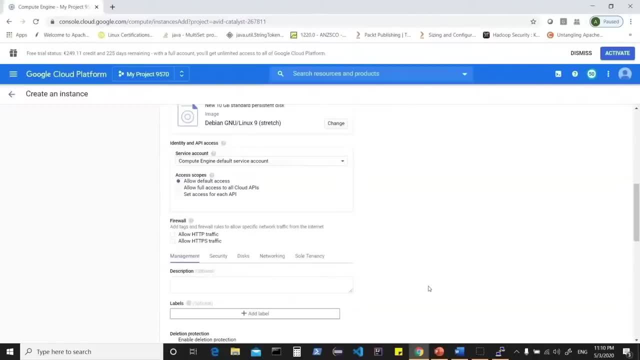 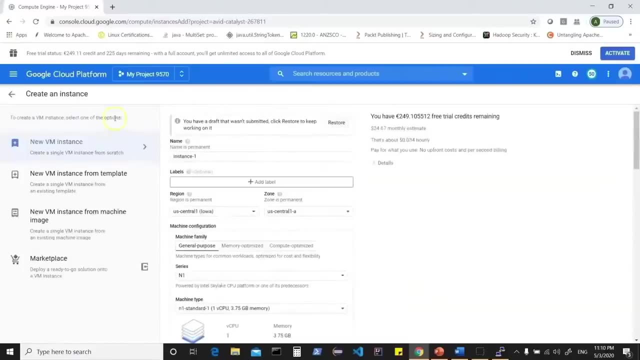 And, if no longer needed, delete the reservation. So these are some of the features of Compute Engine. What we have done is we have created Compute Engine using the console. Now you can go back. You can also do that using cloud shell, and you can click on this one, which activates. 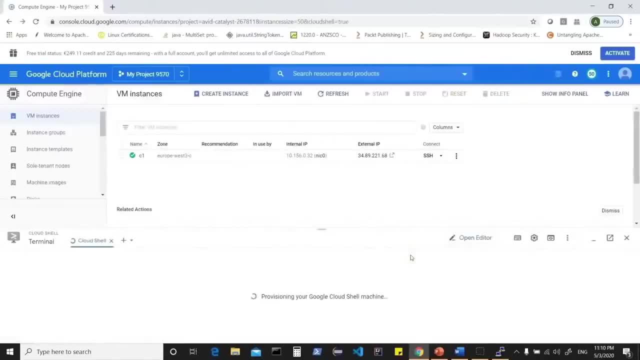 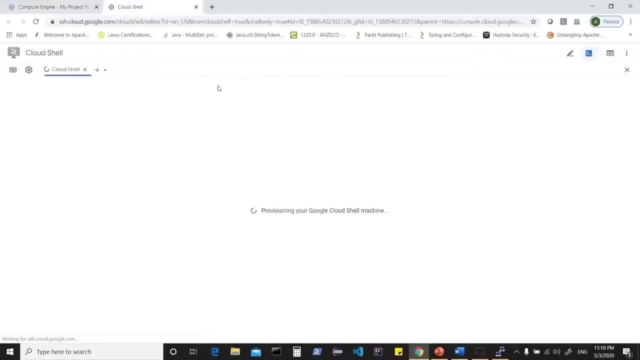 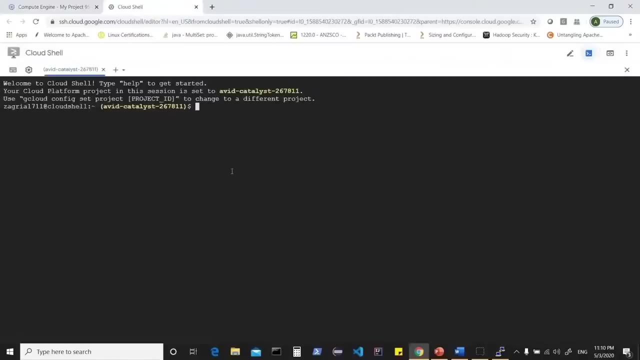 cloud shell. You could also have the cloud SDK support on set up on your machine which can be used. Now I can just open this in a new window and from here I can start giving commands If I would be interested in setting up an instance from my command line. 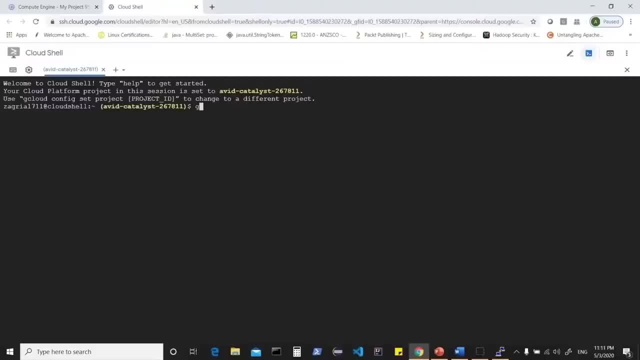 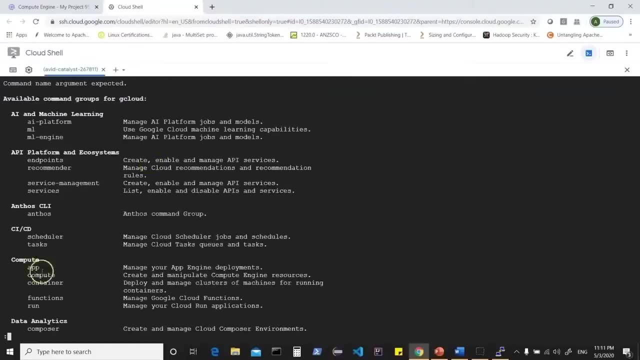 So here you have different options. Now, to begin with you can just do a G cloud Okay, You can just hit enter and that will show you different options which are available, which can be used. So you have G cloud compute here which shows an option to create and manipulate Compute. 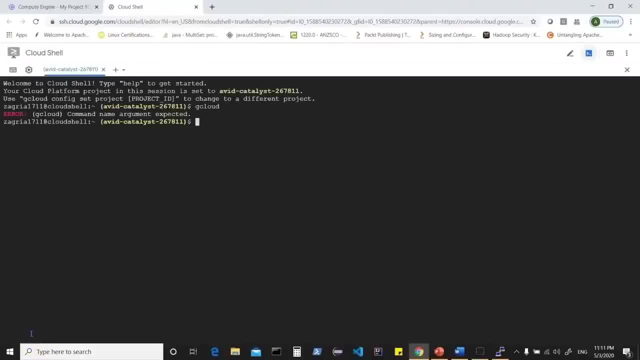 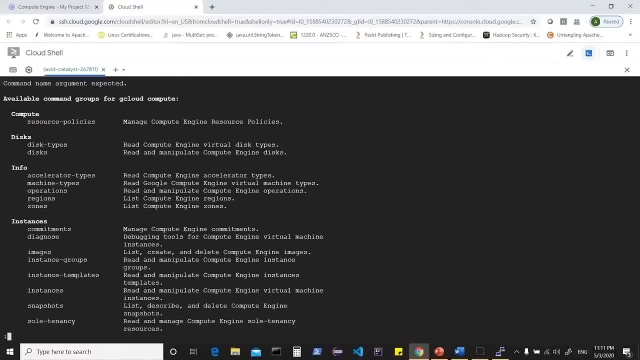 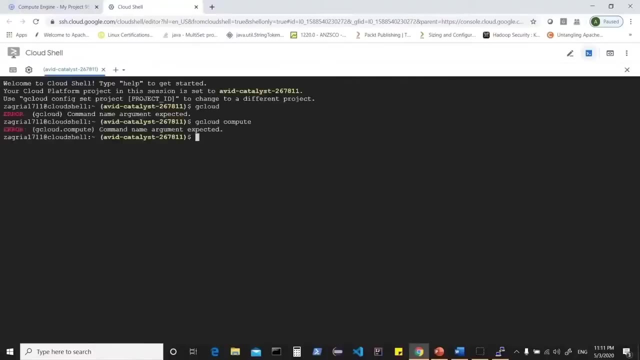 Engine resources. Now I can just do a queue to quit, I can do G cloud compute and that basically will again show me different options which are available if you would be interested in setting up instances from the command line. So here I can say G cloud compute. 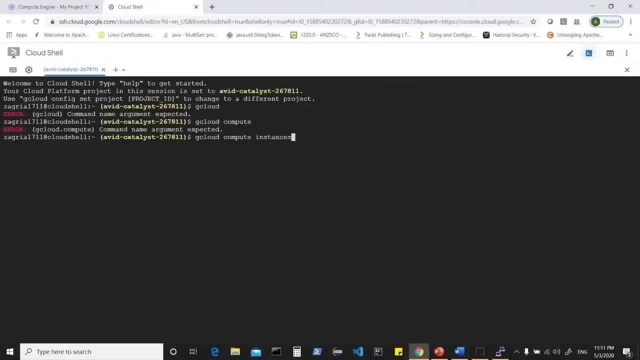 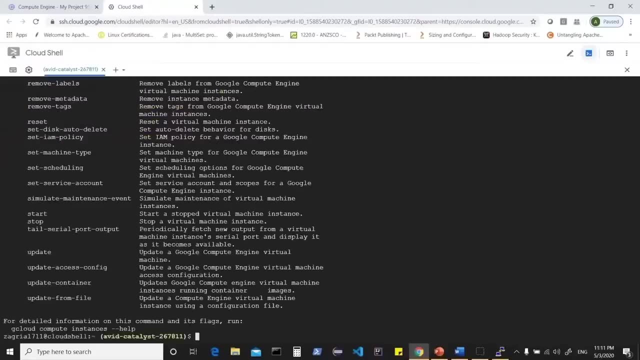 And then go for instances and if you do not know the commands you can just hit enter. That will show you all the different options which we have. So here we have different options such as list or create or start or update, For example. I can just do a list here to see what instances I have and the instance. 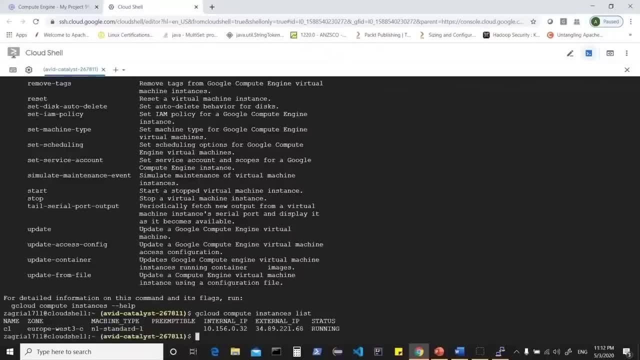 which we just created shows up here. It says that status is running. I can just stop this instance. I can delete this instance. I can even create an instance by using a create command here And you can just do a create help which will show you what are the different options. you. 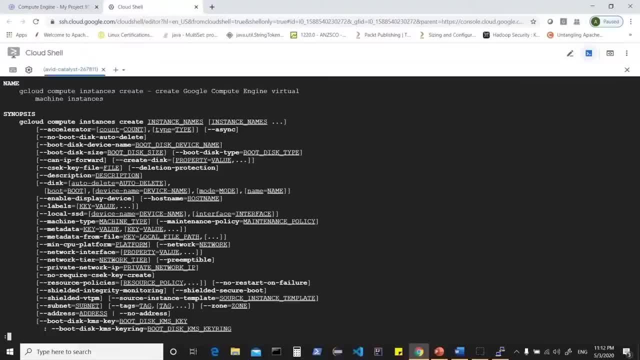 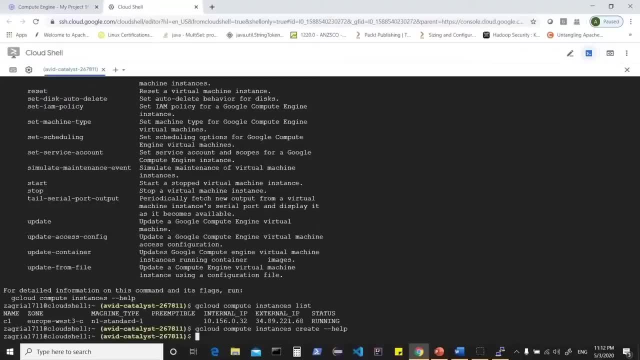 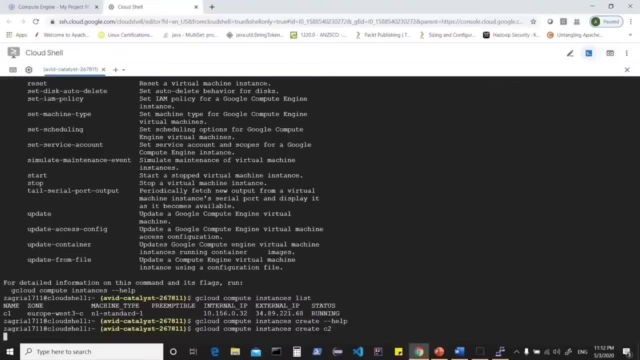 can give. So it says: instance name is what you need. You can choose an accelerator, You can choose the boot disk and various other options. So I can just say create and then I can give a name, for example C2.. And once I click on this one it says: did you mean? 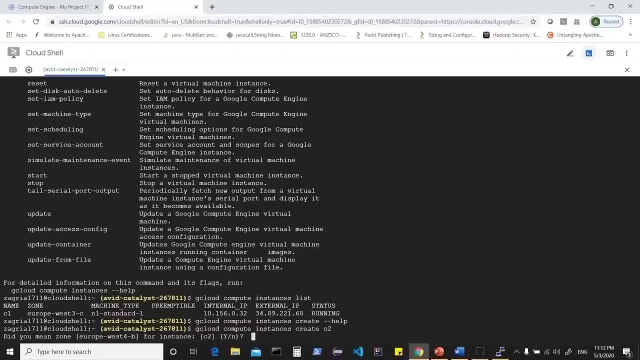 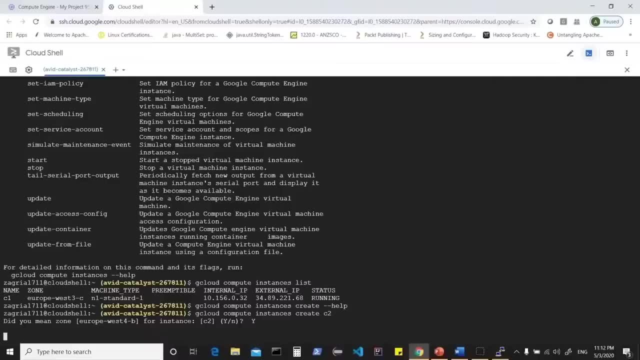 Did you name it So you can create a name? and then, once I click on the settings, it gives us the settings that we need and then I will give a name for the instance And I can also set the file name for this instance to create that. 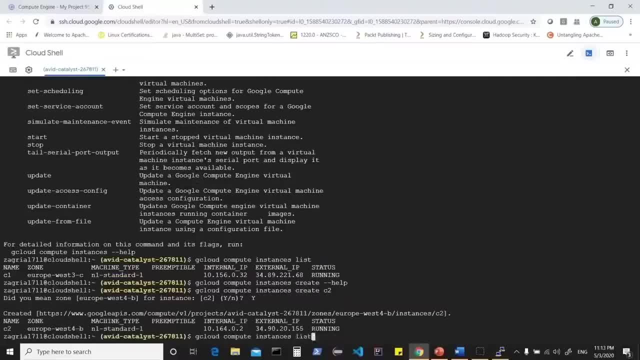 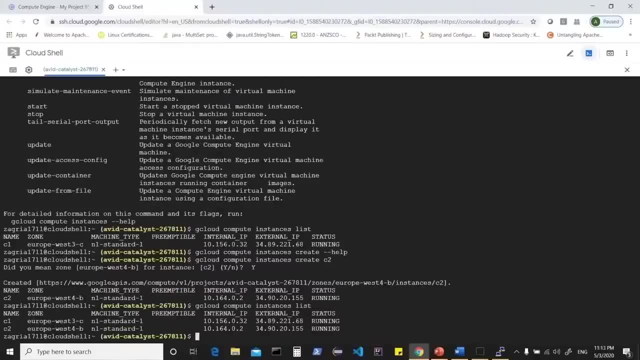 So, just like this, I can just go ahead and add a name to that, and then I can create an example for that And that's it. So, for instance, I want to create a new field. I can name it as part of my profile. 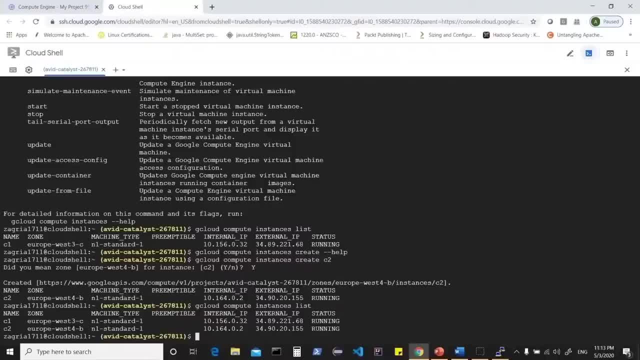 So now I have created an example. So it is asking me for the region and the zone- and I can say yes, do a describe- to look at the different options here. so gcloud basically allows you different commands which you can use to work with your instance: to create instances, to change the. 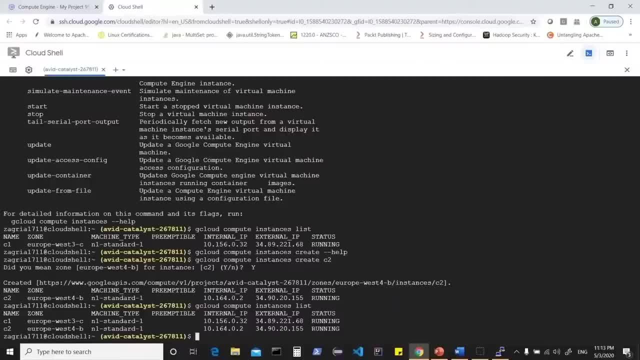 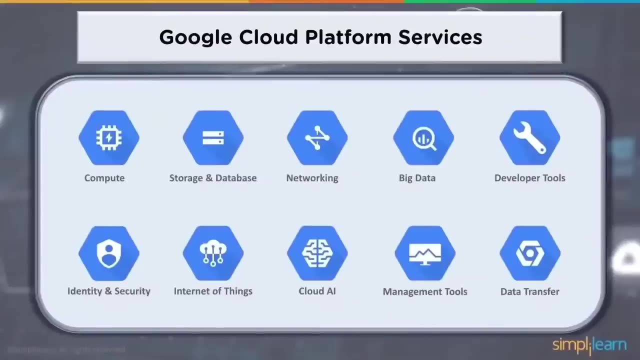 metadata, if you would want to change the region, if you would want to add a startup script, all those options are possible from the command line, which we can learn in detail in later sessions. so this is your compute engine as a service, now that we have learned about the compute domain. 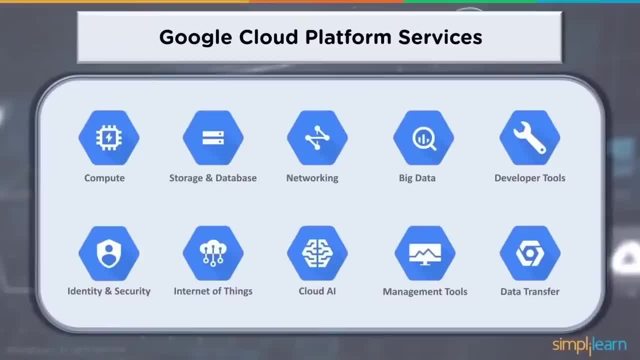 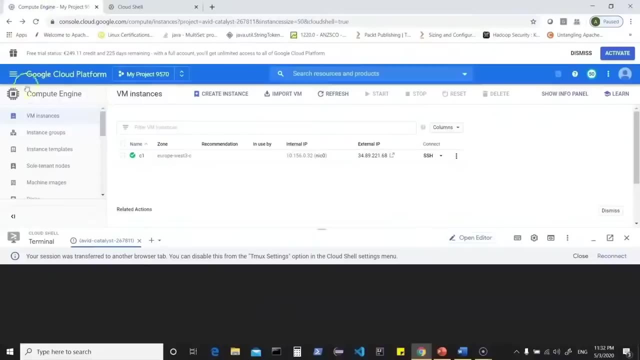 and g compute services, which is offered by gcp. let's also learn about storage and databases. that's again within the storage domain and the services which are offered by google cloud platform. now you can go back to console and here you can click on this one and here you can just. 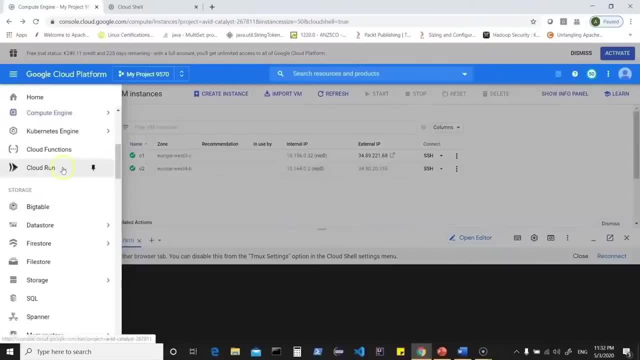 scroll down to see what are the different options in storage. so you have options such as big table, you have data store, fire store, file store, you have sql based services, you have storage which is object storage and then you have other options which are available. so google cloud platform offers different storage. 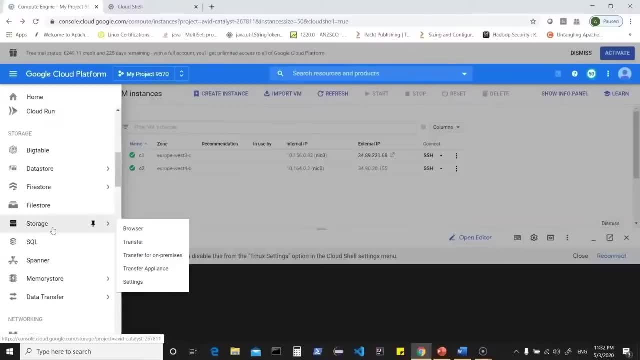 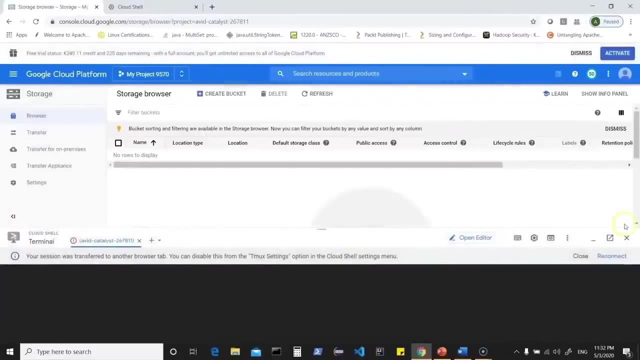 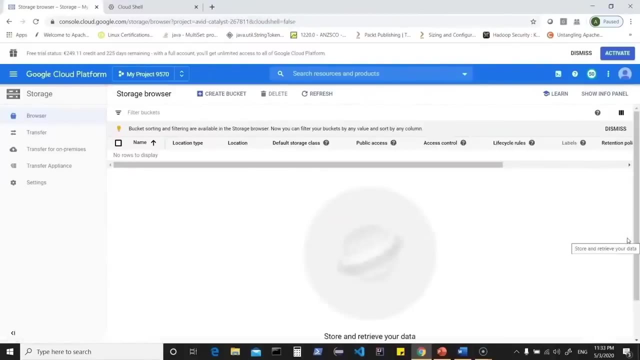 based services, out of which storage, which is your object storage, is quite popular. one click on storage and that basically shows you an option which talks about storage browser. so this is your google clouds object storage. so when we talk about object storage, it is basically a storage where you could store any kind of data. and when we talk about object storage, 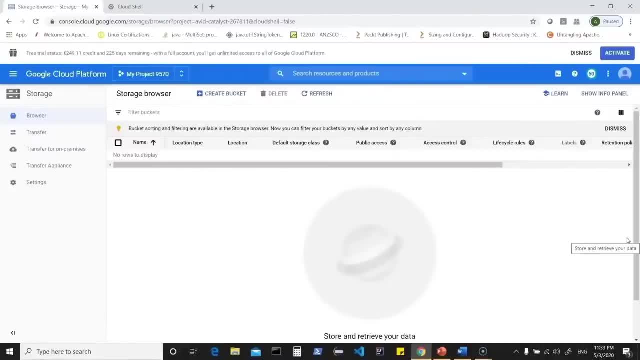 it is a bunch of bytes which we address, wherein every object will have a unique key. these unique keys are in the form of url which allows you to access the object. so cloud storage is comprised of what we call as targets, which are used to store and hold your storage objects. these storage objects are immutable. 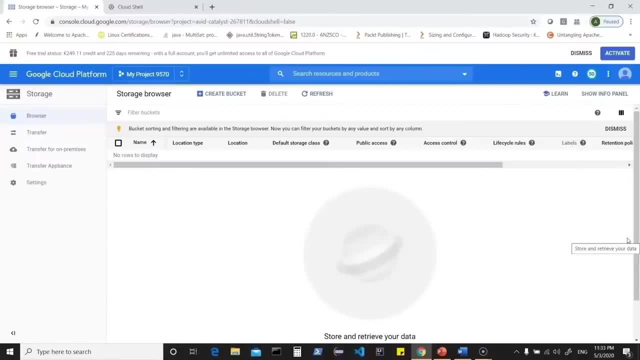 and every change creates a new version. now you can also have control access via iam, that is, identity access management, or via access control list. so there is also an option called object versioning, which basically says, if it is on, every time you try to store the same object, a new version of the object would be. 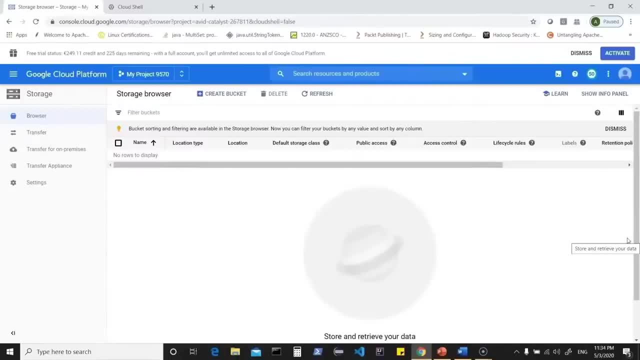 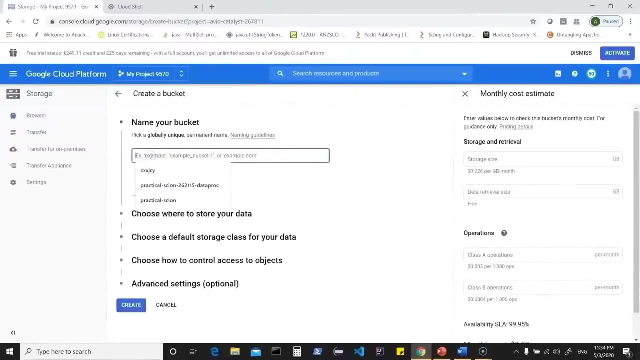 created. otherwise newer option will override old one, as we cannot archive the old version. so let's see how we work with this object storage. so here you can click on create bucket. now, once you click on create bucket, it needs a name. so let's say test bucket and here i can just give, say, number one. 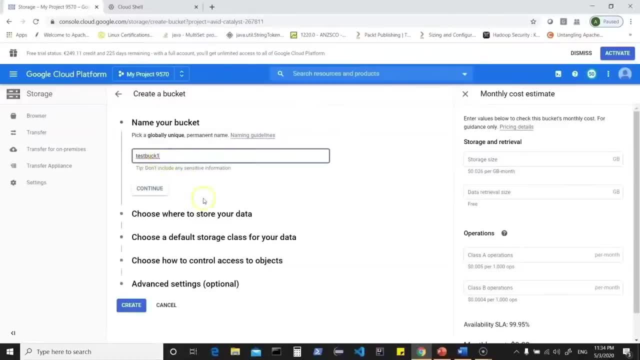 so that says this is the name of my bucket. now i can directly click on continue or it would be good to look at different options which are available here. so when you click on, choose where to store your data. so it already gives me an option. it says the bucket name is already taken. so let me. 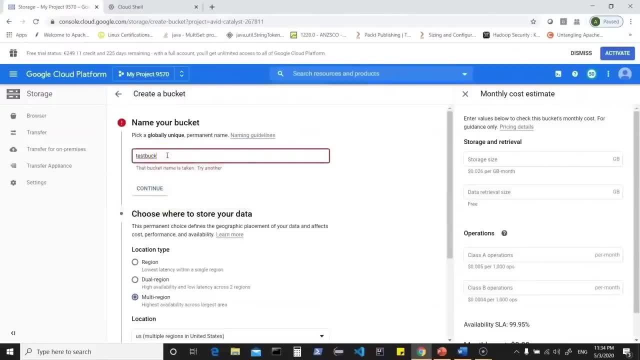 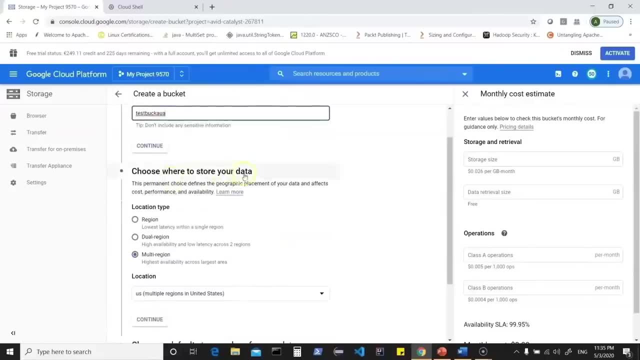 give it a unique name. so let's say test buck and let's call it aua, so that should be unique. now here it says: choose where to store your data. so this one gives you location type, so you can have region specific bucket which give you lowest latency, that is, fastest response time, within a single region. however, it 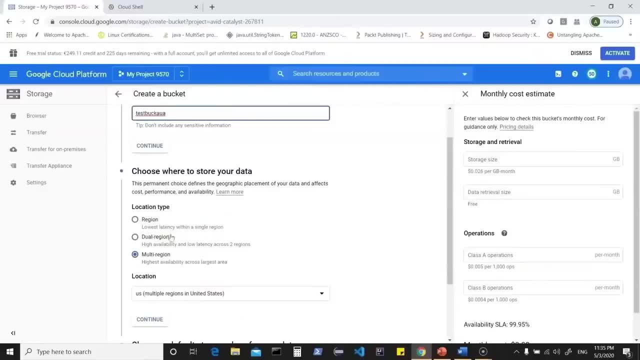 does not make your storage highly available. you can make a dual region, which is basically allowing your bucket or storage to be accessible across regions. you can also make it multi-region, which is highest availability offered. as of now, we can choose region specific. and now it asks you: 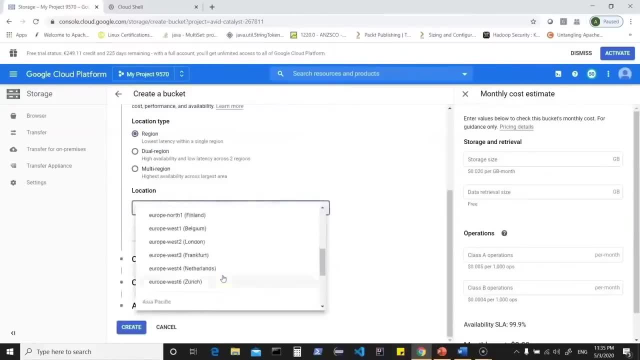 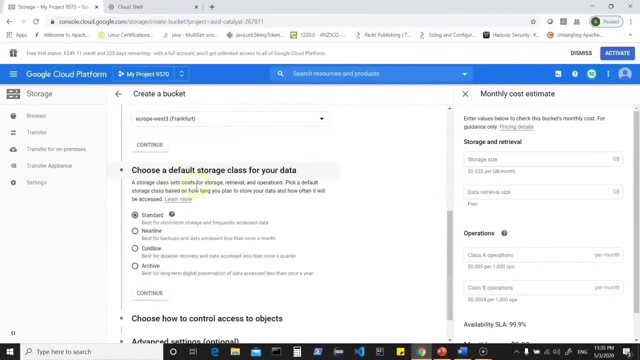 to choose a location. now, as always, i will choose frankfurt. now i can click on continue and rest all the rest. let all the storage options be default, or you can click on a default storage class. now that tells you based on your storage class. there are variant costs when it comes to storing, retrieving or doing any kind of operations. 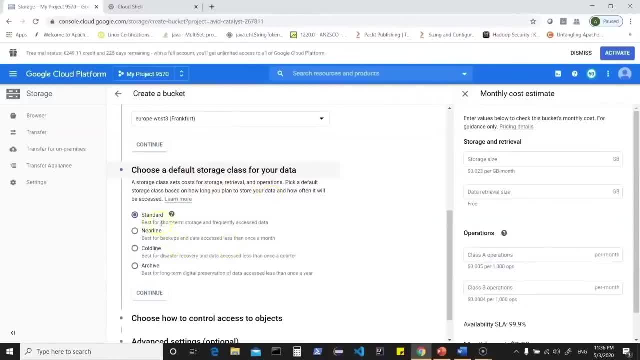 so you have a standard option which says best for short-term storage and frequently access data. you can also go for cold storage, such as near line, which is best for backups and data access less than once a month. you can go for freezing storage, such as cold line, best for. 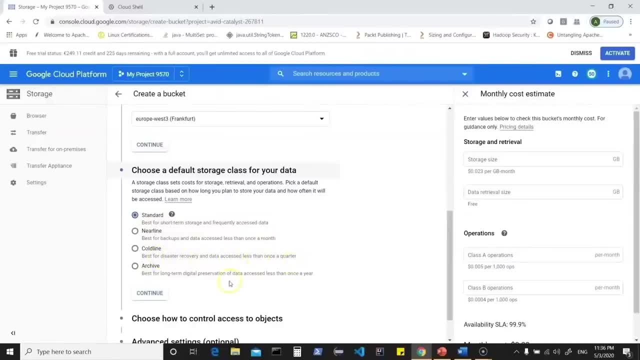 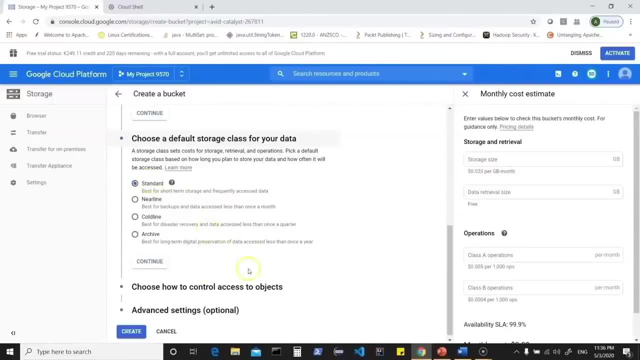 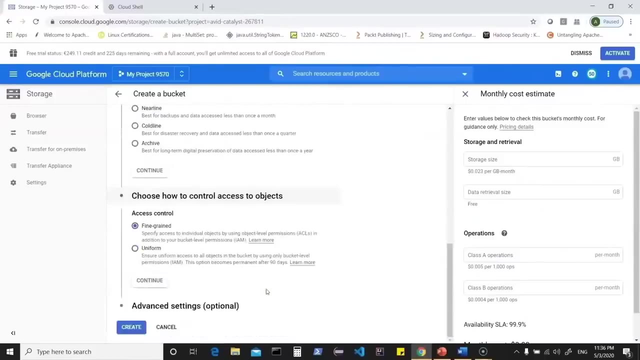 disaster recovery and data accessed less than once a quarter, or you can go for archiving where the data is accessed less than once a year. let's go for standard as of now, and now you can choose how to control access to objects, so you have fine grained or uniform. let it be fine grained wherein. 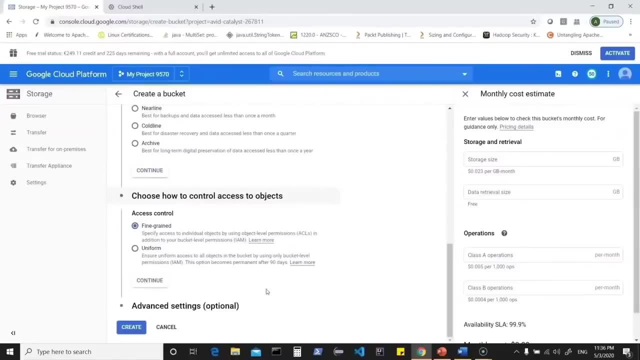 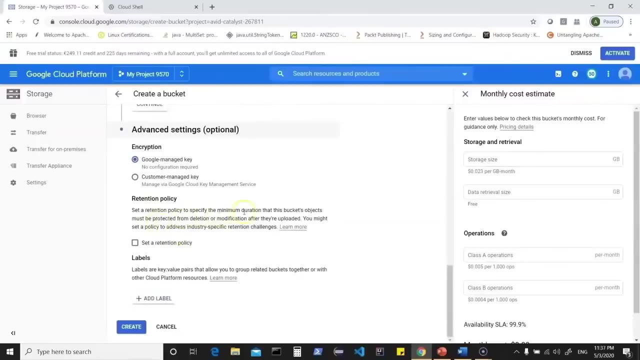 you can give additional permissions at bucket level using iam or object level permissions, using access control list. in advanced settings you can choose the encryption and you can also choose a retention policy. so a retention policy to specify the minimum duration that this bucket's objects must be protected from deletion or modification after they are uploaded. 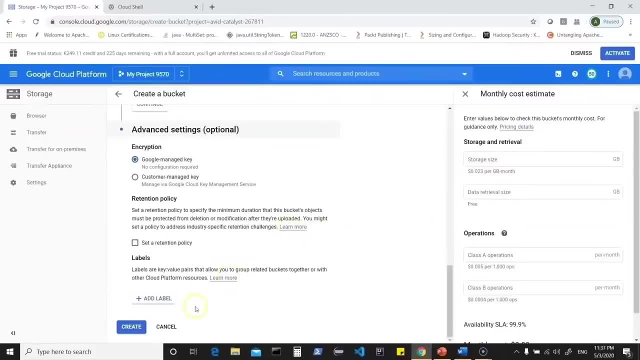 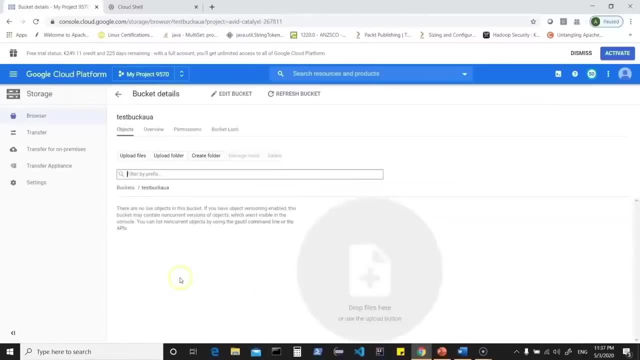 you can always learn about this more by clicking here. now, once i've chosen all the relevant options, i can click on create, and that basically will create a bucket by the name i have given. i can click on overview to basically see brief details about my bucket, such as region, what is the default storage class, and it also shows you the link url which can: 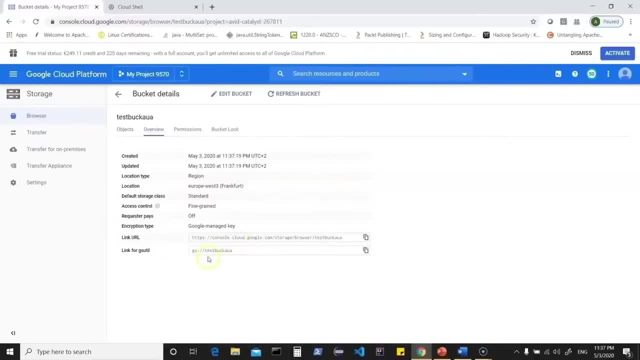 be used to access your bucket. it also gives you the link for gsutil. now, gsutil is a command which can be used in your cloud shell to basically work with your buckets. you can click on permissions to basically see what kind of permissions are already in place and you can then make changes. you can basically add. 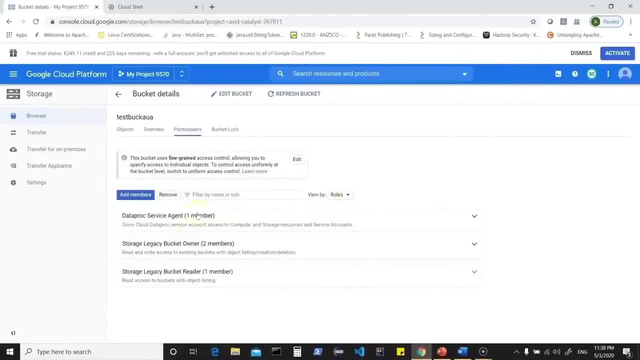 members you can view by different roles. so for example, here, by default it shows other services, such as data proc or your bucket owner or bucket reader related permissions which have been already granted. now, once i have looked at my bucket, i can start using it. i can drag and drop and. 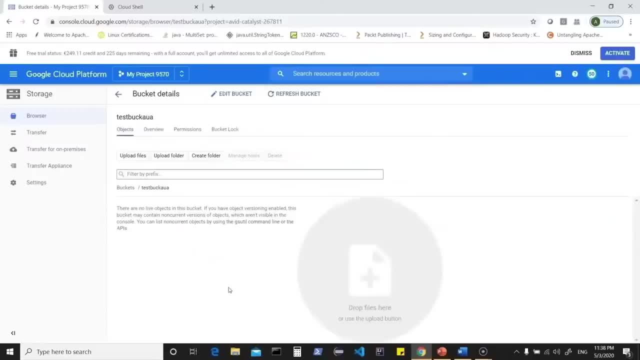 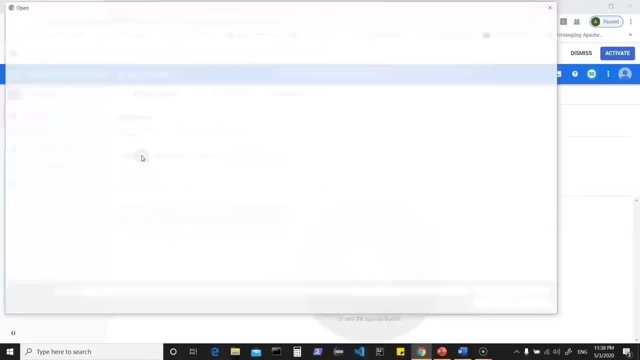 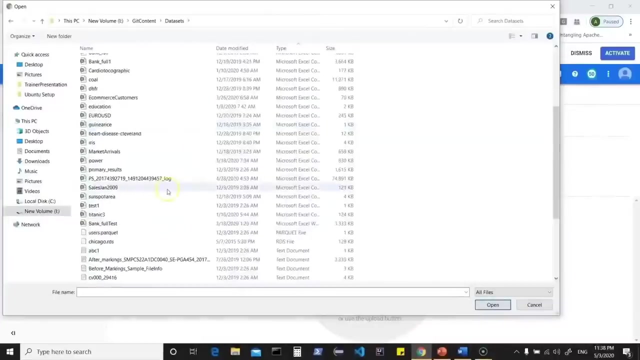 push in files here. so as of now, there are no live objects in my object storage. that is in my bucket. what i can do is i can click on upload files and then i can choose a location from my machine. for example, i'll go into data sets. 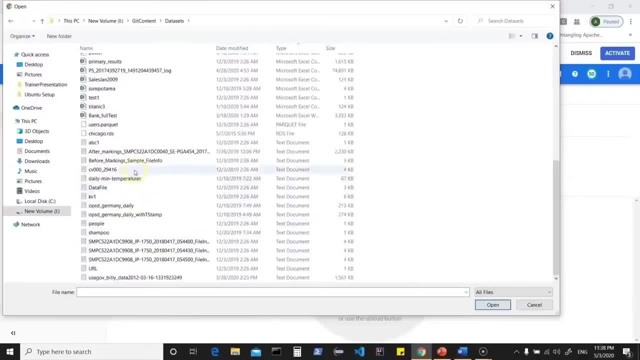 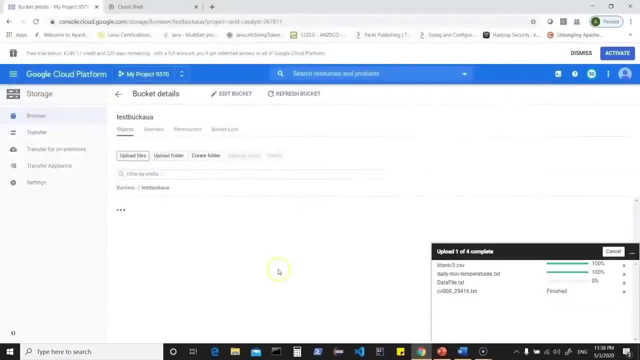 and what i can do is i can choose some of the files here in any format- let's choose csv or text and just to open. so this one will basically upload my data sets here. now, once i've uploaded the files, i can basically close this one. i can look into options here, which. 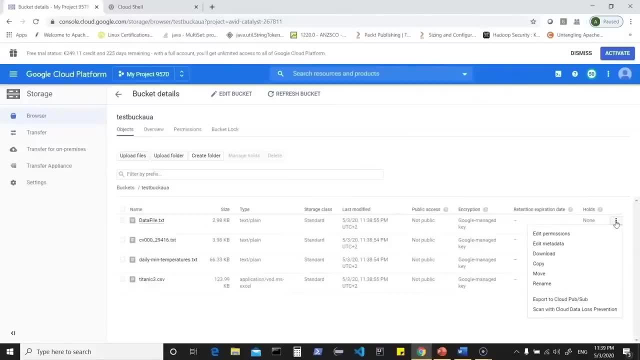 says edit permissions and edit metadata. if you would want to download it, if you would want to copy, move or rename it, if you would want to export to a different service called cloud pub sub, which is publish subscribing messaging system. you can scan the data now. you can click on a particular. 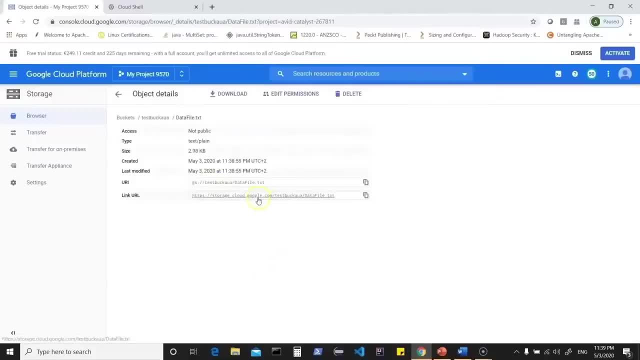 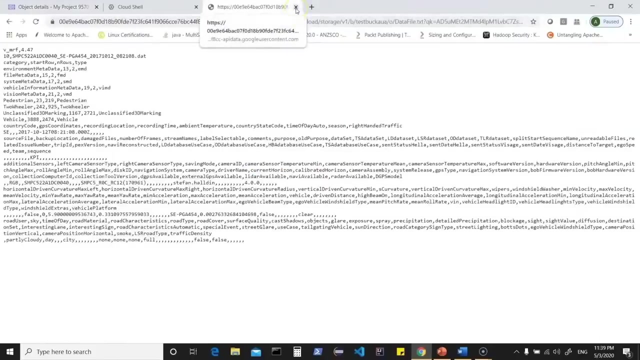 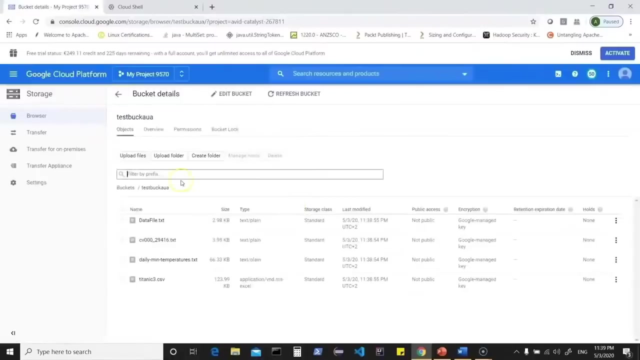 file and that basically shows you the url, which basically shows you the data set. and then you can see the data set which basically allows you to access this file. you can try copying this. you can click on download and download this file. you can even try accessing this from public and that basically shows you the content of this file based on the permissions. so this is basically your object storage, which is one of the service which is offered. what you can also do is you can create folders and within folders, you can then upload your data. so this is your google cloud storage. 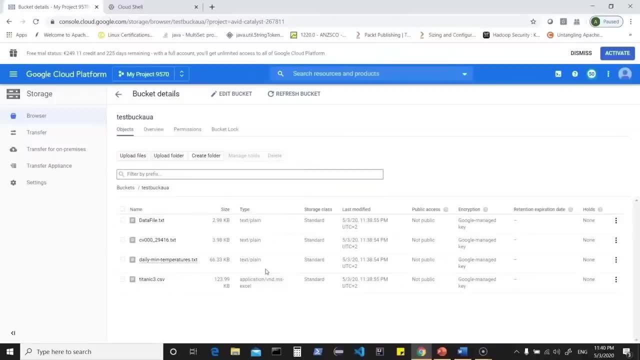 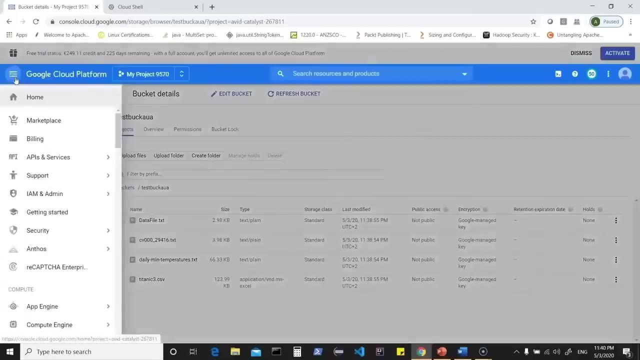 storage option, which is for your object storage, that is, you can add different items, you can give different permissions and you can use this google cloud platforms storage service offering. now you also have other options, such as big table, and we can go into that by clicking here and click on big. 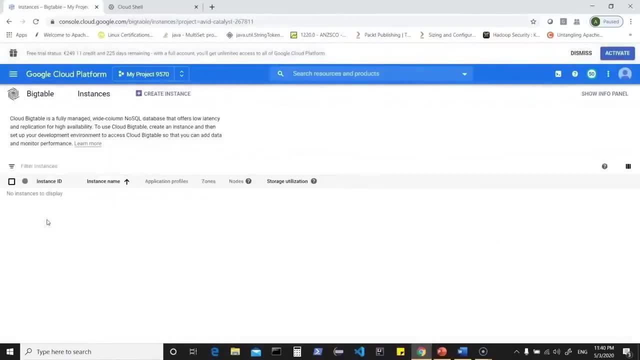 table. so big table is one of the service which kick-started no sql databases. today in market we see the big table and we can go into that by clicking here and click on big table. so big table see different no sql databases such as cassandra, hbase, mongodb, couchdb, neo4j and many others. so you 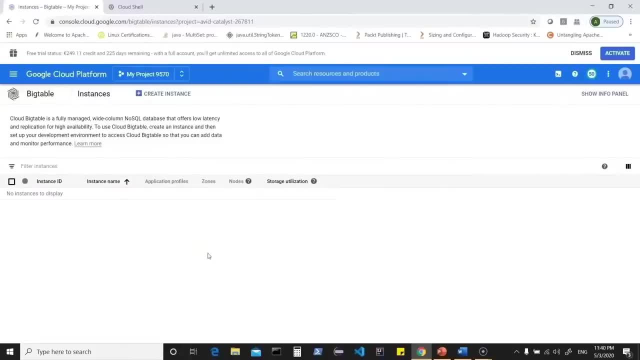 can basically use big table, which was the pioneer when it comes to your no sql databases or not only sql databases. so the problem initially faced by google was that the web indexes behind search engine were taking too long to build, so company wanted to build database that would not be able to build, a database that would not be able to build. a database that. 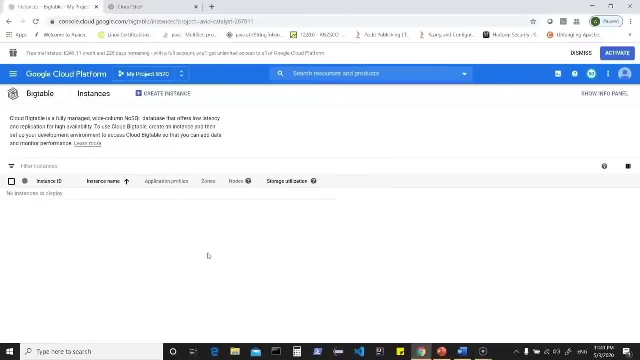 would provide real-time access to petabytes of data, and that's where big table began. so big table powers different other google services, such as gmail, google maps and other services, and in 2015, it was launched as a service for customers. so, when it comes to scalability with use of big table, 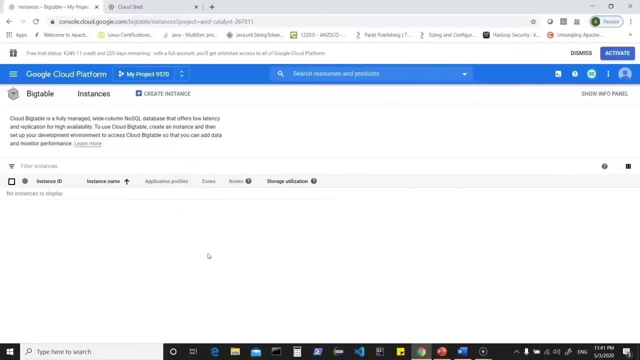 you can increase your machine count without any downtime and you can handle admin tasks like upgrades, restarts and so on. so when it comes to scalability with use of big table, you can increase your machine count without any downtime and you can handle admin tasks like upgrades, restarts and so on. 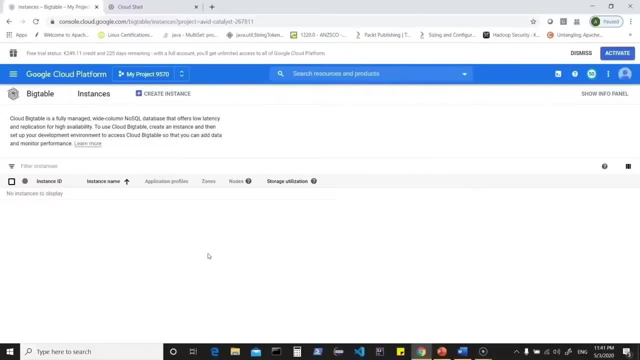 which are basically taken care by the cloud provider. data present in cloud big table is encrypted and you can use im roles to specify access. so data written to or from big table is through data service layers such as managed virtual machines, hbase rest servers, java services, hbase client and so on. here, if i would want to use big table, i can click on create instance. 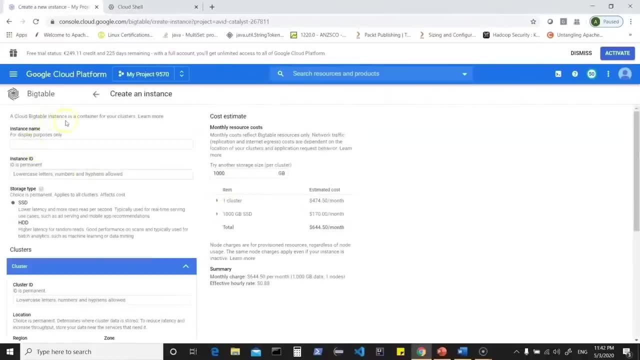 and that, basically, will take me to the big table. and it will take me to the big table and i can click on create instance and that, basically, will take me to the big table and i can click on create instance tells me: cloud big table. instance is a container for your clusters. now, here you can give a instance. 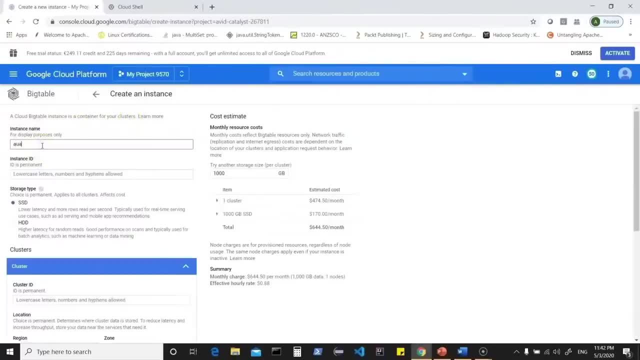 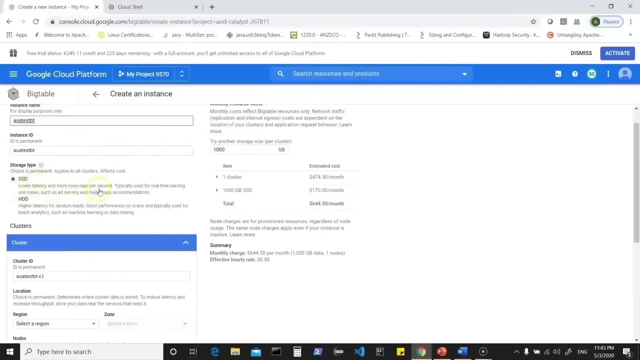 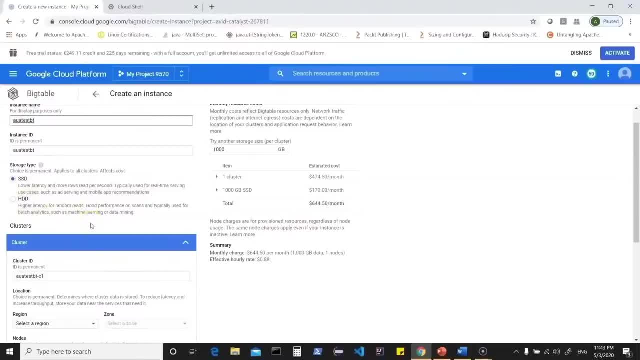 or you can go for lower latency- more rows read per second, typically used for real-time serving use cases. or you can go for sdds, which have higher latency for random reads, good performance on scans and good performance on scans. and good performance on scans and typically used for batch analytics. so 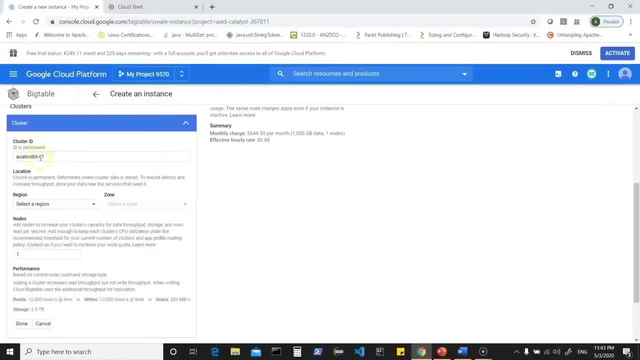 typically used for batch analytics. so, typically used for batch analytics. so let's go for ssds as of now. here you, let's go for ssds as of now. here you, let's go for ssds as of now. here you have cluster id, which is auto populated. 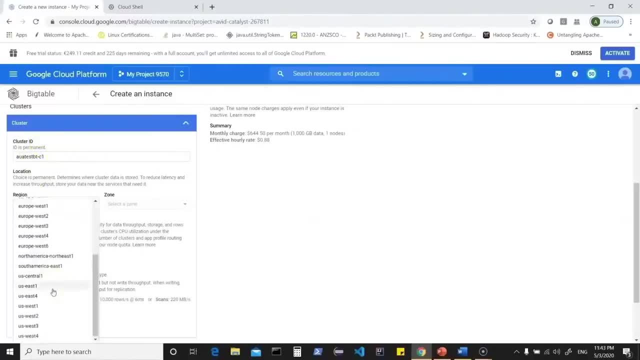 have cluster id which is auto populated. have cluster id, which is auto populated. you can choose a region, so let's go for. you can choose a region, so let's go for. you can choose a region. so let's go for our favorite one here where i can say: 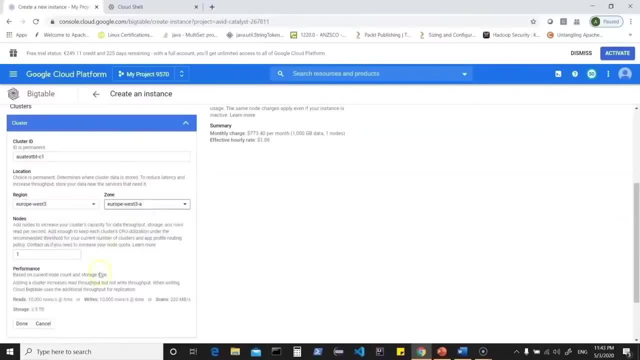 our favorite one here where i can say our favorite one here where i can say: europe west 3, i can choose a zone here: europe west 3. i can choose a zone here: europe west 3. i can choose a zone here, and i can then choose how many nodes. 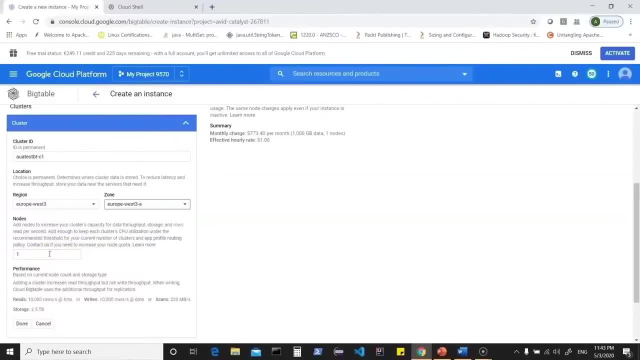 and i can then choose how many nodes. and i can then choose how many nodes would i want to use for my big table. so would i want to use for my big table. so would i want to use for my big table. so, when you talk about big table service, 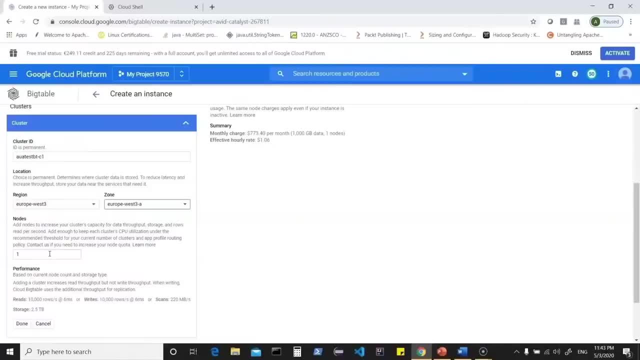 when you talk about big table service. when you talk about big table service, it will have a cluster underlying which it will have a cluster underlying which it will have a cluster underlying which will have various nodes which will will have various nodes which will will have various nodes which will contour your data throughput storage and 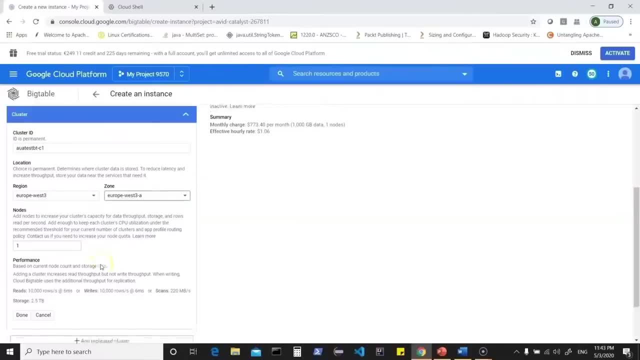 contour your data throughput storage. and contour your data throughput storage and rows read per second. so as of now, let it rows read per second. so as of now, let it rows read per second. so as of now, let it be just one node and that's enough for. 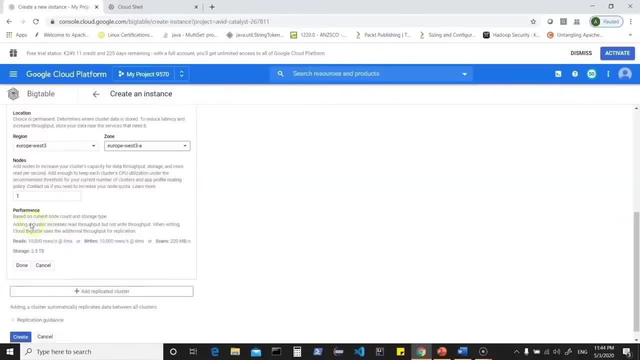 be just one node, and that's enough for be just one node, and that's enough for our demo. when we talk about performance, our demo, when we talk about performance, our demo, when we talk about performance, it basically tells you, based on the. it basically tells you based on the: 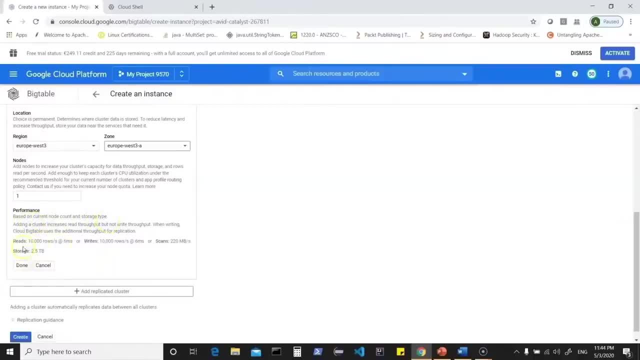 it basically tells you, based on the current node and storage type. it tells current node and storage type. it tells current node and storage type. it tells you how many reads can happen at you, how many reads can happen at you, how many reads can happen at milliseconds. so it says 10 000 rows per. 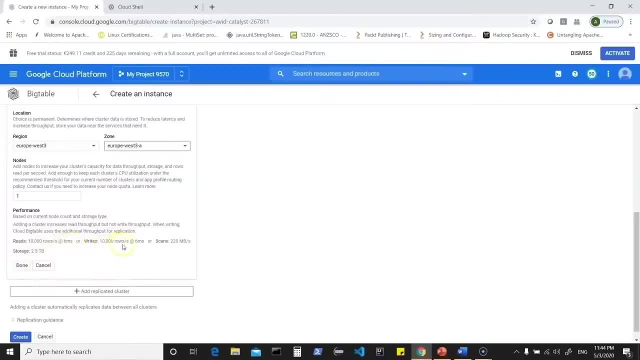 milliseconds. so it says 10 000 rows per milliseconds. so it says 10 000 rows per second at 6 millisecond. you have writes second: at 6 millisecond. you have writes second: at 6 millisecond. you have writes which are 10 000 rows per second, or you. 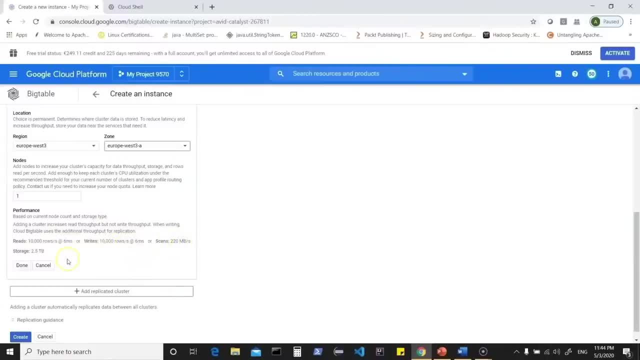 which are 10 000 rows per second, or you, which are 10 000 rows per second, or you have scans which are 220 megabytes per have, scans which are 220 megabytes per have, scans which are 220 megabytes per second storage which is taken care here. 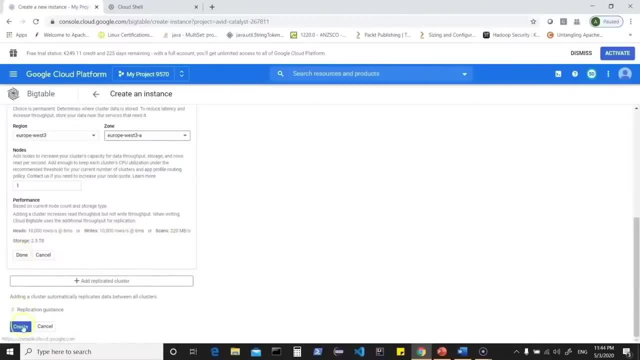 second storage which is taken care here, second storage which is taken care here- would be 2.5 terabytes and i can then would be 2.5 terabytes and i can then would be 2.5 terabytes and i can then basically click on create. now there is. 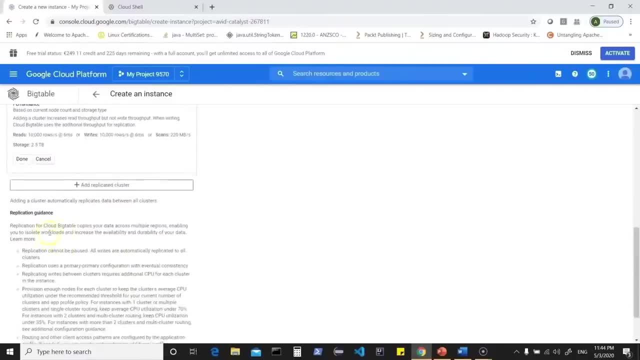 basically click on create. now. there is basically click on create. now there is also some option called replication, also some option called replication, also some option called replication. guidance, which basically says guidance, which basically says guidance, which basically says: replication for cloud table big table. replication for cloud table, big table. 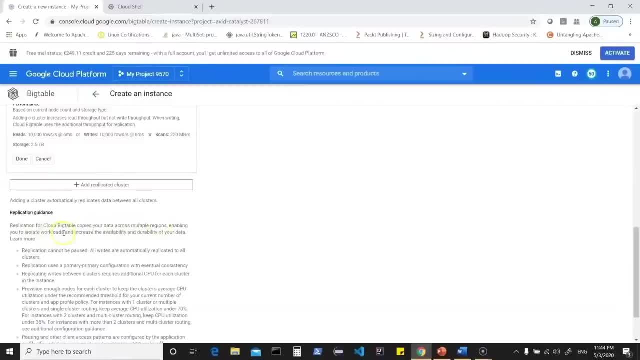 replication for cloud table: big table. copies your data across multiple regions. copies your data across multiple regions. copies your data across multiple regions, enabling you to isolate workload. and enabling you to isolate workload. and enabling you to isolate workload and increase the availability and durability. increase the availability and durability. 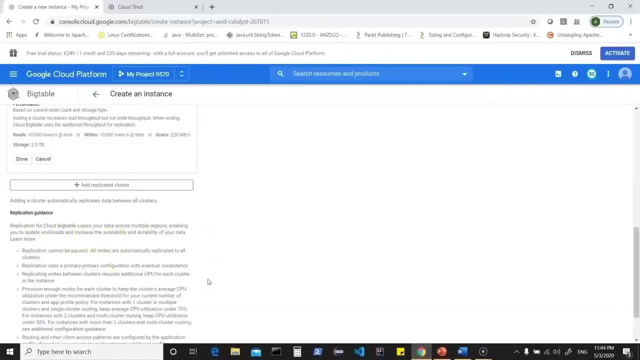 increase the availability and durability of your data, depending on your use case of your data. depending on your use case of your data. depending on your use case, you can have big table which can be used. you can have big table which can be used. you can have big table which can be used to have your data across regions. now you 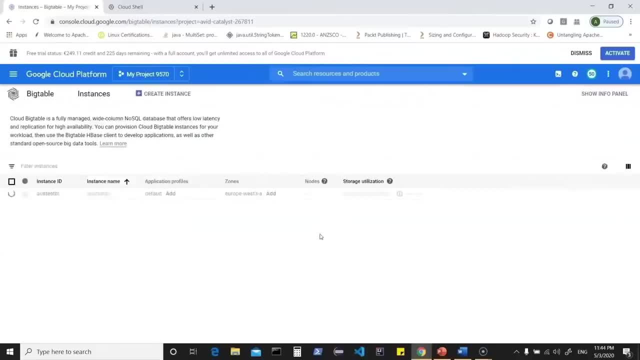 to have your data across regions. now you to have your data across regions. now you can click on create with all. your can click on create with all. your can click on create with all your specifications chosen and that's going to specifications chosen and that's going to. 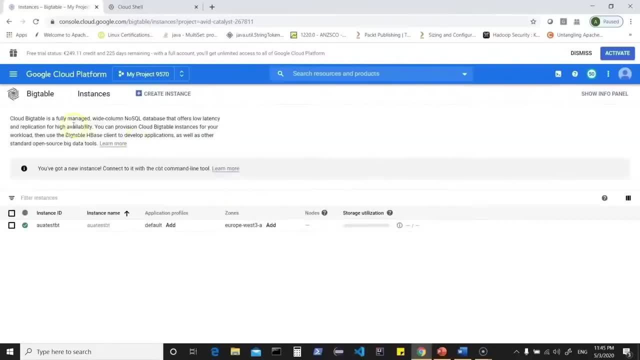 specifications chosen and that's going to set up a cluster. or you can say a fully set up a cluster, or you can say a fully set up a cluster, or you can say a fully managed no sql database, which will give managed no sql database, which will give. 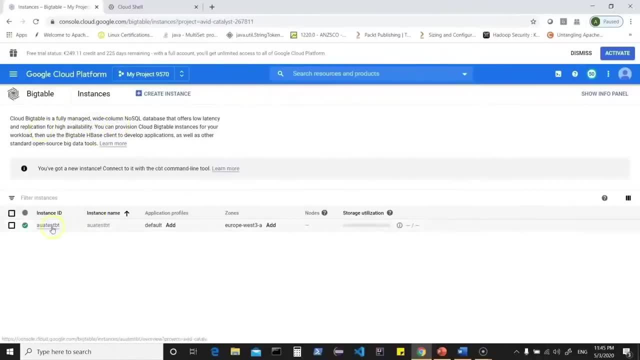 managed no sql database which will give you low latency and replication for high you low latency and replication for high you low latency and replication for high availability. now, once we have a new availability, now, once we have a new availability, now, once we have a new instance, you can connect to it with the. 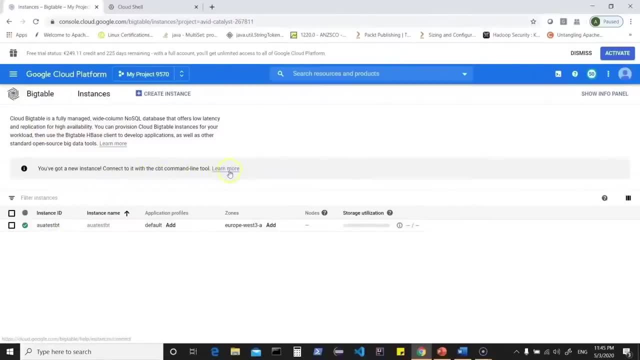 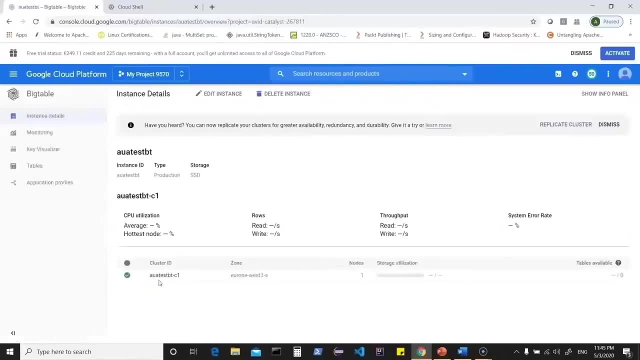 instance. you can connect to it with the instance, you can connect to it with the to see the details again. if you would to see the details again, if you would to see the details again, if you would want to look into your big table setup, want to look into your big table setup. 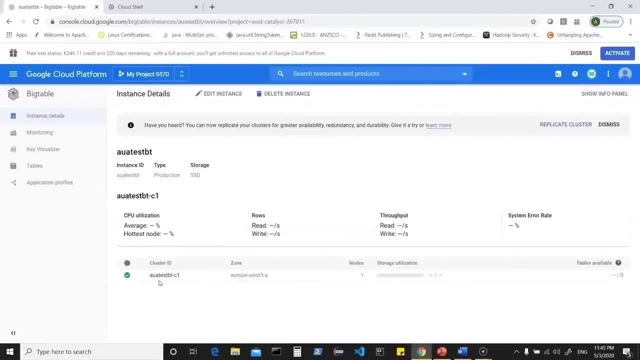 want to look into your big table setup. so it tells me here that we have one. so it tells me here that we have one. so it tells me here that we have one instance. what is the CPU utilization instance? what is the CPU utilization instance? what is the CPU utilization time? how many rows were read or written? 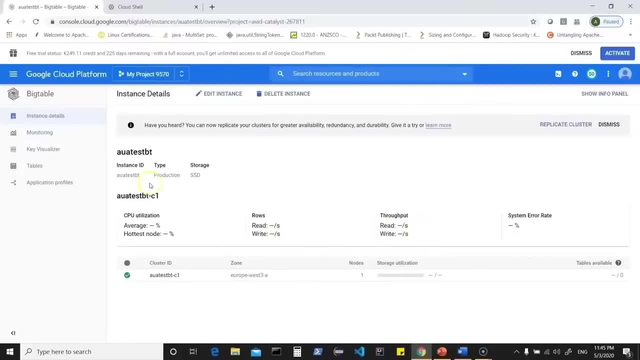 time: how many rows were read or written. time: how many rows were read or written. what is the throughput and this is auto. what is the throughput and this is auto. what is the throughput and this is auto. populated based on your usage. you can. populated based on your usage. you can. 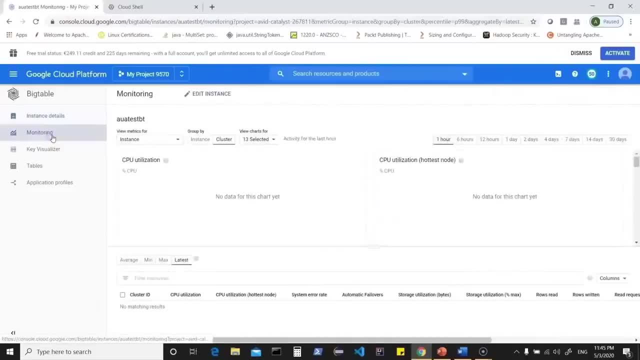 populated based on your usage. you can click on monitoring and that basically click on monitoring and that basically click on monitoring and that, basically, will give you different widgets, which will give you different widgets, which will give you different widgets which will display information for your CPU, will display information for your CPU. 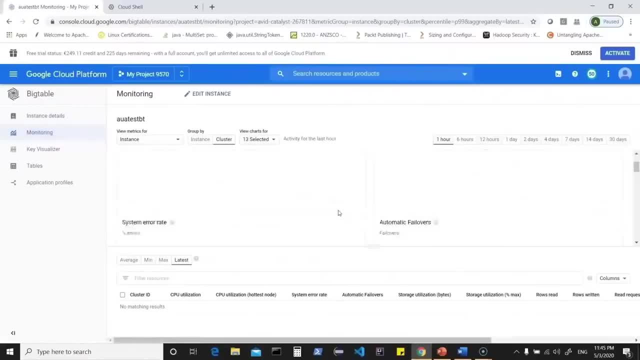 will display information for your CPU utilization. what is your hottest node utilization? what is your hottest node utilization? what is your hottest node, depending on how many nodes you have? depending on how many nodes you have, depending on how many nodes you have. system errors- automatic failovers. system errors- automatic failovers. 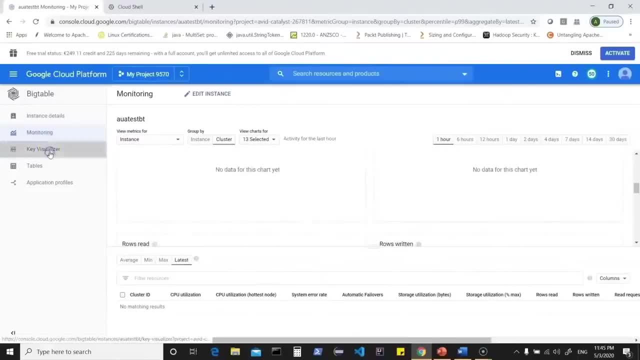 system errors, automatic failovers, storage utilization, and so on. you can storage utilization and so on. you can storage utilization, and so on. you can click on key visualizer, which will allow. click on key visualizer, which will allow. click on key visualizer which will allow you to look into your table, if you have. 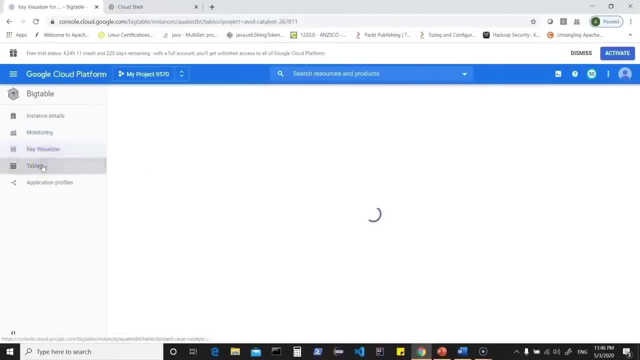 you to look into your table, if you have you to look into your table, if you have already created some data here and you already created some data here and you already created some data here and you can click on tables to see how many. can click on tables to see how many. 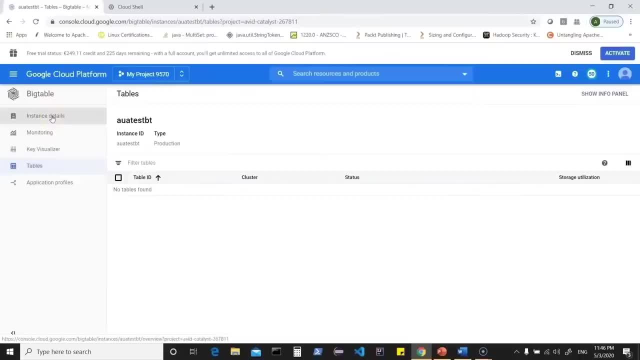 can click on tables to see how many tables you have added here. so that's in tables you have added here. so that's in tables you have added here. so that's in brief about your big tables, which is one. brief about your big tables, which is one. 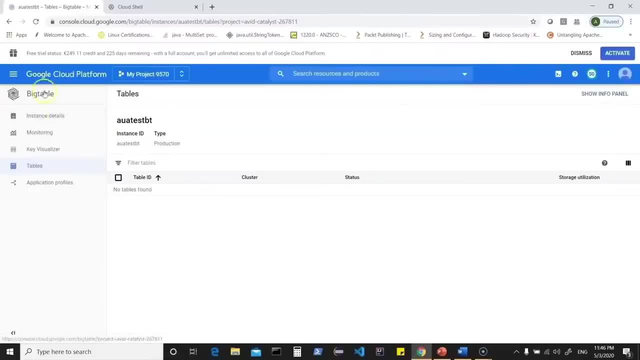 brief about your big tables, which is one thing which we need to remember. is it's thing which we need to remember. is it's thing which we need to remember? is it's not good for all use cases, so should be. not good for all use cases, so should be? 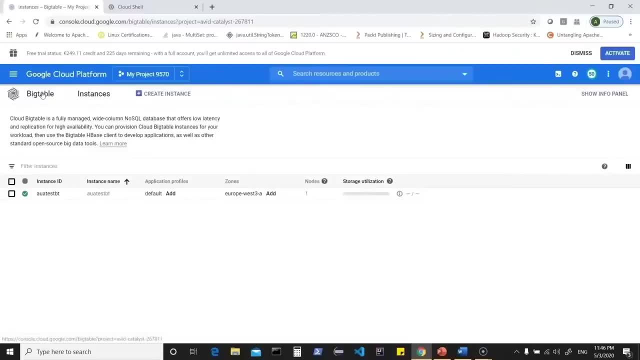 not good for all use cases, so should be used for low latency access. that is fast used for low latency access. that is fast used for low latency access. that is fast access and good if at least data is access. and good if at least data is access. and good if at least data is greater than one terabyte for smaller. 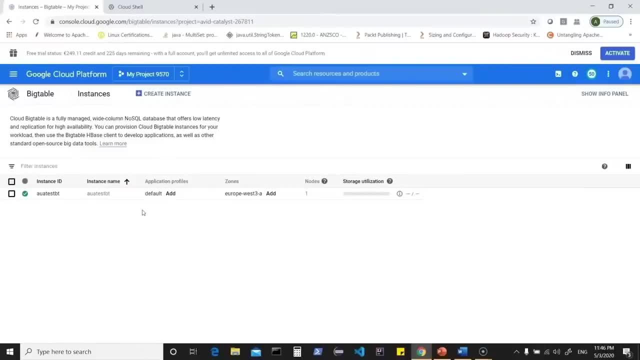 greater than one terabyte for smaller. greater than one terabyte. for smaller amount of data: the overhead is too high. amount of data: the overhead is too high. amount of data: the overhead is too high. so big tables performance will suffer if. so big tables performance will suffer if. 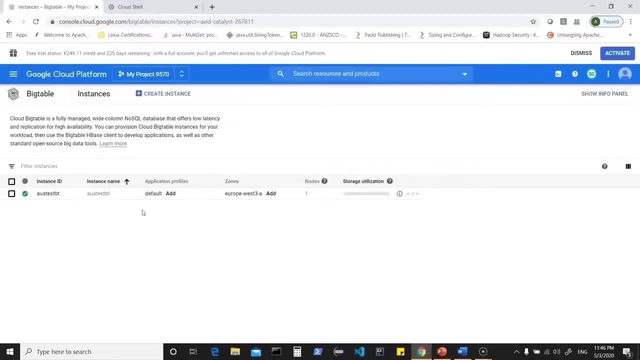 so big tables performance will suffer if you store individual elements. larger you store individual elements. larger you store individual elements. larger than 10 megabytes if you want to store than 10 megabytes. if you want to store than 10 megabytes. if you want to store bigger objects such as images, video, 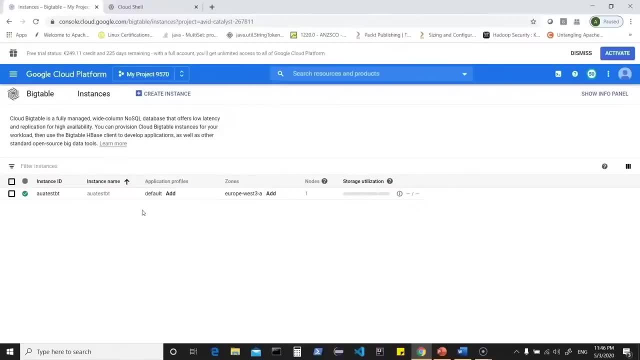 bigger objects such as images, video, bigger objects such as images, video files, then go for object storage and files then go for object storage and files then go for object storage and that would be a better option. so always that would be a better option. so always that would be a better option. so always remember big table is not a relational. 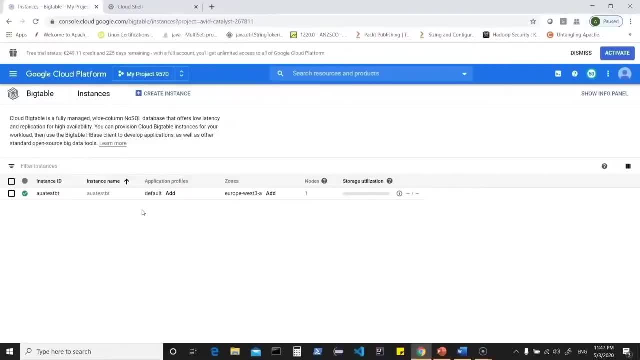 remember, big table is not a relational. remember, big table is not a relational database, it's a no SQL database. and when database, it's a no SQL database and when database, it's a no SQL database. and when you talk about multi-row transactions, or you talk about multi-row transactions, or 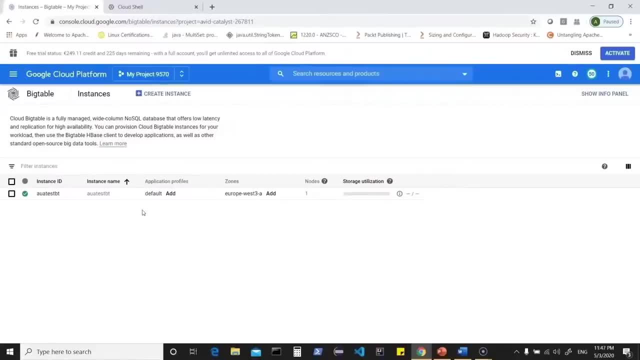 you talk about multi-row transactions or online transaction processing. big table. online transaction processing big table. online transaction processing big table- is not the right choice. so it can be. is not the right choice. so it can be. is not the right choice. so it can be used for wide range of applications. 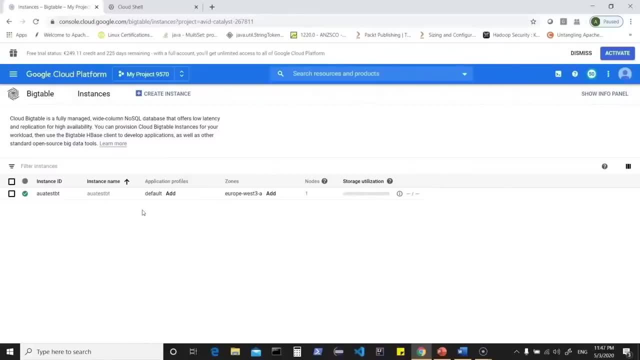 used for wide range of applications. used for wide range of applications, especially when you talk about your, especially when you talk about your, especially when you talk about your. OLAP, that is, online analytical processing. OLAP, that is online analytical processing. OLAP, that is online analytical processing, so it is designed to store key value. 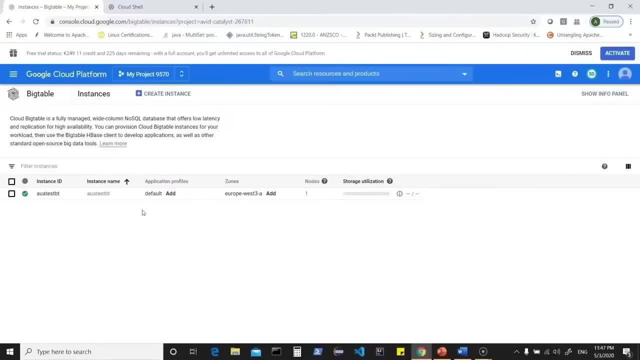 so it is designed to store key value. so it is designed to store key value pairs and there can be different use pairs and there can be different use pairs and there can be different use- or cloud data proc where you would want, or cloud data proc where you would want. 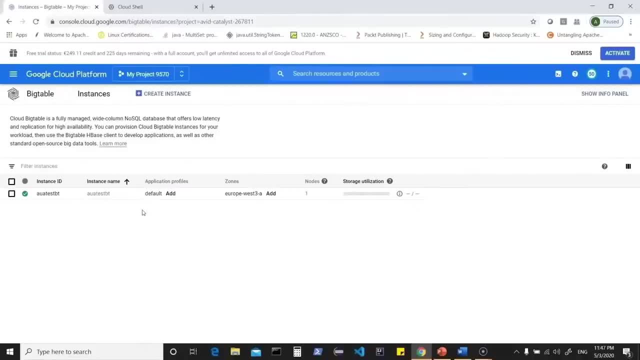 or cloud data proc where you would want map reduce kind of operations. big table: map reduce kind of operations. big table: map reduce kind of operations. big table can act as a good storage because it has can act as a good storage because it has can act as a good storage because it has very high throughput and scalability and 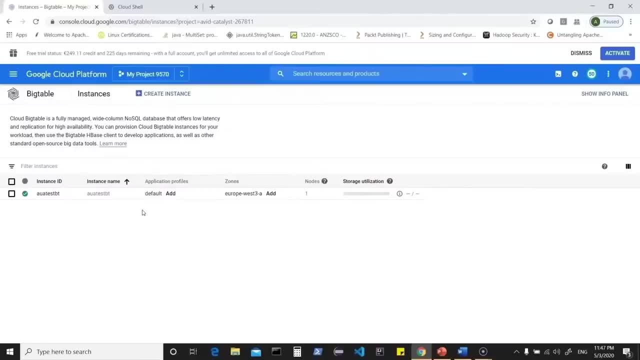 very high throughput and scalability and very high throughput and scalability and the best thing is that it supports. the best thing is that it supports- the best thing is that it supports: HBase API does, allowing easy integration. HBase API does, allowing easy integration. HBase API does allowing easy integration with Apache, Hadoop and spark clusters. 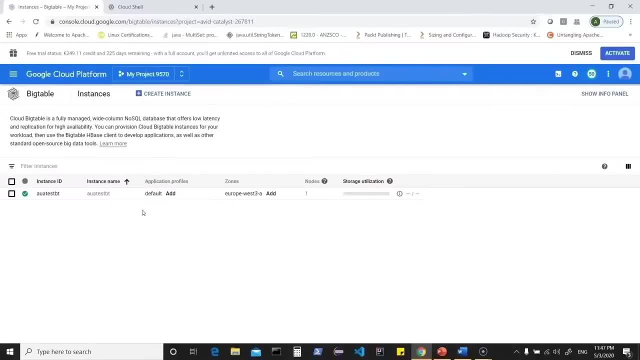 with Apache Hadoop and spark clusters, with Apache Hadoop and spark clusters, which you can bring up using one more, which you can bring up using one more, which you can bring up using one more service which Google cloud platform service, which Google cloud platform service, which Google cloud platform offers, which is called cloud data proc. 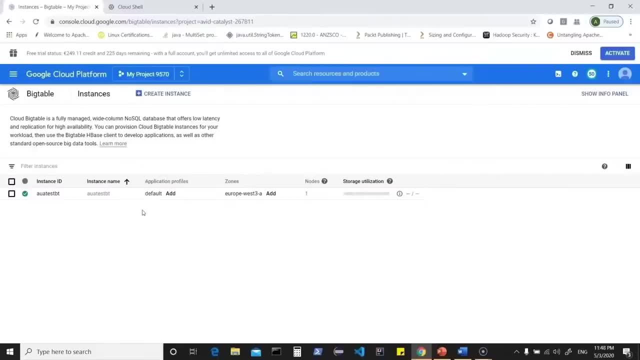 offers, which is called cloud data proc. offers, which is called cloud data proc. so big table is good for real-time. so big table is good for real-time. so big table is good for real-time analytics. it's commonly seen in analytics. it's commonly seen in analytics. it's commonly seen in financial services, IOT and others. and if 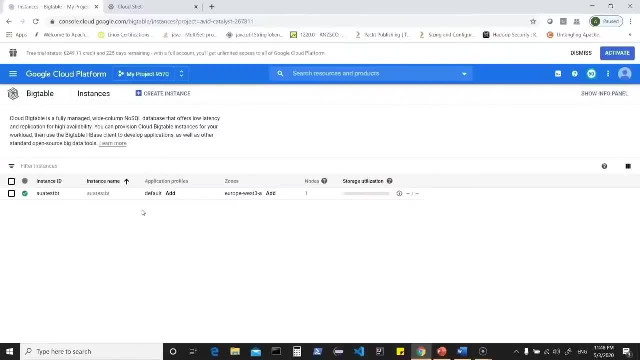 financial services, IOT and others. and if financial services, IOT and others, and if you are thinking of running interactive, you are thinking of running interactive, you are thinking of running interactive SQL, then big table would not be the SQL, then big table would not be the SQL, then big table would not be the right choice. but the other choice would 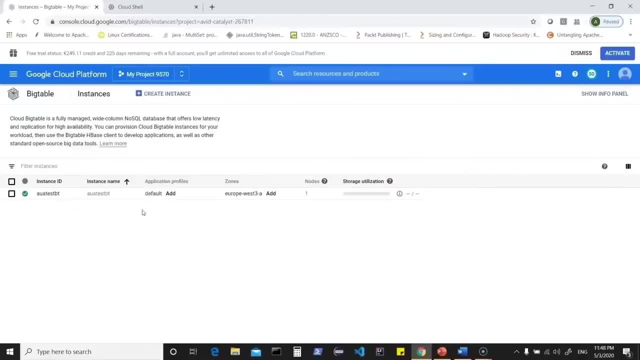 right choice, but the other choice would right choice, but the other choice would be BigQuery. you should also remember be BigQuery. you should also remember be BigQuery. you should also remember that this has a cluster running and you, that this has a cluster running and you. 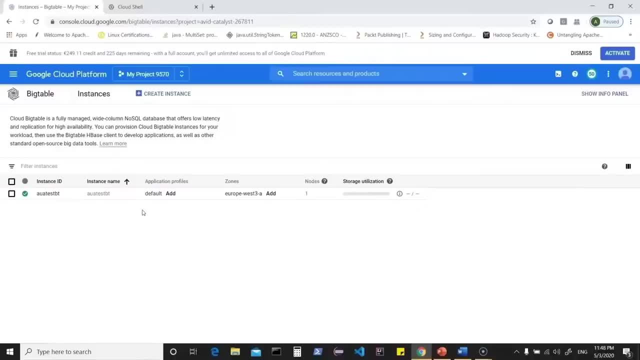 that this has a cluster running and you would be charged if this cluster kept on. would be charged if this cluster kept on. would be charged if this cluster kept on running. so you have to be very careful running. so you have to be very careful running. so you have to be very careful in your free account when you are using. 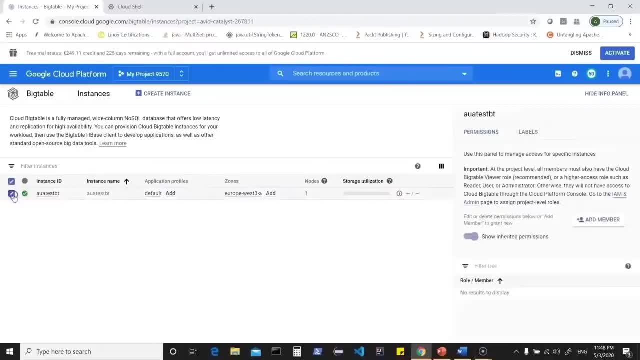 in your free account when you are using, in your free account, when you are using such services. now we have clicked on such services. now we have clicked on such services. now we have clicked on this one, so I can select this one and this one, so I can select this one and. 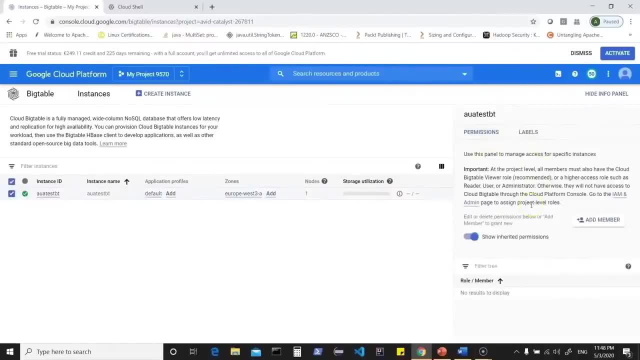 this one, so I can select this one and basically I can look at the permissions. basically I can look at the permissions. basically I can look at the permissions. I can look at the labels I can look at. I can look at the labels I can look at. I can look at the labels. I can look at inherited permissions. here I can also. 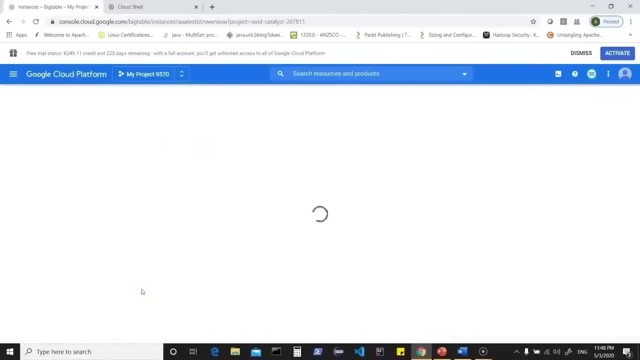 inherited permissions. here I can also inherited permissions. here I can also click on my instance, which we created. click on my instance, which we created. click on my instance, which we created, and either you can edit or you can just, and either you can edit or you can just. 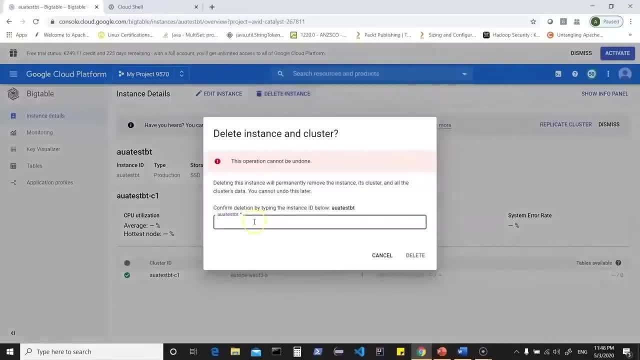 and either you can edit or you can just do a delete. so, as of now, we will just do a delete. so, as of now, we will just do a delete. so, as of now, we will just delete this, which needs you to give in, delete this, which needs you to give in. 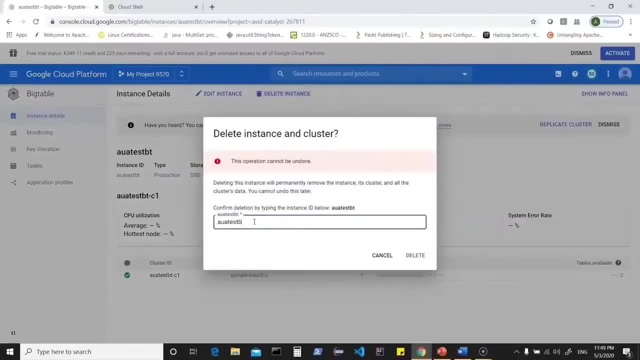 delete this, which needs you to give in the name. so we'll say au a test B D and the name. so we'll say au a test B D and the name. so we'll say au a test B D and then click on delete. so whenever you. 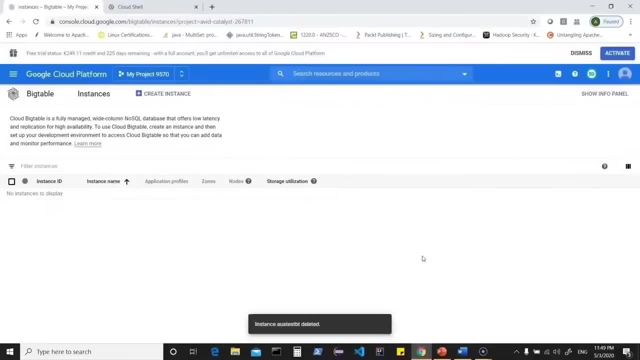 then click on delete. so whenever you then click on delete, so whenever you are trying out different services, the first are trying out different services, the first are trying out different services- the first approach should be setting up. these approach should be setting up. these approach should be setting up these different services, seeing how they work. 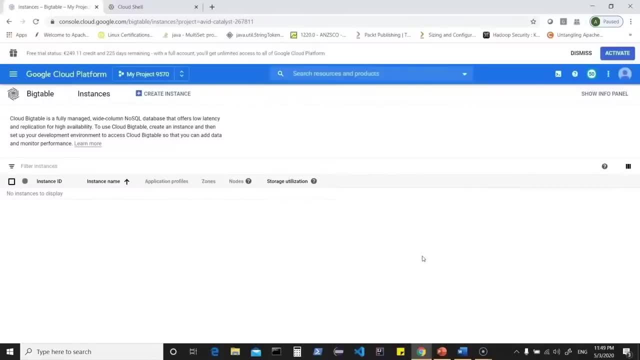 different services, seeing how they work, different services, seeing how they work, basically trying connecting to them and basically trying connecting to them, and basically trying connecting to them. and once you are satisfied with the initial, once you are satisfied with the initial, once you are satisfied with the initial test, then you can plan your actions and 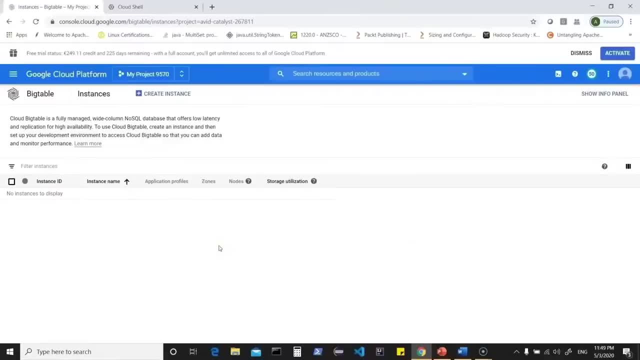 test, then you can plan your actions and test, then you can plan your actions and come back and use the service for a come back and use the service for a. come back and use the service for a longer duration- now that's your big table. longer duration- now that's your big table. 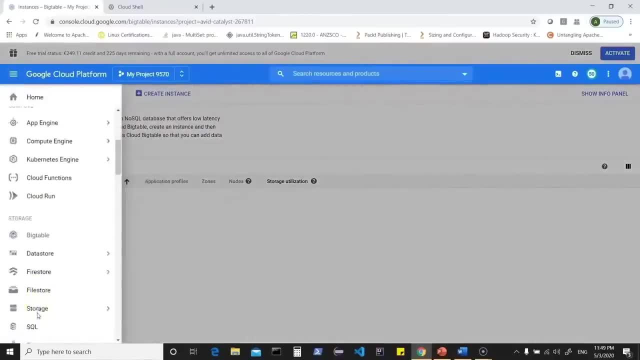 longer duration. now that's your big table, which is one of the offerings we can go, which is one of the offerings we can go, which is one of the offerings we can go back into storage, and here you have back into storage, and here you have back into storage, and here you have other options which are available. so for 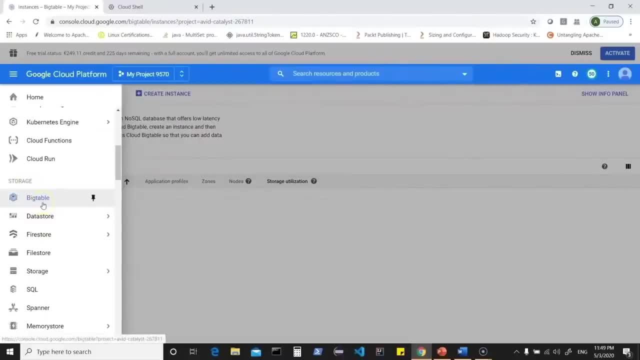 other options which are available. so, for other options which are available. so, for example, we were in big table. you also example, we were in big table. you also example, we were in big table. you also have an option such as cloud data store. have an option such as cloud data store. 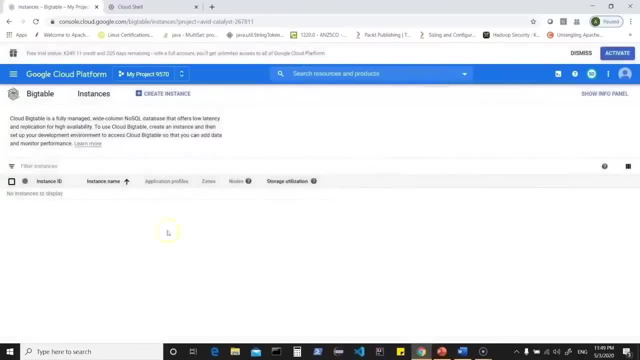 have an option such as cloud data store. now that's one more service which is now that's one more service, which is now that's one more service which is offered by Google cloud platform, when it offered by Google cloud platform, when it offered by Google cloud platform when it comes to storage domain. so Google added. 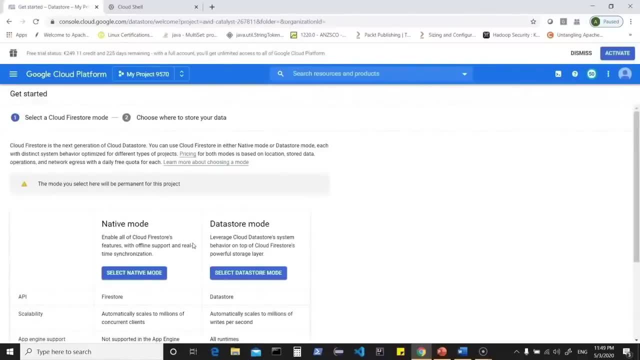 comes to storage domain, so Google added: comes to storage domain, so Google added software on top of big table. which software on top of big table? which software on top of big table which supports more than simple key value? supports more than simple key value. supports more than simple key value pairs. when you talk about secondary 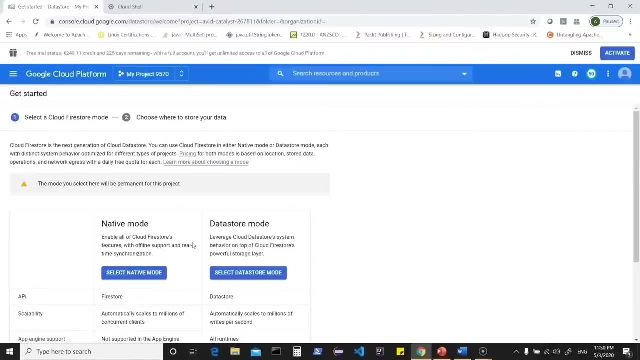 pairs, when you talk about secondary pairs, when you talk about secondary indexes, instead of just having one indexes, instead of just having one indexes, instead of just having one primary index. when you talk about asset primary index. when you talk about asset primary index, when you talk about asset properties for reliable transactions. 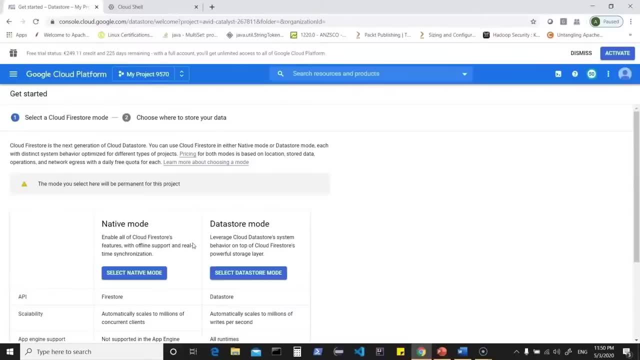 properties for reliable transactions. properties for reliable transactions, such as SQL query like language. so such as SQL query like language. so such as SQL query like language. so these features or these services were these features, or these services were these features or these services were added to or on top of your big table. 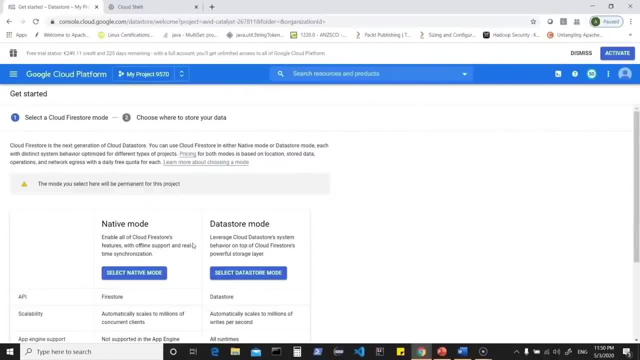 added to or on top of your big table- added to or on top of your big table- which gave birth to a new service. which which gave birth to a new service. which which gave birth to a new service which was released as cloud datastore. so this was released as cloud datastore. so this 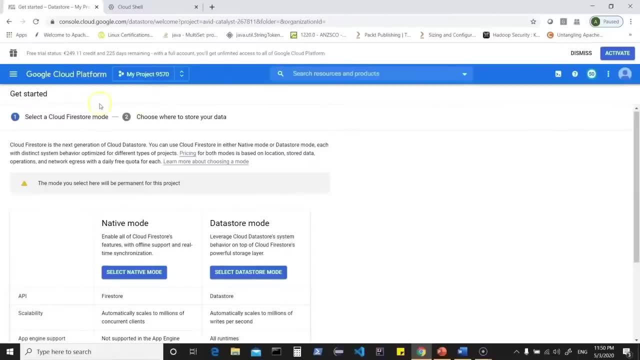 was released as cloud datastore. so this is where you have cloud datastore and is where you have cloud datastore and is where you have cloud datastore and you can select a cloud firestore mode. so you can select a cloud firestore mode. so you can select a cloud firestore mode so you can go for a native mode: enable all. 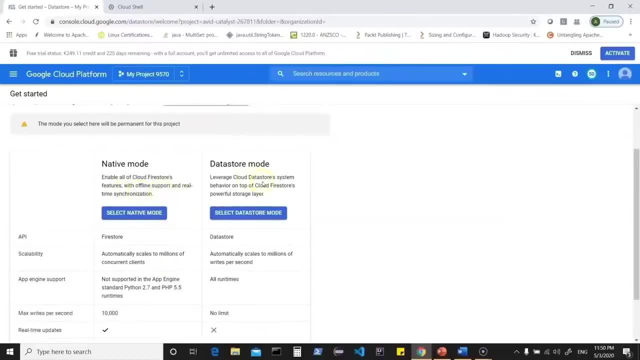 you can go for a native mode: enable all. you can go for a native mode enable all. cloud fire stores. features with offline cloud fire stores, features with offline cloud fire stores, features with offline support. or you can go for clouds datastore support. or you can go for clouds datastore. 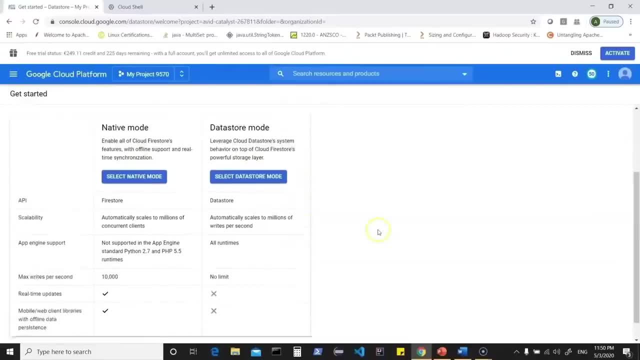 support. or you can go for clouds datastore system on top of clouds fire system on top of clouds fire system on top of clouds fire store. so these are different options here. store, so these are different options here. store, so these are different options here and here we look at the API or 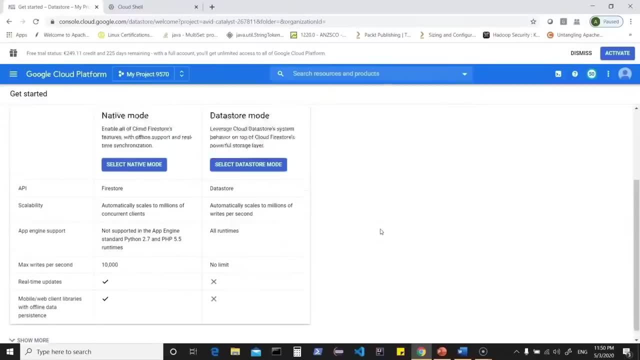 and here we look at the API. or- and here we look at the API- or scalability engine support: how many scalability engine support? how many scalability engine support, how many rights it supports, and so on. you can rights it supports, and so on. you can rights it supports, and so on. you can choose one of these and then you can. 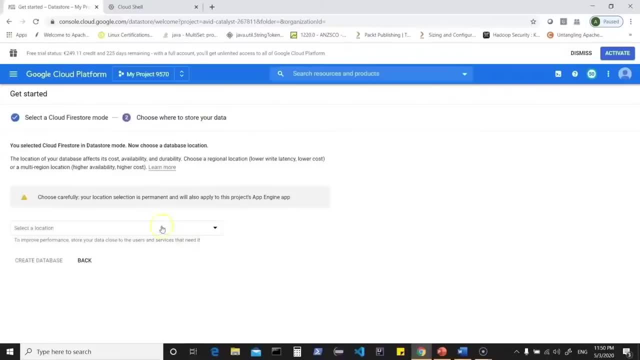 choose one of these, and then you can choose one of these, and then you can choose where to store your data. so for, choose where to store your data. so for, choose where to store your data. so, for example, if I click on this one, then it. example: if I click on this one, then it. 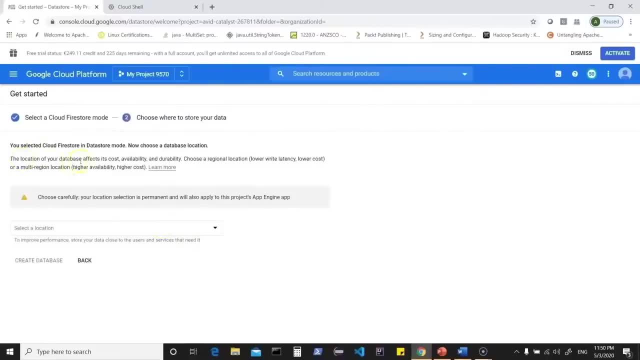 example, if I click on this one, then it choose. asks me to choose a location, so choose. asks me to choose a location, so choose. asks me to choose a location. so it says the location of your database. it says the location of your database. it says the location of your database affect its cost, availability and. 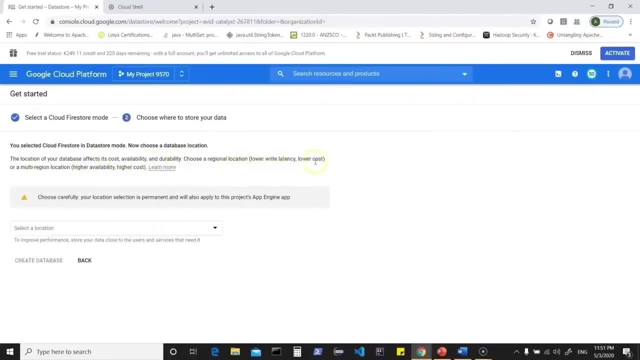 affect its cost availability. and affect its cost availability and durability. choose a regional location- durability. choose a regional location- durability. choose a regional location: lower right latency: lower cost or multi. lower right latency: lower cost or multi. lower right latency. lower cost or multi region location. here I can basically. 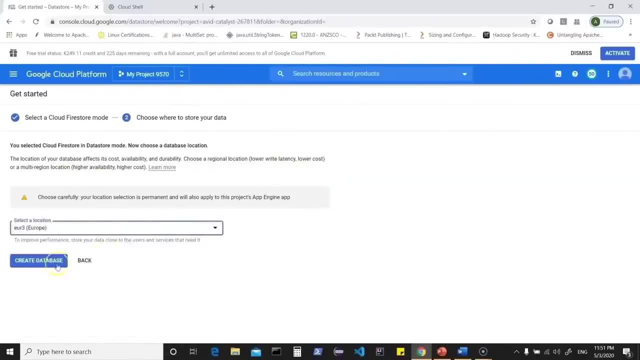 region location: here I can basically region location. here I can basically choose, for example, Europe, and then I can choose, for example, Europe, and then I can choose, for example, Europe, and then I can go ahead and create a database so it. go ahead and create a database, so it. 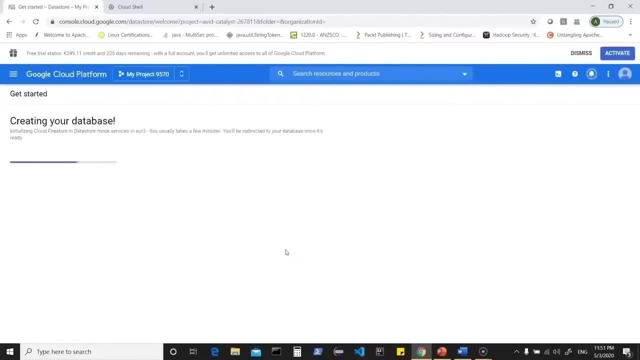 go ahead and create a database. so it says initializing cloud fire store. in says initializing cloud fire store. in says initializing cloud fire store in datastore mode services in eu3: this datastore mode services in eu3. this datastore mode services in eu3. this usually takes a few minutes. you will be. 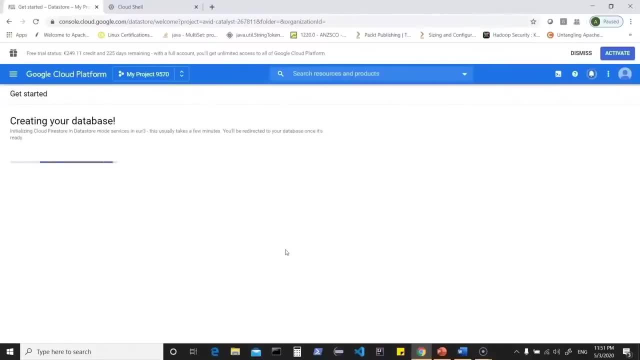 usually takes a few minutes. you will be- usually takes a few minutes- you will be redirect to your database. once it is redirect to your database, once it is redirect to your database, once it is ready. so if we compare the pricing ready, so if we compare the pricing, 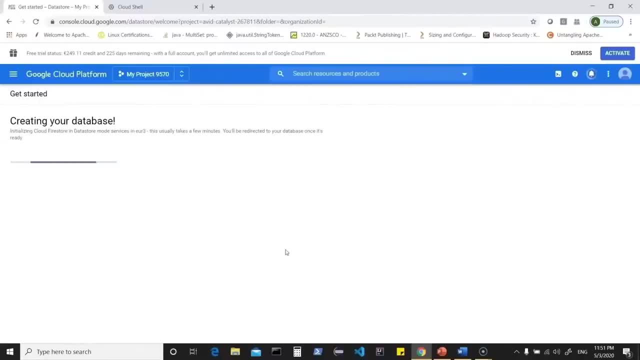 ready. so if we compare the pricing structure between cloud datastore and structure between cloud datastore and structure between cloud datastore and cloud bigtable, always remember cloud cloud bigtable. always remember cloud cloud bigtable. always remember cloud datastore: you pay for monthly storage. datastore: you pay for monthly storage. 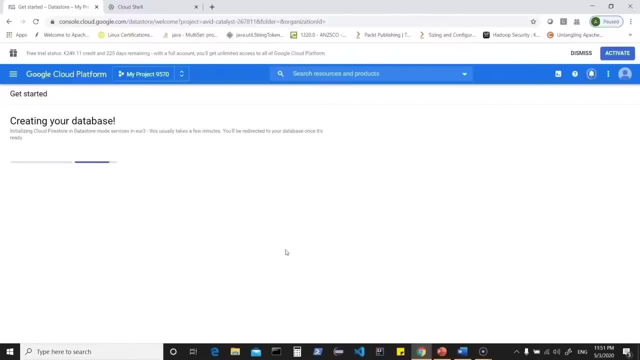 datastore, you pay for monthly storage, which is also in the case of big table, which is also in the case of big table, which is also in the case of big table. however, here you are paying for monthly. however, here you are paying for monthly. however, here you are paying for monthly storage for reads and writes. but in case 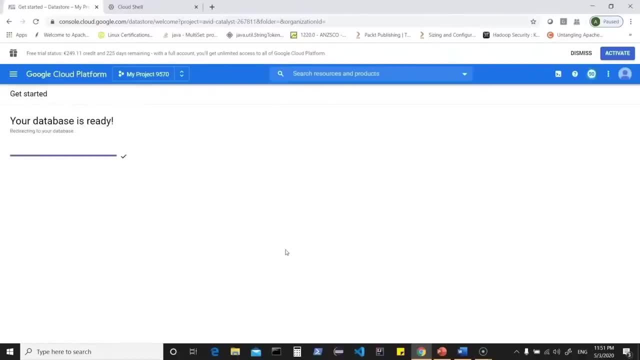 storage for reads and writes. but in case storage for reads and writes. but in case of big table, you are paying for cluster of big table. you are paying for cluster of big table. you are paying for cluster when it is running, so cloud datastore is when it is running, so cloud datastore is. 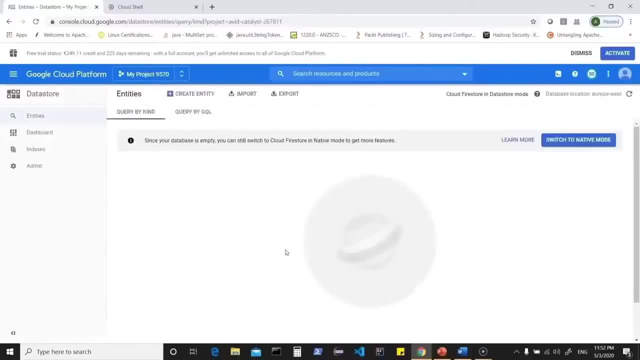 when it is running. so cloud datastore is a good option for small data in a good option for small data, in a good option for small data in frequent access, and it acts cheaper when frequent access and it acts cheaper when frequent access and it acts cheaper when you talk about large amount of data or 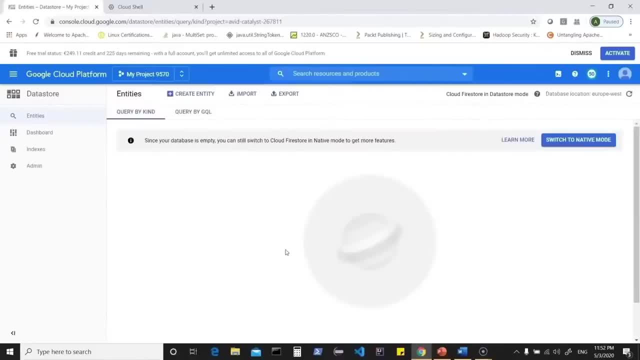 you talk about large amount of data. or you talk about large amount of data or big data and frequent access, then you big data and frequent access. then you big data and frequent access. then you are talking about cloud- big table so big. are talking about cloud, big table, so big. 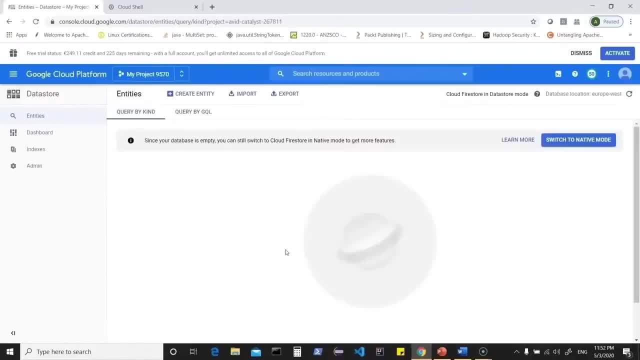 are talking about cloud big table. so big table is cheaper when you talk about table is cheaper when you talk about table is cheaper when you talk about larger amount of data. so here it says: larger amount of data. so here it says: larger amount of data. so here it says: since your database is empty, you can. 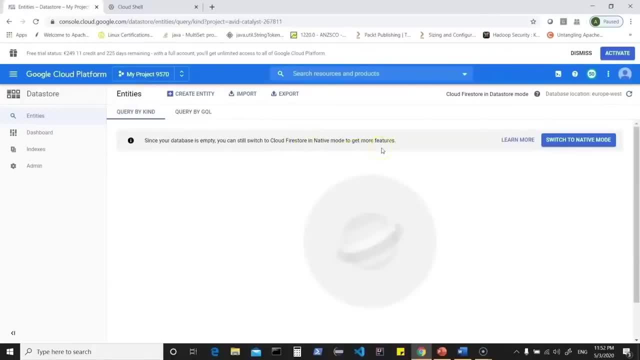 since your database is empty, you can. since your database is empty, you can still switch to cloud fire store in. still switch to cloud fire store in. still switch to cloud fire store in native mode to get more features. you native mode to get more features. you native mode to get more features. you could do that, you could learn, you could. 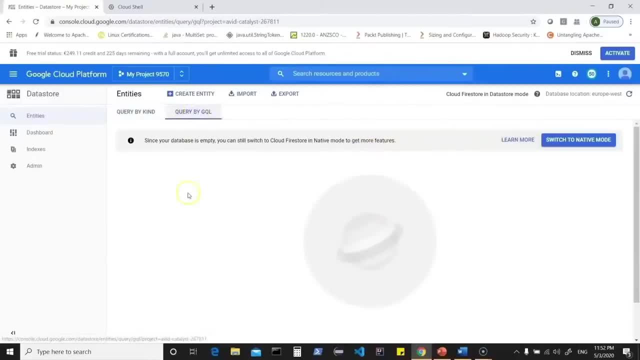 could do that you could learn you could. could do that you could learn. you could say query by GQL. as of now, we don't have say query by GQL. as of now, we don't have say query by GQL. as of now. we don't have any data here. let's look at the. 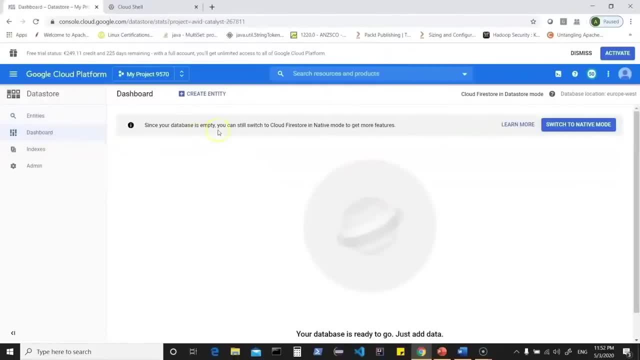 any data here. let's look at the any data here. let's look at the dashboard which says: since your database dashboard, which says: since your database dashboard, which says, since your database is empty, you can still switch to cloud is empty, you can still switch to cloud is empty, you can still switch to cloud fire store in native mode to get more. 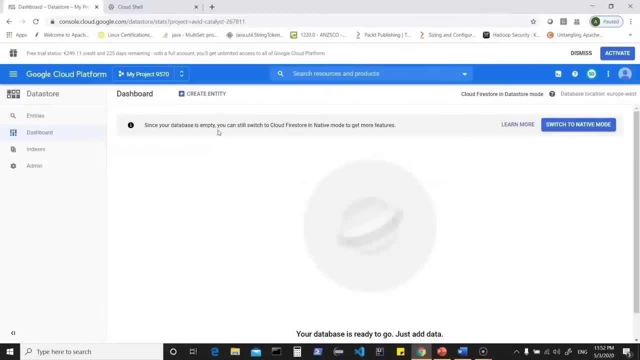 fire store in native mode to get more. fire store in native mode to get more features. so this is your cloud data features. so this is your cloud data features. so this is your cloud data store and it has many features which store and it has many features which. 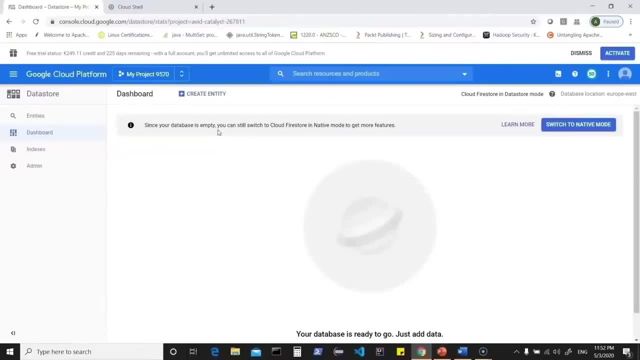 store and it has many features which help you to work with your data, however, help you to work with your data, however, help you to work with your data. however, some features or important features of some features or important features of some features or important features of our DBMS's were still missing, and that's. 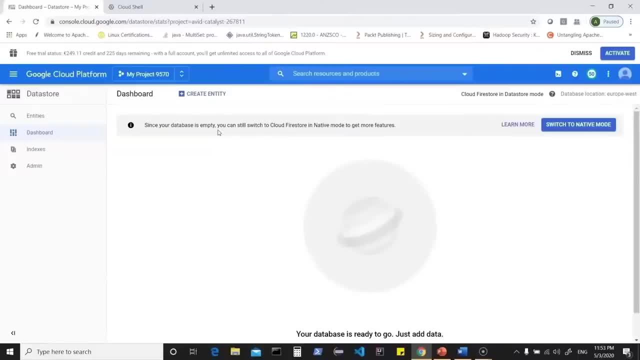 our DBMS's were still missing. and that's: our DBMS's were still missing. and that's where Google created yet another big, where Google created yet another big, where Google created yet another big table based service called cloud spanner. table based service called cloud spanner. 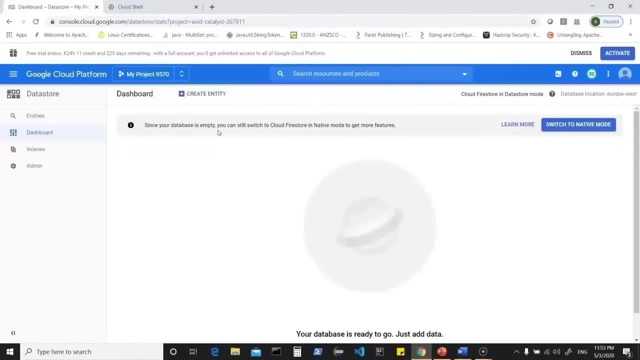 table based service called cloud spanner. now we can continue working on cloud. now we can continue working on cloud. now we can continue working on cloud datastore, which basically gives you one datastore, which basically gives you one datastore, which basically gives you one option to work with your data. you can. 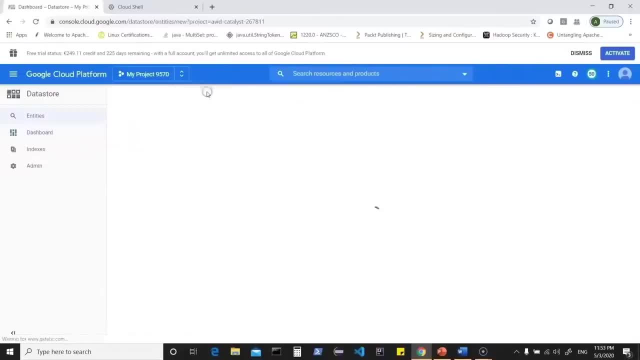 option to work with your data. you can option to work with your data. you can create an entity here by clicking on create an entity here, by clicking on create an entity here, by clicking on create entity, and that basically gives create entity, and that basically gives create entity and that basically gives you options such as default namespace. 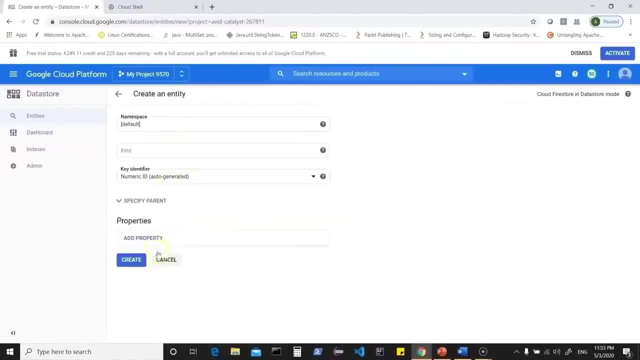 you you options such as default namespace. you you options such as default namespace. you can give a kind. you can give numeric. you can give a kind. you can give numeric. you can give a kind. you can give numeric ID and you can start adding properties: ID and you can start adding properties. 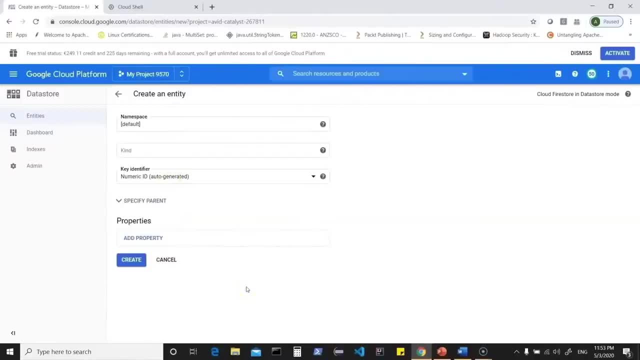 ID and you can start adding properties. but to learn more about datastore- we. but to learn more about datastore- we. but to learn more about datastore, we will learn about this in further, will learn about this in further, will learn about this in further sessions. so, as of now, I'm going to click. 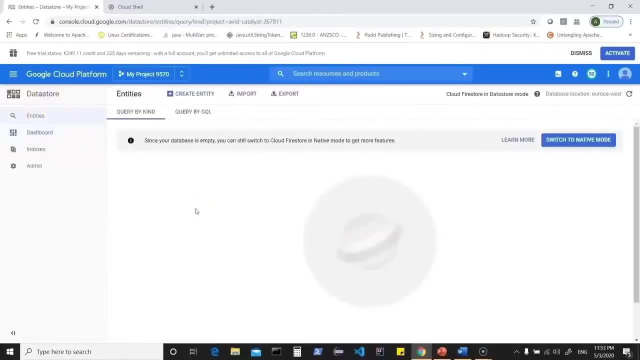 sessions. so as of now, I'm going to click sessions. so as of now, I'm going to click on cancel. I am going to go back to my on cancel. I am going to go back to my on cancel. I am going to go back to my datastore and this, basically, let's go to. 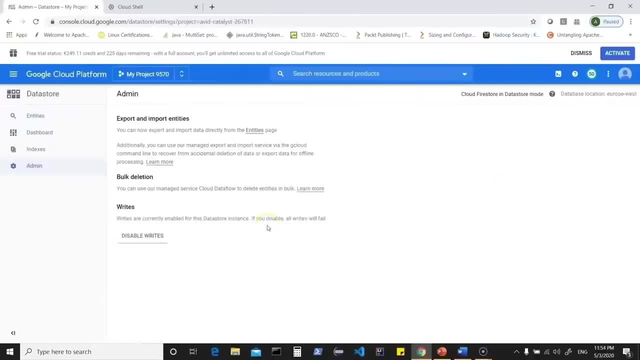 datastore and this basically let's go to datastore. and this basically let's go to datastore option. or I can go into admin datastore option, or I can go into admin datastore option, or I can go into admin here, which basically says: if you have. here, which basically says: if you have. 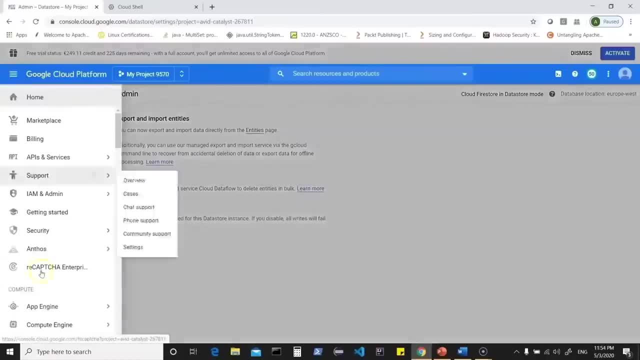 here, which basically says: if you have entities, you can import or export them. so entities, you can import or export them. so entities, you can import or export them. so let's go back and let's again look, let's go back and let's again look, let's go back and let's again look into storage options. so as of now, we were in. 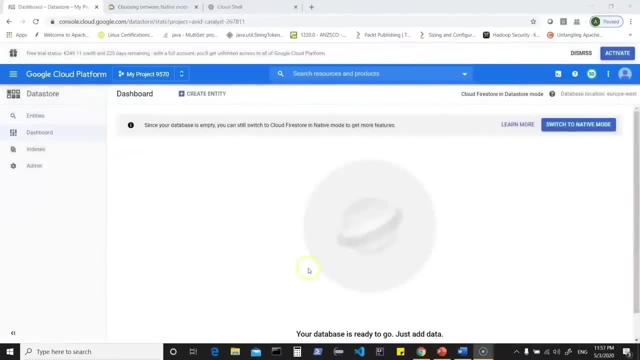 into storage options. so, as of now, we were in into storage options. so, as of now, we were in datastore. let's click on this one. so datastore. let's click on this one. so datastore. let's click on this one. so, as I mentioned your cloud datastore, as I mentioned your cloud datastore, 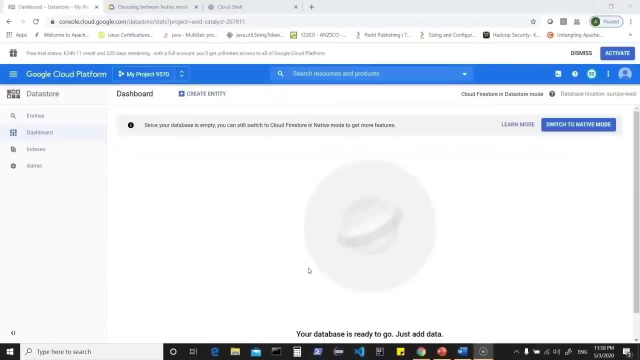 as I mentioned, your cloud datastore, which basically gives you some, which basically gives you some, which basically gives you some additional features on top of your big additional features, on top of your big additional features on top of your big table. but what Google also did was it table, but what Google also did was it. 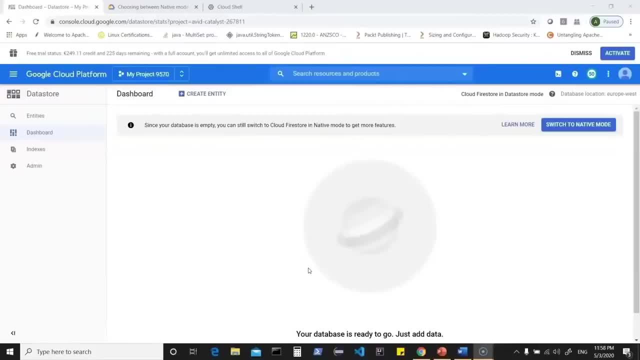 table. but what Google also did was it realized that there was in need for our, realized that there was in need for our, realized that there was in need for our DBMS feature support. that is, there were DBMS feature support. that is, there were DBMS feature support. that is, there were a lot of features. now, here we have. 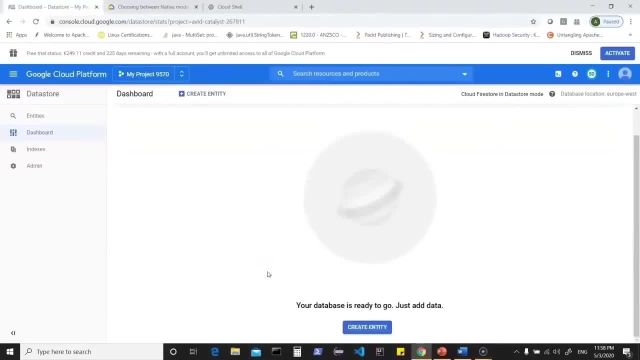 a lot of features now here. we have a lot of features now here. we have created a datastore and it says your created a datastore. and it says your created a datastore and it says your database is ready to go, just add data. database is ready to go, just add data. 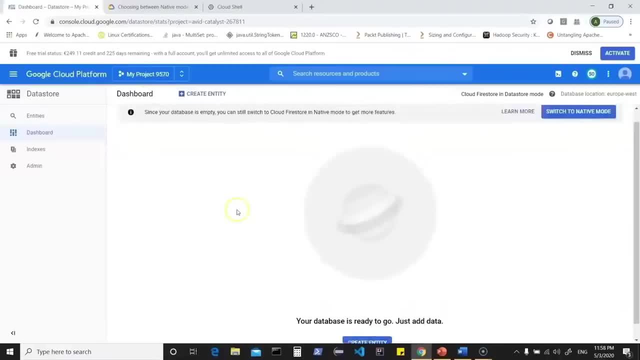 database is ready to go. just add data. you can create entity, start putting in. you can create entity, start putting in. you can create entity, start putting in data, and then you can go ahead and query data, and then you can go ahead and query data, and then you can go ahead and query this. so if you would want to learn more, 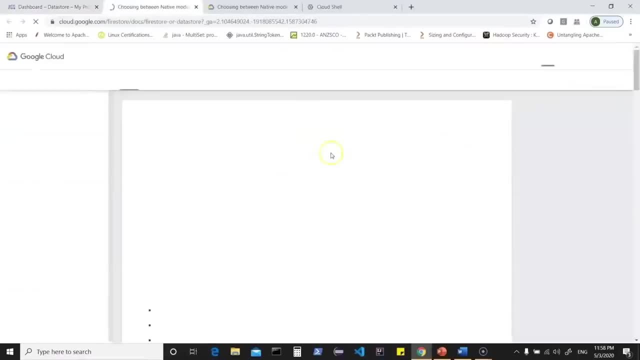 this. so if you would want to learn more this, so if you would want to learn more about your datastore, you can just click about your datastore. you can just click about your datastore, you can just click on this one and that takes you to the on this one, and that takes you to the. 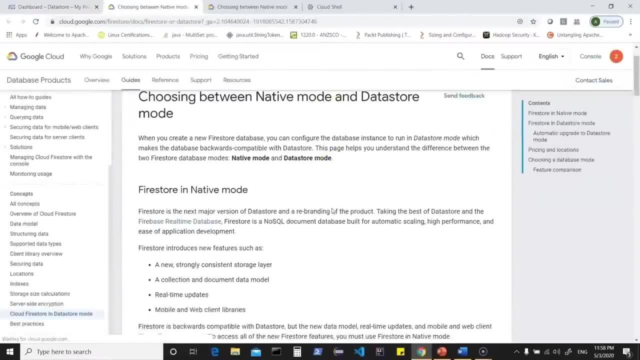 on this one, and that takes you to the complete documentation of native mode and complete documentation of native mode and complete documentation of native mode and datastore mode. what is fire store in datastore mode? what is fire store in datastore mode? what is fire store in native mode? what is in datastore mode? 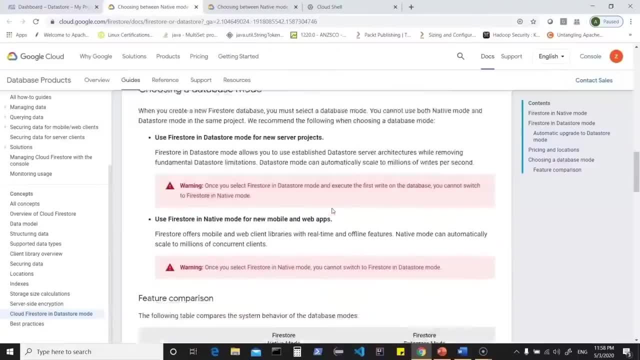 native mode. what is in datastore mode? native mode. what is in datastore mode? what are pricing and locations, how you. what are pricing and locations, how you, what are pricing and locations, how you choose a database mode. what are the choose a database mode. what are the choose a database mode. what are the feature comparisons, what you can do, what. 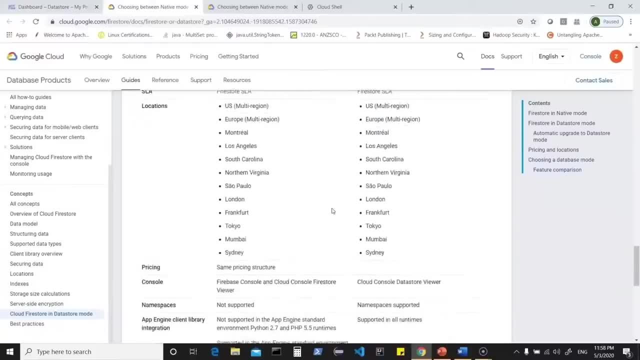 feature comparisons: what you can do. what feature comparisons, what you can do, what you are allowed to do here, what you are allowed to do here, what you are allowed to do here, what programming languages can be used. programming languages can be used. programming languages can be used, different regions, pricing and so on. as 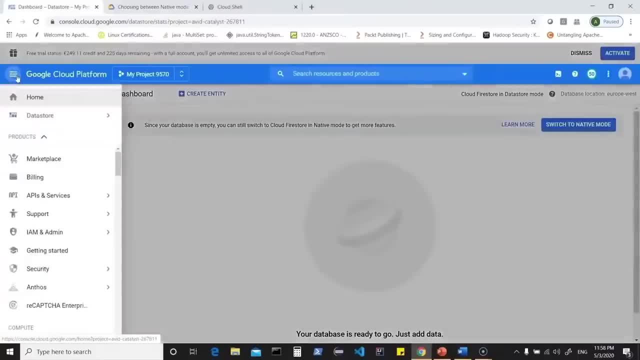 different regions, pricing, and so on. as different regions, pricing, and so on, as of now, we'll click on this one and let's of now, we'll click on this one, and let's of now, we'll click on this one. and let's look at one advanced service, which 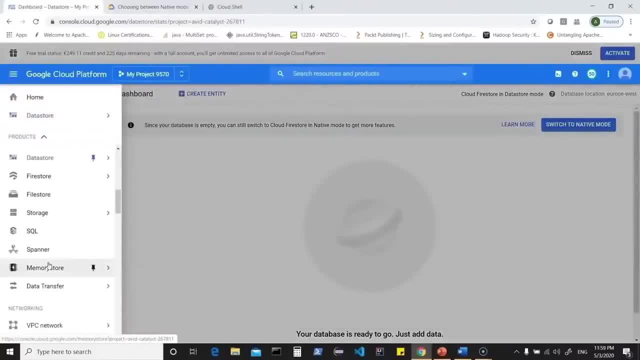 look at one advanced service, which. look at one advanced service which Google Cloud came up with. when it comes, Google Cloud came up with. when it comes, Google Cloud came up with when it comes to your additional features of our DBMS, to your additional features of our DBMS. 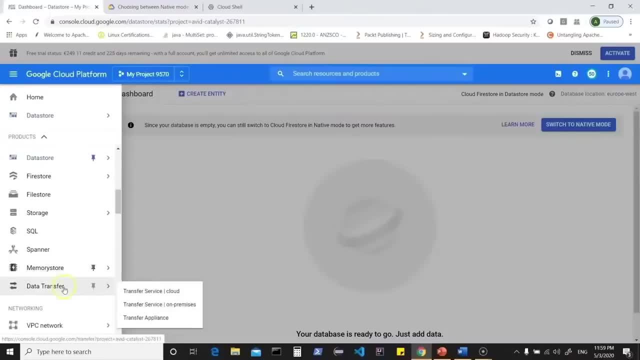 to your additional features of our DBMS. so Google created yet another big table. so Google created yet another big table. so Google created yet another big table based service called cloud spanner. now based service called cloud spanner. now based service called cloud spanner. now, that you might not see here, but if you 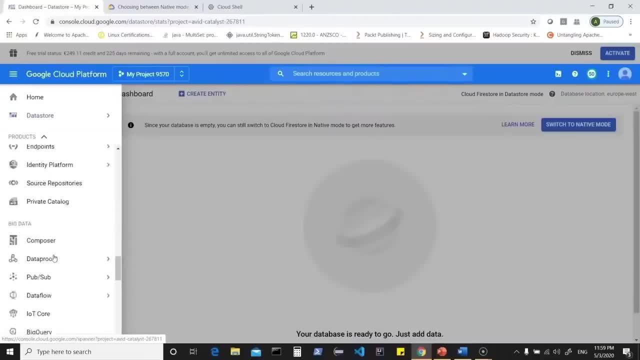 that you might not see here, but if you that you might not see here, but if you scroll down, you should be able to see scroll down. you should be able to see scroll down. you should be able to see your cloud spanner in the options here. your cloud spanner in the options here. 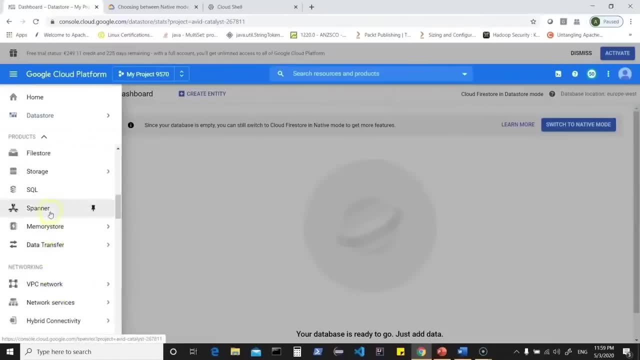 your cloud spanner in the options here? or did we miss it on the top, so let's. or did we miss it on the top, so let's. or did we miss it on the top, so let's again. look here: yeah, so it is here. and again. look here. yeah, so it is here. and 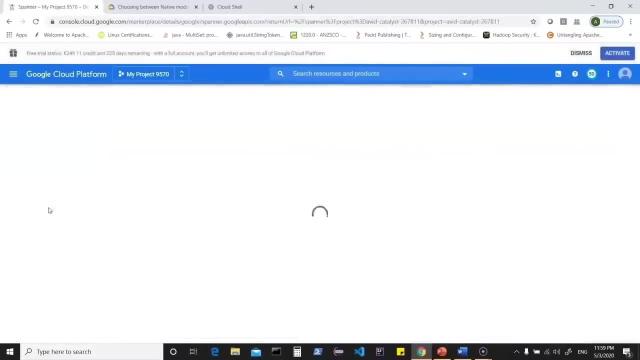 again. look here. yeah, so it is here and you can click on spanner so cloud. you can click on spanner so cloud. you can click on spanner so cloud. spanner was released in 2017 it. spanner was released in 2017 it. 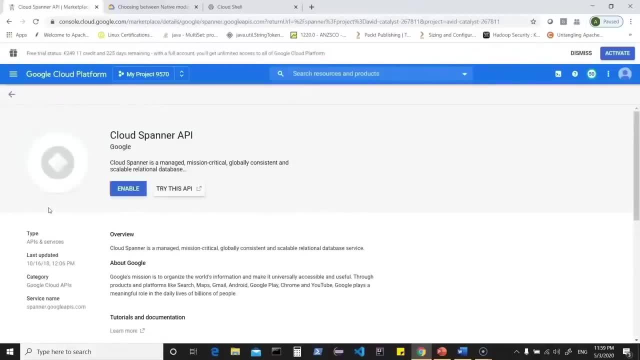 spanner was released in 2017. it basically supports relational schema, so basically supports relational schema. so basically supports relational schema. so it offers strong consistency for all. it offers strong consistency for all. it offers strong consistency for all. queries which can be SQL based, you can. queries which can be SQL based, you can. 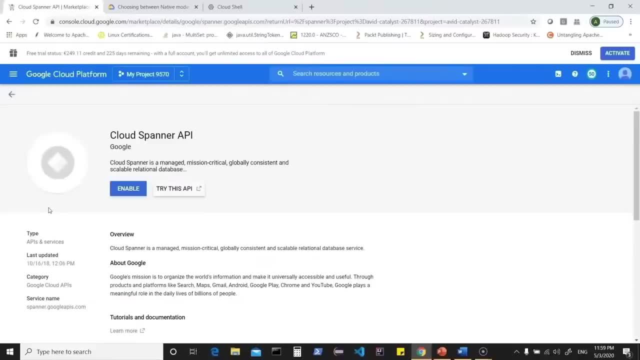 queries which can be SQL based. you can have multi region deployment. now when it have multi region deployment. now when it have multi region deployment. now when it comes to massive scalability requirement, comes to massive scalability requirement, comes to massive scalability requirement and strong consistency. cloud spanner is: 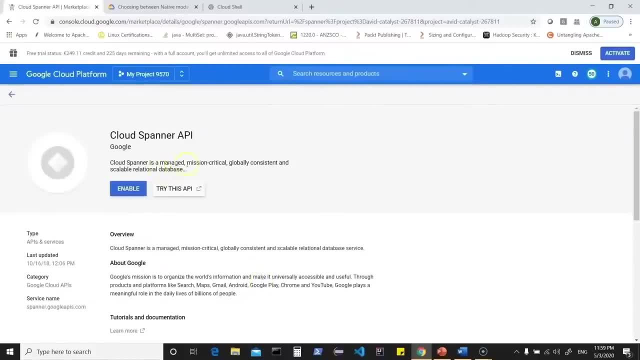 and strong consistency cloud spanner is. and strong consistency, cloud spanner is a good option. so it says cloud spanner a good option. so it says cloud spanner a good option. so it says cloud spanner is a managed mission-critical globally, is a managed mission-critical globally. 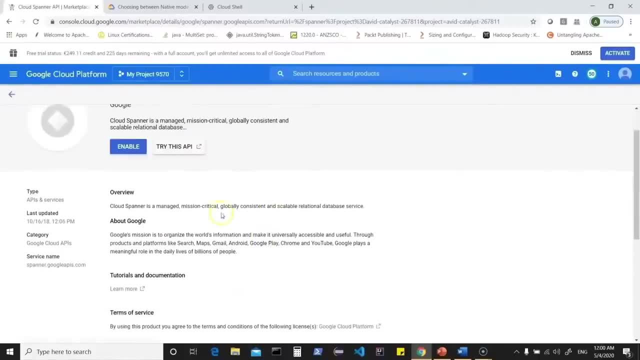 is a managed, mission-critical, globally consistent and scalable relational, consistent and scalable relational, consistent and scalable relational database. so if you would want to use this database, so if you would want to use this database, so if you would want to use this, then you will have to enable this API. 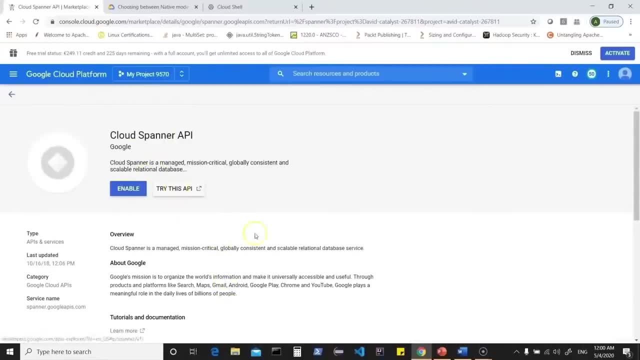 then you will have to enable this API. then you will have to enable this API which shows you an option here. it says: which shows you an option here. it says: which shows you an option here. it says: try this API, so it's a managed service. try this API, so it's a managed service. 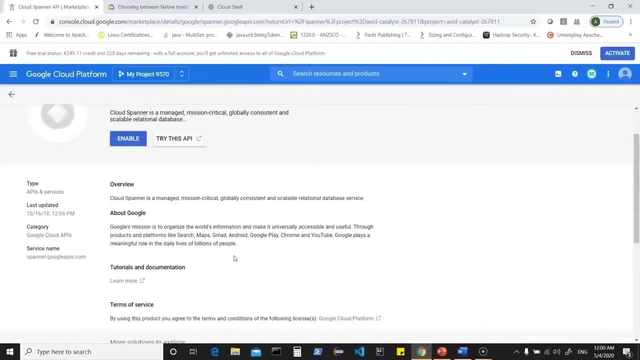 try this API. so it's a managed service. so it is one of the Google's most so it is one of the Google's most so it is one of the Google's most expensive database services. there is expensive database services. there is expensive database services. there is also one more database service, which is 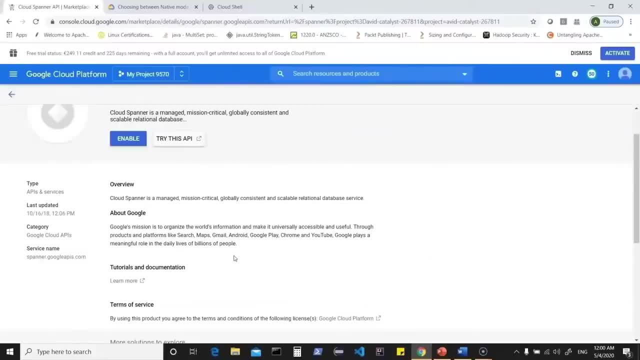 also one more database service, which is also one more database service, which is cloud SQL, which can be used. so when we cloud SQL which can be used, so when we cloud SQL which can be used, so when we talk about your cloud spanner, it is talk about your cloud spanner, it is. 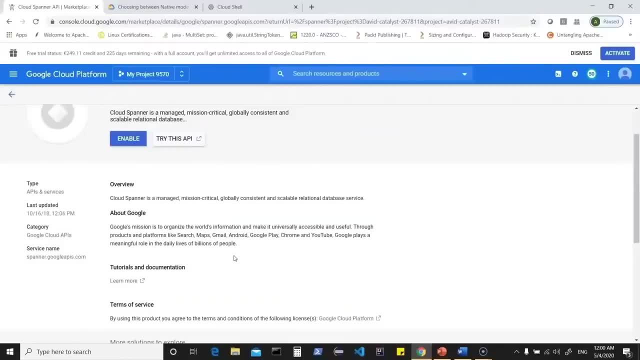 talk about your cloud spanner. it is fully managed relational database. fully managed relational database. fully managed relational database service. it is massively distributed. you service: it is massively distributed. you service- it is massively distributed. you can have millions of machines across. can have millions of machines across, can have millions of machines across hundreds of data centers with support. 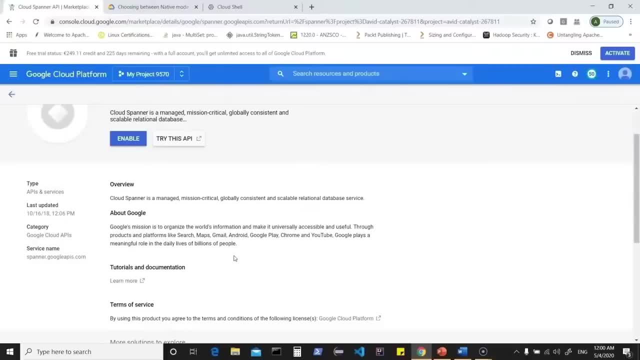 hundreds of data centers with support. hundreds of data centers with support, automatic sharding and synchronous automatic sharding and synchronous automatic sharding and synchronous replication. it gives you low latency and replication. it gives you low latency and replication. it gives you low latency and schema updates without downtime making. 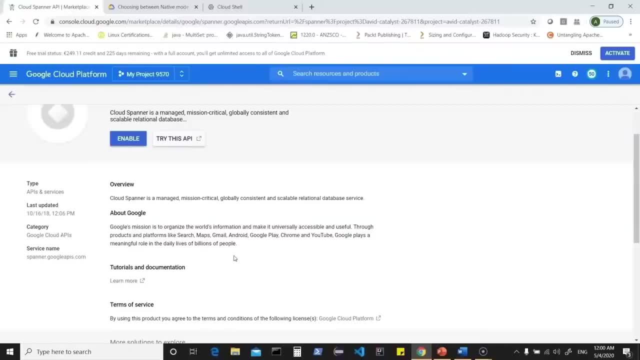 schema updates without downtime. making schema updates without downtime. making data high availability and reliability. data high availability and reliability. data high availability and reliability. so we learn about cloud spanner with. so we learn about cloud spanner with. so we learn about cloud spanner with more details later, in other sessions now. 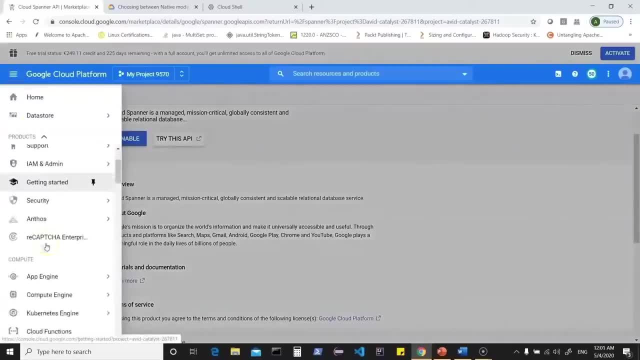 more details later in other sessions. now, more details later in other sessions. now we can also go back to storage and we, we can also go back to storage and we, we can also go back to storage and we can look at the different options, which can look at the different options which we have here. so you have object: storage: 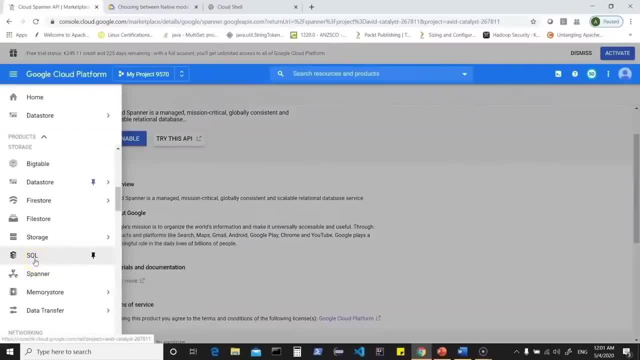 we have here, so you have object storage. we have here, so you have object storage. you have spanner. you also have your SQL. you have spanner. you also have your SQL, you have spanner. you also have your SQL based service, which is yet another based service, which is yet another. 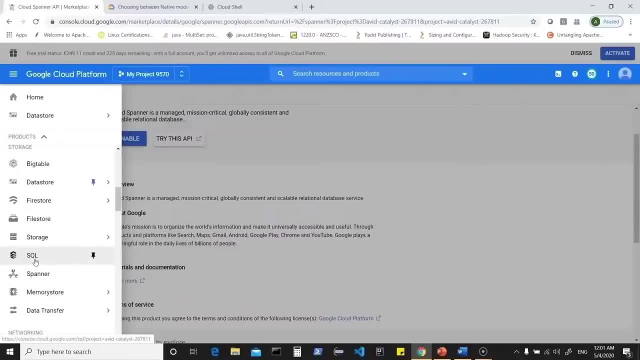 based service, which is yet another managed service offered by cloud, or managed service offered by cloud, or managed service offered by cloud or Google cloud. I would say so, that's Google cloud. I would say so, that's Google cloud. I would say so, that's called cloud SQL. so this is basically a 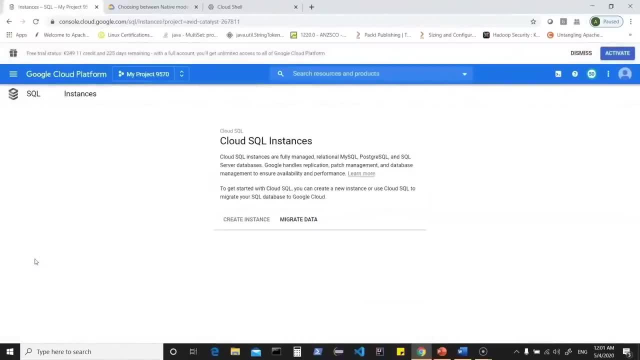 called cloud SQL, so this is basically a called cloud SQL. so this is basically a service which allows you to have fully service, which allows you to have fully service, which allows you to have fully managed relational MySQL, Postgres and SQL. managed relational MySQL, Postgres and SQL. 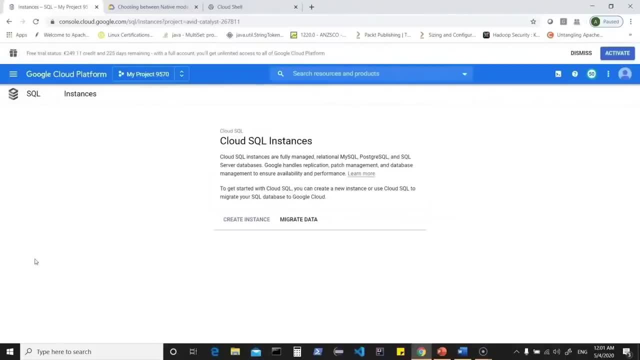 managed relational MySQL, Postgres and SQL server databases. Google handles server databases. Google handles server databases. Google handles replication, patch management database. replication patch management database, replication, patch management, database management and other things which are management and other things which are management and other things which are related to this. managed or fully managed. 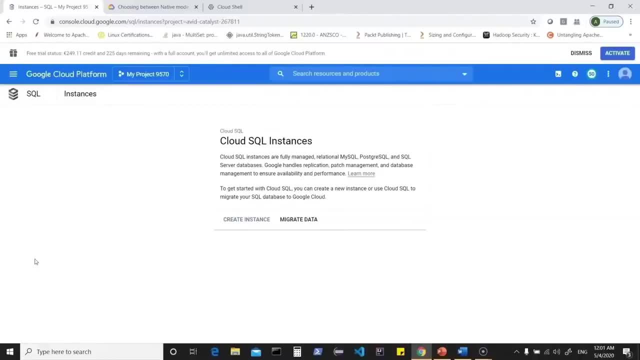 related to this: managed or fully managed. related to this: managed or fully managed database service. it can allow you to database service. it can allow you to database service. it can allow you to handle terabytes of storage capacity with. handle terabytes of storage capacity with. handle terabytes of storage capacity with 40,000 IOPS with huge amount of RAM per. 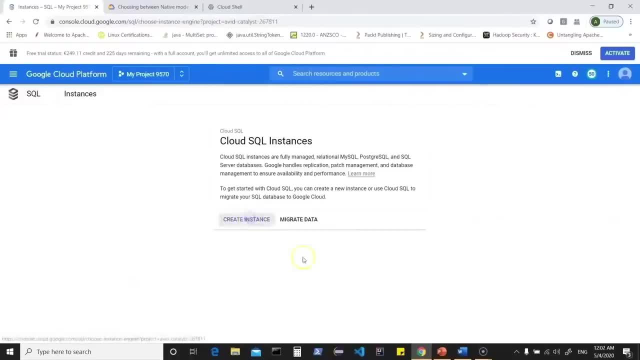 40,000 IOPS with huge amount of RAM per 40,000 IOPS with huge amount of RAM, per instance. so you can click on create instance. so you can click on create instance, so you can click on create instance here and then you can choose one. 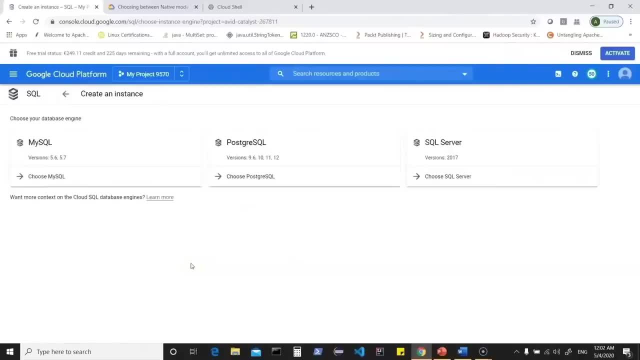 instance here, and then you can choose one instance here, and then you can choose one of the database which you would want, of the database which you would want, of the database which you would want to use. so cloud SQL is a managed service to use, so cloud SQL is a managed service. 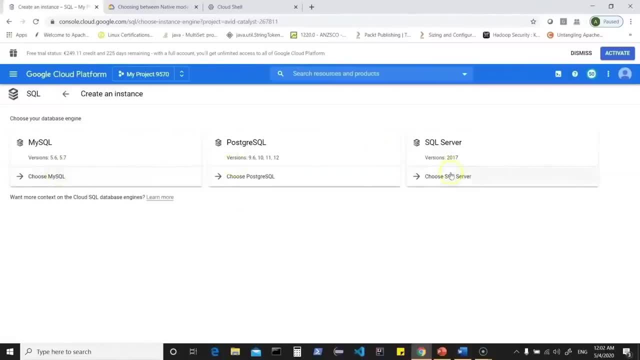 to use. so cloud SQL is a managed service. you can choose one of your MySQL, or you can choose one of your MySQL, or you can choose one of your MySQL or Postgres and SQL server. say, for example, Postgres and SQL server. say, for example, Postgres and SQL server. say, for example, I choose MySQL. now that basically tells: 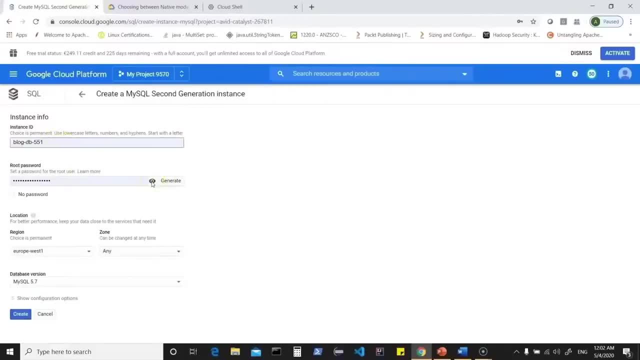 I choose MySQL now. that basically tells: I choose MySQL now. that basically tells me what is the instance ID. it sets up a me. what is the instance ID. it sets up a me. what is the instance ID. it sets up a password. you can always change the password. you can always change the. 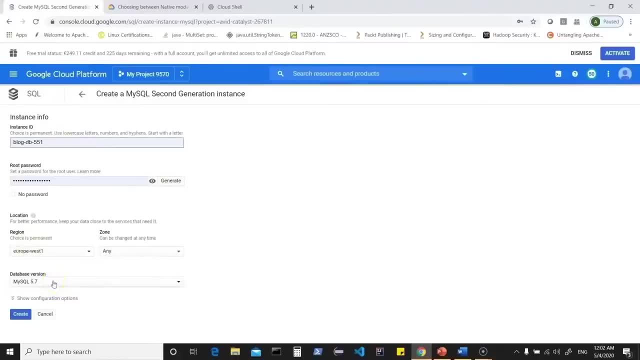 password. you can always change the password. you can change the region. you can password. you can change the region. you can change the region. you can choose your database version and then choose your database version, and then choose your database version, and then you can also look at other configuration. 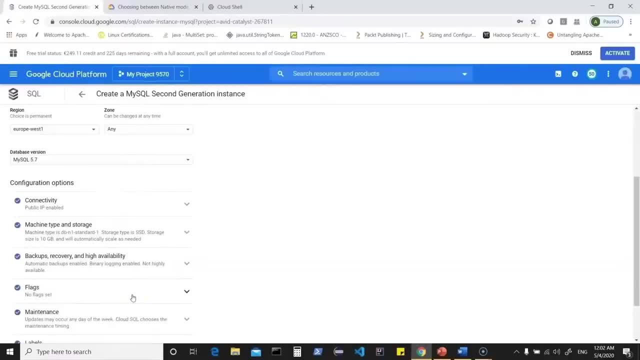 you can also look at other configuration. you can also look at other configuration options which talk about machine type options, which talk about machine type options, which talk about machine type which will be used. what is about your, which will be used? what is about your, which will be used? what is about your? backup and recovery, maintenance and all. 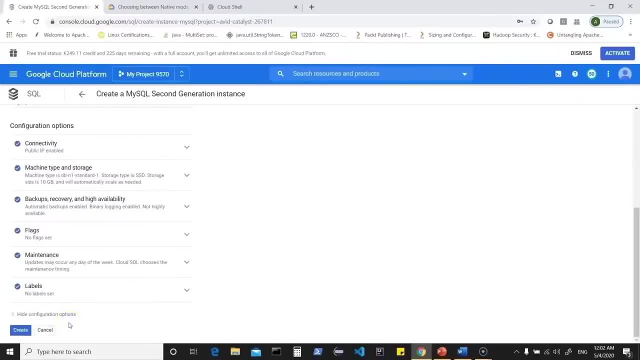 backup and recovery maintenance and all backup and recovery maintenance and all that. and if you click on create this, will that, and if you click on create this, will that, and if you click on create this, will basically create a fully managed SQL. basically create a fully managed SQL. 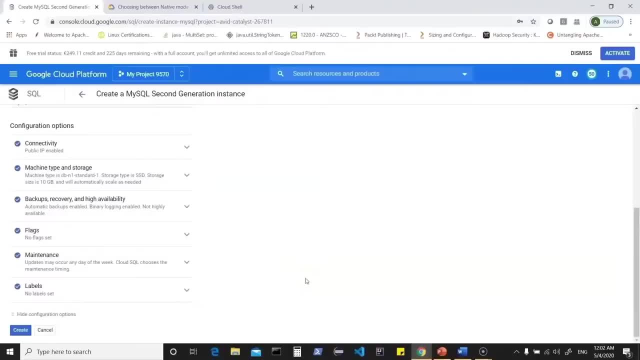 basically create a fully managed SQL service which can allow you to service, which can allow you to service, which can allow you to, straight away, start using MySQL on cloud. straight away, start using MySQL on cloud. straight away, start using MySQL on cloud, thus allowing you to store your 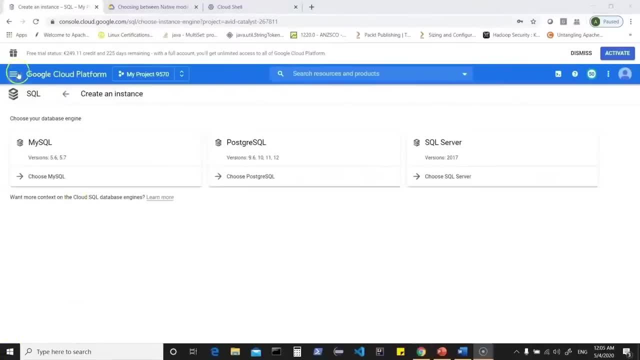 thus allowing you to store your, thus allowing you to store your relational data. when we talk about relational data, when we talk about relational data, when we talk about storage options, how can we not talk storage options? how can we not talk storage options? how can we not talk about a data warehouse solution, or? 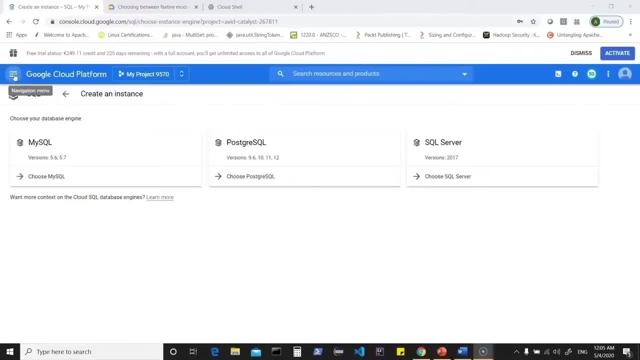 about a data warehouse solution, or about a data warehouse solution, or basically an option which allows you to, basically an option which allows you to, basically an option which allows you to run your queries by directly updating. run your queries by directly updating, run your queries by directly updating data, so you can use a data warehouse. 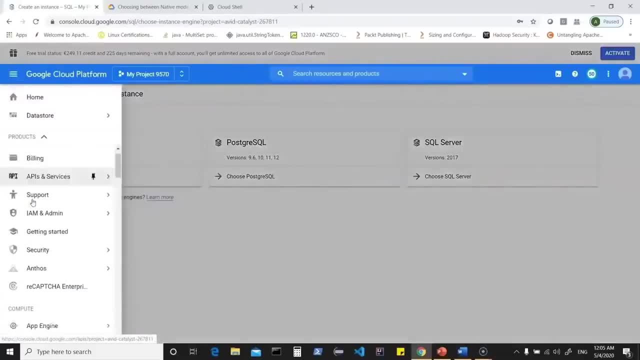 data so you can use a data warehouse data. so you can use a data warehouse service which Google Cloud Platform service, which Google Cloud Platform service, which Google Cloud Platform offers and that's called big query, so offers and that's called big query. so basically, you can be looking into the. 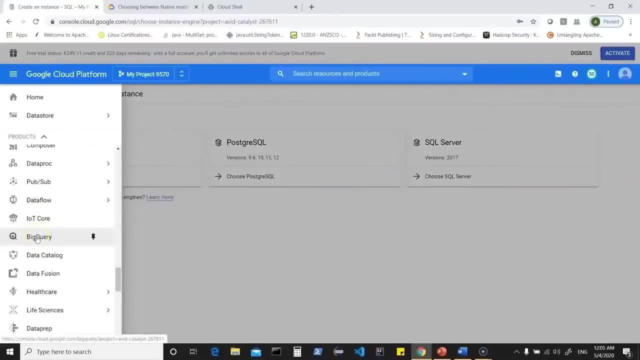 basically you can be looking into the. basically you can be looking into the big data section here and here you have big data section here and here you have big data section here and here you have an option called big query, so this: an option called big query, so this. 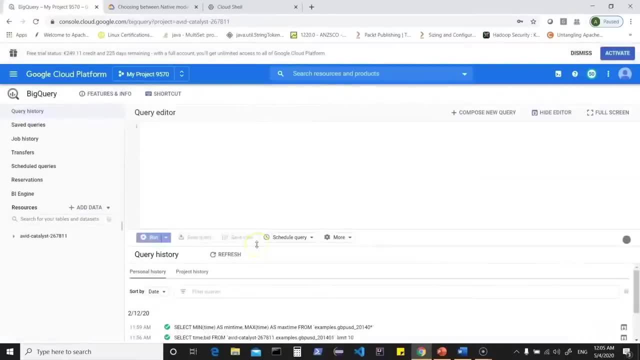 an option called big query. so this basically brings ease of implementation, basically brings ease of implementation, basically brings ease of implementation and speed. so building your own data and speed, so building your own data and speed, so building your own data warehouse- can be expensive time consuming. warehouse can be expensive, time consuming. 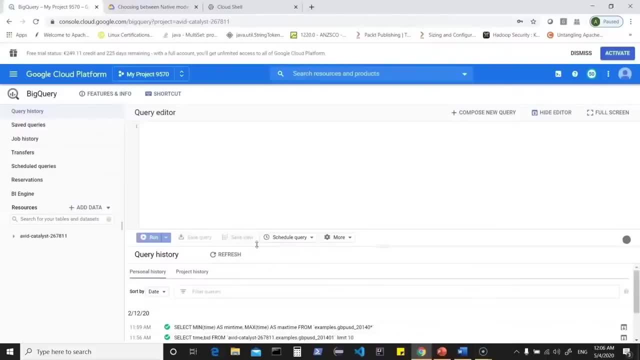 warehouse can be expensive, time consuming and difficult to scale. so with big query and difficult to scale. so with big query and difficult to scale. so with big query, you just load data and pay only for what. you just load data and pay only for what. you just load data and pay only for what you use. so it, when it comes to features, 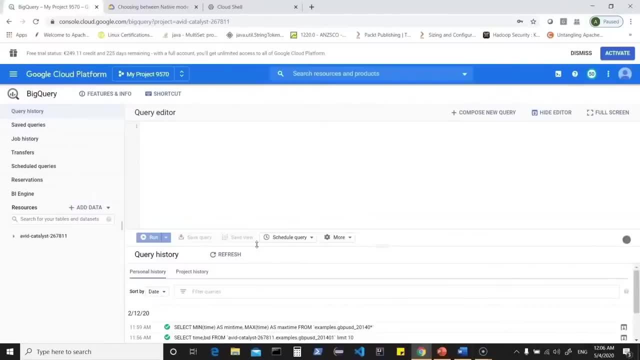 and if you would want to do real-time and if you would want to do real-time and if you would want to do real-time analysis of streaming data, that is also analysis of streaming data. that is also analysis of streaming data. that is also possible here. so here we have clicked on. 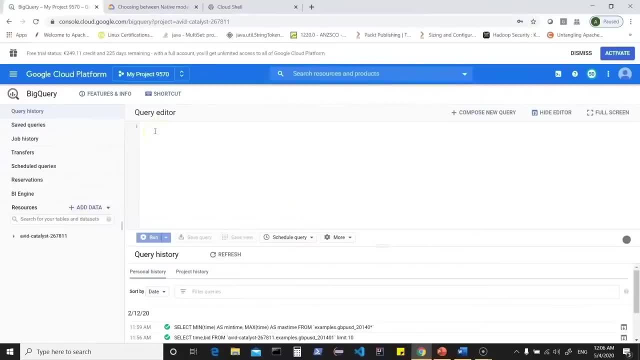 possible here. so here we have clicked on possible here. so here we have clicked on big query, which basically shows you the big query, which basically shows you the big query, which basically shows you the option where you can start typing your option where you can start typing your. 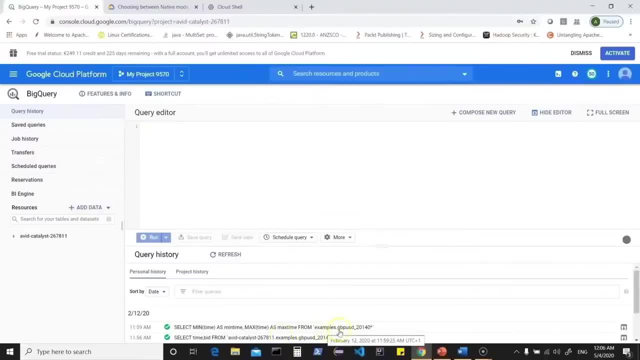 option where you can start typing your query and test your data access for query and test your data access for query and test your data access, for example, if I have uploaded some data. so example: if I have uploaded some data. so example: if I have uploaded some data. so it shows me there are some queries which 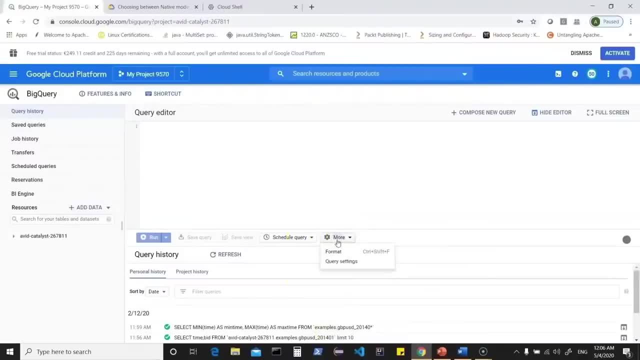 it shows me there are some queries which it shows me there are some queries which are saved here. now I can schedule. your are saved here. now I can schedule your are saved here. now I can schedule your query. I can basically choose the format query. I can basically choose the format. 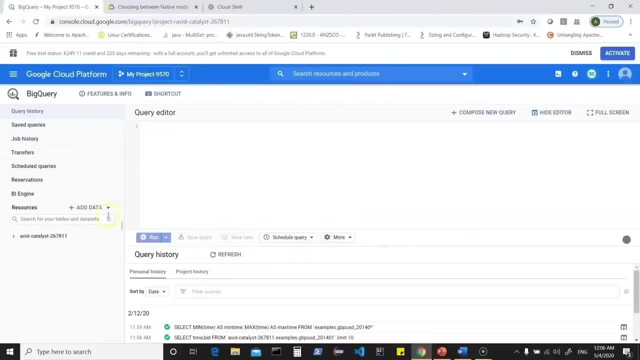 query. I can basically choose the format of a particular query by clicking on of a particular query. by clicking on of a particular query, by clicking on this more. here I have an option which this more. here I have an option which this more. here I have an option which says add data, so I can pin it to a. 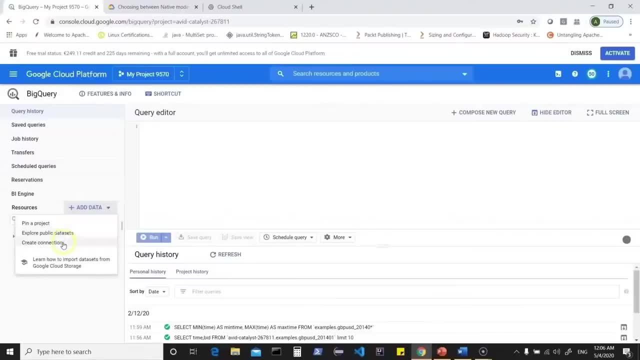 says add data so I can pin it to a says add data so I can pin it to a particular project. I can explore public particular project. I can explore public particular project. I can explore public data sets. I can create a connection so data sets. I can create a connection so. 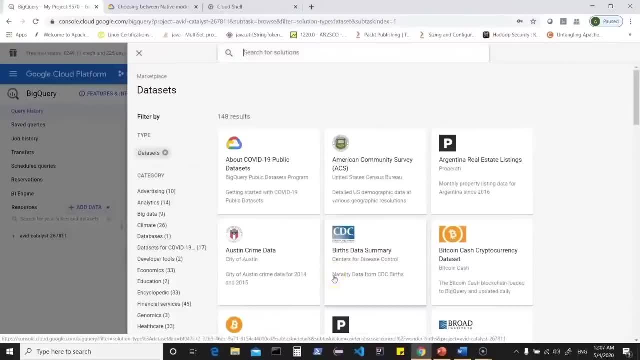 data sets. I can create a connection. so if I click on explore public data sets, if I click on explore public data sets, if I click on explore public data sets, then it takes me to a page from where. then it takes me to a page from where. then it takes me to a page from where you can get different kind of data sets. 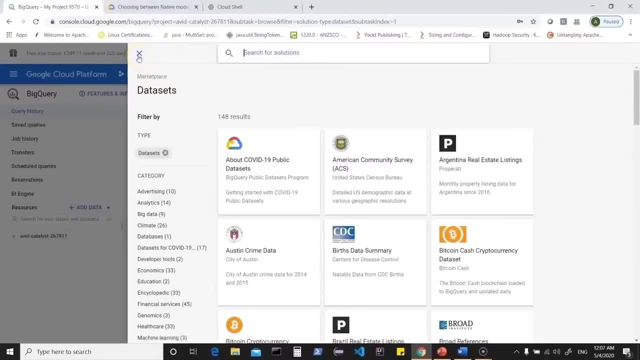 you can get different kind of data sets. you can get different kind of data sets: which are already available, which you which are already available, which you which are already available, which you can put into your big query and start can put into your big query and start can put into your big query and start querying your data. by default, it shows: 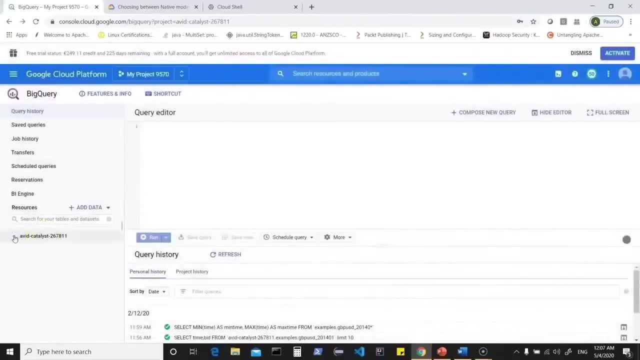 querying your data by default. it shows querying your data by default. it shows that it is aligned to my project and I that it is aligned to my project and I that it is aligned to my project and I don't need to worry about it. I can look. 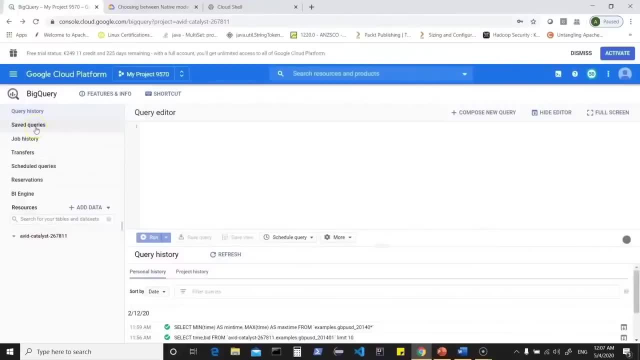 don't need to worry about it, I can look. don't need to worry about it. I can look at saved queries. if I have already saved queries, if I have already saved a particular query, I can look at job. saved a particular query, I can look at job. 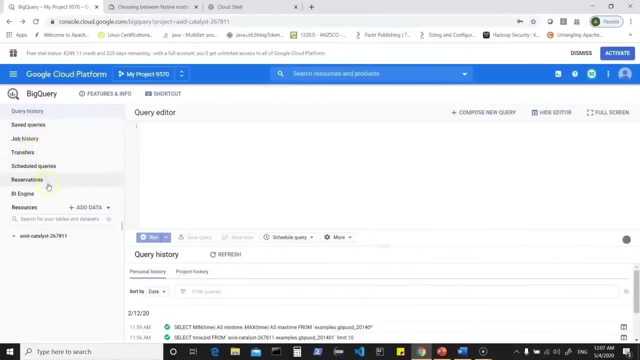 saved a particular query. I can look at job history. I can look at transfers history. I can look at transfers history. I can look at transfers, scheduled queries and reservations. so scheduled queries and reservations. so scheduled queries and reservations. so BigQuery basically initially had its own. BigQuery basically initially had its own. 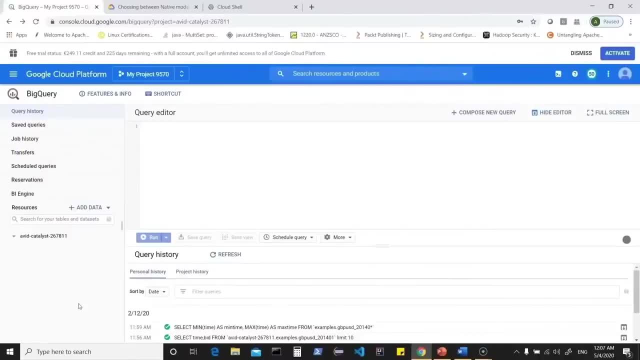 BigQuery basically initially had its own version of SQL, which was slightly version of SQL, which was slightly version of SQL, which was slightly different from standard SQL, but in 2016, different from standard SQL, but in 2016 different from standard SQL. but in 2016, BigQuery 2 was released that supports. 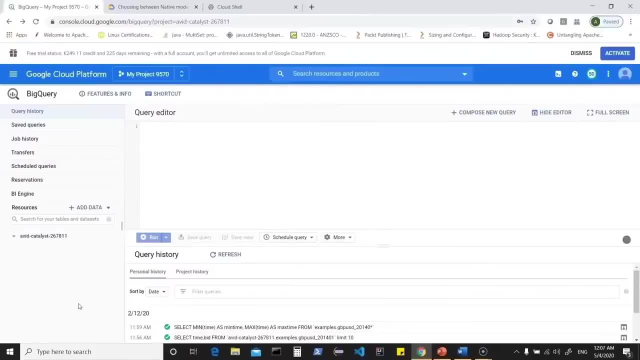 BigQuery 2 was released that supports BigQuery 2 was released that supports SQL 2011 standard. you can always select SQL 2011 standard. you can always select SQL 2011 standard. you can always select standard SQL. now BigQuery when it comes. 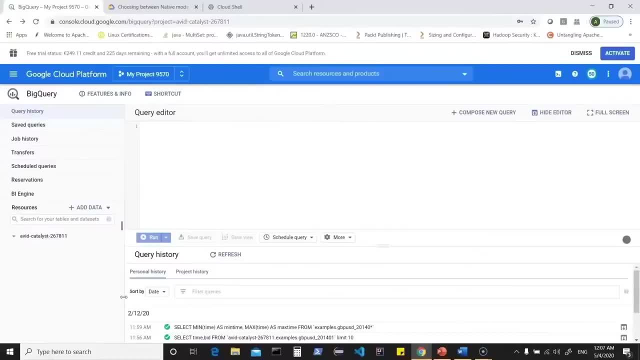 standard SQL, now BigQuery when it comes. standard SQL, now BigQuery. when it comes to pricing, we need to remember that the to pricing. we need to remember that the to pricing. we need to remember that the storage is where the storage costs is. storage is where the storage costs is. 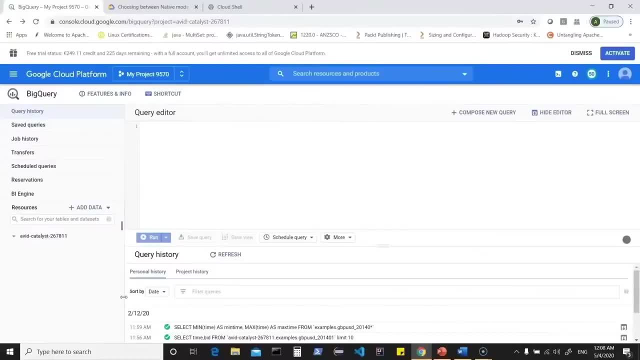 storage is where the storage costs is very less. here, approximately 0.02 cents. very less here, approximately 0.02 cents. very less here, approximately 0.02 cents per GB per month. it is almost similar to per GB per month. it is almost similar to. 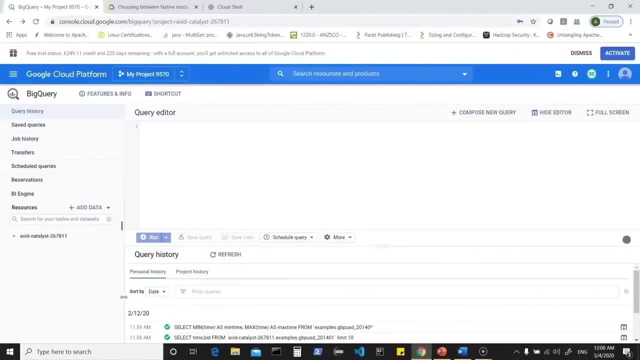 per GB per month. it is almost similar to nearline, where you can also have low nearline, where you can also have low nearline, where you can also have low cost, that is, 0.01 cents per gigabyte per cost. that is, 0.01 cents per gigabyte per. 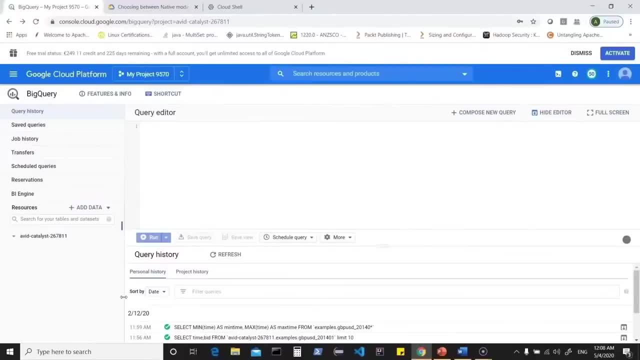 cost, that is, 0.01 cents per gigabyte per month. there is no charge for reading month. there is no charge for reading month. there is no charge for reading data from storage, when it comes to data from storage, when it comes to data from storage, when it comes to querying, and that's where the cost is. 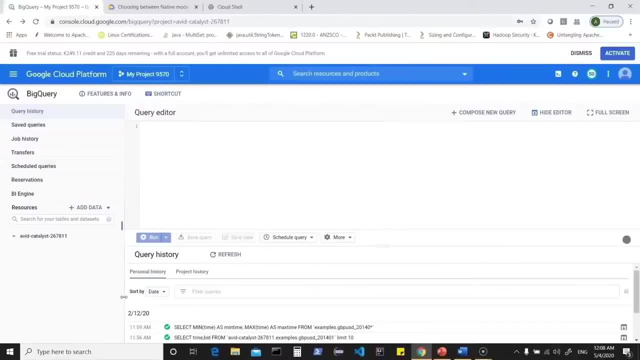 querying and that's where the cost is querying and that's where the cost is incurred. so 1 terabyte per month is free incurred. so 1 terabyte per month is free incurred. so 1 terabyte per month is free and after that it costs few cents per. 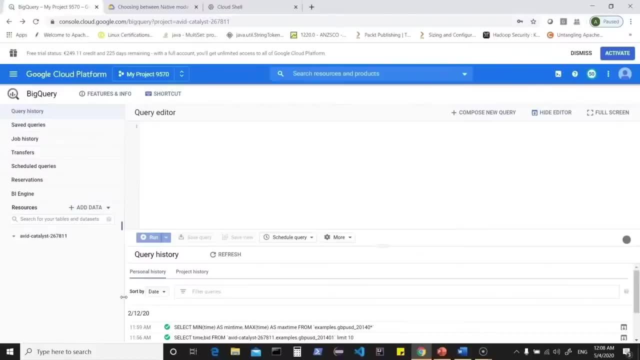 and after that it costs few cents per and after that it costs few cents per gigabyte. so this is mainly for high gigabyte. so this is mainly for high gigabyte. so this is mainly for high volume customers. there is a flat rate by volume customers. there is a flat rate by. 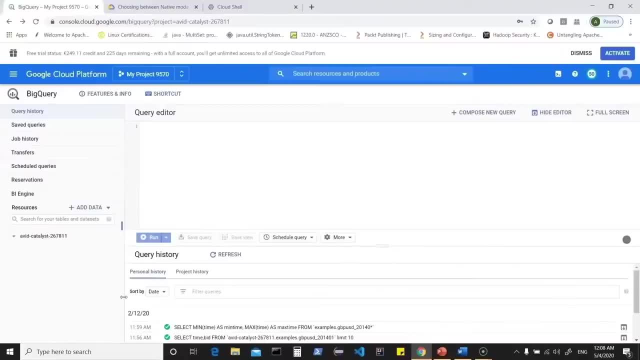 volume customers. there is a flat rate by pricing which can be used. so when you pricing which can be used, so when you pricing which can be used, so when you talk about querying, you can save your talk about querying. you can save your talk about querying. you can save your query results. you can create data set to: 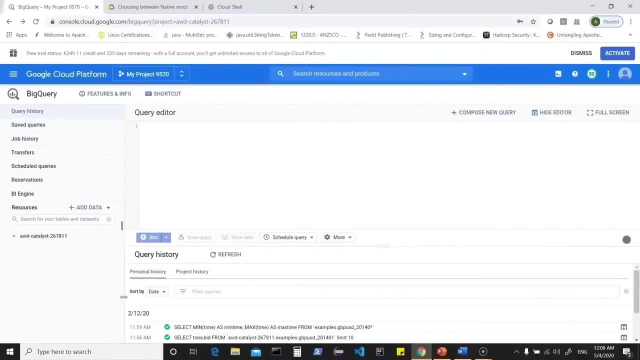 query results. you can create data set to query results. you can create data set to store the results. now. results are put in store. the results now. results are put in store. the results now. results are put in a temp table in cache and after you are. a temp table in cache and after you are. 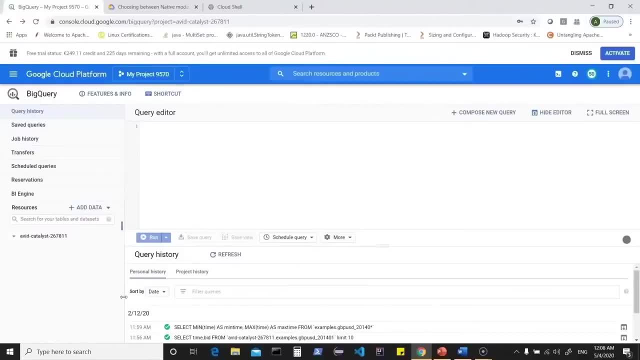 a temp table in cache and after you are done with that, you can delete data set. done with that, you can delete data set. done with that, you can delete data set and delete all the data. so when you talk and delete all the data. so when you talk. 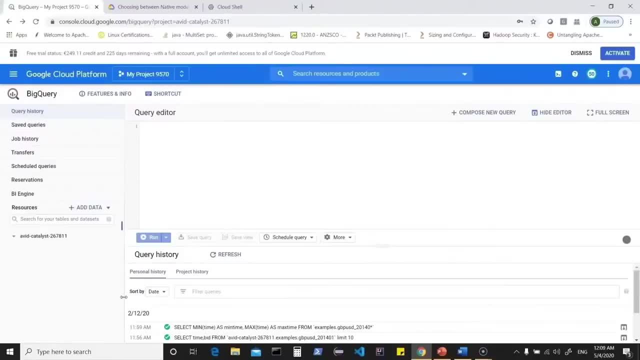 and delete all the data. so, when you talk about loading data into BigQuery, you can about loading data into BigQuery. you can about loading data into BigQuery. you can get the data from cloud storage. Google get the data from cloud storage. Google get the data from cloud storage. Google Drive cloud data store stack driver. 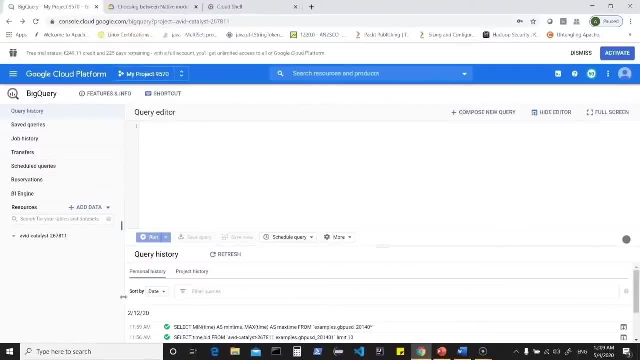 drive cloud data store stack driver. drive cloud data store stack driver- stack driver- other options. you have cloud stack driver other options? you have cloud stack driver other options? you have cloud bigtable or other web interfaces so you bigtable or other web interfaces. so you bigtable or other web interfaces so you can download from URL such as CSV JSON. 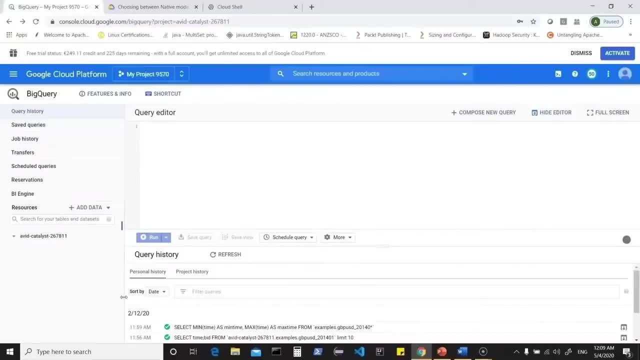 can download from URL such as CSV JSON. can download from URL such as CSV JSON. Avro: you can create data set. create Avro. you can create data set. create Avro. you can create data set, create table and create from source by doing a table and create from source by doing a. 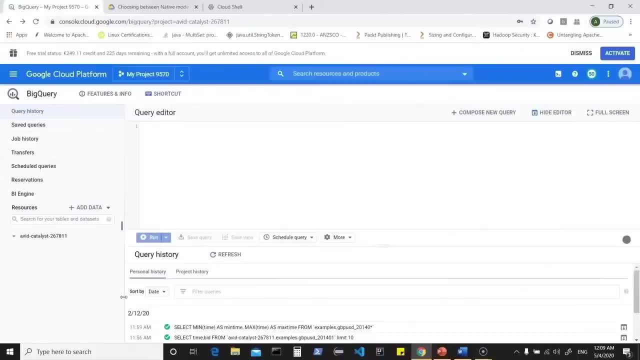 table and create from source by doing a file upload, so 10 megabyte or less files. file upload, so 10 megabyte or less files. file upload, so 10 megabyte or less. files can be uploaded using web interface as an can be uploaded using web interface as an. 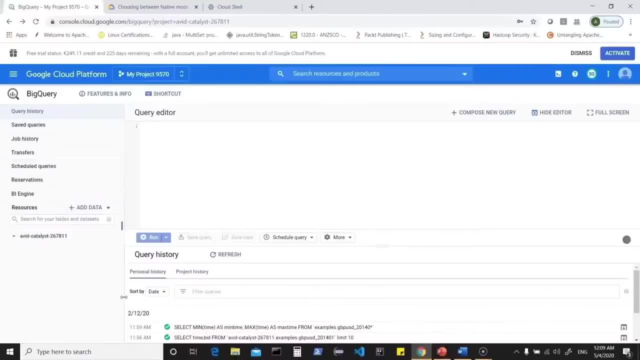 can be uploaded using web interface as an option. you can also use command line option. you can also use command line option. you can also use command line, and then you can start working with your, and then you can start working with your, and then you can start working with your big query. so here you can also work with. 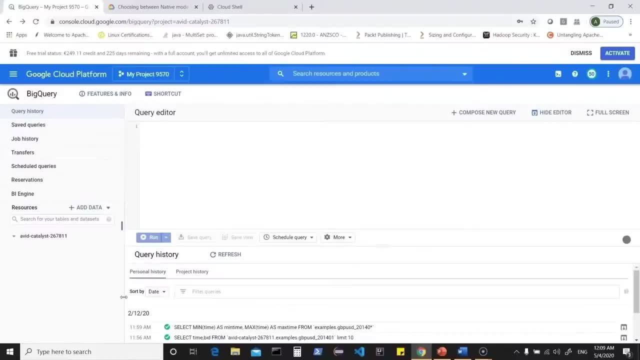 big query. so here you can also work with big query. so here you can also work with streaming data by basically pushing in streaming data, by basically pushing in streaming data, by basically pushing in streaming data into your big query, which streaming data into your big query, which streaming data into your big query which allows you to add one record at a time. 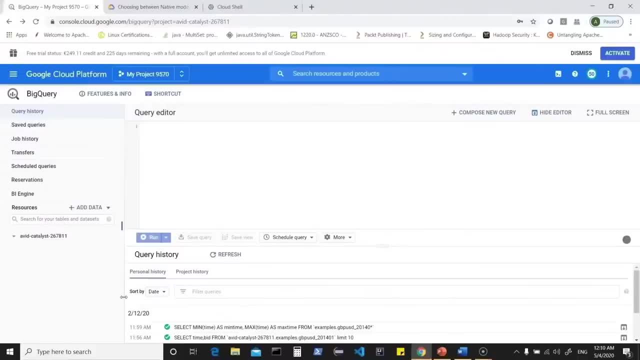 allows you to add one record at a time. allows you to add one record at a time. now you could use something like cloud. now you could use something like cloud. now you could use something like cloud data flow, which allows you to use a data flow which allows you to use a. 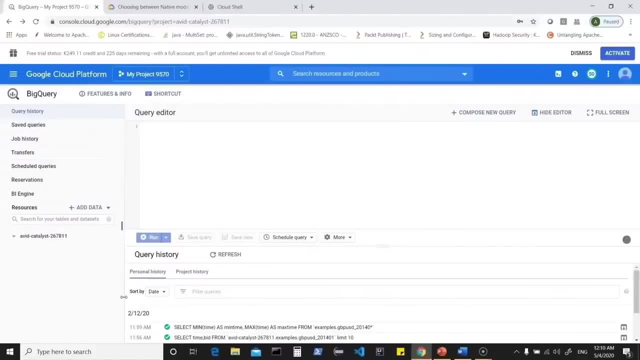 data flow which allows you to use a particular pipeline about cloud data flow, particular pipeline about cloud data flow, particular pipeline about cloud data flow. we will learn later so you can benefit. we will learn later so you can benefit. we will learn later so you can benefit from different features of big query and 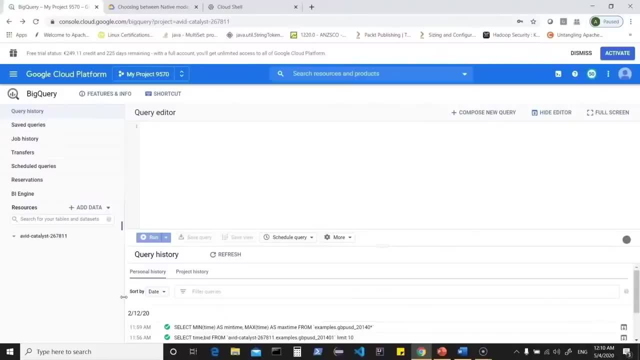 from different features of big query and from different features of big query and thus use Google's offering to work on. thus use Google's offering to work on. thus use Google's offering to work on your structured data, or I would say data, your structured data, or I would say data. 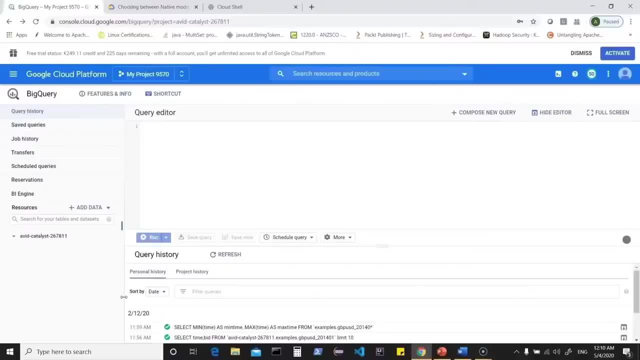 your structured data, or I would say data which suits well in data warehouses now, which suits well in data warehouses now, which suits well in data warehouses now. these are some of the storage related. these are some of the storage related. these are some of the storage related services which Google Cloud offers. 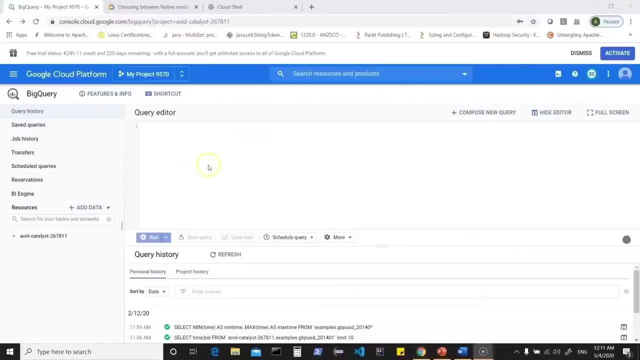 services which Google Cloud offers. services which Google Cloud offers, although we will learn about using big. although we will learn about using big. although we will learn about using big query and running or uploading some data query and running or uploading some data by creating add data set here by say: 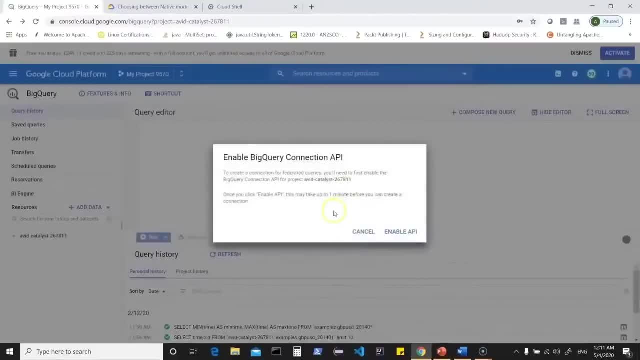 by creating add data set here, by, say, by creating add data set here, by, say, creating connection or using a public creating connection or using a public creating connection or using a public data set. so as of now, I have this you data set. so as of now, I have this you. 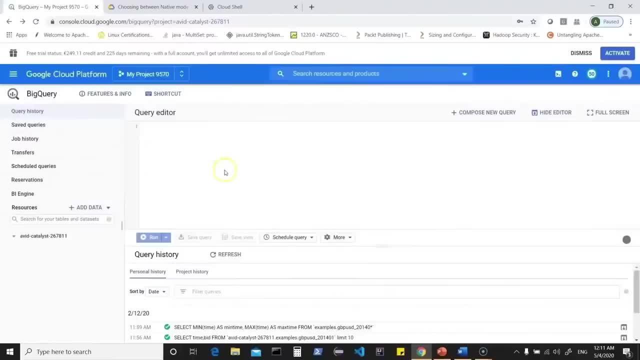 data set. so as of now I have this, you can also access the command line to work. can also access the command line to work. can also access the command line to work with this. but we will learn in detail with this. but we will learn in detail with this. but we will learn in detail about big query in later sessions. now, 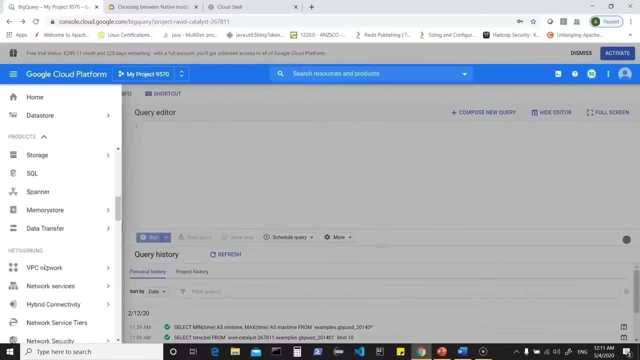 about big query in later sessions. now about big query in later sessions. now, here you can scroll down and you also here you can scroll down and you also here you can scroll down and you also have an option within big data space and have an option within big data space and 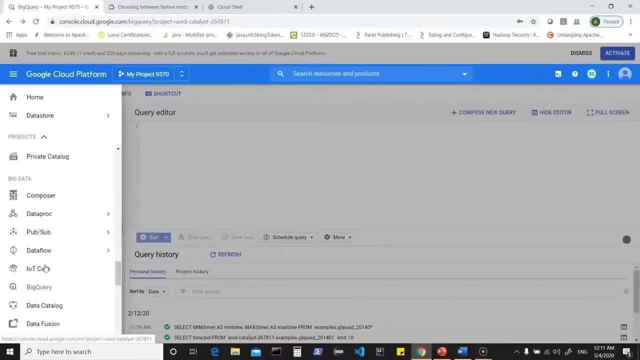 have an option within big data space and that is your data proc. so when you talk, that is your data proc. so when you talk, that is your data proc. so when you talk about data proc, this is again a managed- about data proc, this is again a managed. 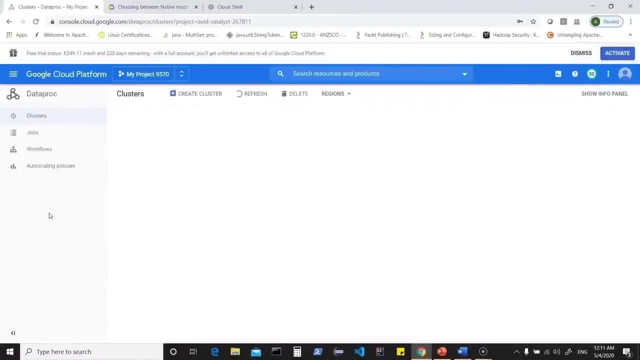 about data proc. this is again a managed service which allows you to run spark, or service which allows you to run spark, or service which allows you to run spark or Hadoop jobs. so especially if you are Hadoop jobs, so especially if you are Hadoop jobs, so especially if you are interested in big data workload. so for 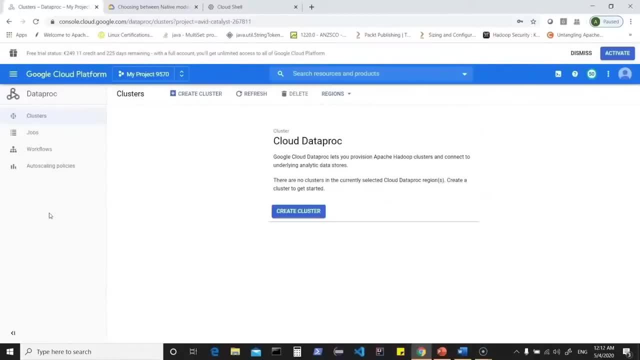 interested in big data workload. so for interested in big data workload, so for big data processing for machine learning, big data processing for machine learning, big data processing for machine learning, you can always use cloud data proc. this, you can always use cloud data proc. this, you can always use cloud data proc. this uses compute engine instances under the 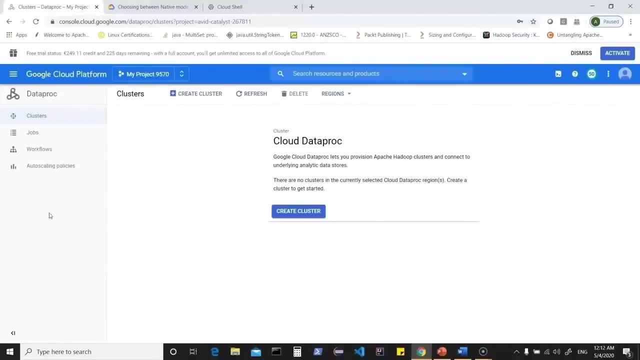 uses compute engine instances under the. uses compute engine instances under the hood, but takes care of management of hood, but takes care of management of hood, but takes care of management of these instances. so it's a, it's a layer on these instances. so it's a, it's a layer on. 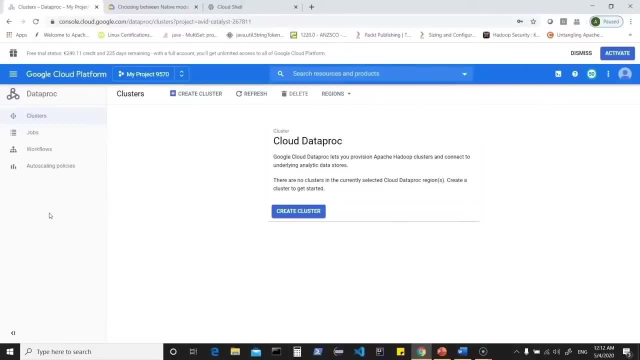 these instances. so it's a. it's a layer on top to spin up clusters. it's a managed top to spin up clusters. it's a managed top to spin up clusters. it's a managed service. it's cheaper pay when the jobs service. it's cheaper pay when the jobs. 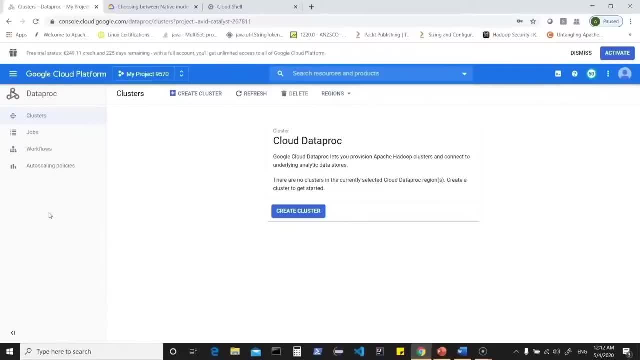 service. it's cheaper pay when the jobs are running. only it's fast because it is are running. only it's fast because it is are running. only it's fast because it is integrated with other Google cloud. integrated with other Google cloud, integrated with other Google cloud services. you have open source components. 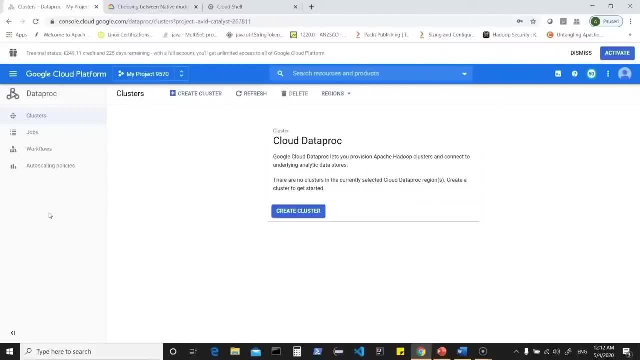 services. you have open source components services. you have open source components pre-installed and data proc is pre-installed and data proc is pre-installed and data proc is integrated with yarn to make cluster integrated with yarn. to make cluster integrated with yarn. to make cluster management easier. when you talk about 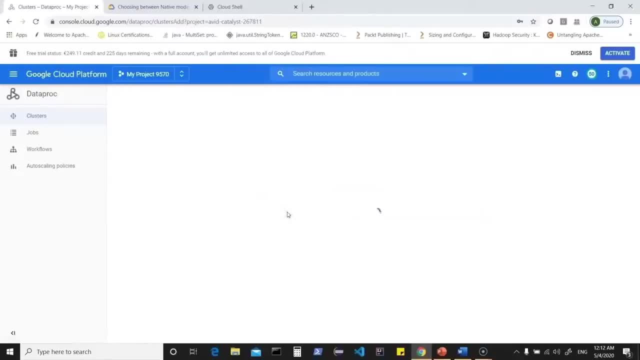 management easier when you talk about management easier when you talk about data proc. you can click on create data proc. you can click on create data proc, you can click on create cluster, and that basically allows you to cluster and that basically allows you to cluster and that basically allows you to set up your cluster by choosing a. 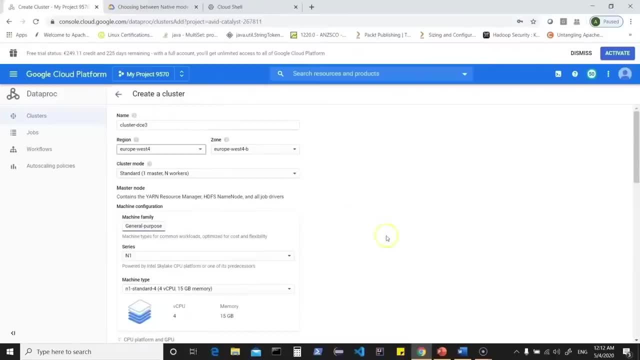 set up your cluster by choosing a. set up your cluster by choosing a particular region which you would want to, particular region which you would want to, particular region which you would want to use. for example, I'll choose Europe use. for example, I'll choose Europe use. for example, I'll choose Europe West, for here it tells what kind of 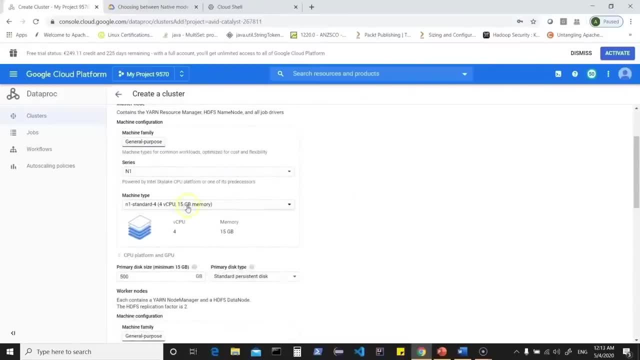 West for here it tells what kind of West for here. it tells what kind of machines you would want to use and by machines you would want to use and by machines you would want to use. and by default it has populated as the machine. default it has populated as the machine. 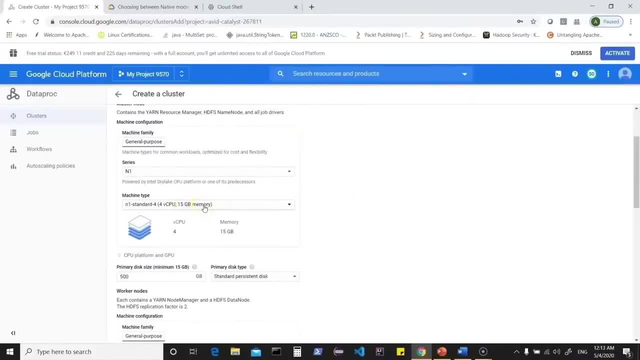 default, it has populated as the machine: here, which is for CPU, and 15 gigabyte, here, which is for CPU and 15 gigabyte, here, which is for CPU and 15 gigabyte. now, since you might be using a free, now, since you might be using a free, 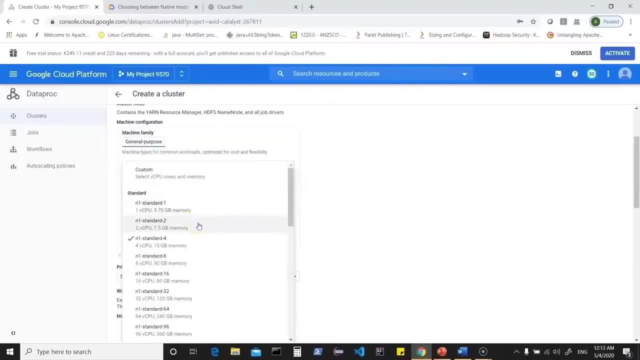 now, since you might be using a free account, let's not go for the high-end account. let's not go for the high-end account. let's not go for the high-end machine. let's go for n1, standard 2 and machine. let's go for n1, standard 2, and. 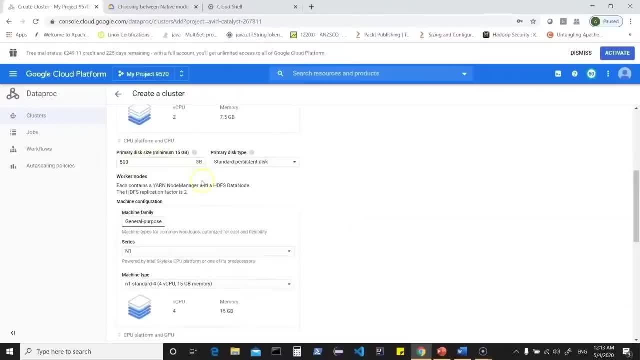 machine. let's go for n1, standard 2, and then you can scroll down. it says what is. then you can scroll down. it says what is. then you can scroll down. it says what is the primary disk, what is the disk type, the primary disk, what is the disk type. 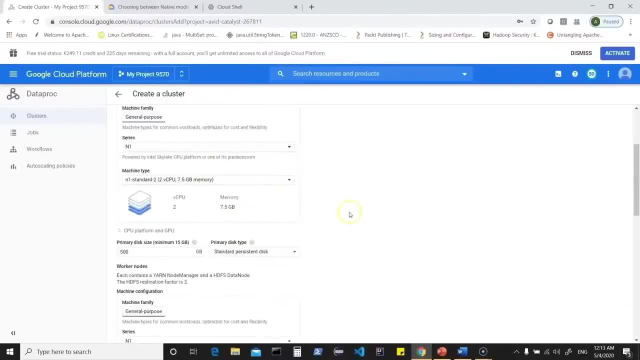 the primary disk. what is the disk type? and this one was for your master machine, and this one was for your master machine. and this one was for your master machine. that is machine which will have the. that is machine which will have the. that is machine which will have the master processes running. then you have 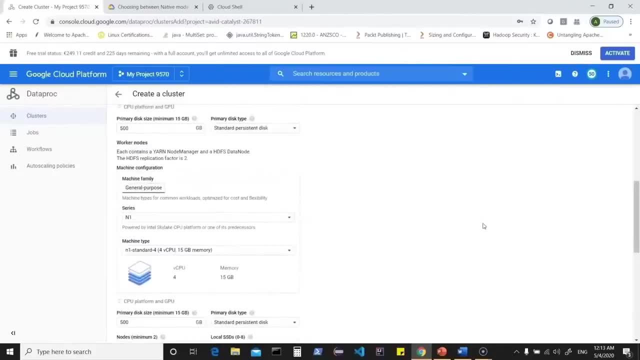 master processes running. then you have master processes running. then you have your worker node configuration, which your worker node configuration, which your worker node configuration, which tells this will be: let's choose a lower. tells this will be: let's choose a lower. tells this will be: let's choose a lower and machine, and we can choose how many. 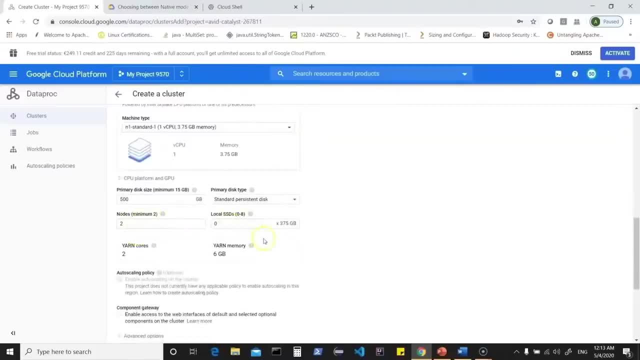 and machine and we can choose how many. and machine and we can choose how many worker nodes you would have. so it says worker nodes you would have. so it says worker nodes you would have. so it says minimum two. you can choose the SSDs and minimum two. you can choose the SSDs and. 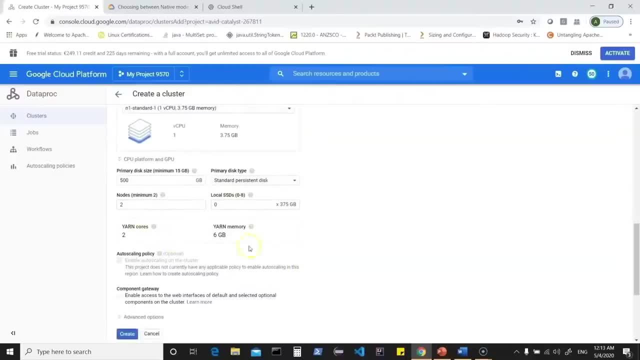 minimum two. you can choose the SSDs and their capacity. it talks about yarn, their capacity. it talks about yarn, their capacity. it talks about yarn cores and yarn memory, which will be cores, and yarn memory, which will be cores, and yarn memory which will be allocated. and here we have then option. 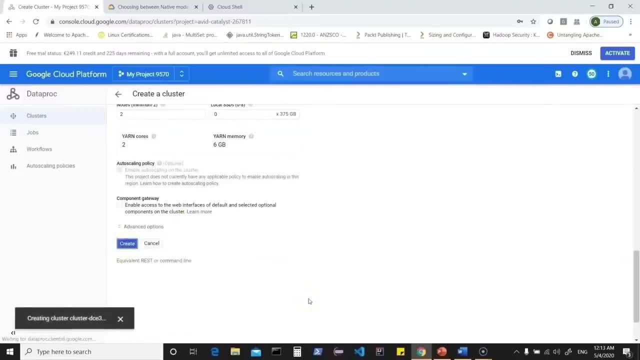 allocated, and here we have then option allocated, and here we have then option of clicking on create. so once you click of clicking on create, so once you click of clicking on create, so once you click on create, this will basically spin up a. on create, this will basically spin up a. 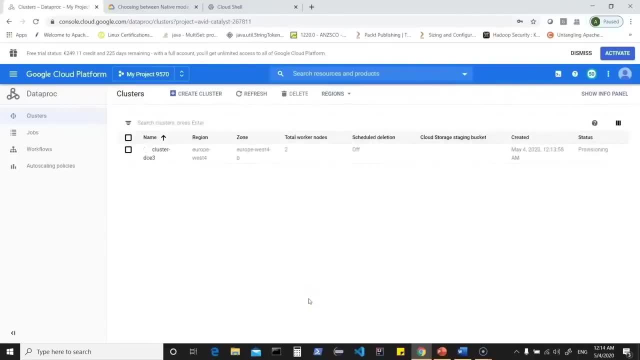 on create. this will basically spin up a cluster wherein you can straight away cluster, wherein you can straight away cluster, wherein you can straight away start submitting jobs to this. you can start submitting jobs to this. you can start submitting jobs to this. you can basically go ahead once your cluster is. 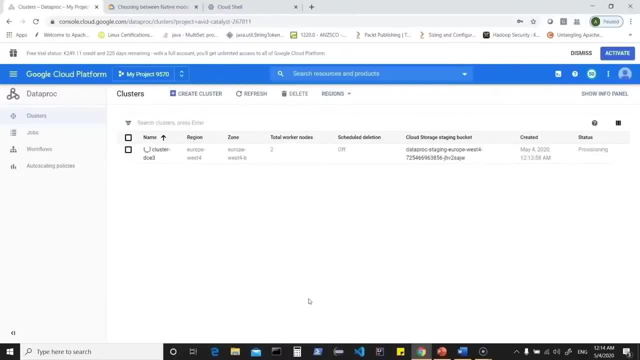 basically go ahead once your cluster is basically go ahead. once your cluster is ready, you can go into the cluster. you ready, you can go into the cluster. you can submit a job. you can choose a type. can submit a job. you can choose a type. can submit a job. you can choose a type which is spark or any other application. 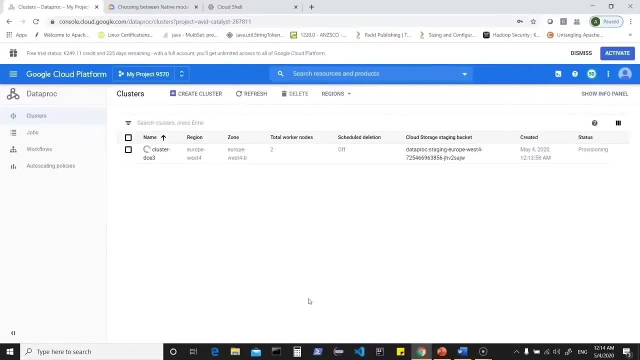 which is spark or any other application which is spark or any other application which you would want to run, and then which you would want to run, and then which you would want to run, and then, basically, you can use this fully managed. basically, you can use this fully managed. 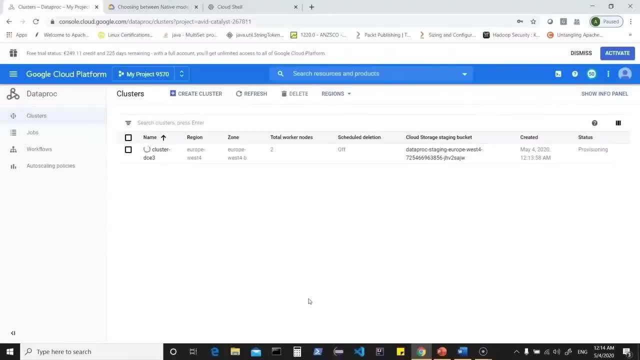 basically, you can use this fully managed service which allows you to run your big service, which allows you to run your big service, which allows you to run your big data clusters. you can obviously control data clusters. you can obviously control data clusters. you can obviously control access via roles or access control list. 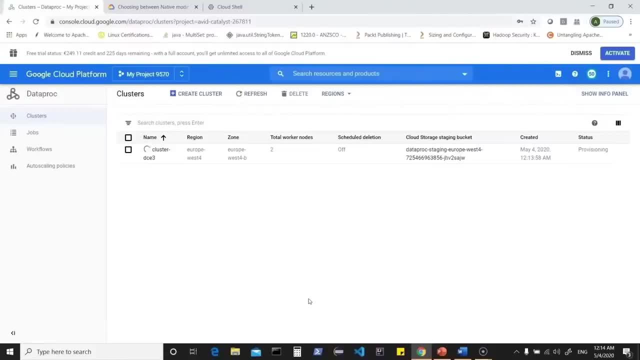 access via roles or access control list. access via roles or access control list. and you can have access as it is at. and you can have access as it is at. and you can have access as it is at project level or based on your Dataproc: project level or based on your Dataproc. 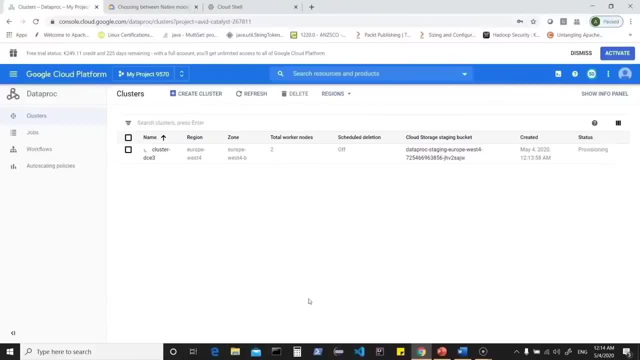 project level or based on your Dataproc cluster or even at your worker notes. so cluster, or even at your worker notes, so cluster, or even at your worker notes. so we'll learn about Dataproc in later. we'll learn about Dataproc in later. 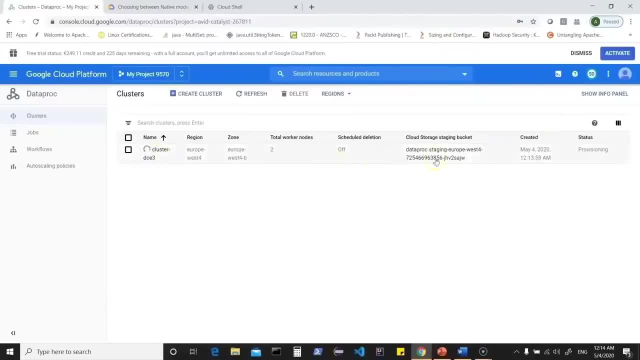 we'll learn about Dataproc in later sessions. so as of now, you see here the sessions. so as of now, you see here the sessions. so as of now you see here the cluster is getting created. it says the cluster is getting created. it says the cluster is getting created. it says the cloud storage bucket which it is using. 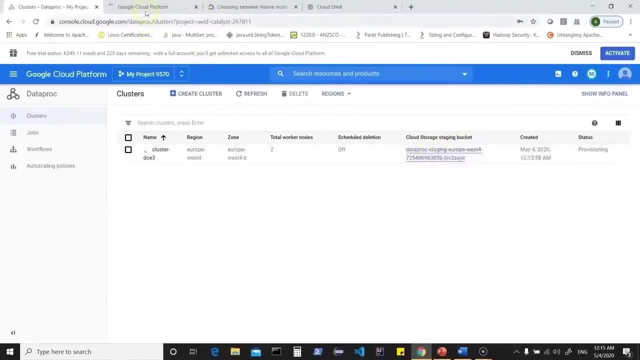 cloud storage bucket which it is using. cloud storage bucket which it is using. is this one now I can click on this? and is this one now I can click on this? and is this one now I can click on this and open link in a new tab? it still takes me. 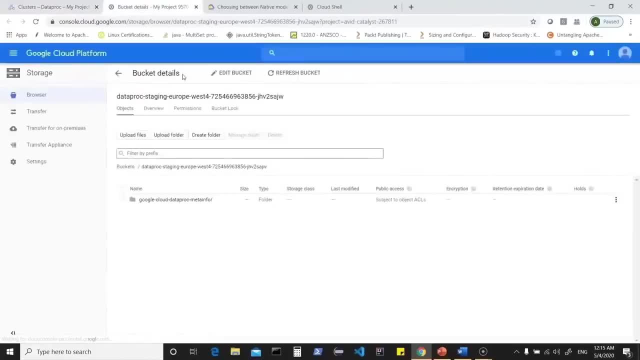 open link in a new tab. it still takes me open link in a new tab. it still takes me into console, but now it is showing me into console. but now it is showing me into console. but now it is showing me the bucket which is being used by your. 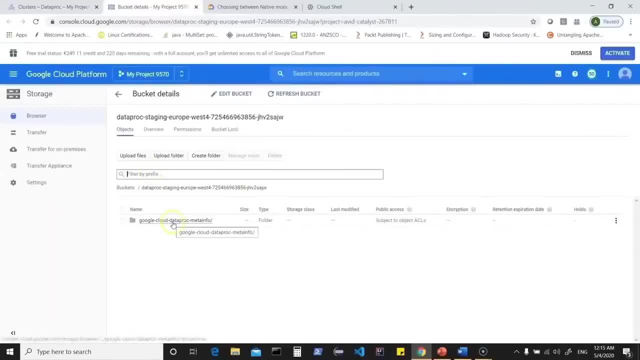 the bucket which is being used by your, the bucket which is being used by your Dataproc cluster. this is the bucket Dataproc cluster. this is the bucket Dataproc cluster. this is the bucket which is being used and it is being used, which is being used and it is being used. 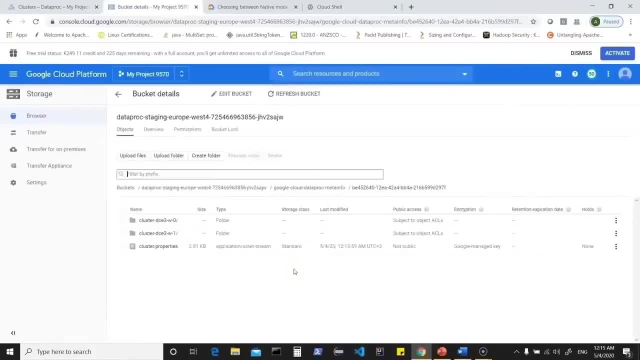 which is being used, and it is being used for an underlying metadata which gets for an underlying metadata which gets for an underlying metadata which gets stored here. so you look at the cluster stored here. so you look at the cluster stored here. so you look at the cluster related folders. you can click in these. 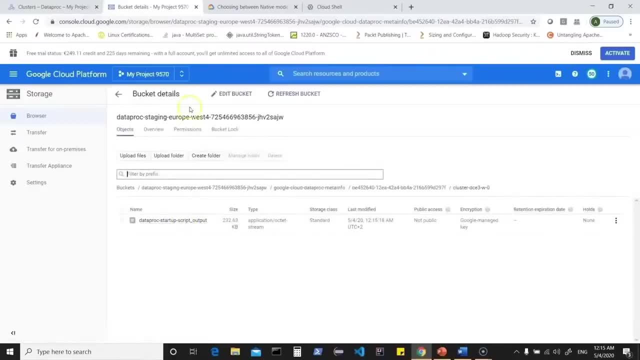 related folders. you can click in these related folders. you can click in these folders and then it can see what is the folders, and then it can see what is the folders, and then it can see what is the script output, what it is doing, and so on. script output, what it is doing, and so on. 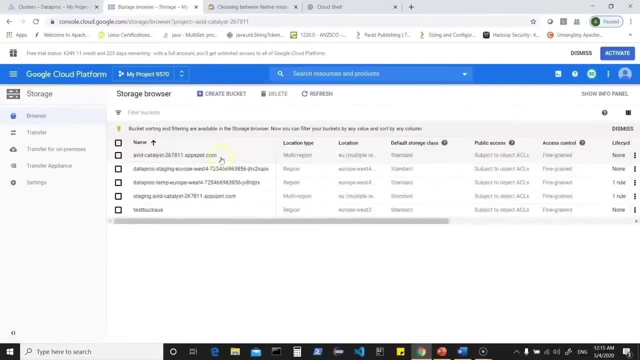 script, output what it is doing, and so on. now I can come back here to my bucket. now I can come back here to my bucket. now I can come back here to my bucket, which will basically show me what kind of, which will basically show me what kind of. 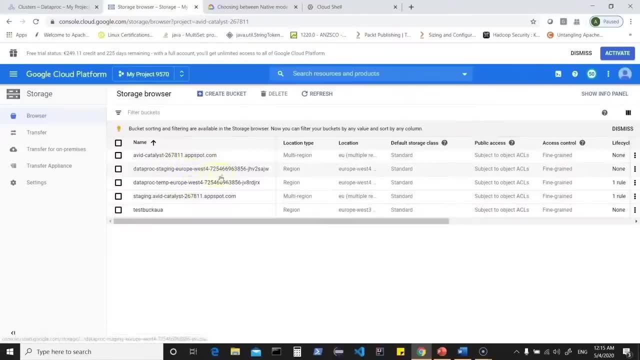 which will basically show me what kind of buckets have been created. so you see buckets have been created. so you see buckets have been created. so you see Dataproc service automatically created Dataproc service automatically created. Dataproc service automatically created some buckets which will be holding some. 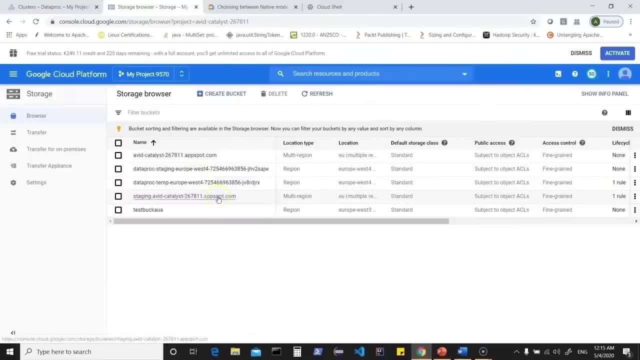 some buckets which will be holding some some buckets which will be holding some data. you also have some other buckets data. you also have some other buckets data. you also have some other buckets which were created based on other, which were created based on other, which were created based on other services which we used the access. 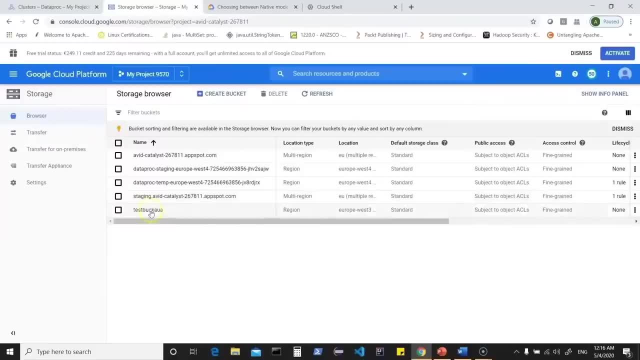 services which we used, the access services which we used, the access control is fine-grained in all cases. control is fine-grained in all cases. control is fine-grained in all cases. plus it also shows our bucket, so plus it also shows our bucket, so plus it also shows our bucket, so underlying it is using compute instances. 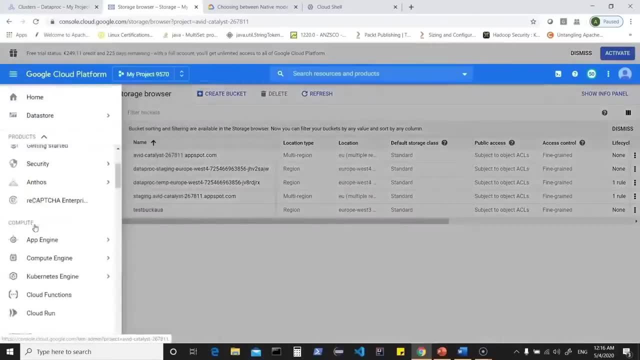 underlying it is using compute instances. underlying it is using compute instances. it is basically using: let's go here. and it is basically using: let's go here. and it is basically using: let's go here and let's go to compute engine and let's, let's go to compute engine and let's. 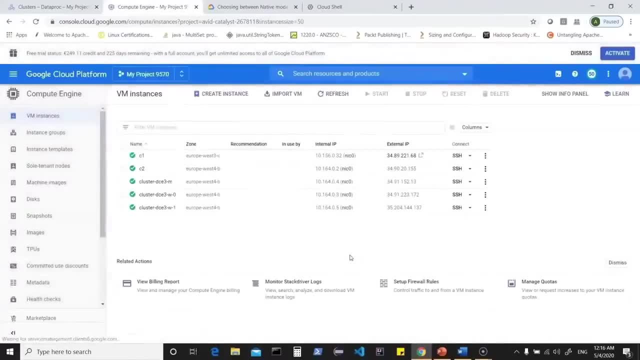 let's go to compute engine and let's look into VM instances. so Dataproc, which look into VM instances, so Dataproc, which look into VM instances, so Dataproc, which is a cluster ready to use, so you can, is a cluster ready to use, so you can. 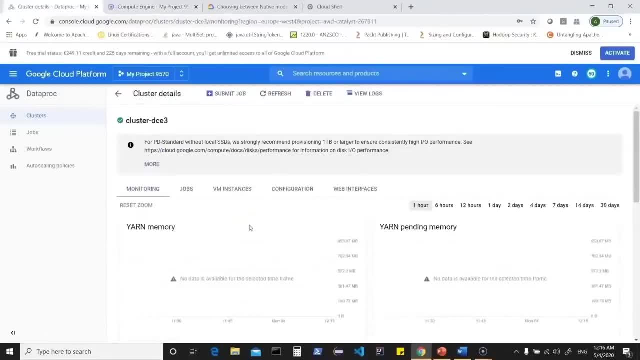 is a cluster ready to use so you can click on this cluster and that shows me: click on this cluster. and that shows me: click on this cluster and that shows me my cluster related details. if there are my cluster related details. if there are my cluster related details. if there are any jobs running. what are VM instances? 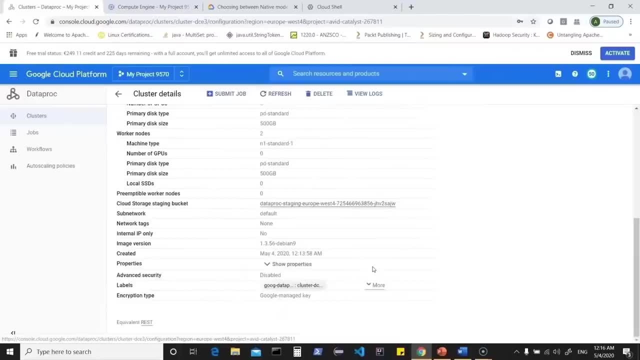 any jobs running. what are VM instances? any jobs running, what are VM instances? what kind of configurations it has used, what kind of configurations it has used, what kind of configurations it has used and you can look at different details. and you can look at different details and you can look at different details here. you can look at the logs. you can. 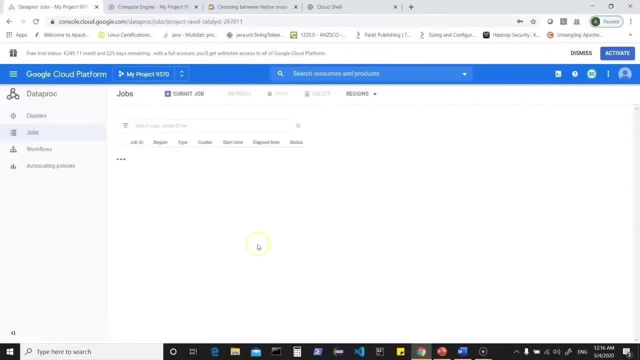 here you can look at the logs. you can- here you can look at the logs. you can click on jobs and that will show you if click on jobs and that will show you if click on jobs and that will show you if you have basically run a job on this. 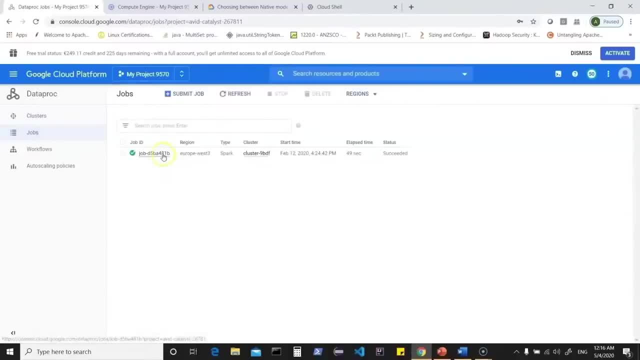 you have basically run a job on this. you have basically run a job on this ready-to-use cluster. so it says there is ready-to-use cluster. so it says there is ready-to-use cluster. so it says there is this particular job which was run, which, this particular job which was run, which. 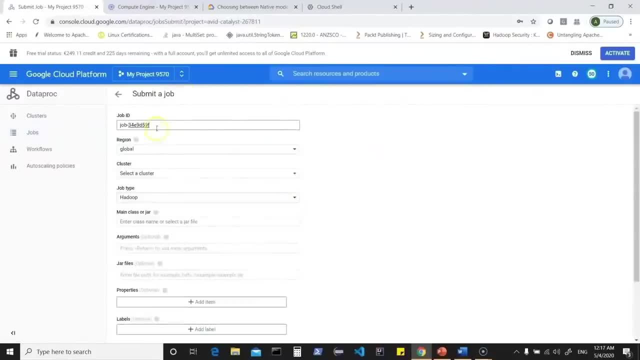 this particular job, which was run, which was a spark job. you can click on submit- was a spark job. you can click on submit, was a spark job. you can click on submit and this one tells you what is the job. and this one tells you what is the job. 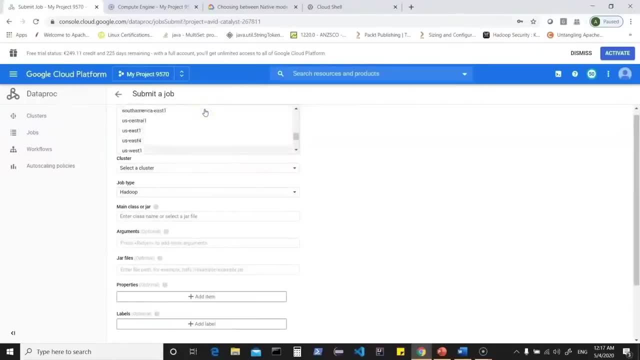 and this one tells you what is the job: ID. what is the region you would choose? ID. what is the region you would choose? ID. what is the region you would choose, for example, we will again choose for, for example, we will again choose for, for example, we will again choose, for example, Europe West, for it tells what is. 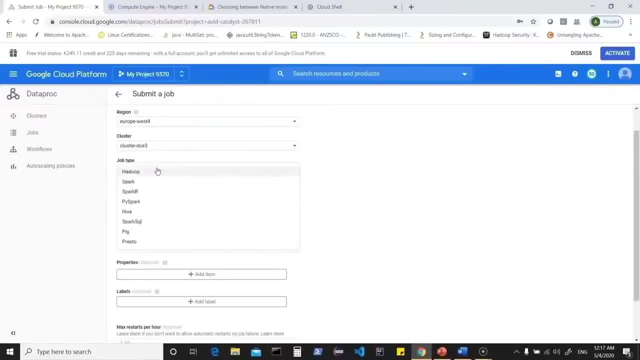 example Europe West, for it tells what is example Europe West, for it tells what is the job type so you can run all these the job type. so you can run all these the job type, so you can run all these type of jobs in this cluster, such as: 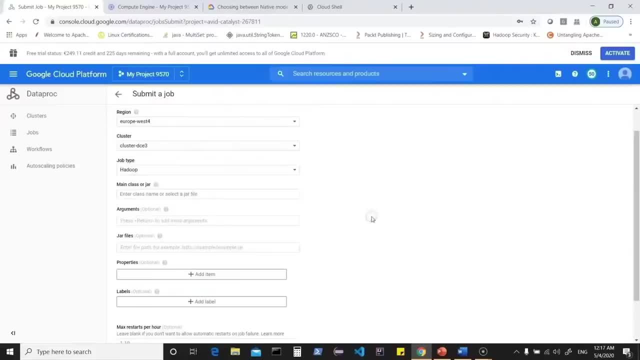 type of jobs in this cluster. such as type of jobs in this cluster such as: Hadoop spark by spark hive pig presto you. Hadoop spark by spark hive pig presto you. Hadoop spark by spark hive pig presto. you can give your jar file. so, if you have, 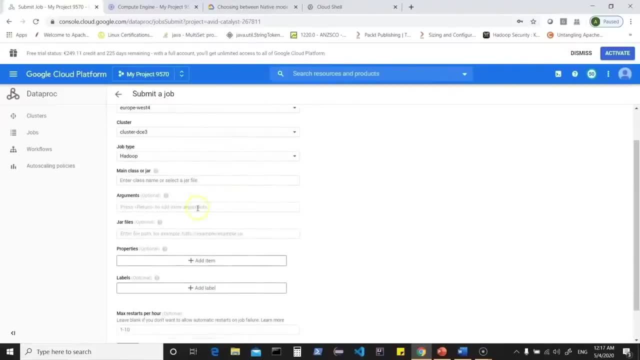 can give your jar file. so if you have, can give your jar file. so if you have packaged your application as a jar, you packaged your application as a jar. you packaged your application as a jar. you can mention that here you can pass in. can mention that here you can pass in. 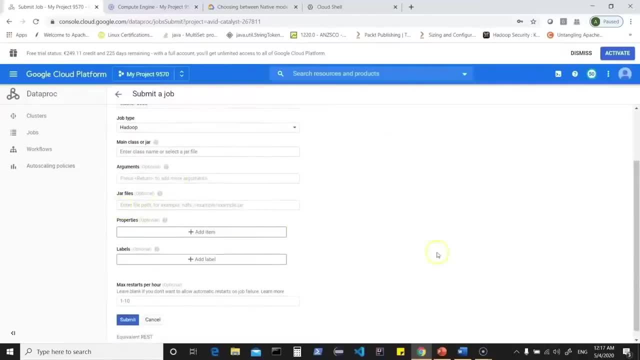 can mention that here you can pass in some arguments. you can also say some some arguments. you can also say some some arguments. you can also say some other jar files. add some properties and other jar files. add some properties and other jar files, add some properties and then click on submit, which will run your. 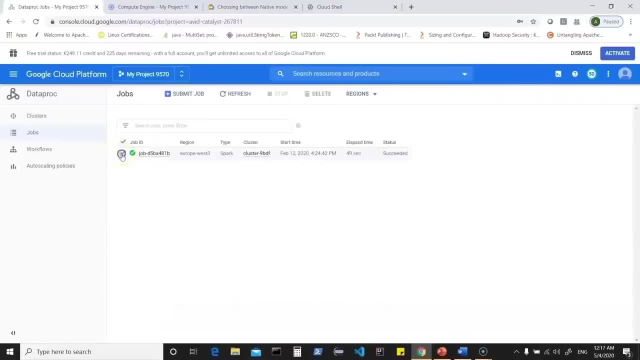 then click on submit, which will run your then click on submit, which will run your. job on this. ready to use cluster now. job on this. ready to use cluster now. job on this. ready to use cluster now. since we have tested it, I can basically. since we have tested it, I can basically. 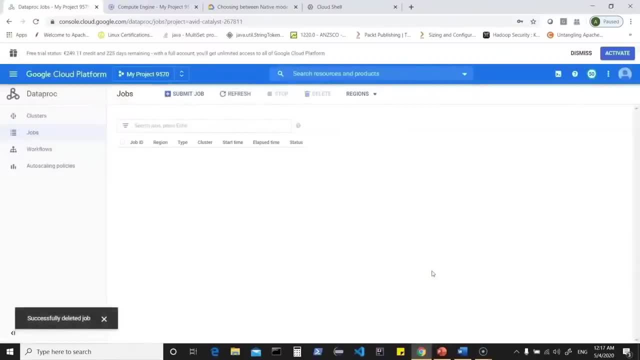 since we have tested it, I can basically go ahead and do a delete. I don't want to go ahead and do a delete. I don't want to go ahead and do a delete. I don't want to incur any cost on these managed services. incur any cost on these managed services. 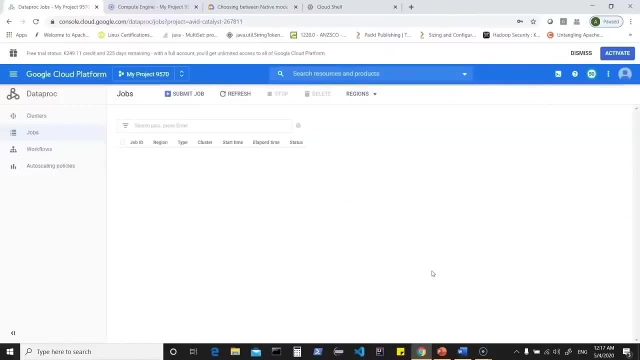 incur any cost on these managed services which are running. so there are a lot which are running. so there are a lot which are running. so there are a lot more information about using these, more information about using these, more information about using these services which Google Cloud platform. 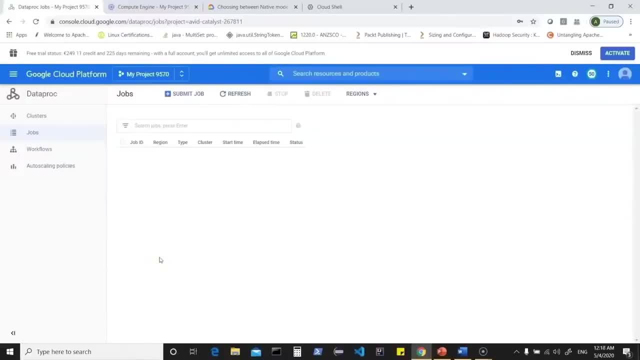 services which Google Cloud platform, services which Google Cloud platform offers, and we can continue learning about offers and we can continue learning about offers and we can continue learning about these services as we explore your these services, as we explore your these services, as we explore your Google Cloud console or even your command. 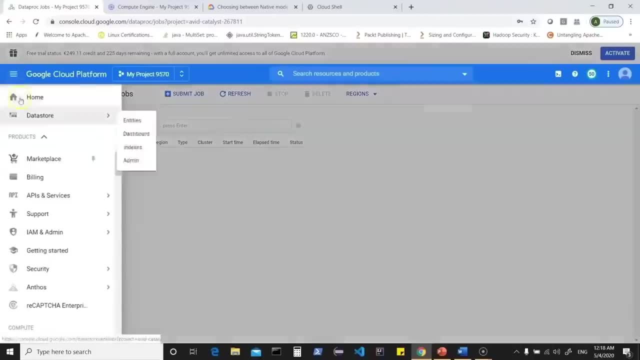 Google Cloud console or even your command Google Cloud console, or even your command line option. now we can come out of this line option. now we can come out of this line option. now we can come out of this one by clicking on this menu and then we one by clicking on this menu and then we. 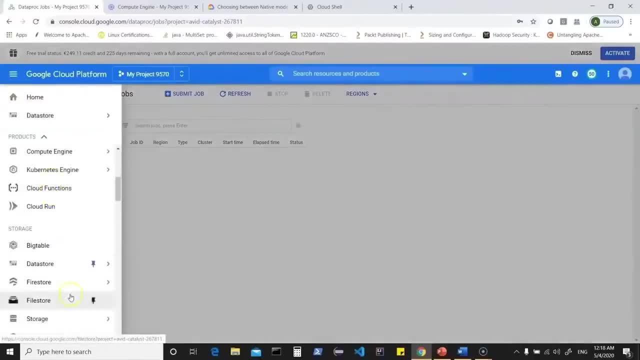 one by clicking on this menu. and then we have other options, such as kubernetes. have other options such as kubernetes. have other options such as kubernetes. you have cloud functions. you have your. you have cloud functions. you have your. you have cloud functions. you have your networking related services monitoring. 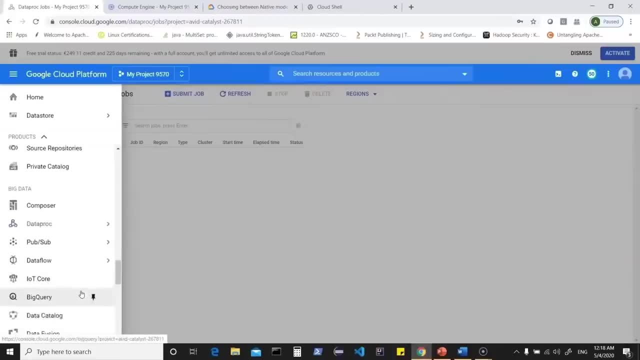 networking related services. monitoring networking related services. monitoring related services. different kind of tools related services. different kind of tools related services, different kind of tools. what you have. you have other big data. what you have. you have other big data. what you have you have. you have other big data, specific services which you can. 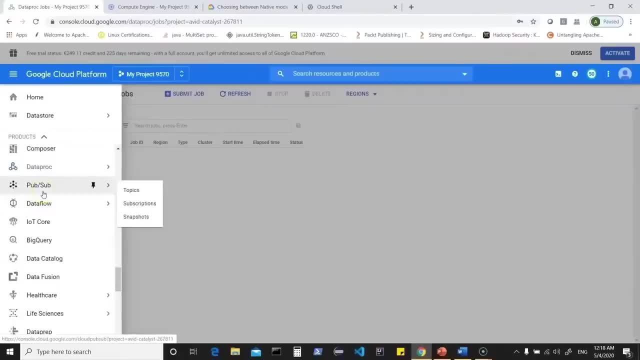 specific services which you can, specific services which you can learn about, and for each of these service learn about, and for each of these service learn about, and for each of these service, Google has a very good documentation. Google has a very good documentation. Google has a very good documentation available, for example, when you talk. 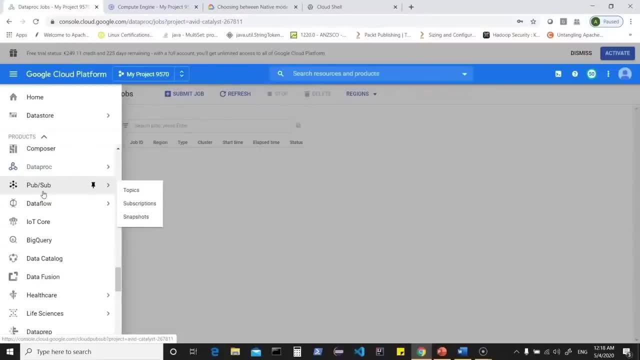 available, for example, when you talk available, for example, when you talk about published subscribed messaging, about published subscribed messaging, about published subscribed messaging system. it is a real-time managed system. it is a real-time managed service which basically is a pioneer service, which basically is a pioneer service, which basically is a pioneer, which was used and now you have a famous 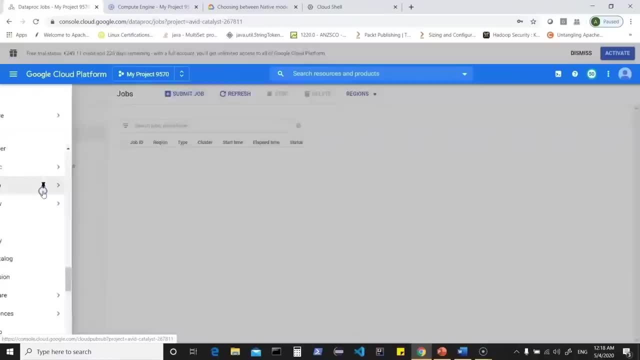 which was used, and now you have a famous which was used, and now you have a famous service such as Kafka, which is being service, such as Kafka which is being service, such as Kafka which is being used for your published subscribing or used for your published subscribing, or 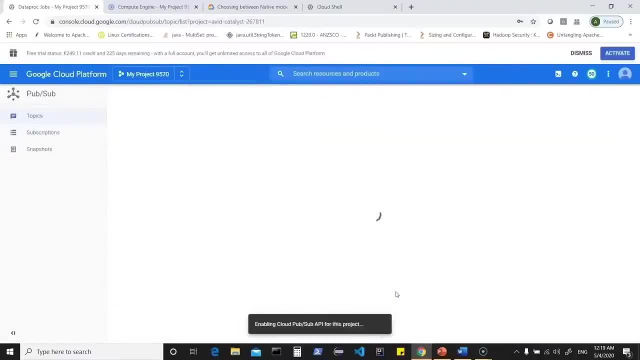 used for your published subscribing or messaging system kind of requirements. so messaging system, kind of requirements. so messaging system, kind of requirements. so to conclude about Google Cloud Platform, to conclude about Google Cloud Platform, to conclude about Google Cloud Platform, services: you can always go to cloud services. you can always go to cloud. 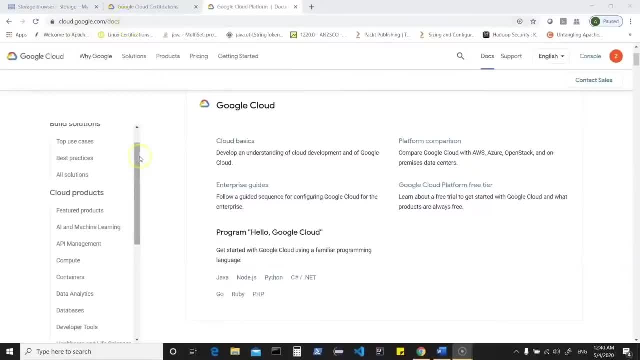 services. you can always go to cloud googlecom and look into the document googlecom and look into the document googlecom and look into the document section now. here you have list of section now. here you have list of section now. here you have list of different featured products. you also 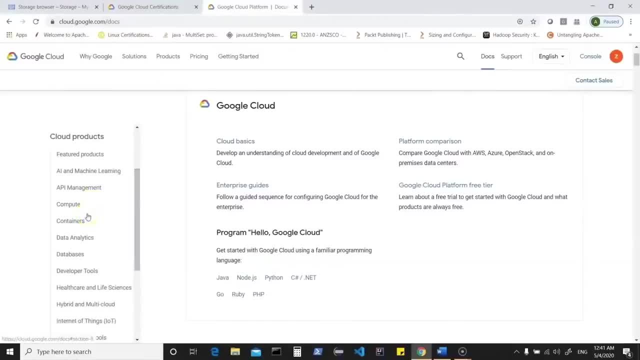 different featured products. you also different featured products. you also have list of your different domains and have list of your different domains and have list of your different domains and services which Google Cloud offers and services which Google Cloud offers and services which Google Cloud offers, and you can learn about all the different. 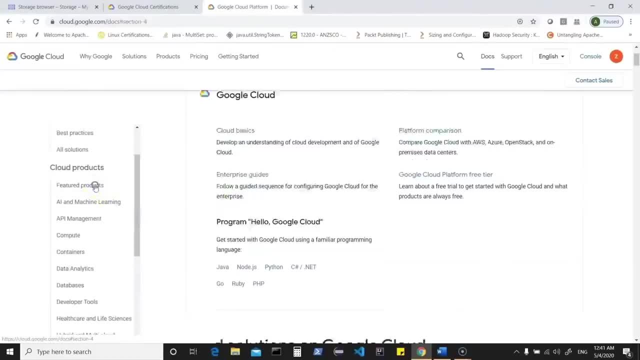 you can learn about all the different. you can learn about all the different services which are offered by Google services which are offered by Google services, which are offered by Google Cloud. here you can click on featured Cloud. here you can click on featured Cloud, here you can click on featured products, and that basically shows you. 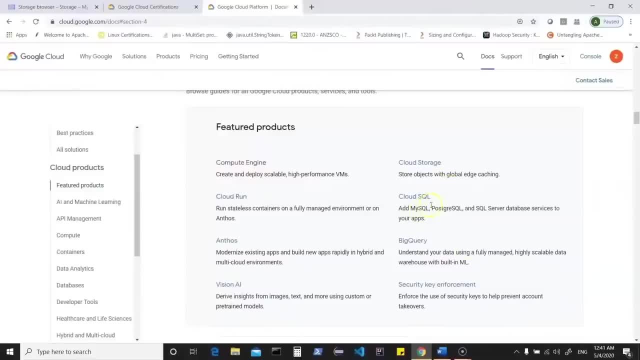 products and that basically shows you products and that basically shows you compute engine: cloud run cloud storage compute engine. cloud run cloud storage compute engine. cloud run cloud storage. you have cloud SQL BigQuery vision AI. you. you have cloud SQL BigQuery vision AI- you. you have cloud SQL BigQuery vision AI. you can scroll down and look at your. 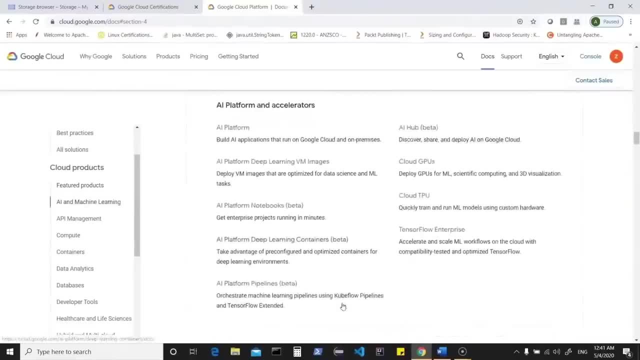 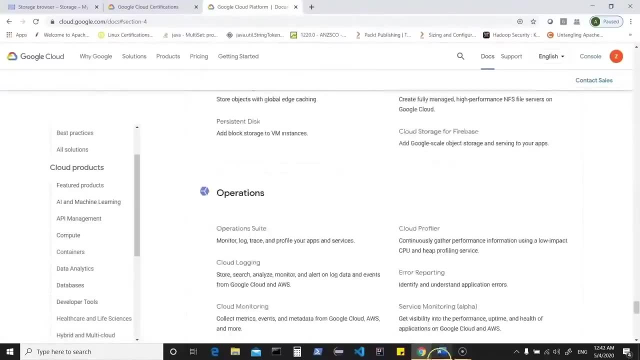 can scroll down and look at your. can scroll down and look at your artificial intelligence and machine artificial intelligence and machine artificial intelligence and machine learning related services. platform and learning related services. platform and learning related services. platform and accelerators- API management- so Google. accelerators API management- so Google. 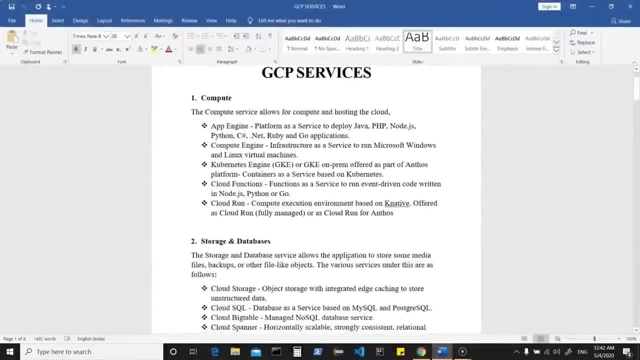 accelerators, API management. so Google cloud platform offers different services. cloud platform offers different services. cloud platform offers different services in mainly in your compute storage and in mainly in your compute storage and in mainly in your compute storage and databases. you have networking related databases. you have networking related. 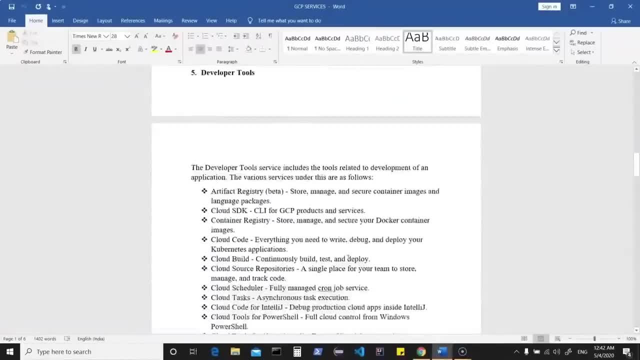 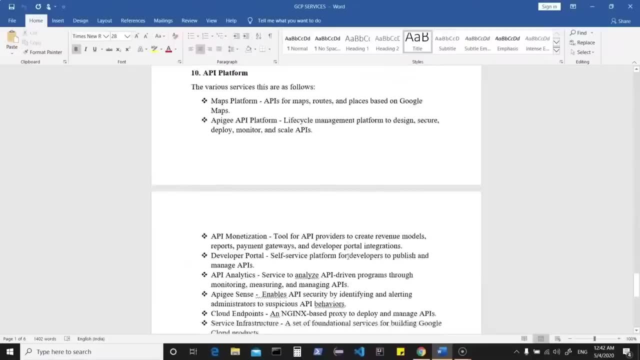 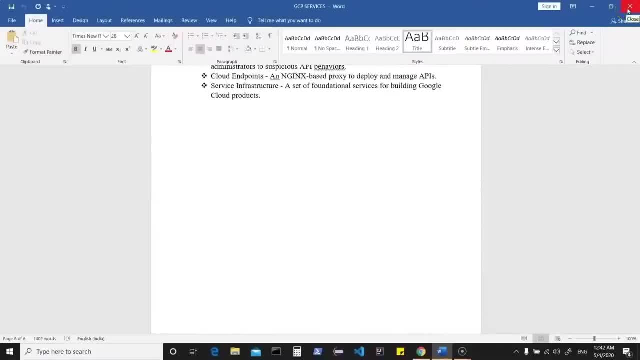 management tools API platform and so on, management tools API platform and so on. so basically learn about the GCP services. so basically learn about the GCP services. so basically learn about the GCP services which Google Cloud Platform offers and which Google Cloud Platform offers and which Google Cloud Platform offers, and in detail you can play around with. 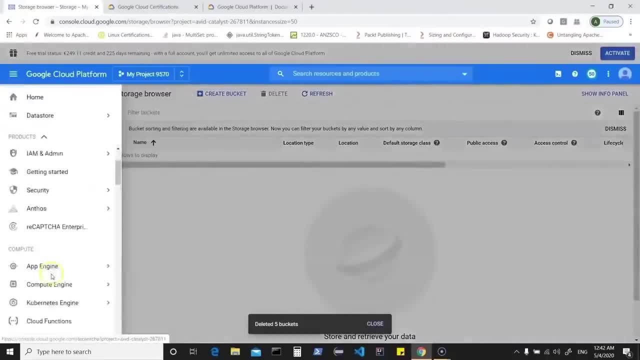 in detail. you can play around with. in detail, you can play around with different services which are offered by different services, which are offered by different services, which are offered by creating a free account and, as I creating a free account and as I creating a free account and as I demonstrated, you can use any one of these. 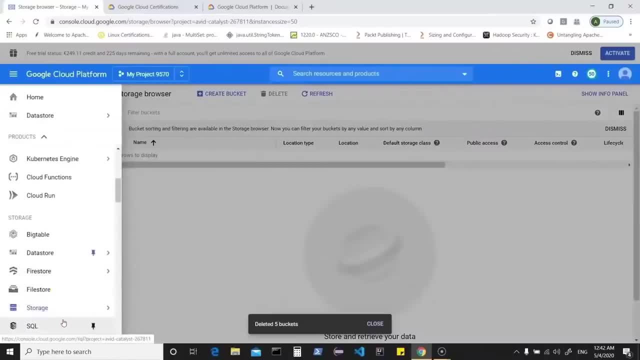 demonstrated you can use any one of these. demonstrated you can use any one of these services. quick. start them, basically services. quick, start them, basically services. quick, start them basically connect to them. put in your data or use. connect to them. put in your data or use. connect to them. put in your data or use a managed service to manage your data. 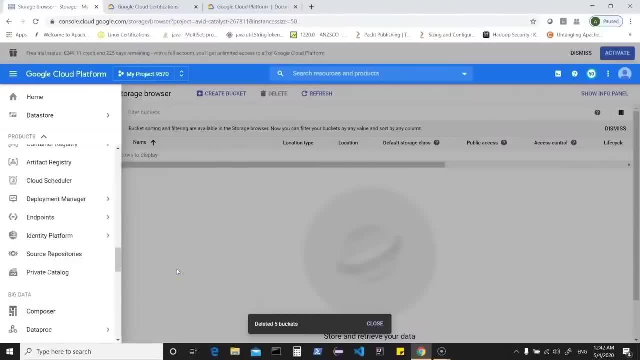 a managed service to manage your data, a managed service to manage your data and benefit from Google Cloud Platform and benefit from Google Cloud Platform and benefit from Google Cloud Platform, thus having modernized infrastructure, thus having modernized infrastructure, thus having modernized infrastructure for your different use cases. hi guys, 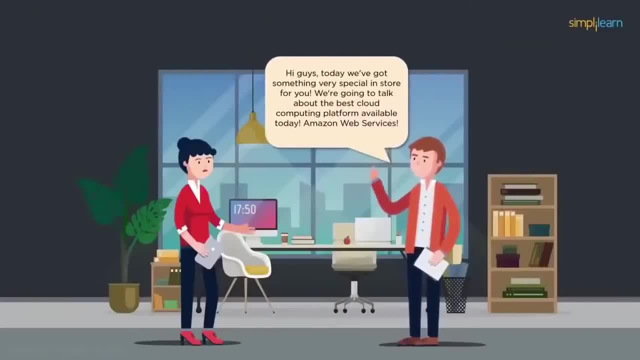 for your different use cases, hi guys, for your different use cases. hi guys, today we've got something very special. today we've got something very special. today. we've got something very special in store for you, we're going to talk. in store for you, we're going to talk. 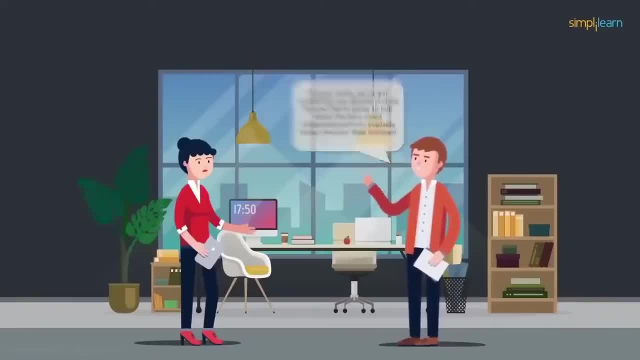 in store for you. we're going to talk about the best cloud computing platform, about the best cloud computing platform, about the best cloud computing platform available. Amazon Web Services. available Amazon Web Services. available- Amazon Web Services. Rahul, I think you said something wrong. Rahul, I think you said something wrong. 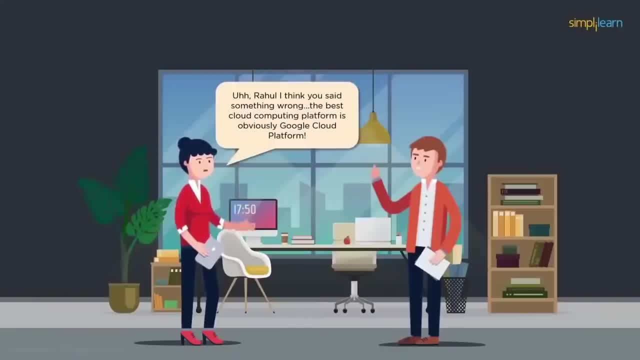 Rahul, I think you said something wrong here. the best cloud computing platform is here. the best cloud computing platform is here. the best cloud computing platform is obviously Google Cloud Platform. no, it obviously Google Cloud Platform. no, it obviously Google Cloud Platform. no, it isn't. AWS has more than hundred services. isn't AWS has more than hundred services. isn't AWS has more than hundred services that span over 80 of domains? all right, that span over 80 of domains- all right, that span over 80 of domains, all right. but Google Cloud Platform has cheaper. but Google Cloud Platform has cheaper. 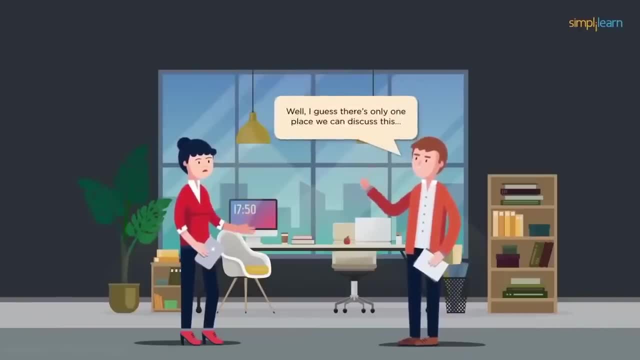 but Google Cloud Platform has cheaper instances. what do you have to say about instances? what do you have to say about instances? what do you have to say about that? well, I guess there's only one place that? well, I guess there's only one place that. well, I guess there's only one place we can actually discuss this: a boxing. 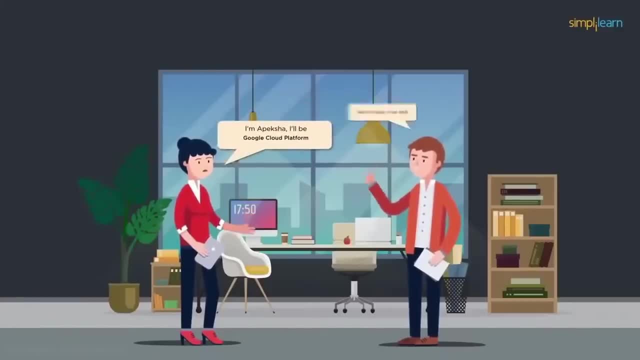 we can actually discuss this a boxing. we can actually discuss this a boxing ring. so, guys, I'm a big shot and I will ring. so, guys, I'm a big shot and I will ring. so, guys, I'm a big shot and I will be Google Cloud platform. I'm Rahul, I'll. 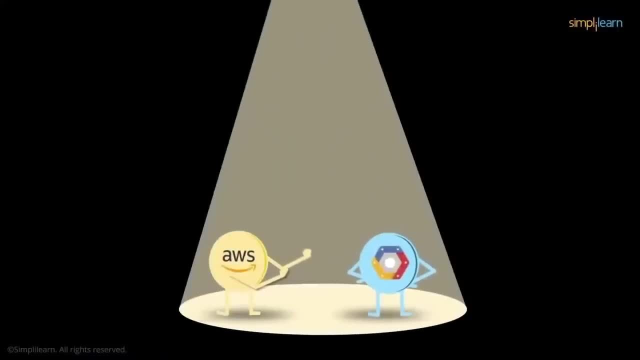 be Google Cloud platform. I'm Rahul. I'll be Google Cloud platform. I'm Rahul. I'll be AWS. so welcome to fight night. this is be AWS. so welcome to fight night. this is be AWS. so welcome to fight night. this is AWS versus GCP. the winner will be chosen. AWS versus GCP, the winner will be chosen AWS versus GCP. the winner will be chosen on the basis of their origin and the on the basis of their origin and the on the basis of their origin and the features. they provide their performance. features: they provide their performance. 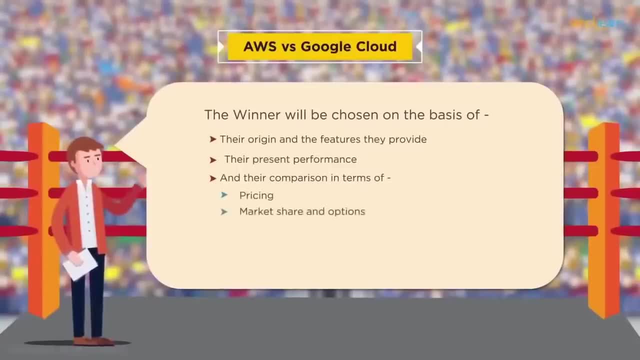 features they provide, their performance in the present day and comparing them on in the present day. and comparing them on in the present day, and comparing them on the basis of pricing market share and the basis of pricing market share and the basis of pricing market share and options, the things they give you for. 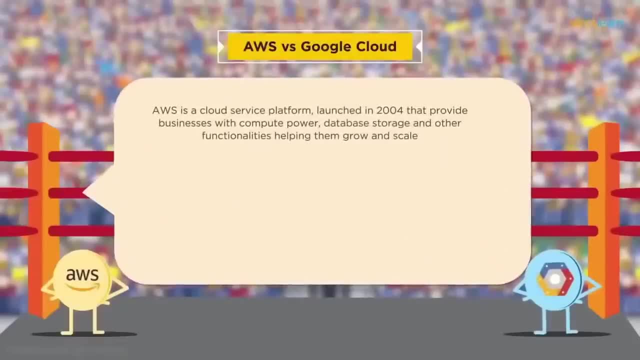 options, the things they give you for options, the things they give you for free. and instance configuration- now free. and instance configuration- now free. and instance configuration now. first, let's talk about AWS. AWS was first. let's talk about AWS. AWS was first. let's talk about AWS. AWS was launched in 2004 and is a cloud service. 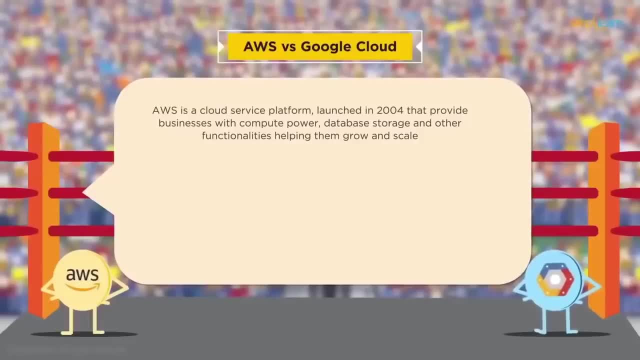 launched in 2004 and is a cloud service. launched in 2004 and is a cloud service platform that helps businesses grow. and platform that helps businesses grow. and platform that helps businesses grow and scale by providing them services in a scale. by providing them services in a 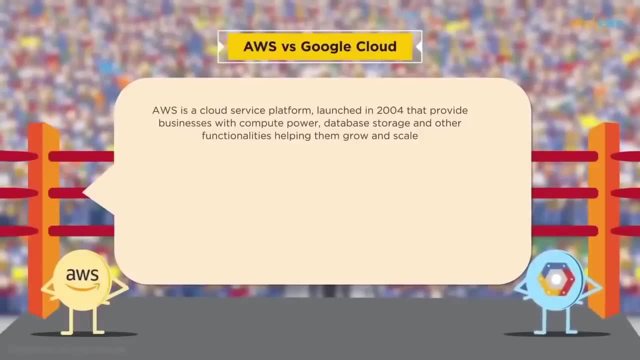 scale by providing them services in a number of different domains. these number of different domains, these number of different domains. these domains include compute database domains, include compute database domains, include compute database, storage migration networking, and so on. a storage migration networking, and so on. a storage migration networking, and so on. a very important aspect about AWS is its 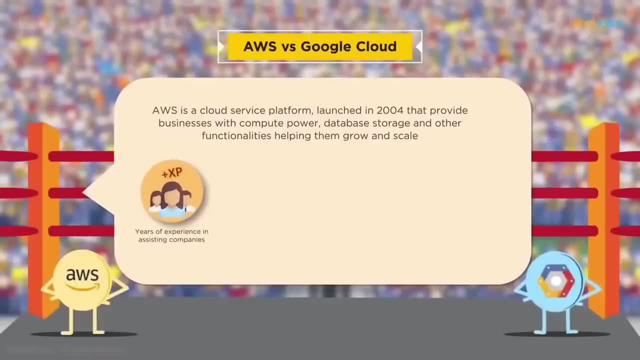 very important aspect about AWS is its very important aspect about AWS is its years of experience. now AWS has been in years of experience now AWS has been in years of experience. now. AWS has been in the market a lot longer than any other, the market a lot longer than any other. 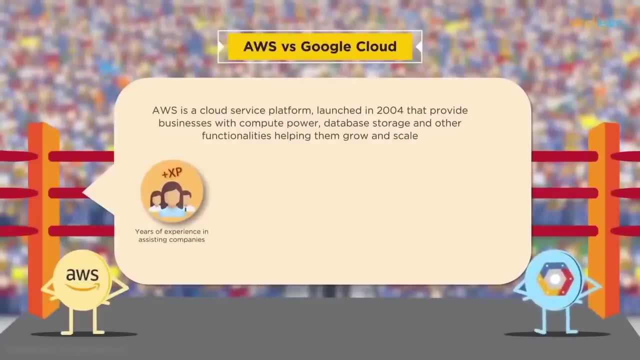 the market a lot longer than any other cloud service platform, which means they cloud service platform. which means they cloud service platform, which means they know how businesses work and how they can know how businesses work and how they can know how businesses work and how they can contribute to the business growing. 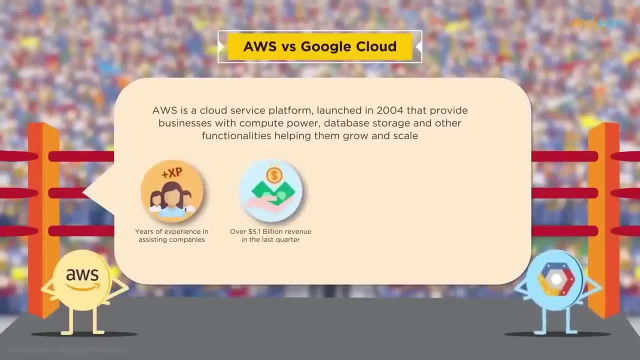 contribute to the business growing. contribute to the business growing. also. AWS has over 5.1 billion dollars of also AWS has over 5.1 billion dollars of. also AWS has over 5.1 billion dollars of revenue in the last quarter. this is a. 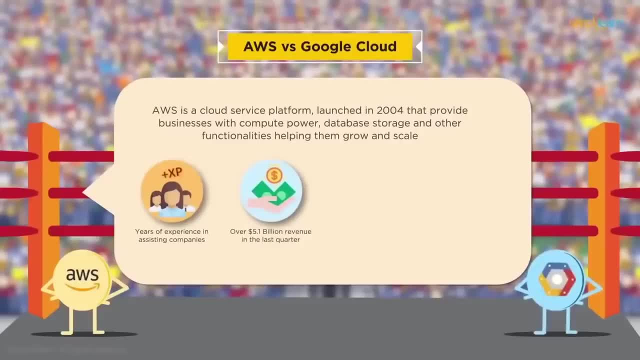 revenue in the last quarter. this is a revenue in the last quarter. this is a clear indication of how much faith and clear indication of how much faith and clear indication of how much faith and trust people have in AWS they occupy trust people have in AWS they occupy. 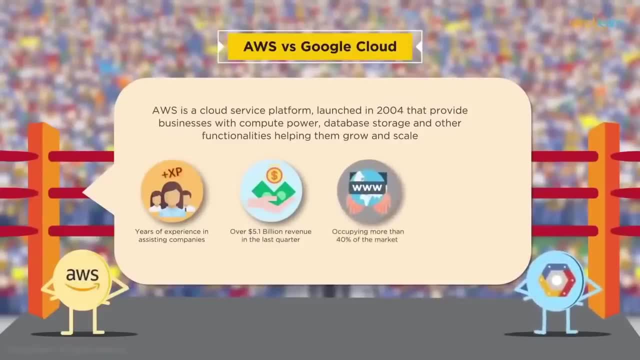 trust people have in AWS. they occupy more than 40% of the market, which is a more than 40% of the market, which is a more than 40% of the market, which is a significant chunk of the cloud computing, significant chunk of the cloud computing. 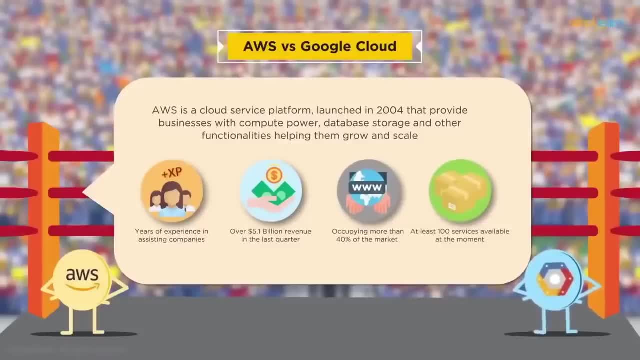 significant chunk of the cloud computing market. they have at least 100 services market. they have at least 100 services market. they have at least 100 services that are available at the moment, which that are available at the moment, which that are available at the moment, which means just about every issue that you 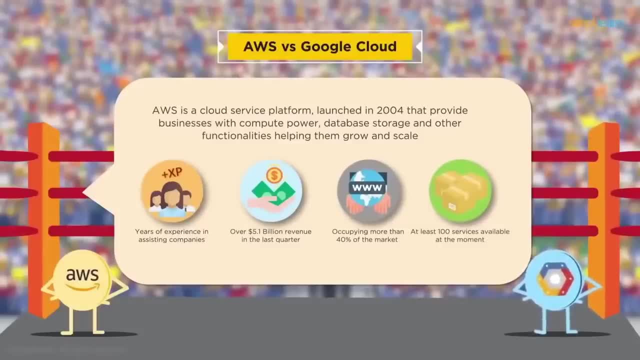 means just about every issue that you means just about every issue that you have can be solved with an AWS service. have can be solved with an AWS service. have can be solved with an AWS service. now that was great, but now can we talk. now that was great, but now can we talk. 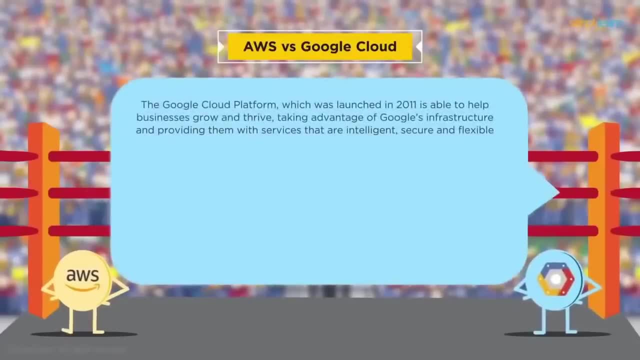 now, that was great, but now can we talk about GCP. I hope you know that GCP was about GCP. I hope you know that GCP was about GCP. I hope you know that GCP was launched very recently, 2011- and it is. 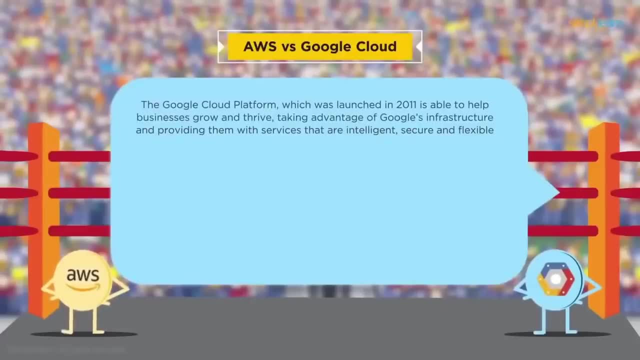 launched very recently, 2011, and it is launched very recently, 2011, and it is already helping businesses significantly, already helping businesses significantly, already helping businesses significantly with a suite of intelligent secure and with a suite of intelligent secure and with a suite of intelligent, secure and flexible cloud computing services. it 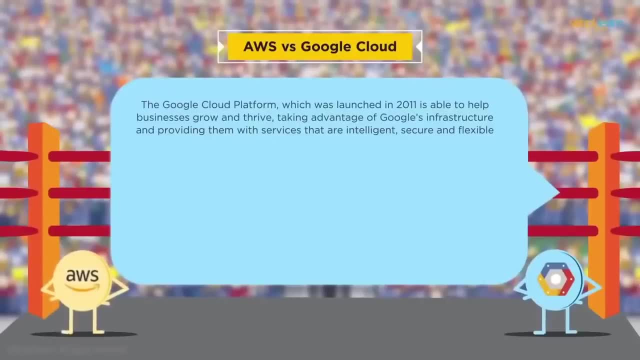 flexible cloud computing services. it flexible cloud computing services. it lets you build, deploy and scale. lets you build, deploy and scale. lets you build, deploy and scale applications website services on the same applications website services on the same applications website services on the same infrastructure as Google. the intuitive, 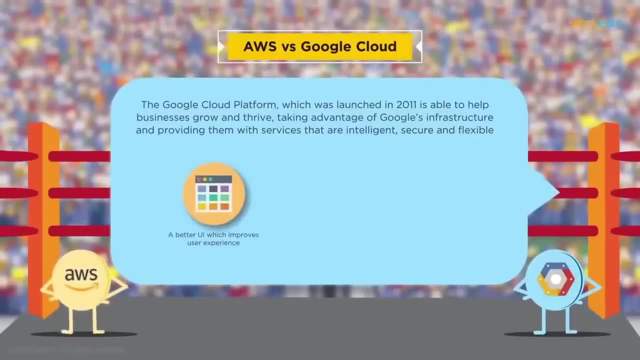 infrastructure as Google, the intuitive infrastructure as Google, the intuitive user experience that GCP provides with user experience. that GCP provides with user experience. that GCP provides with dashboards. wizards is way better in all dashboards. wizards is way better in all dashboards. wizards is way better in all the aspects. GCP has just stepped in the. 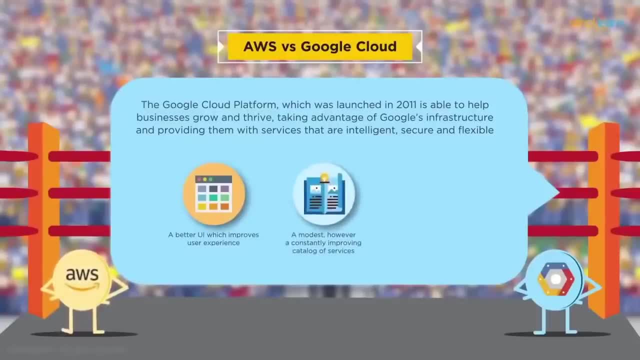 the aspects GCP has just stepped in the the aspects GCP has just stepped in the market and it is already offering a market. and it is already offering a market and it is already offering a modest number of services and the number- modest number of services and the number. 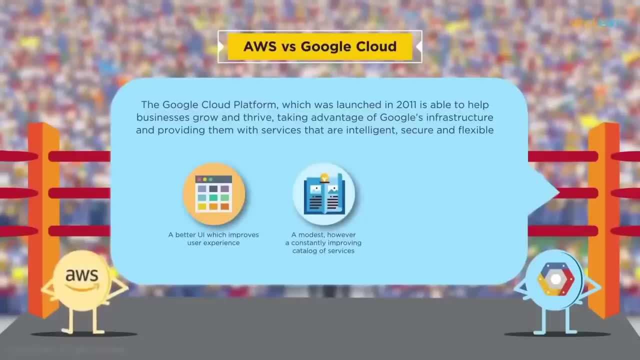 modest number of services and the number is rapidly increasing and the cost for a is rapidly increasing. and the cost for a is rapidly increasing and the cost for a CPU instance or region storage, that GCP CPU instance or region storage, that GCP CPU instance or region storage that GCP provides, is a whole lot cheaper and you 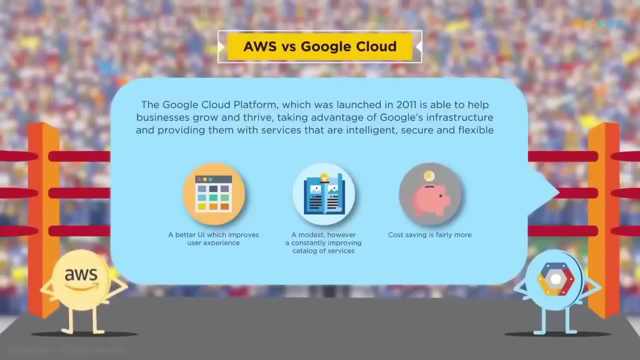 provides is a whole lot cheaper, and you provides is a whole lot cheaper, and you also get a multi regional cloud storage. also get a multi regional cloud storage. also get a multi regional cloud storage. now, what do you have to say on that? I'm now. what do you have to say on that? I'm. now, what do you have to say on that? I'm so glad you asked let's look at present. so glad you asked let's look at present. so glad you asked: let's look at present day. in fact, let's look at the cloud day. in fact, let's look at the cloud. 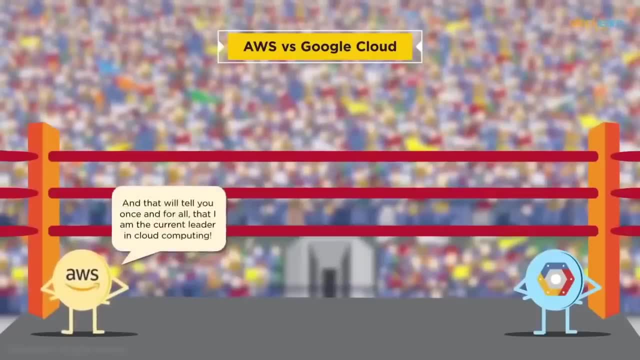 day. in fact, let's look at the cloud market share of the fourth quarter of market share of the fourth quarter of market share of the fourth quarter of 2017. this will tell you once and for all: 2017. this will tell you once and for all. 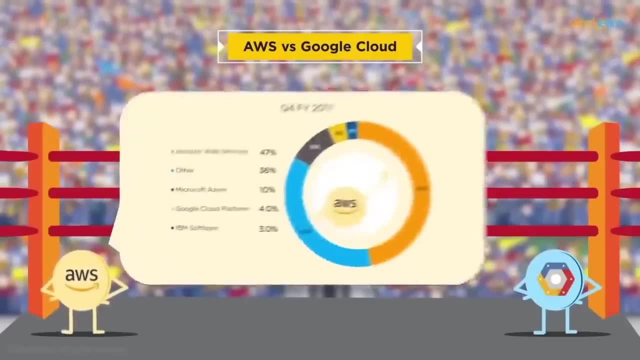 2017. this will tell you once and for all that AWS is the leader when it comes to that. AWS is the leader when it comes to that. AWS is the leader when it comes to cloud computing, Amazon Web Services. cloud computing- Amazon Web Services. cloud computing- Amazon Web Services contributes 47% of the market share. 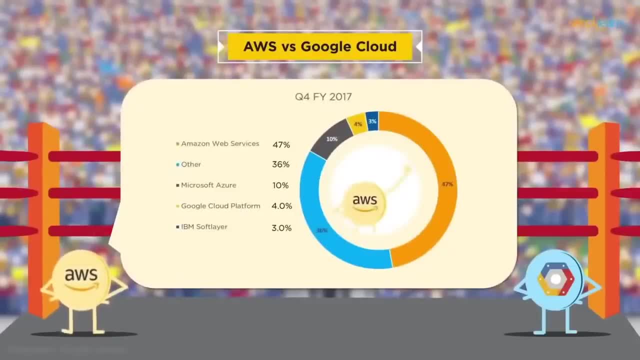 contributes 47% of the market share. contributes 47% of the market share. others like Rackspace or Verizon cloud. others like Rackspace or Verizon cloud. others like Rackspace or Verizon cloud. contribute 36% Microsoft Azure. contribute 36% Microsoft Azure. 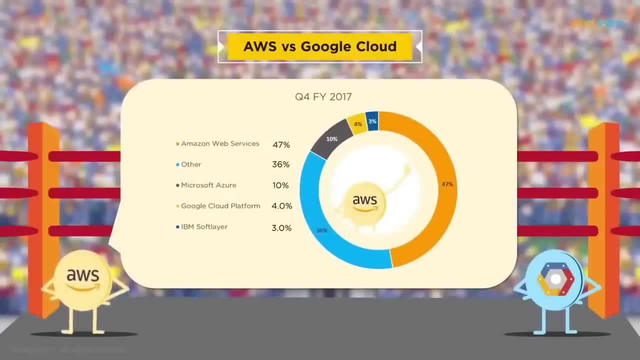 contribute 36%. Microsoft Azure contributes 10%. the Google Cloud contributes 10%. the Google Cloud contributes 10%. the Google Cloud platform contributes 4% and IBM software platform contributes 4% and IBM software platform contributes 4% and IBM software contributes 3%- 47% of the market share. 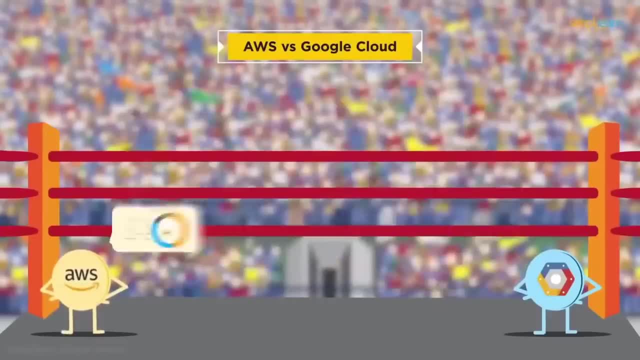 contributes 3%- 47% of the market share contributes 3%. 47% of the market share is contributed by AWS. you need me to is contributed by AWS. you need me to is contributed by AWS. you need me to convince you anymore. wait, wait, wait all. 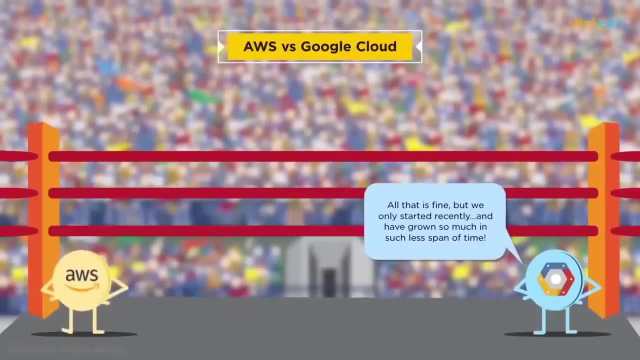 convince you anymore, wait, wait, wait, all convince you anymore, wait, wait, wait. all that is fine, but we only started a few. that is fine. but we only started a few, that is fine. but we only started a few years back and have already grown so. years back and have already grown so. 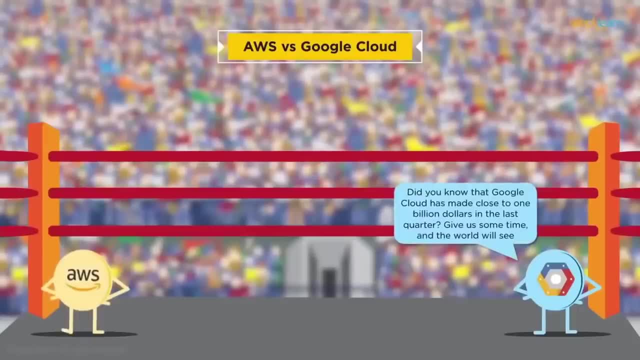 years back and have already grown so much in such a less span of time. having much in such a less span of time, having much in such a less span of time. having to hurt the latest news: our revenue is to hurt the latest news. our revenue is to hurt the latest news. our revenue is already a billion dollars per quarter. 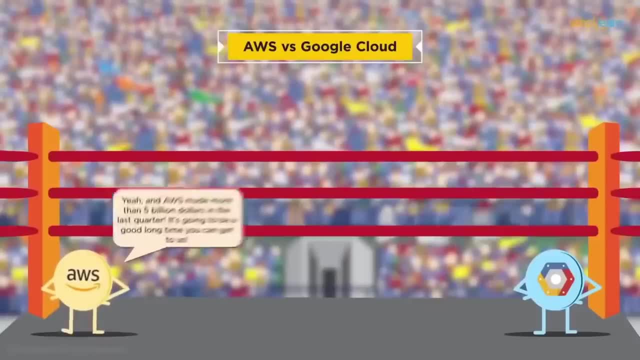 already a billion dollars per quarter. already a billion dollars per quarter. wait for a few more years, and the world wait for a few more years. and the world wait for a few more years and the world shall see. and AWS makes 5.3 billion. shall see, and AWS makes 5.3 billion. 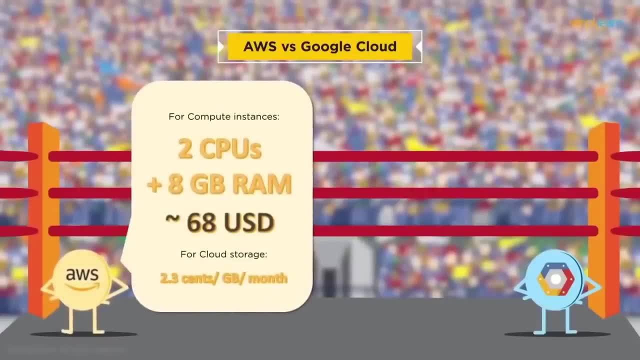 shall see, and AWS makes 5.3 billion of two CPUs in 8gb RAM. costs of two CPUs in 8gb RAM. costs of two CPUs in 8gb RAM costs approximately 68 US dollars now a. approximately 68 US dollars now a. 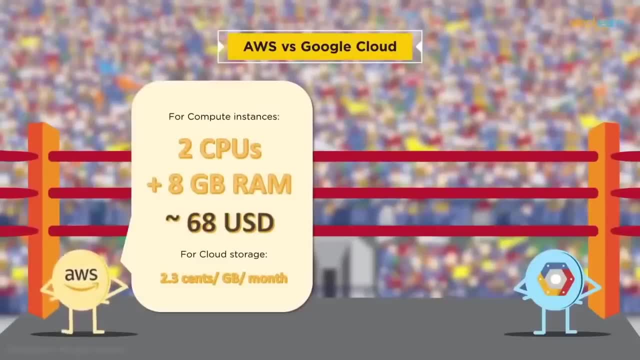 approximately 68 US dollars now, a computer. instance of a virtual machine computer. instance of a virtual machine computer. instance of a virtual machine in which you can specify what operating, in which you can specify what operating, in which you can specify what operating system, RAM or storage you want to have. 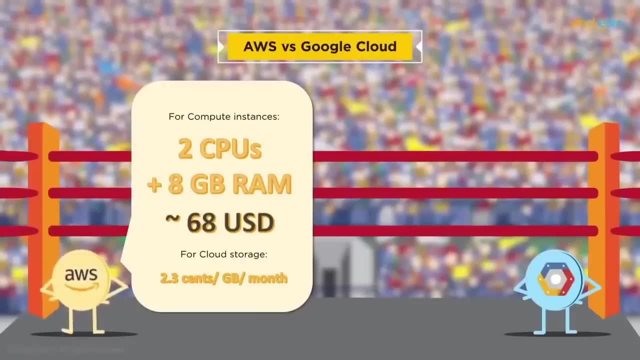 system RAM or storage. you want to have system RAM or storage. you want to have for cloud storage. it costs 2.3 cents per for cloud storage. it costs 2.3 cents per for cloud storage. it costs 2.3 cents per GB per month with AWS. you really want to. 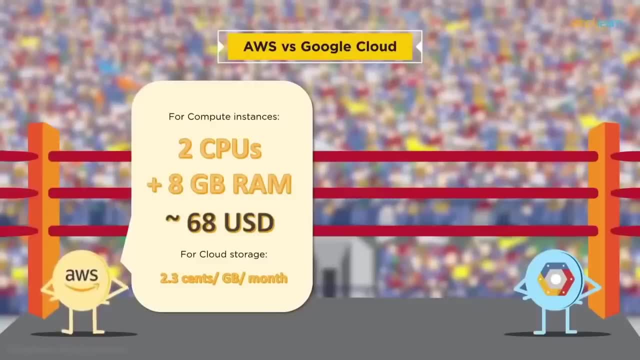 GB per month with AWS. you really want to GB per month with AWS. you really want to do that because GCP wins this hands-down. do that because GCP wins this hands-down. do that because GCP wins this hands-down. let's take the same compute instance of: 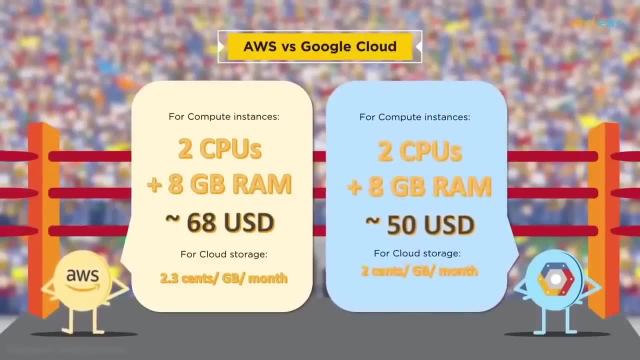 let's take the same compute instance of. let's take the same compute instance of two CPUs with 8gb RAM. it will cost two CPUs with 8gb RAM. it will cost two CPUs with 8gb RAM. it will cost approximately 50 dollars per month with. 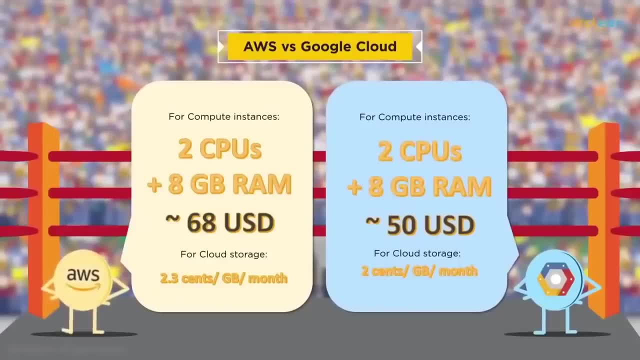 approximately 50 dollars per month, with approximately 50 dollars per month with GCP. and as for my calculations, that's a GCP. and as for my calculations, that's a GCP. and as for my calculations, that's a 25% annual cost reduction when compared. 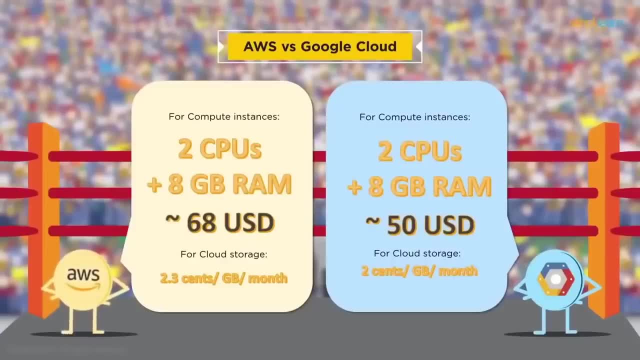 25% annual cost reduction. when compared: 25% annual cost reduction. when compared to AWS talking about clouds to which to AWS talking about clouds to which to AWS talking about clouds to which. cause it is only 2 cents per GB per month. cause it is only 2 cents per GB per month. 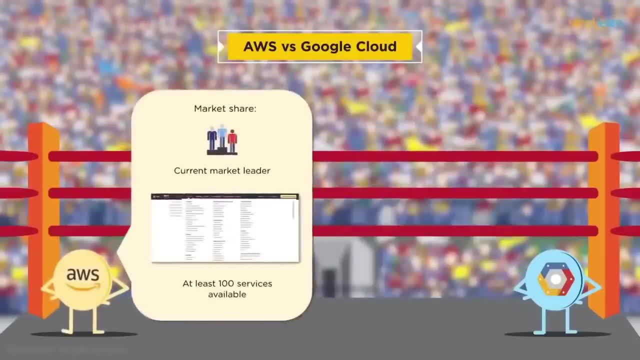 cause it is only 2 cents per GB per month with GCP. what else do you want me to say with GCP? what else do you want me to say with GCP? what else do you want me to say? let's talk about market share and 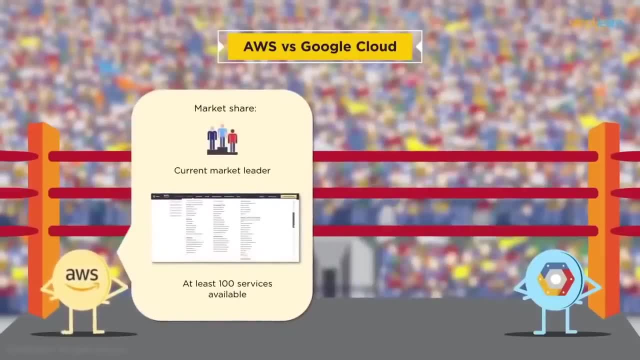 let's talk about market share, and let's talk about market share and options. now, AWS is the current market options. now, AWS is the current market options. now, AWS is the current market leader when it comes to cloud computing. leader when it comes to cloud computing. leader when it comes to cloud computing. now, as you remember, we contribute at 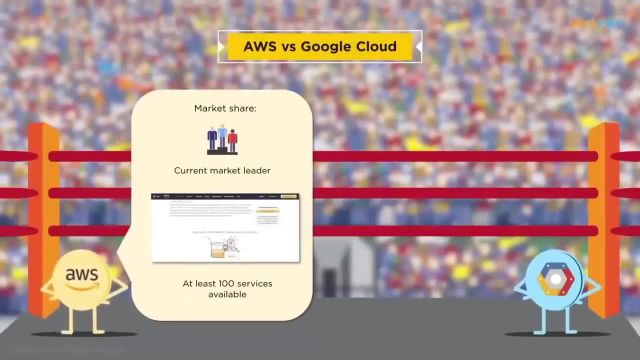 now, as you remember, we contribute at now. as you remember, we contribute at least 47% of the entire market share. least 47% of the entire market share. least 47% of the entire market share. AWS also has at least 100 services. AWS also has at least 100 services. 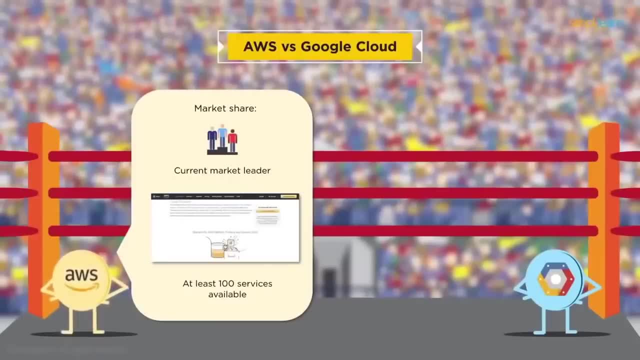 AWS also has at least 100 services available at the moment, which is a available at the moment. which is a available at the moment, which is a clear indication of how well AWS. clear indication of how well AWS. clear indication of how well AWS understands businesses and helps them. 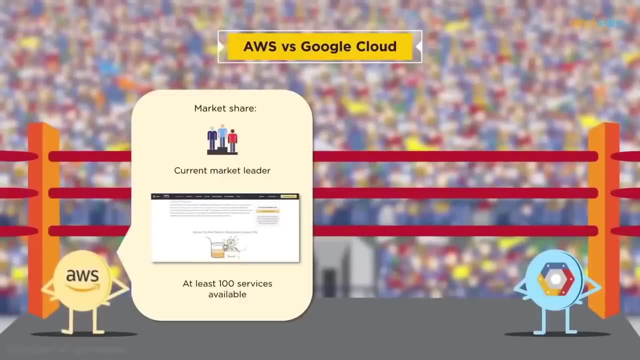 understands businesses and helps them. understands businesses and helps them grow. yeah, that's true, but you should grow. yeah, that's true, but you should grow. yeah, that's true, but you should also know that GCP is steadily growing. also know that GCP is steadily growing. also know that GCP is steadily growing. we have over 60 services that are up and. 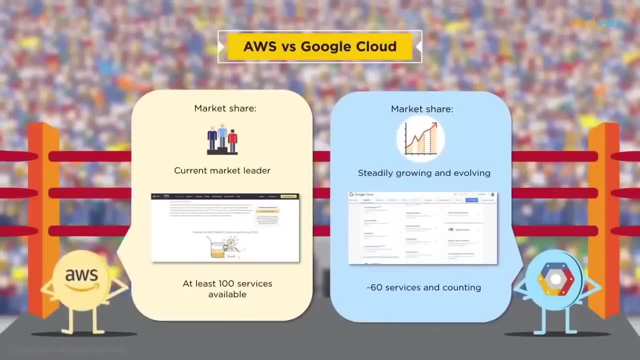 we have over 60 services that are up, and we have over 60 services that are up and running, as you can see here, and a lot running, as you can see here, and a lot running, as you can see here, and a lot more to come. it's only a matter of time. 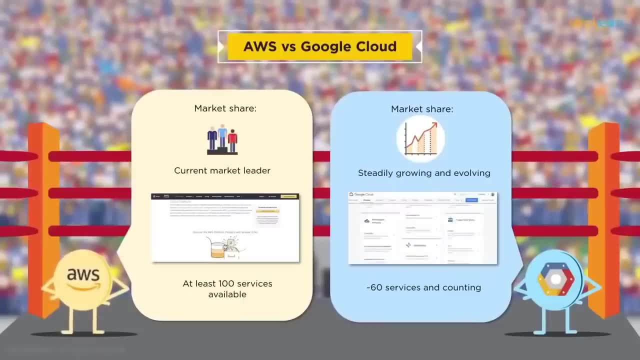 more to come. it's only a matter of time. more to come. it's only a matter of time when we will have as many services as when we will have as many services as when we will have as many services as you do many companies have already. you do many companies have already. 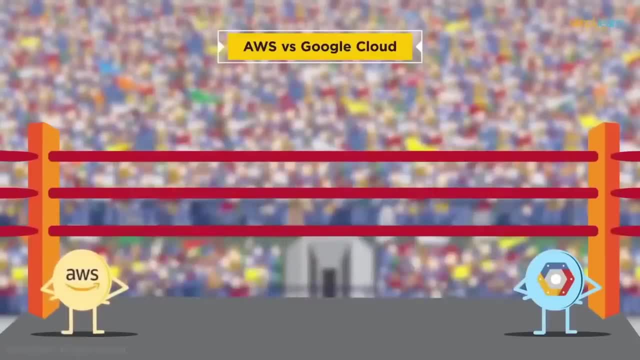 you do. many companies have already started adopting GCP as a cloud service, started adopting GCP as a cloud service, started adopting GCP as a cloud service provider. now let's talk about things- provider. now, let's talk about things- provider. now, let's talk about things you get for free with AWS. you get access. 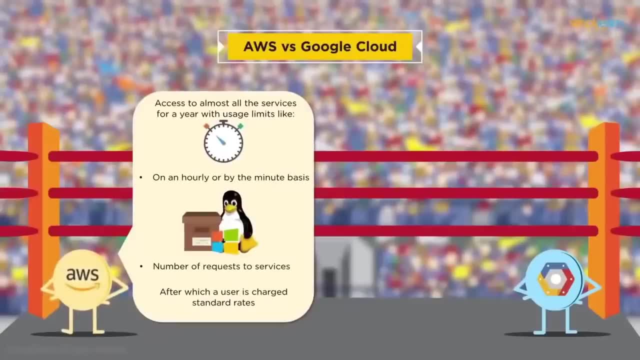 you get for free with AWS: you get access. you get for free with AWS: you get access to almost all the services for an entire, to almost all the services for an entire, to almost all the services for an entire. year with usage limits- now these limits. year with usage limits- now these limits. 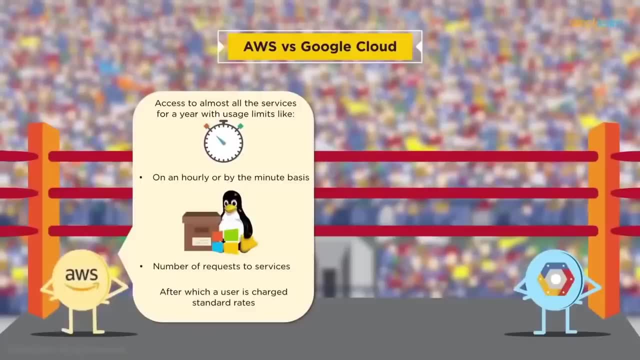 year with usage limits. now these limits include an hourly or by the minute basis? include an hourly or by the minute basis. include an hourly or by the minute basis. for example, with Amazon ec2, you get 750. for example, with Amazon ec2, you get 750. 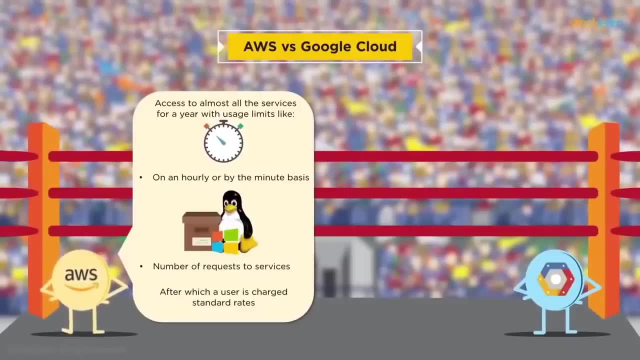 for example, with Amazon ec2, you get 750 hours per month. you also have limits on hours per month. you also have limits on hours per month. you also have limits on the number of requests to services, for the number of requests to services. for the number of requests to services, for example, with AWS lambda, you have 1. 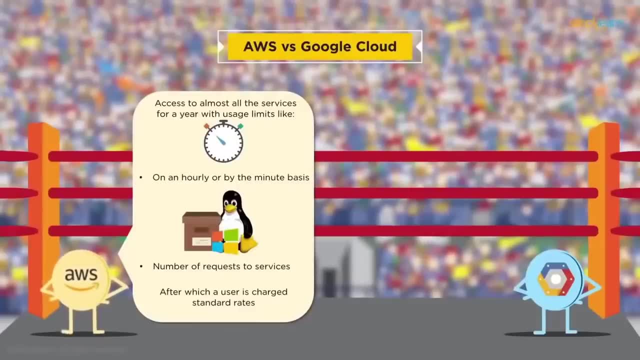 example, with AWS lambda. you have 1 example with AWS lambda. you have 1 million requests per month. now, after million requests per month, now, after million requests per month, now, after these limits across, you get charged, these limits across, you get charged. these limits across, you get charged. standard rates with GCP, you get access. 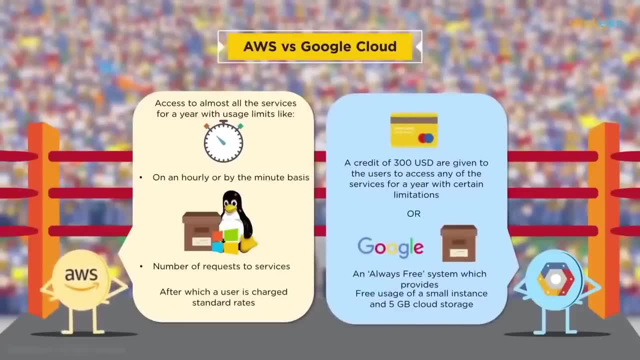 standard rates with GCP, you get access standard rates. with GCP, you get access to all cloud platform products. like to all cloud platform products. like to all cloud platform products like firebase, Google Maps API and so on. you firebase Google Maps API and so on. you firebase Google Maps API and so on. you also get $300 in credit to spend over a. 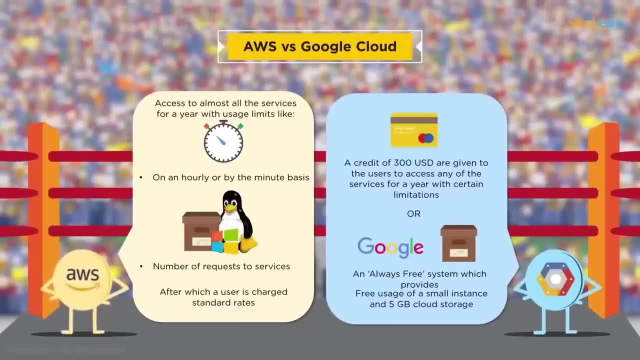 also get $300 in credit to spend over a. also get $300 in credit to spend over a 12-month period on all the cloud 12-month period. on all the cloud 12-month period on all the cloud platform products and, interestingly, platform products and interestingly. 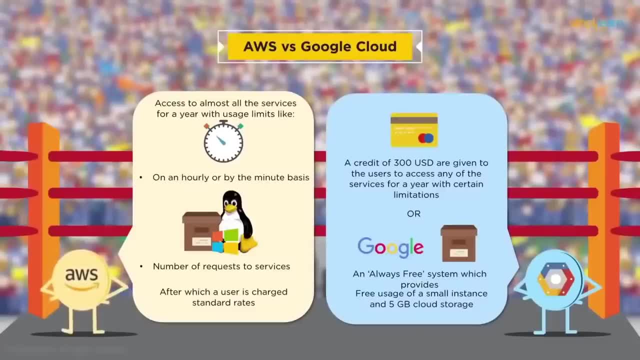 platform products and, interestingly, after the free trial ends, you won't be. after the free trial ends, you won't be. after the free trial ends, you won't be charged unless you manually upgrade to a charged, unless you manually upgrade to a charged, unless you manually upgrade to a paid account. now there is also the 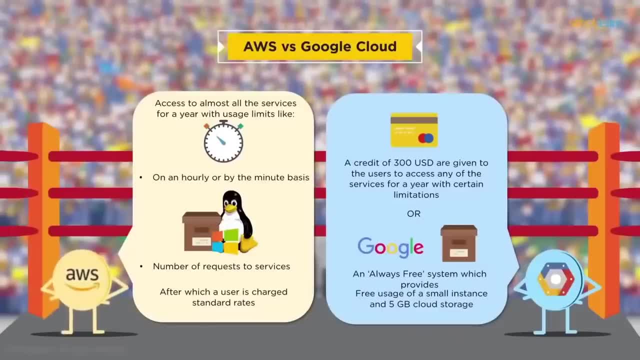 paid account. now there is also the paid account. now there is also the always free version, for which you will always free version, for which you will always free version, for which you will need an upgraded billing account here. need an upgraded billing account here. need an upgraded billing account. here you get to use a small instance for free. 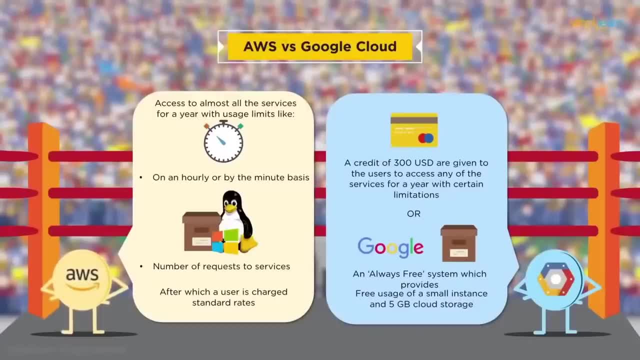 you get to use a small instance for free. you get to use a small instance for free and 5gb of cloud storage- any usage. and 5gb of cloud storage- any usage. and 5gb of cloud storage- any usage. above this, always free usage limits will be. 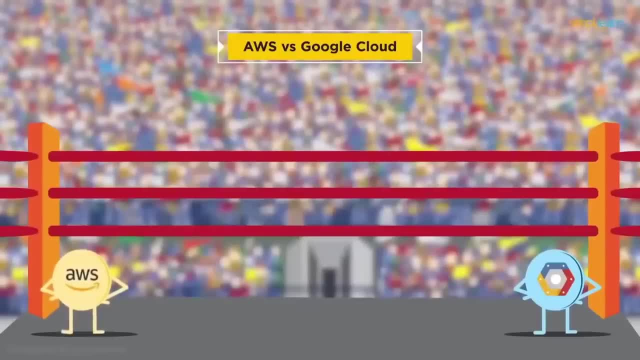 above this, always free usage limits will be. above this, always free usage limits will be automatically billed at standard rates. automatically billed at standard rates, automatically billed at standard rates. now, let's talk about how you can now, let's talk about how you can. now, let's talk about how you can configure instances with AWS, the largest. 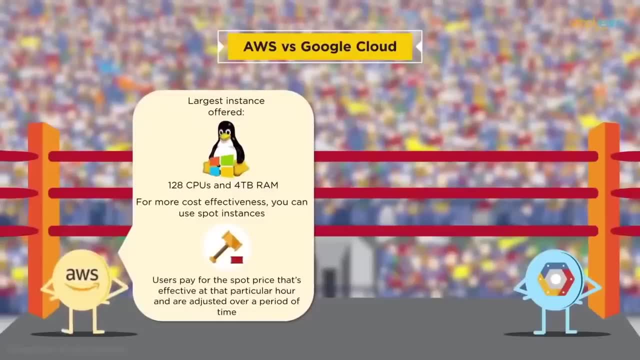 configure instances with AWS. the largest. configure instances with AWS. the largest instance as offered is of 128 CPUs and instance as offered is of 128 CPUs, and instance as offered is of 128 CPUs and 4 TVs of RAM now, other than the 4 TVs of RAM now other than the. 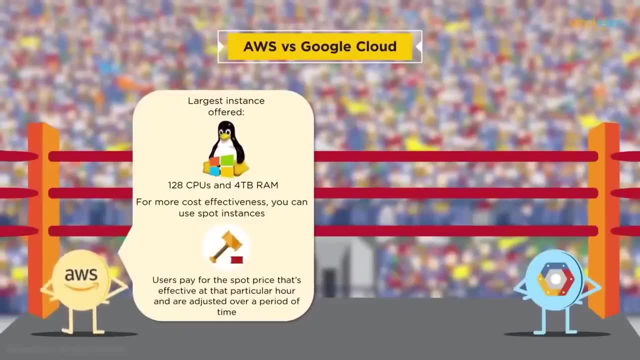 4 TVs of RAM. now, other than the on-demand method, like I mentioned before. on-demand method, like I mentioned before. on-demand method, like I mentioned before, you can also use spot instances. now you can also use spot instances now, you can also use spot instances now. these are four situations where your 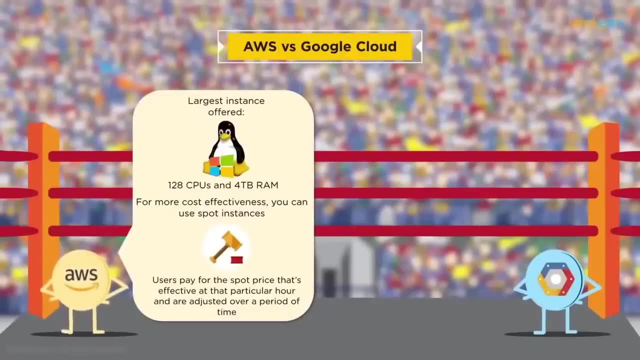 these are four situations where your- these are four situations where your application is more fault tolerant and application is more fault tolerant and application is more fault tolerant and can handle an interruption now you pay. can handle an interruption now you pay. can handle an interruption now you pay for the spot price which is effective at for the spot price which is effective at. for the spot price which is effective at a particular. are now these spot prices a particular? are now these spot prices a particular? are now these spot prices? do fluctuate, but are adjusted over a. do fluctuate, but are adjusted over a. 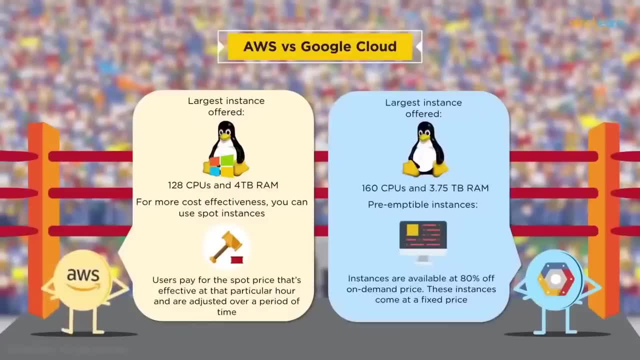 do fluctuate but are adjusted over a period of time. the largest instance period of time: the largest instance period of time. the largest instance offered with Google Cloud is 160 CPUs and offered with Google Cloud is 160 CPUs, and offered with Google Cloud is 160 CPUs and 3.75 TVs from like spot. instances of 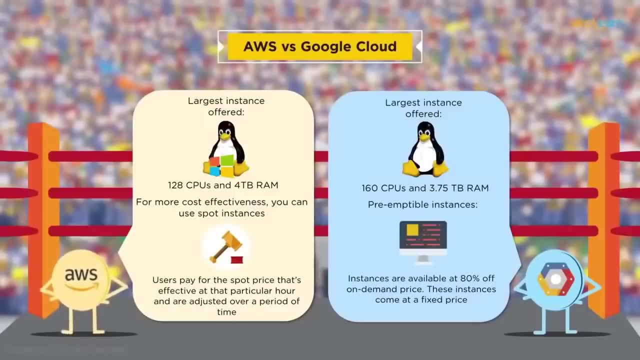 3.75 TVs from like spot. instances of 3.75 TVs from like spot. instances of AWS. Google Cloud offers short-lived compute AWS. Google Cloud offers short-lived compute AWS. Google Cloud offers short-lived compute instances suitable for bad jobs. instances suitable for bad jobs. 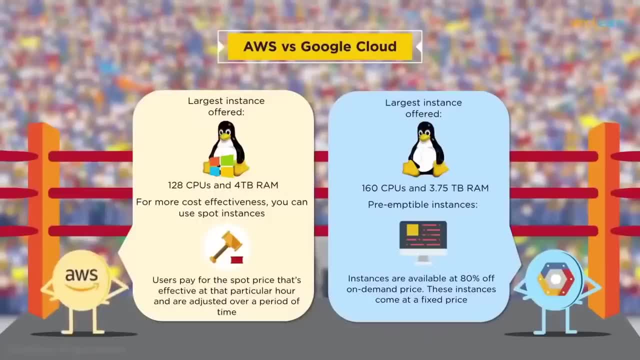 instances suitable for bad jobs and fault tolerant workloads. they are and fault tolerant workloads. they are, and fault tolerant workloads. they are called as preemptible instances, so these called as preemptible instances, so these called as preemptible instances, so these instances are available at 80% off on. 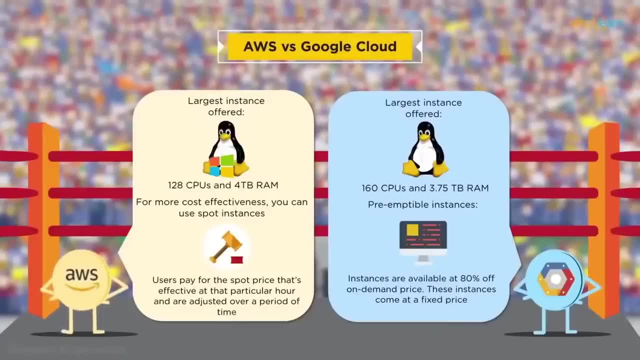 instances are available at 80% off on instances are available at 80% off on on-demand price. hence they reduce your on-demand price. hence they reduce your on-demand price. hence they reduce your compute engine costs significantly and compute engine costs significantly and compute engine costs significantly. and, unlike AWS, these come at a fixed price. 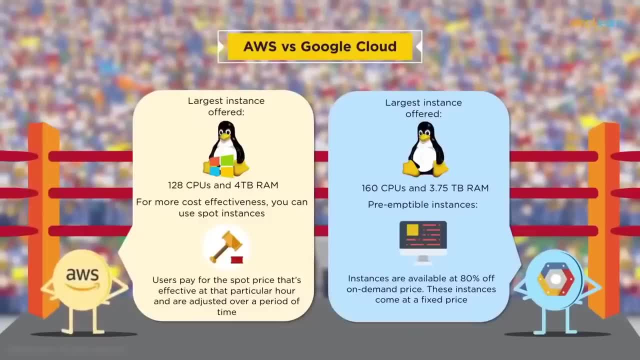 unlike AWS, these come at a fixed price. unlike AWS, these come at a fixed price. Google Cloud platform is a lot more. Google Cloud platform is a lot more. Google Cloud platform is a lot more flexible when it comes to instance flexible when it comes to instance flexible. when it comes to instance configuration, you simply choose your CPU. 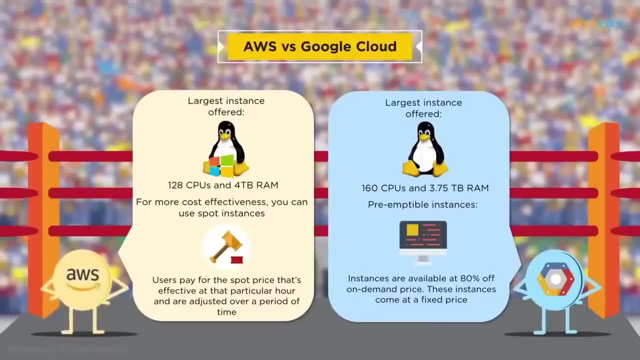 configuration. you simply choose your CPU configuration. you simply choose your CPU and RAM combination. of course you can. and RAM combination: of course you can. and RAM combination: of course you can even create your own instance types. this, even create your own instance types. this, even create your own instance types this way. before we wrap it up, let's compare. 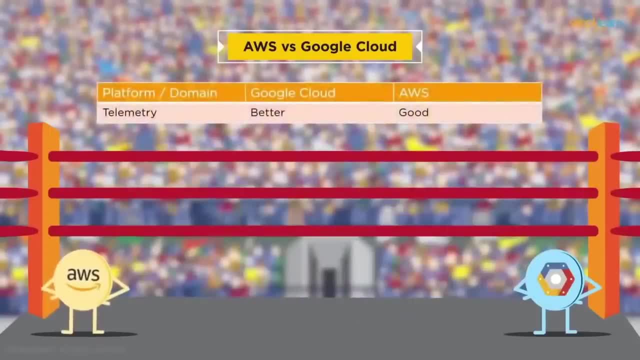 way before we wrap it up, let's compare. way before we wrap it up, let's compare on some other things as well. telemetry, on some other things as well. telemetry on some other things as well. telemetry, it's a process of automatically. it's a process of automatically. 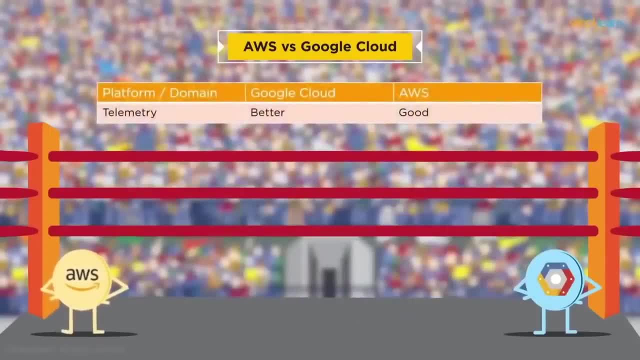 it's a process of automatically collecting periodic measurements. from collecting periodic measurements, from collecting periodic measurements from remote devices, for example, GPS GCP is remote devices. for example, GPS GCP is remote devices. for example, GPS GCP is obviously better because they have, obviously better because they have. 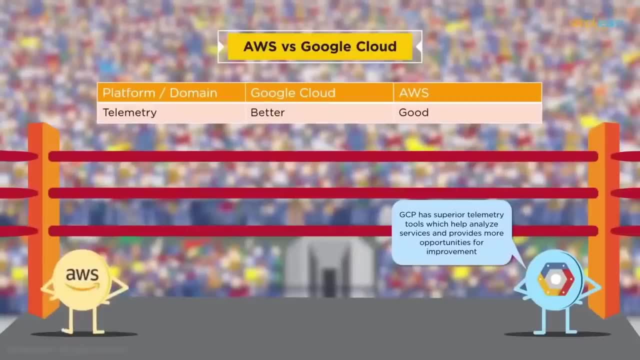 obviously better because they have superior telemetry tools which help in superior telemetry tools which help in superior telemetry tools which help in analyzing services and providing more analyzing services and providing more analyzing services and providing more opportunities for improvement when it opportunities for improvement, when it opportunities for improvement when it comes to application support. AWS is 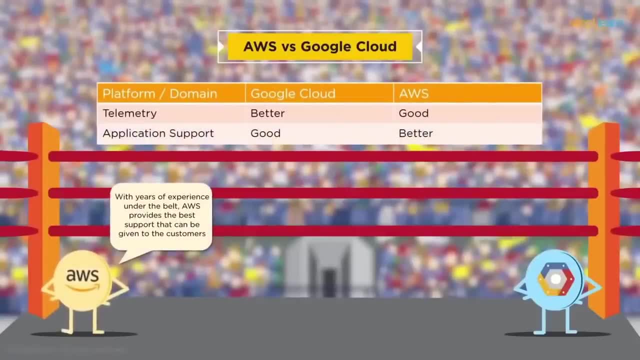 comes to application support, AWS is comes to application support, AWS is obviously better since they have years of obviously better, since they have years of obviously better, since they have years of experience under their bed. AWS provides experience under their bed. AWS provides experience under their bed. AWS provides the best support that can be given to 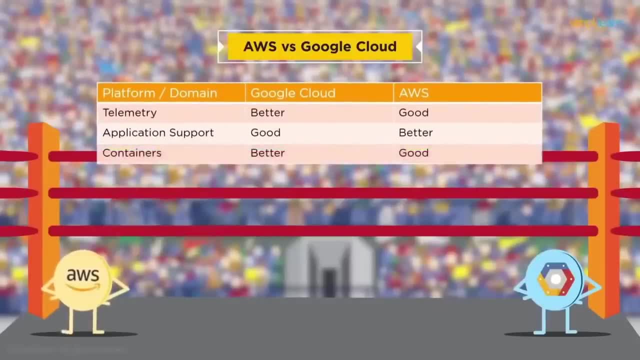 the best support that can be given to the best support that can be given to the customers. containers are better with the customers. containers are better with the customers. containers are better with GCP- a container is a virtual process. GCP- a container is a virtual process. GCP: a container is a virtual process running in user space. as cuban it is was. 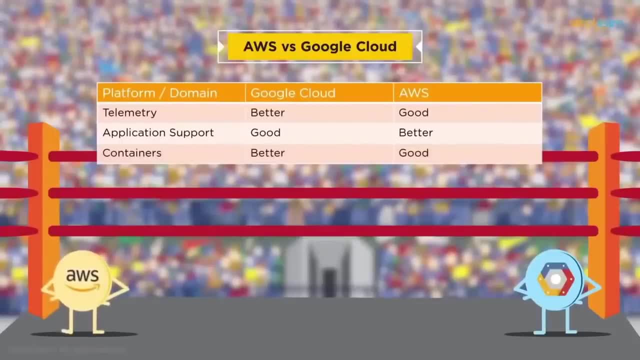 running in user space as cuban it is was running in user space as cuban it is was originally developed by Google. GCP has originally developed by Google. GCP has originally developed by Google. GCP has full native support for the tool other. full native support for the tool other. 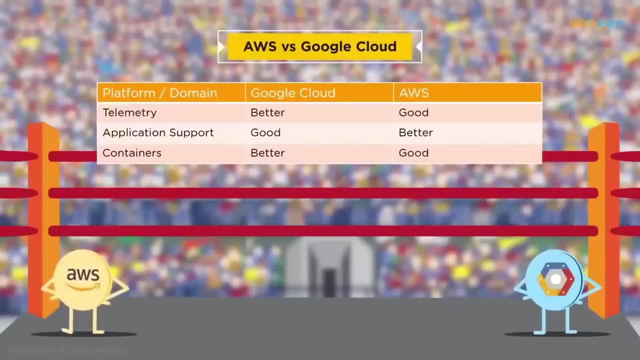 full native support for the tool. other cloud services are just fine-tuning a cloud services are just fine-tuning a. cloud services are just fine-tuning a way to provide human. it is as a service way to provide human. it is as a service way to provide human. it is as a service also, the containers help with. 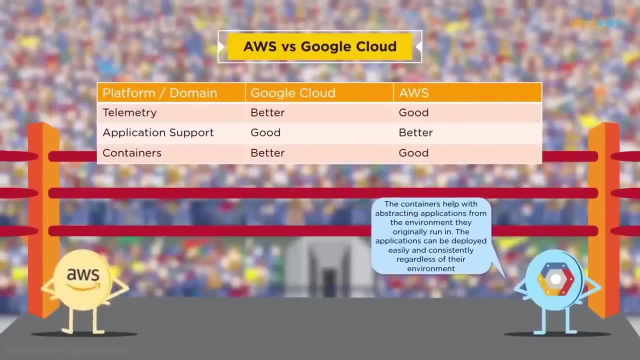 also the containers help with. also the containers help with abstracting applications from their abstracting applications, from their abstracting applications from their environment. they originally planet the environment. they originally planet the environment. they originally planet the applications can be deployed easily. applications can be deployed easily. applications can be deployed easily regardless of their environment when it. 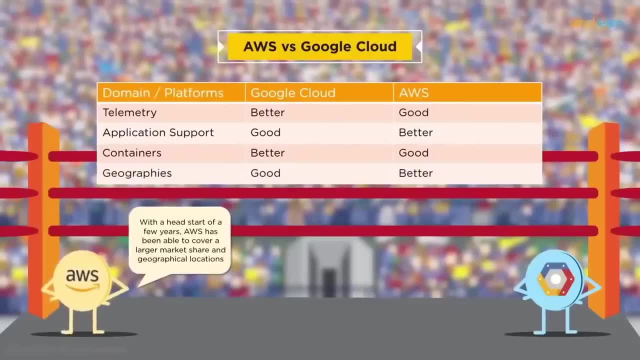 regardless of their environment, when it regardless of their environment. when it comes to geographies in a place is better. comes to geographies in a place is better. comes to geographies in a place is better, since they have a head start of a few, since they have a head start of a few. 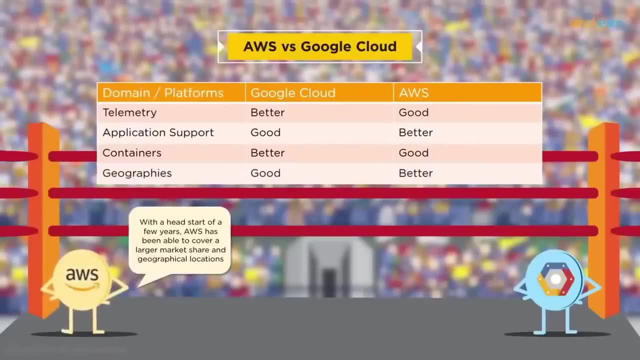 since they have a head start of a few years. AWS in this span of time has been years. AWS in this span of time has been years. AWS in this span of time has been able to cover a larger market share and able to cover a larger market share. and. 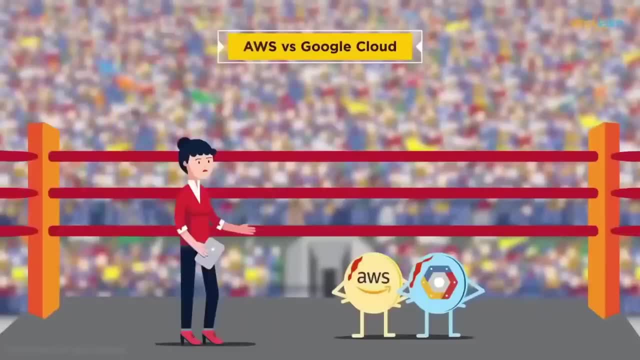 able to cover a larger market share and geographical locations. now it's time for geographical locations. now it's time for geographical locations. now it's time for the big decision. so who's going to be the big decision? so who's going to be the big decision? so who's going to be? yeah, who is it going to be? GCP or AWS? I? 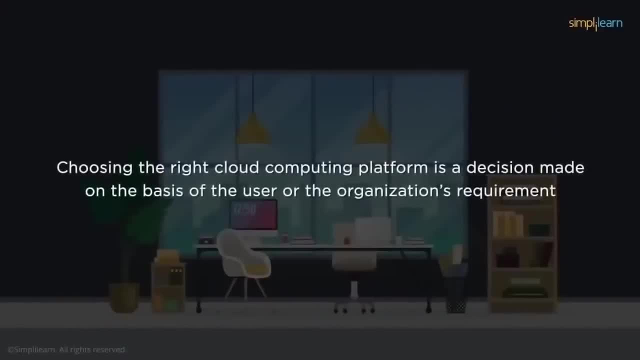 yeah, who is it going to be? GCP or AWS? I yeah, who is it going to be GCP or AWS? I think I'm going to go for choosing the think I'm going to go for choosing the think I'm going to go for. choosing the right cloud computing platform is the. 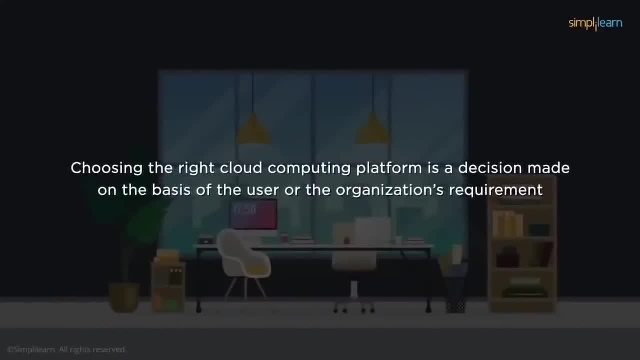 right cloud computing platform. is the right cloud computing platform? is the decision that's made on the basis of the decision that's made on the basis of the decision that's made on the basis of the user or the organization's requirement? user or the organization's requirement. 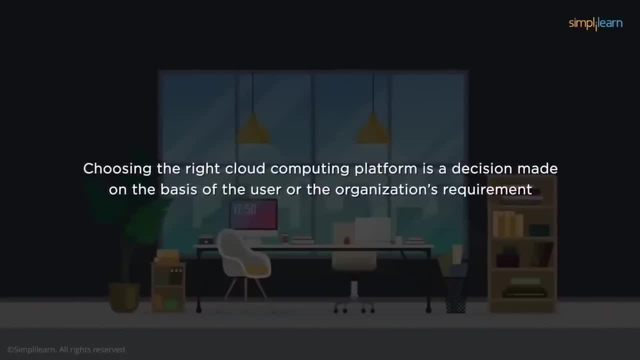 user or the organization's requirement. on that note. I believe it's time for us on that note. I believe it's time for us. on that note. I believe it's time for us to wrap this video up. we hope you guys to wrap this video up. we hope you guys. 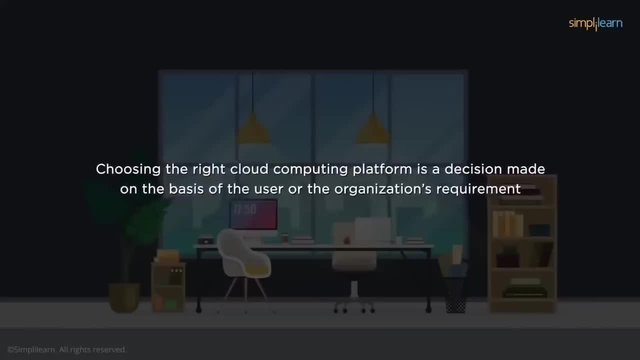 to wrap this video up, we hope you guys enjoy this video and learn something new. enjoy this video and learn something new. enjoy this video and learn something new: that AWS is better right. know that that AWS is better right. know that that AWS is better right. know that choosing a platform entirely depends on. 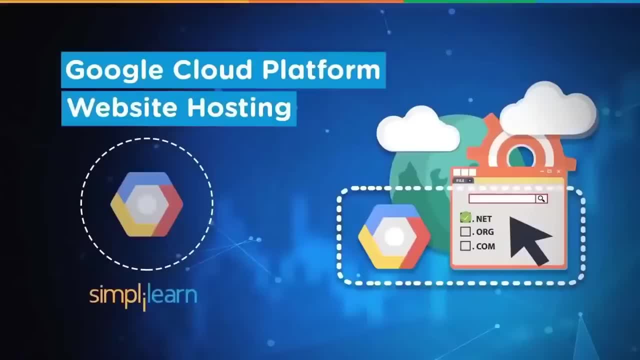 choosing a platform entirely depends on choosing a platform entirely depends on you and your organization's requirement. you and your organization's requirement, you and your organization's requirement. hello everyone. welcome to the session on hello everyone, welcome to the session on hello everyone, welcome to the session on Google cloud platform. website hosting. 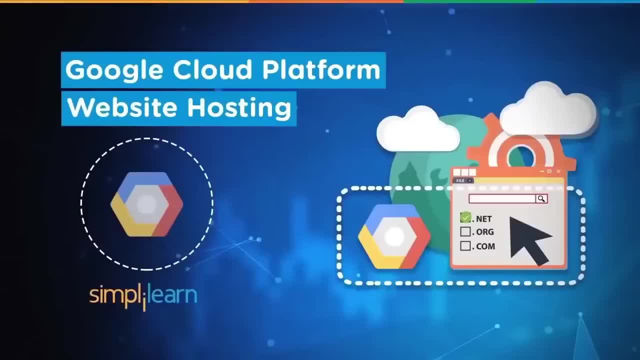 Google cloud platform website hosting. Google cloud platform website hosting, and let's understand what Google cloud and let's understand what Google cloud and let's understand what Google cloud platform offers when it comes to your platform offers, when it comes to your platform offers when it comes to your web hosting requirements. here we will. 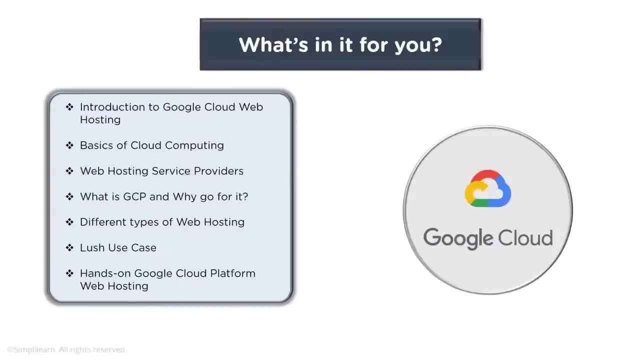 web hosting requirements: here we will web hosting requirements. here we will learn about Google cloud web hosting. some learn about Google cloud web hosting. some learn about Google cloud web hosting. some basics of cloud computing web hosting. basics of cloud computing web hosting. basics of cloud computing web hosting service providers. what is GCP and why go? 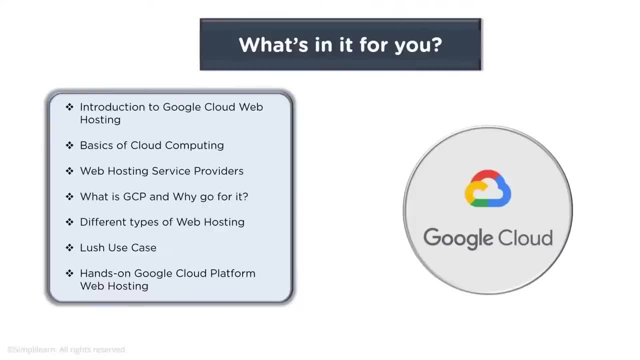 service providers. what is GCP and why go service providers? what is GCP and why go for it? different types of web hosting for it. different types of web hosting for it. different types of web hosting which are possible. a use case such as: which are possible. a use case such as: 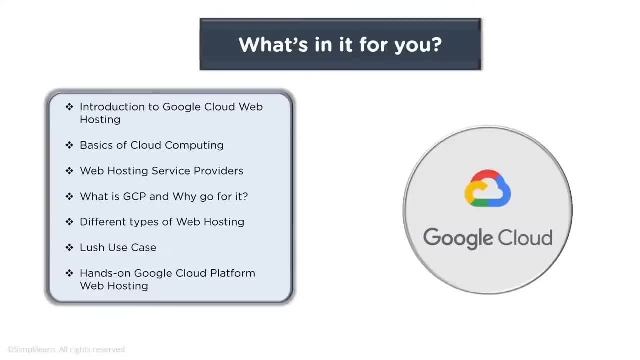 which are possible: a use case such as lush and a quick hands-on on using GCP lush and a quick hands-on on using GCP lush and a quick hands-on on using GCP for web hosting. when you talk about for web hosting, when you talk about 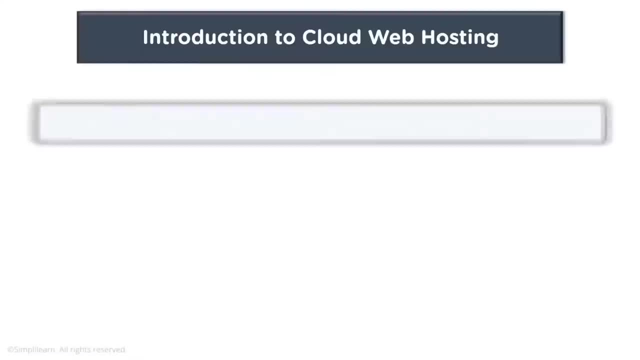 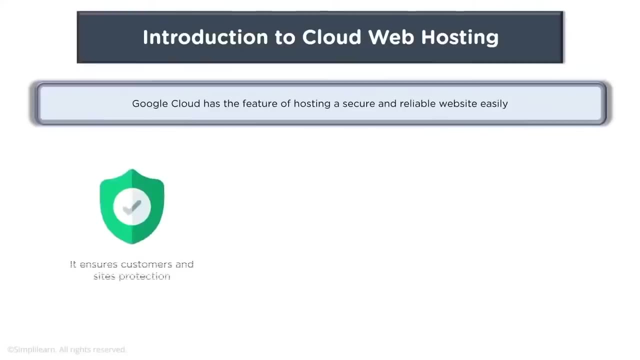 for web hosting. when you talk about cloud web hosting, Google Cloud has the cloud web hosting. Google Cloud has the cloud web hosting. Google Cloud has the feature of hosting a secure and reliable feature of hosting a secure and reliable feature of hosting a secure and reliable websites easily. it ensures customers and. 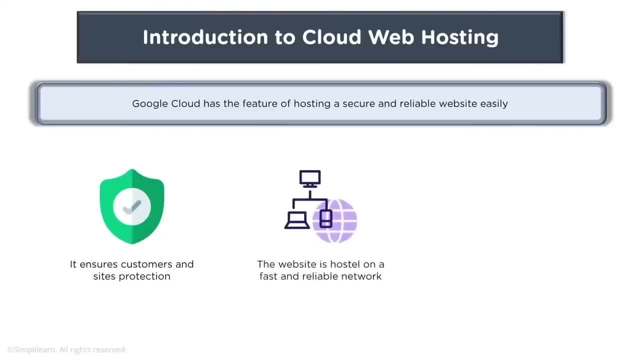 websites easily. it ensures customers and websites easily. it ensures customers and sites protection. the website is a is sites protection. the website is a is sites protection. the website is a is hosted on a fast and reliable network. hosted on a fast and reliable network. hosted on a fast and reliable network, you can do more work for less price with. 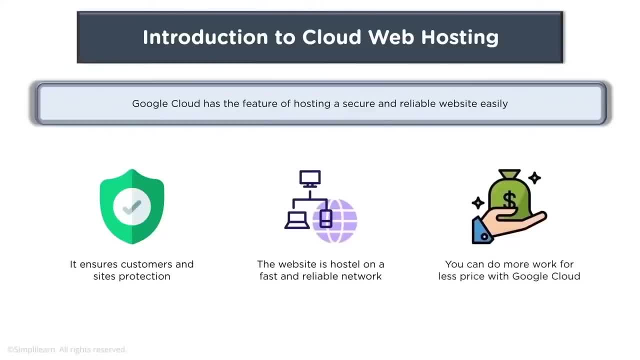 you can do more work for less price with. you can do more work for less price with Google Cloud. now, when we talk about Google Cloud, now when we talk about Google Cloud, now when we talk about Google Cloud, it is always good to know Google Cloud, it is always good to know. 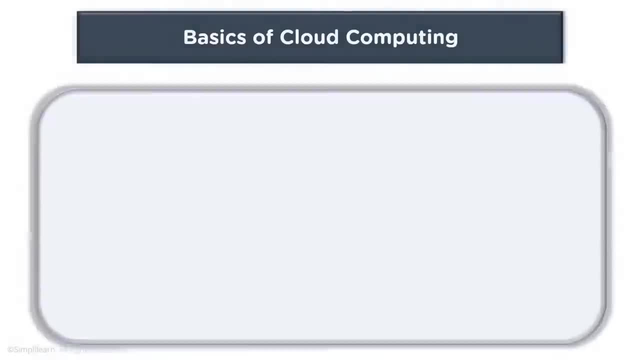 Google Cloud. it is always good to know some basics over cloud computing now, some basics over cloud computing now, some basics over cloud computing. now, when we talk about cloud computing cloud, when we talk about cloud computing cloud, when we talk about cloud computing, cloud computing is basically using resources. 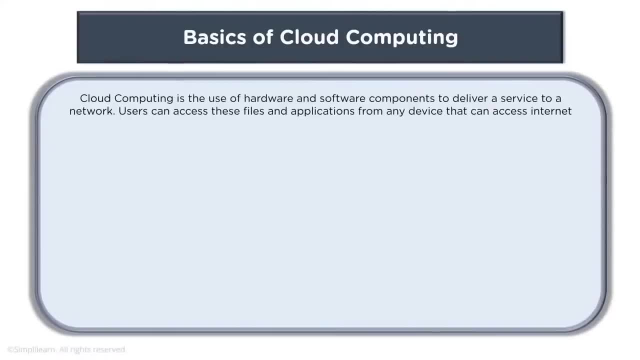 computing is basically using resources. computing is basically using resources which are provided by your cloud service, which are provided by your cloud service, which are provided by your cloud service provider, such as Google Cloud, and cloud provider such as Google Cloud and cloud provider such as Google Cloud. and cloud computing basically means using. 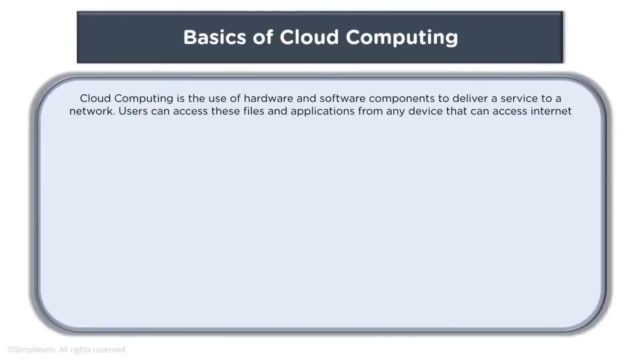 computing basically means using. computing basically means using hardware and software components to hardware and software components. to hardware and software components to deliver a service on a network- now here. deliver a service on a network- now here. deliver a service on a network. now here users can access files, applications from. 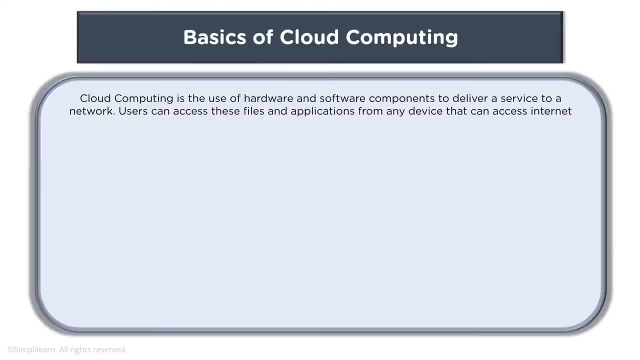 users can access files, applications from. users can access files, applications from any device that can access Internet. so any device that can access Internet, so any device that can access Internet. so when we talk about cloud computing, this, when we talk about cloud computing, this, when we talk about cloud computing, this is basically using services which are 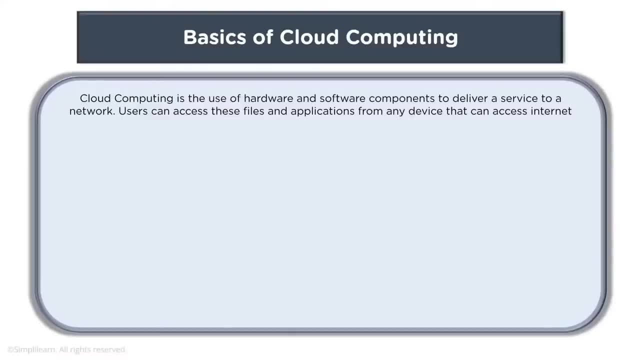 is basically using services which are is basically using services which are hosted on the infrastructure managed by hosted on the infrastructure managed by hosted on the infrastructure managed by cloud provider. when we talk about cloud provider, when we talk about cloud provider, when we talk about resources which can be used, that may 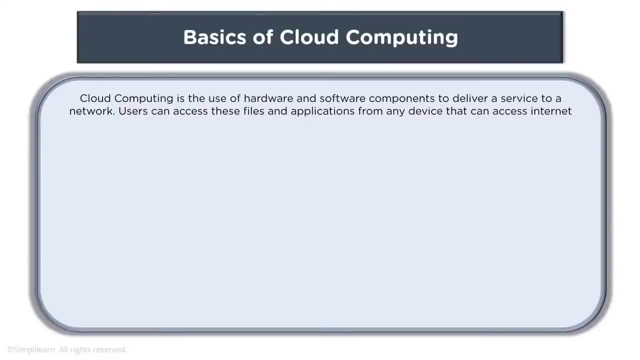 resources which can be used. that may resources which can be used. that may include big data services. storage options. include big data services. storage options. include big data services. storage options. you are computing options, networking. you are computing options, networking, you are computing options, networking options and various other services which. 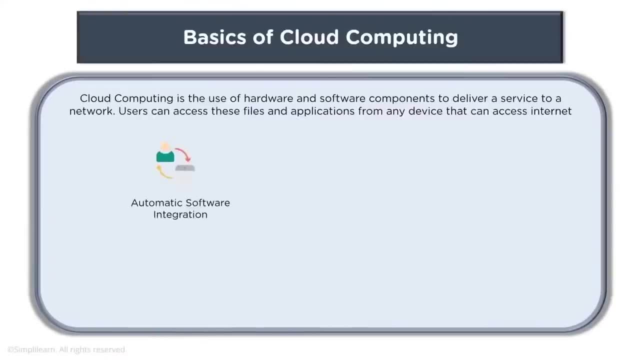 options and various other services. which options and various other services which a cloud provider offers cloud computing. a cloud provider offers cloud computing. a cloud provider offers cloud computing. has various different service models. has various different service models. has various different service models, such as you have platform as a service. 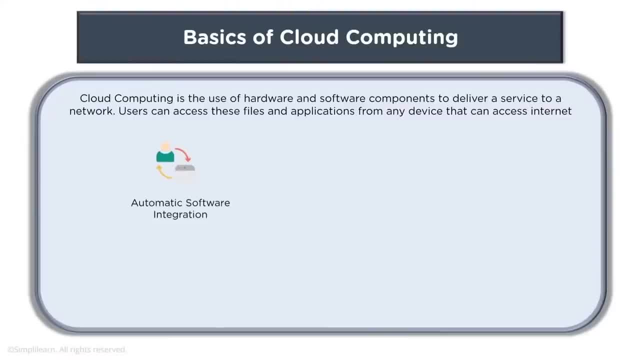 such as you have platform as a service, such as you have platform as a service, software as a service, infrastructure as a software as a service, infrastructure as a software as a service, infrastructure as a service. also these days we talk about service. also these days we talk about 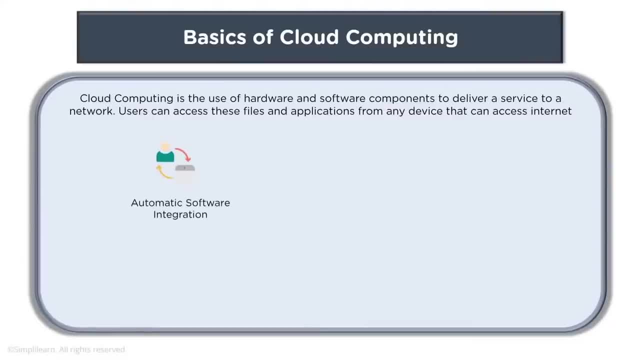 service. also, these days, we talk about containers as a service and these are containers as a service and these are containers as a service. and these are your different computing service models, your different computing service models, your different computing service models which are being offered by cloud service, which are being offered by cloud service. 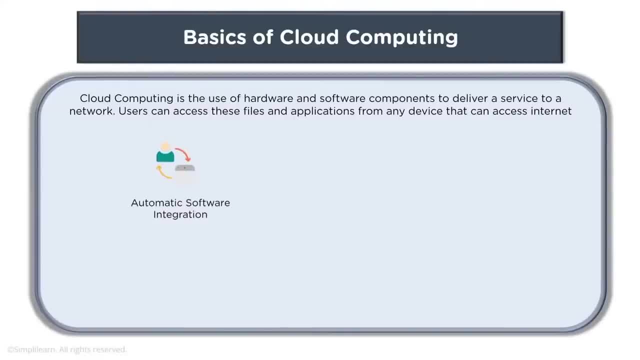 which are being offered by cloud service providers, which allow you for automatic providers, which allow you for automatic providers which allow you for automatic integration with your existing integration, with your existing integration with your existing environment, or if you would want to environment, or if you would want to. 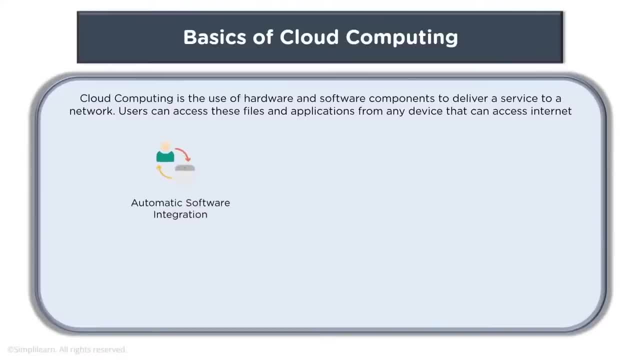 environment, or if you would want to benefit from modernization by using a benefit from modernization, by using a benefit from modernization by using a cloud providers infrastructure. you have cloud providers infrastructure. you have cloud providers infrastructure. you have different services which are offered some different services which are offered some. 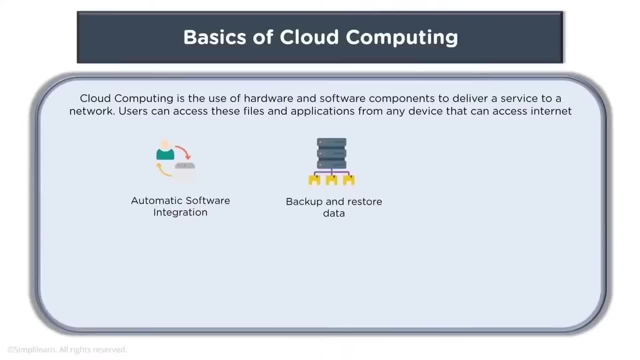 different services which are offered. some of them are for auto software, of them are for auto software. of them are for auto software. integration or migration backing up and integration or migration backing up and integration or migration backing up and restoring data. scaling your storage. restoring data. scaling your storage. 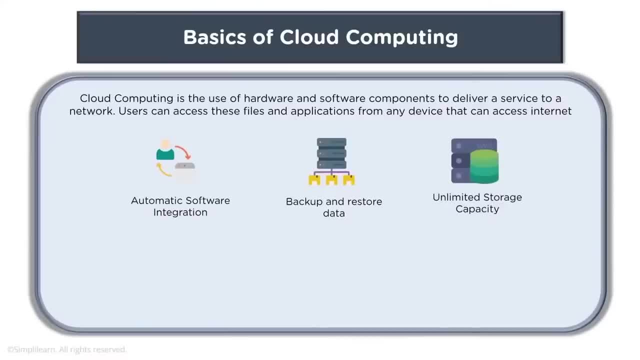 restoring data, scaling your storage capacity. that is going for an unlimited capacity. that is going for an unlimited capacity, that is going for an unlimited storage capacity. and using a resource storage capacity and using a resource storage capacity and using a resource provided by cloud service provider: provided by cloud service provider. 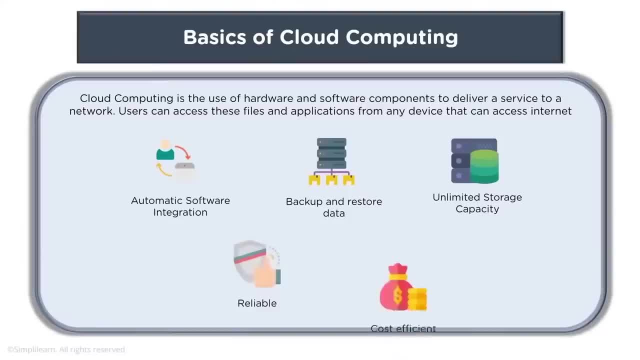 provided by cloud service provider. benefiting from reliability: cost benefiting from reliability: cost benefiting from reliability- cost efficiency, which is offered by a cloud efficiency, which is offered by a cloud efficiency which is offered by a cloud provider. in this case, we are talking provider. in this case, we are talking. 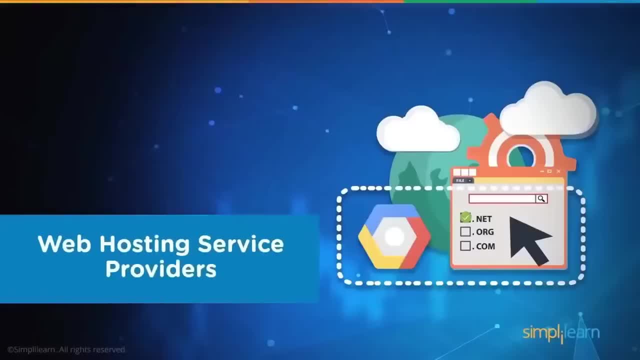 provider. in this case, we are talking about Google Cloud. when you talk about about Google Cloud, when you talk about about Google Cloud, when you talk about web hosting service providers, there are web hosting service providers. there are web hosting service providers. there are various web hosting service providers. 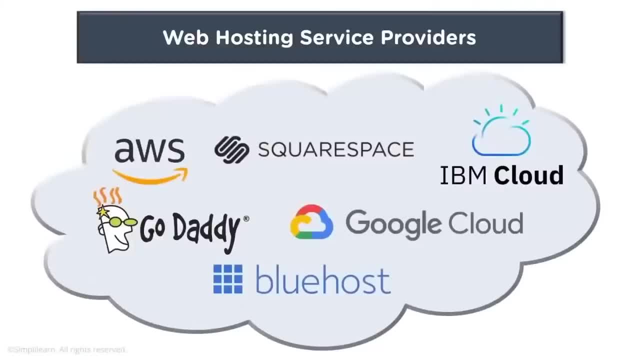 various web hosting service providers. various web hosting service providers. you have AWS. you have Squarespace IBM. you have AWS. you have Squarespace IBM. you have AWS. you have Squarespace IBM. cloud, GoDaddy, Bluehost and Google Cloud cloud, GoDaddy, Bluehost and Google Cloud. 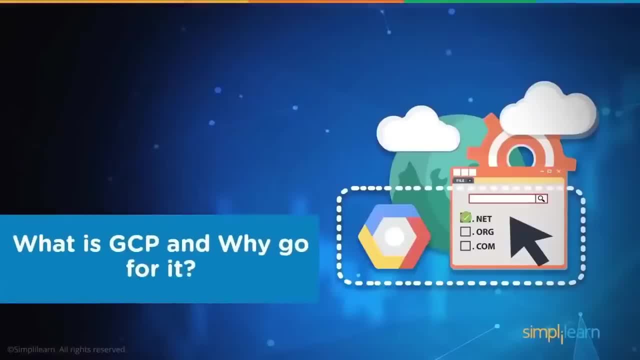 cloud: GoDaddy, Bluehost and Google Cloud. so what is GCP and why go for it? when? so, what is GCP and why go for it when? so what is GCP and why go for it? when you talk about GCP, or as we call it, as 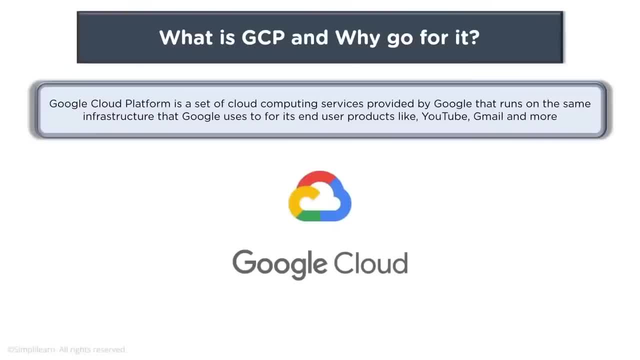 you talk about GCP or as we call it. as you talk about GCP, or as we call it as Google Cloud Platform, it is set of cloud- Google Cloud Platform. it is set of cloud- Google Cloud Platform. it is set of cloud computing services provided by Google. 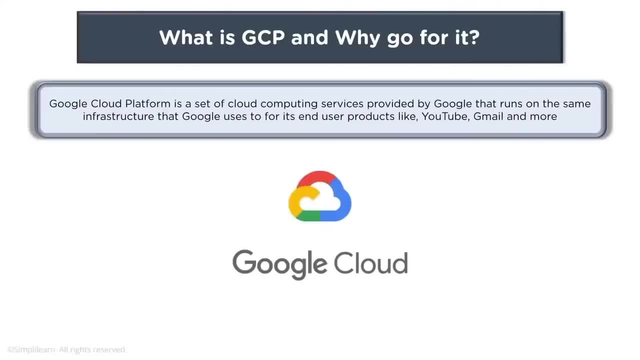 computing services provided by Google. computing services provided by Google that runs on the same infrastructure that. that runs on the same infrastructure that Google uses for it end-user products. Google uses for it end-user products. Google uses for it end-user products like YouTube, Gmail and much more. when you 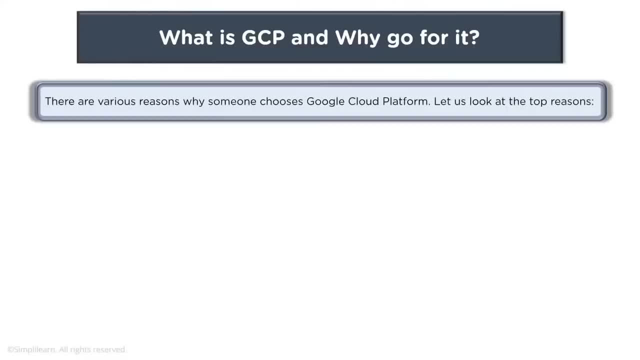 like YouTube, Gmail and much more, when you like YouTube, Gmail and much more. when you talk about GCP: there are various talk about GCP. there are various talk about GCP. there are various reasons why anyone would choose it. for reasons why anyone would choose it for. 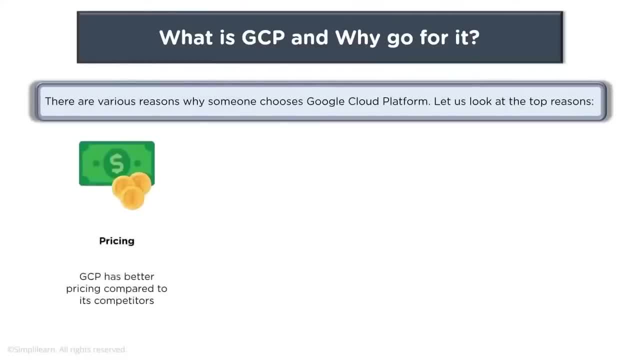 reasons why anyone would choose it for their use cases. now let's look at some their use cases. now let's look at some their use cases. now. let's look at some reasons when you talk about pricing- GCP reasons when you talk about pricing- GCP reasons when you talk about pricing: GCP has better pricing compared to its. 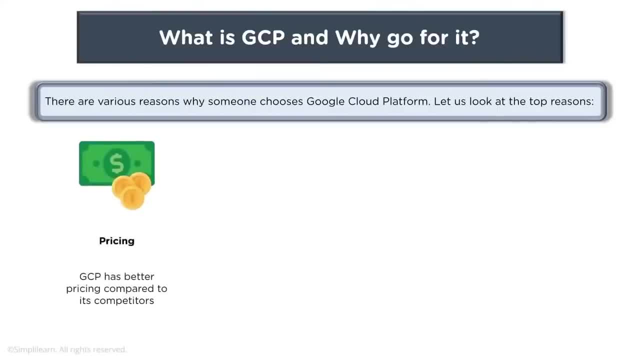 has better pricing compared to its. has better pricing compared to its competitors, depending on the services competitors, depending on the services competitors, depending on the services which you would use, whether that would which you would use, whether that would which you would use, whether that would and running your applications on them, or 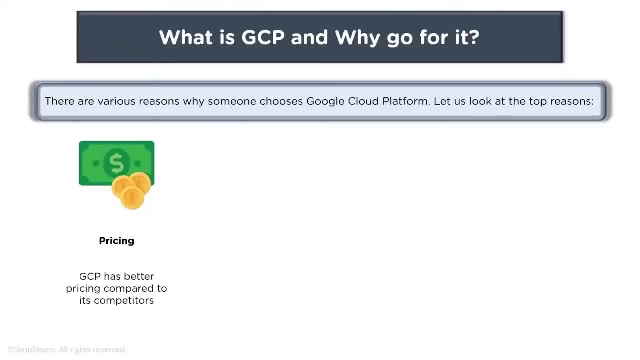 and running your applications on them, or and running your applications on them, or might be a managed service, such as data might be a managed service, such as data might be a managed service, such as data. proc or big table or your big query. proc or big table or your big query. 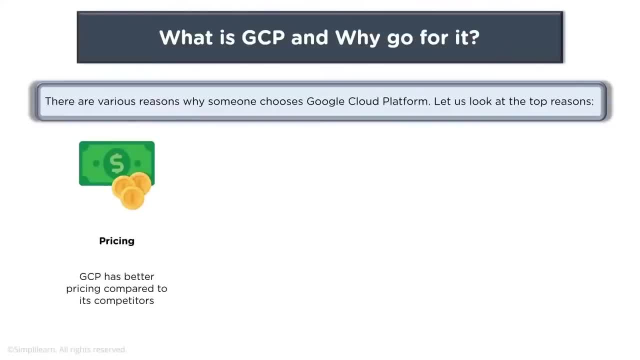 proc or big table or your big query where you can have your Hadoop clusters, where you can have your Hadoop clusters, where you can have your Hadoop clusters running or store huge amount of data, or running or store huge amount of data, or running or store huge amount of data, or even build your data warehouse wherein 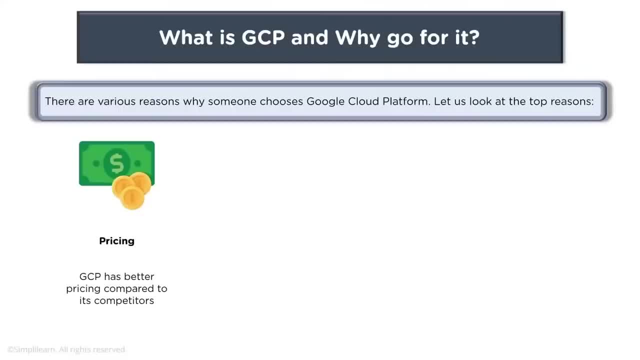 even build your data warehouse wherein. even build your data warehouse wherein you can store structured data. so there you can store structured data. so there you can store structured data. so there are different services with GCP offers are different services with GCP offers are different services with GCP offers and pricing has been a better option in. 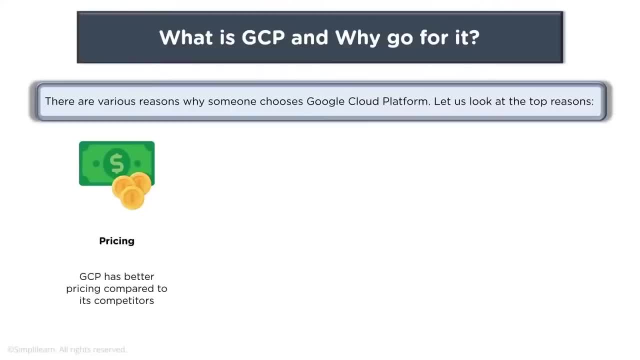 and pricing has been a better option in, and pricing has been a better option in case of Google in comparison to other case of Google, in comparison to other case of Google, in comparison to other competitors. when you talk about speed competitors, when you talk about speed competitors, when you talk about speed and performance, it's very fast and 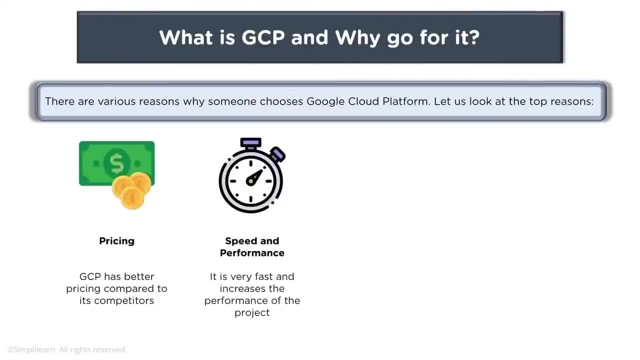 and performance- it's very fast. and and performance: it's very fast and increases the performance of your project. increases the performance of your project. increases the performance of your project if you use different services offered by, if you use different services offered by. if you use different services offered by Google. 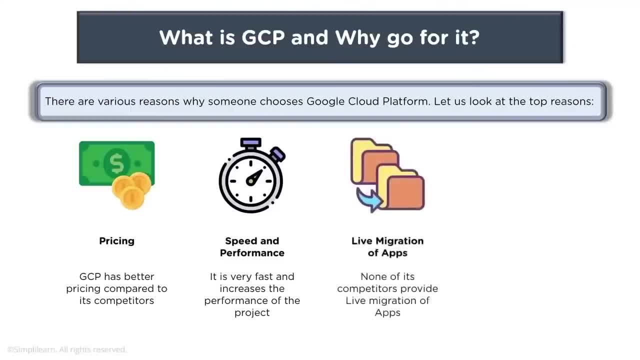 Google, Google. when you talk about live migration of when you talk about live migration of when you talk about live migration of apps, this is one of the features which apps. this is one of the features which apps. this is one of the features which organizations usually like, which none of 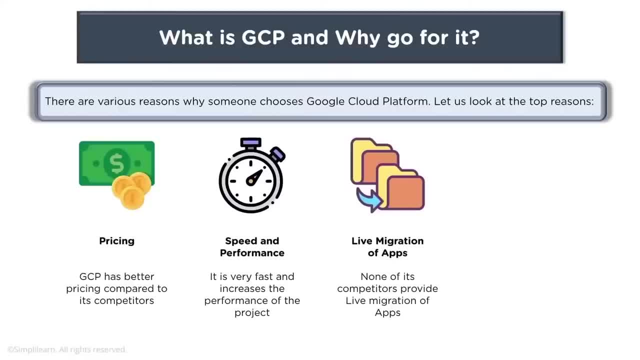 organizations usually like which, none of organizations usually like which, none of the application of apps. so there are the application of apps, so there are the application of apps. so there are specific features. for example, when you specific features, for example, when you specific features, for example, when you talk about computer engine, there is a 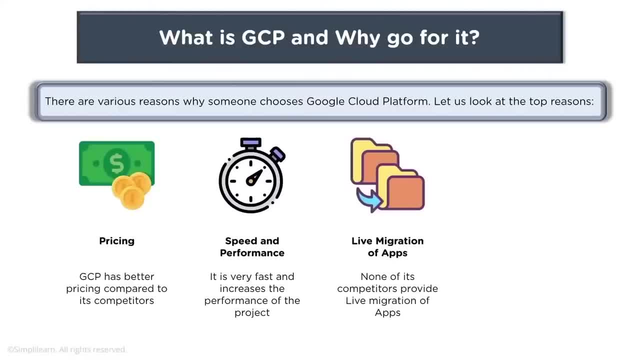 talk about computer engine. there is a talk about computer engine. there is a feature stating live migration, wherein feature stating live migration, wherein feature stating live migration wherein your resources or your instances, which your resources or your instances, which your resources or your instances which are running applications, would be. 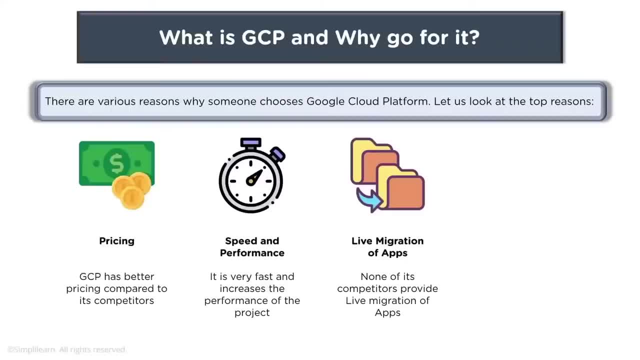 are running applications would be. are running applications would be migrated during, say, maintenance from one migrated during, say, maintenance from one. migrated during, say, maintenance from one underlying host to another underlying underlying host to another. underlying underlying host to another underlying host without affecting your applications. host without affecting your applications. 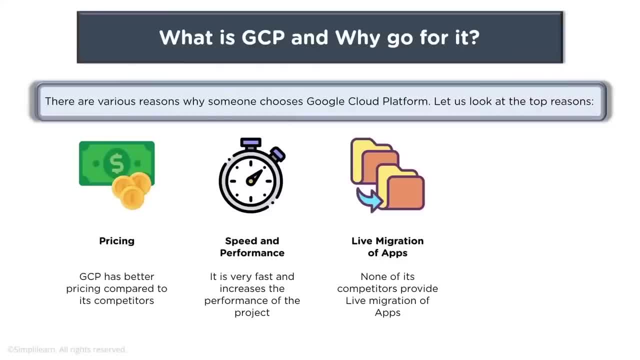 host without affecting your applications performance, and you can benefit from that. when you talk about big data- Google, when you talk about big data Google, when you talk about big data, Google Cloud has various offerings in big data. Cloud has various offerings in big data. Cloud has various offerings in big data space, and that's one of the advantages. 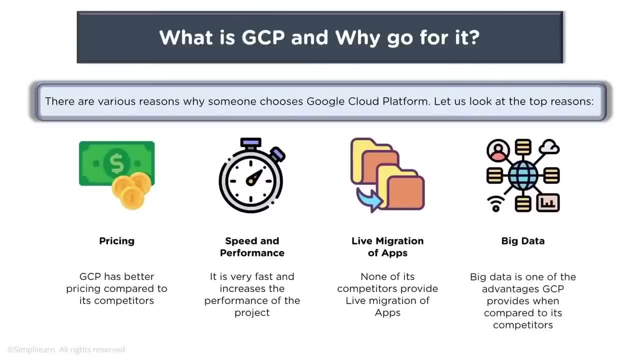 space, and that's one of the advantages. space and that's one of the advantages of GCP in comparison to other competitors of GCP. in comparison to other competitors of GCP. in comparison to other competitors, you have different services for your big. you have different services for your big. 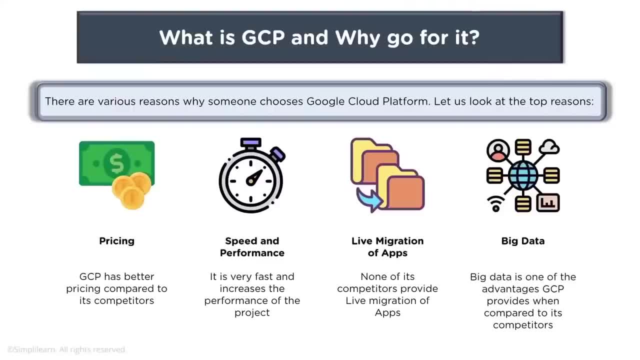 you have different services for your big data needs, such as pub sub for publish data needs, such as pub sub for publish data needs, such as pub sub for publish subscribing messaging system or going subscribing messaging system, or going subscribing messaging system or going for data proc, which basically allows you. 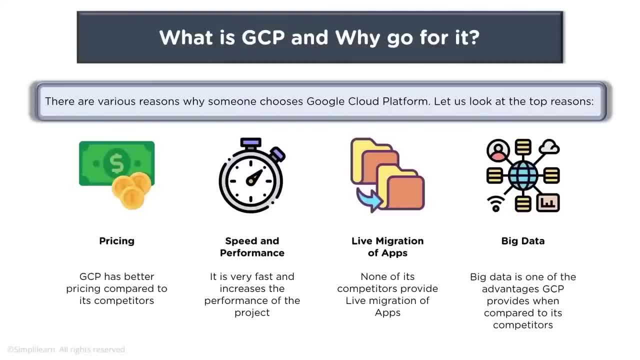 for data proc, which basically allows you for data proc, which basically allows you to spin up your Hadoop and spark to spin up your Hadoop and spark, to spin up your Hadoop and spark clusters to run your different jobs and clusters to run your different jobs. and. 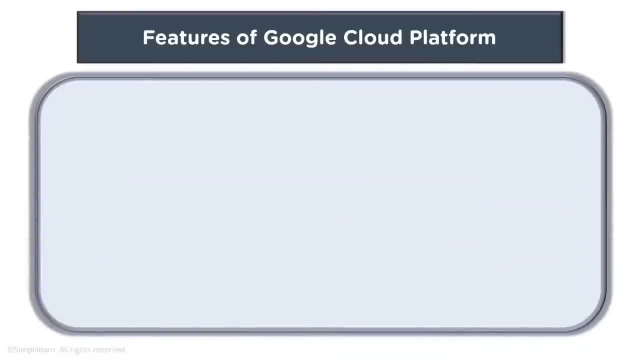 clusters to run your different jobs and so on. so when we talk about features of so on, so when we talk about features of so on, so when we talk about features of Google Cloud Platform, it offers high Google Cloud Platform. it offers high Google Cloud Platform. it offers high productivity because you are using the 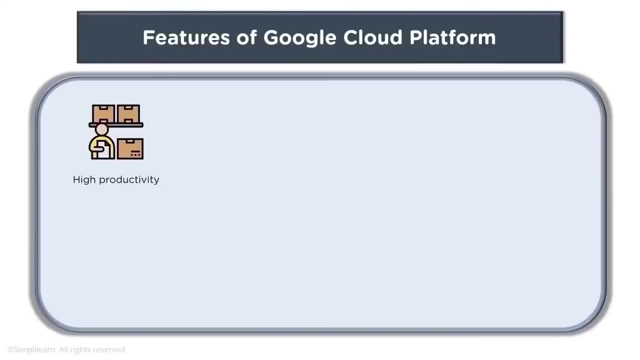 productivity, because you are using the productivity, because you are using the resources which are based on the same resources, which are based on the same resources which are based on the same infrastructure which Google uses for its infrastructure, which Google uses for its infrastructure, which Google uses for its own different use cases, you can work. 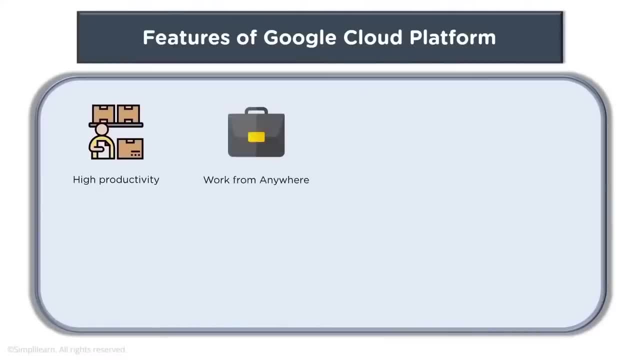 own different use cases. you can work, own different use cases. you can work from anywhere, provided you have internet from anywhere. provided you have internet from anywhere, provided you have internet connection and you can connect to the connection, and you can connect to the connection and you can connect to the cloud platform and use different services. 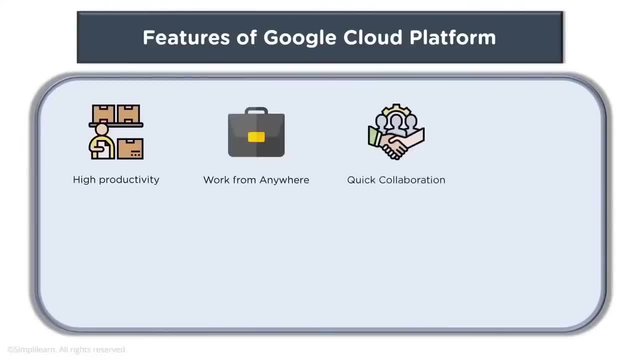 cloud platform and use different services. cloud platform and use different services offered via web. you can quickly offered via web. you can quickly offered via web. you can quickly collaborate with different teams or collaborate with different teams or collaborate with different teams or different colleagues working on different, different colleagues working on different. 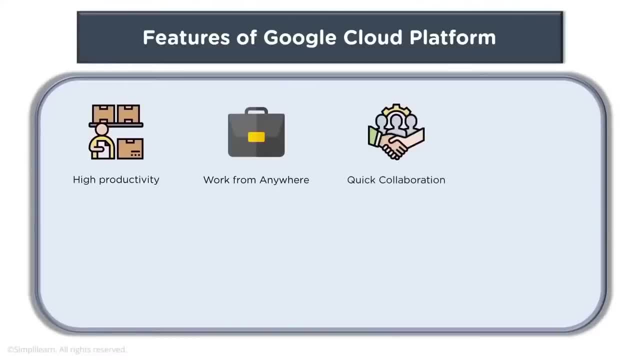 different colleagues working on different projects which might be sharing, projects which might be sharing, projects which might be sharing or using different GCP resources. you are or using different GCP resources. you are, or using different GCP resources. you are benefiting from high security, and benefiting from high security, and. 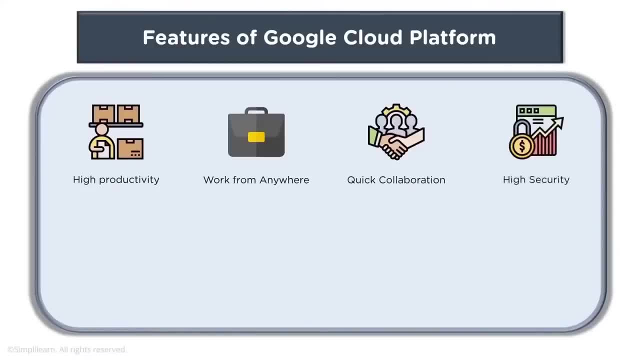 benefiting from high security and different encryption and security. different encryption and security, different encryption and security. mechanisms with GCP offers. now there are mechanisms with GCP offers. now there are mechanisms with GCP offers. now there are fewer sources or you could say data. fewer sources or you could say data. 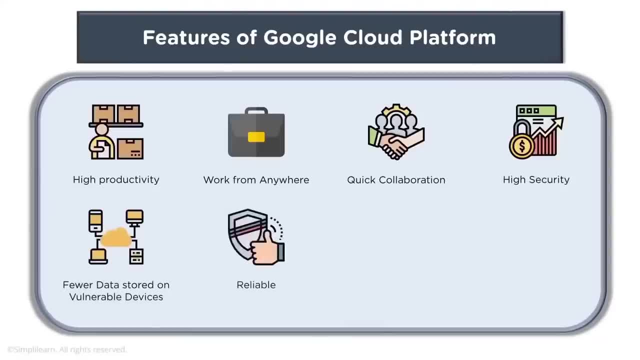 fewer sources, or you could say data which is stored or vulnerable devices which is stored, or vulnerable devices which is stored, or vulnerable devices. there is high reliability, flexibility, or there is high reliability, flexibility, or there is high reliability, flexibility or scalability, which GCP offers and the cost. 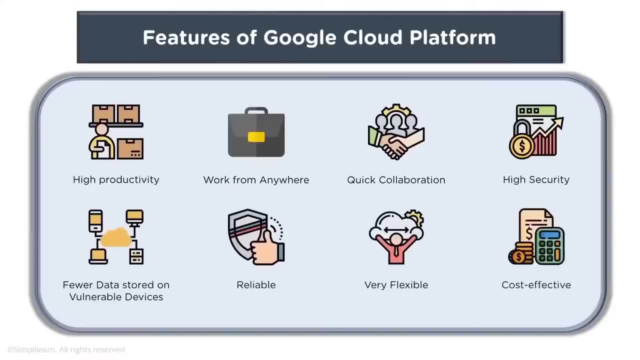 scalability which GCP offers and the cost scalability which GCP offers, and the cost effectiveness really makes it as a good effectiveness, really makes it as a good effectiveness, really makes it as a good choice when you would want to benefit, choice when you would want to benefit. 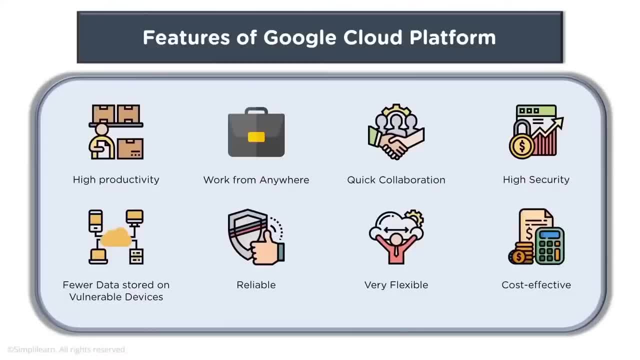 choice when you would want to benefit from infrastructure modernization and from infrastructure modernization and from infrastructure modernization and using a cloud platform solution for your, using a cloud platform solution for your, using a cloud platform solution for your use case- now when you talk about use case, now when you talk about. 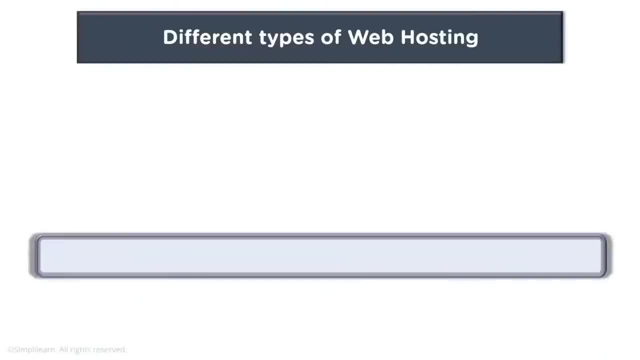 use case now when you talk about different types of web hosting, Google, different types of web hosting, Google, different types of web hosting. Google Cloud offers three types of web hosting. Cloud offers three types of web hosting. Cloud offers three types of web hosting. you have WordPress now. it is a free and 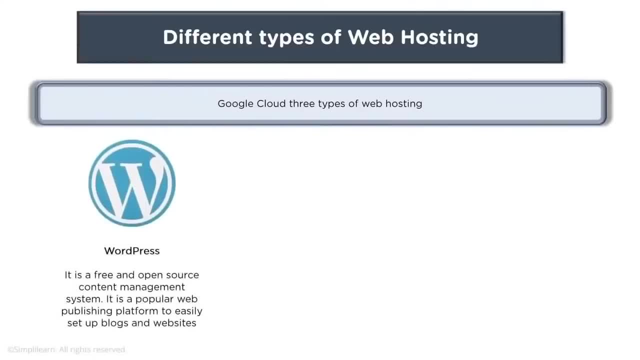 you have WordPress now it is a free. and you have WordPress now it is a free and open source content management system. open source content management system. open source content management system you might have used in past or have you might have used in past, or have you might have used in past, or have heard about WordPress, where a lot of 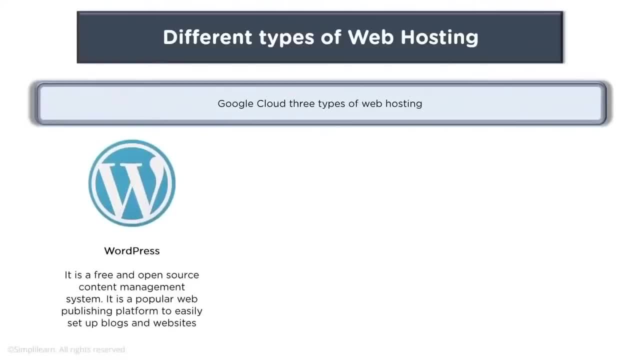 heard about WordPress, where a lot of heard about WordPress, where a lot of websites are being created. it is a websites are being created. it is a websites are being created. it is a popular web publishing platform to easily popular web publishing platform to easily popular web publishing platform to easily set up blogs and websites and thus used. 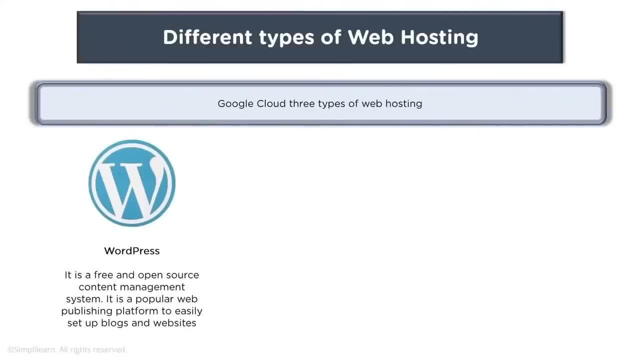 set up blogs and websites and thus used. set up blogs and websites and thus used by organizations or even individual by organizations, or even individual by organizations, or even individual users for having their blogs or running users for having their blogs or running users for having their blogs or running their websites or promoting their. 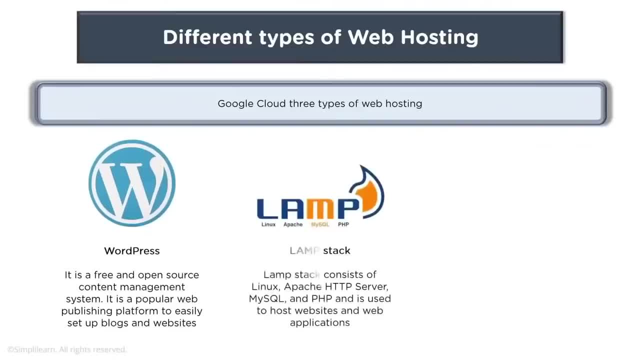 their websites or promoting their their websites or promoting their products. you have lamp which stands for products. you have lamp which stands for products. you have lamp which stands for Linux, Apache, MySQL and PHP, and lamp Linux, Apache, MySQL and PHP, and lamp Linux, Apache, MySQL and PHP, and lamp stack consists of Linux, Apache, HTTP. 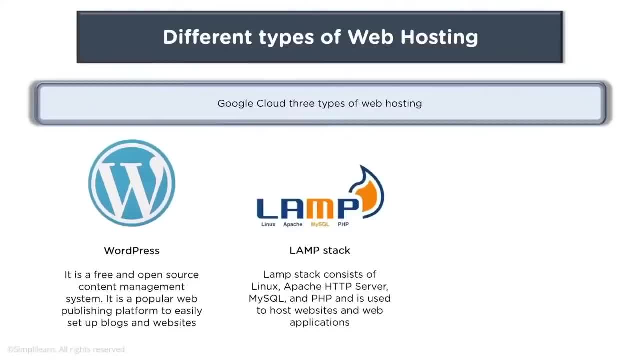 stack consists of Linux Apache. HTTP stack consists of Linux Apache HTTP server, MySQL and PHP, and is used to host server MySQL and PHP. and is used to host server MySQL and PHP, and is used to host websites and web applications. you also websites and web applications. you also. 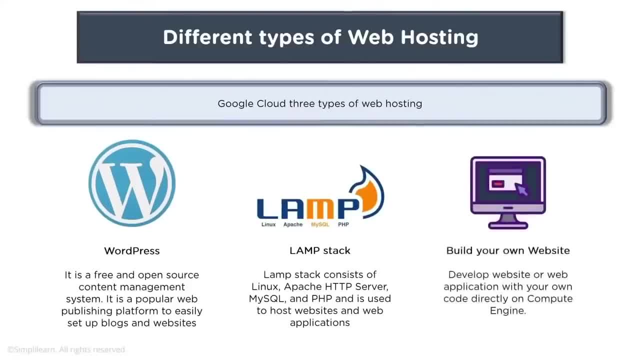 websites and web applications. you also have your option of building your own. have your option of building your own. have your option of building your own website so you can develop website or web website. so you can develop website or web website. so you can develop website or web application with your own code. 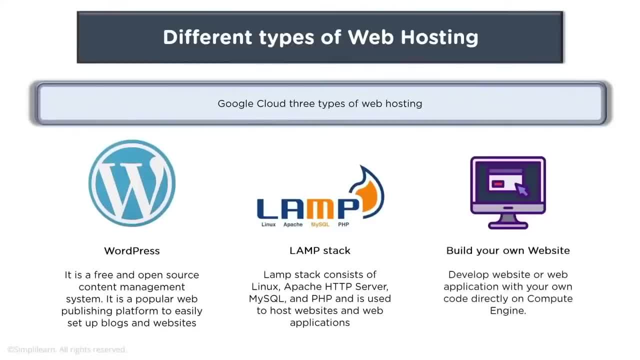 application with your own code. application with your own code directly on Compute Engine. now, let's look directly on Compute Engine. now let's look directly on Compute Engine. now let's look at a use case and understand what at a use case, and understand what at a use case and understand what happened here when we talk about lush. so 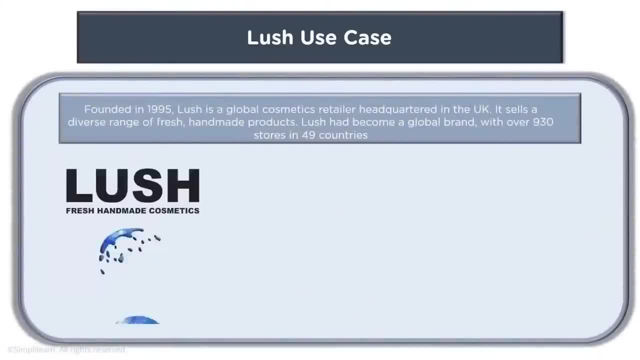 happened here when we talk about lush. so happened here when we talk about lush. so lush was founded in 1995, it's you might. lush was founded in 1995, it's you might. lush was founded in 1995. it's you might have seen this brand somewhere in the 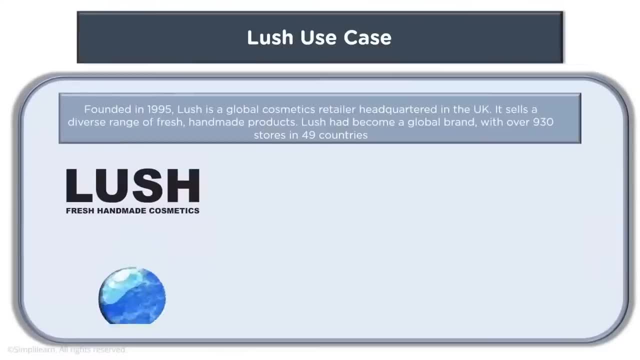 have seen this brand somewhere in the. have seen this brand somewhere in the streets. it is a global cosmetics retailer streets. it is a global cosmetics retailer streets. it is a global cosmetics retailer headquartered in UK. it sells a diverse headquartered in UK. it sells a diverse headquartered in UK. it sells a diverse range of fresh handmade products- lush. 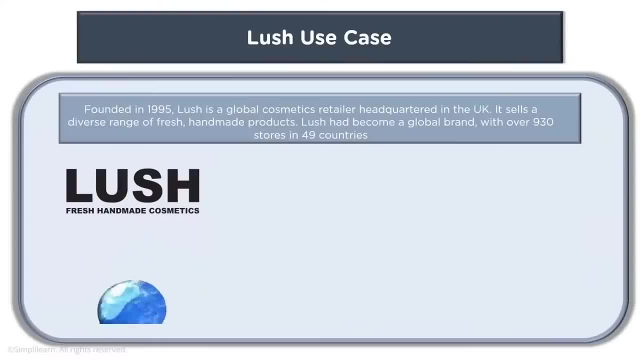 range of fresh handmade products. lush range of fresh handmade products. lush had become a global brand with over 930. had become a global brand with over 930. had become a global brand with over 930 stores in 49 countries. so the challenges: stores in 49 countries. so the challenges. 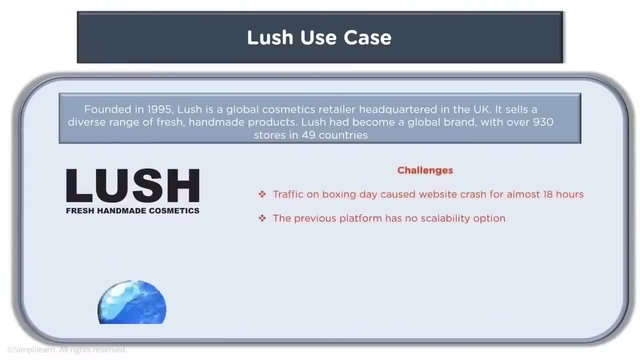 stores in 49 countries. so the challenges which were faced here was traffic on which were faced here was traffic on which were faced. here was traffic on Boxing Day caused website crash for Boxing Day, caused website crash for Boxing Day, caused website crash for almost 18 hours, and this is something. 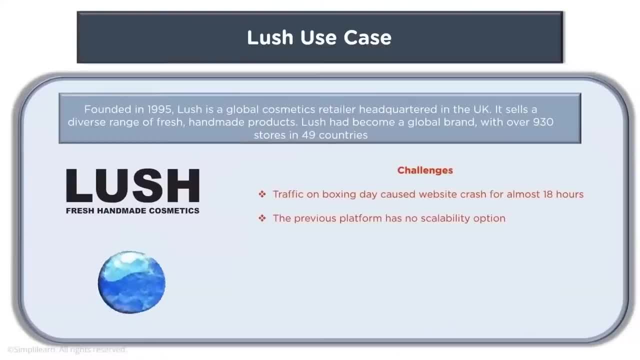 almost 18 hours, and this is something- almost 18 hours- and this is something which had a devastating effect on their, which had a devastating effect on their, which had a devastating effect on their business. the previous platform had no business. the previous platform had no business. the previous platform had no scalability option. what was the solution? 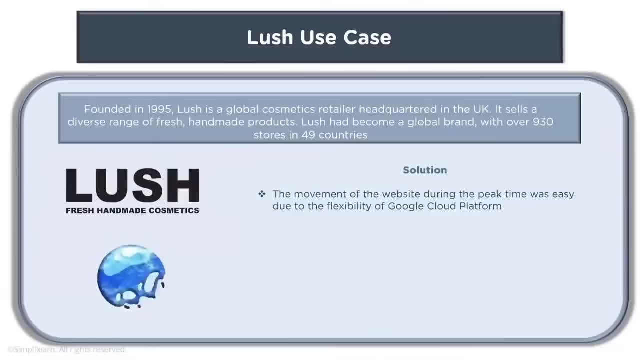 scalability option. what was the solution? scalability option: what was the solution? the movement of website during the peak. the movement of website during the peak. the movement of website during the peak time was easy due to flexibility of GCP. time was easy due to flexibility of GCP. 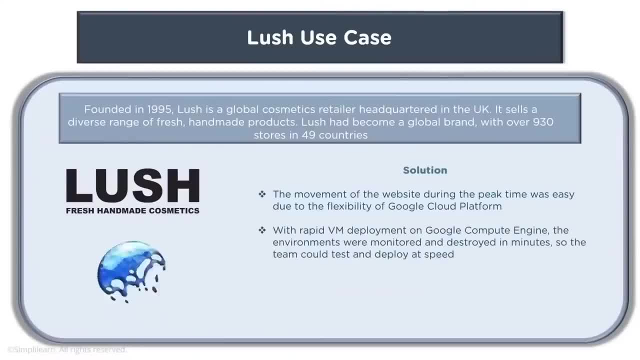 time was easy due to flexibility of GCP platform, with rapid VM deployment on platform. with rapid VM deployment on platform. with rapid VM deployment on Google Compute Engine. the environments- Google Compute Engine. the environments- Google Compute Engine. the environments were monitored and destroyed in minutes. were monitored and destroyed in minutes. 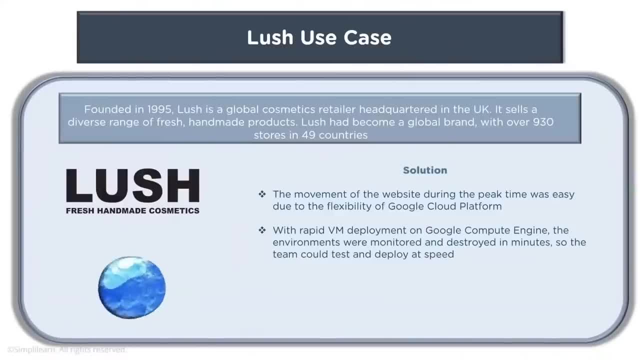 were monitored and destroyed in minutes. so the team could test and deploy at. so the team could test and deploy at. so the team could test and deploy at speed by using Google Cloud SQL lush to speed. by using Google Cloud SQL lush to speed. by using Google Cloud SQL lush to complete control of its infrastructure. 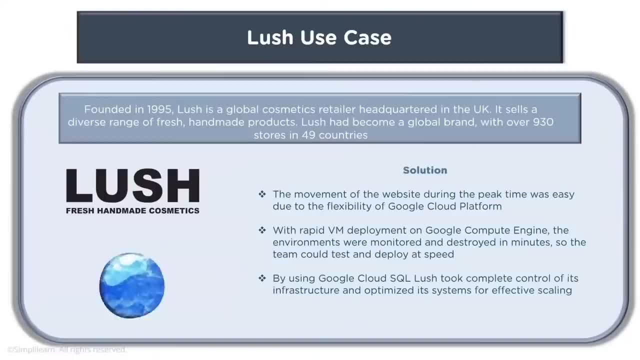 complete control of its infrastructure. complete control of its infrastructure and optimize its systems for effective. and optimize its systems for effective. and optimize its systems for effective. scaling overall. the platform resulted in scaling overall. the platform resulted in scaling overall. the platform resulted in lower cost. that led to a bright future. 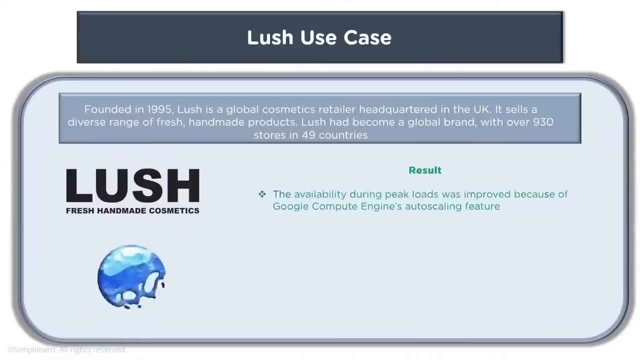 lower cost that led to a bright future. lower cost that led to a bright future for lush cosmetics. now, what was the for lush cosmetics now? what was the for lush cosmetics now? what was the result of all this? the availability result of all this. the availability result of all this: the availability during peak loads was improved because 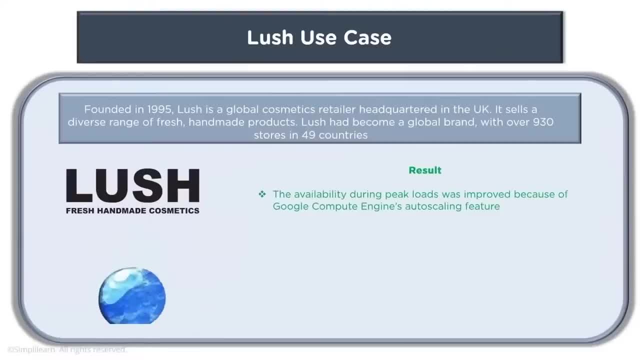 during peak loads was improved. because during peak loads was improved because of Google Compute Engines auto scaling of Google Compute Engines. auto scaling of Google Compute Engines auto scaling feature. the infrastructure hosting costs feature: the infrastructure hosting costs feature. the infrastructure hosting costs were reduced by 40%. streamline data. 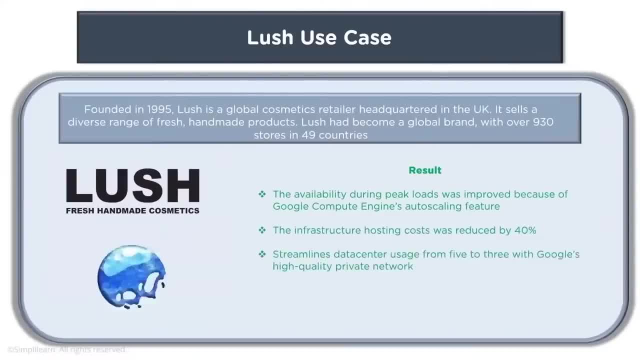 were reduced by 40%. streamline data were reduced by 40%. streamline data center usage from 5 to 3 with Google's center usage from 5 to 3 with Google's center usage from 5 to 3 with Google's high-quality private network. really, 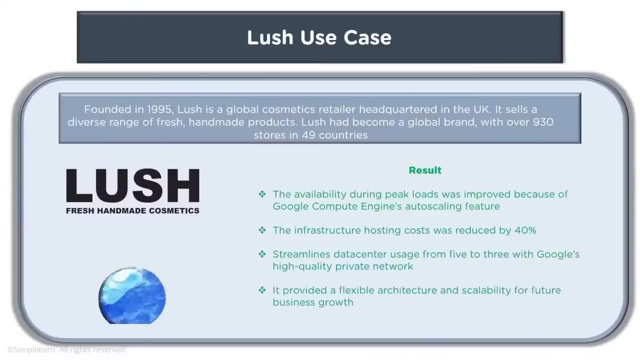 high-quality private network, really high-quality private network, really benefited lush and it provided a benefited lush and it provided a benefited lush and it provided a flexible architecture and scalability, flexible architecture and scalability, flexible architecture and scalability for future business growth: now what we for. future business growth: now what we. 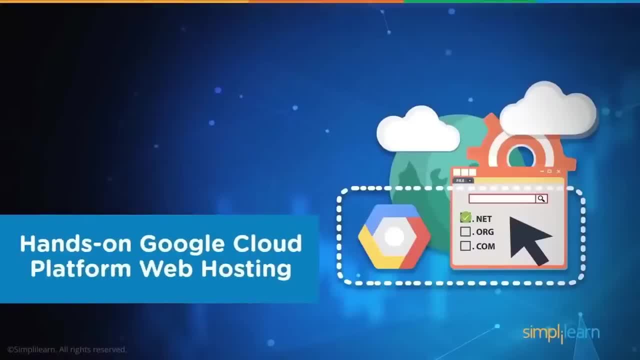 for future business growth. now, what we have seen here is that your Google Cloud have seen here is that your Google Cloud have seen here is that your Google Cloud and its web hosting basically offers and its web hosting basically offers and its web hosting basically offers users to run their websites or use a. 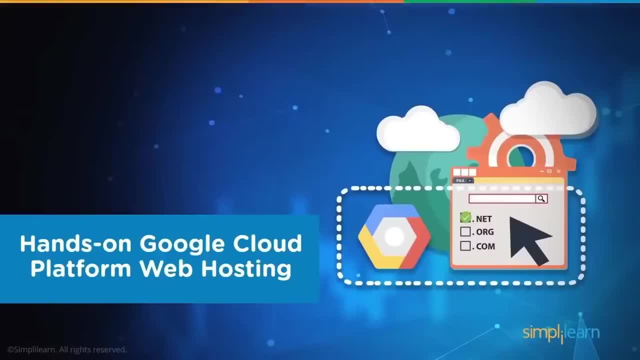 users to run their websites, or use a users to run their websites, or use a web hosting solution that can benefit in web hosting solution that can benefit in web hosting solution that can benefit in more than one way. the simplest approach. more than one way. the simplest approach. 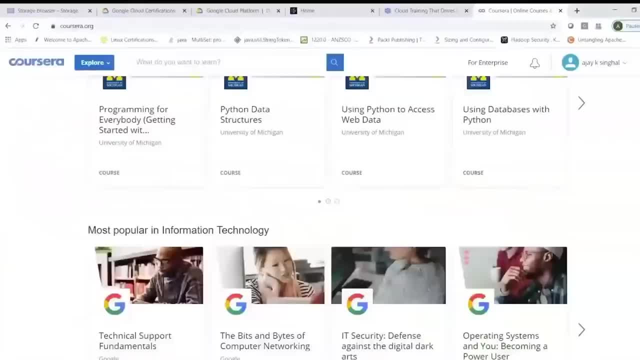 more than one way. the simplest approach could be seen is by clicking and setting could be seen is by clicking and setting could be seen is by clicking and setting up a VM instance by going to your console. up a VM instance by going to your console. up a VM instance by going to your console, for example, if we go in to the Google. 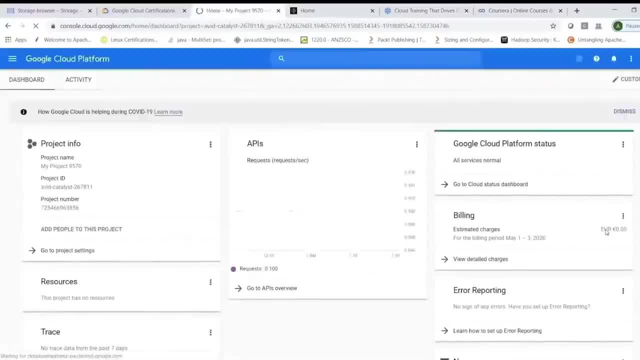 for example, if we go in to the Google, for example, if we go in to the Google Cloud platform, clicking on console and Cloud platform, clicking on console and Cloud platform, clicking on console. and here the easiest way I could test it is here the easiest way I could test it is. 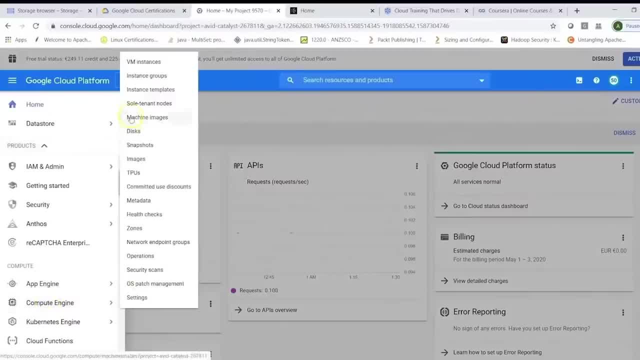 here. the easiest way I could test it is by going to my Compute Engine VM. by going to my Compute Engine VM, by going to my Compute Engine VM instances, and here I can spin up an instances. and here I can spin up an instances. and here I can spin up an instance I can click on create now in my 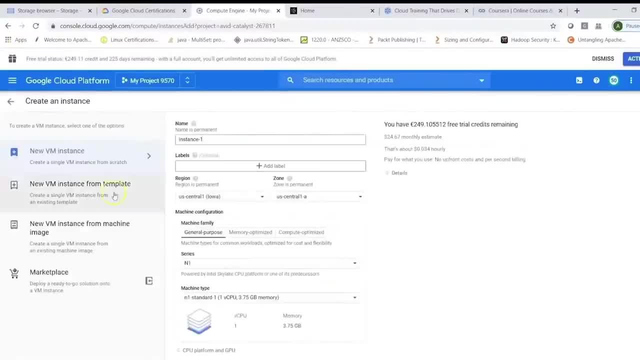 instance, I can click on create now. in my instance, I can click on create now. in my previous sessions, I have also explained previous sessions. I have also explained previous sessions. I have also explained about how you could create a template, about how you could create a template, about how you could create a template and run an instance from that we can. 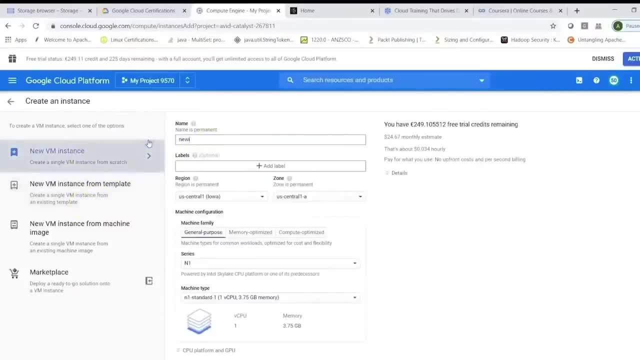 and run an instance from that. we can and run an instance from that. we can. also click on new VM instance. let's call- also click on new VM instance. let's call- also click on new VM instance. let's call it new instance. I will choose a region. 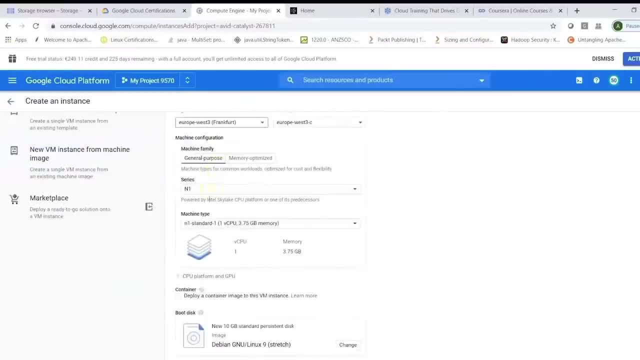 it new instance. I will choose a region. it new instance. I will choose a region, for example, Frankfurt. I will let it be, for example, Frankfurt. I will let it be, for example, Frankfurt. I will let it be general-purpose machines. let this general-purpose machines, let this general-purpose machines, let this machine be one virtual CPU core and 3.75. 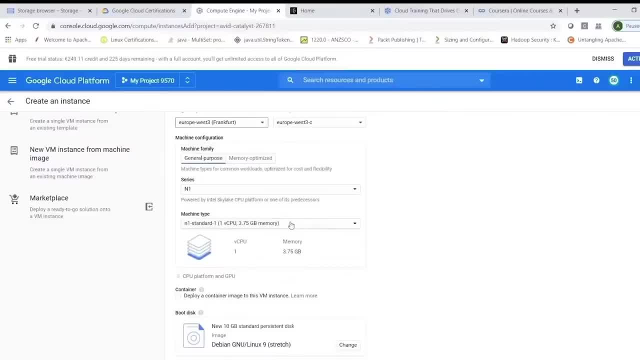 machine be one virtual CPU core and 3.75 machine be one virtual CPU core and 3.75 gigabyte RAM. if I am looking for a gigabyte RAM. if I am looking for a gigabyte RAM, if I am looking for a heavier website which might have more. 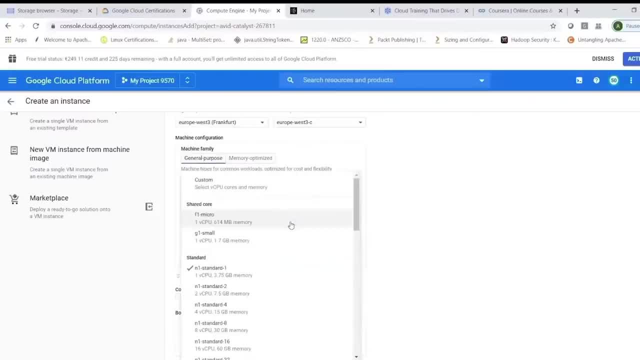 heavier website, which might have more heavier website, which might have more users logging in, and so on. then I can users logging in, and so on. then I can users logging in, and so on. then I can choose a higher configuration machine. choose a higher configuration machine, choose a higher configuration machine. here we have the option to choose our 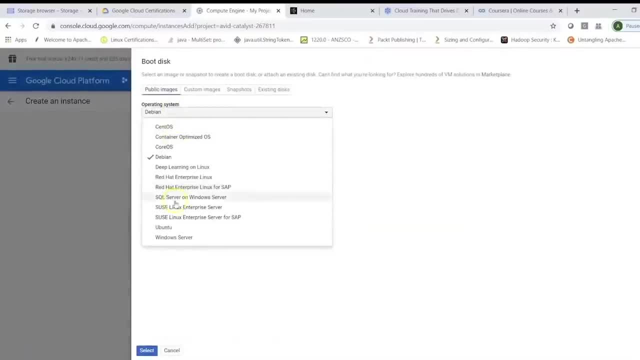 here we have the option to choose our. here we have the option to choose our distribution. so, for example, I can choose distribution. so, for example, I can choose distribution. so, for example, I can choose Ubuntu and then I can choose a Ubuntu and then I can choose a. 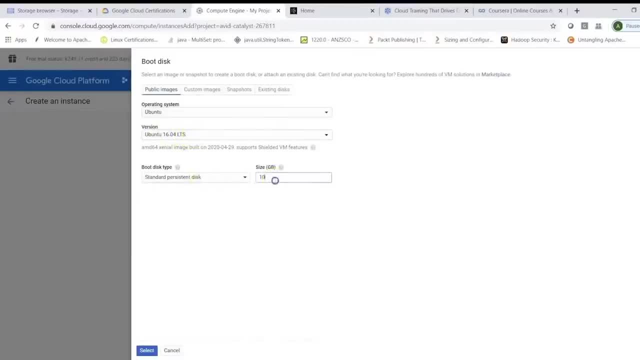 Ubuntu, and then I can choose a distribution version. so it let it be distribution version. so it let it be distribution version. so it let it be 16.04. we can choose the disk size to be 16.04. we can choose the disk size to be. 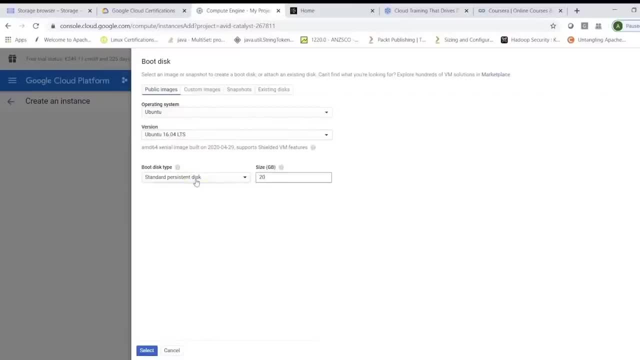 16.04 we can choose the disk size to be 20 gigabyte and we can use SSDs or HDDs. 20 gigabyte and we can use SSDs or HDDs- 20 gigabyte and we can use SSDs or HDDs. so as of now it is standard persistent. 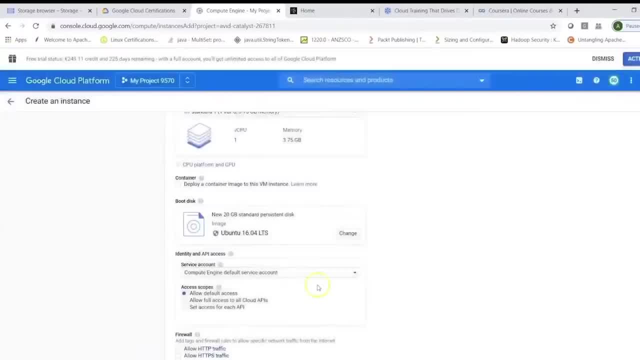 so as of now, it is standard persistent. so as of now, it is standard persistent disk. that is HDD and that should be disk. that is HDD and that should be disk. that is HDD, and that should be enough. let's click on select here, I will enough. let's click on select here, I will. 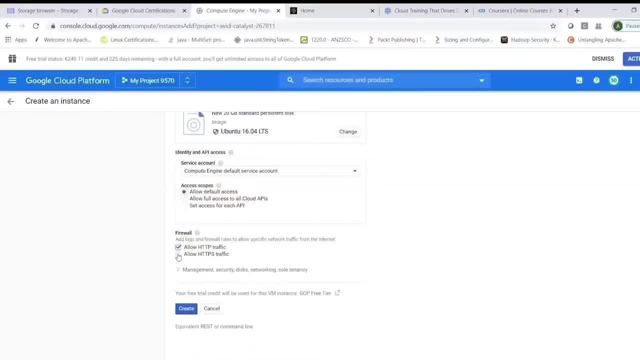 enough, let's click on select here. I will say allow default access. I would say say allow default access. I would say say allow default access. I would say allow HTTP and HTTP s, so that if I have allow HTTP and HTTP s, so that if I have allow HTTP and HTTP s, so that if I have a website content hosted on this machine. 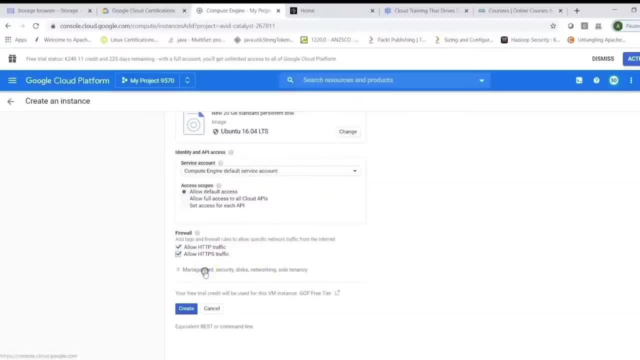 a website content hosted on this machine. a website content hosted on this machine. I can access it over HTTP. now here you. I can access it over HTTP. now here you. I can access it over HTTP. now here you have management options for your. have management options for your. 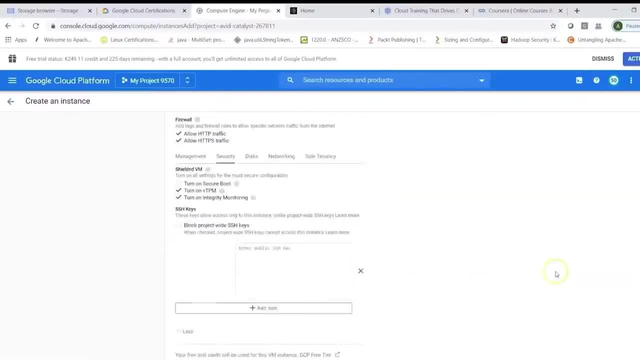 have management options. for your instance you have security option. which instance you have security option? which instance you have security option, which basically allows you to provide a public, basically allows you to provide a public, basically allows you to provide a public key if you are interested in using an. 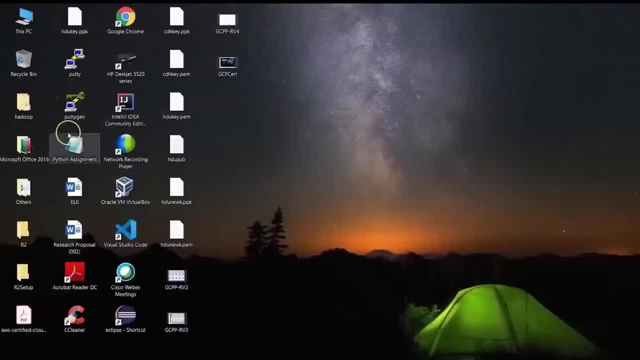 key if you are interested in using an key. if you are interested in using an external SSH client to connect, now I external SSH client to connect. now I external SSH client to connect. now I have used putty gen and I have already have used putty gen and I have already 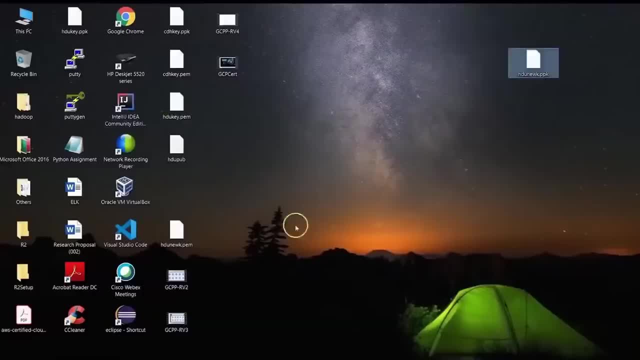 have used putty gen and I have already created a private key, which is here. I created a private key, which is here. I created a private key, which is here. I have also converted that as a PEM file, have also converted that as a PEM file, have also converted that as a PEM file and anytime if I would want to use this. 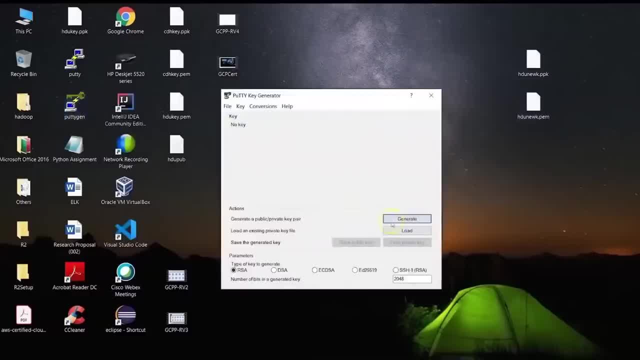 and anytime if I would want to use this and anytime if I would want to use this key, all I need to do is click on putty key. all I need to do is click on putty key. all I need to do is click on putty gen, where I had earlier created this PPK. 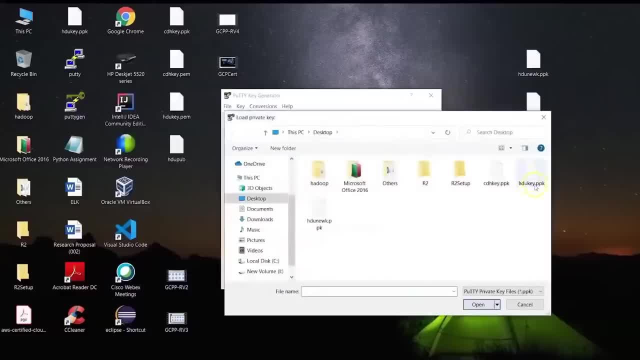 gen, where I had earlier created this PPK gen, where I had earlier created this PPK file. now I can just do a load and I can file. now I can just do a load and I can file. now I can just do a load and I can choose the key which I have here and I 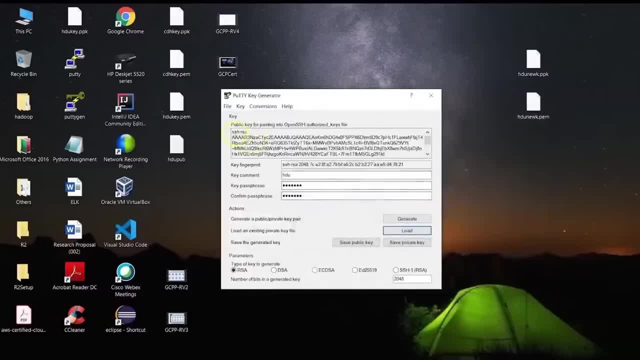 choose the key which I have here and I choose the key which I have here and I can give the pass face click on OK and can give the pass face click on OK and can give the pass face click on OK and that shows you the public key. let's copy. 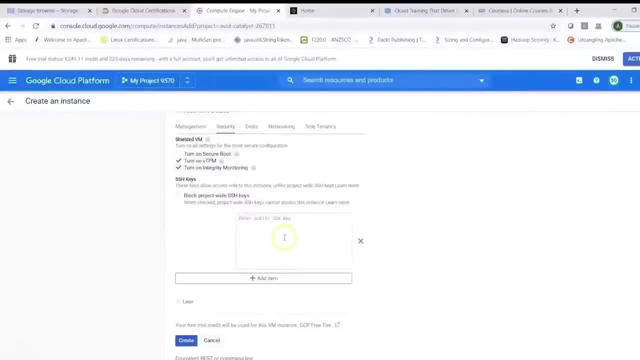 that shows you the public key. let's copy. that shows you the public key. let's copy the public key from here. let's go into the public key from here. let's go into the public key from here. let's go into our instance and I can give this here: 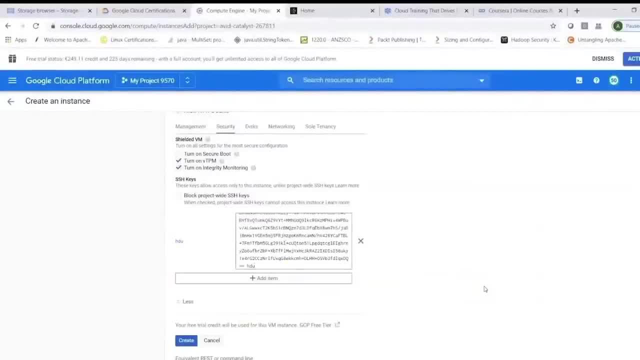 our instance and I can give this here our instance, and I can give this here: that resolves the name. so I have the that resolves the name. so I have the that resolves the name. so I have the private key saved on my machine and private key saved on my machine and. 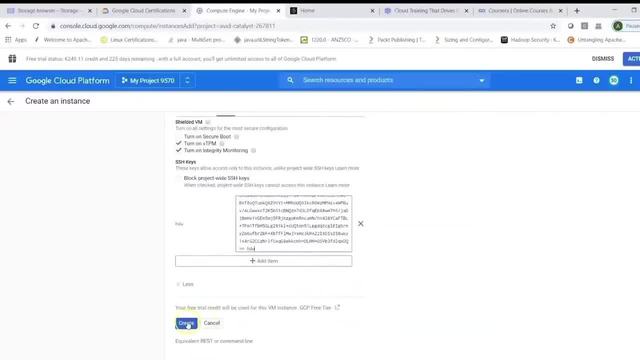 private key saved on my machine and public key, which will be pushed into the public key, which will be pushed into the public key, which will be pushed into the machine I can click on create and that machine I can click on create and that machine I can click on create and that should create my instance, to which you. 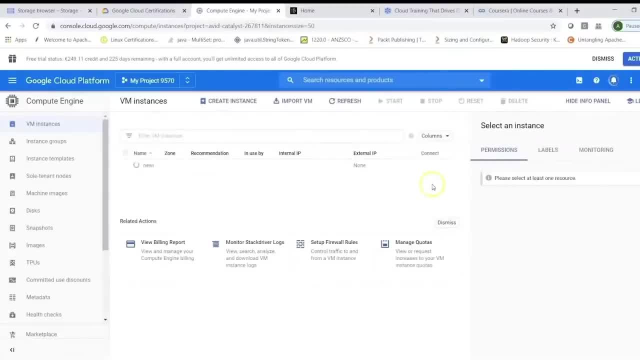 should create my instance, to which you should create my instance, to which you can connect using SSH from the console. can connect using SSH from the console. can connect using SSH from the console itself or using a external client such itself, or using a external client such itself, or using a external client, such as putty, which will then need the public. 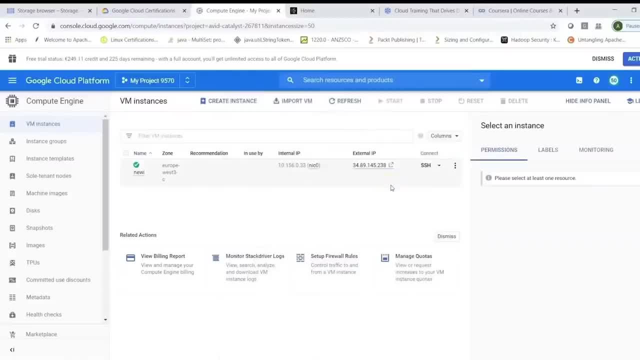 as putty, which will then need the public as putty, which will then need the public IP of this instance, the PPK file. what we as putty, which will then need the public IP of this instance, the PPK file, what we have and you can connect to this. 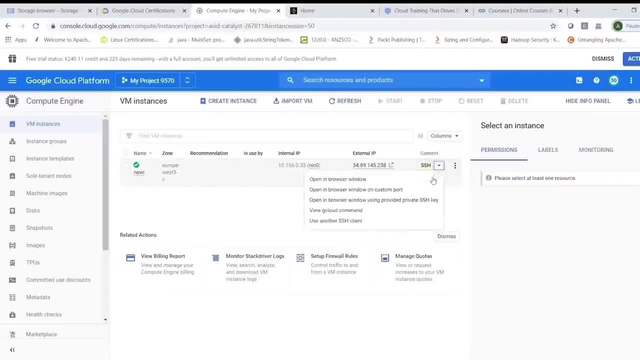 have and you can connect to this have and you can connect to this instance. what I can also do is I can just instance. what I can also do is I can just instance. what I can also do is I can just do a simple SSH from here and that will. 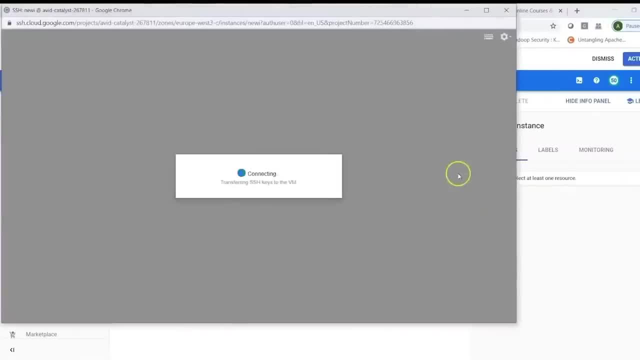 do a simple SSH from here and that will do a simple SSH from here and that will basically allow me to connect to the basically allow me to connect to the basically allow me to connect to the instance- what we also need to remember, instance, what we also need to remember. 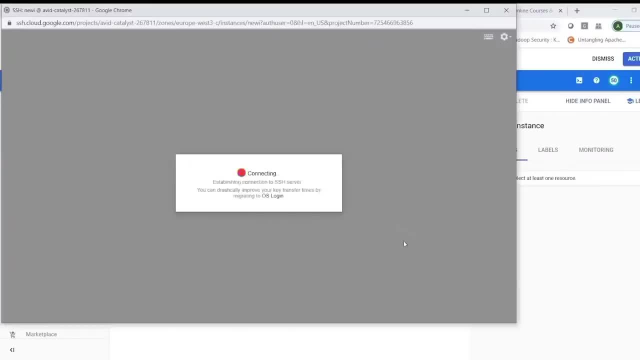 instance. what we also need to remember is each instance. what we create in is each instance. what we create in is each instance. what we create in compute is also having some default compute, is also having some default compute, is also having some default firewall rules. now I have corrected to my 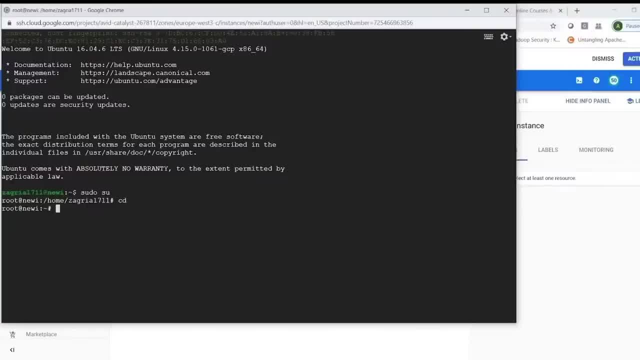 firewall rules. now I have corrected to my firewall rules. now I have corrected to my instance. I can click on sudo su. I can instance. I can click on sudo su. I can instance. I can click on sudo su. I can login as root and here, if I would want, I. 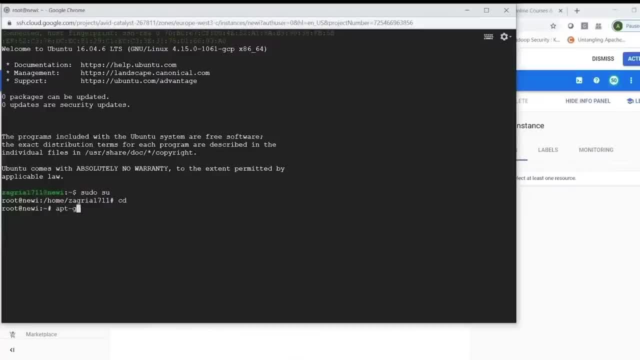 login as root. and here, if I would want, I login as root, and here, if I would want, I can install a particular service. so can install a particular service. so can install a particular service. so let's say Apache, let's say apt-get. let's say Apache, let's say apt-get. 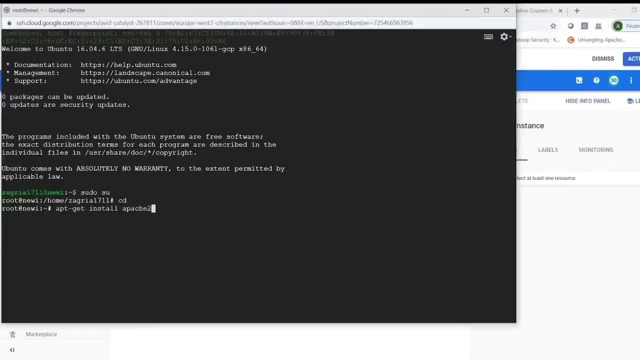 let's say Apache, let's say apt-get- install, and then I can say Apache 2 or install, and then I can say Apache 2 or install, and then I can say Apache 2 or HTTP D. that is basically to host your HTTP D, that is basically to host your. 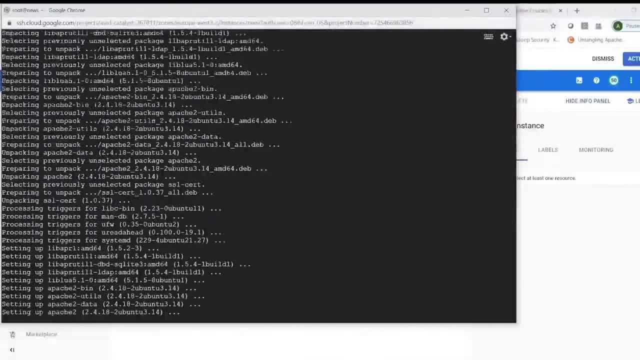 HTTP D. that is basically to host your web application. so I'm installing the web application. so I'm installing the web application, so I'm installing the service, and here I can check if the service. and here I can check if the service. and here I can check if the service is running by doing a service. 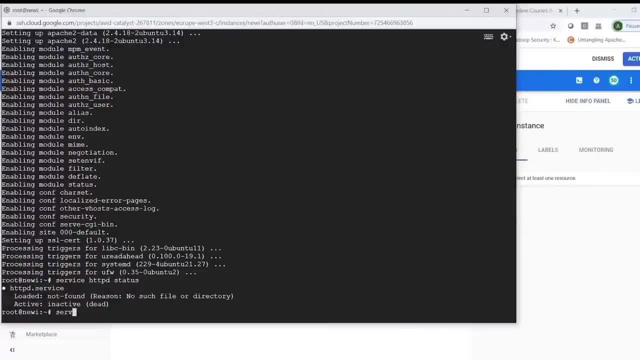 service is running by doing a service. service is running by doing a service: HTTP D status, or I can say service HTTP D status, or I can say service HTTP D status, or I can say service Apache 2 status. it says it is already. Apache 2 status. it says it is already. 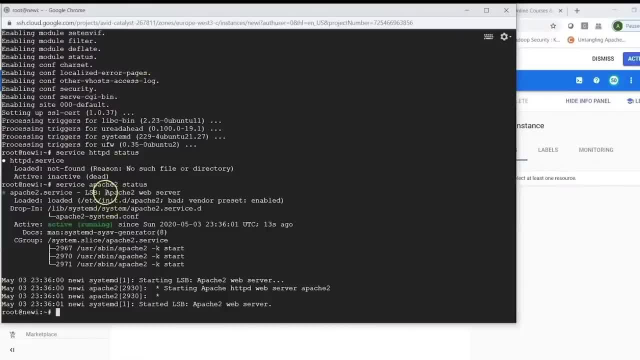 Apache 2 status. it says it is already running. that means the Apache web server running. that means the Apache web server running. that means the Apache web server page will be accessible from HTTP. page will be accessible from HTTP. page will be accessible from HTTP, provided my firewall rules allow that. 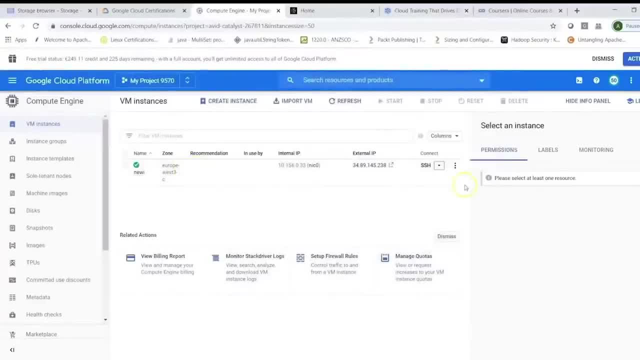 provided my firewall rules allow that, provided my firewall rules allow that. now, before we look into this, we can also now, before we look into this, we can also, now, before we look into this, we can also, for our instance, look at the firewall. for our instance, look at the firewall. 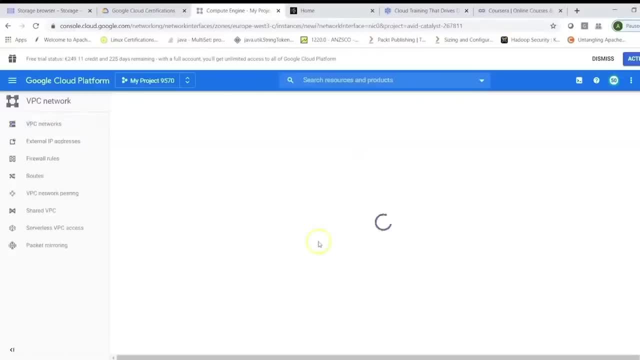 for our instance, look at the firewall rules. so here you have network details rules. so here you have network details rules. so here you have network details. now, since we created an instance by now, since we created an instance, by now, since we created an instance by default, Google has created some firewall. default. Google has created some firewall default. Google has created some firewall rules which allow default HTTP HTTP s. rules which allow default HTTP HTTPS. rules which allow default HTTP HTTPS ICMP- your default internal access, RDP ICMP- your default internal access, RDP ICMP, your default internal access, RDP and SSH access. and here it says these: 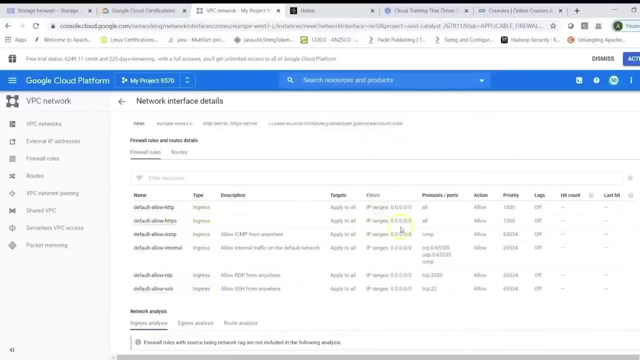 and SSH access, and here it says these and SSH access and here it says these ingress rules which allow incoming ingress rules which allow incoming ingress rules which allow incoming traffic are allowed from anywhere we can. traffic are allowed from anywhere we can. traffic are allowed from anywhere we can customize that as specific IP addresses. 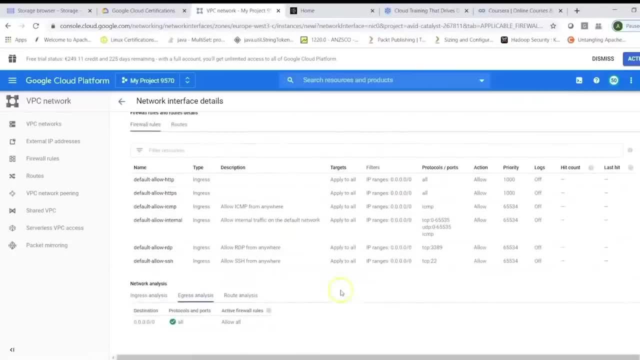 customize that as specific IP addresses. customize that as specific IP addresses. we can also look at egress, which is. we can also look at egress, which is. we can also look at egress, which is basically outgoing traffic, and this is basically outgoing traffic and this is. 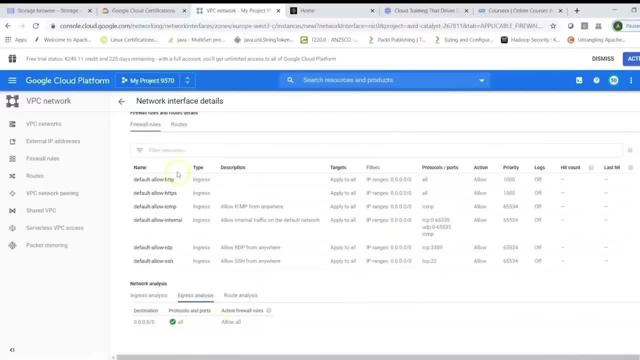 basically outgoing traffic. and this is again saying my machine can connect to, again saying my machine can connect to, again saying my machine can connect to the external world in different ways, the external world in different ways, the external world in different ways, using different protocols. so you can. 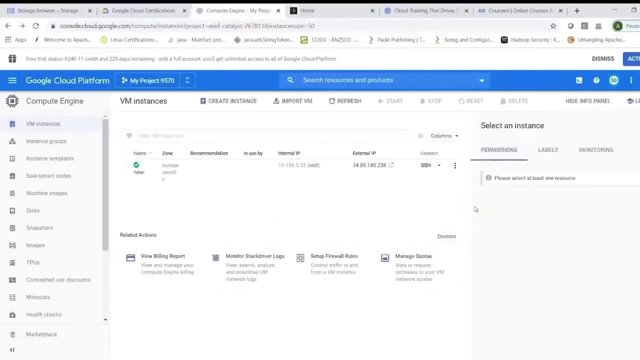 using different protocols so you can. using different protocols, so you can customize these firewall rules as of now. customize these firewall rules as of now. customize these firewall rules as of now. I'm going to let it be default now we. I'm going to let it be default now we. 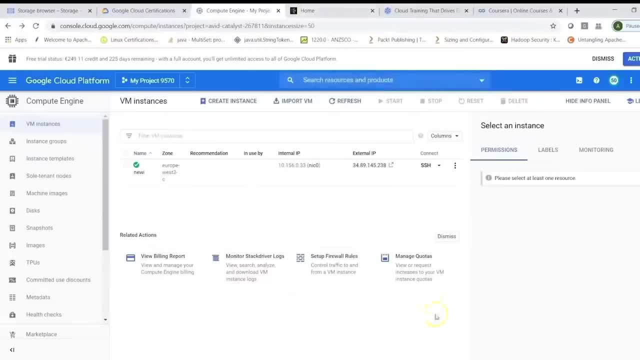 I'm going to let it be default now. we connected to our instance from the, connected to our instance from the, connected to our instance from the browser and we were basically checking browser and we were basically checking browser and we were basically checking how you can use this browser by clicking. 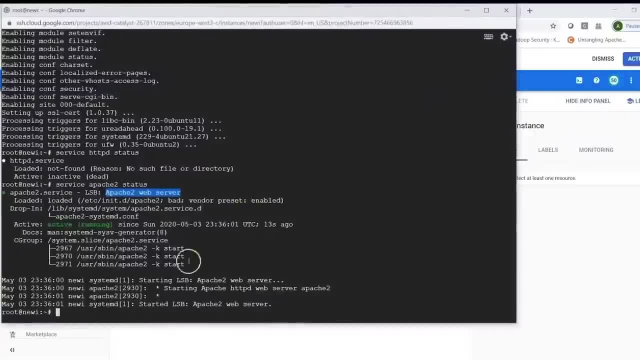 how you can use this browser by clicking. how you can use this browser by clicking on this now. what I can also do is here, on this now. what I can also do is here on this now. what I can also do is here. I'm logged into the instance, my Apache. 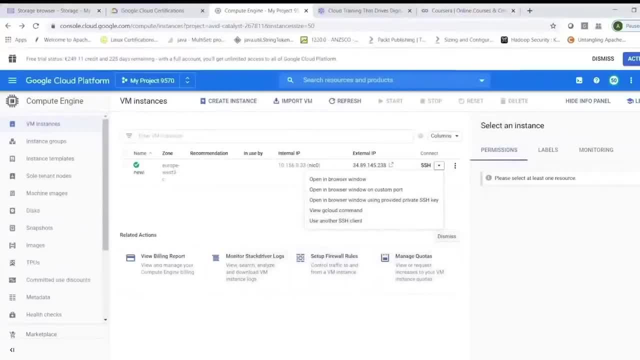 I'm logged into the instance my Apache. I'm logged into the instance my Apache server is running. so the best way to server is running, so the best way to server is running. so the best way to check if the Apache web server is: check if the Apache web server is. 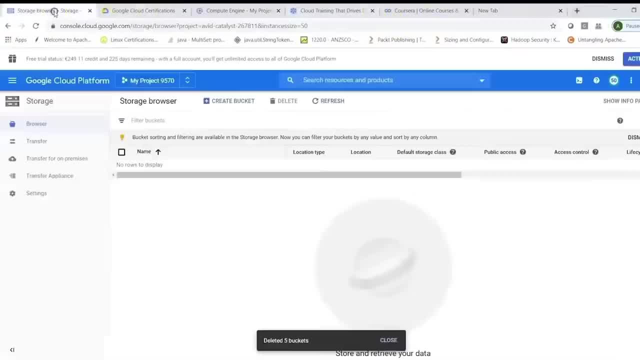 check if the Apache web server is accessible via HTTP. all I need is my accessible via HTTP. all I need is my accessible via HTTP. all I need is my public IP. so let's copy this, let's go. public IP- so let's copy this, let's go. 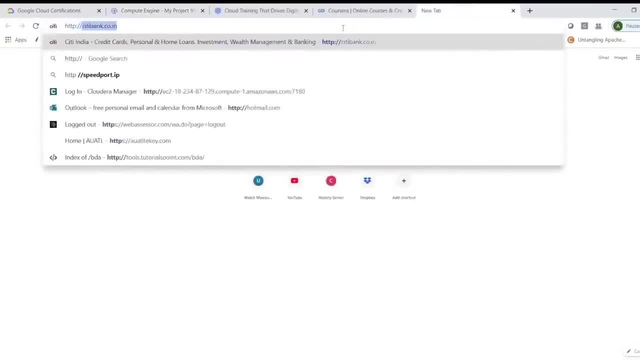 public IP. so let's copy this, let's go here and I will say HTTP slash slash. here, and I will say HTTP slash slash. here and I will say HTTP slash slash. just give you a public IP, and that shows. just give you a public IP and that shows. 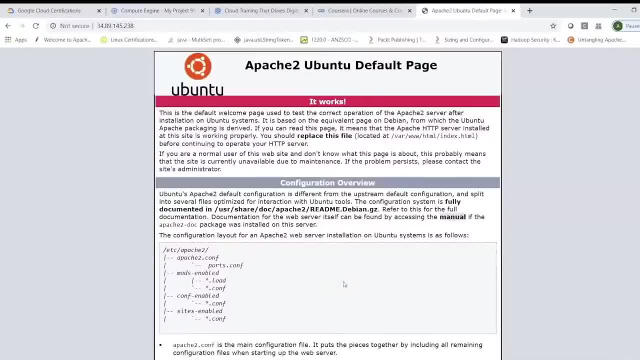 just give you a public IP and that shows your Apache to web server page, that your Apache to web server page, that your Apache to web server page. that means the Apache service has already, means the Apache service has already, means the Apache service has already been run. now here it tells: if you would 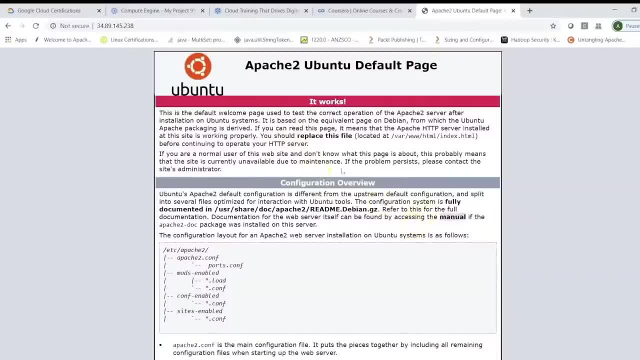 been run now. here it tells if you would been run now. here it tells if you would want to host a particular page, what you want to host a particular page, what you want to host a particular page. what you will have to do is as it says. here it is. 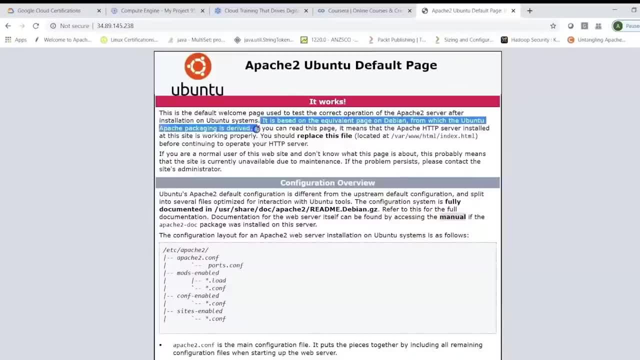 will have to do is as it says here it is will have to do is as it says here. it is: based on equivalent page on DBN from. based on equivalent page on DBN from. based on equivalent page on DBN from which Ubuntu Apache packaging is. 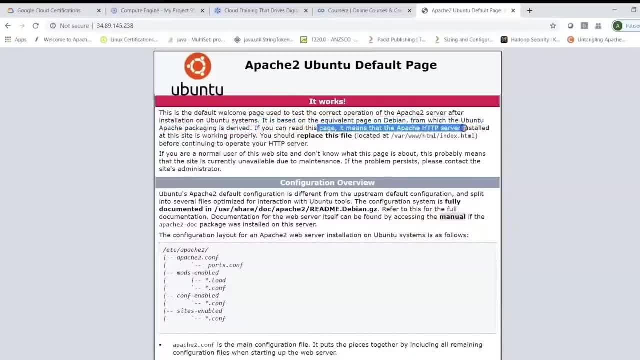 which Ubuntu Apache packaging is which Ubuntu Apache packaging is derived. if you can read this page, it derived. if you can read this page, it derived. if you can read this page. it means Apache HTTP server is installed. means Apache HTTP server is installed. means Apache HTTP server is installed at this site is working properly now you. 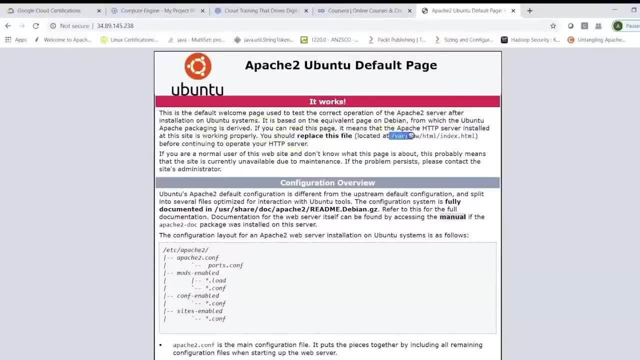 at this site is working properly now. you at this site is working properly now. you can replace this file located at var. can replace this file located at var. can replace this file located at var- wwwhtml- indexhtml. before continuing wwwhtml- indexhtml. before continuing wwwhtml- indexhtml. before continuing page. and you will be able to host your 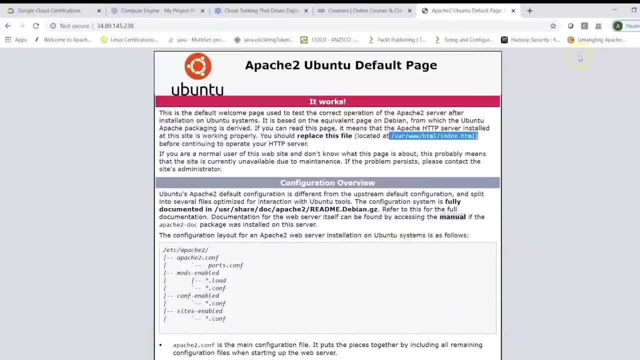 page and you will be able to host your page and you will be able to host your website on this particular ec2 instance website, on this particular ec2 instance website, on this particular ec2 instance. what we can do is we can check this. so what we can do is we can check this. so. 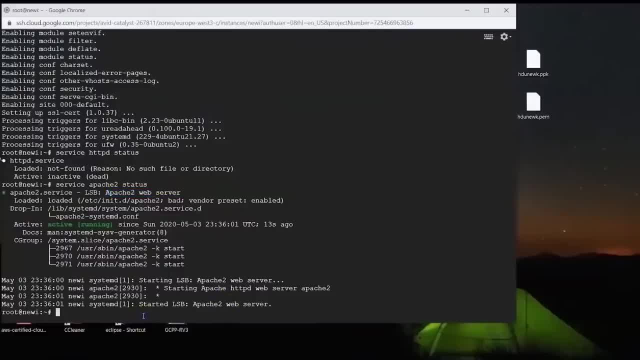 what we can do is we can check this. so we can go into the browser and we can. we can go into the browser and we can. we can go into the browser and we can look in var www and that has an HTML. look in var www and that has an HTML. 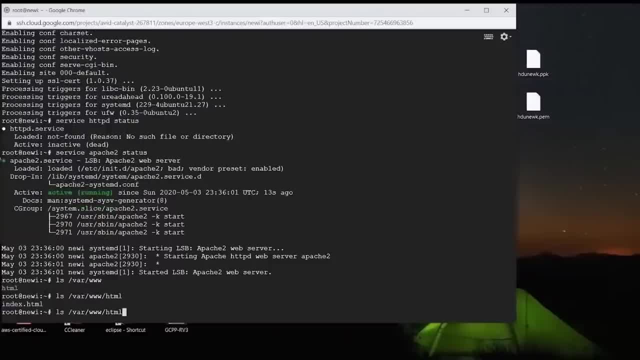 look in var. www and that has an HTML folder- look into this. and as of now, you folder look into this and as of now, you folder look into this and as of now, you have a index dot HTML and that have a index dot HTML and that have a index dot HTML and that, basically, is the page, what we are seeing. 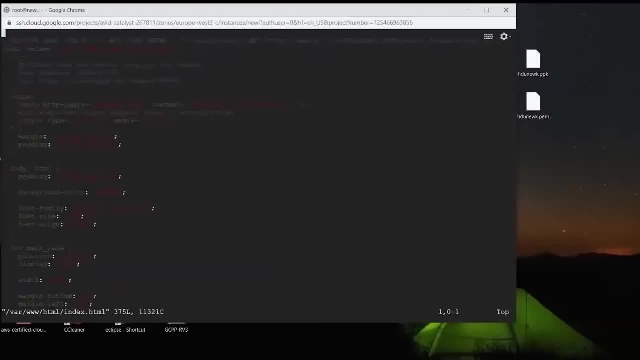 basically is the page what we are seeing. basically is the page what we are seeing. now I can click on this one and I can. now, I can click on this one and I can. now, I can click on this one and I can see. I have a small HTML page which is: 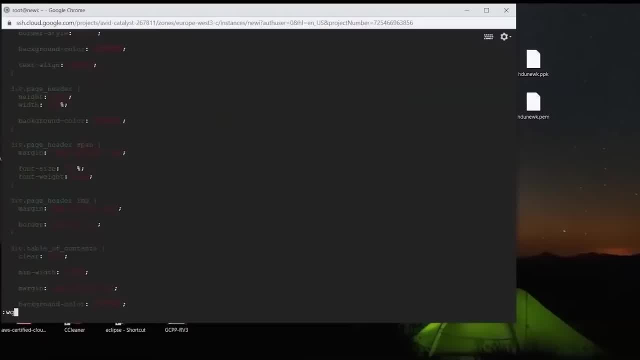 see, I have a small HTML page which is: see, I have a small HTML page which is basically showing me what we are seeing, basically showing me what we are seeing, basically showing me what we are seeing on our web server. what I can also do is on our web server. what I can also do is: 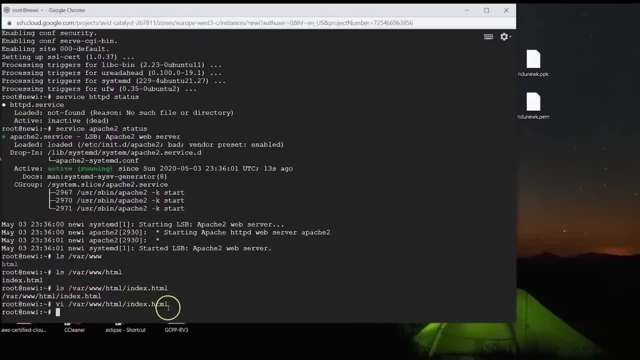 on our web server. what I can also do is, for now, I can test it out and I can put. for now, I can test it out and I can put. for now, I can test it out and I can put in a different HTML page and see how. 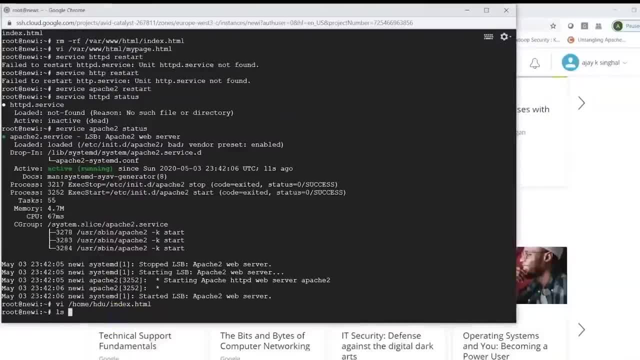 in a different HTML page and see how in a different HTML page and see how that works. so we had basically the page that works. so we had basically the page that works. so we had basically the page here in var www and then we had the here in var www and then we had the. 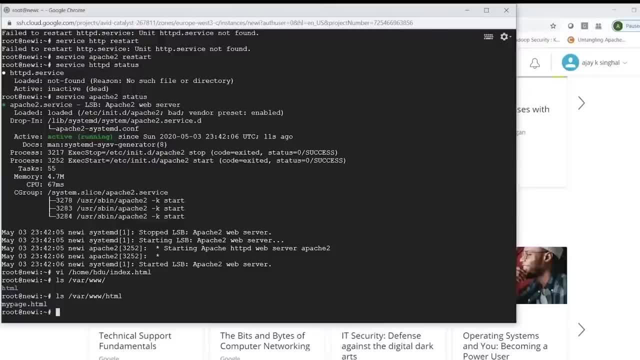 here in var www, and then we had the HTML folder and in HTML folder what I HTML folder and in HTML folder, what I HTML folder and in HTML folder, what I had was this index file, so as of now I had was this index file. so as of now I. 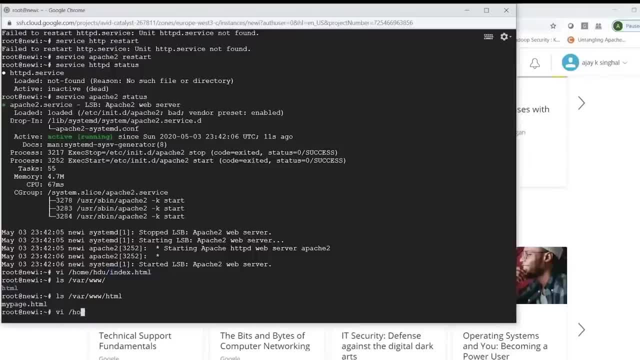 had was this index file. so, as of now, I just moved it and I put it in a, just moved it and I put it in a, just moved it and I put it in a different location. so if I look in my different location, so if I look in my 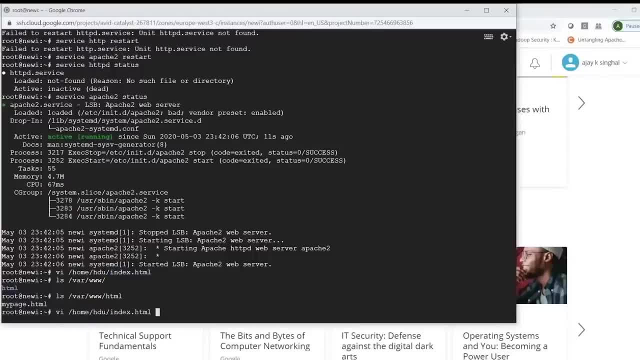 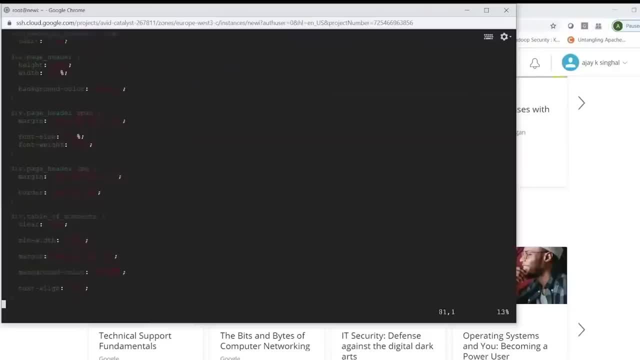 different location. so if I look in my home HD, you index dot HTML that shows home HD. you index dot HTML that shows home HD. you index dot HTML that shows me the complete HTML page, what we were me the complete HTML page, what we were me, the complete HTML page, what we were seeing on our web server, and here it. 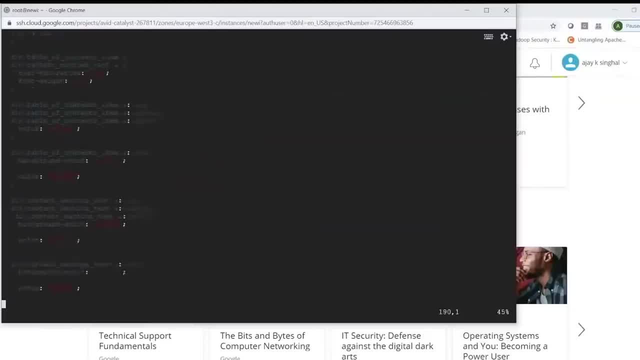 seeing on our web server. and here it seeing on our web server, and here it shows you what this page would display. shows you what this page would display. shows you what this page would display if you run it on your HTTP. it says: if you run it on your HTTP, it says: 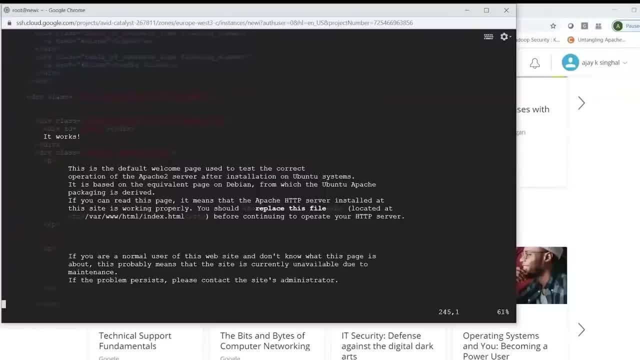 if you run it on your HTTP. it says Apache to window default page. it shows Apache to window default page. it shows Apache to window default page. it shows it works. it shows the content, and so on. it works, it shows the content and so on. it works, it shows the content, and so on. so for just testing, I move this page out. 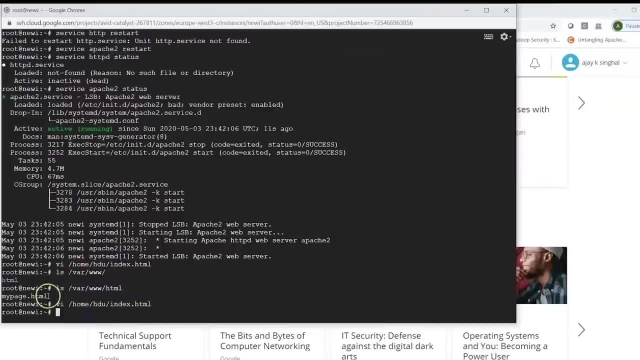 so, for just testing, I move this page out. so, for just testing, I move this page out from this location and what I did was I from this location and what I did was I from this location and what I did was I added a different page here so that 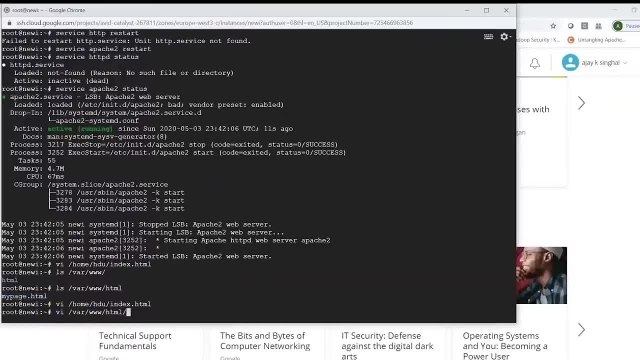 added a different page here, so that added a different page here. so that page. if you look in HTML and then look in page. if you look in HTML and then look in page. if you look in HTML and then look in my page, dot HTML section. I've just 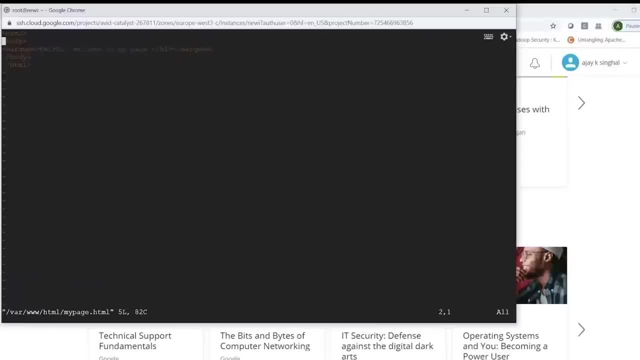 my page dot HTML section. I've just my page dot HTML section. I've just added some basic details of creating, added some basic details of creating, added some basic details of creating HTML. I'm saying body, I'm using marquee HTML. I'm saying body, I'm using marquee. 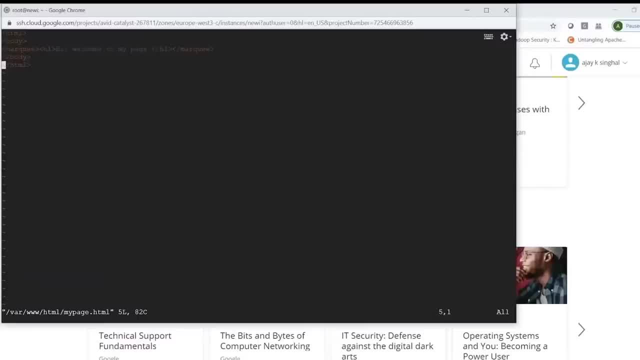 HTML. I'm saying body, I'm using marquee, and then I'm closing this with HTML tag, and then I'm closing this with HTML tag, and then I'm closing this with HTML tag. now, this is a simple HTML page which I. now, this is a simple HTML page which I. 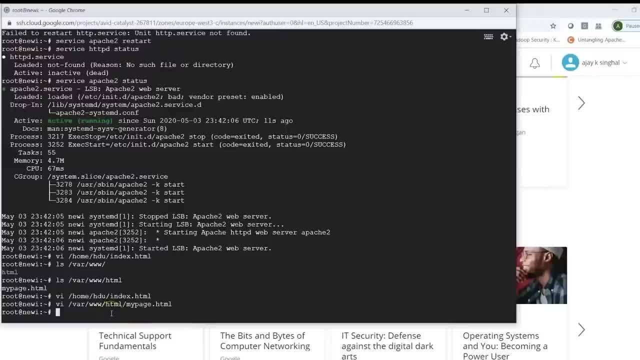 now, this is a simple HTML page which I created, and now what I did was once created, and now what I did was once created, and now what I did was once. I've done this. I basically did a service. I've done this. I basically did a service. 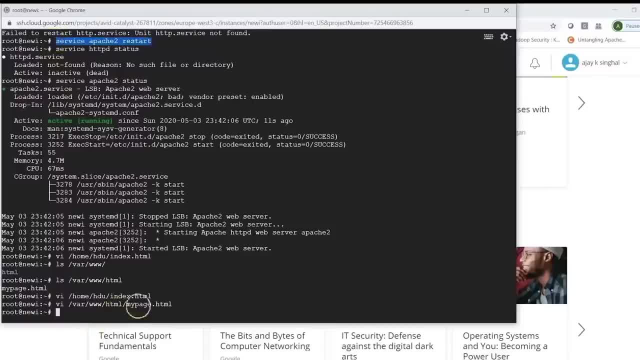 I've done this. I basically did a service: Apache restart. so once you do that, it Apache restart. so once you do that, it Apache restart. so once you do that, it will take up your new page. and once you will take up your new page and once you. 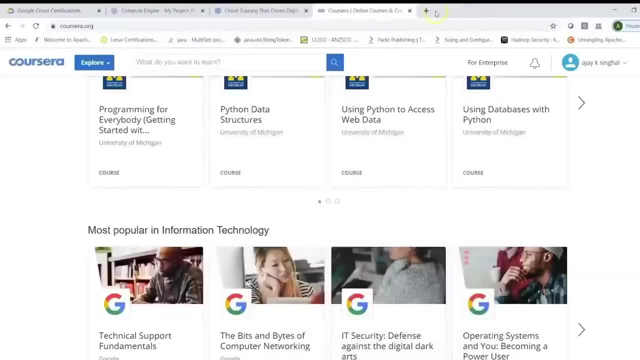 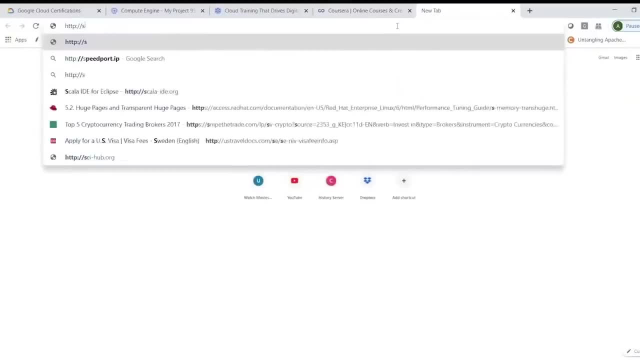 will take up your new page and once you have done that, now you can access that. have done that now, you can access that. have done that now. you can access that by going to your HTTP given your details, by going to your HTTP, given your details, by going to your HTTP, given your details and then basically give your public IP. 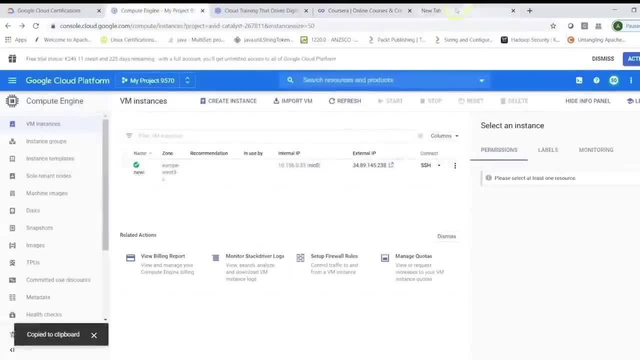 and then basically give your public IP and then basically give your public IP which we can get from here, and just which we can get from here and just which we can get from here, and just paste it here now. hit on this so that. paste it here now. hit on this so that. 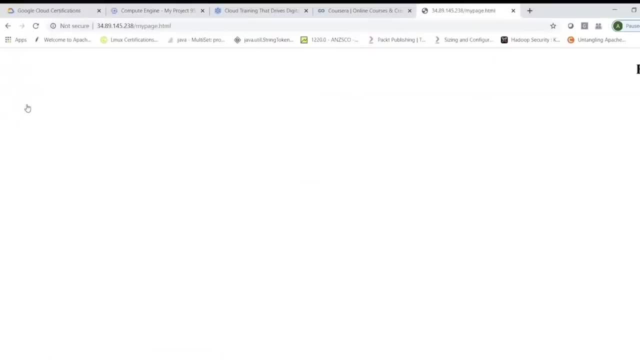 paste it here now. hit on this so that shows me there is a my page dot HTML. I shows me there is a my page dot HTML. I shows me there is a my page dot HTML. I can click on this and that. basically can click on this and that, basically. 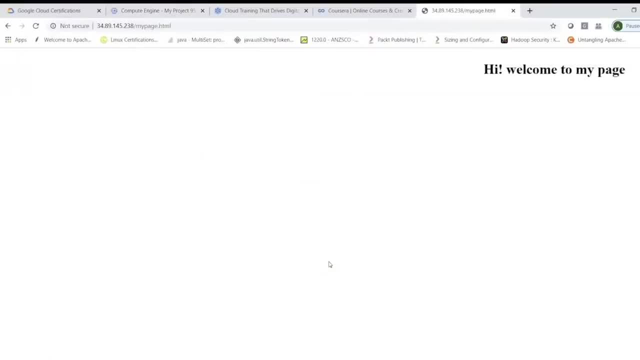 can click on this and that basically shows the symbol page which I created. so shows the symbol page which I created. so shows the symbol page which I created. so, as of now, this is my web page which I. as of now, this is my web page which I. 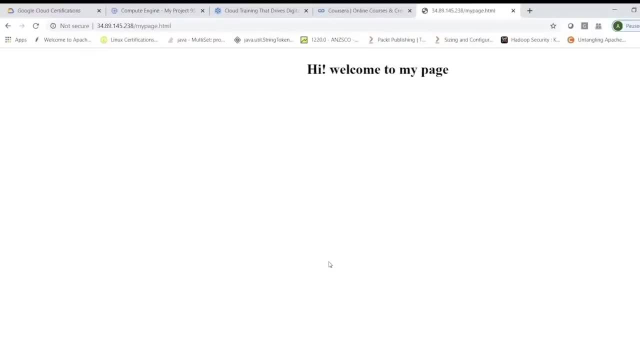 as of now, this is my web page, which I have created and this is hosted on my. have created and this is hosted on my. have created and this is hosted on my compute instance now. obviously we can compute instance now. obviously we can compute instance now. obviously we can create a more complex website, backed up. 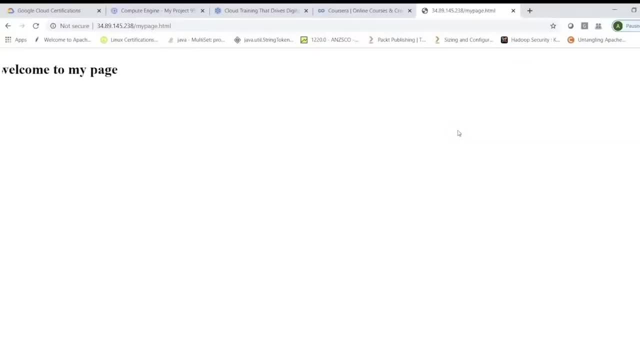 create a more complex website backed up. create a more complex website backed up by a database. use PHP. use mysql to store by a database. use PHP. use mysql to store by a database. use PHP. use mysql to store the data and then host your website on a the data and then host your website on a. 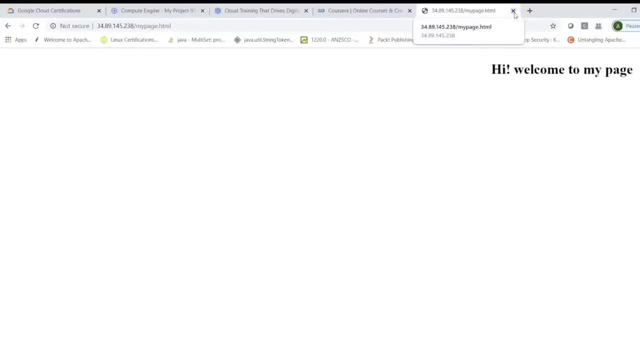 the data and then host your website on a Google cloud platform service, such as Google cloud platform service, such as Google cloud platform service, such as compute, where your actual code is compute, where your actual code is compute, where your actual code is running, so we can learn about your web. 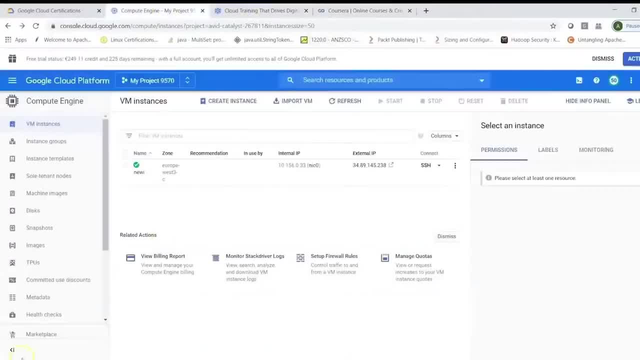 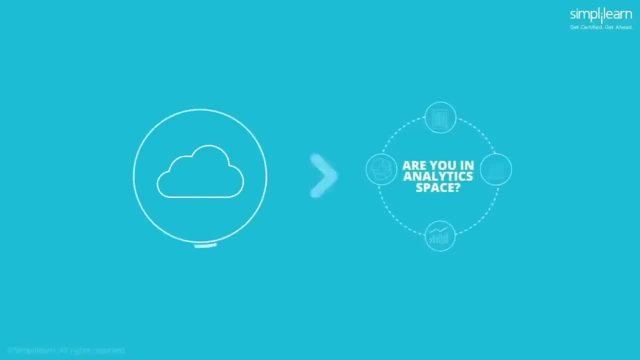 running so we can learn about your web running. so we can learn about your web hosting on compute instances in further hosting on compute instances in further hosting on compute instances in further sessions. are you in the analytics space sessions? are you in the analytics space sessions? are you in the analytics space? have you ever wondered how data 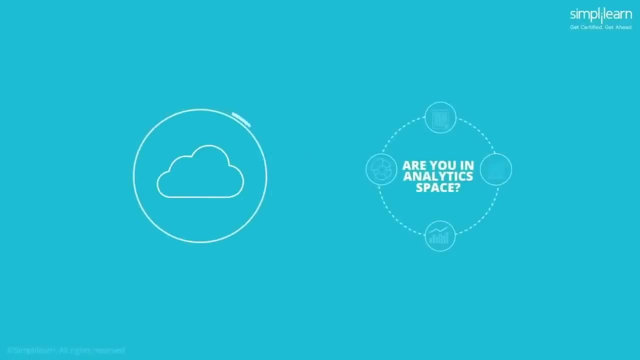 have you ever wondered how data, have you ever wondered how data processing in the cloud is changing? the processing in the cloud is changing. the processing in the cloud is changing the analytic space. if the answer is yes, this analytic space. if the answer is yes, this analytic space. if the answer is yes, this is the course for you all: major. 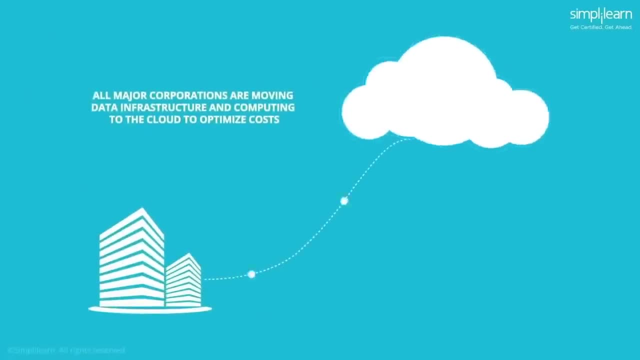 is the course for you all. major is the course for you all. major corporations are moving data. corporations are moving data. corporations are moving data infrastructure and computing to the cloud infrastructure and computing to the cloud infrastructure and computing to the cloud. to optimize costs to make analyzing. to optimize costs to make analyzing. 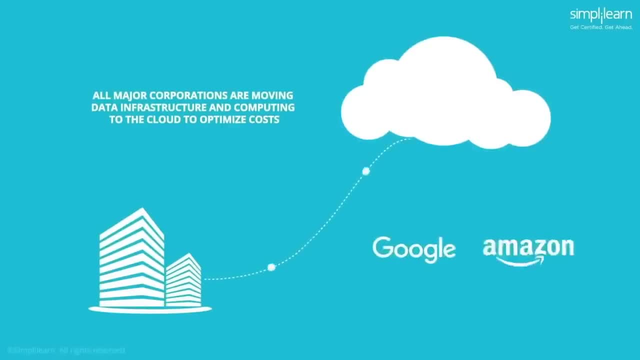 to optimize costs, to make analyzing data seamless technology. leaders like data seamless technology leaders like data seamless technology leaders like Google and Amazon are investing heavily. Google and Amazon are investing heavily. Google and Amazon are investing heavily in SAS tools on the cloud. Google is a in SAS tools on the cloud. Google is a. 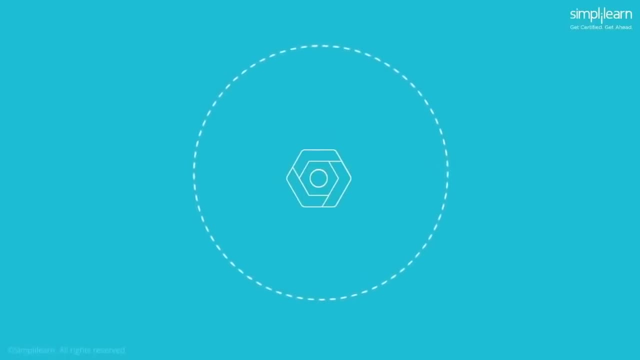 in SAS tools on the cloud. Google is a pioneer in this space. the Google big pioneer in this space. the Google big pioneer in this space. the Google big cloud data and machine learning platform. cloud data and machine learning platform. cloud data and machine learning platform provides cloud databases managed Hadoop. 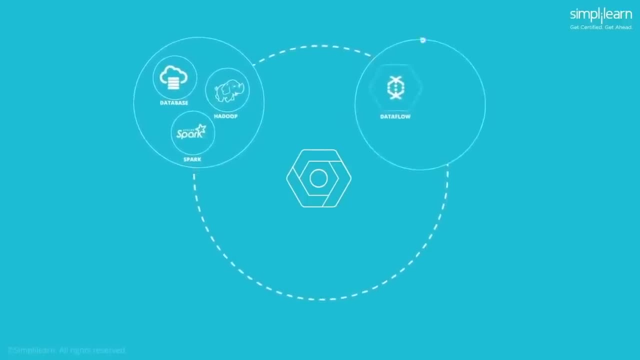 provides cloud databases managed. Hadoop. provides cloud databases managed. Hadoop and its spark services with tools like: and its spark services with tools like: and its spark services. with tools like data flow and data proc. the platform data flow and data proc. the platform data flow and data proc. the platform allows for highly scalable and reliable. 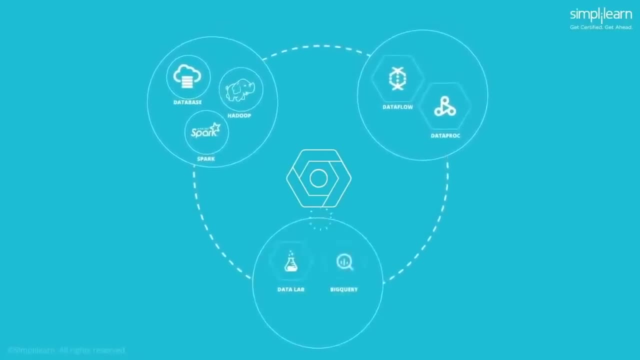 allows for highly scalable and reliable. allows for highly scalable and reliable data processing. the data lab, big query data processing. the data lab, big query data processing. the data lab big query and cloud machine learning features. make and cloud machine learning features. make and cloud machine learning features. make it a great choice for business. 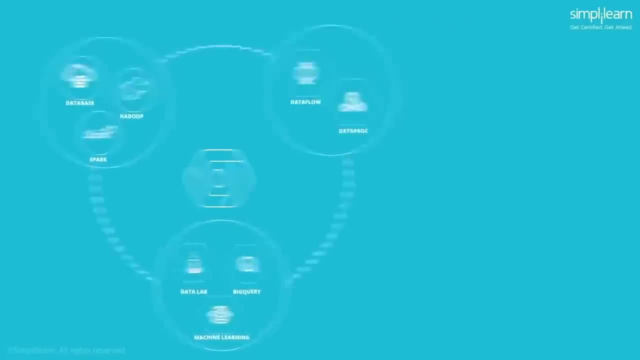 it a great choice for business. it a great choice for business. intelligence: large-scale analytics and intelligence- large-scale analytics and intelligence- large-scale analytics and machine learning. its best-in-class machine learning. its best-in-class machine learning, its best-in-class performance and low-cost makes Google. 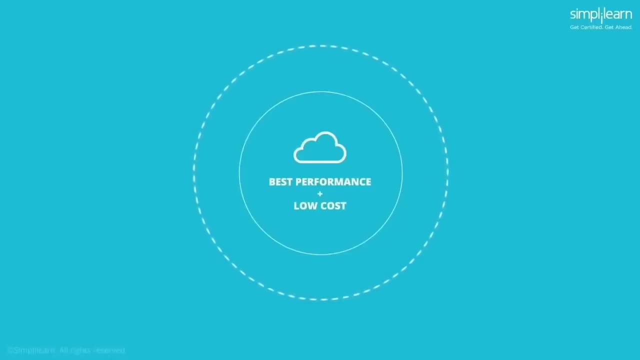 performance and low-cost makes Google performance and low-cost makes Google cloud popular and sought-after cloud popular and sought-after cloud popular and sought-after technology giants like Spotify and Apple technology giants like Spotify and Apple technology giants like Spotify and Apple have implemented the Google cloud, have implemented the Google cloud. 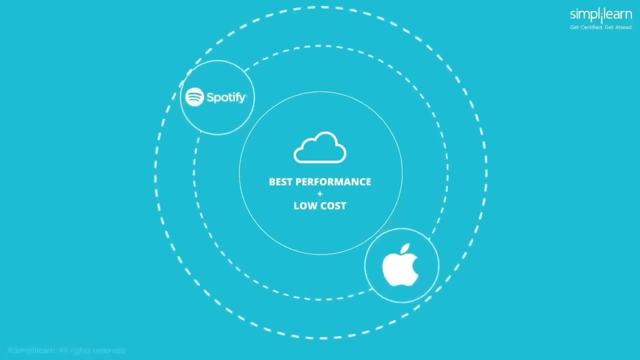 have implemented the Google cloud platform at their organizations and platform at their organizations and platform at their organizations. and healthcare and consumer goods leaders. healthcare and consumer goods leaders. healthcare and consumer goods leaders like Philips and coca-cola are like Philips and coca-cola are. 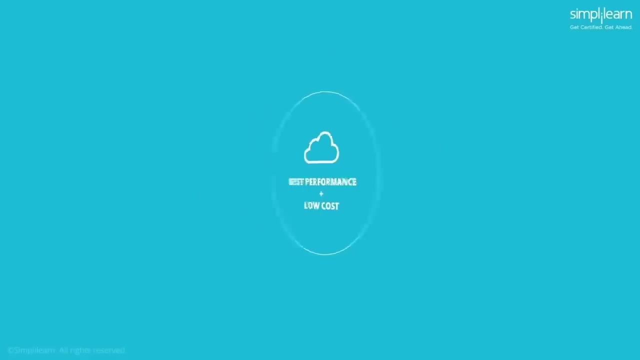 like Philips and coca-cola, are migrating to Google cloud for their data, migrating to Google cloud for their data. migrating to Google cloud for their data analytics. needs a Google data engineer analytics. needs a Google data engineer analytics. needs a Google data engineer with expertise in Google cloud machine. 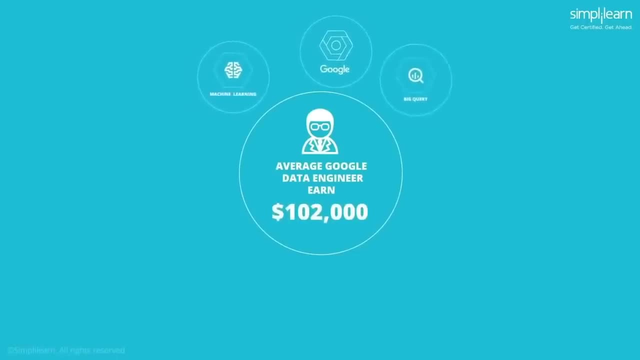 with expertise in Google cloud machine, with expertise in Google cloud machine learning and big query earns one hundred learning and big query earns one hundred learning and big query earns one hundred and two thousand dollars per year on and two thousand dollars per year on and two thousand dollars per year on average. and the demand for Google data. 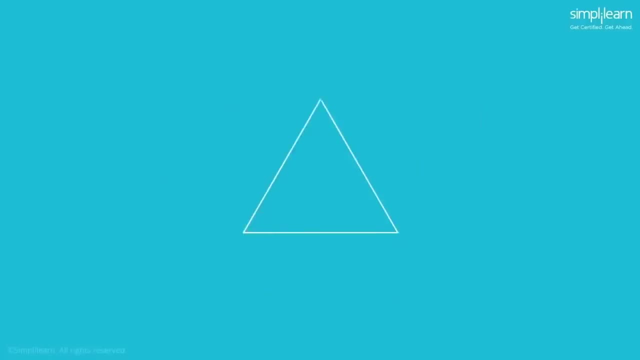 average and the demand for Google data average and the demand for Google data engineer certifications has never been engineer certifications has never been engineer certifications has never been higher. simply learns Google Cloud higher. simply learns Google Cloud higher. simply learns Google Cloud. platform. big data and machine learning platform. big data and machine learning. 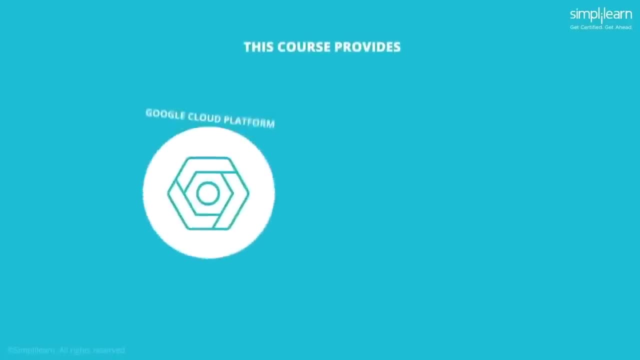 platform, big data and machine learning. fundamentals or cpb100 course. offers a fundamentals or cpb100 course. offers a fundamentals or cpb100 course. offers a thorough overview of the Google cloud. thorough overview of the Google cloud. thorough overview of the Google cloud platform, covering its data processing. 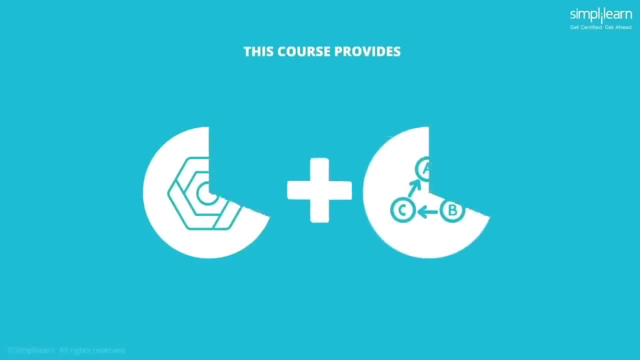 platform covering its data processing platform, covering its data processing capabilities with various use case capabilities, with various use case capabilities, with various use case studies. it's the perfect course for data studies. it's the perfect course for data studies. it's the perfect course for data analysts, business analysts and data. 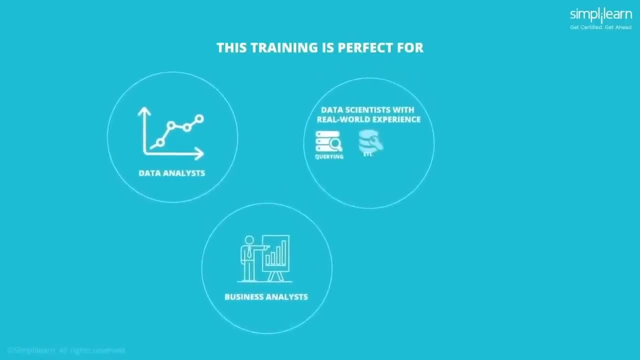 analysts, business analysts and data analysts. business analysts and data scientists with real-world experience in scientists with real-world experience in scientists with real-world experience in querying ETL data modeling or machine querying ETL data modeling or machine querying, ETL data modeling or machine learning. IT decision makers evaluating. 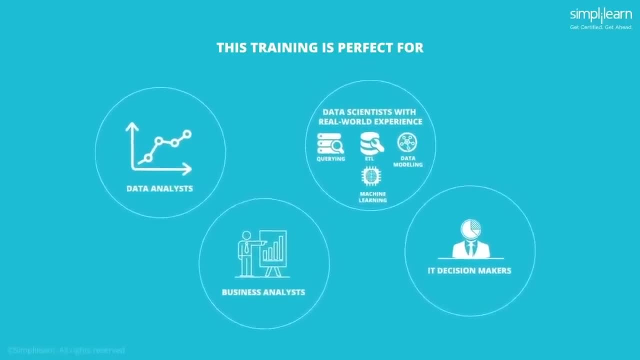 learning IT decision makers. evaluating learning IT decision makers. evaluating the Google cloud platform. have also the Google cloud platform. have also the Google cloud platform. have also found the training very useful. the found the training very useful. the found the training very useful. the course will cover everything you need to. 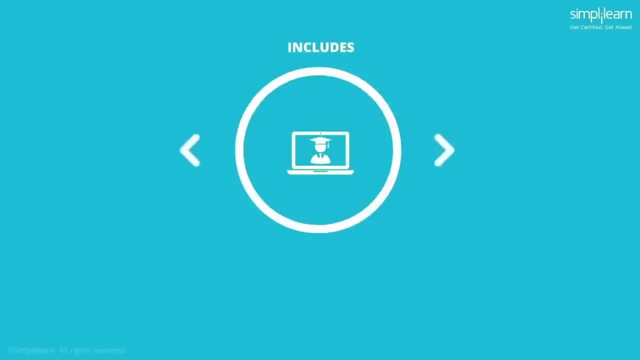 course will cover everything you need to course will cover everything you need to know about the Google cloud platform and know about the Google cloud platform and know about the Google cloud platform. and includes eight hours of instructor led. includes eight hours of instructor led. includes eight hours of instructor led training modules on big data and machine. 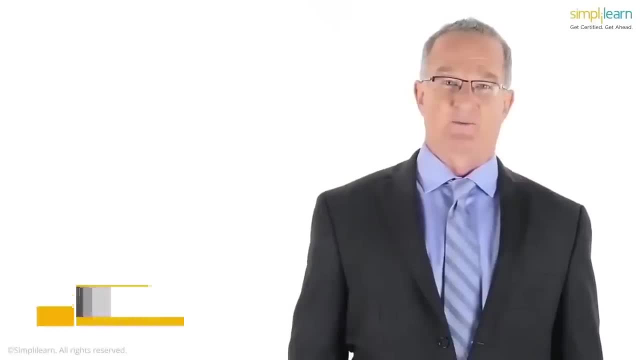 training modules on big data and machine training modules on big data and machine learning with the Google cloud. hi, my learning with the Google cloud. hi, my learning with the Google cloud. hi, my name is Randolph kale and I'm the name is Randolph kale and I'm the. 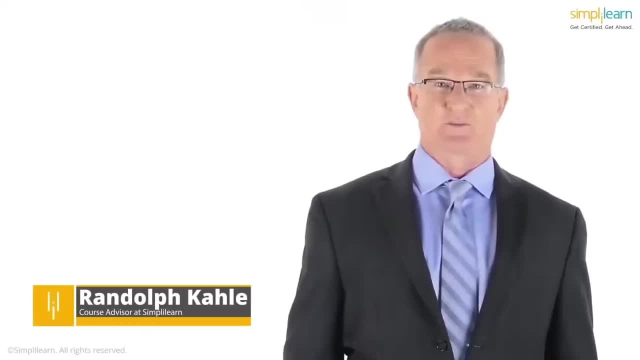 name is Randolph kale and I'm the co-author of the Google cloud platform. co-author of the Google cloud platform. co-author of the Google cloud platform and a course advisor at simply learn. I and a course advisor at simply learn. I and a course advisor at simply learn. I have over 40 years experience in the. 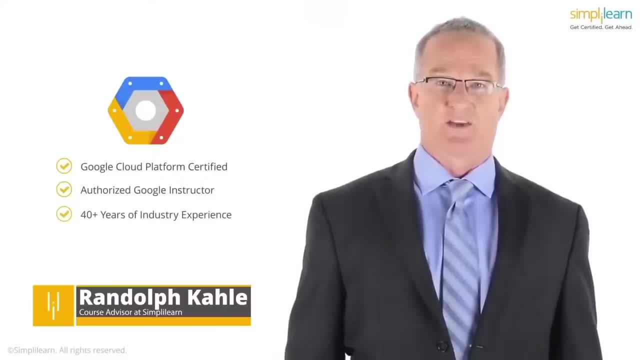 have over 40 years experience in the have over 40 years experience in the industry, spanning different roles from industry. spanning different roles from industry. spanning different roles from development managing cloud development, managing cloud development, managing cloud infrastructure to product management infrastructure, to product management infrastructure, to product management. I've partnered with. simply learn to. 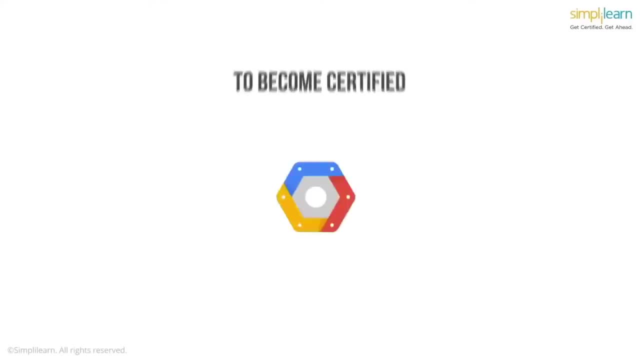 I've partnered with simply learn to. I've partnered with simply learn to ensure that you have the best. ensure that you have the best, ensure that you have the best opportunity to become certified in, opportunity to become certified in, opportunity to become certified in various Google cloud platform. 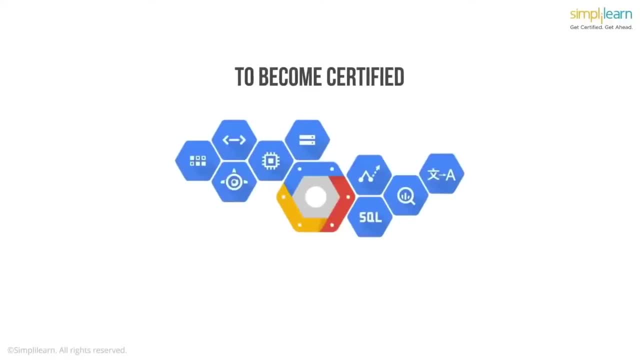 various Google cloud platform. various Google cloud platform technologies. gain hands-on experience on technologies. gain hands-on experience on technologies. gain hands-on experience on the cloud and make you job ready before the cloud. and make you job ready before the cloud. and make you job ready before we discuss the course and the reasons it. 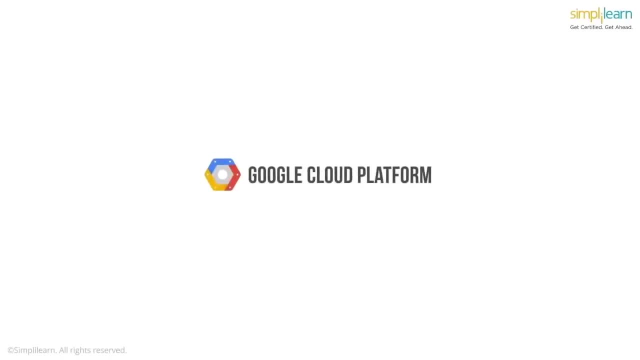 we discuss the course and the reasons it. we discuss the course and the reasons it will help you. let me first introduce you will help you. let me first introduce you will help you. let me first introduce you to Google cloud platform when you use, to Google cloud platform when you use. 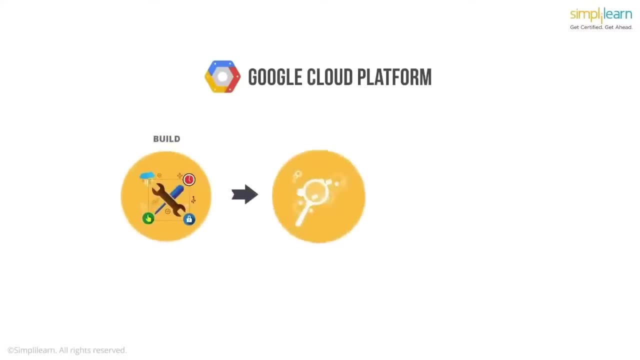 to Google cloud platform. when you use the Google cloud platform, you are the Google cloud platform. you are the Google cloud platform. you are empowered to build, test and deploy. empowered to build, test and deploy. empowered to build, test and deploy applications at Google scale. the move to applications at Google scale, the move to. 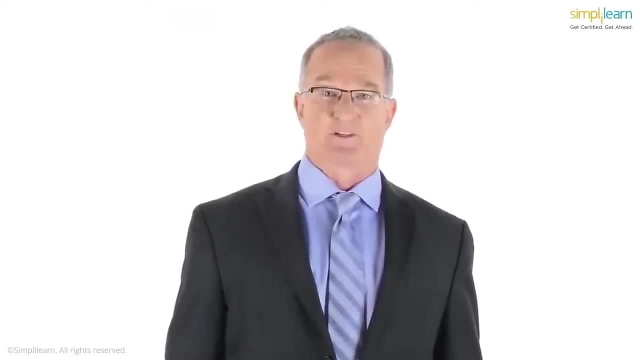 applications at Google scale. the move to the cloud is happening today. there is a? the cloud is happening today. there is a the cloud is happening today. there is a broad industry adoption. when I teach broad industry adoption, when I teach broad industry adoption, when I teach classes, I see the pace accelerating. 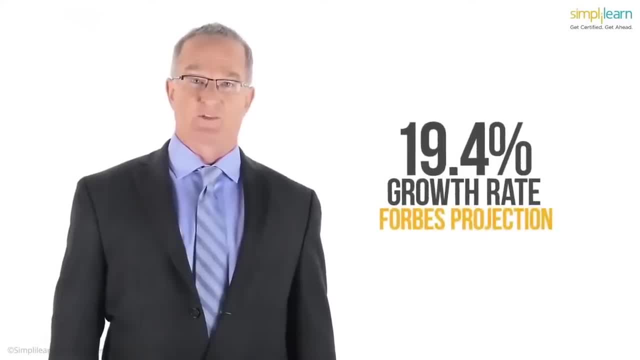 classes. I see the pace accelerating classes. I see the pace accelerating across all companies. Forbes projects: a across all companies. Forbes projects a across all companies. Forbes projects: a 19% growth rate to 140 billion US. 19% growth rate to 140 billion US. 19% growth rate to 140 billion US dollars. on cloud services by 2019. how? 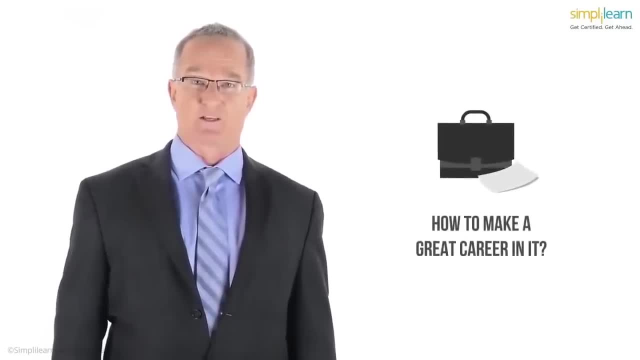 dollars on cloud services by 2019. how dollars on cloud services by 2019? how can you move to the cloud? how can you? can you move to the cloud? how can you? can you move to the cloud? how can you make a career in this fast-growing part? 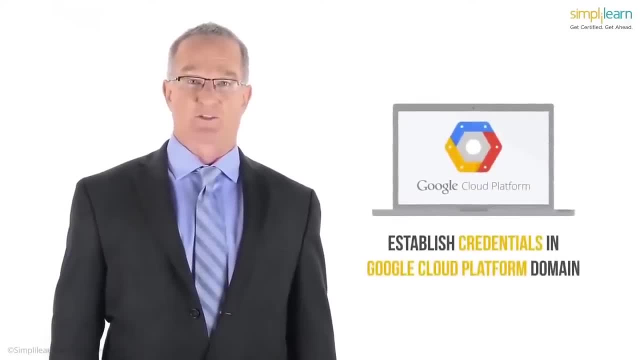 make a career in this fast-growing part. make a career in this fast-growing part of the industry. your first step is of the industry. your first step is of the industry. your first step is establishing your credentials in the, establishing your credentials in the, establishing your credentials in the Google Cloud Platform domain, and you can. 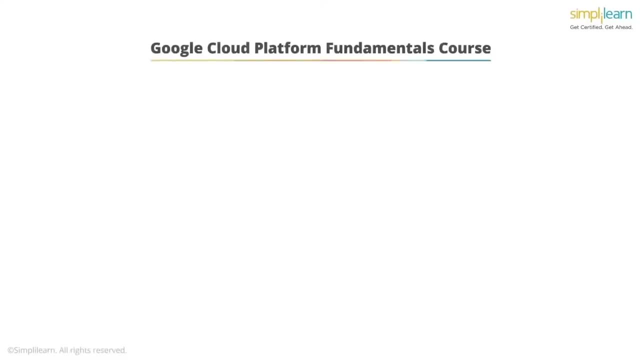 Google Cloud Platform domain and you can Google Cloud Platform domain and you can do that by getting certified the Google. do that by getting certified, the Google do that by getting certified. the Google Cloud Platform fundamentals course- Cloud Platform fundamentals course- Cloud Platform fundamentals course- introduces you to the Google Cloud. 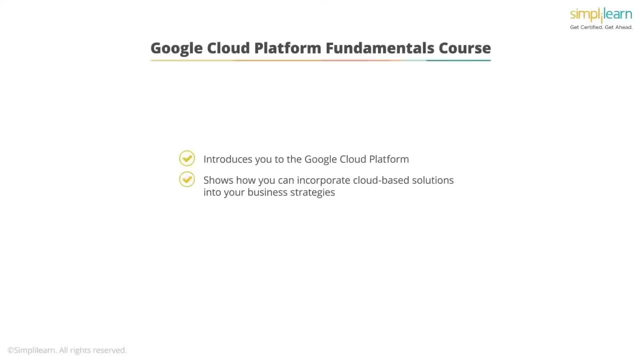 introduces you to the Google Cloud, introduces you to the Google Cloud Platform and shows you how you can Platform. and shows you how you can Platform and shows you how you can incorporate cloud-based solutions into incorporate cloud-based solutions, into incorporate cloud-based solutions into your business strategies. the course is: 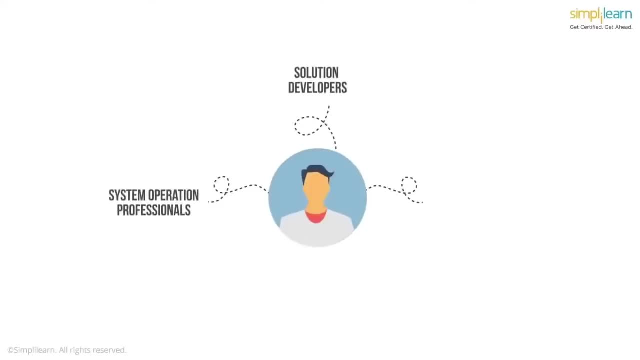 your business strategies. the course is your business strategies. the course is intended for solution developers. system intended for solution developers. system intended for solution developers. system operation professionals and solution operation professionals and solution operation professionals and solution architects planning to deploy architects. planning to deploy architects. planning to deploy applications and create application. 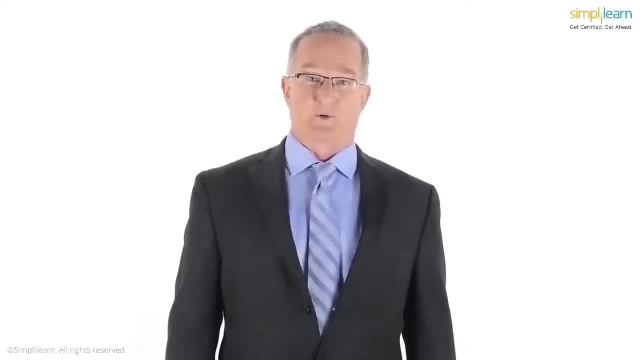 applications and create application environments on the Google Cloud environments. on the Google Cloud environments. on the Google Cloud Platform. it is also appropriate for Platform. it is also appropriate for Platform. it is also appropriate for executives and business decision makers. executives and business decision makers, executives and business decision makers: evaluating the potential of Google Cloud. 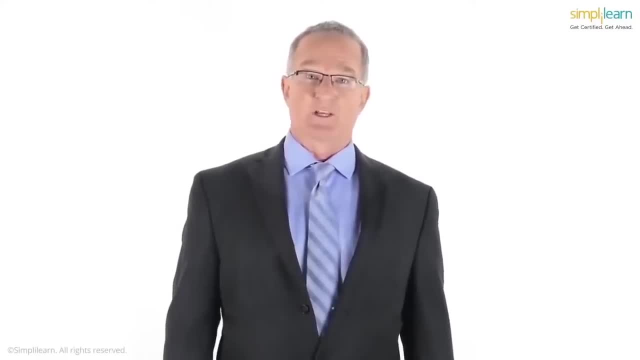 evaluating the potential of Google Cloud. evaluating the potential of Google Cloud Platform to address their business needs. Platform to address their business needs. Platform to address their business needs. completing this course will give you the completing this course will give you the completing this course will give you the skills and the confidence to take full. 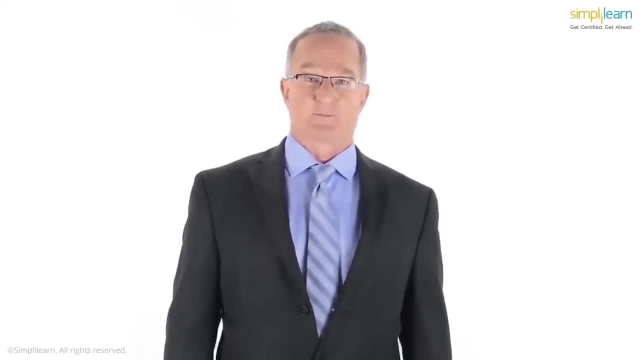 skills and the confidence to take full skills and the confidence to take full advantage of the Google Cloud Platform. advantage of the Google Cloud Platform. advantage of the Google Cloud Platform: ecosystem- simply learn. offers you ecosystem- simply learn. offers you ecosystem- simply learn. offers you extensive training to help you. 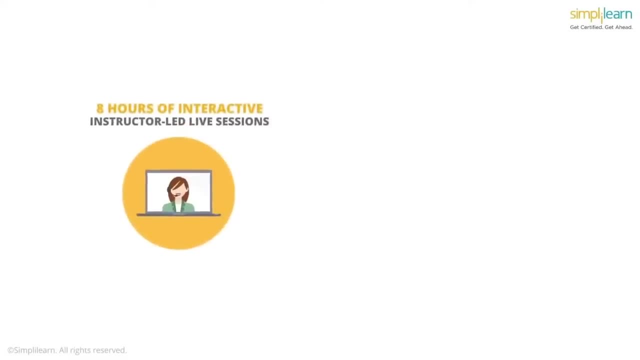 extensive training to help you. extensive training to help you understand the platform. you get eight. understand the platform, you get eight. understand the platform. you get eight hours of interactive instructor led live hours of interactive instructor led live hours of interactive instructor led live online sessions, along with the course. 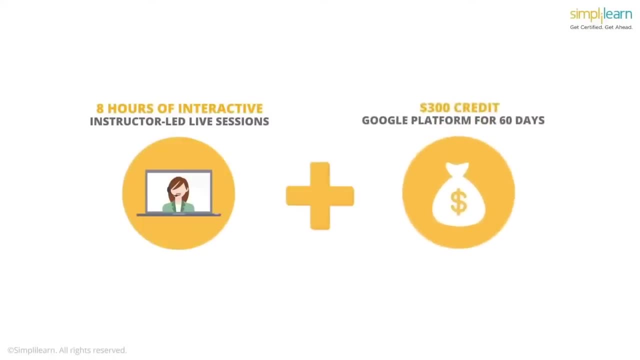 online sessions along with the course. online sessions along with the course. you receive a free trial account. with you receive a free trial account. with you receive a free trial account with $300 credit toward the use of Google, $300 credit toward the use of Google. $300 credit toward the use of Google Cloud Platform for 60 days. the 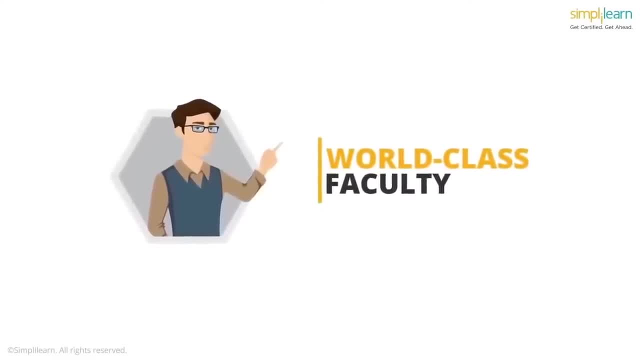 Cloud Platform for 60 days. the Cloud Platform for 60 days. the instructors are Google authorized trainers. instructors are Google authorized trainers. instructors are Google authorized trainers. the content is engaging and all the content is engaging. and all the content is engaging and all the topics are very well explained with 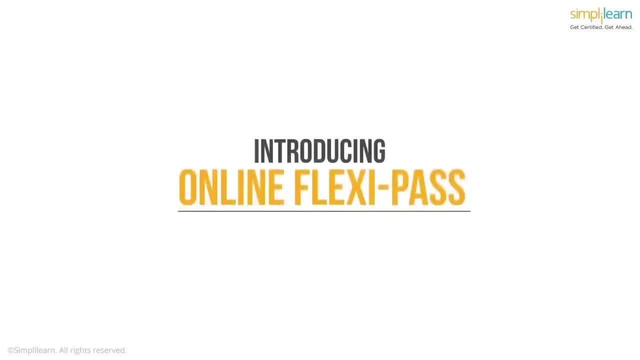 the topics are very well explained with. the topics are very well explained with simply learn. you'll be enrolling for the simply learn. you'll be enrolling for the simply learn. you'll be enrolling for the online classroom flexi pass, which gives online classroom flexi pass, which gives 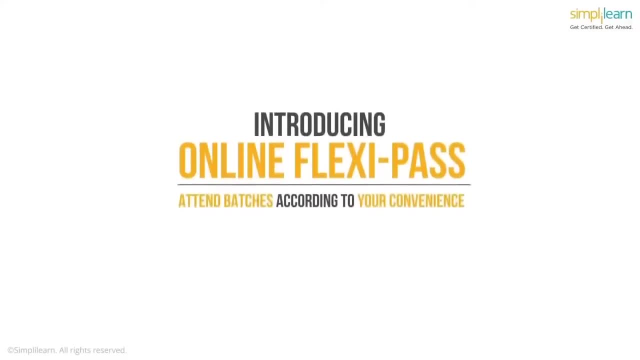 online classroom flexi pass, which gives you the flexibility to attend any of the you. the flexibility to attend any of the you. the flexibility to attend any of the weekday and weekend batches according to weekday and weekend batches: according to weekday and weekend batches, according to your convenience. another thing that's 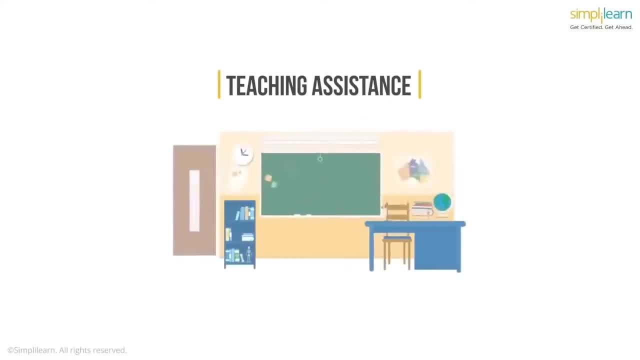 your convenience. another thing that's your convenience. another thing that's impressive is the proactive teaching. impressive is the proactive teaching. impressive is the proactive teaching assistance: where experts resolve all assistance, where experts resolve all assistance, where experts resolve all your course related, project related, or your course related, project related, or 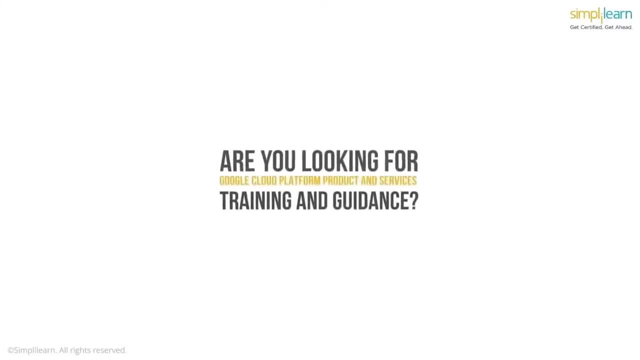 your course related, project related or technical questions while pursuing a technical questions, while pursuing a technical questions while pursuing a course. so, if you're looking for the course, so if you're looking for the course, so if you're looking for the training and guidance, you need to have a 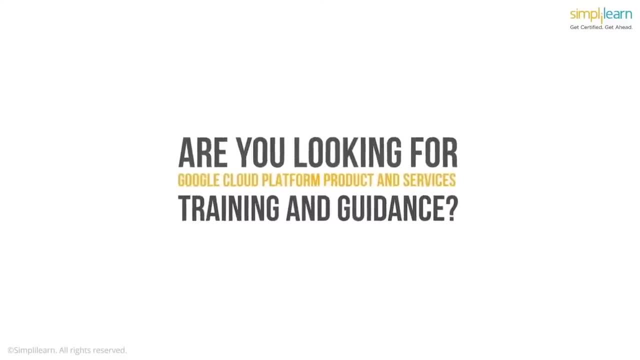 training and guidance. you need to have a training and guidance. you need to have a deeper understanding about Google Cloud. deeper understanding about Google Cloud, deeper understanding about Google Cloud platform products and services. this is platform products and services. this is platform products and services. this is the best course for you for the course. 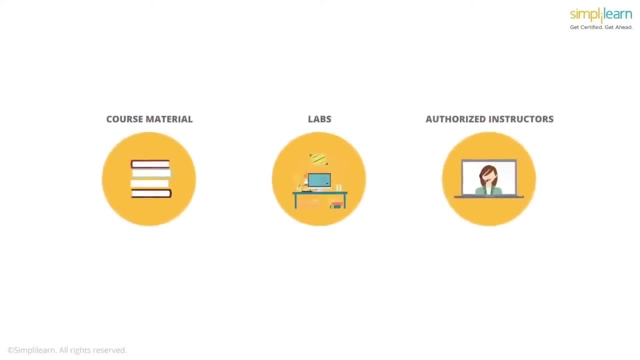 the best course for you for the course. the best course for you for the course? material labs and authorized instructors. material labs and authorized instructors. material labs and authorized instructors with extensive experience. I don't think. with extensive experience, I don't think with extensive experience, I don't think you'll need to go anywhere else. take. 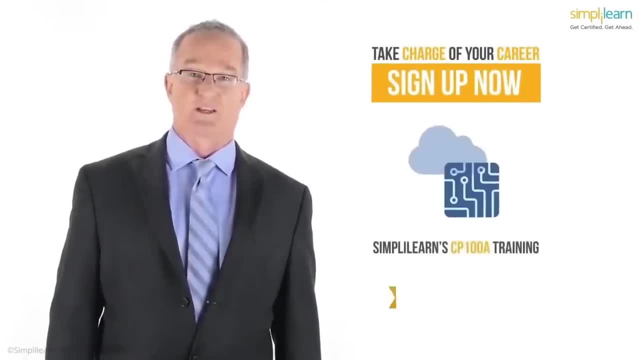 you'll need to go anywhere else. take you'll need to go anywhere else. take charge of your career. sign up for charge of your career. sign up for charge of your career. sign up for: simply learn CP 108 training, all the. simply learn CP 108 training, all the. 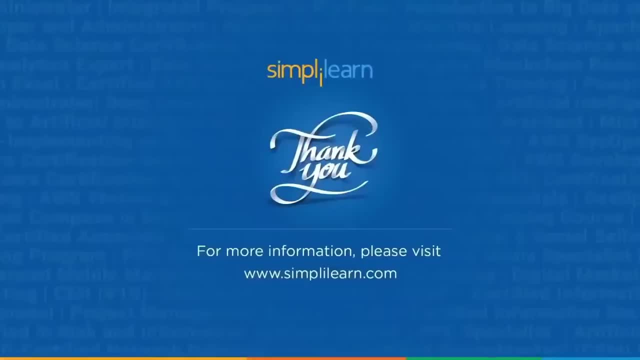 simply learn CP 108 training. all the best to you, and with that we have come best to you, and with that, we have come best to you. and with that we have come to the end of this video on Google Cloud, to the end of this video on Google Cloud. 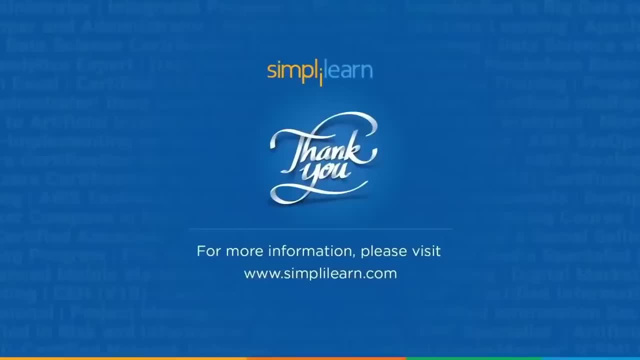 to the end of this video on Google Cloud platform. for course, I hope you found it platform. for course, I hope you found it platform. for course, I hope you found it informative and interesting. if you have informative and interesting. if you have informative and interesting. if you have any questions about the topics covered. 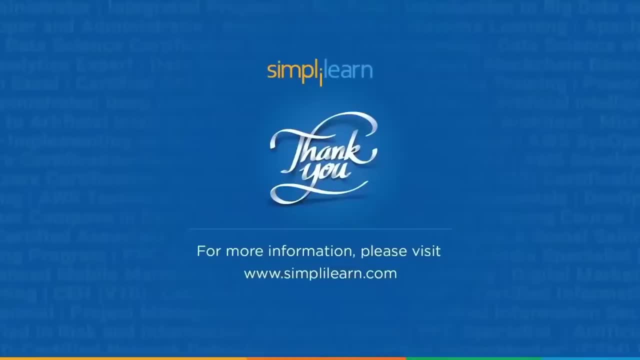 any questions about the topics covered. any questions about the topics covered in this video, please ask away in the in this video. please ask away in the in this video. please ask away in the comment section below. a team will help. comment section below: a team will help. comment section below: a team will help you solve your queries. thank you for. 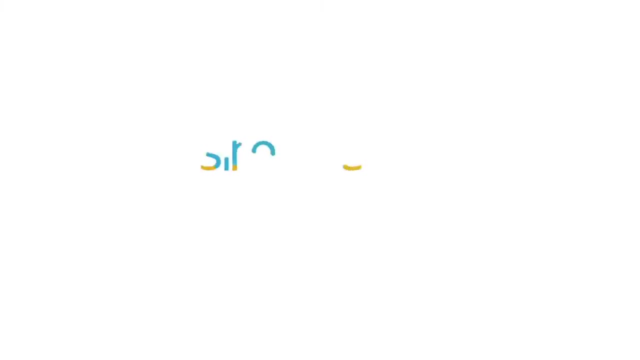 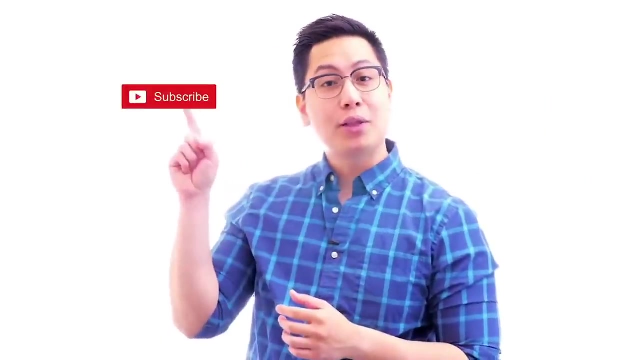 you solve your queries. thank you for you solve your queries. thank you for watching. stay safe and keep learning hi watching. stay safe and keep learning hi watching. stay safe and keep learning hi there. if you like this video, subscribe there. if you like this video, subscribe there. if you like this video, subscribe to the simply learn YouTube channel and. 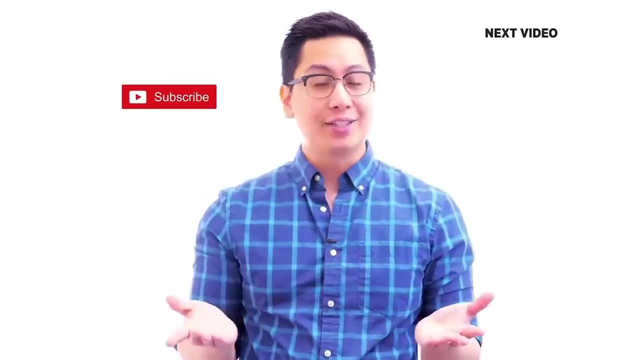 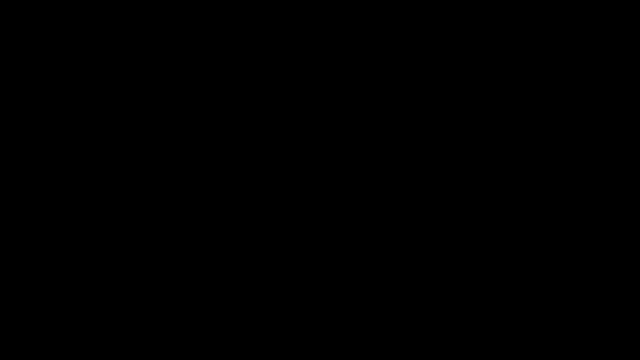 to the simply learn YouTube channel and to the simply learn YouTube channel and click here to watch similar videos. to click here to watch similar videos. to click here to watch similar videos. to nerd up and get certified: click here. click here to watch similar videos. to nerd up and get certified: click here.